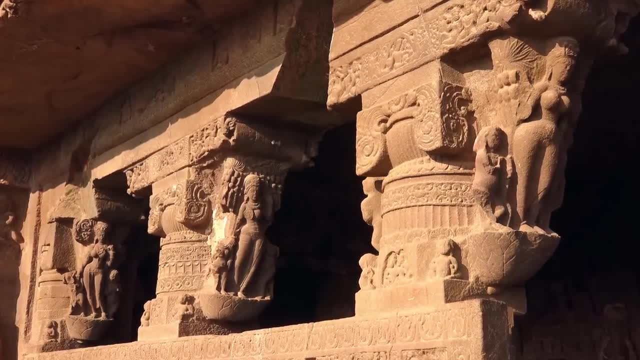 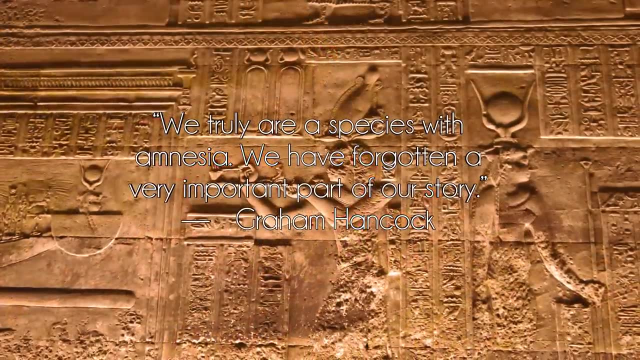 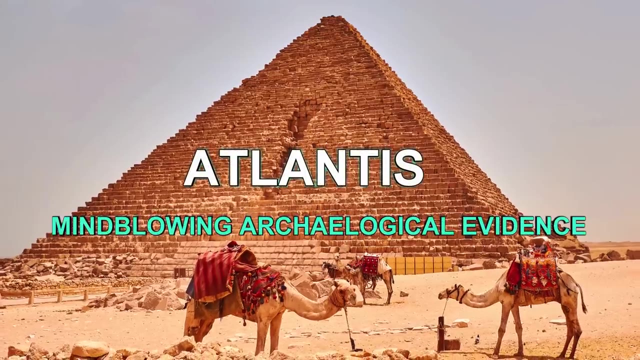 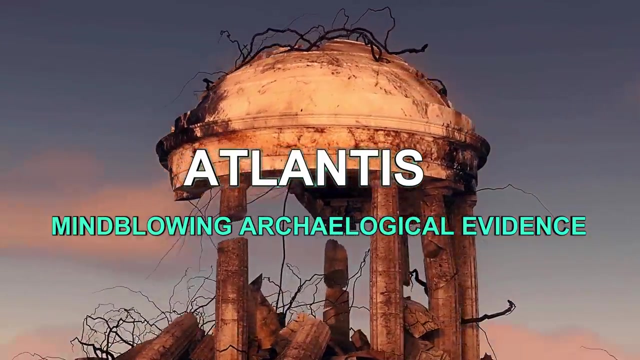 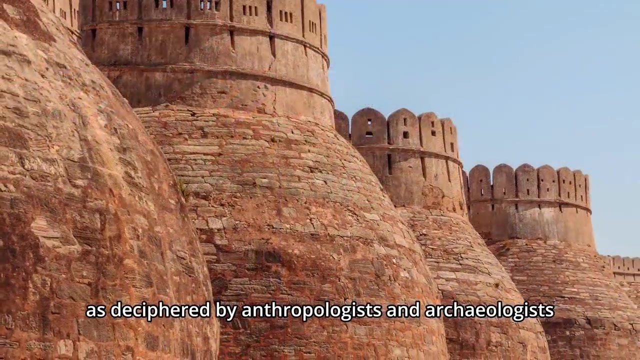 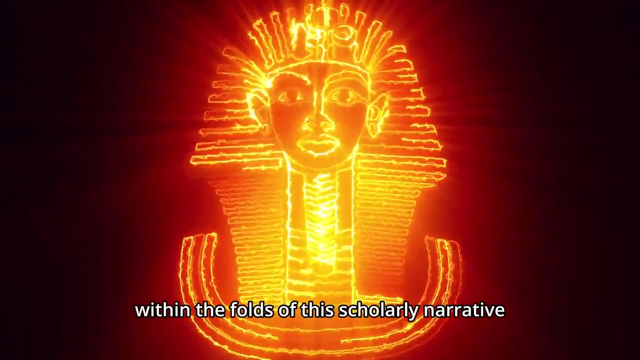 The epic tale of our human history and evolution, as deciphered by anthropologists and archaeologists, has been embraced by the scientific community as a remarkable saga. Nonetheless, within the folds of this scholarly narrative, a curious constellation of gaps and anomalies beckons the curious minds among us. 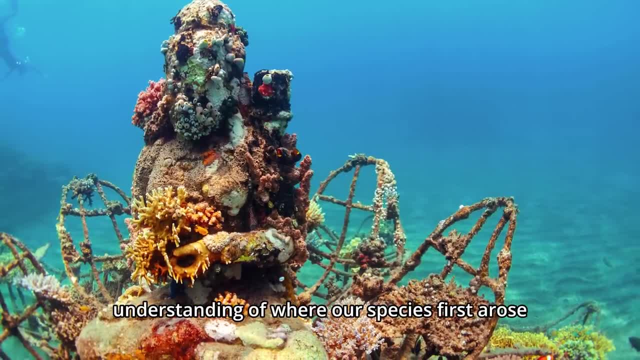 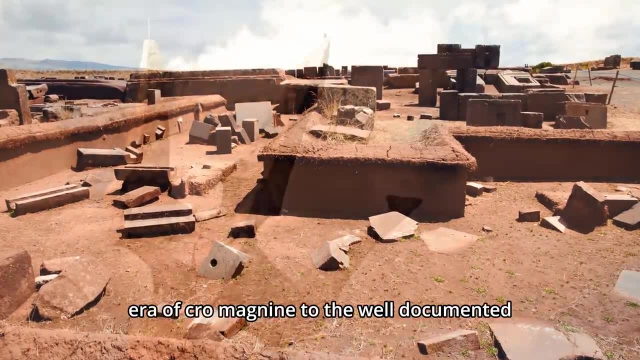 casting intriguing shadows upon the conventional understanding of where our species first arose and how it ventured to every corner of the globe: The expanse of time bridging the era of Cro-Magnon to the well-documented emergence of Middle and Far Eastern civilizations some ten millennia ago. 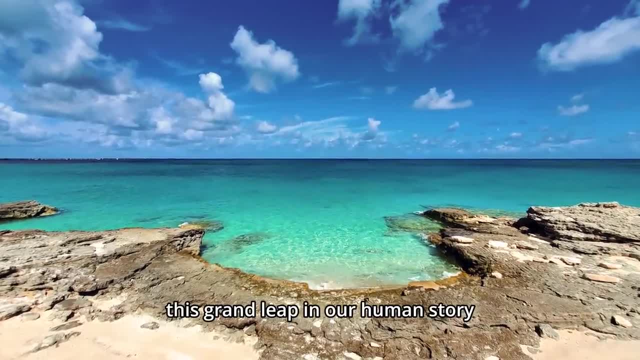 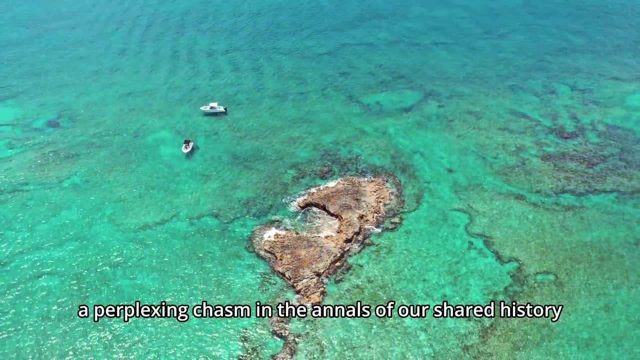 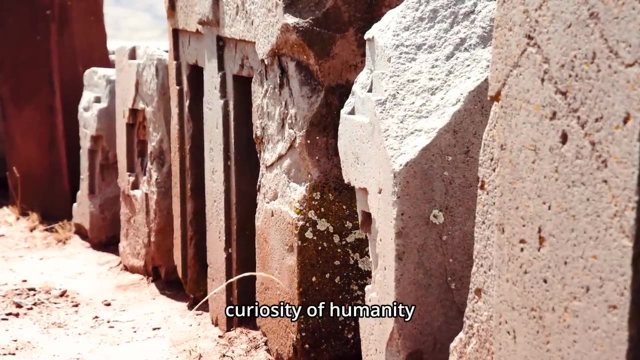 beckons us with its cloak of obscurity. This grand leap in our human story, spanning thousands of years, stands as a tantalizing void, a perplexing chasm in the annals of our shared history, a chapter lost in the mists of time, waiting to be unveiled by the relentless curiosity of humanity. 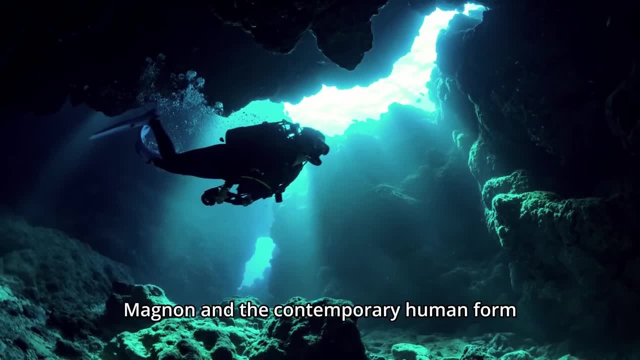 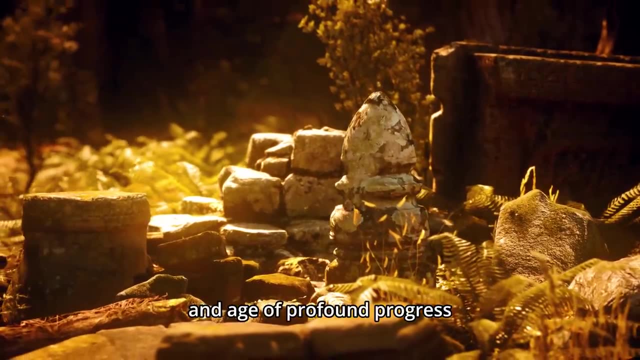 In the twilight realm between the indistinguishable Cro-Magnon and the contemporary human form. one might anticipate that these elusive millennia would echo with the resonance of transformation, an age of profound progress both in the realms of technology and intellect, paving the way for a heightened comprehension of the world. 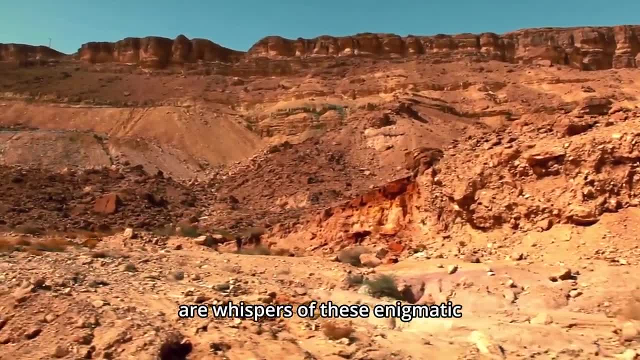 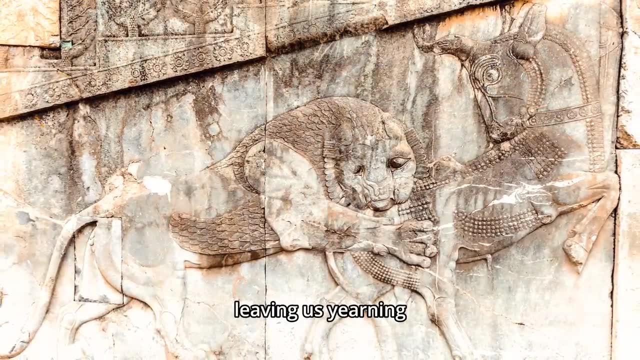 Regrettably, what we grasp instead are whispers of these enigmatic missing links within the intricate tapestry of civilization, cloaked in legend and shrouded in mystery, leaving us yearning for insights into these transitional epochs of our shared journey. 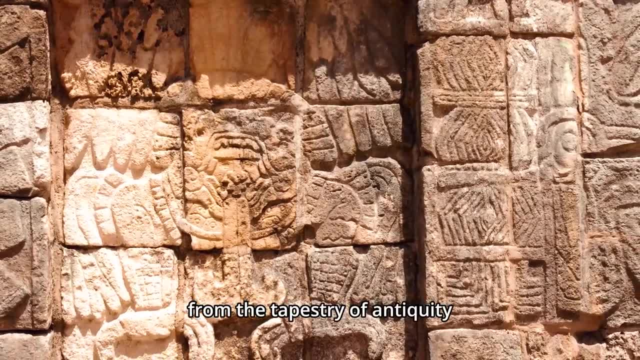 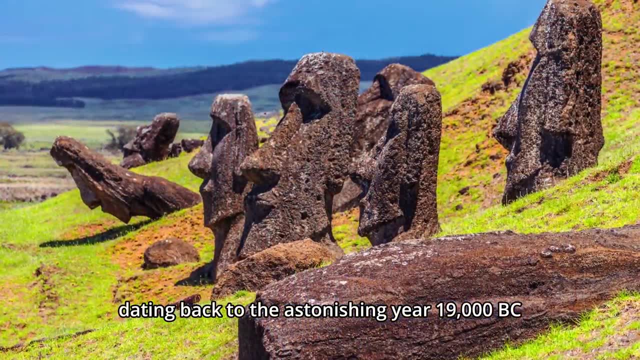 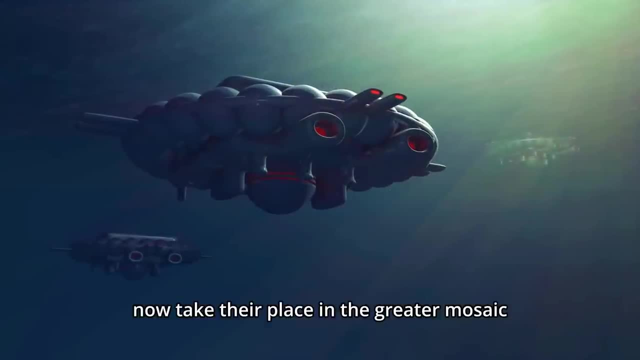 A singular exception rises from the tapestry of antiquity: a string of recent revelations unveiling the presence of hunting tribes in North America dating back to the astonishing year 19,000 BC. These tribes, like fragments of a larger enigma, now take their place in the greater mosaic. 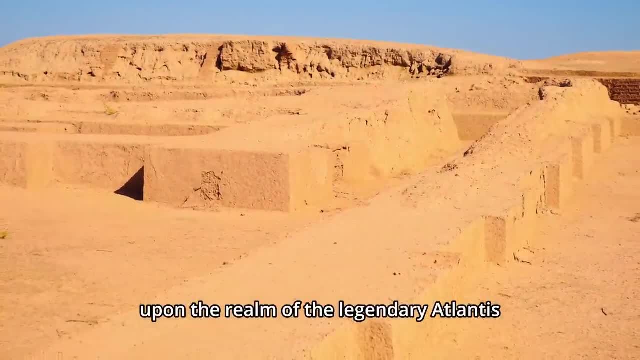 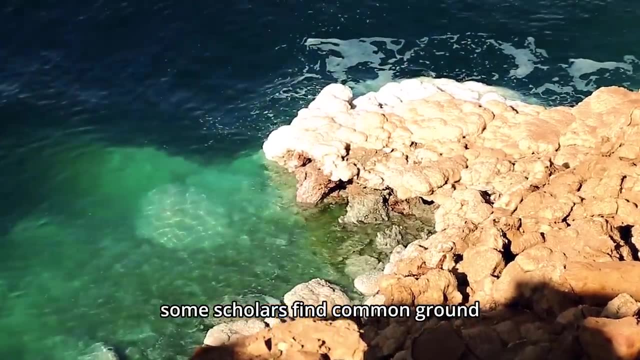 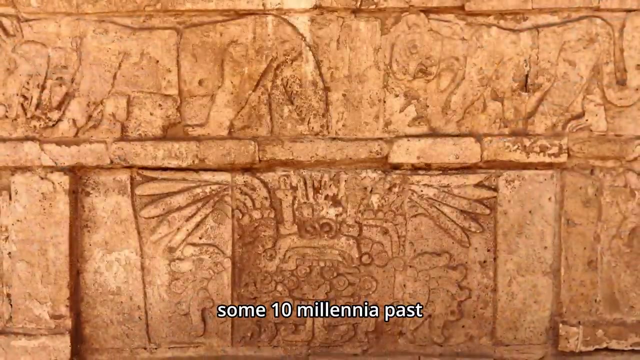 casting their intriguing shadows upon the realm of the legendary Atlantis, a fabled continent In the labyrinthine depths of geological contemplation. some scholars find common ground suggesting that Atlantis, a realm of myth and intrigue, may indeed have met its watery demise some ten millennia past. 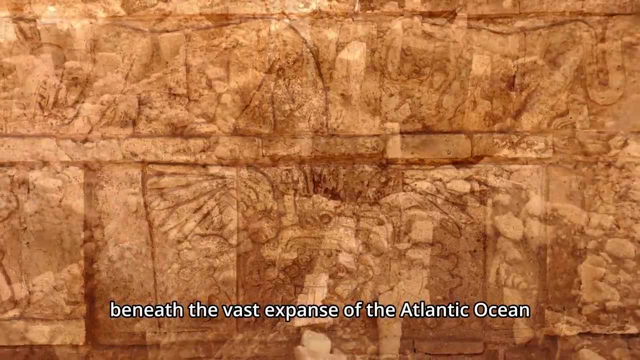 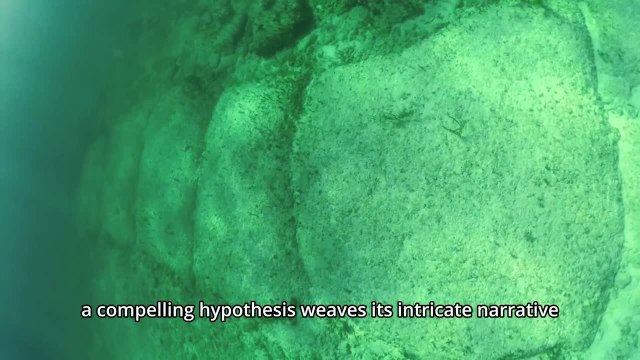 resting in eternal slumber beneath the vast expanse of the Atlantic Ocean. Among the annals of esteemed historians and anthropologists, a compelling hypothesis weaves its intricate narrative: a belief in the existence of a vast island continent that nurtured a profoundly advanced civilization. 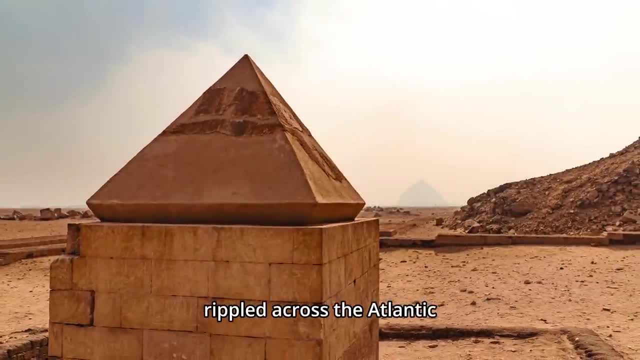 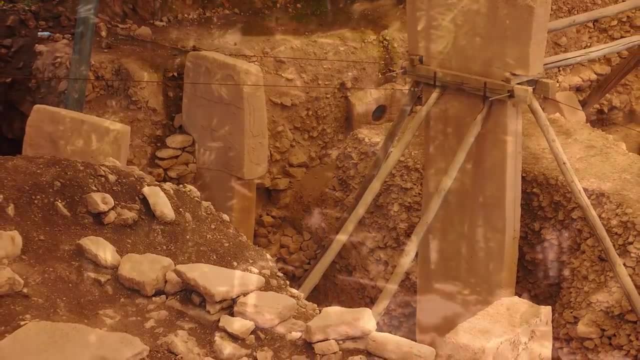 It is proposed that this culture's influence rippled across the Atlantic, leaving indelible imprints on the later great societies that blossomed on both sides of this expansive ocean. The captivating parallels between the realms of science, art and religion. 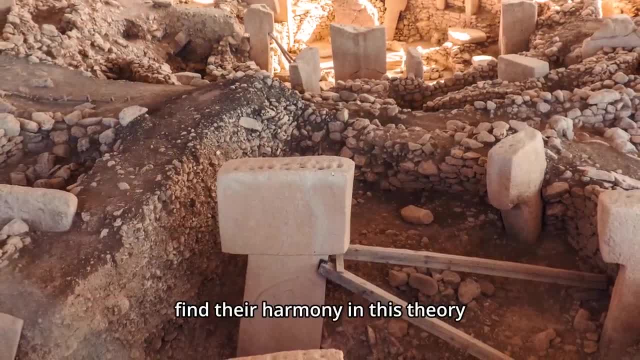 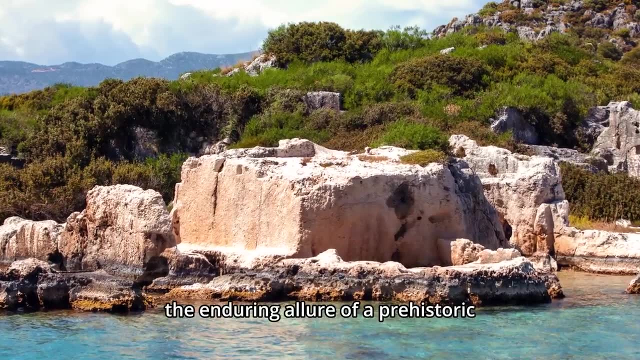 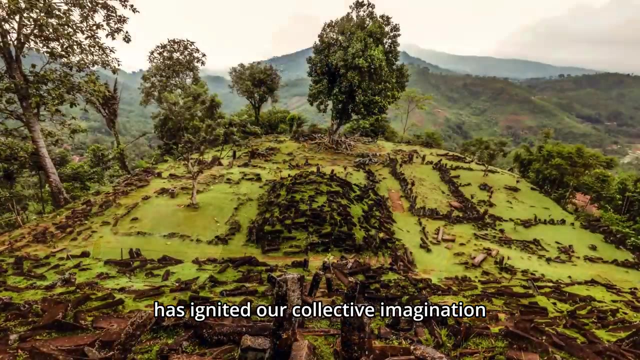 shared by Native American and Middle Eastern cultures find their harmony in this theory, fortified by the compelling foundations of rigorous archaeological inquiry. The enduring allure of a prehistoric Atlantic-bound continent vanquished by a cataclysmic event has ignited our collective imagination. 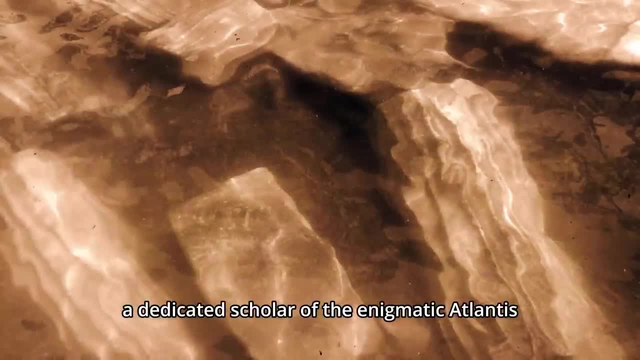 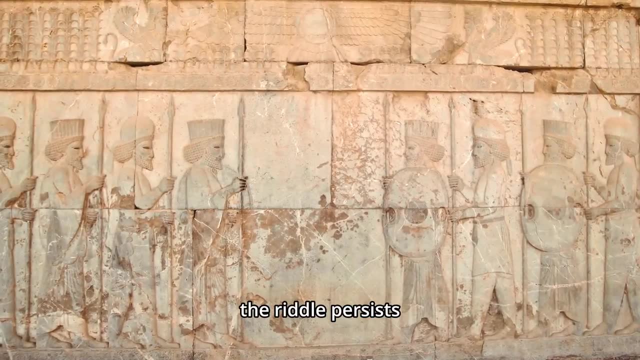 German scientist Otto Muck, a dedicated scholar of the enigmatic Atlantis, observes that though thousands of tomes have sought to unfurl the enigma's shroud, the riddle persists evergreen and unyielding Few themes outside the realm of religious narratives. 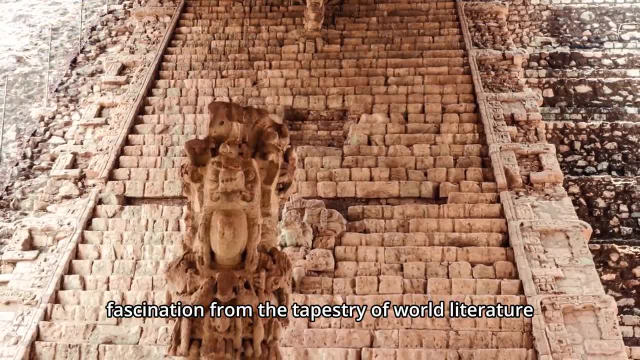 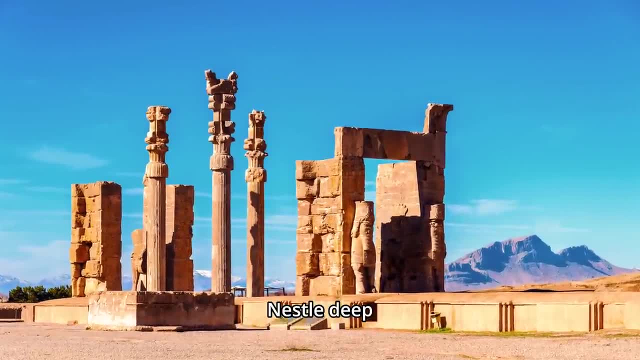 have drawn forth such ceaseless fascination from the tapestry of world literature, imprinting themselves indelibly upon the annals of human curiosity and storytelling, Nestled deep within the ancient pages of two of Plato's dialogues, Timaeus and Criscus. 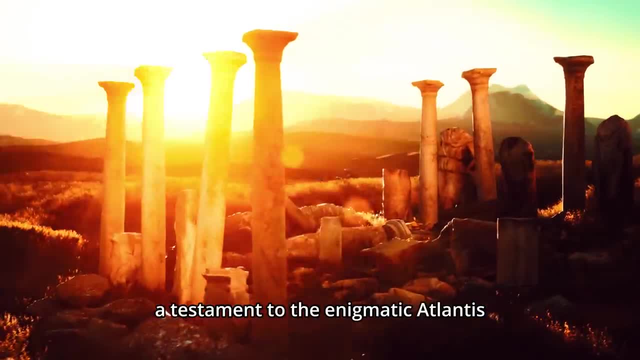 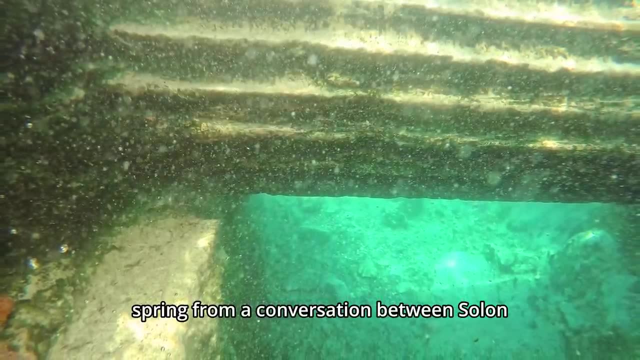 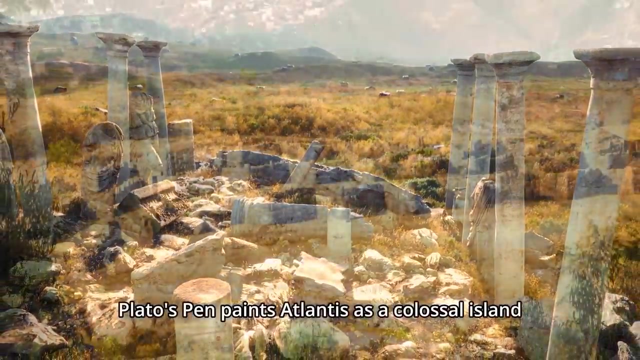 a time-worn treasure of knowledge unveils itself a testament to the enigmatic Atlantis. The origins of this enigmatic land spring from a conversation between Solon and an Egyptian priest, a dialogue that bridges antiquity and curiosity. Plato's pen paints Atlantis as a colossal island. 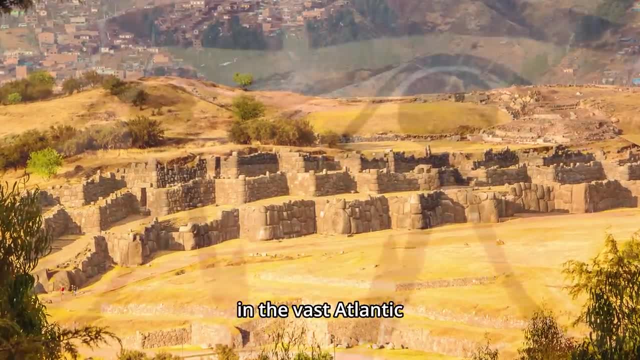 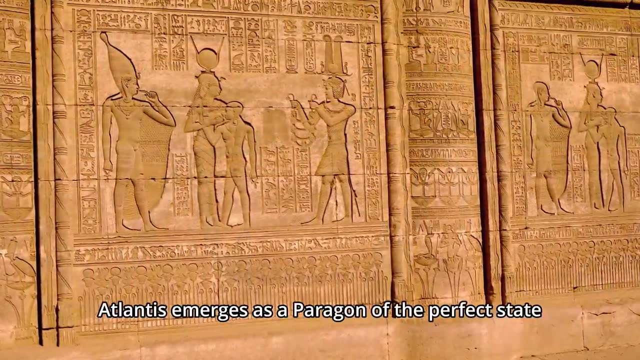 its resting place to the west of Gibraltar in the vast Atlantic, concealed beneath the waves, for a staggering 9,000 years. Within Plato's words, Atlantis emerges in the vast Atlantic. within Plato's words, Atlantis emerges in the vast Atlantic as a paragon of the perfect state. 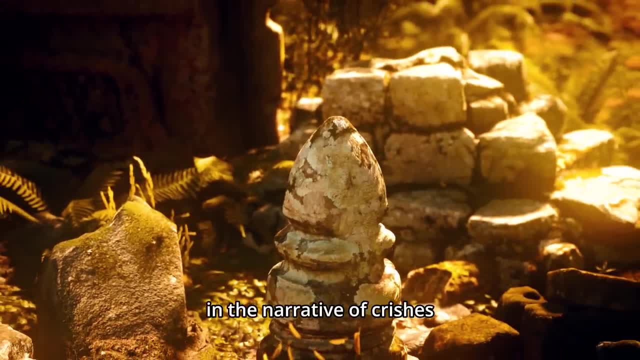 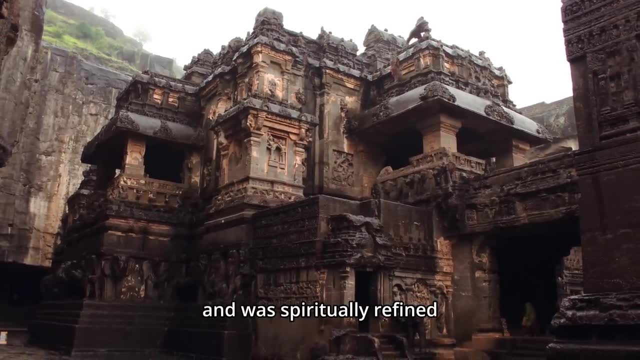 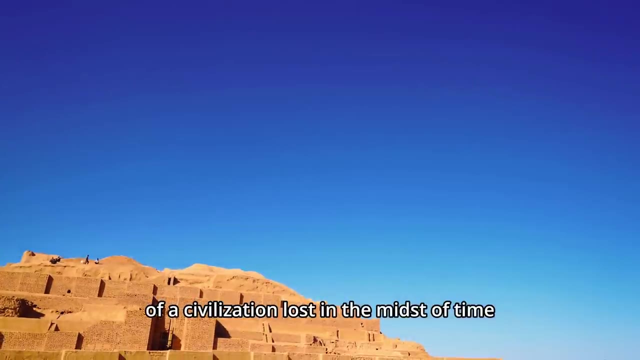 a dream woven into the fabric of history. In the narrative of Criscus, the Atlantean populace gleams with prosperity, wielded power and was spiritually refined, hinting at the possibility of their mastery over advanced technologies. an age-old echo of a civilization lost in the mists of time. Across the tapestry of generations. as long as the celestial spark of their essence endured, they remained bound to the sacred tenets, embracing the divine connection that coursed through their being. Within the depths of their souls, they preserved a majestic spirit. 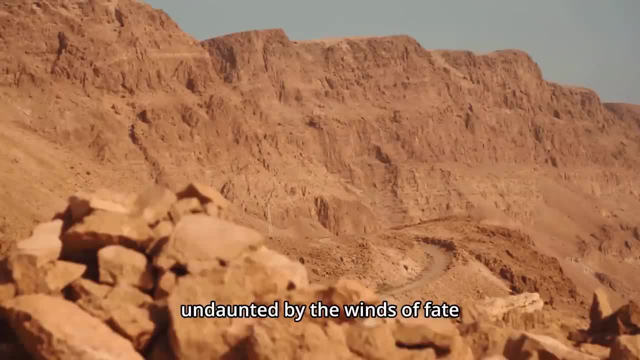 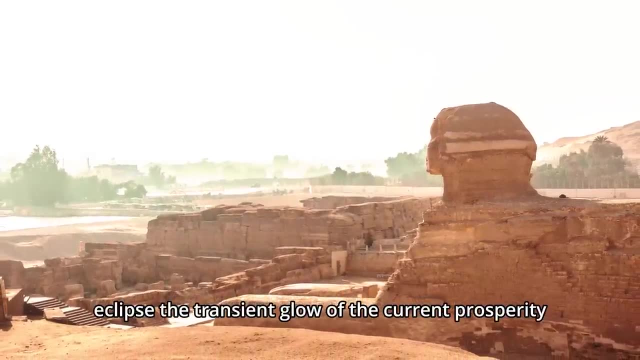 a beacon of wisdom and patience, undaunted by the whims of fate and their interactions with fellow beings. In their estimation, the enduring qualities of character eclipsed the transient glow of their current prosperity. They shouldered the weight of their riches and worldly possessions with grace. 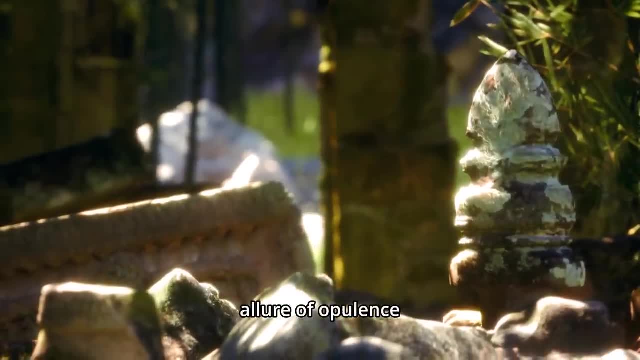 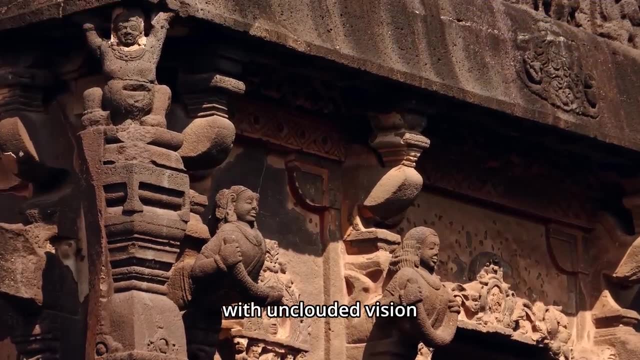 their hearts unburdened by the intoxicating allure of opulence. Their elevated standard of living never clouded their judgment or led them astray, for they perceived, with unclouded vision, that all these treasures thrived only in the fertile ground of communal benevolence and individual integrity. 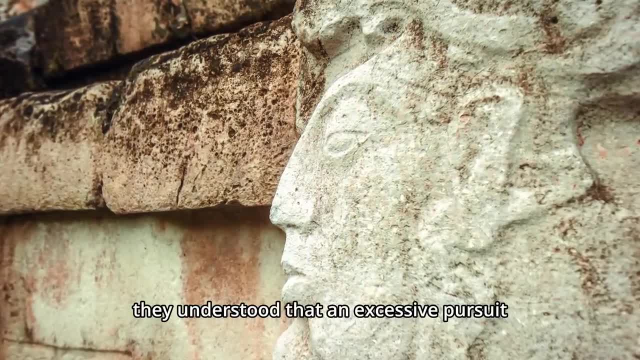 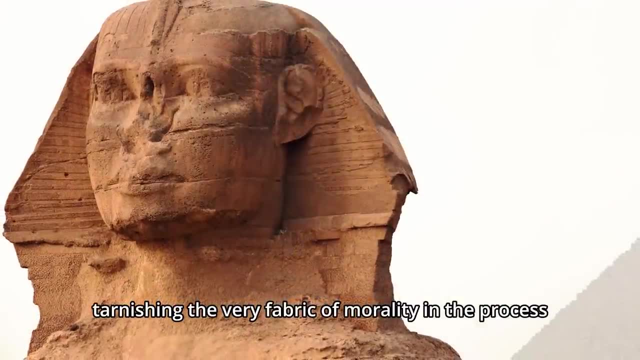 With sober contemplation, they understood that an excessive pursuit and overestimation of such material wealth could in fact be the harbinger of their own undoing, tarnishing the very fabric of morality in the process, While these guiding principles and their celestial essence stood unwavering. 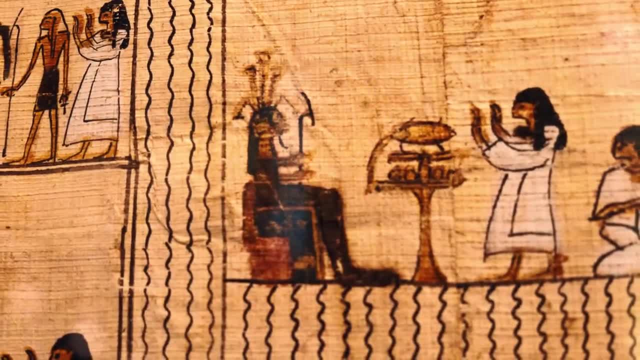 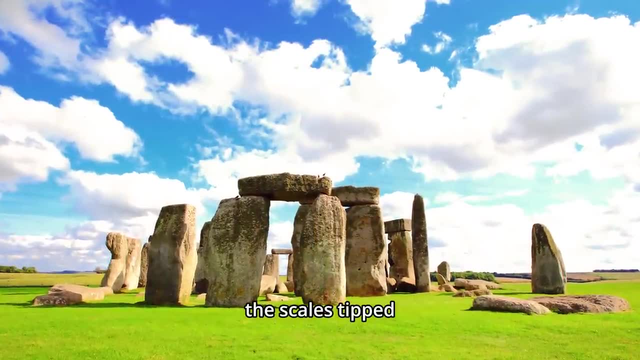 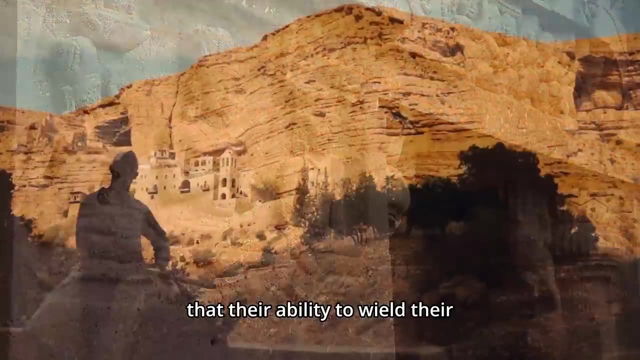 the described prosperity flourished relentlessly. However, as the divine spark within them dimmed, diluted by frequent mingling with mortal traits, the scales tipped and the human aspect of their nature began to assert dominance. It was at this pivotal juncture that their ability to wield their prosperity with measured grace began to erode. 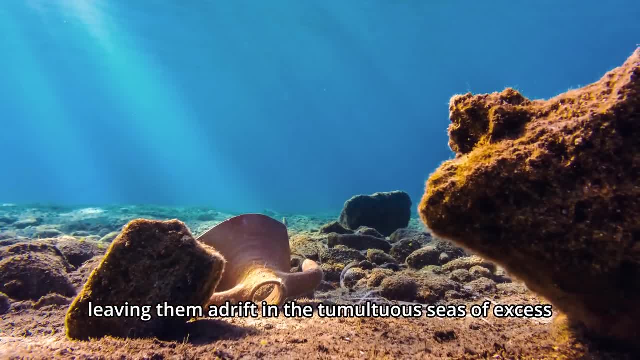 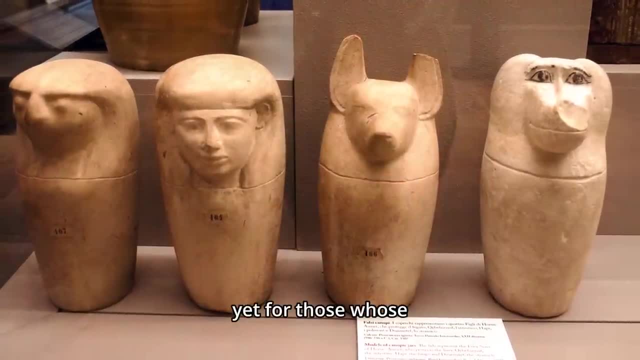 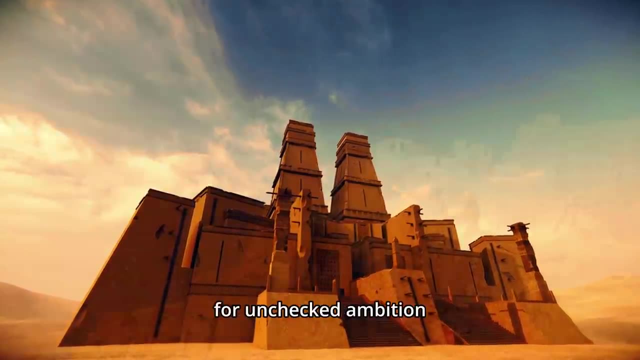 leaving them adrift in the tumultuous seas of excess. For those with discerning insight, the profound depths of their decline were starkly apparent. Yet for those whose understanding of genuine happiness was obscured, the Atlanteans driven by their insatiable thirst for unchecked ambition and boundless power. 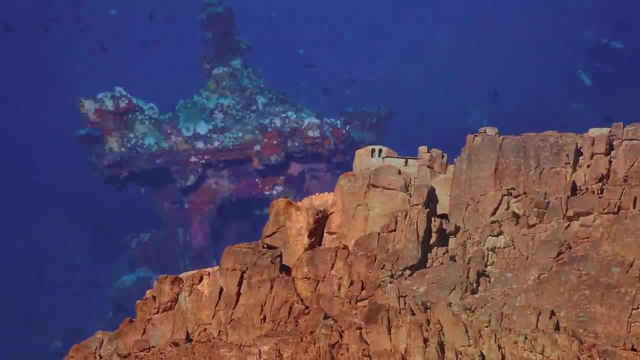 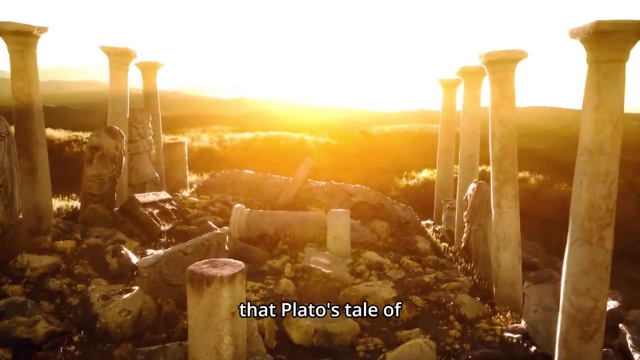 appeared to soar to the pinnacle of renown and affluence. Archaeological whispers shrouded in the sands of time tantalizingly hinted a possibility that Plato's tale of Atlantis might, against all odds, carry a grain of historical truth. 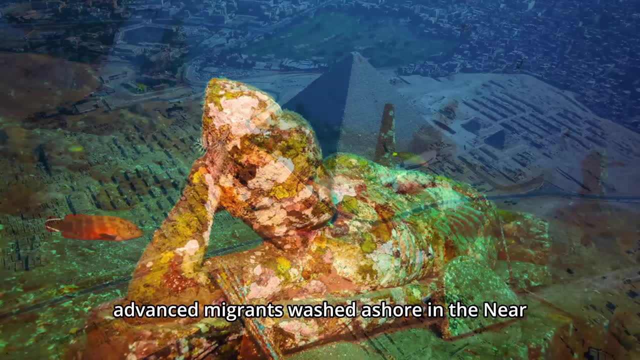 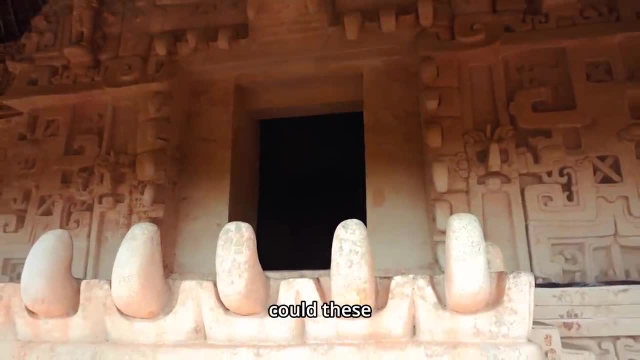 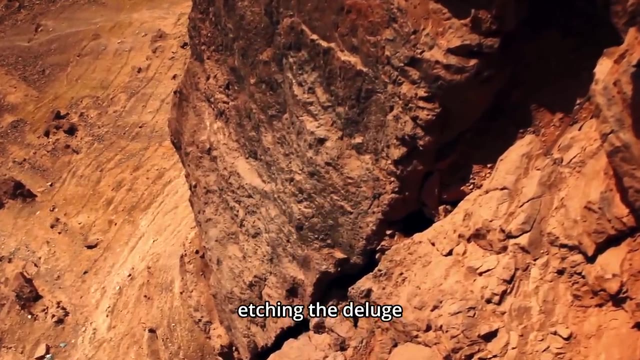 An enigmatic surge of remarkably advanced migrants washed ashore in the Near East during the latter half of the 8th millennium BC, raising intriguing speculations. Could these enigmatic settlers be the remnants of Plato's vanquished Western cultures? Plato's account etching the deluge at around 10,000 BC raises an intriguing question. 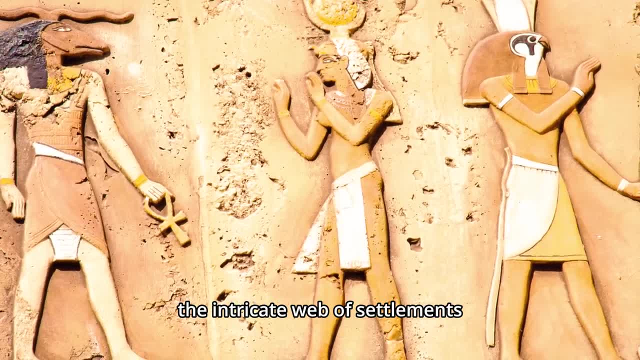 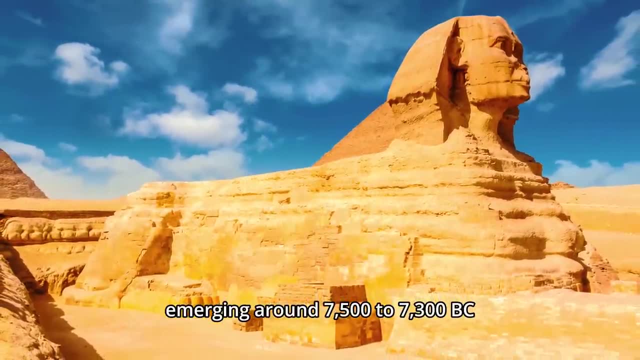 Is this timeline substantiated by the intricate web of settlements sprouting in the East like seeds sown in fertile soil, emerging around 7,500 to 7,300 BC? The echoes of ancient history may yet hold secrets waiting to be uncovered. 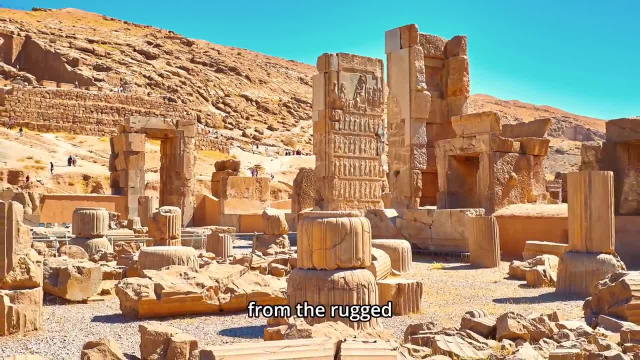 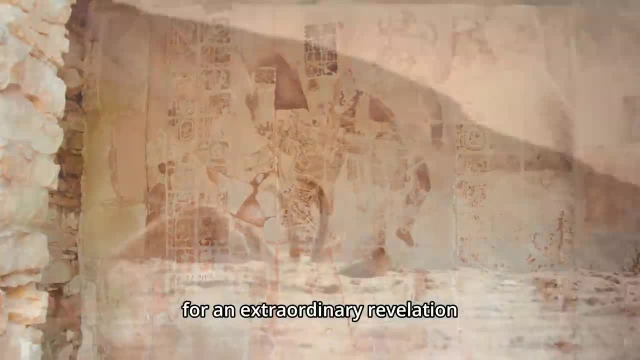 From the cradle of Syria to the heartland of Palestine, from the rugged expanse of eastern Anatolia to the mystic heights of the Zagros Mountains, the stage was set for an extraordinary revelation. Seemingly from the veil of obscurity, these advanced communities appeared. 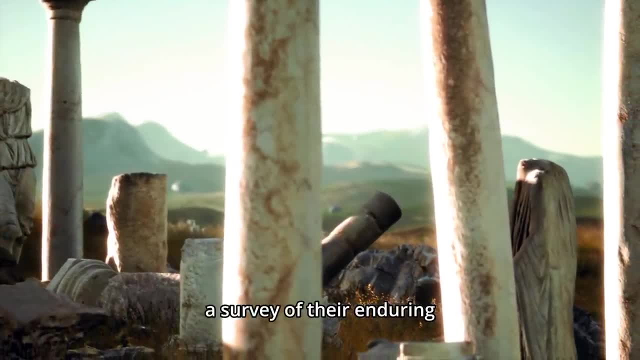 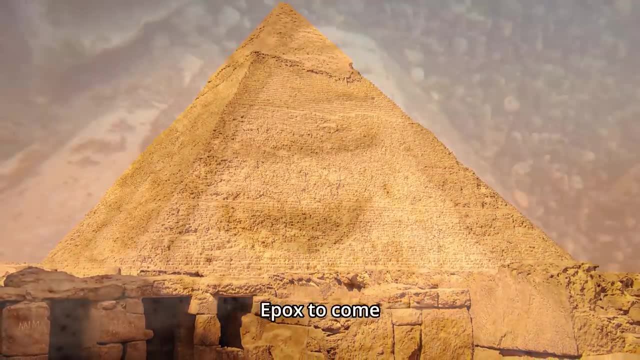 bearing the seeds of a future yet unseen. A survey of their enduring legacies reveals a breathtaking mosaic: the very foundations upon which the grand civilizations of epochs to come would be erected. In this simultaneous burst of ingenuity, these newcomers brought forth a tapestry of marvels. 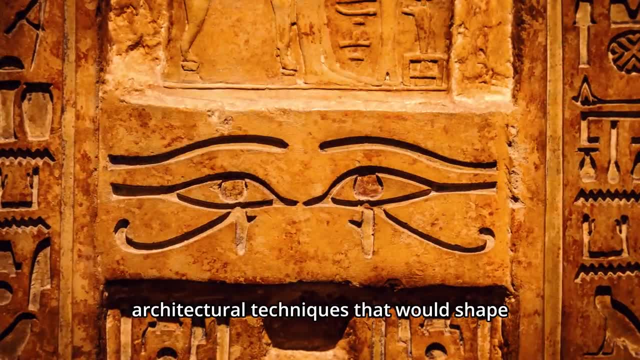 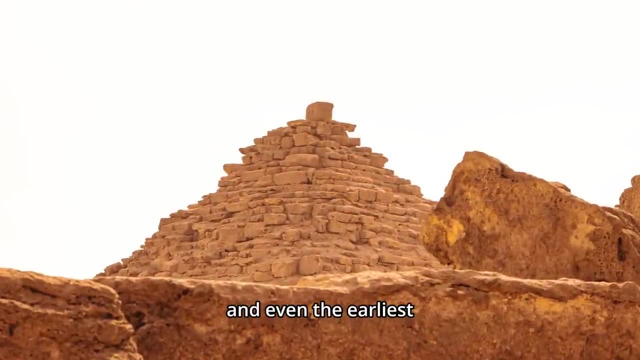 complex hybrid grains to nourish the hungry architectural techniques that would shape the skylines of ages, to follow functional pottery with a touch of artistry and even the earliest echoes of metalwork, casting the die for the industrial evolution that would dawn upon humanity. 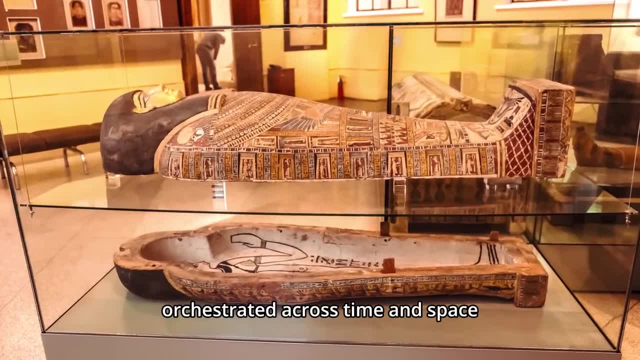 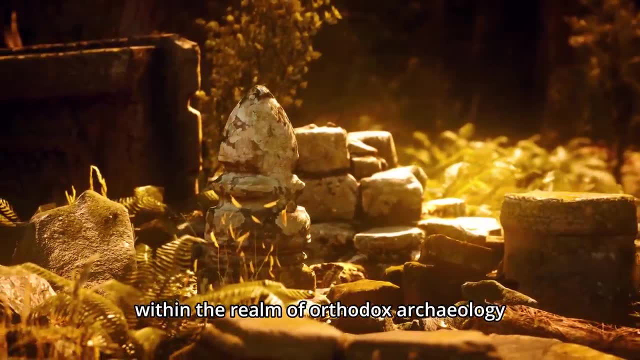 It was a symphony of innovation orchestrated across time and space by hands now enshrouded in the sands of history. Yet within the realm of orthodox archaeology and academia, the authenticity of Plato's Atlantis account remains shrouded in a persistent haze of doubt. 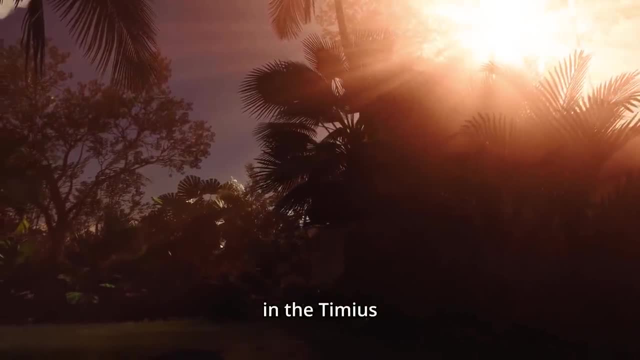 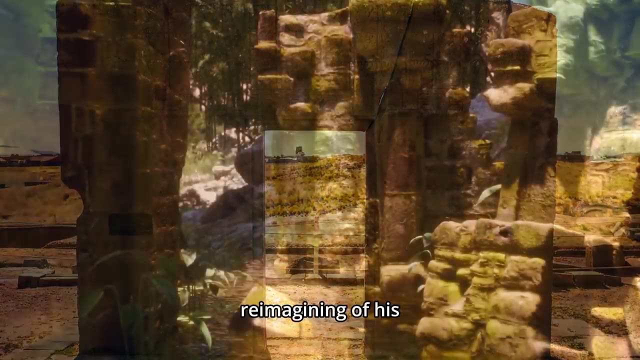 Skeptics argue that Plato's narrative in the Timaeus and Cretaceous should be perceived as nothing more than the exquisite tapestries of his imagination, a fictional reimagining of his utopian ideals, rather than a portrayal of a historical reality. 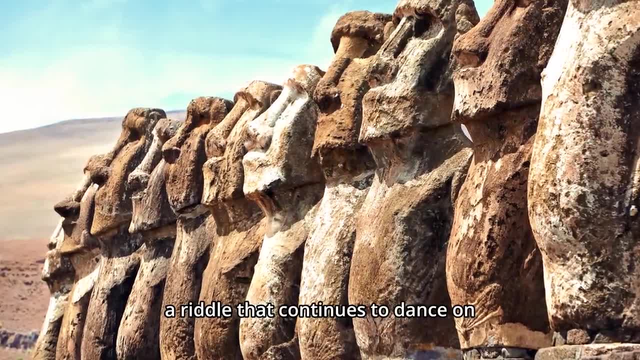 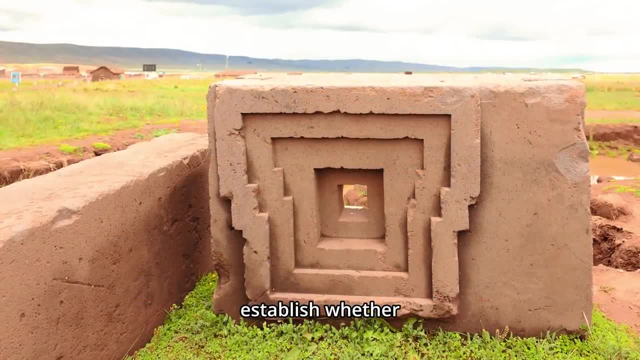 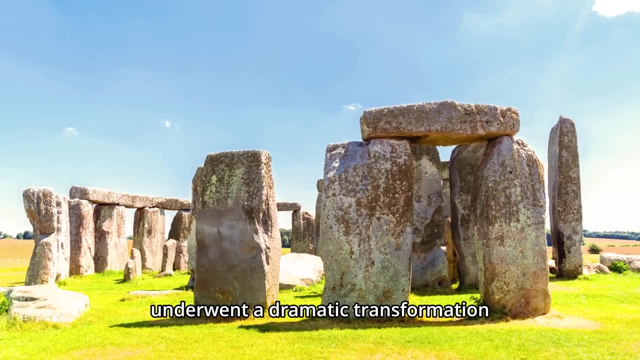 The enigma of Plato's Atlantis endures a riddle that continues to dance on the fine line between fact and fancy. No concrete evidence exists to definitively establish whether the land that lent its name to the vast Atlantic was indeed an island that plunged into the abyss or a continent that underwent a dramatic transformation. 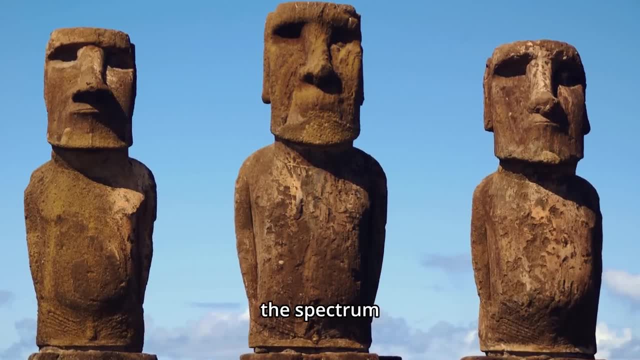 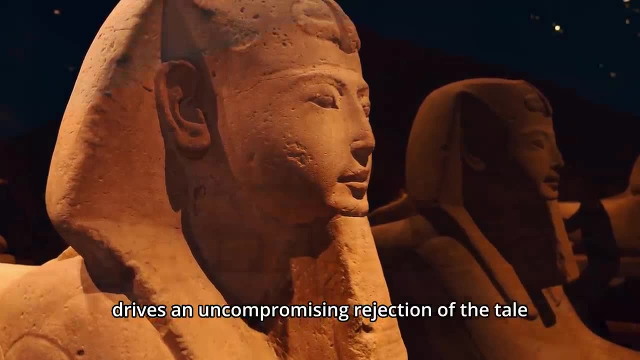 changing its identity. On one end of the spectrum, faith is kindled by the fire of intuition. on the other, extreme, unyielding skepticism drives an uncompromising rejection of the tale. The mystery persists, beckoning the curious to explore its enigmatic depths. 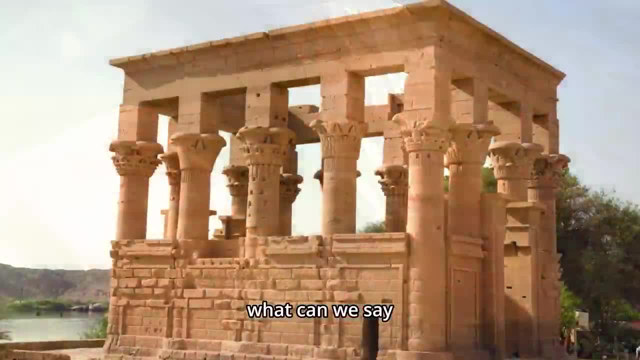 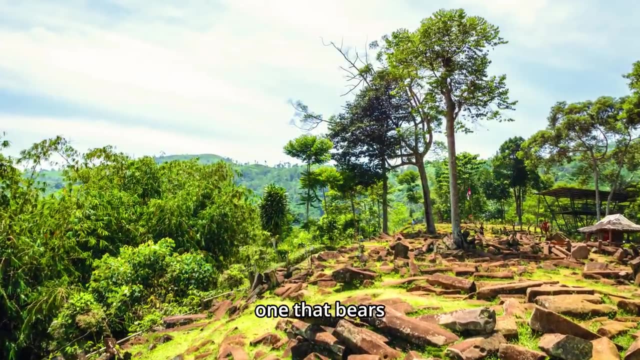 Amidst the swirling tides of speculation, what can we say for certain? The belief in the existence of Atlantis finds its bedrock in an ancient text, one that bears the mark of authenticity, documented and vetted through the annals of time. 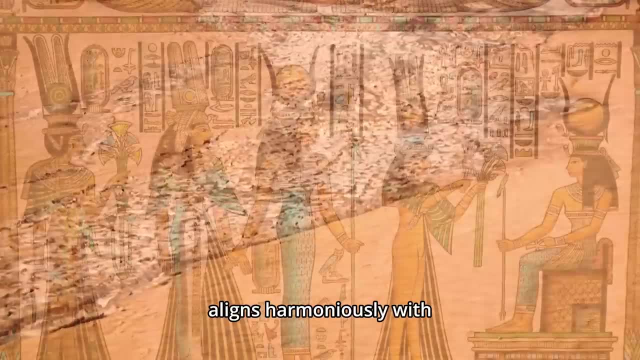 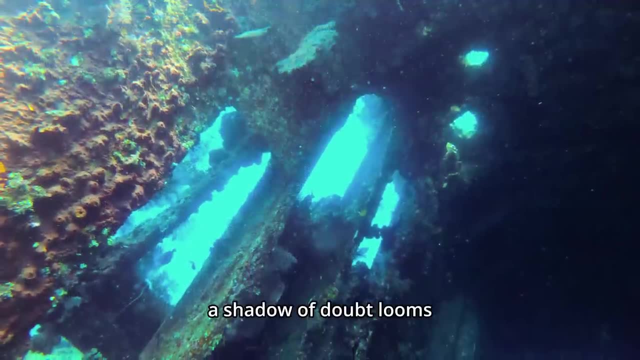 This text, a treasure from antiquity, aligns harmoniously with the principles of logic and remains open to the scrutiny of scientific inquiry. In opposition, a shadow of doubt looms, a suspicion that Plato may have woven the tapestry of Atlantis as a scaffold for his grand theories. 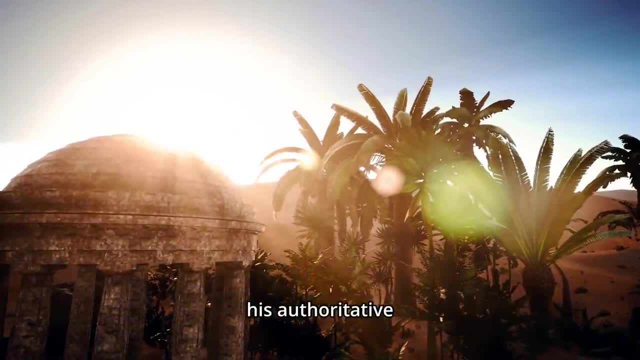 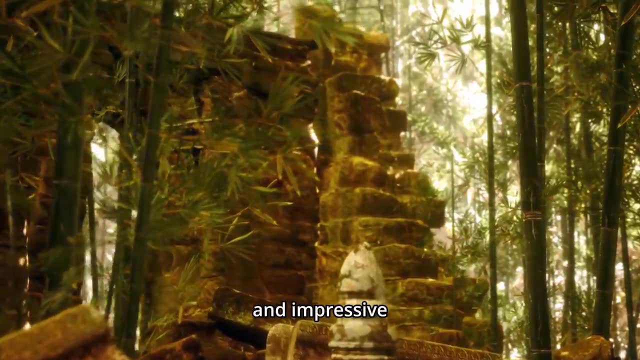 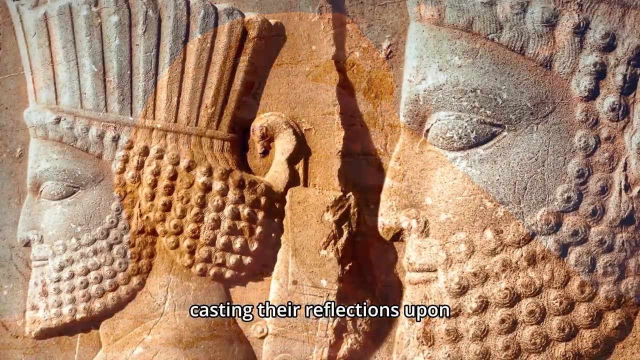 Perhaps, in his wisdom, he sought to clothe his authoritative political ideals in the beguiling attire of this captivating saga, an attempt to render them more palatable and impressive through the allure of a mesmerizing story. Two distinct narratives intertwine, casting their reflections upon the enigmatic waters of history. 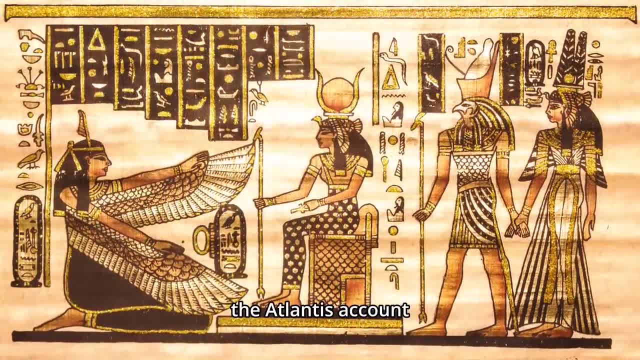 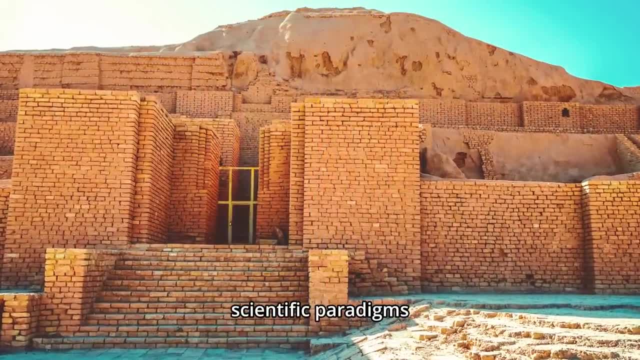 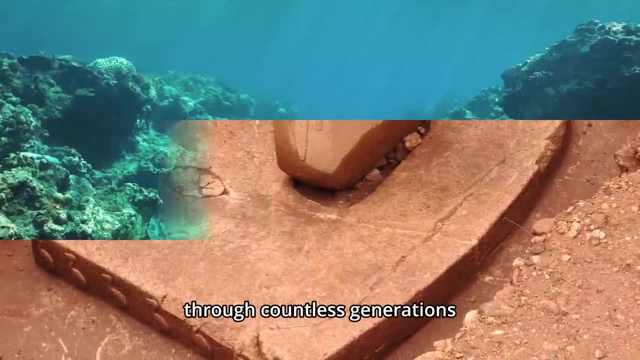 The debate rages on, with many facets of the Atlantis account veering into the realm of the extraordinary, challenging the harmonious union with established scientific paradigms. The age-old conundrum persists, a tantalizing enigma that has resisted resolution through countless generations. 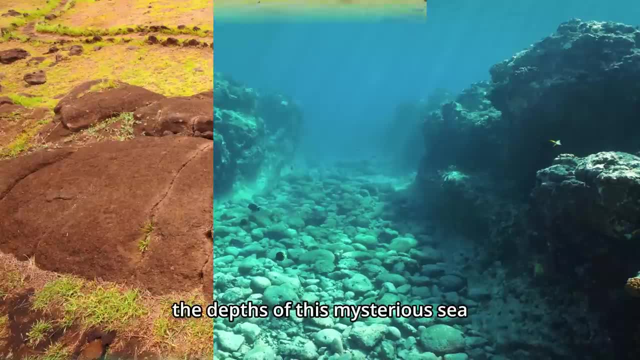 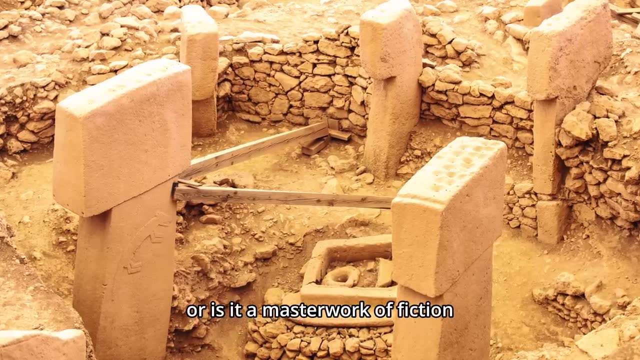 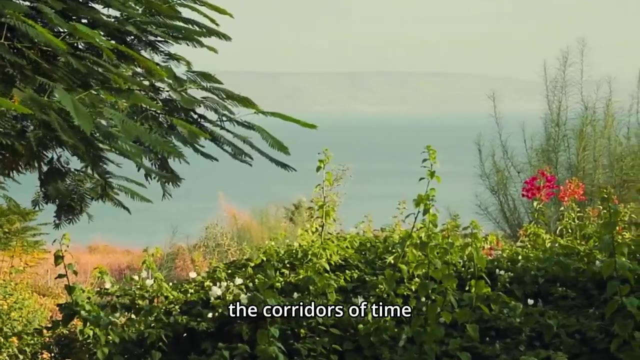 Ultimately, a single pivotal question emerges from the depths of this mysterious sea: Is Plato's treatise on Atlantis an authentic testament to history or is it a masterwork of fiction woven by the hand of a philosopher? It is a question that lingers an unresolved chord echoing through the corridors of time. 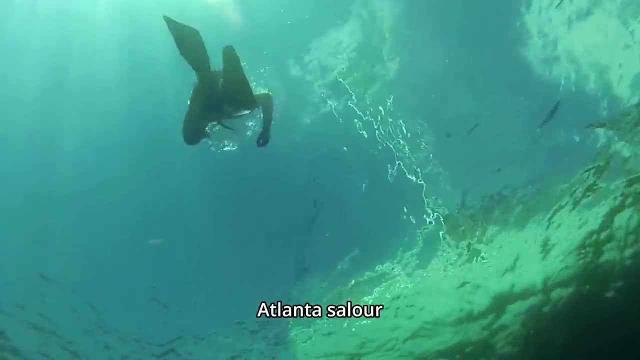 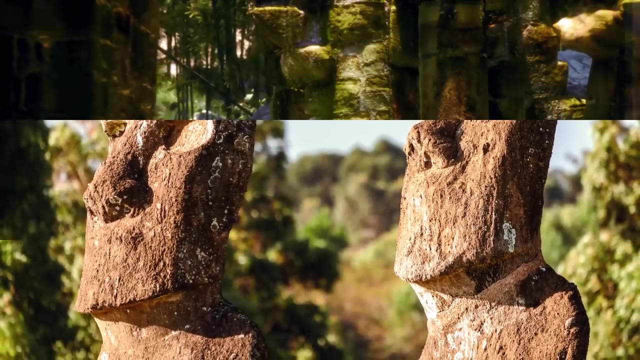 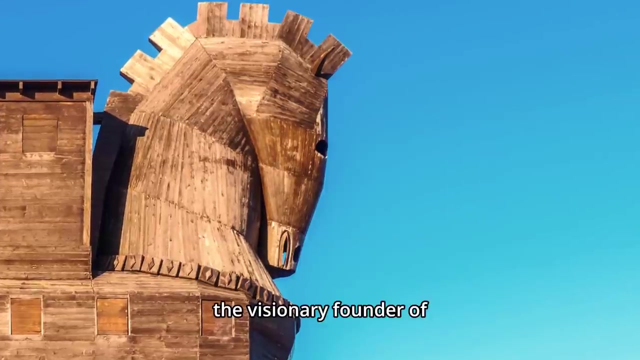 In the tapestry of modernity, the flames of Atlantis allure were rekindled during the 1800s, igniting a fervor of books, monographs and newspaper articles. Amid this resurgence, one luminary figure stood out: the remarkable H P Blavatsky, the visionary founder of the Theosophical Society. 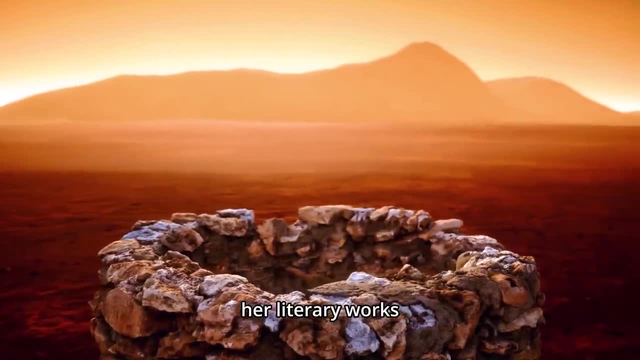 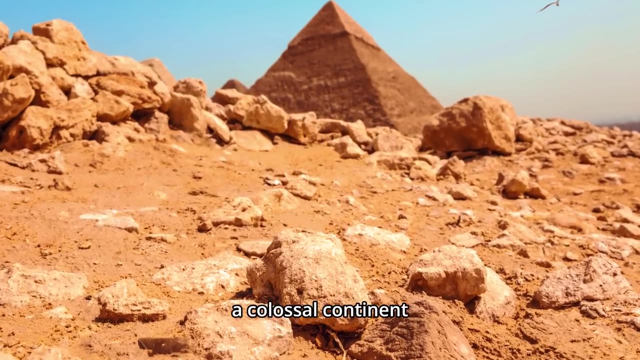 She wove the Atlantis narrative into her literary works Isis Unveiled and The Secret Doctrine. Blavatsky's vision painted a portrait of Atlantis as a colossal continent, a veritable leviathan that once stretched from the shores of South America to the western reaches of Africa in the south. 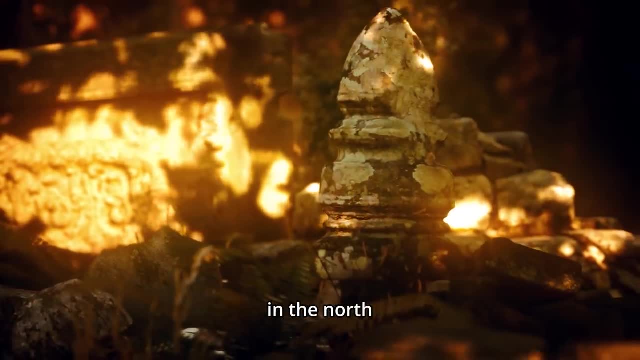 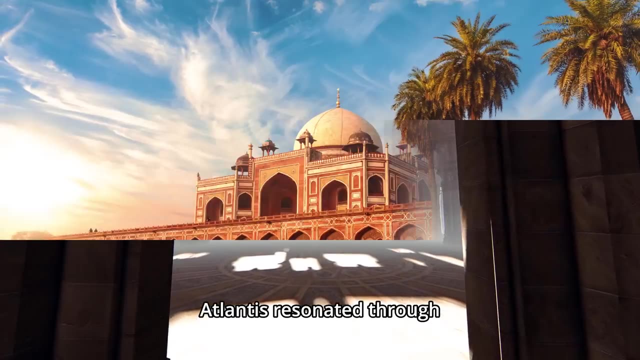 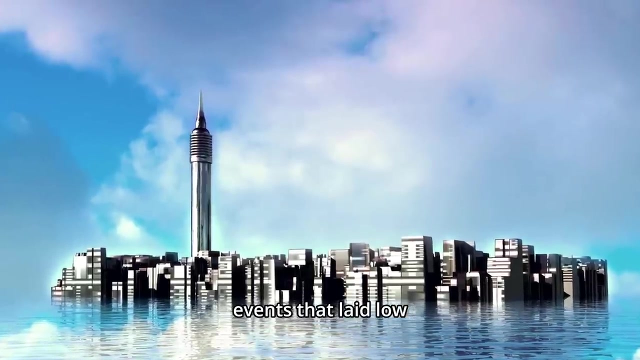 and from the pristine coasts of Newfoundland to the ancient land of Spain in the north. In her words she unravelled the enigmatic story of a lost realm, and the echo of Atlantis resonated through her intricate prose. Yet the passage of time bore witness to a string of cataclysmic events that laid low the colossal continent. 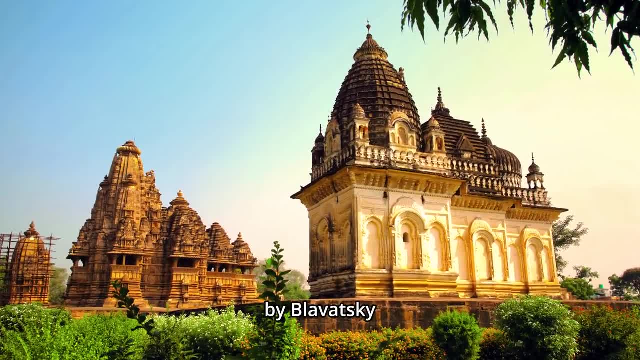 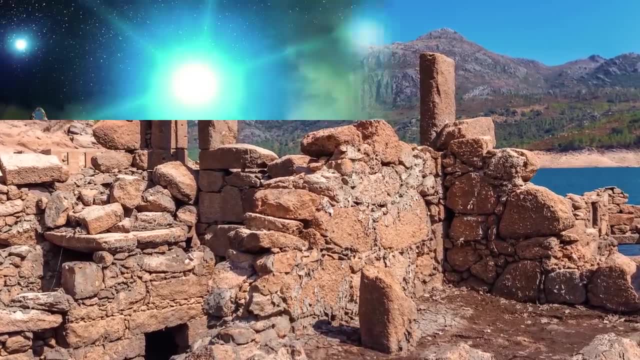 leaving in its wake two grand islands christened Ruta by Blavatsky, in the sultry tropics of the south, and Datia in the northern expanse, nestled near the Azores. Alongside these titans, a constellation of smaller islands and chains emerged. 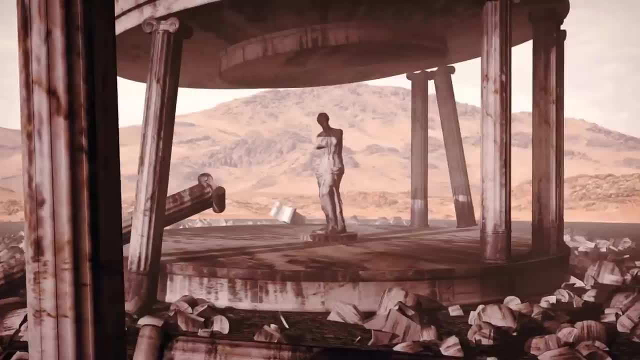 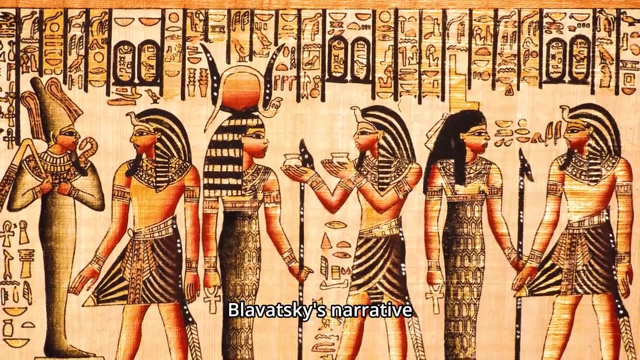 dotting the narrative of Atlantis with intrigue and mystery. The story unfolded like the map of a dream, painted with the strokes of geological upheaval. According to Blavatsky's narrative, the fate of Ruta unfolded as a tragic dance with time. 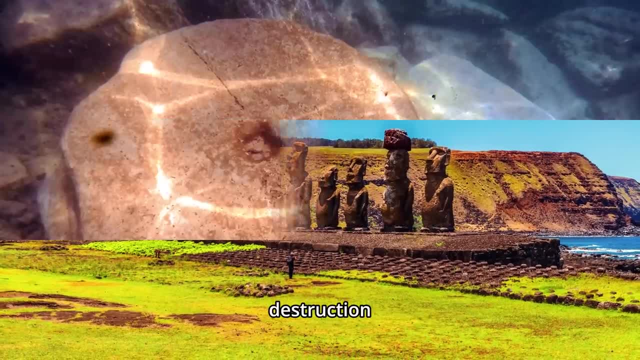 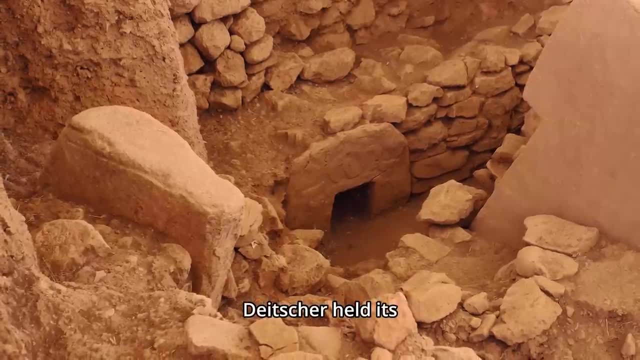 as it bore the brunt of a geomagnetic shift that unfurled its destruction, an ordeal spanning back nearly 850,000 years. In a poignant contrast, Datia held its ground for eons, enduring the relentless march of history, until approximately 270,000 years ago. 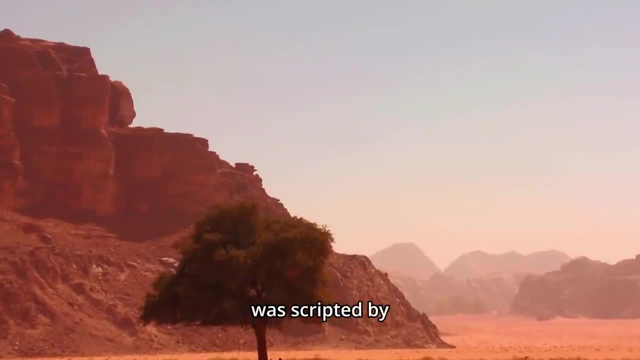 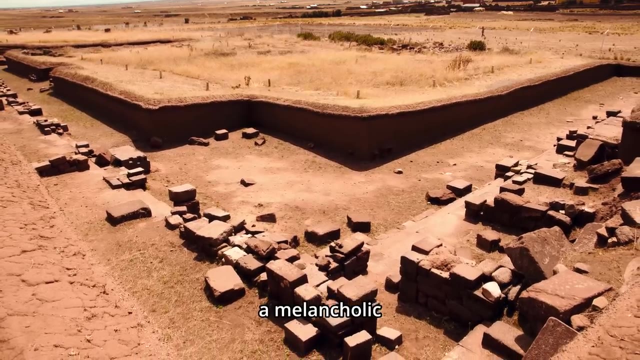 At this juncture. its final chapter was scripted by a series of undisclosed cataclysms, leaving behind only the hauntingly desolate island chain of the Azores. a melancholic testament to a world now lost to the annals of time. 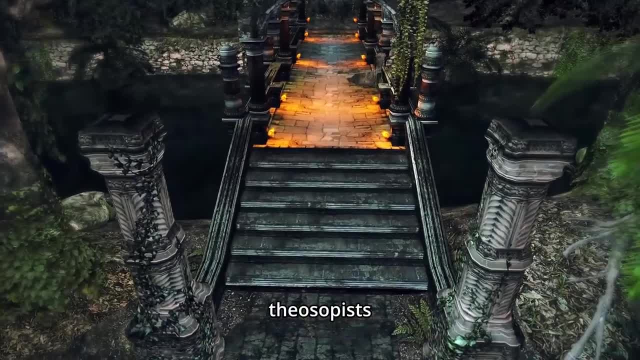 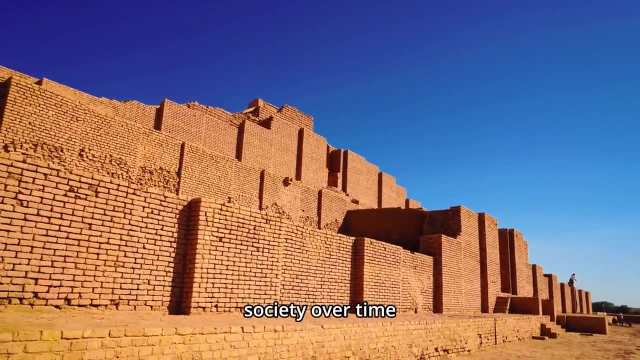 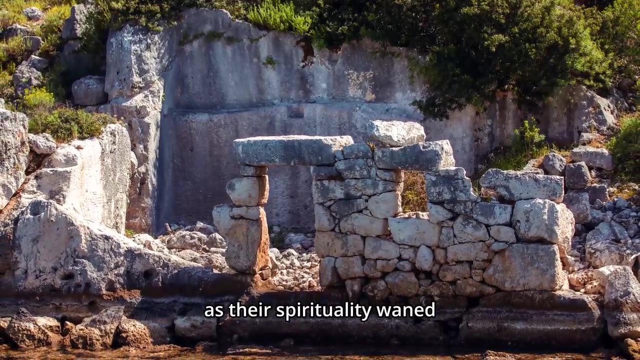 Rudolf Steiner, a luminary among Austrian theosophists, wove a profound narrative of Atlantis. He postulated that the Atlantean society over time descended into a spiral of moral decay and unbridled materialism. As their spirituality waned, they delved into the abyss of black magic. 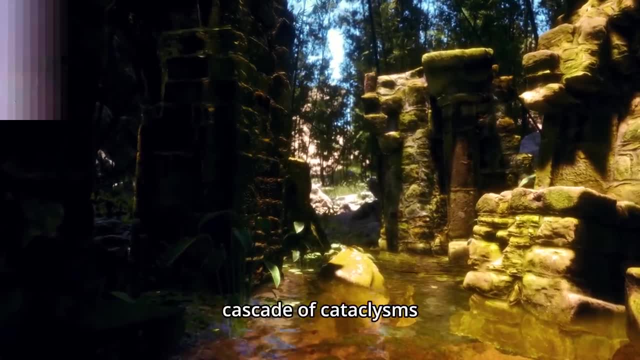 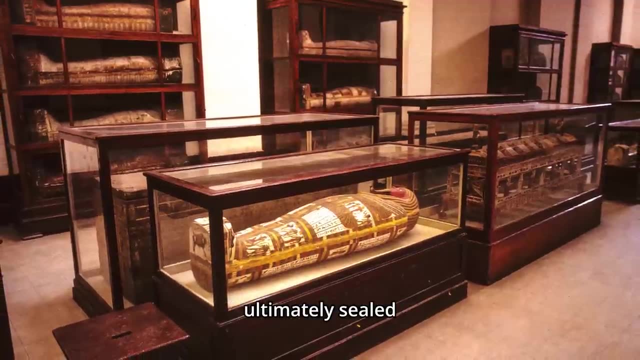 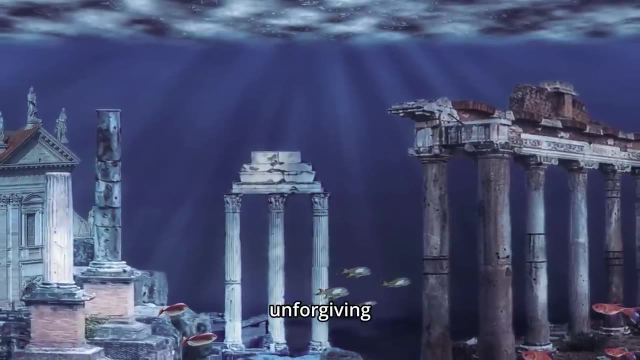 wielding forces of destruction that unleashed a tempestuous cascade of cataclysms upon their island. These cataclysms, born of hubris and wayward intentions, ultimately sealed the fate of Atlantis, submerging not only the land but also the majority of its inhabitants beneath the unforgiving depths of history. 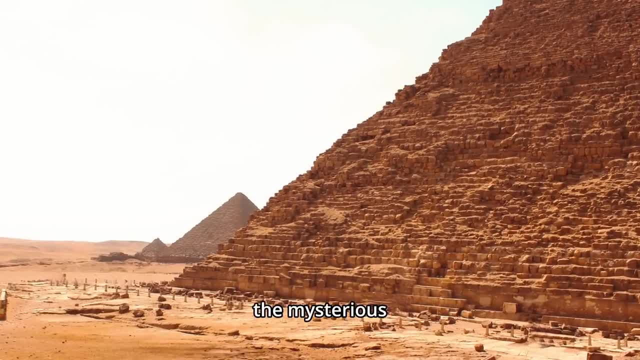 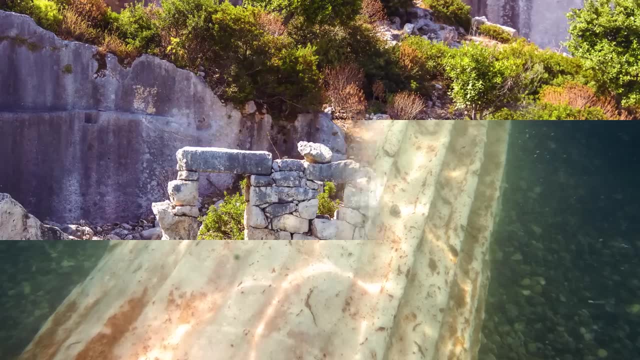 In the Theosophical Tapestry of Belief, the mysterious Lemuria emerges as yet another lost continent, its existence shrouded in the veil of history, Stretching from the eastern fringes of Africa to the sweeping landscapes of Australia in the Southern Pacific. 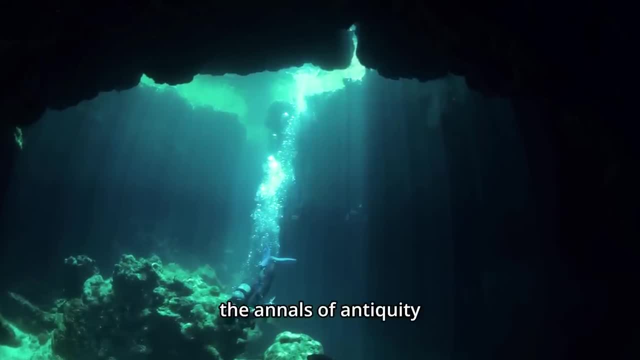 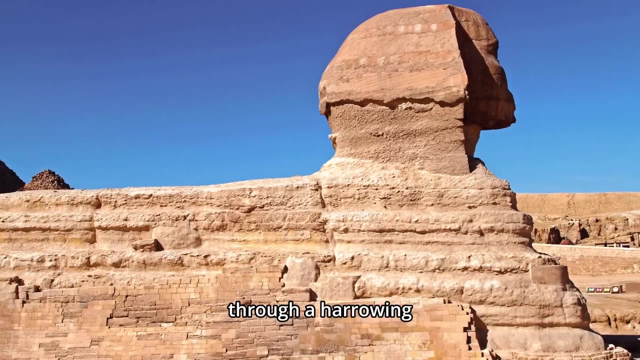 this enigmatic realm has its own chapter in the annals of antiquity. Like its Atlantean counterpart, Lemuria is said to have met its untimely demise through a harrowing series of cataclysmic events, a saga etched with the strokes of destruction. 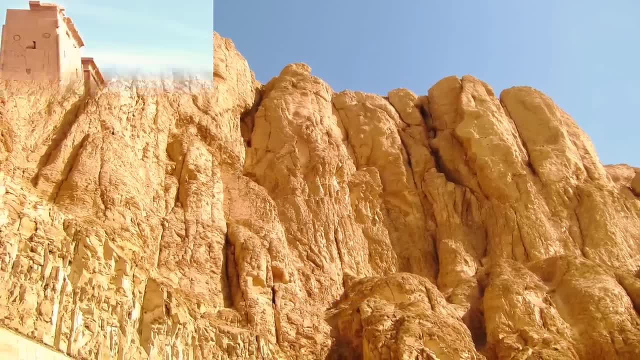 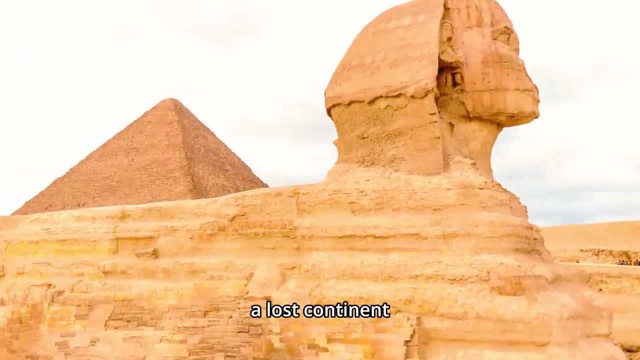 leaving only the whispers of its existence to reverberate across time. Within the rich tapestry of Theosophical Beliefs, there unfurls the enigmatic legend of Lemuria, a lost continent veiled in the mists of ages past. Its sprawling territory extended from the far reaches of eastern Africa. 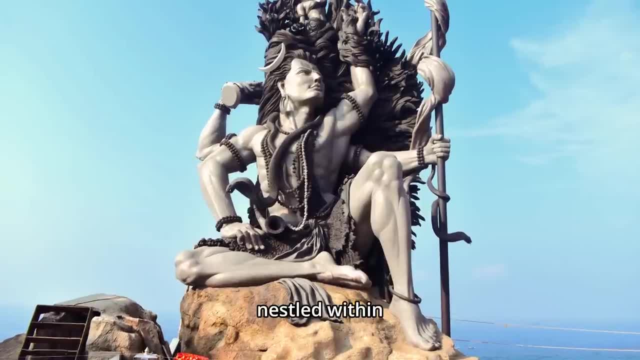 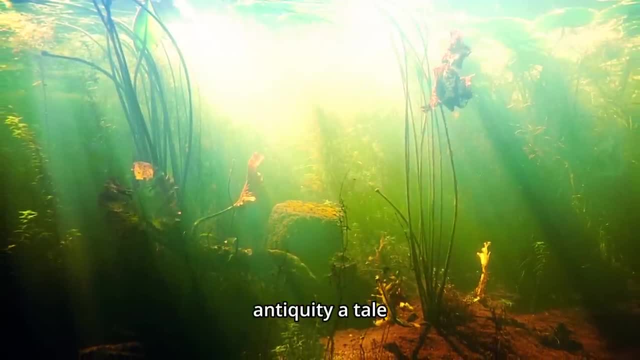 to the majestic landscapes of Australia. nestled within the vast expanse of the Southern Pacific, This cryptic realm scribed its own chapter in the annals of antiquity, a tale akin to its Atlantean counterpart, marked by a tragic symphony of cataclysms. 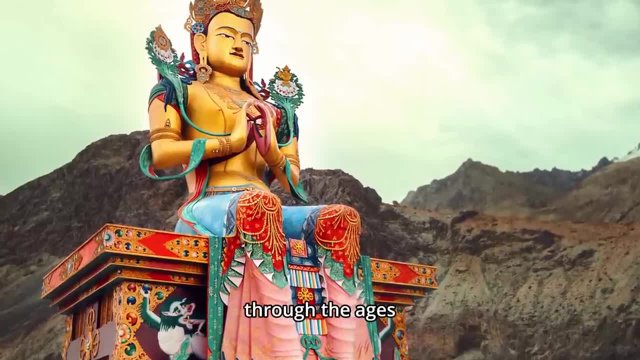 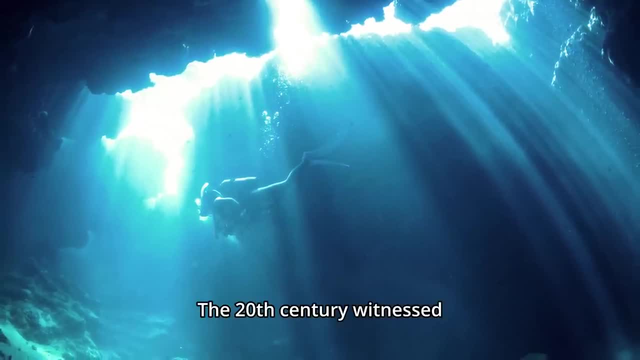 The strokes of this destructive epic echoed through the ages, leaving naught but elusive whispers to tell the story of Lemuria's existence. The 20th century witnessed the enduring allure of Atlantis, captivating not only the general public but also the intrigue of journalists, scholars. 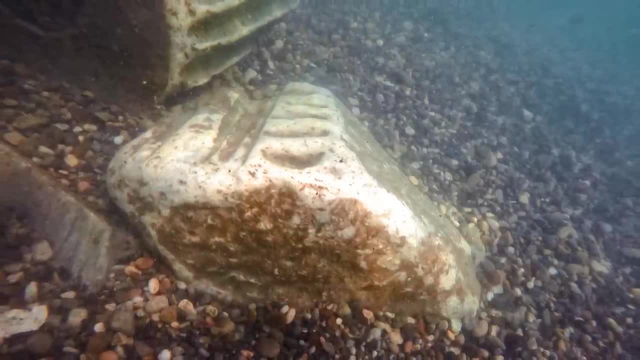 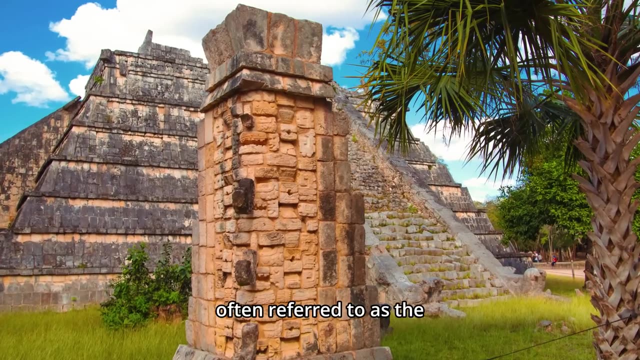 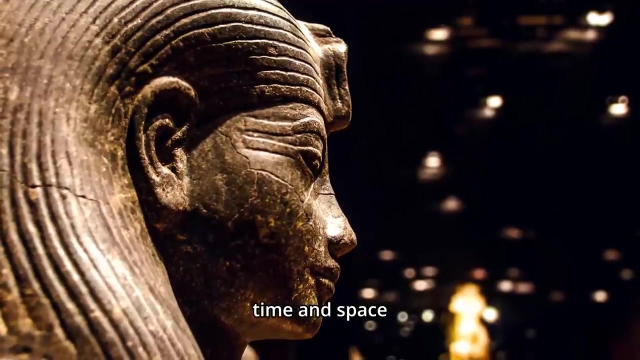 and even individuals with more mystical inclinations. Among these enigmatic figures, one standout persona was Edgar Cayce, a celebrated American psychic, often referred to as the Sleeping Prophet. In his mesmerizing trance states, he ventured into the depths of time and space. 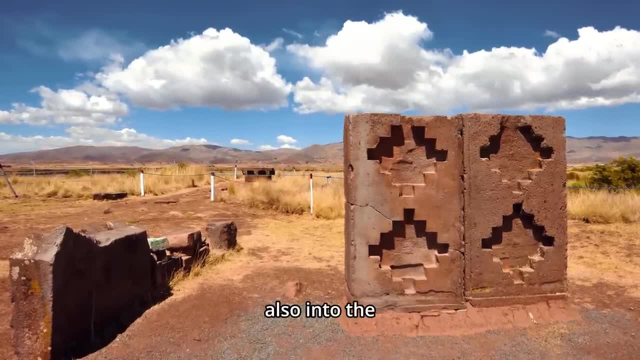 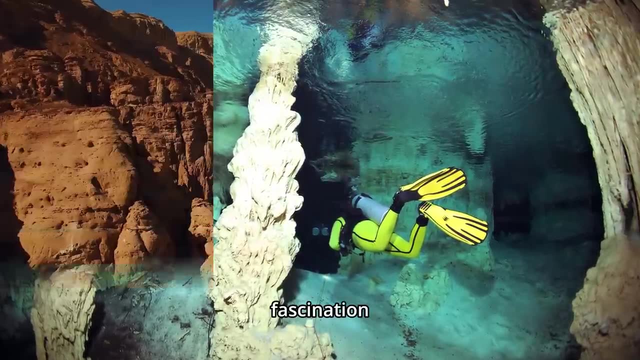 revealing insights not only into individuals' past lives, but also into the enigmatic realm of Atlantis. Cayce's unique ability unveiled hidden facets of history, sparking fascination and wonder in those drawn to the mysteries of our shared human story. As per Cayce's mystical revelations, 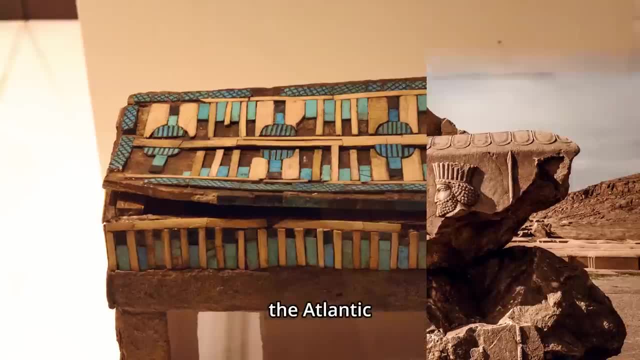 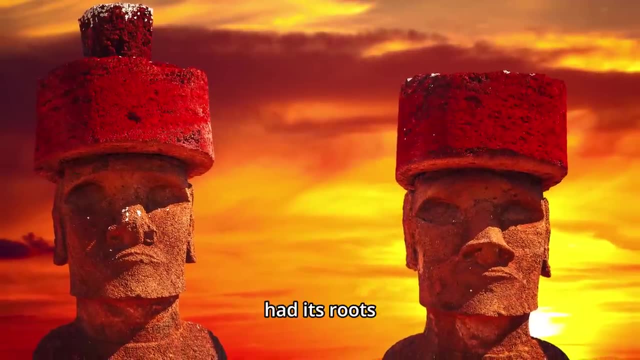 Atlantis staked its claim in the vast expanse of the Atlantic, stretching from the Saragossa Sea to the Azores. Within these waters, a splendid civilization had its roots, tracing its origins back to an astonishing 200,000 years ago. 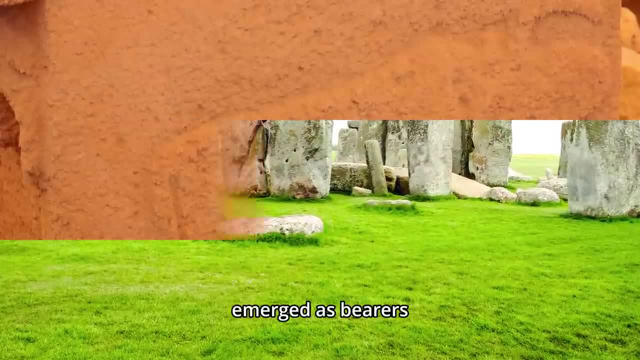 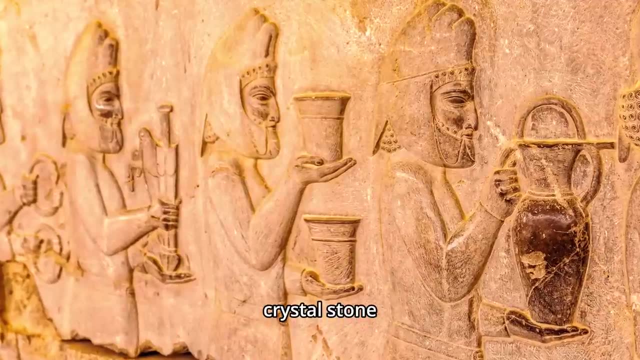 The Atlanteans, in Cayce's vision, emerged as bearers of a profoundly advanced culture. They held in their possession a mysterious crystal stone, a marvel that could harness the radiant energy of the sun. In the corridors of their ingenuity, 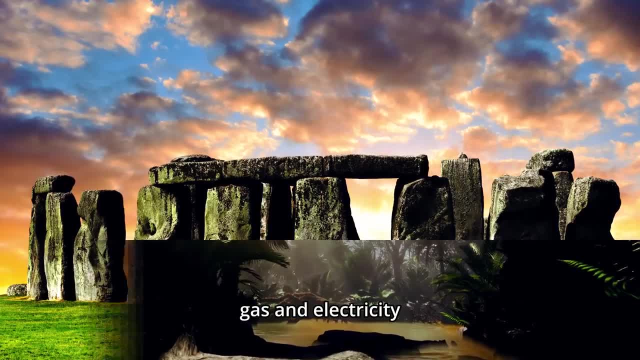 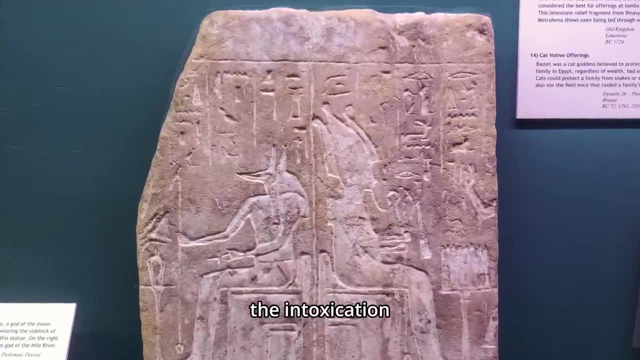 they also harnessed the powers of steam gas and electricity, painting a picture of a society on the cusp of unparalleled innovation. Regrettably, the intoxication of boundless prosperity eventually led the Atlanteans down the treacherous path of greed and moral decay. 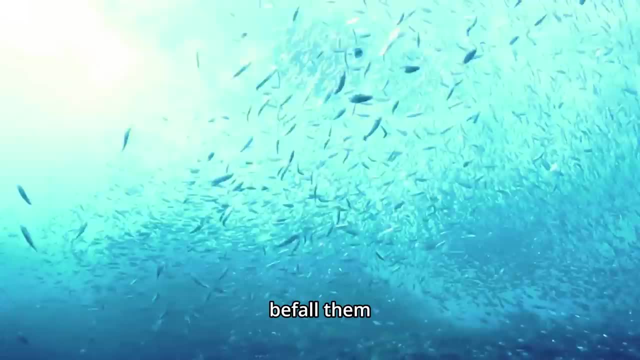 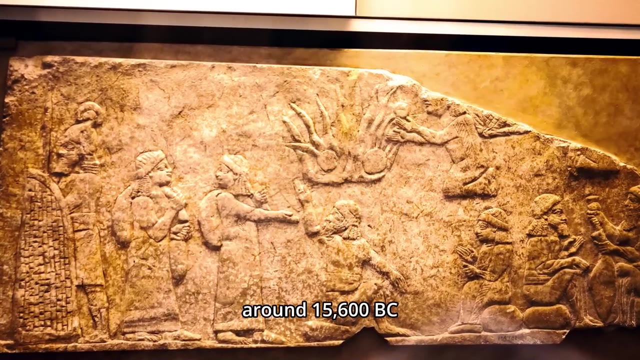 rendering them ripe for the cataclysmic reckoning that would ultimately befall them. This destiny unfurled in waves, with one significant upheaval striking around 15,600 BC and the final devastating blow around 10,000 BC. 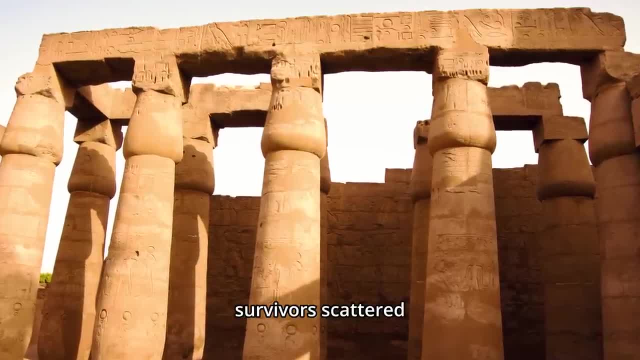 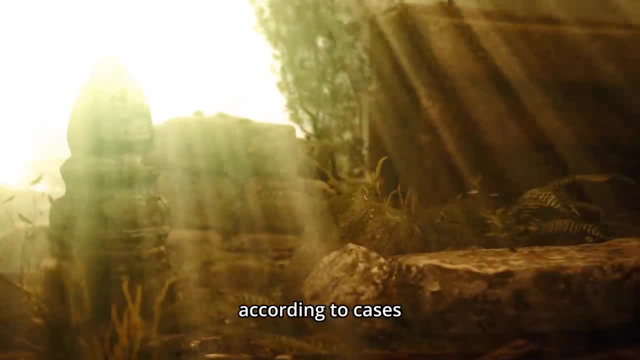 In the wake of their homeland's demise, the Atlantean survivors scattered like seeds in the wind, finding new homes in the realms of Europe and South America. According to Cayce's prophetic visions, remnants of their ancient wisdom and records would be scattered across the globe. 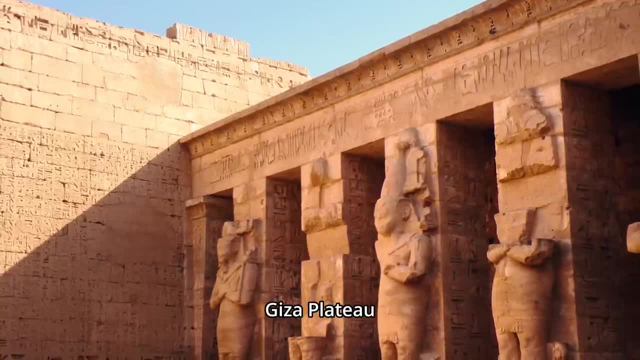 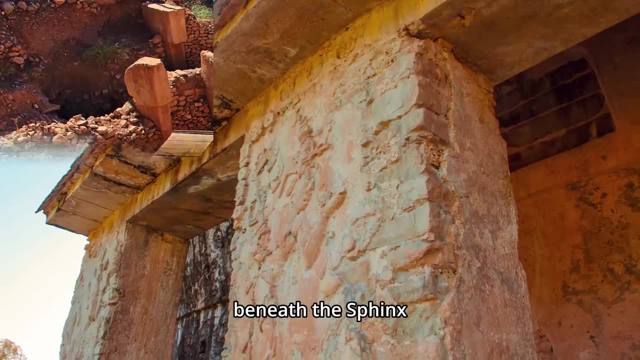 with some hidden in the enigmatic shadows of the Giza Plateau. He even foresaw the discovery of documents affirming Atlantis's existence tucked away in a chamber beneath the Sphinx, waiting to rewrite the pages of history In the early decades of the 20th century. GI Gurdjieff. 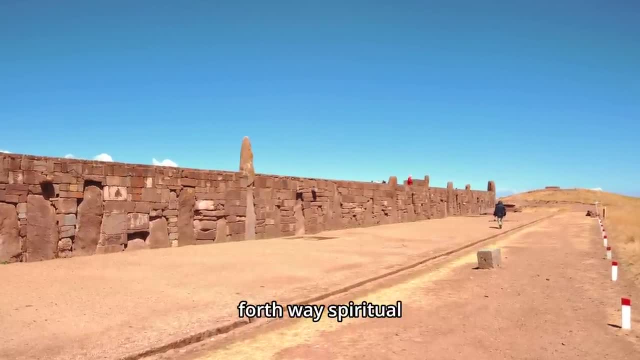 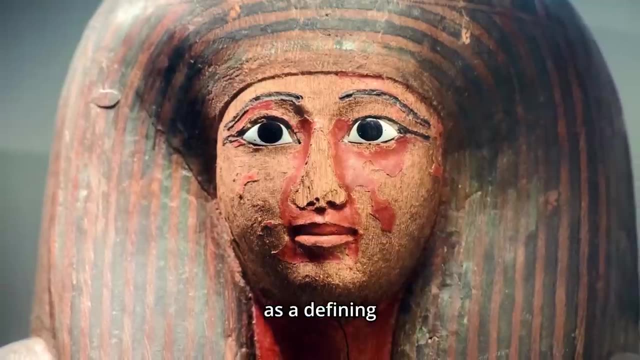 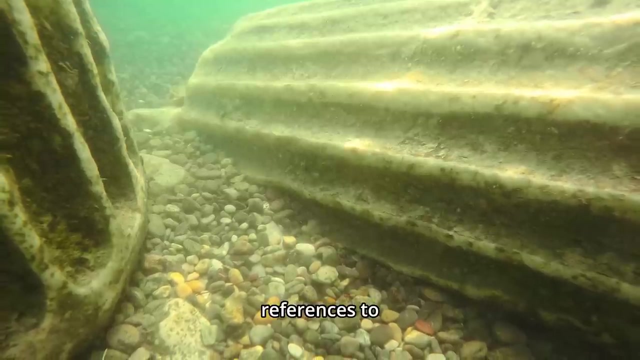 a herald of the transformative fourth-way spiritual path in the Western world. cast his gaze upon the annals of human history, He painted Atlantis as a defining turning point, an epoch-shaping moment. Within the tapestry of his teachings and writings, references to Atlantis resonated like whispered secrets. 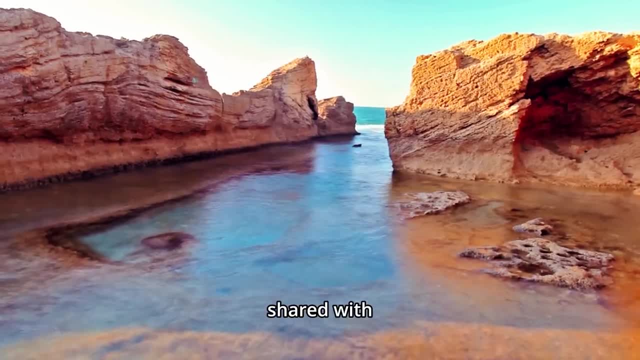 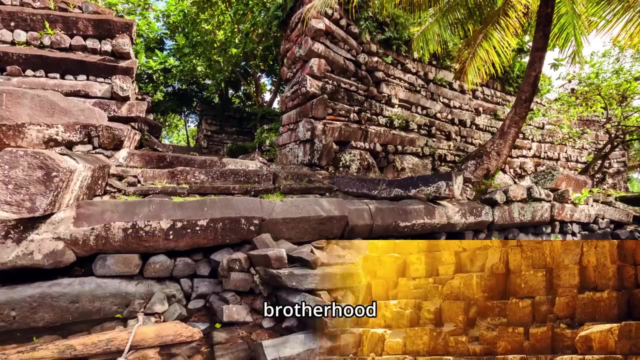 Gurdjieff, in his wisdom, shared with his devoted students the belief that the famed rock paintings gracing the caverns of Lasso, France, bore witness to a sacred brotherhood. This fraternity, he contended, emerged in the aftermath. 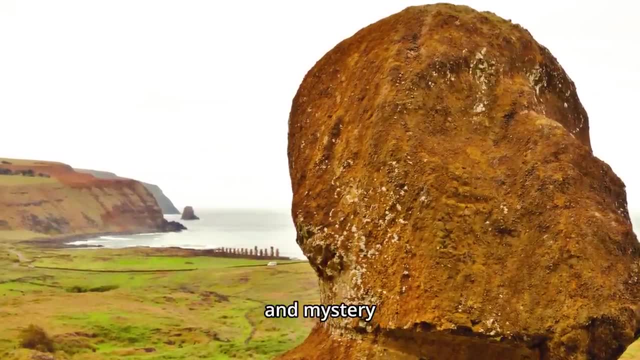 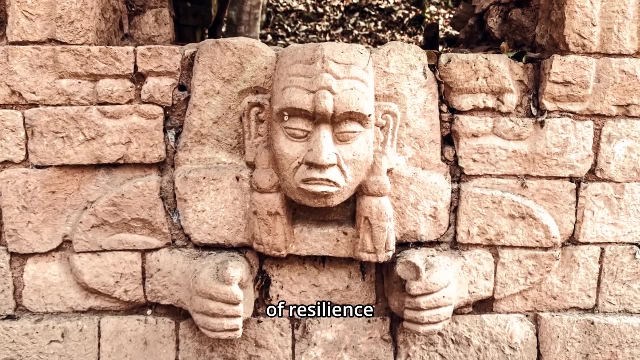 of the catastrophic loss of Atlantis, an era drenched in myth and mystery. The echoes of this ancient legacy lingered within the strokes of those ancient artists, telling a story of resilience and renewal in the face of profound upheaval. John G Bennett, a dedicated disciple of Gurdjieff. 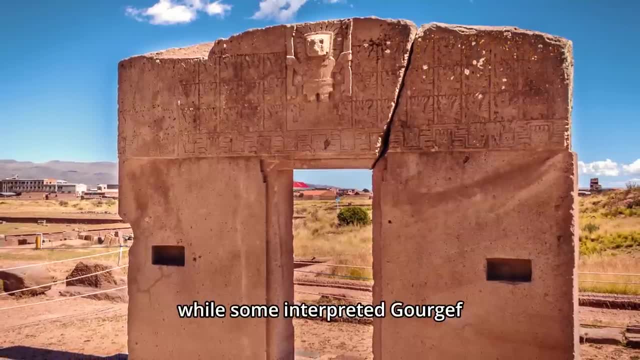 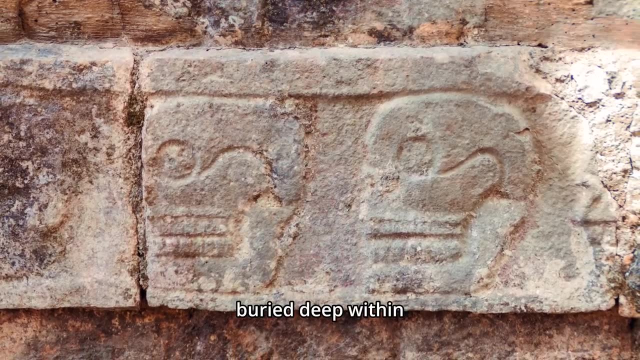 illuminated a facet of his teacher's perspective. While some interpreted Gurdjieff's allusions to Atlantis as metaphorical, portraying the notion of a submerged conscience buried deep within the recesses of the human psyche, there remained a steadfast belief that Gurdjieff intended the story of Atlantis. 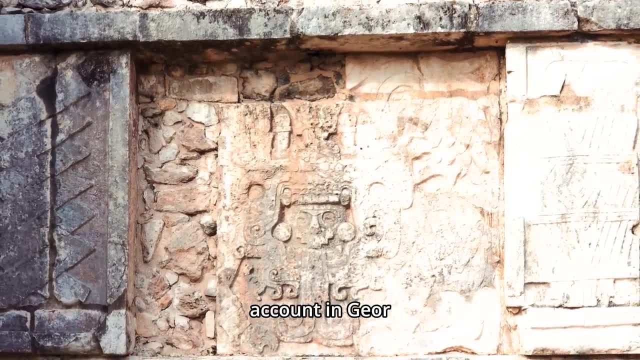 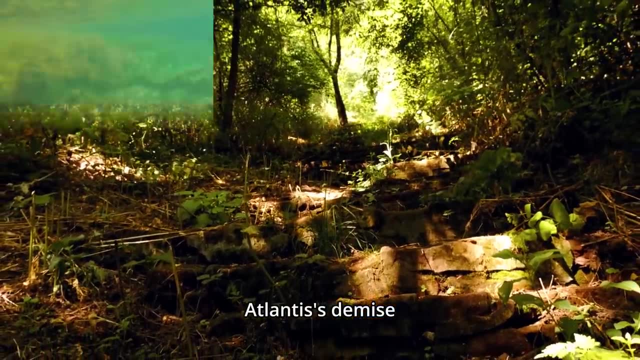 to be embraced as a literal account In Gurdjieff's magnum opus Beelzebub's Tales. to His Grandson he unfurled the saga of Atlantis's demise. According to his narrative, this calamity was marked by what he crippled. 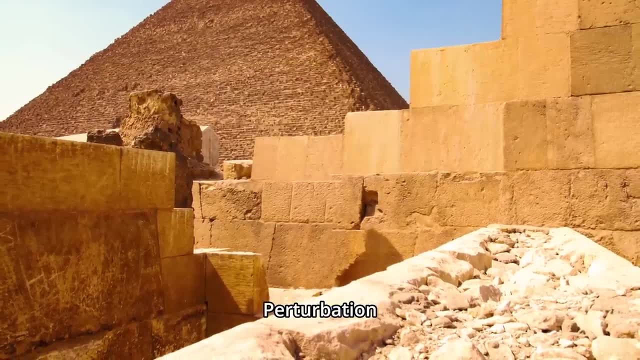 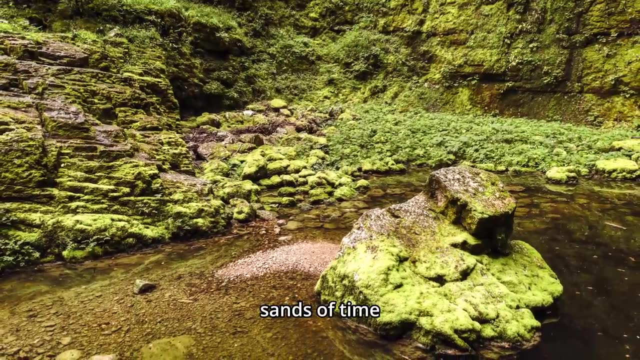 and was practically referred to as the Second Transypanian Perturbation, a cataclysmic event that echoed through the ages as a testament to a once great civilization lost in the sands of time Amidst the throes of a second great catastrophe that befell their planet. 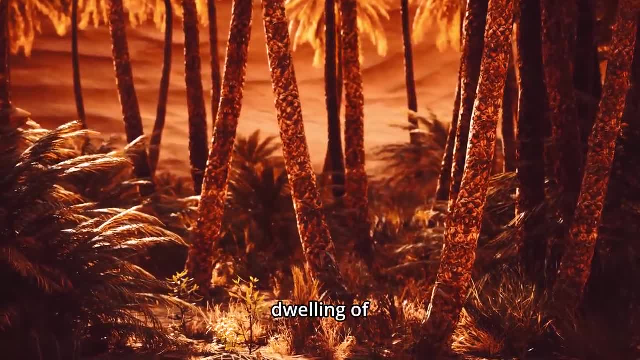 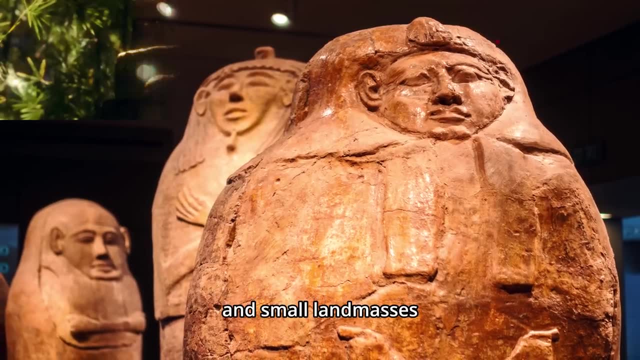 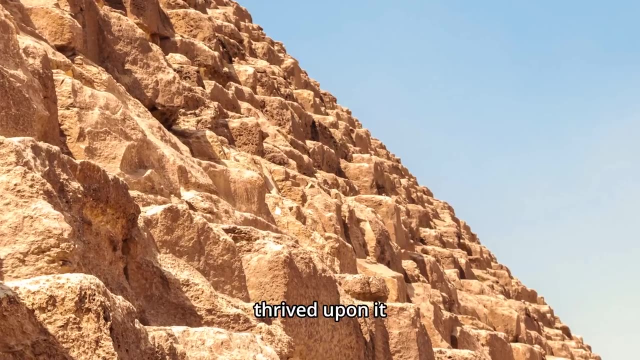 the mighty Atlantis, once the grandest of continents and the paramount dwelling of the three-brained beings, met a somber fate. Alongside countless other large and small landmasses, Atlantis was swallowed by the planet's tumultuous depths, carrying with it the existence of the three-brained beings who had thrived upon it. 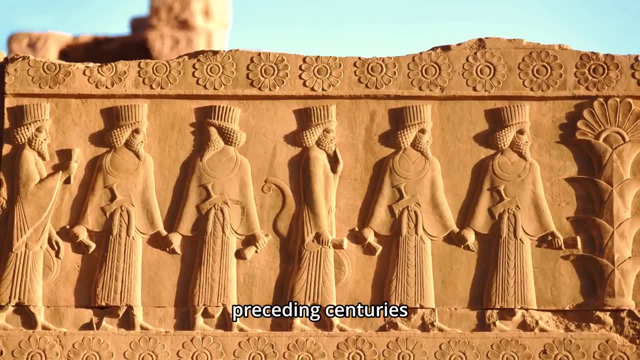 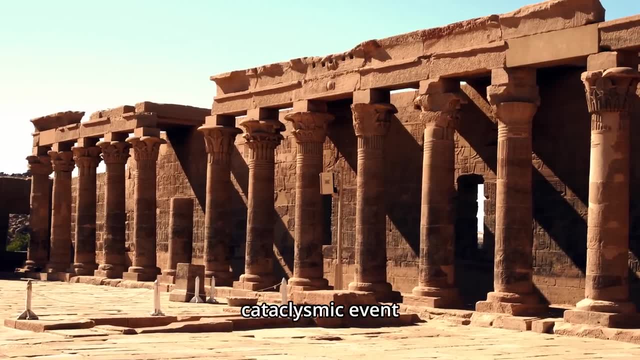 Everything they had toiled and striven for over the span of countless preceding centuries was claimed by the merciless embrace of the Earth's inner forces. In the wake of this cataclysmic event, a transformation unfurled within the planet's bosom. 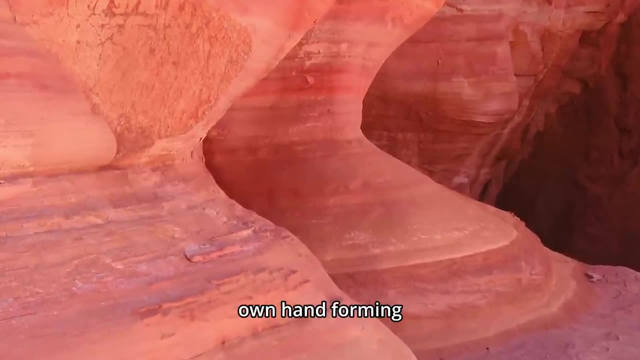 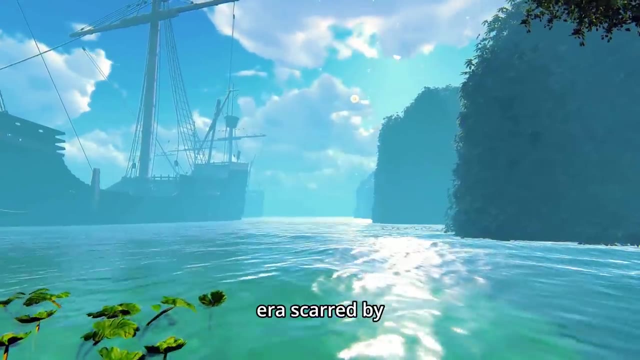 New lands emerged, sculpted by the planet's own hand, forming fresh continents and islands that now define the modern world. These remnants of a bygone era, scarred by the ancient tides of fate, stand as silent witnesses to the profound cycles of creation and destruction. 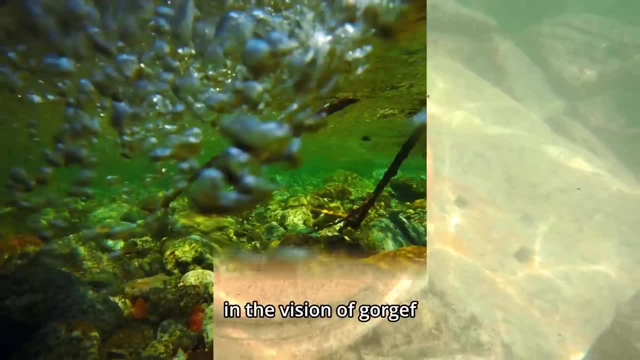 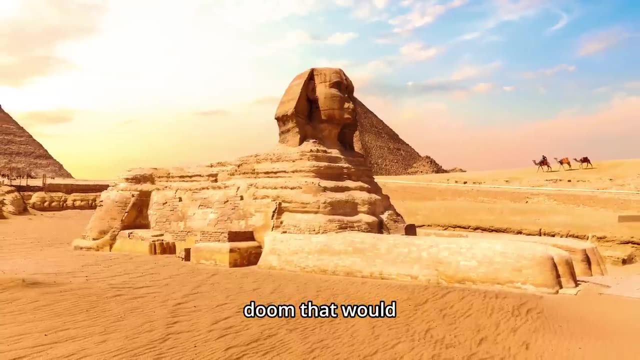 that have woven the tapestry of our cosmic history. In the vision of Gurdjieff, the seers of Atlantis possessed the gift of foresight and they had gazed upon the impending doom that would befall their cherished land. These visionaries, driven by the weight of prophecy, 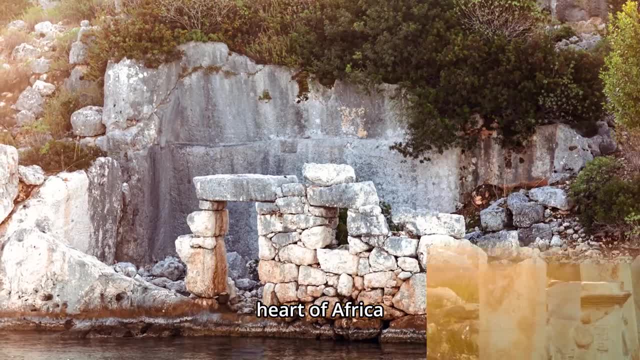 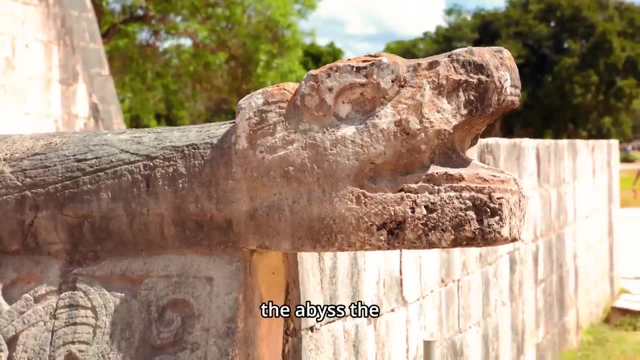 led a migration of many Atlanteans towards the heart of Africa, where the ancient source of the Nile lay. When the catastrophic hour struck and Atlantis crumbled into the abyss, the tenacious survivors managed to escape to the sanctuary of Central Africa. 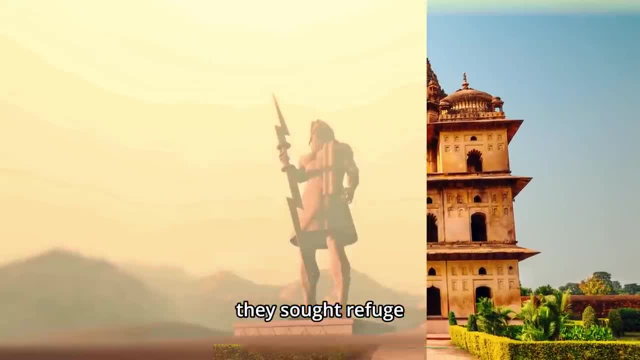 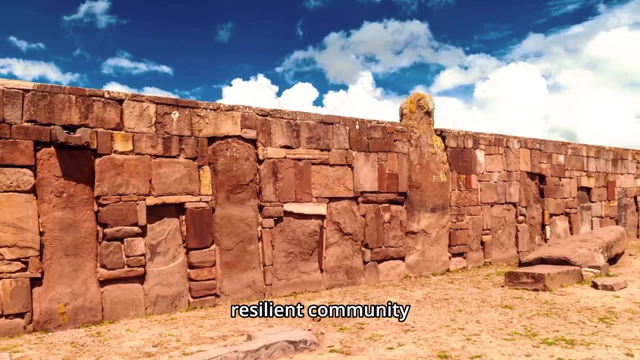 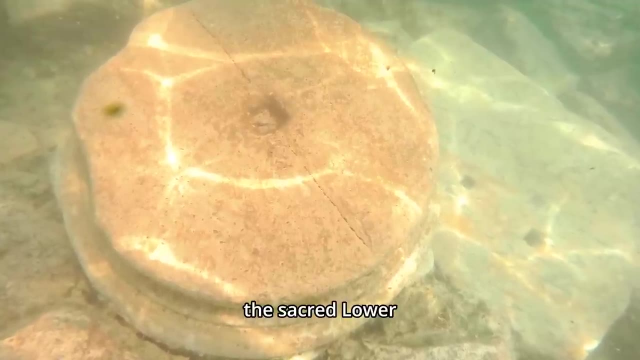 There, amidst the lush heart of the continent, they sought refuge, carrying with them the torch of their society's profound initiations. With time, this resilient community ventured northward and eastward, embarking on a journey of survival and enlightenment until they reached the sacred lower Nile valley. 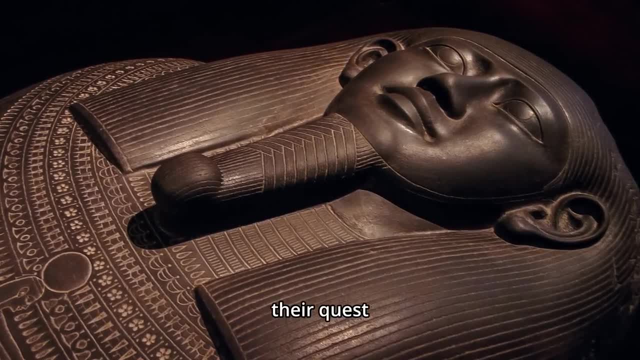 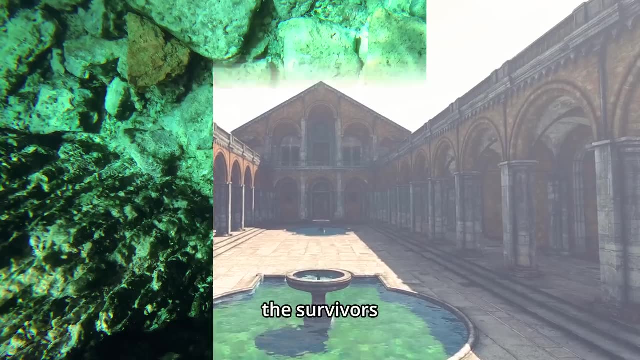 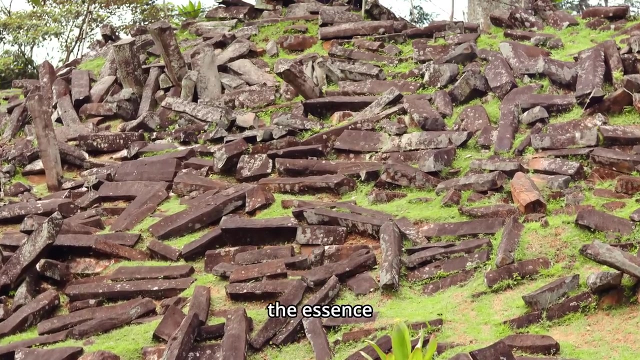 In this haven of isolation, they continued their quest, unwavering in their dedication to the sacred tasks laid out by their initiatory society. Among the survivors of Atlantis, who sought sanctuary in the ancient cradle of Egypt, a remarkable legacy endured: The essence of their profound wisdom teachings. 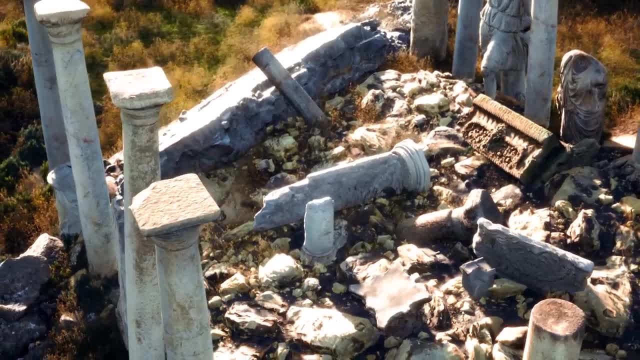 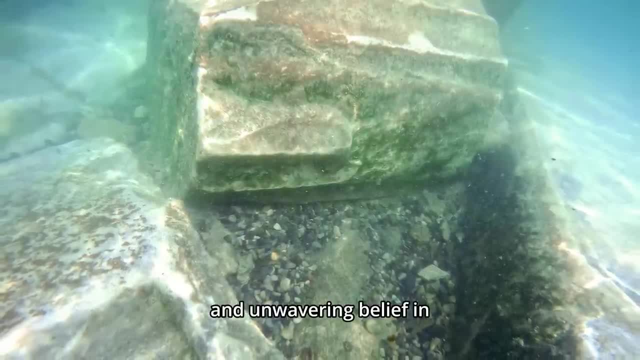 born of their ancestral homeland remained undiminished For generations that followed the fall of Atlantis. a profound and instinctive knowing persisted within them, an unwavering belief in the concept of completed personal being, In the hallowed presence of these beings. 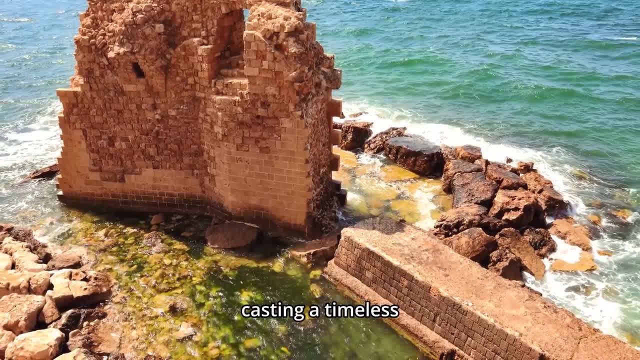 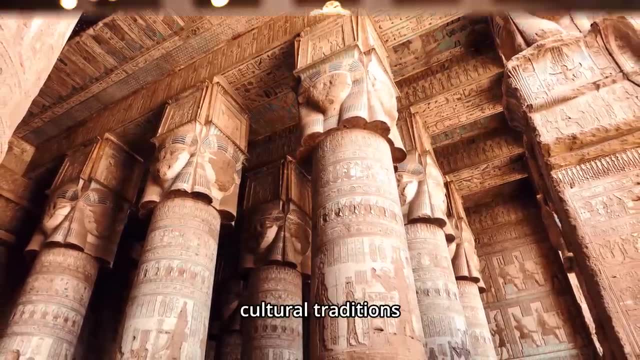 the wisdom of their Atlantean ancestors thrived, casting a timeless shadow upon the ever-evolving tapestry of human understanding. In the mosaic of our world's cultural traditions, the enigmatic whispers of Atlantis find resonance in the myths and legends of diverse societies. 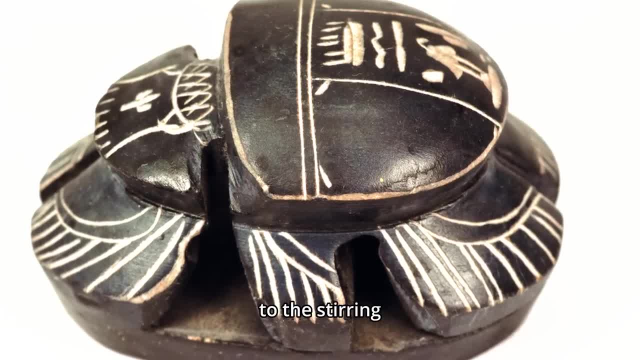 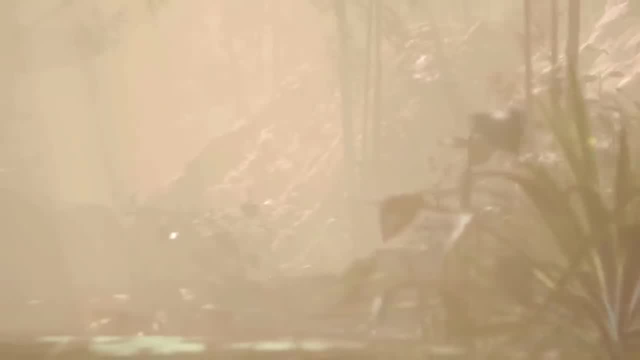 From the annals of Egyptian and Phoenician mythology to the stirring sagas of Mongolian nomads, the echoes of Atlantis transcend the confines of time and geography. Greek myths, rich with their own interpretations of this lost realm, stand as testament to its enduring allure. 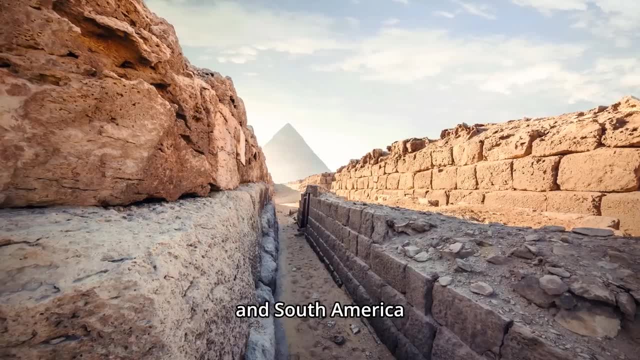 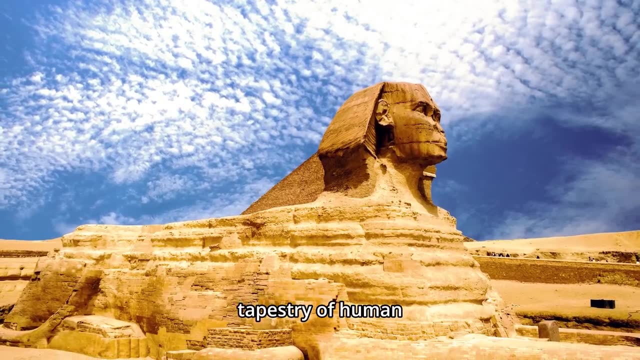 Even in the cherished tales of the indigenous peoples of North and South America, the enigmatic Atlantis weaves its enigmatic threads, uniting the world through the shared tapestry of human imagination and wonder, Deep within the collective memory of the Hopi Indians. 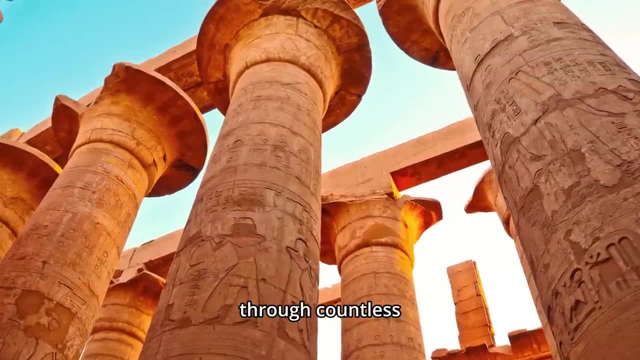 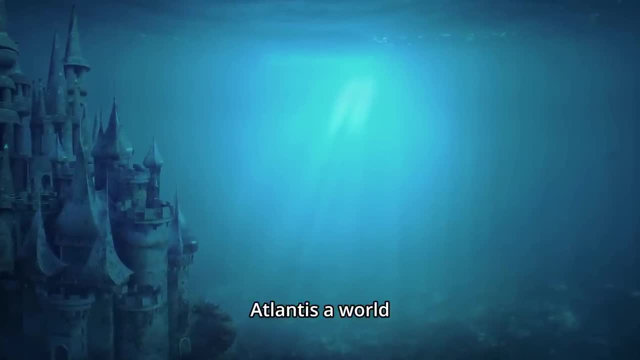 a sacred legend has been lovingly nurtured, passed down through countless generations, a beacon of wisdom shining through the ages. Their ancestral tale weaves a tapestry of Atlantis, a world teeming with a burgeoning population thriving amidst grand cities and mastery of advanced crafts. 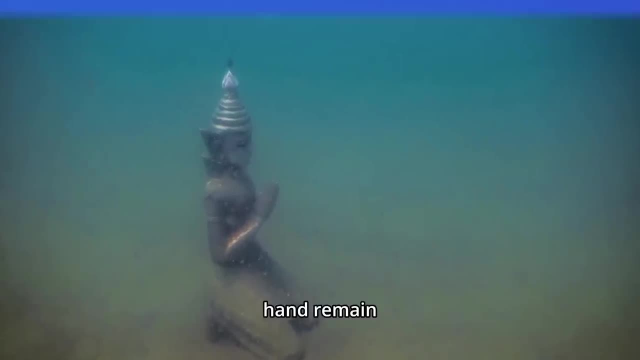 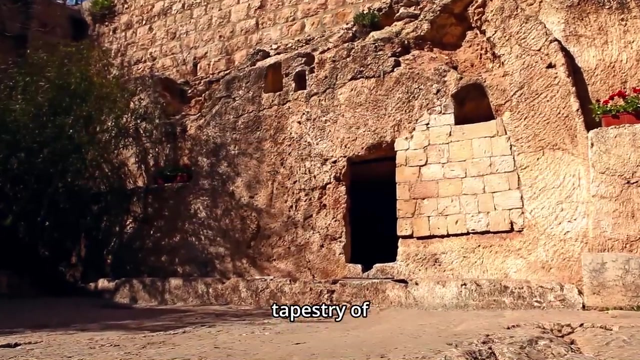 The echoes of this tale, whispered by time's gentle hand, remain eternally relevant, offering us a glimpse into the ancient marvels of human history. In the tapestry of their history, the people of Atlantis crafted a remarkable contrivance. 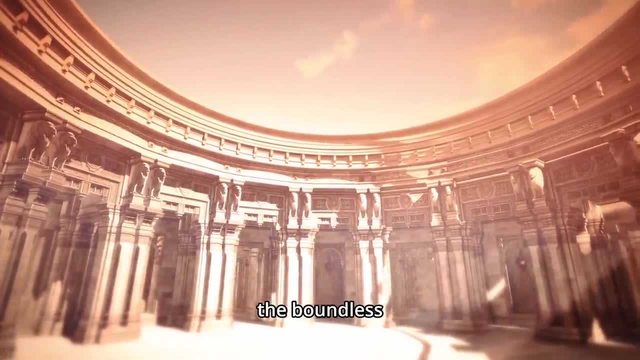 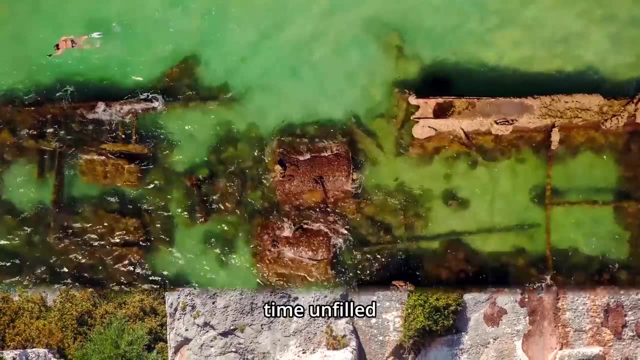 a shield of hide, soaring gracefully through the boundless skies, bearing passengers into the realm of aerial warfare. Yet as the pages of time unfurled, corruption wove its insidious tendrils, casting a shadow upon their world. In the final reckoning, 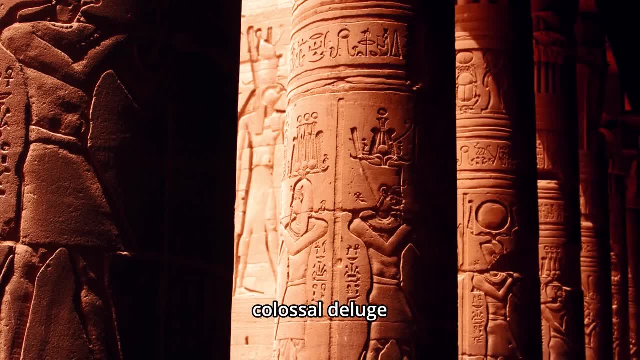 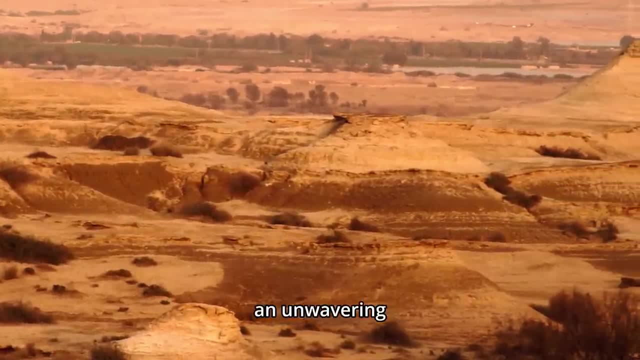 a cataclysm of unfathomable proportions descended a colossal deluge. its waves, towering higher than the mightiest mountains, inundated the land. Continents once solid and unwavering, fractured asunder and yielded to the relentless embrace of the insatiable seas. 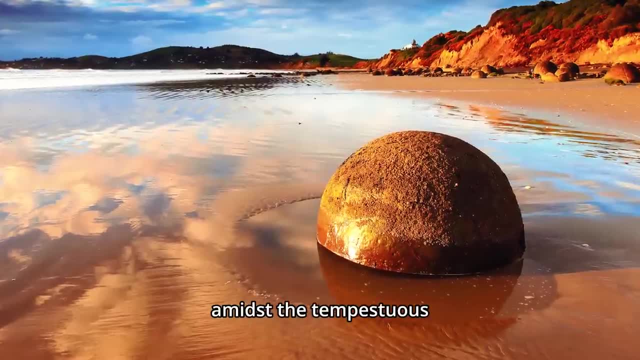 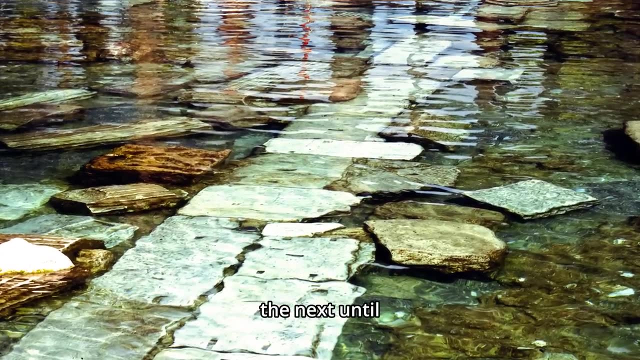 leaving a world forever transformed. Amidst the tempestuous cataclysm, a resilient few found salvation in boats embarking on a journey from one island to the next, until they at last alighted upon a vast continent. It was here, in the crucible of survival and renewal. 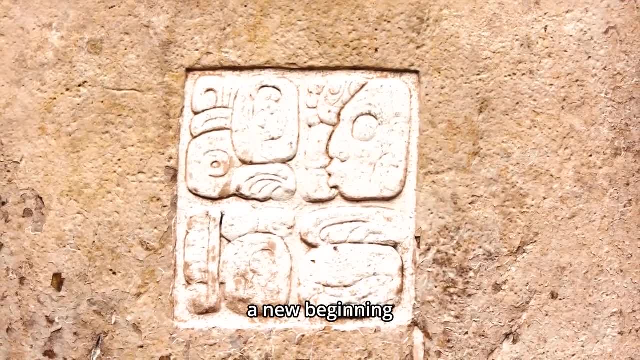 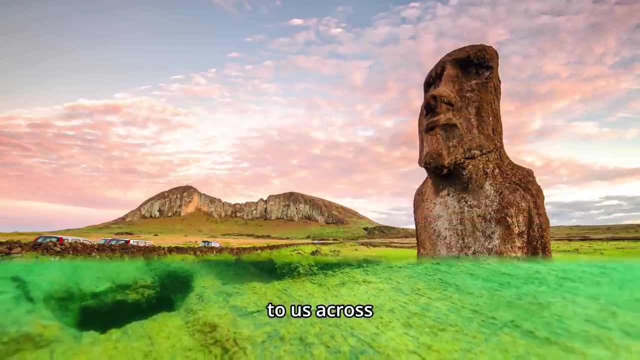 that the story of the Hopi people commenced a new beginning, born from the crucible of ancient Atlantis. Intriguingly, a mosaic of evidence beckons to us across the mists of time, suggesting that the Hopi, along with the Iroquois, 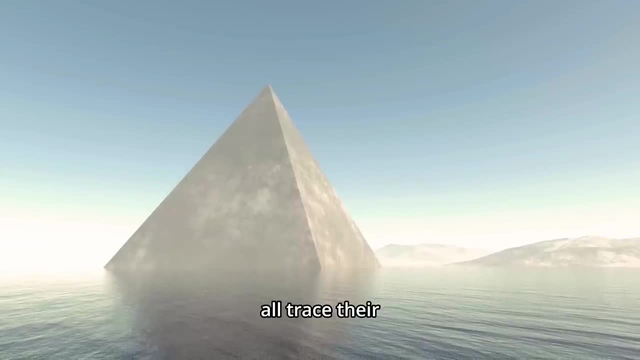 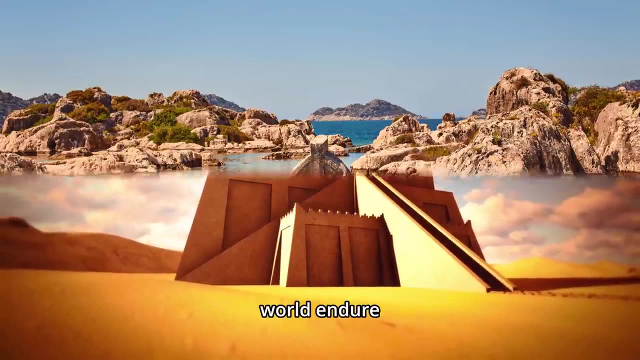 the mound builders and myriad other North American tribes all trace their lineage back to the Atlanteans. Through these indigenous societies, the echoes of an ancient and lost world endure whispering tales of resilience, heritage and the timeless connections that bind humanity. 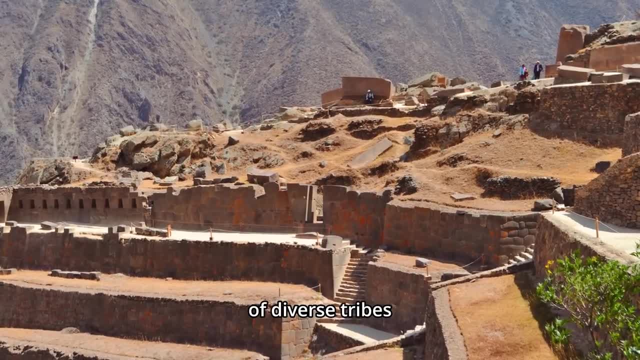 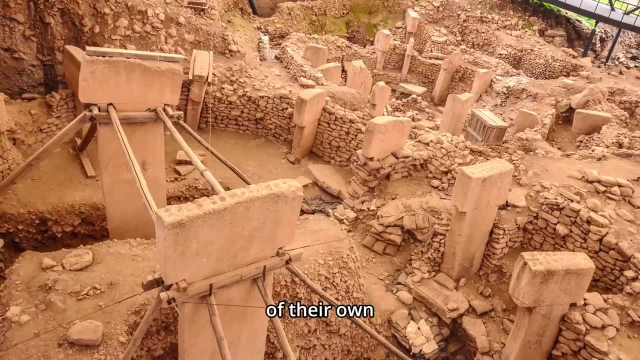 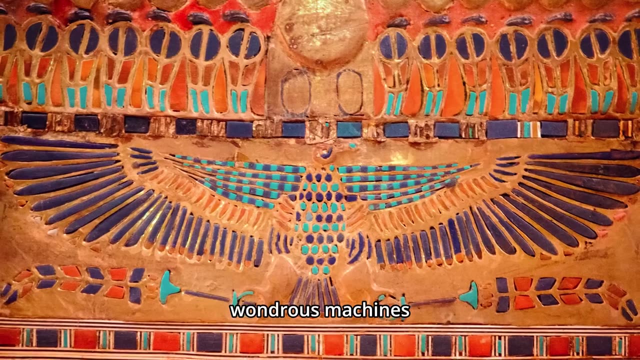 Across the tapestry of diverse tribes, a common refrain echoes through the ages, a tale of the great deluge that once swept across the earth and the genesis of their own ancestral lineage. These legends converge upon a land of unparalleled beauty, where wondrous machines and marvels of innovation stirred the imagination. 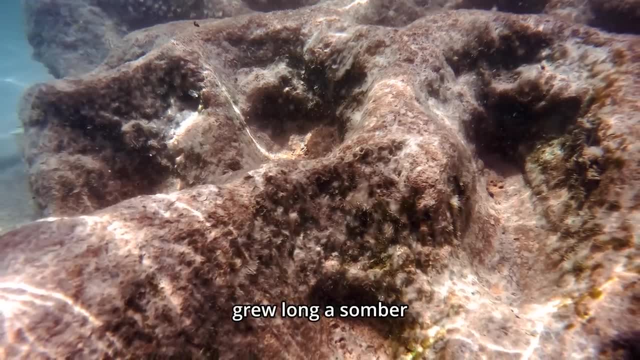 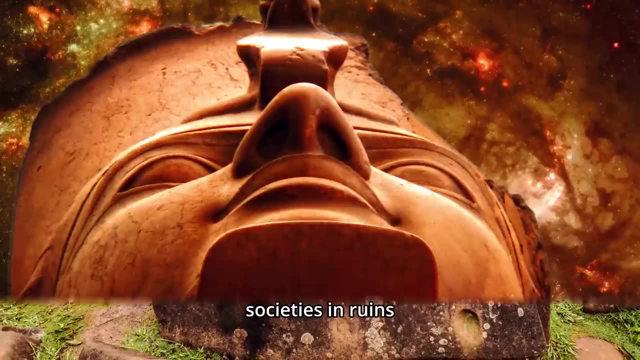 Yet, as the shadows of moral corruption grew long, a somber verdict was cast a reckoning: a cataclysmic purging that left the once thriving societies in ruins. In these shared narratives, humanity grapples with its own history. 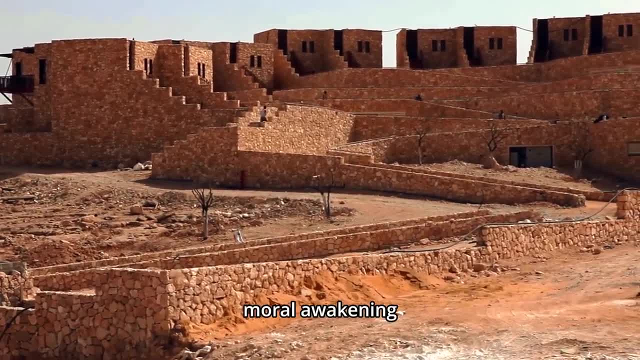 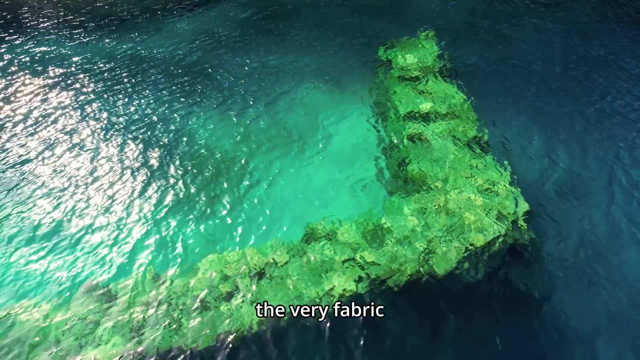 an intricate dance of light and shadow, innovation and moral awakening, resilience and renewal. One of the most intriguing threads in the tapestry of Atlantis is woven from the very fabric of archaeological and anthropological evidence. It's in these remnants of the past that we unearth the echoes of history. 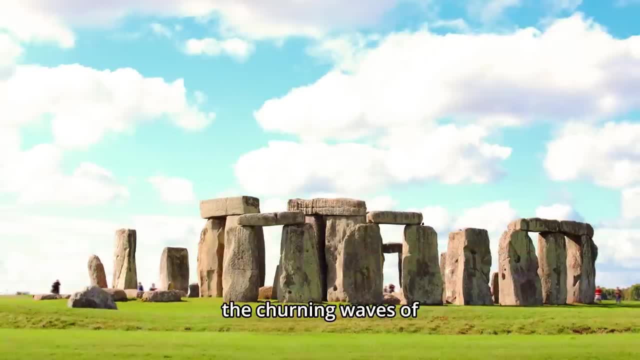 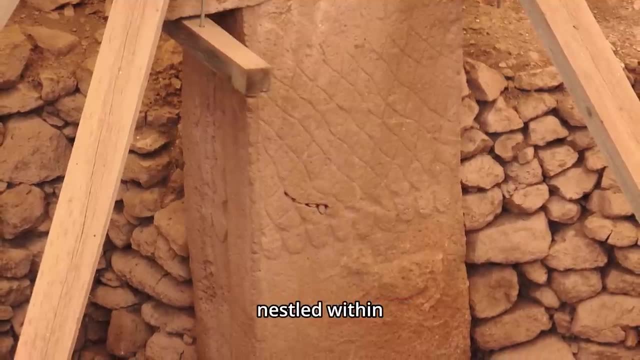 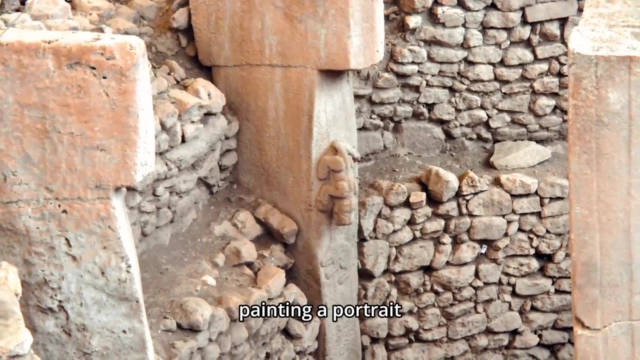 a profound resonance that transcends the churning waves of the Atlantic. Remarkably, we find striking similarities, like hidden treasures nestled within the annals of ancient cultures. These echoes transcend the boundaries of East and West, painting a portrait of interconnectedness that defies the limits of time and space. 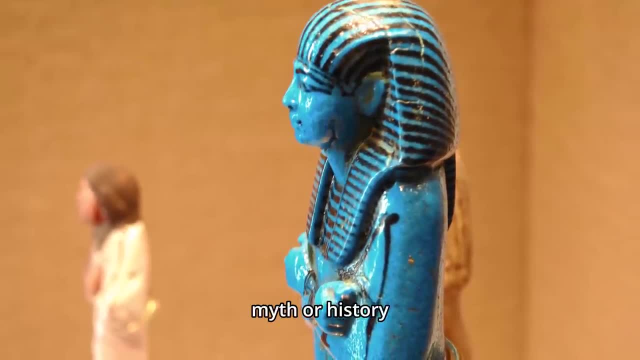 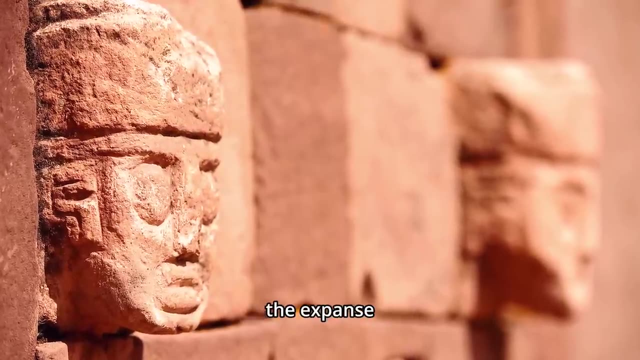 The legacy of Atlantis, whether shrouded in myth or history, leaves its indelible mark on the rich tapestry of our human story. Amid the labyrinth of history and across the expanse of continents, a compelling tapestry of shared connections emerges. 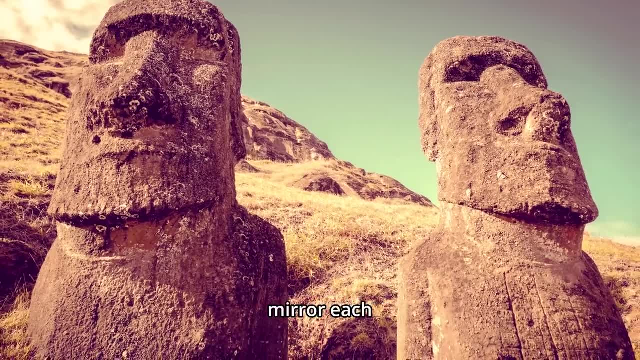 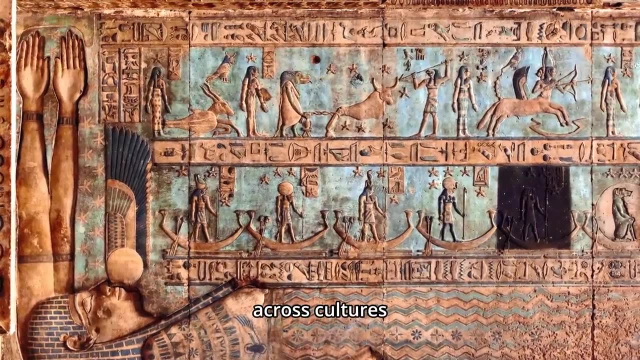 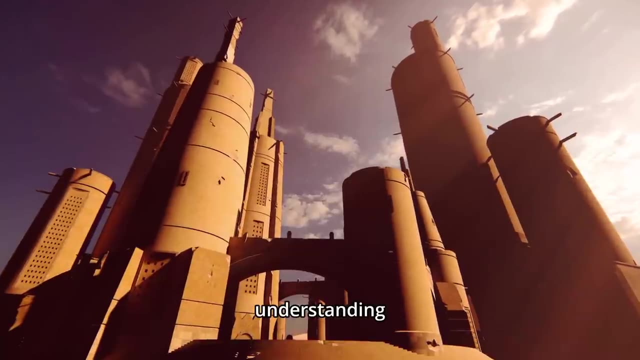 Creation. myths passed through the generations mirror each other, weaving a narrative of unity. The echo of a great flood resounds across cultures, a testament to shared ancestral memory. As we delve deeper, we uncover the footsteps of an advanced understanding of the cosmos. 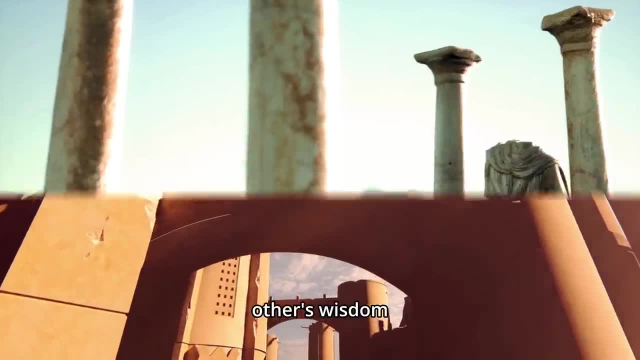 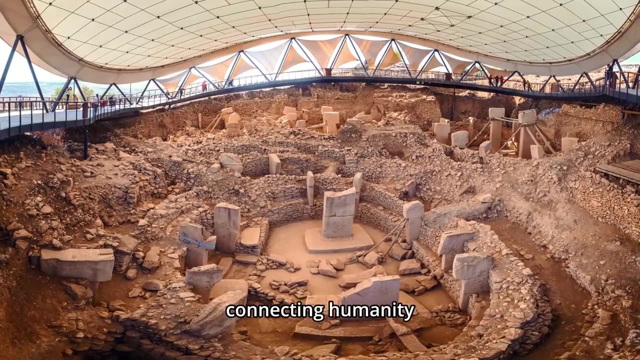 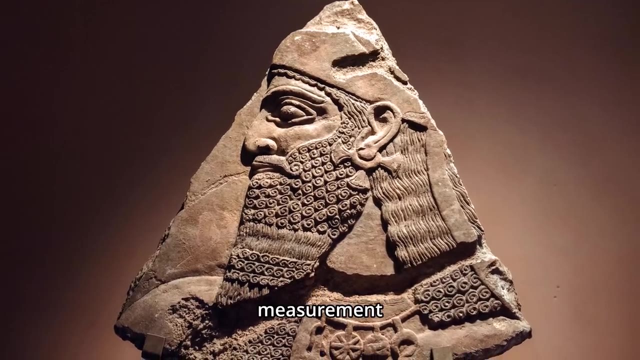 sophisticated astronomical alignments that mirror each other's wisdom. Knowledge of the 25,900-year procession of the equinoxes unfolds like a celestial thread connecting humanity through time Across shores and civilizations. we find an uncanny resonance in units of measurement with feet, fathoms, cubits and stadia echoing through the ages. 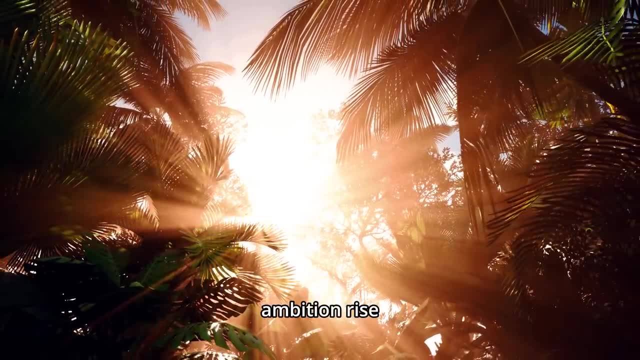 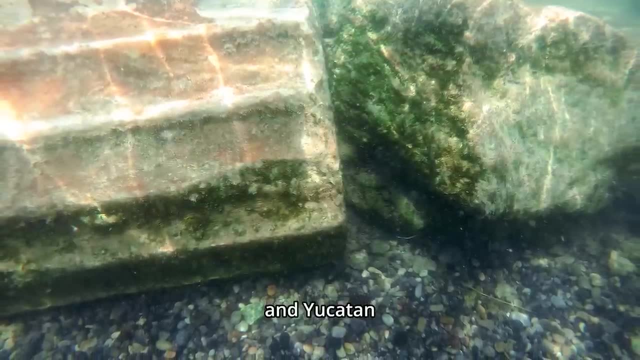 Step pyramids, symbols of ancient ambition, rise both in Central America and the Middle East, echoing the vision of humankind. In both Iberia and Yucatan, the vibrant tradition of ball games is played, a testament to shared practices and joys. 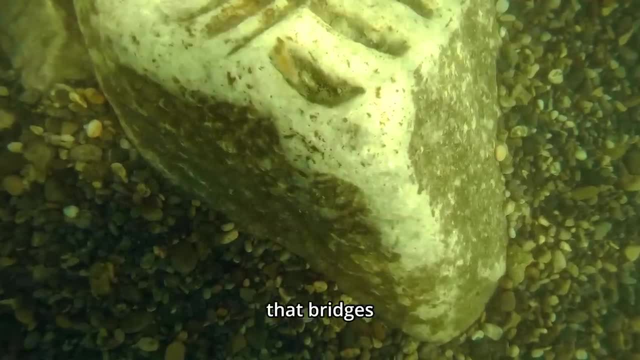 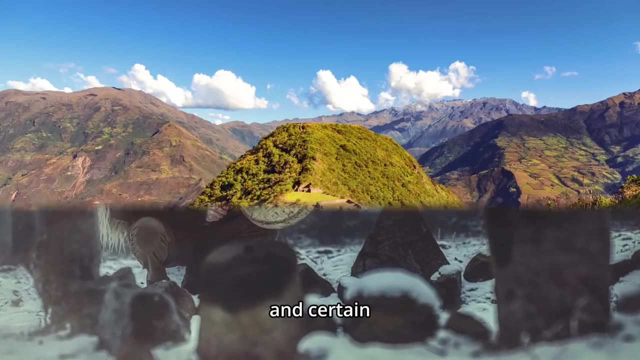 The art of embalming the dead speaks to an intimate knowledge that bridges cultures. Linguistic and phonetic echoes resonate as well with the languages of the Basque people and certain Central American cultures, sharing commonalities Even in physicality. the similarities are striking. 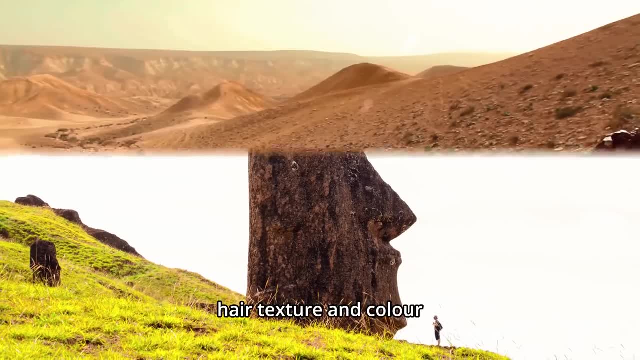 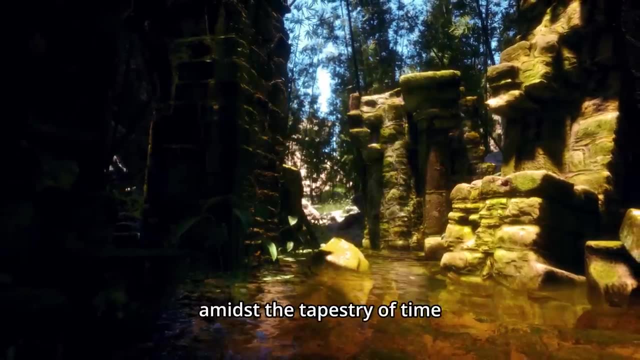 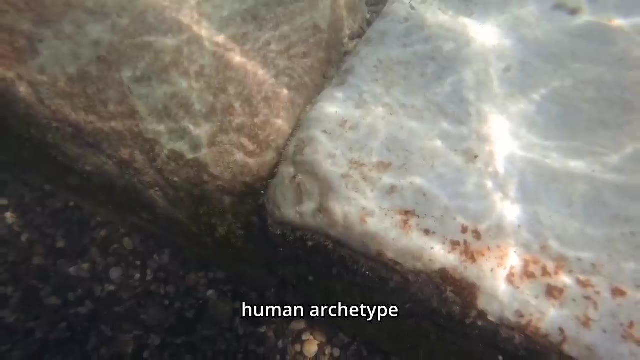 from skin color to facial features, hair texture and color, musculature and stature, painting a portrait of shared humanity across the globe. Amidst the tapestry of time, we find compelling anthropological and archaeological evidence pointing to the emergence of a more refined human archetype. 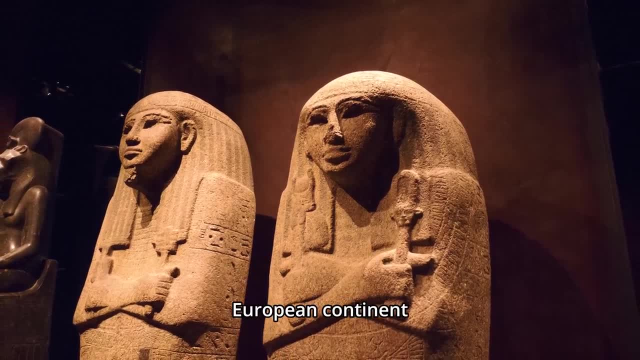 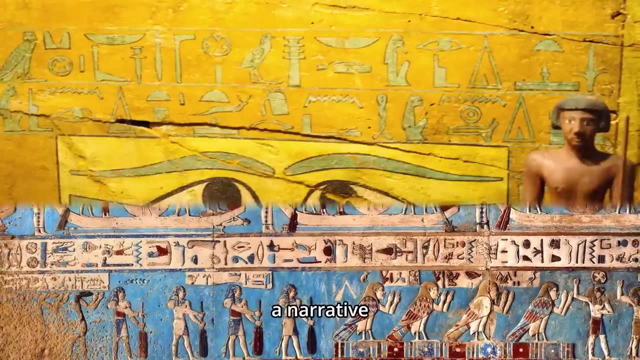 the Cro-Magnon Flourishing across the western expanse of the European continent. their presence graced the annals of history from at least 30,000 to 10,000 BC. Tradition weaves a narrative of migration, an east-to-west odyssey that unfolded gradually over millennia. 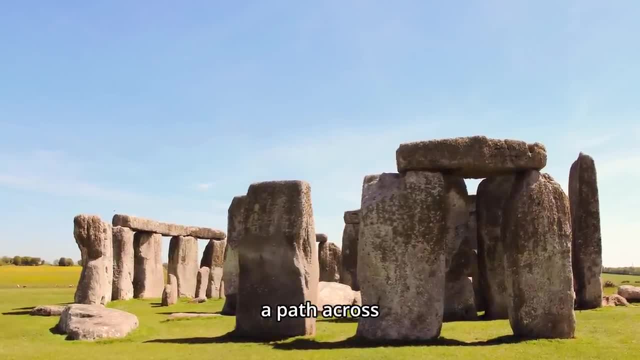 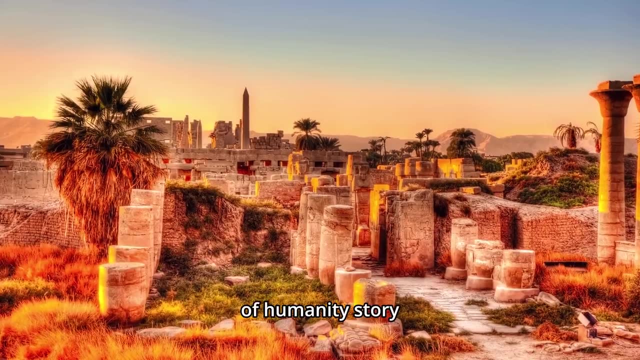 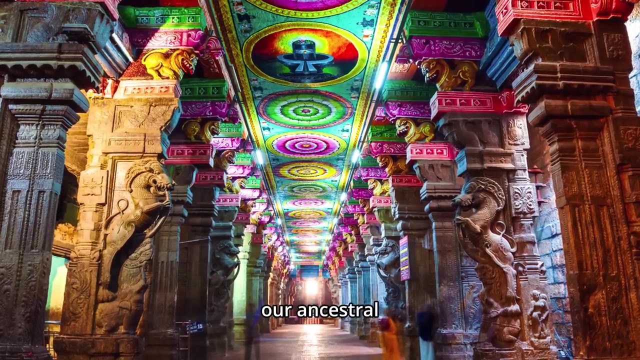 In this epic journey, the Cro-Magnon people forged a path across Europe, their evolving culture intersecting with the ebbing remnants of the Neanderthals. The evolution of humanity's story, marked by a dance of progress and adaptation, left a mark etched deep into the soil of our ancestral homeland. 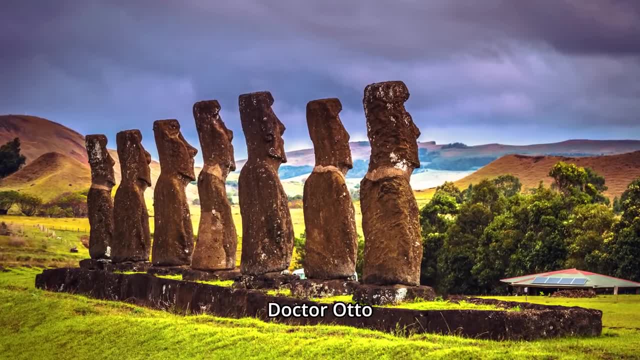 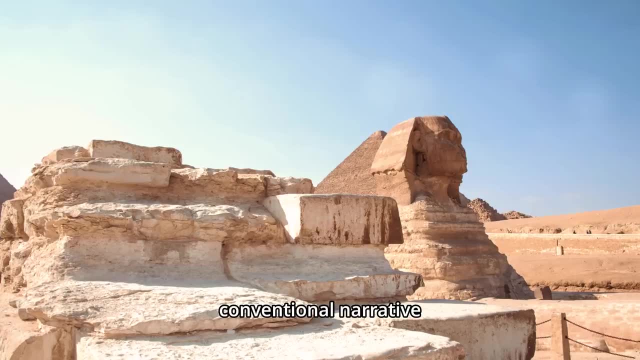 In the uncharted territories of research. luminaries like Dr Otto Muck present an alternative perspective. They propose a remarkable reversal of the conventional narrative, contending that the Cro-Magnon's migratory path led them from west to east with Atlantis as their origin. 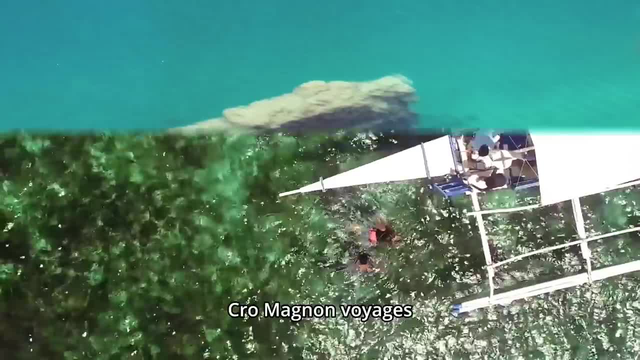 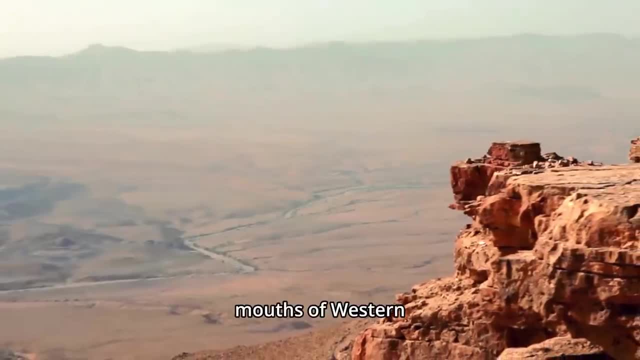 According to this theory, Cro-Magnon voyagers embarked on a bold maritime journey traversing the vast expanse of the Atlantic, the destination being the river mouths of Western Europe. From these coastal points, they ventured inland following the winding course of rivers. 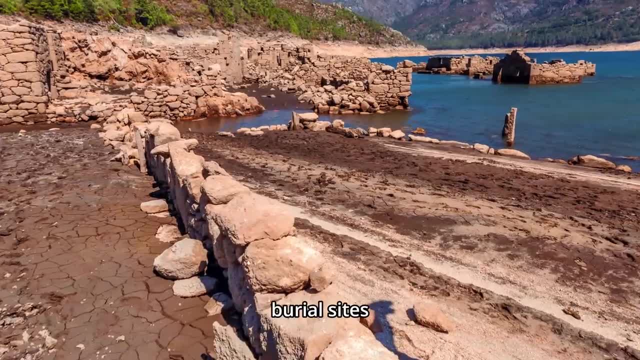 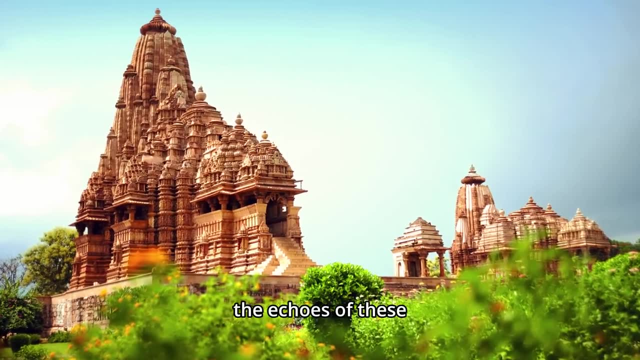 What sets their path apart are the distinct burial sites left behind by the Cro-Magnons, a stark departure from the Neanderthal traditions. In the echoes of these ancient graveyards, Dr Muck and like-minded researchers find clues to rewrite the narrative of our prehistoric past. 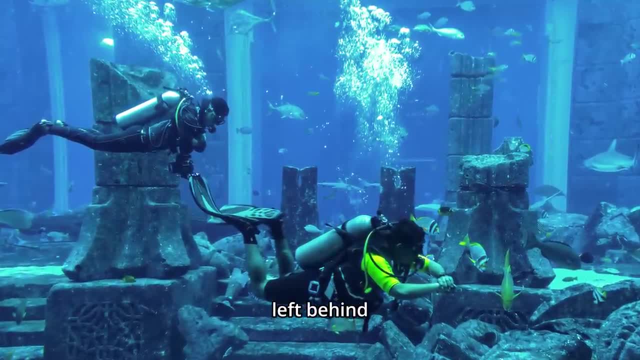 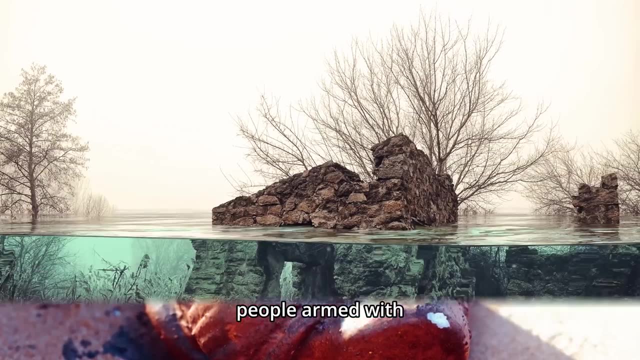 As we sift through the sands of time, the relics left behind by these ancient civilizations tell a tale of artistic brilliance and superior weapons. The Cro-Magnon people, armed with more advanced tools of war, likely exerted a formidable influence over the Neanderthals. 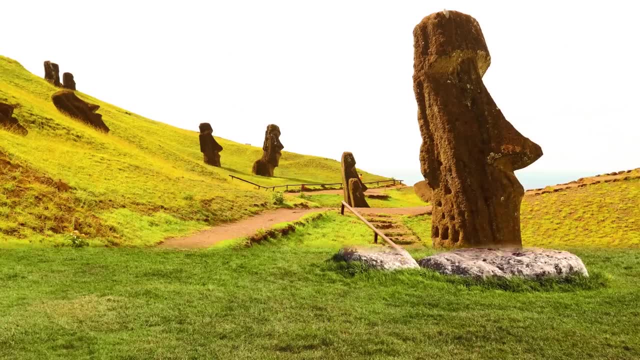 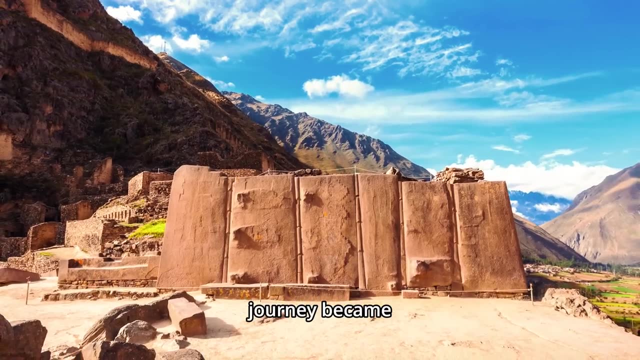 driving them back toward the sheltering embrace of alpine retreats. Intriguingly, the Testament of Excavations We Unearth emboldens the theory that the Cro-Magnons, in their westward journey, became the harbingers of cultural and technological progress. 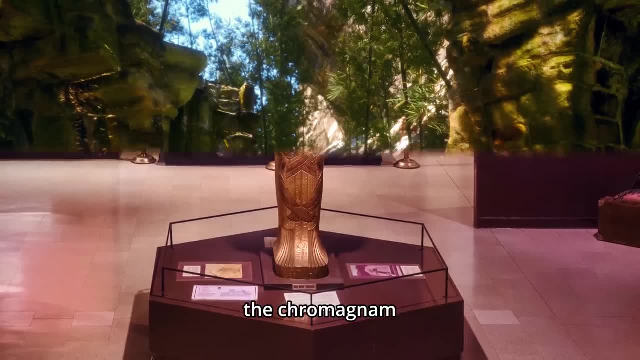 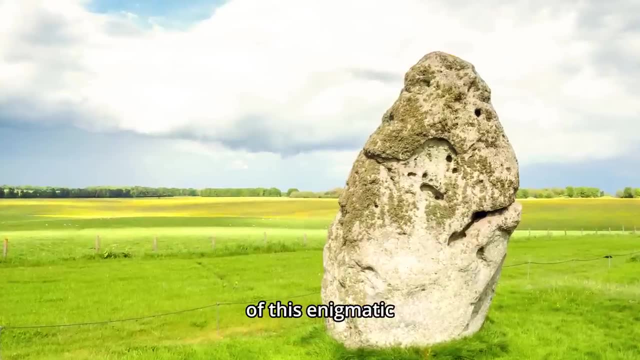 It is in these regions, rich with the finds of the Cro-Magnon people, that echoes of Plato's Atlantis resonate, reigniting the debate surrounding the origins of this enigmatic civilization. Clues etched into the soil of Western Europe hint at a fascinating tapestry of human migration. It appears that this ancient continent was graced by the footfalls of successive waves of Cro-Magnons, the pioneers of a grand odyssey that may have originated from the fabled Atlantis. These journeys might have taken the form of small, organized hunting expeditions. 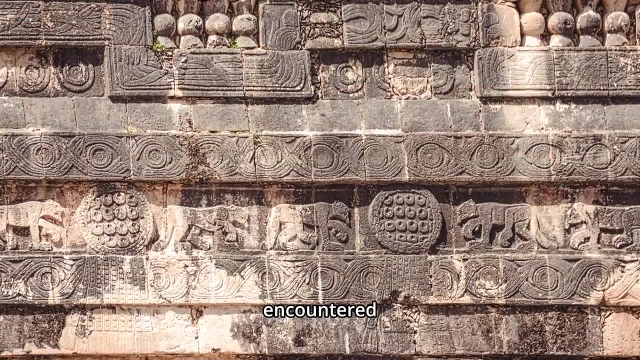 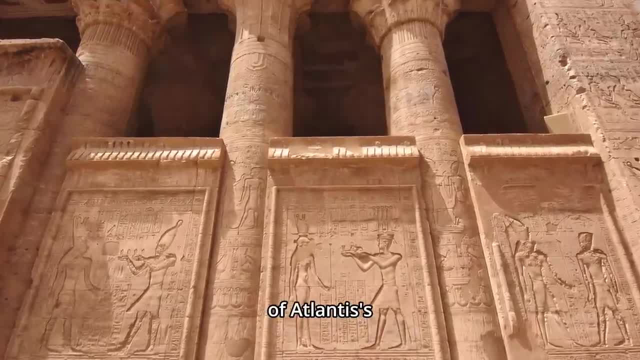 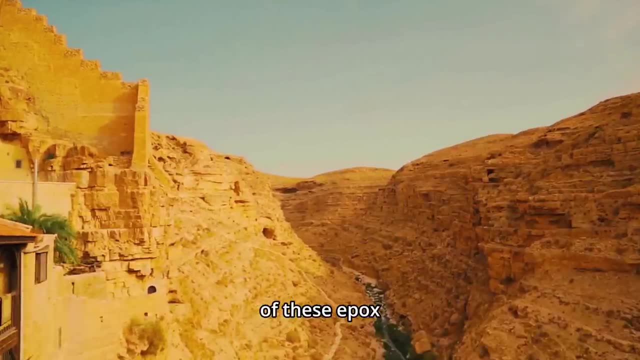 each leaving a mark on the landscape and culture they encountered. Remarkably, the colonization of Western Europe likely commenced before the somber chapter of Atlantis's submersion, during a transitional period marking the ebb and flow of ice ages. In the shifting tides of these epochs, humanity's spirit of adventure and exploration was kindled. 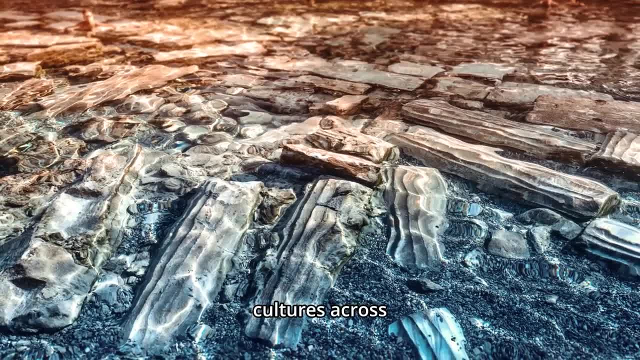 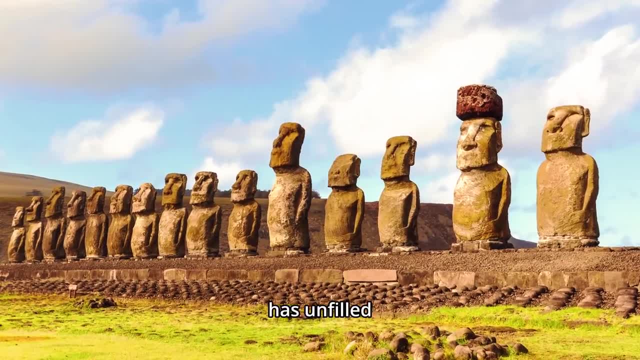 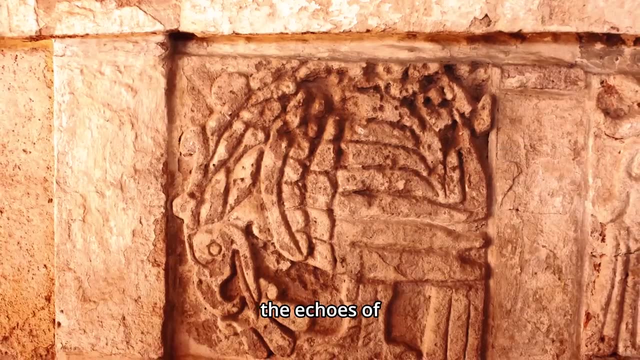 leading to the emergence of vibrant cultures across the European landscape. In the enigmatic corridors of research, a curious revelation has unfurled a remarkable kinship in physical attributes between the Cro-Magnons and the indigenous tribes of North America. The echoes of their existence resonate in skeletal type and the hue of their skin. 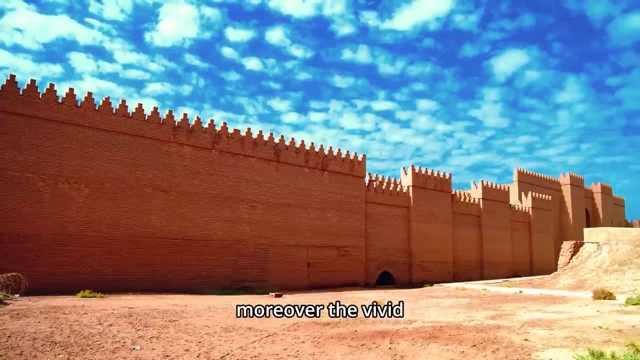 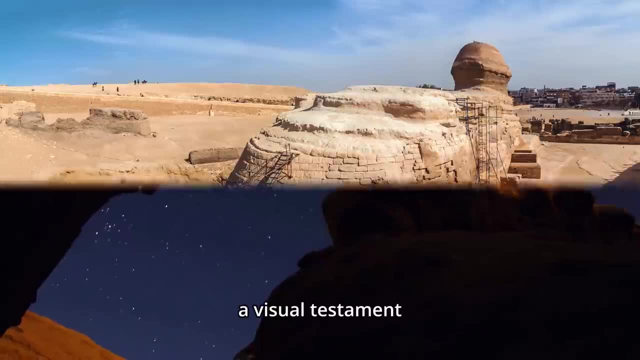 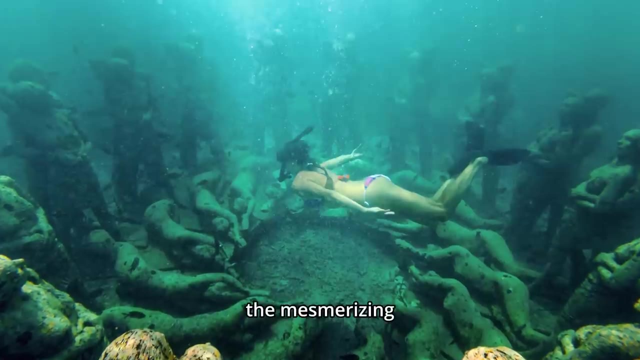 forging a connection that transcends time and space. Moreover, the vivid cave paintings attributed to the Cro-Magnon people portray them as red-skinned individuals, a visual testament to their unique identity. As we stand on the precipice of discovery, we can't help but be drawn to the mesmerizing link that binds these ancient artists from east to west. 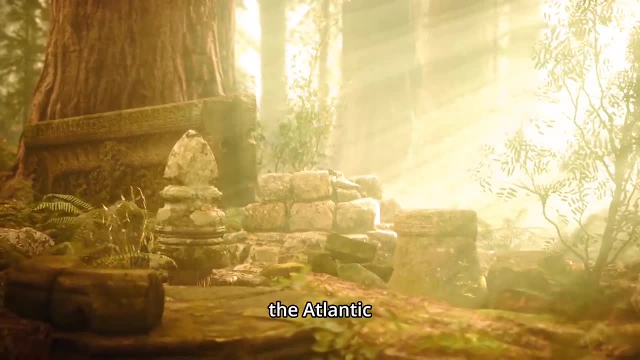 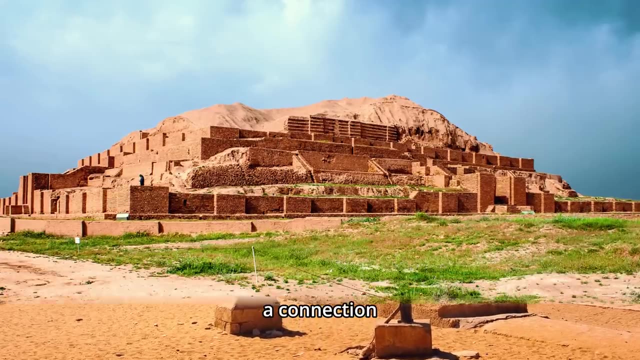 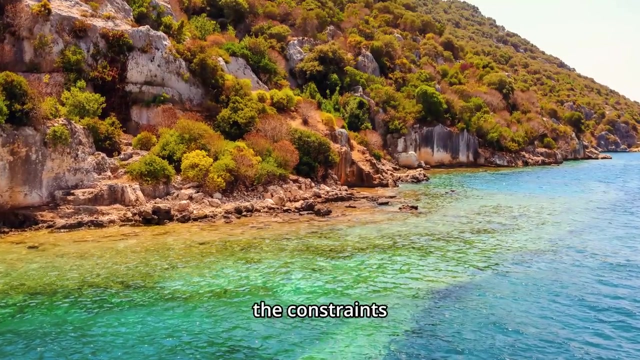 The cave paintings on both sides of the Atlantic share an essential kinship, reflecting the characteristics of the North American Indian races. This is a connection that beckons us to explore the enduring mysteries of human history, stretching across the boundless seas and defying the constraints of oceans and continents. 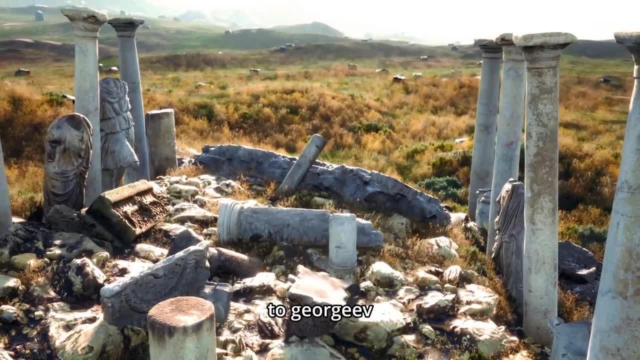 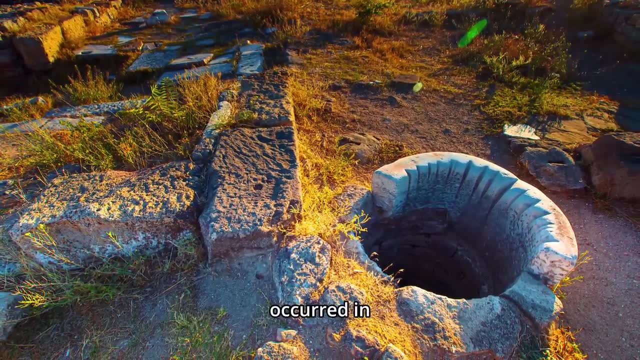 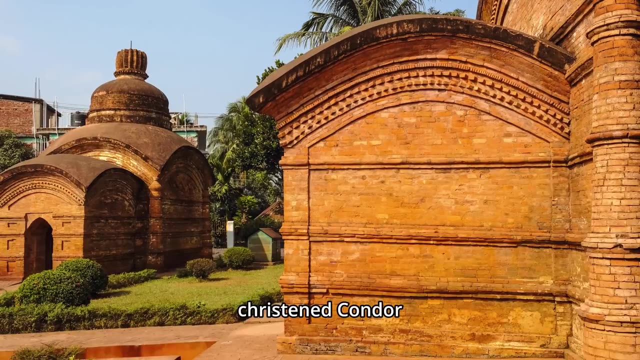 In the annals of our planet's history, according to Gurdjieff, a saga of calamities unfolds across the tapestry of time. The first great catastrophe occurred in the infancy of the Earth. a cosmic dance of destruction, A celestial visitor, a comet, christened Condor by his account, descended upon our young world with cataclysmic force. 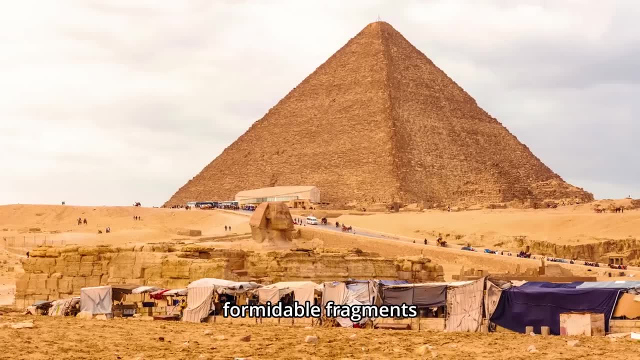 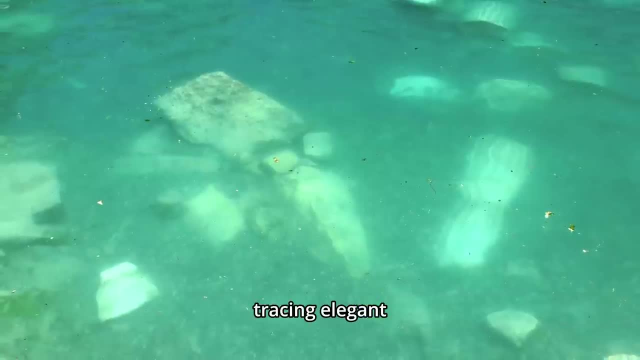 In the violent collision, the Earth gave birth to two formidable fragments flung into the cosmos. With time, these celestial orphans found their own path, tracing elegant elliptical orbits around our planetary cradle, carving an enduring tale of cosmic destiny. 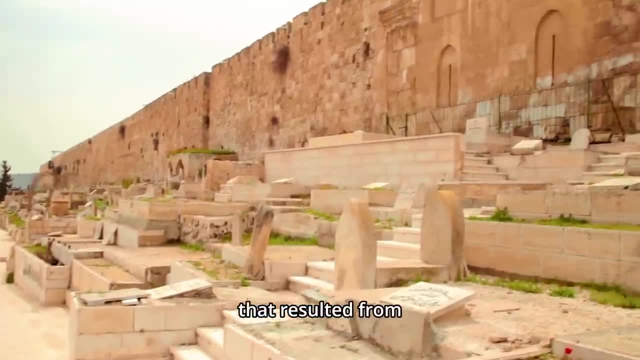 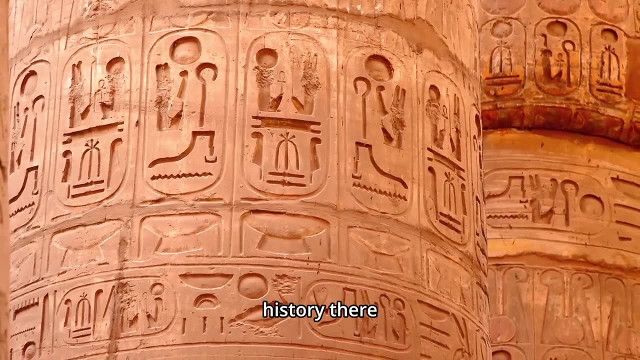 In this celestial ballet, the grander fragment that resulted from the collision has graced the night sky for eons, known to us as the Moon. Yet in the shadow of history, there exists a lesser-known figure in this cosmic drama: Anulios, a smaller body born of the same celestial event. 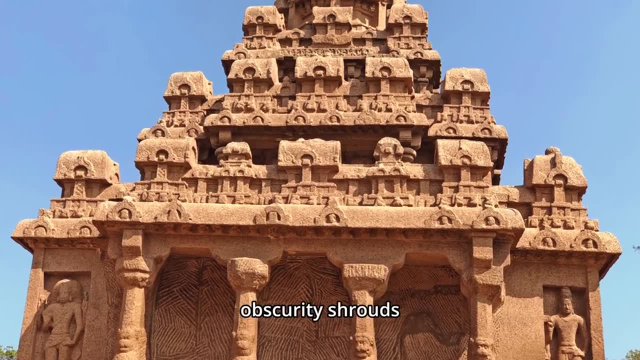 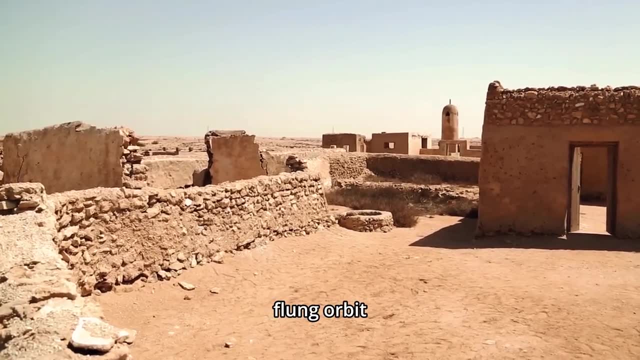 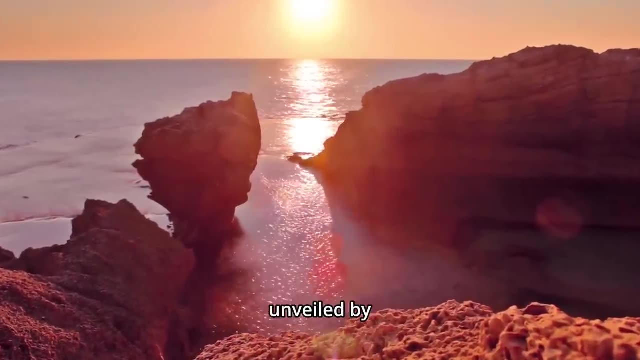 Alas, the veil of obscurity shrouds Anulios from the awareness of contemporary three-brained beings. Its diminutive size and its far-flung orbit conspire to render it virtually invisible to our mortal eyes. a hidden gem in the cosmic tapestry waiting to be unveiled by the seekers of knowledge. 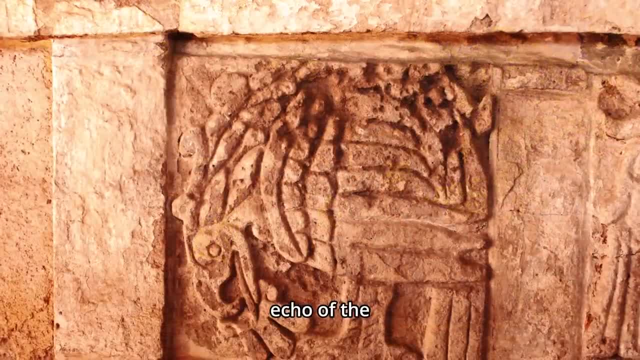 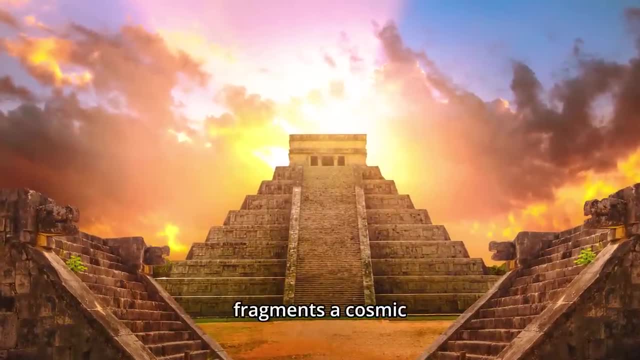 The second great calamity, it seems, was an echo of the cosmic disharmony sown by the first cataclysm. In the aftermath of the separation of two significant fragments, a cosmic center of gravity found itself suspended in an unfamiliar equilibrium. 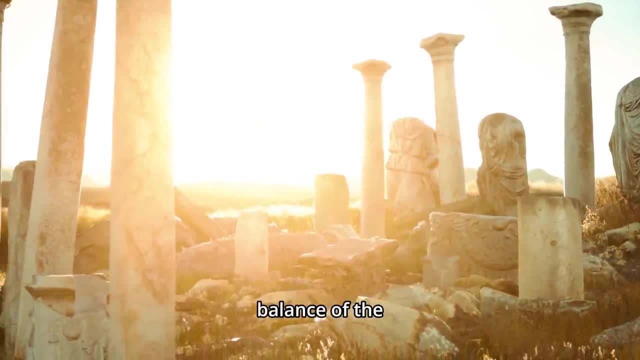 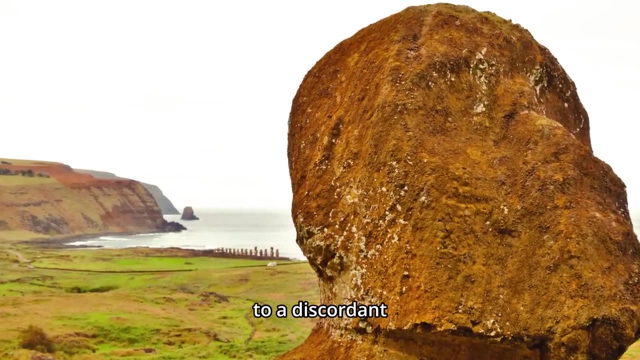 This newfound cosmic rhythm was out of sync with the inherent balance of the Earth, leaving the planet in a state of upheaval For a time. this terrestrial sphere danced to a discordant cosmic tune, manifesting as internal turmoil and substantial shifts upon its surface. 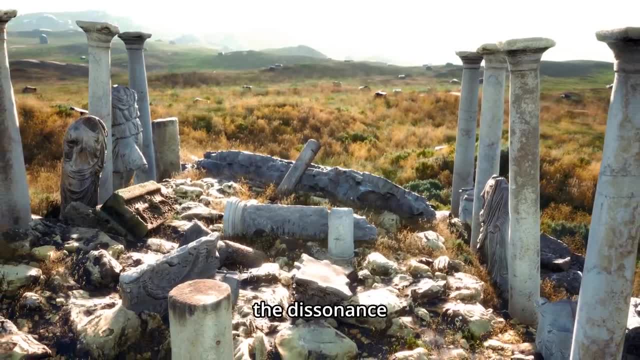 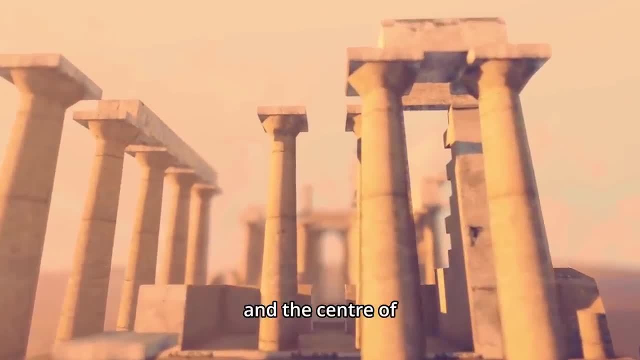 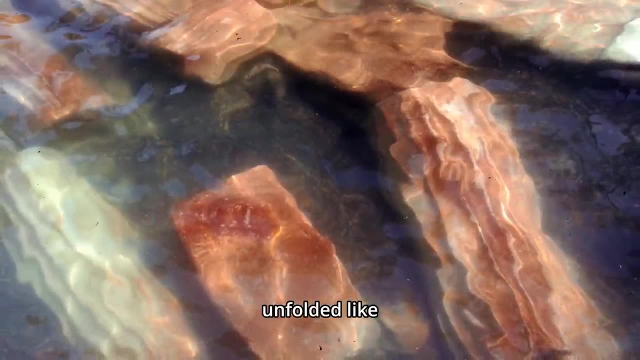 This period of unrest persisted, leading to the dissonance created by the initial catastrophe. It was only when the cosmic forces found the true equilibrium and the center of gravity of the Earth aligned itself in its rightful place that the second great catastrophe unfolded, like a cosmic crescendo in the grand symphony of our planet's history. 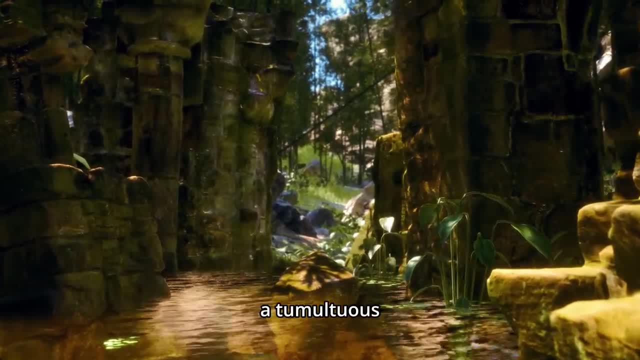 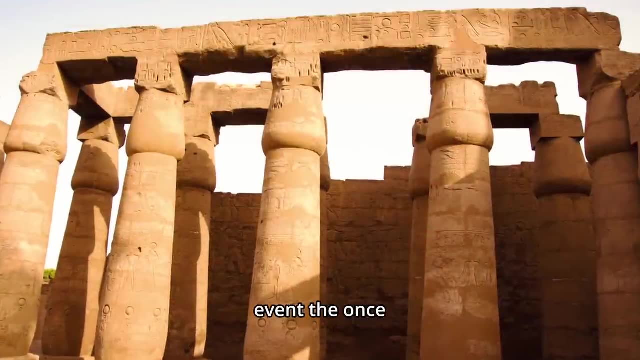 The second transopalnean perturbation unfolded, with a tumultuous display of cosmic might, shaking the very foundations of our world. In the throes of this titanic event, the once great continent of Atlantis succumbed to the relentless Earth tremors. 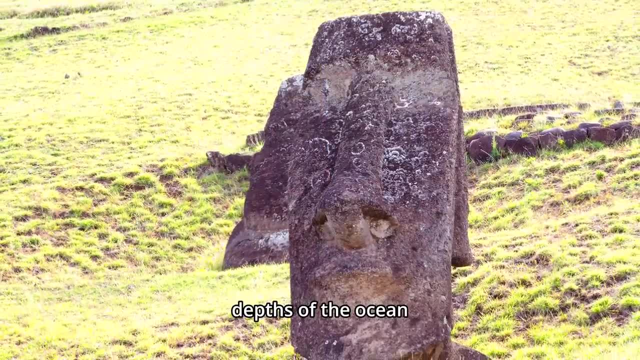 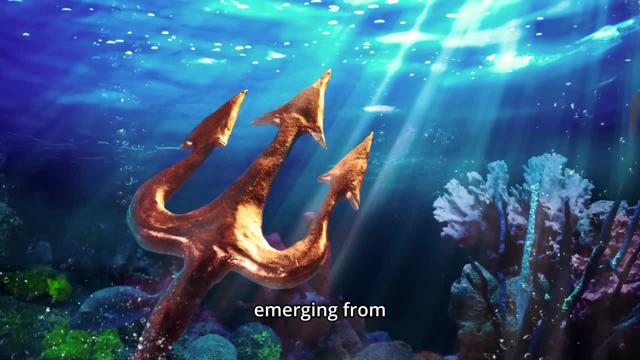 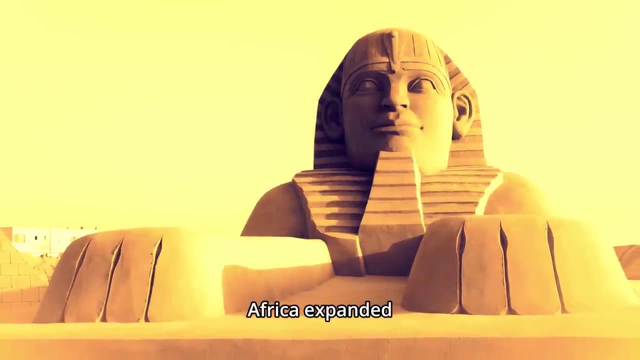 its grandeur, swallowed by the unforgiving depths of the ocean. Yet even amidst this colossal destruction, new realms arose from the heart of the Earth, emerging from the watery abyss. As a result of this profound upheaval, the continent we now know as Africa expanded significantly. 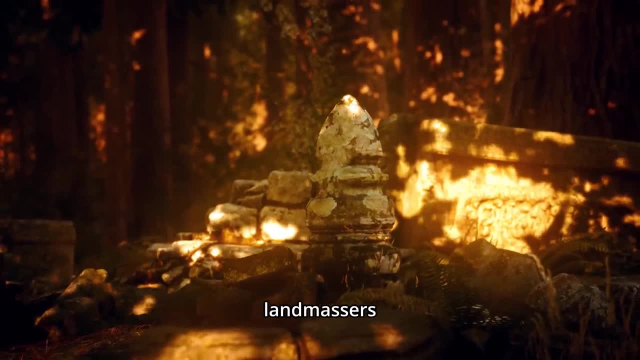 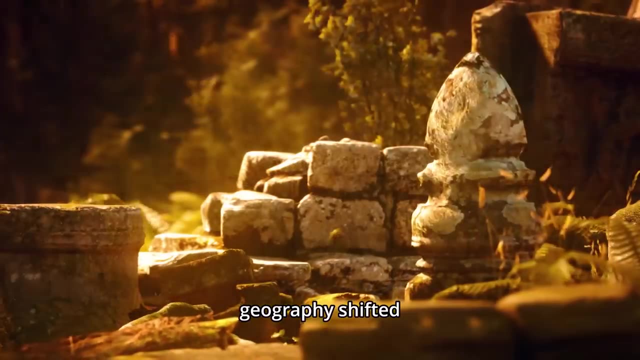 its territory, stretching to encompass the newly created landmasses. In the grand reshuffling of Earth's landscapes, the threads of history were woven anew as the planet's geography shifted and redefined itself In the wake of the tumultuous second terrestrial catastrophe. 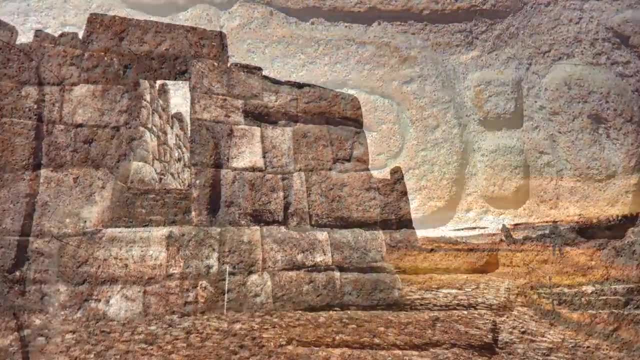 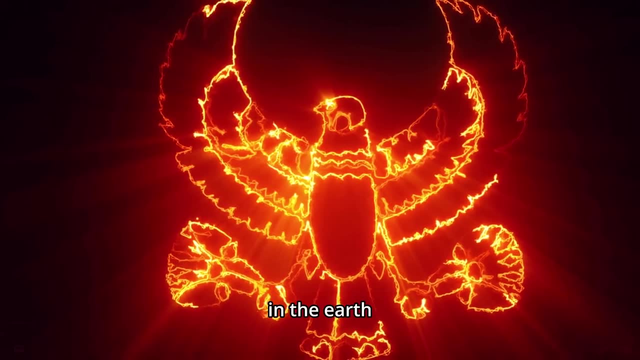 the world as we knew it bore the weight of profound transformations. Several regions of the once vast continent of Asia, under the tumultuous duress of these events, delved within the Earth, their history buried in the annals of time. Yet from the watery depths, new landmasses emerged. 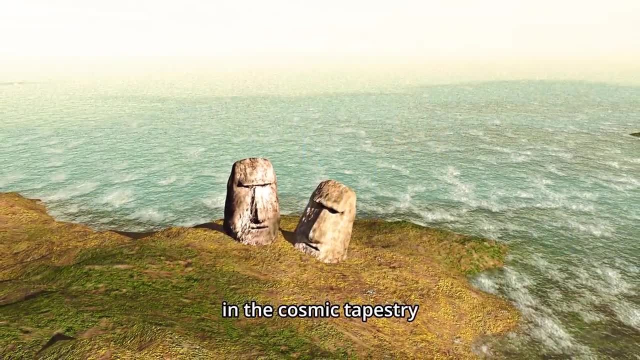 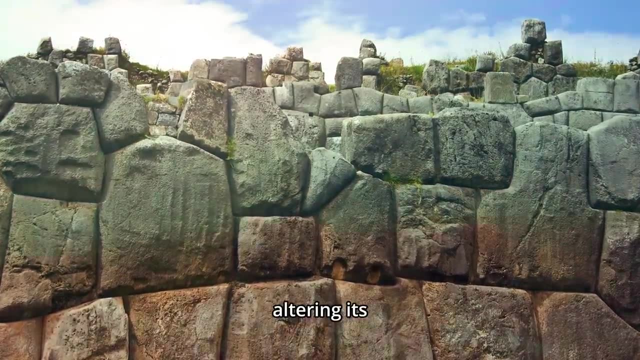 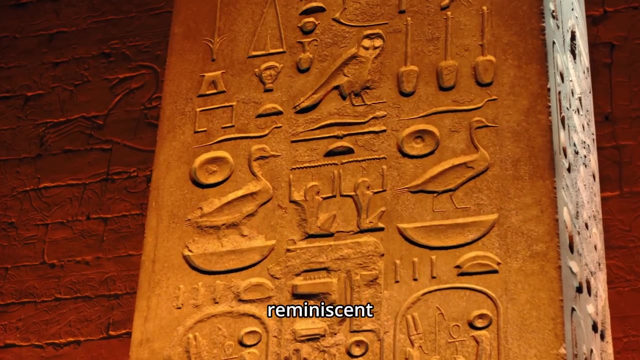 like newborn stars in the cosmic tapestry, These fledgling terraformers, in their tender embrace, fused with the continent of Asia, forever altering its identity In the grand theatre of terrestrial evolution, Asia shed its former shape and dimensions, reminiscent of the great continent of Atlantis that had once reigned as a celestial jewel. 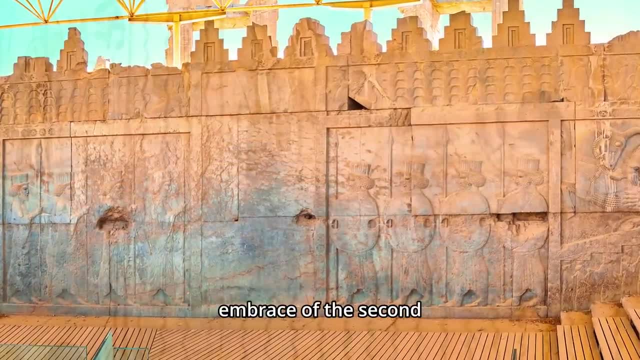 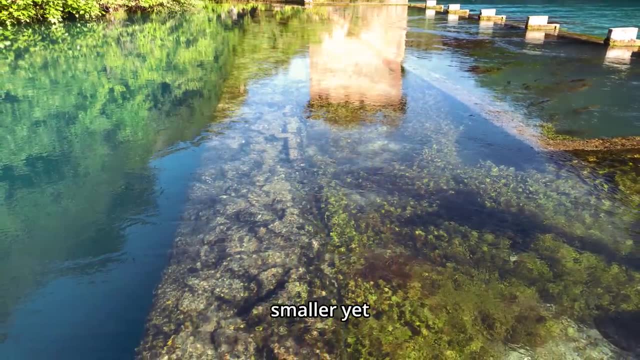 upon our planet's surface before the cataclysmic embrace of the second terrestrial catastrophe. Within the tapestry of our planet's history, Gurdjieff unveils a series of smaller yet significant catastrophes, each etching its own chapter in the cosmic narrative. 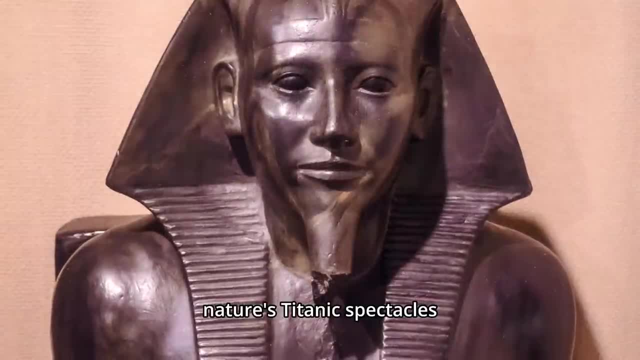 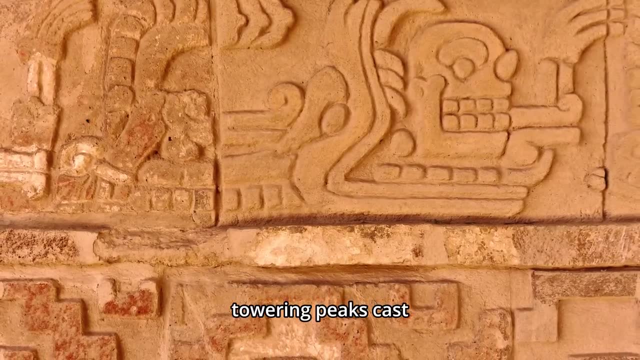 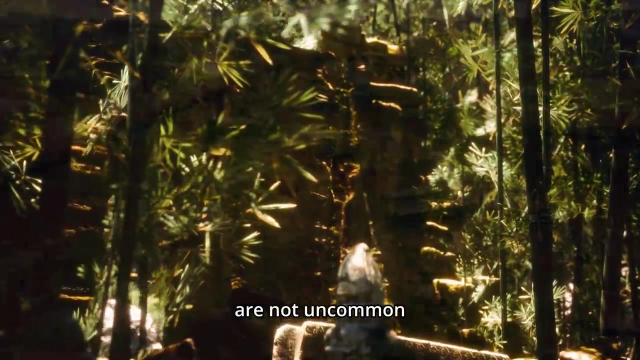 Among these disruptions are the powerful earthquakes, nature's titanic spectacles resulting from the burgeoning heights of newly formed mountain ranges. These towering peaks cast their profound influence upon the Earth's delicate atmosphere. While planetary tremors and earthquakes are not uncommon, many of the seismic disturbances that have resonated through our planet's crust 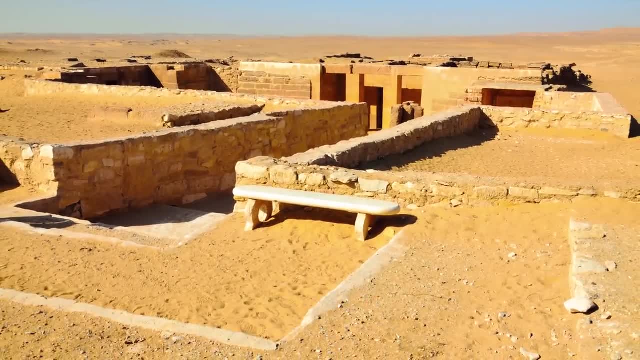 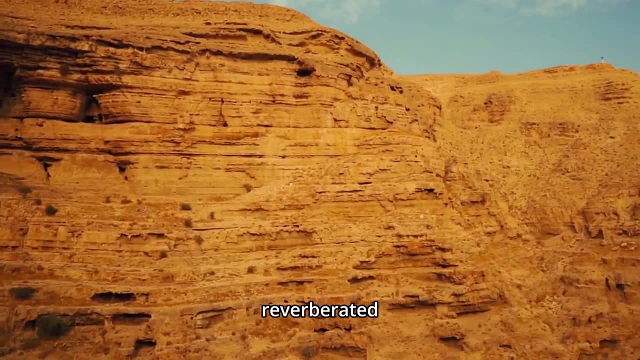 are attributed to the resonance of interplanetary disharmonies. These cosmic perturbations, born from the shadows of the two great trans-Apollonian cataclysms, have reverberated through the Earth's core. Yet, as Gurdjieff warns, 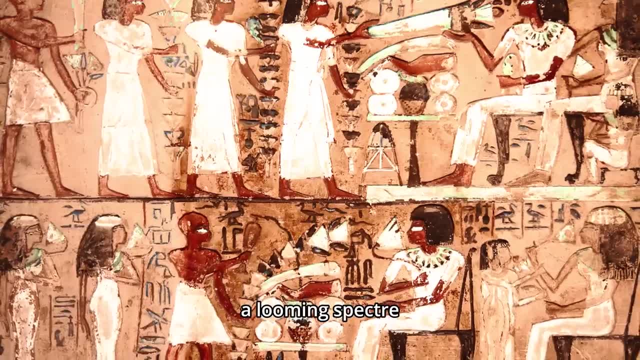 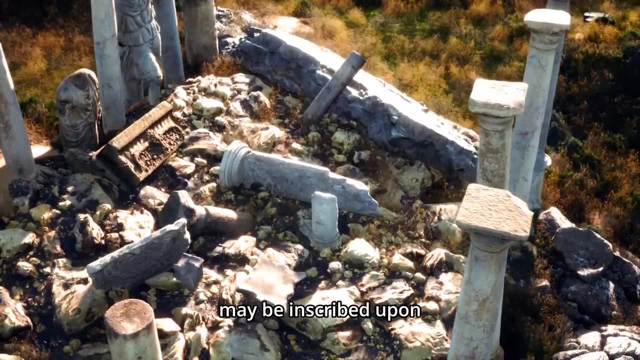 the abnormal growth of the Tibetan mountains presents a looming spectre. If this unrelenting ascent persists, a catastrophic event of unparalleled cosmic magnitude may be inscribed upon the celestial calendar, foretelling a grand cosmic transformation awaiting us in the folds of time. 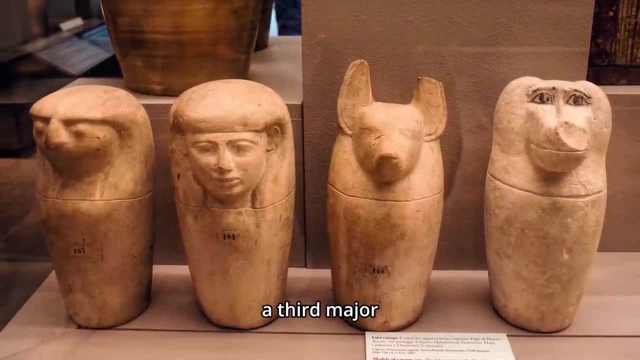 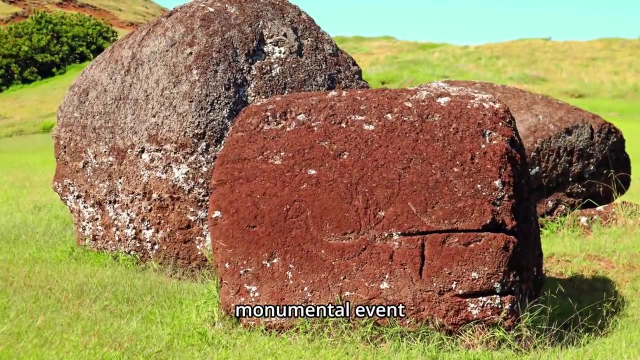 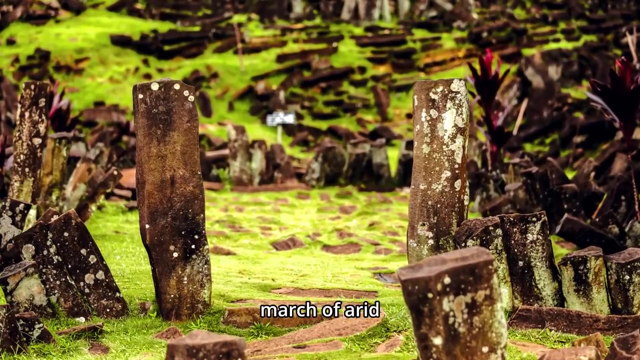 In the intricate tale of Earth's history, a third major catastrophe unfolded, one that would forever reshape the contours of our planet. During this monumental event, vast stretches of fertile lands were swallowed by the relentless advance of the sands. This relentless march of arid desolation gave birth to what we now know as the Gobi Desert. 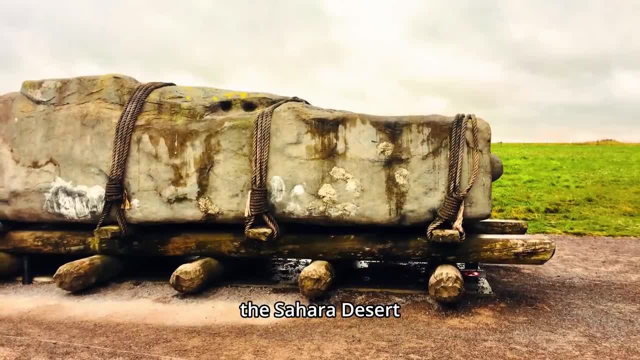 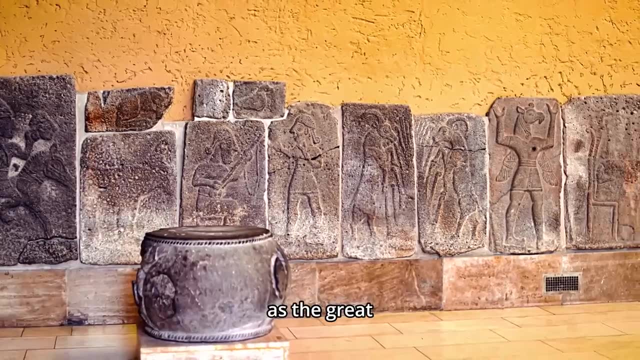 a sprawling sea of dunes and, at a later date, the Sahara Desert with its vast scorching expanse. This tumultuous era, often referred to as the Great Transmigration of Races, was a time of profound upheaval. 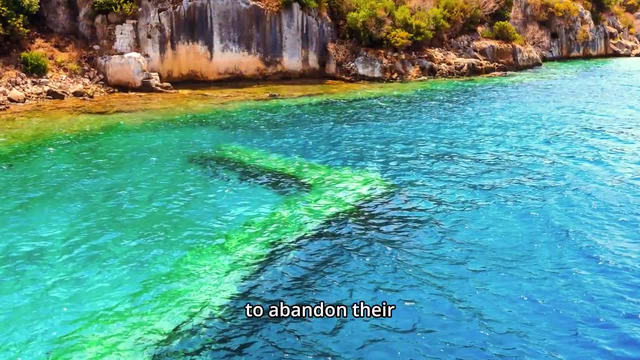 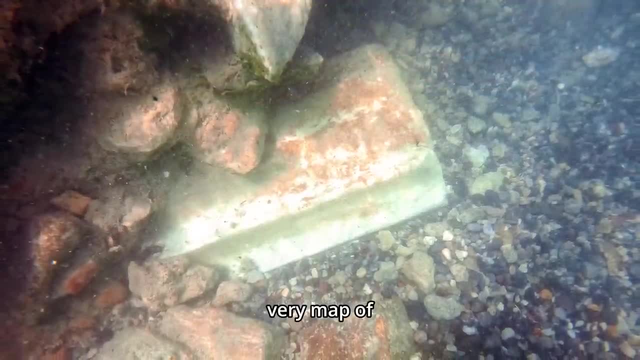 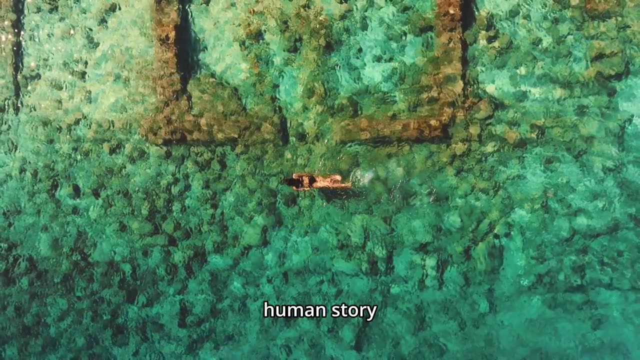 Inhabitants of these once fertile regions were compelled to abandon their ancestral homes, embarking on forced journeys of migration. It was a chapter in which the very map of human existence was redrawn, as cultures dispersed and new horizons beckoned, making a seismic shift in the human story. 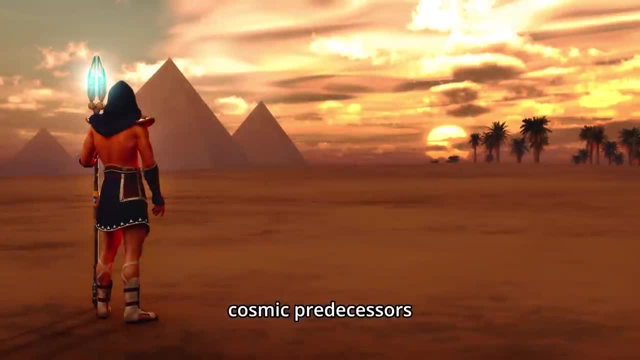 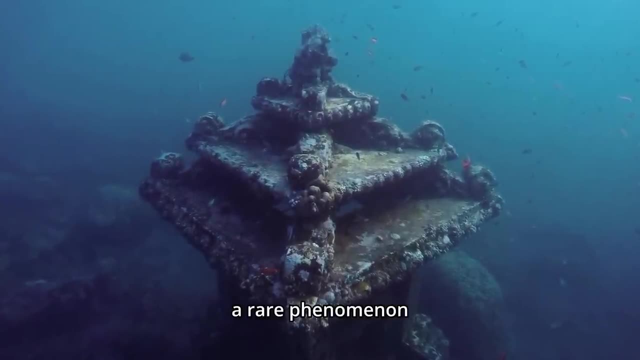 The third calamity, in contrast to its grand cosmic predecessors, bore a local imprint, a tale etched on a more intimate scale. This chapter unfurled, due to a rare phenomenon, a tempestuous dance of what scientists term accelerated displacements of the parts of the atmosphere. 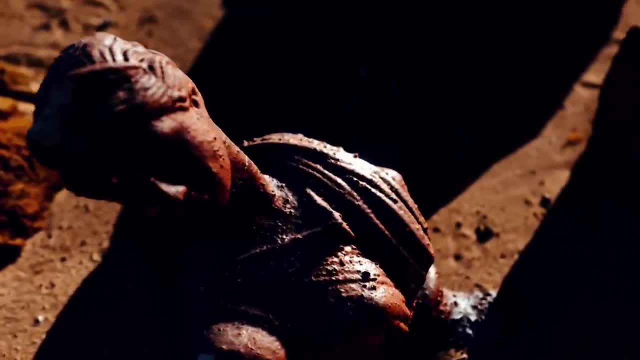 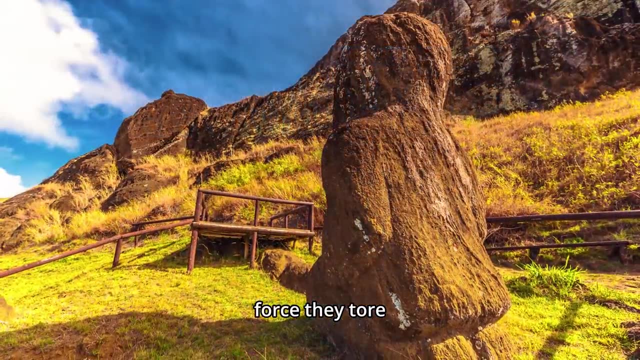 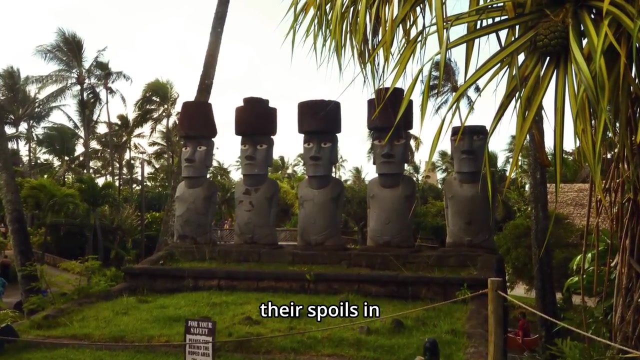 or in simpler terms, great winds of unprecedented power. With a fury unmatched, these exceptional winds set in motion a relentless and relentless force. They tore through the land's elevated sturdy terra firma parts, eroding their proud stature, and deposited their spoils in the hollows and depressions below. 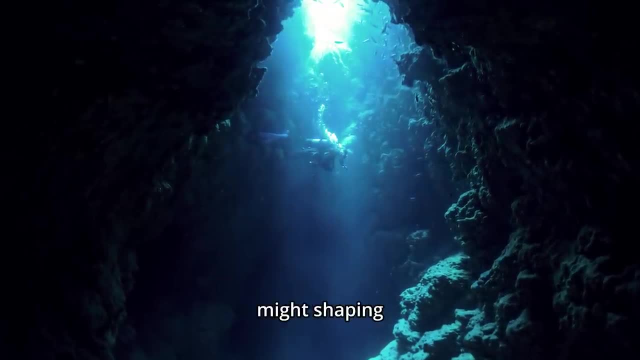 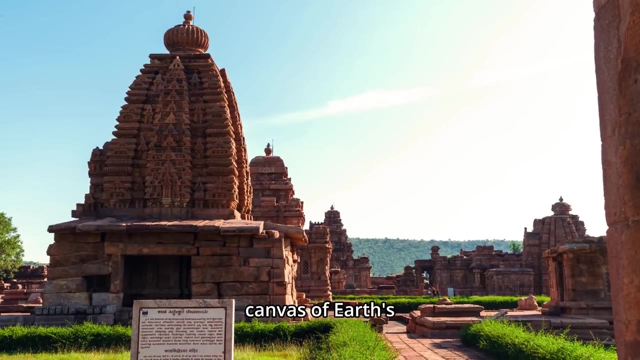 It was a tale of wind's unrelenting might shaping the Earth's canvas in the grand tapestry of time. These hollows and depressions etched a profound mark on the canvas of Earth's landscapes. Among them were the two pivotal nations. 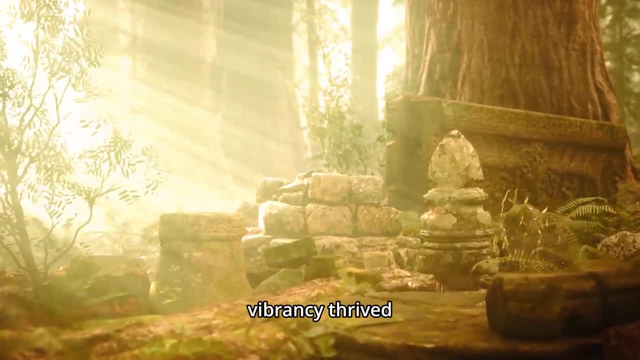 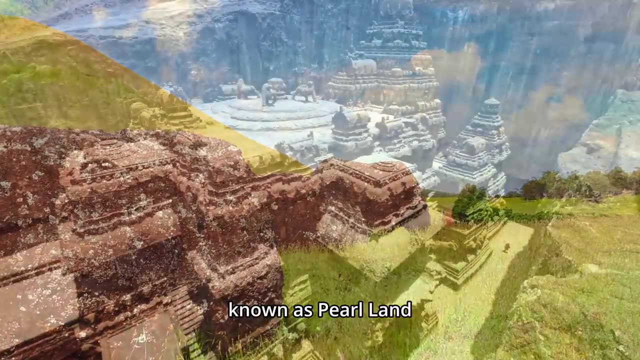 at the heart of the Asian continent, where life's vibrancy thrived. In tandem, the relentless sands invaded pockets of the bountiful land of India known as Pearl Land and the central territory within the African continent called Graben Sea. 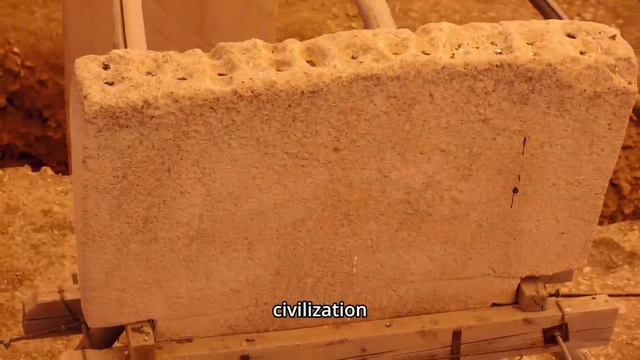 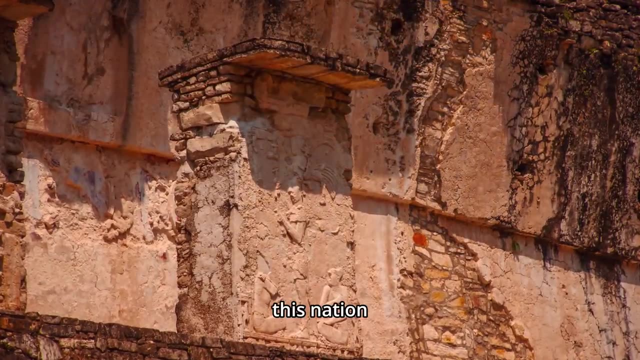 It was in this hallowed soil, a sanctuary of culture and civilization, that the center of culture for all three brain beings thrived. post Atlantis's fall. This nation, once a beacon of prosperity, is now recognized as the unforgiving Sahara Desert. 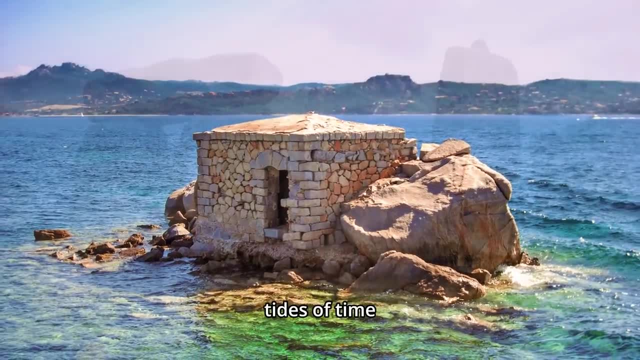 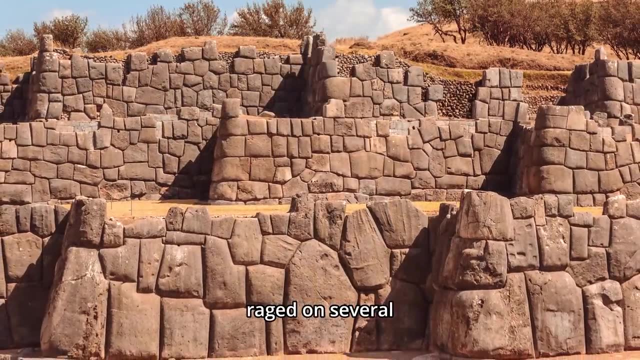 a stark testament to the shifting tides of time and the vicissitudes of our planet's history. As the tempestuous winds of that turbulent age raged on, several other modest stretches of terra firma on our beleaguered planet succumbed to their fury. 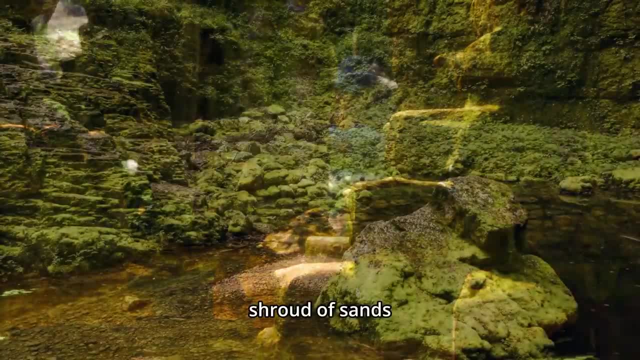 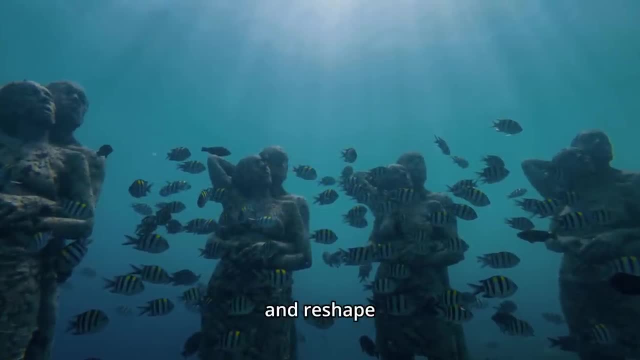 becoming engulfed by the relentless shroud of sands. It was an era where the very Earth seemed to writhe in the throes of transformation, as nature's forces shaped and reshaped the world's visage, The echoes of a cataclysmic universal deluge. 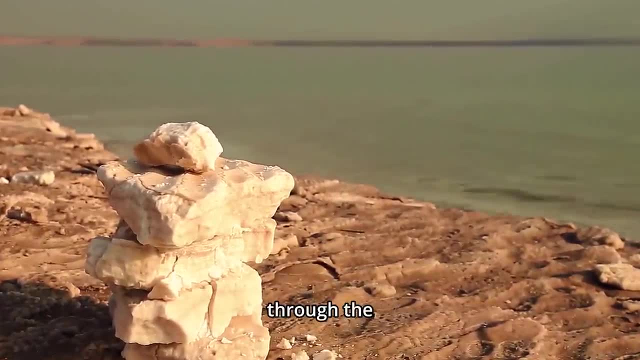 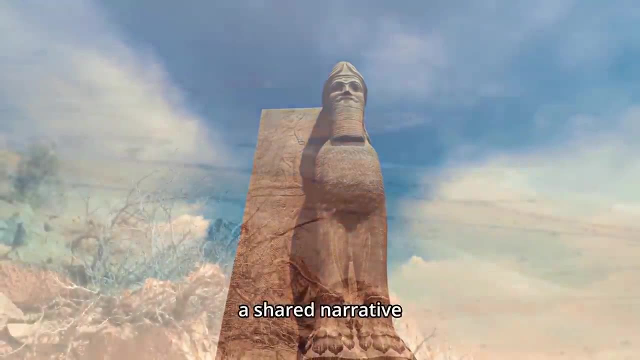 reverberate through the annals of time, woven into the myths and legends of over five hundred diverse cultures that span the globe, A shared narrative of profound significance. their accounts paint a picture of something extraordinary and calamitous. The emerging body of evidence testifies. 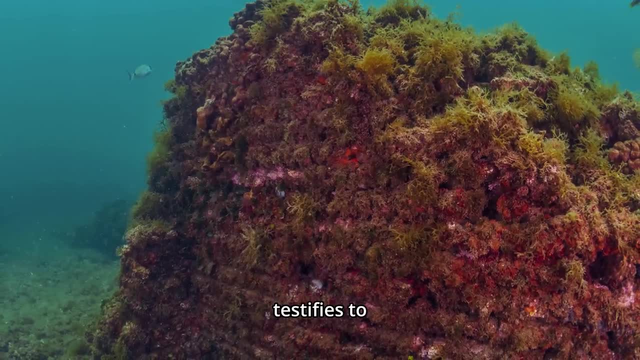 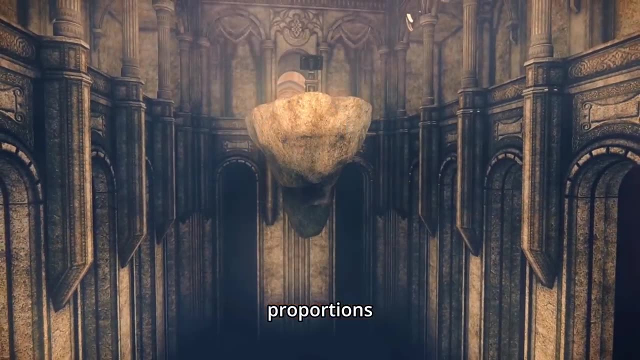 to the severity of this earth-shaking event. It stands as a witness to a cataclysm of monumental proportions, one that will never be forgotten, and one that will never be forgotten, One that reshaped our world. in its wake, The aftermath brought devastation. 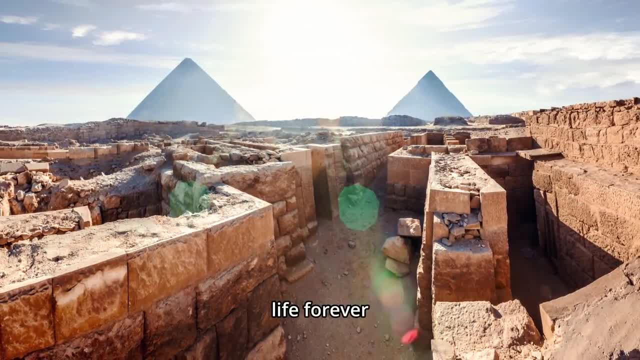 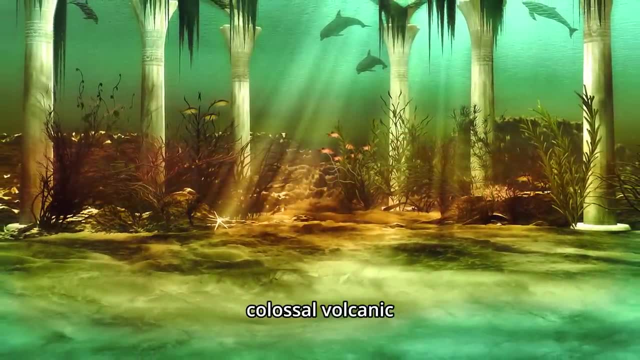 to the realm of life, forever altering the course of nature. It upthrust towering mountain ranges, sparked colossal volcanic explosions, etched deep valleys and fjords and left colossal deposits of stone and gravel strewn like a cosmic mosaic across the vast expanse of our planet's landmasses. 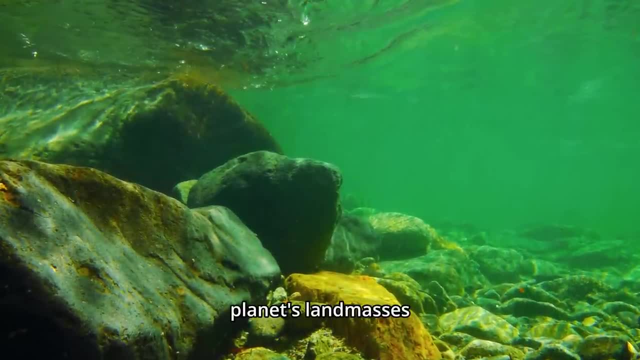 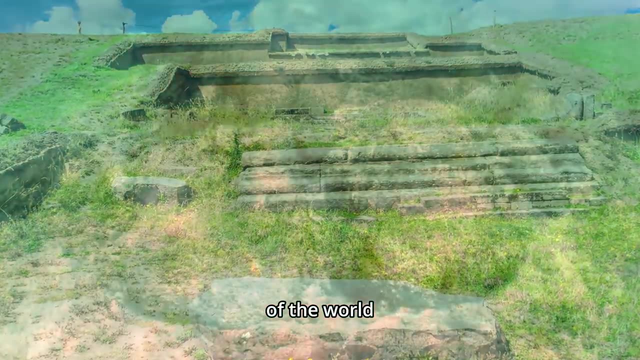 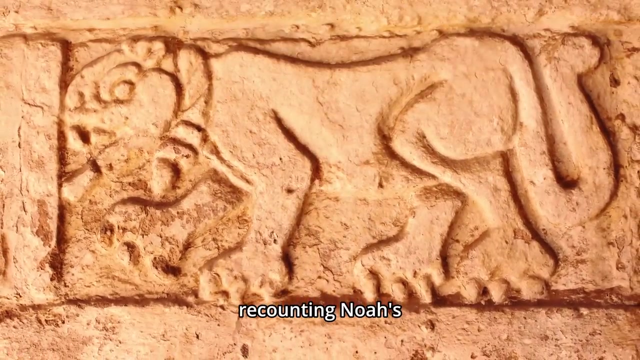 The tales of catastrophic events and the Great Flood are not confined to one corner of the world. They are not confined to one corner of the world. They resonate through the tapestry of human culture. They weave their threads through the Old Testament, recounting Noah's Ark. 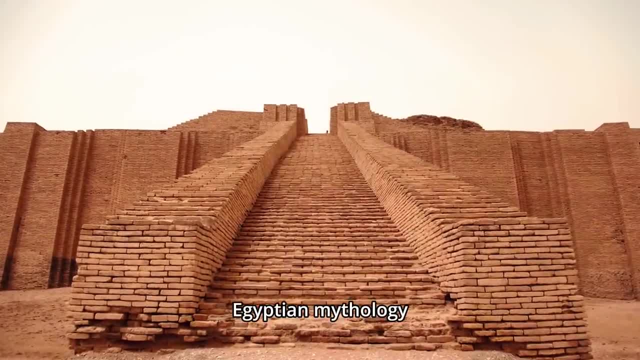 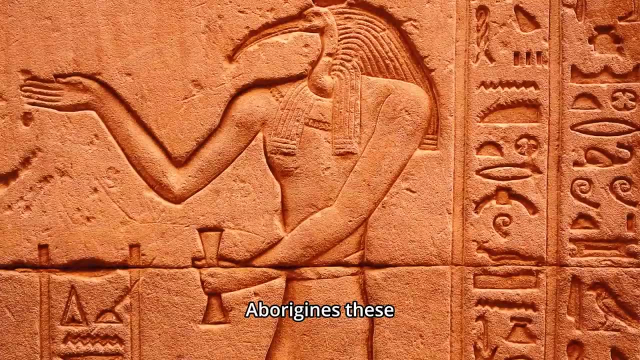 and the epic tales of the Sumerians. They find their place in the annals of Egyptian mythology, echo through the timeless Greek myths and resonate within the traditional narratives of the Australian Aborigines. These stories transcend the boundaries of geography and culture. 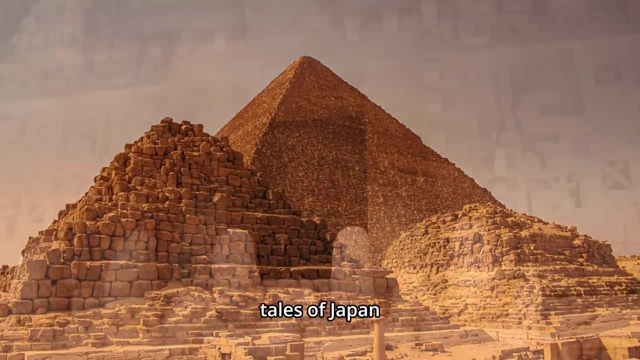 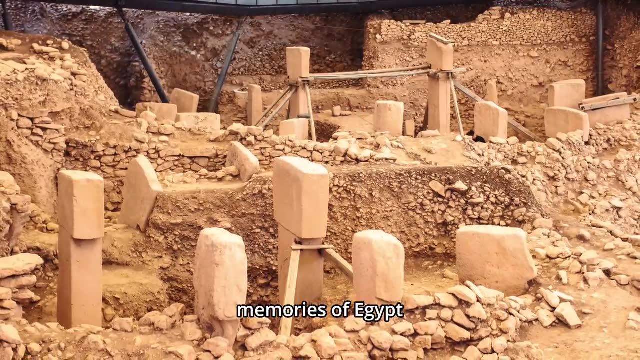 transcending borders and languages. They unfold in the tales of Japan, China, Thailand, Laos and India. in the East, They linger in the ancient memories of Egypt and the Congo. in Africa, In Europe, they find their voice in the stories of Greece, Germany. 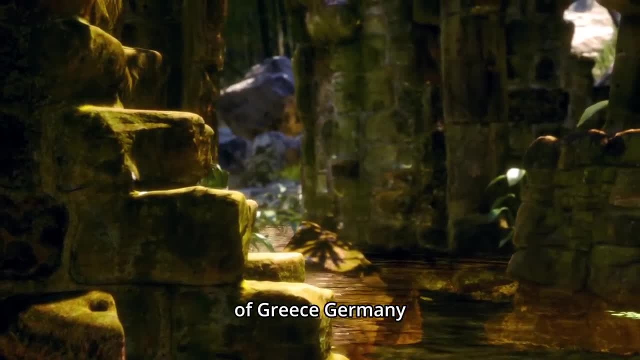 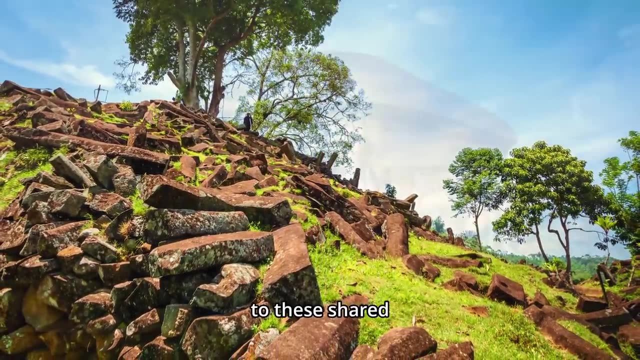 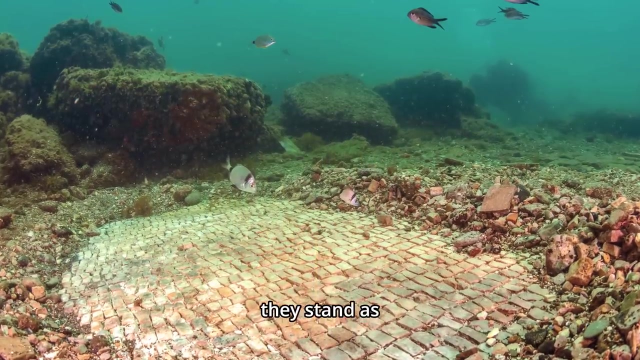 and Scandinavia, and in the New World. indigenous tribes of North, Central and South America bear witness to these shared legends. For many ethnologists, these myths represent more than mere folklore. They stand as potential legends into history. The possibility exists. 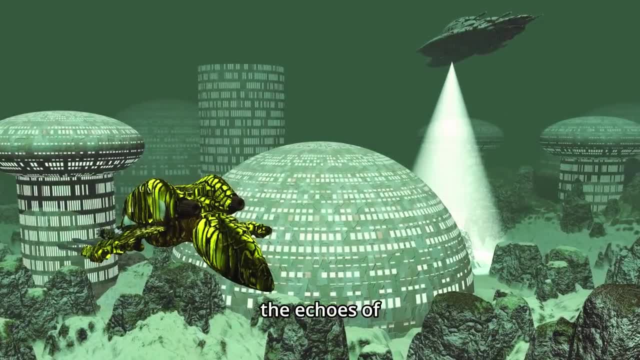 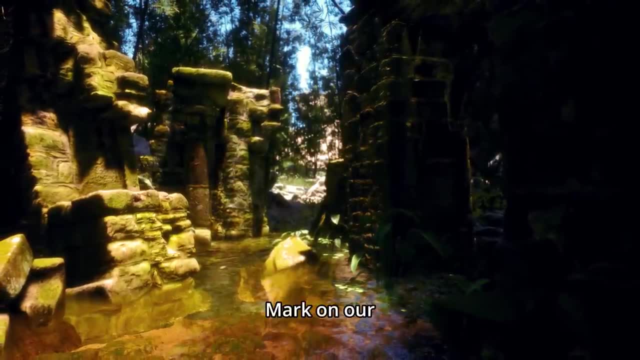 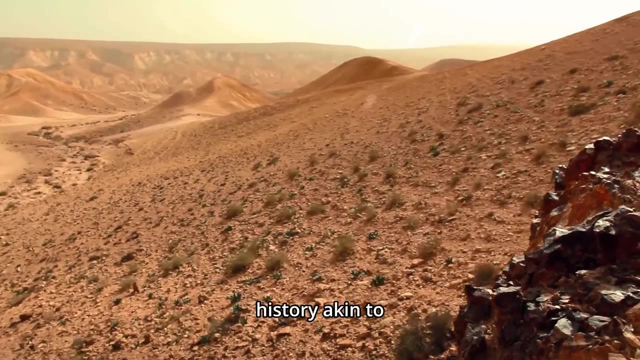 that they are the echoes of accurate records preserved and passed down through generations, perhaps bearing witness to events that have left an indelible mark on our collective past. The echoes of the Great Flood reverberate through the corridors of history, akin to the cataclysmic deluge. 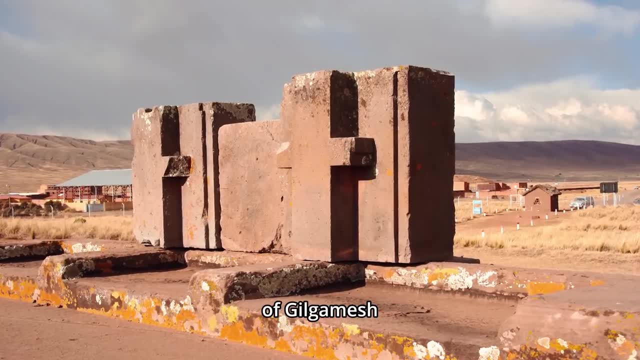 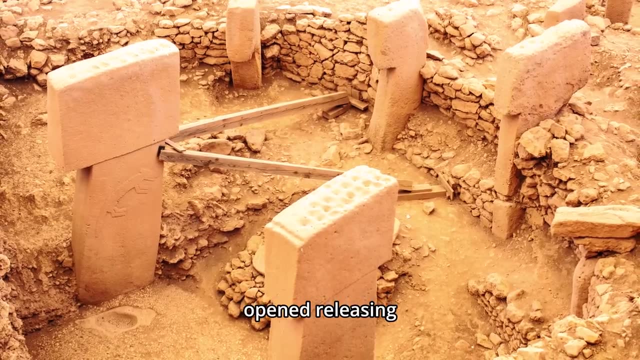 recounted in the Old Testament In the ancient Sumerian epic of Gilgamesh. when its inundation unfolds, the floodgates of heaven truly opened, releasing torrents of rain Springs, once small and tranquil, turned into surging rivers. 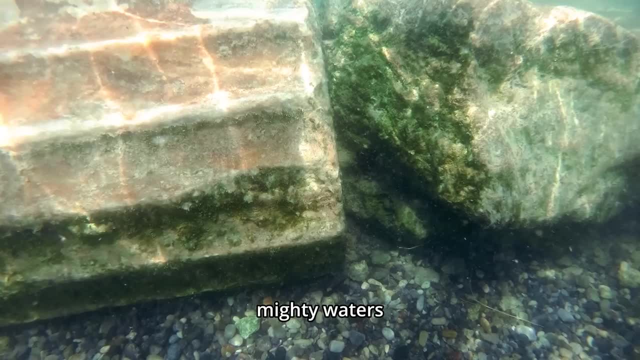 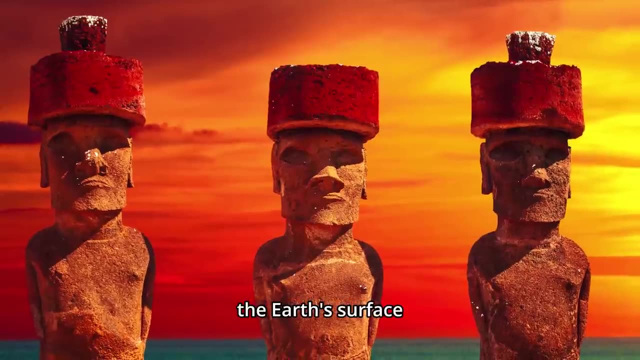 swelling in response to the tremendous downpours. These mighty waters mingled with the tidal waves, giving birth to overwhelming floods that blanketed vast expanses of the earth's surface. In the wake of this relentless deluge, all life was swallowed. 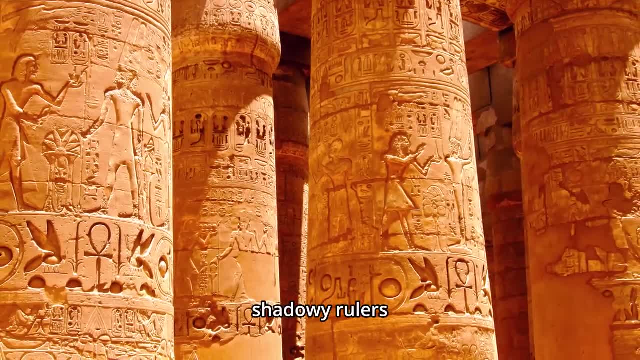 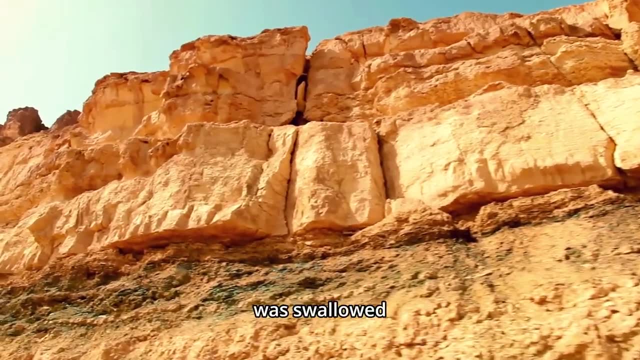 the waters. In a bygone era, the shadowy rulers of the night unleashed a fearsome tempest from the heavens. At the break of dawn, the once blue sky was swallowed by clouds as dark as midnight itself. Malevolent spirits stirred. 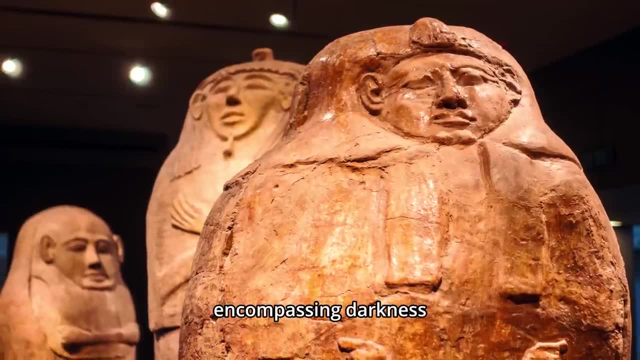 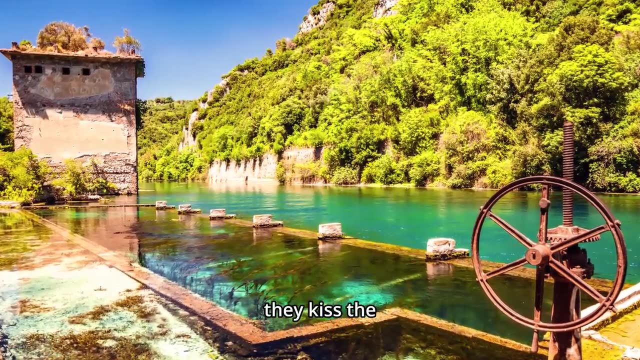 and the very essence of light succumbed to an all-encompassing darkness. A tempestuous southerly gale howled with an unholy fury, propelling the waters to rise and swell until they kissed the very mountains. And in this relentless deluge, 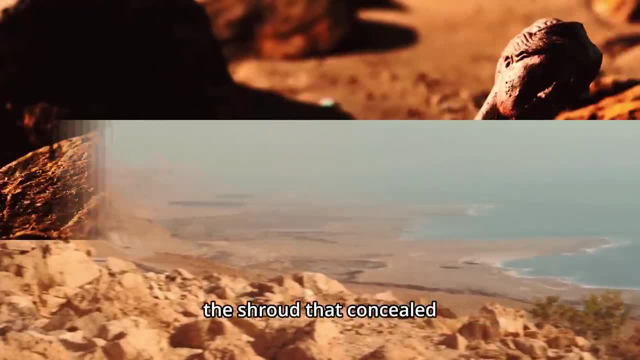 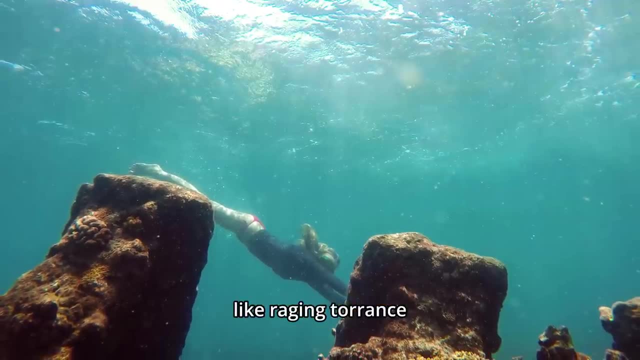 the waters became the shroud that concealed the world's inhabitants. For six long days and six unending nights, the rain roared forth like raging torrents, a cataclysmic force beyond reckoning. Then, on the seventh day, a tranquil hush fell over the land. 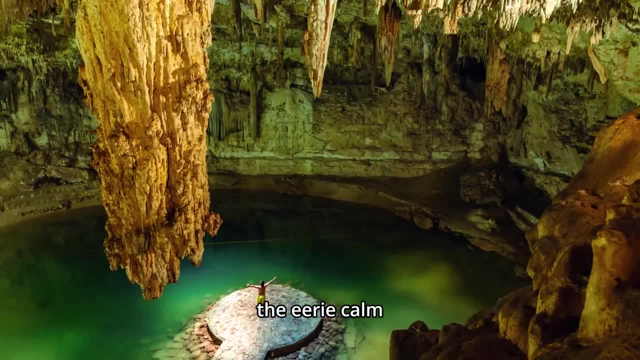 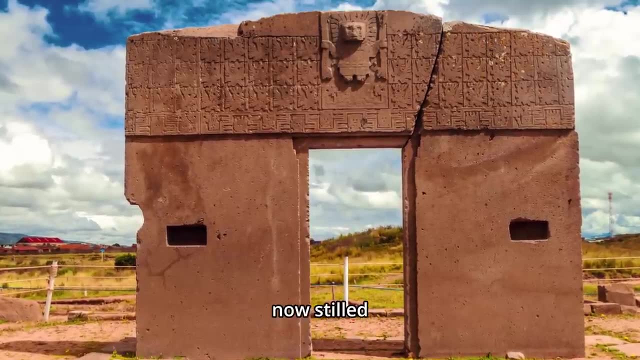 akin to the eerie calm that follows a tumultuous battle. The once mighty sea, which had raged with an insatiable hunger, now stilled its tempestuous heart. The storm of catastrophe relented and I gazed upon the world. 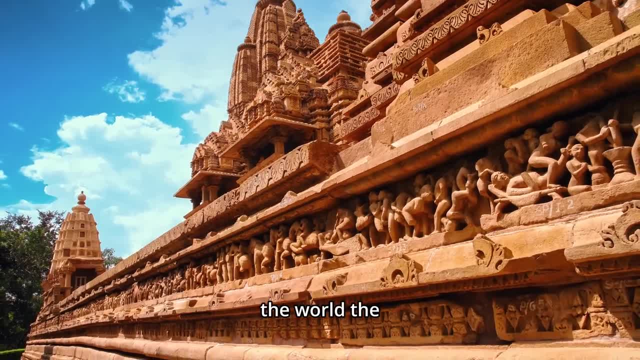 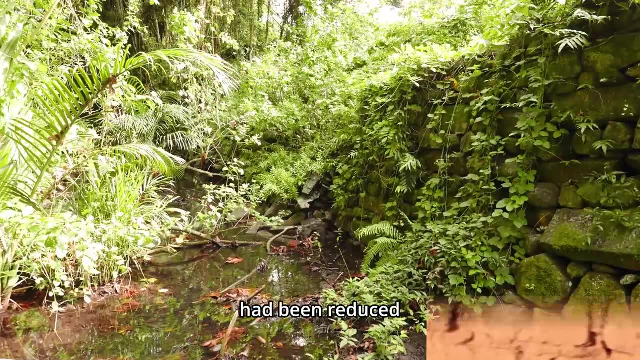 the air now laden with an eerie stillness. A macabre transformation had occurred, as all the people had been reduced to little more than mud, their existence a mere memory. The very earth beneath their feet had been stripped of life, rendering the landscape a desolate. 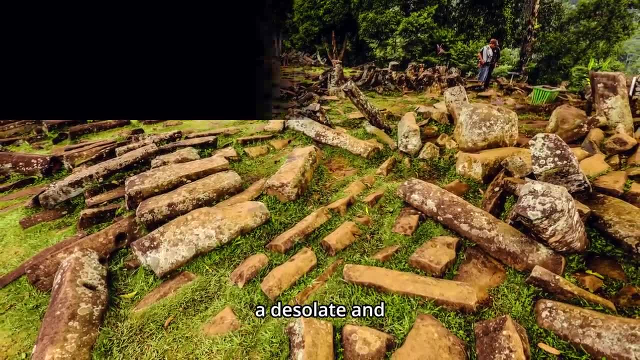 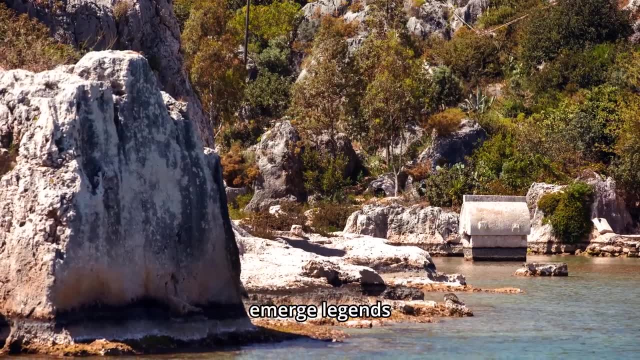 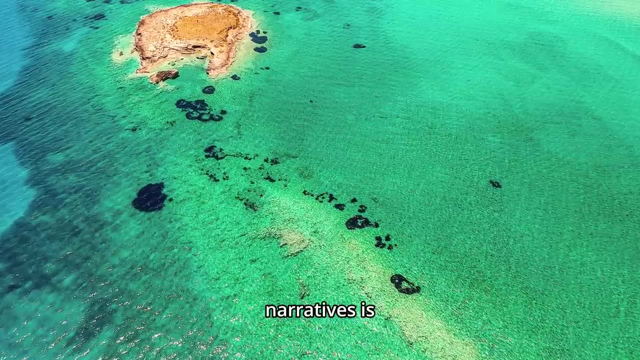 and barren wasteland. From the diverse tapestry of North- and South-American indigenous cultures emerged a beautiful, ferocious legend that mirrored tales of fierce earthquakes followed by deluges that wrought widespread havoc. Among these narratives is the flood myth of the Haida. 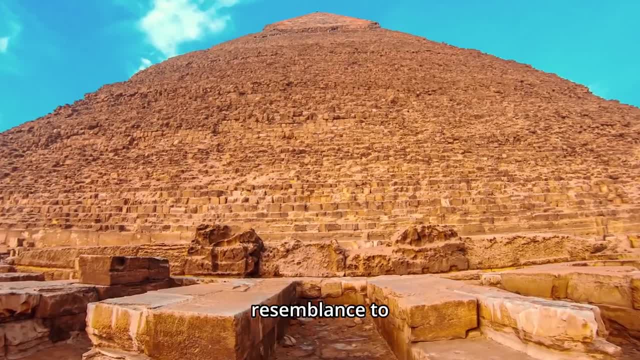 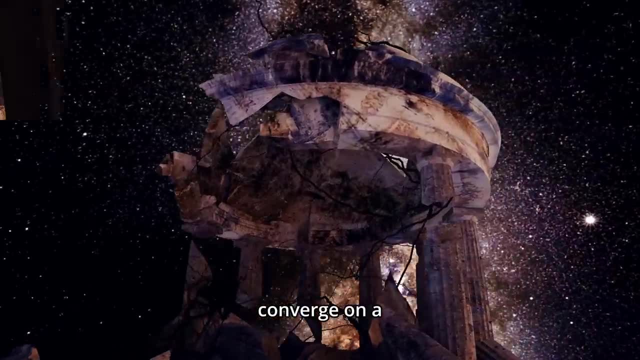 in British Columbia, a story that bears a remarkable resemblance to the ancient Sumerian myth. These tales, spoken across the expanse of the earth, converge on a singular narrative: The sun itself strays from its ordained course, veering from the expected path. 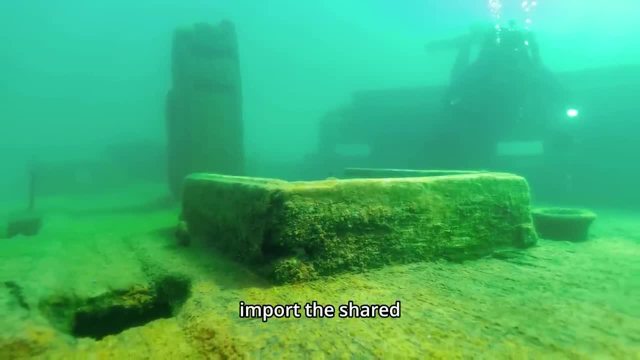 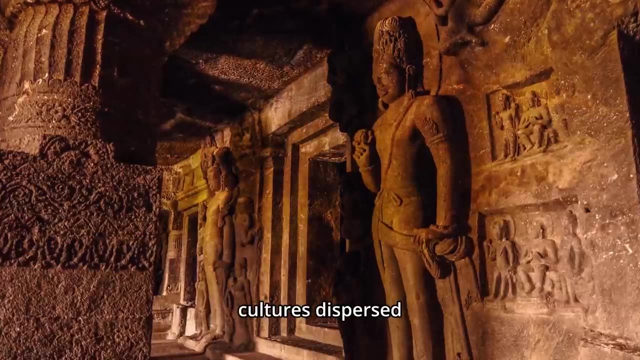 in a celestial anomaly of profound import. The shared thread of these accounts weaves a tapestry of our planet's history, where common motifs echo through the voices of cultures dispersed across time and geography. The heavens themselves seem to plummet earthward, and the very ground beneath our feet 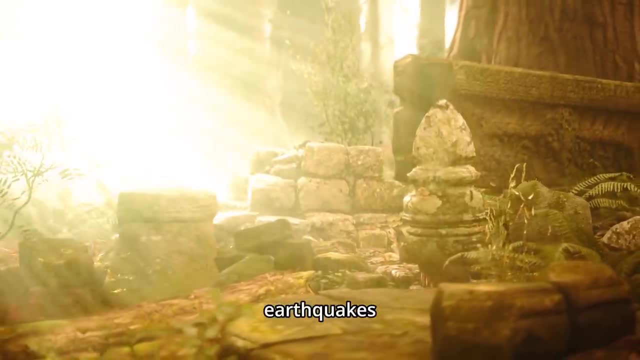 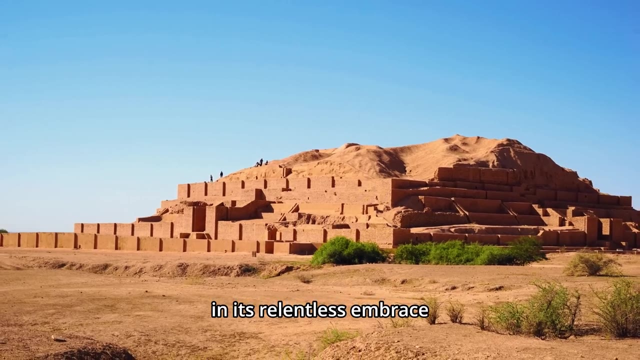 convulses and writhes in the throes of powerful earthquakes. In the climactic crescendo, an immense wall of water sweeps across the globe, swallowing all in its relentless embrace. As the stories unfurl many indigenous tribes, a common refrain resounds: 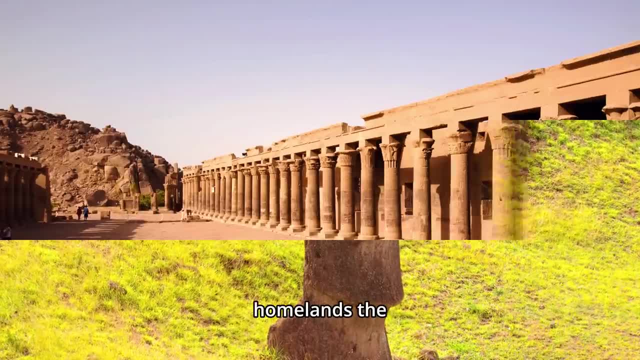 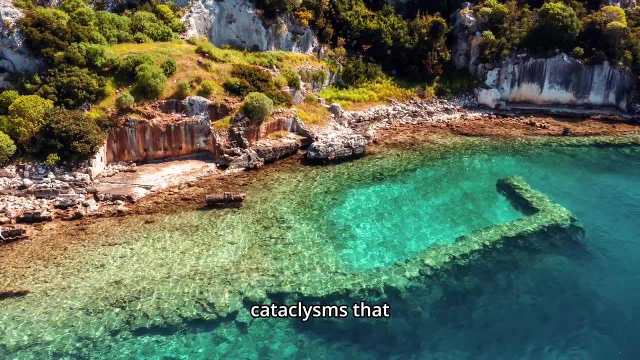 a world-shaking flood of colossal proportions inundated their homelands. The tales are told in countless variations, a testament to the shared human experience of these tumultuous cataclysms that reshaped the lands they called home In the icy realms of Alaska. 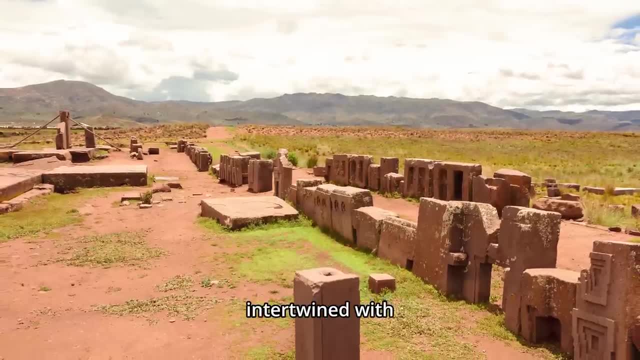 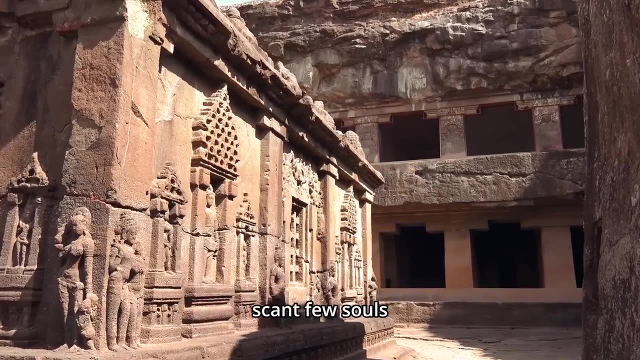 the Inuit people spoke of a harrowing deluge intertwined with the violent tremors of an earthquake. This catastrophic force swept across the land with such swiftness that only a scant few souls were able to seek refuge, clinging to their canoes. 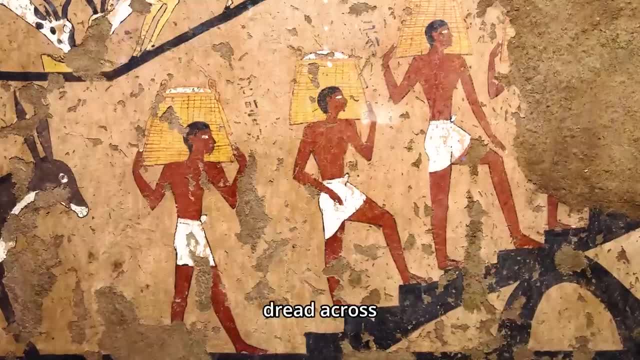 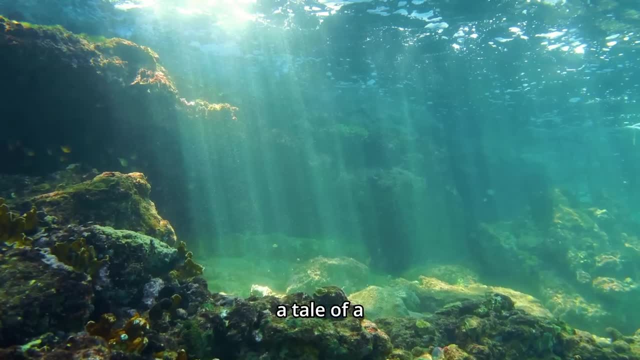 or huddled atop the mightiest mountains, gripped by paralyzing dread. Across the sun-drenched expanses of lower California, the Luiseno shared their own legend, a tale of a flood that rose to shroud the very mountains, unleashing its destructive fury upon the masses of humankind. 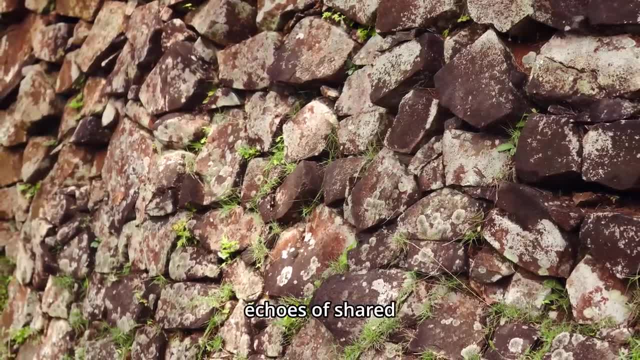 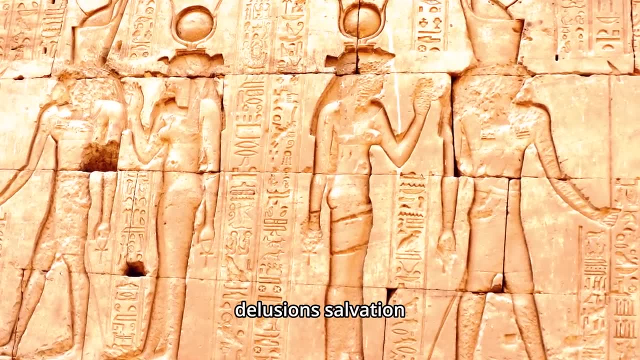 In these diverse narratives, we glimpse the echoes of shared human experiences as communities faced the relentless might of nature's wrath. Among these perilous deluges, salvation came to but a fortunate few, those who sought refuge on the loftiest peaks which, alone, remained untouched. 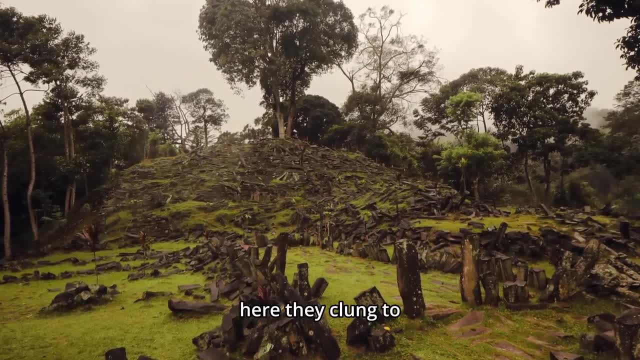 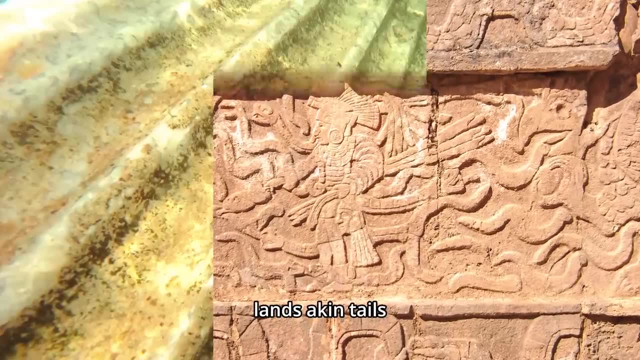 when the rest of the world succumbed to the inundation, Here they clung to their sanctuary until the watery tempest's fury was spent In the northern lands. akin tales unfolded Among the Huron kindred myths of the Great Flood. 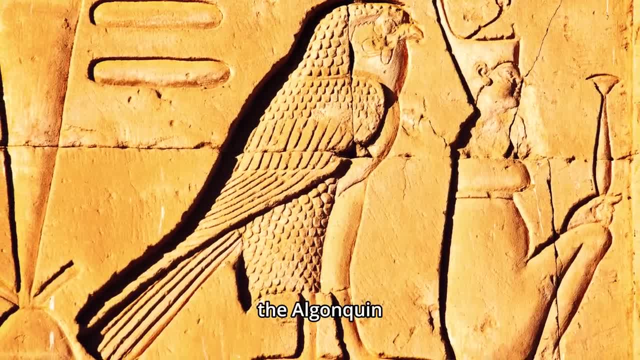 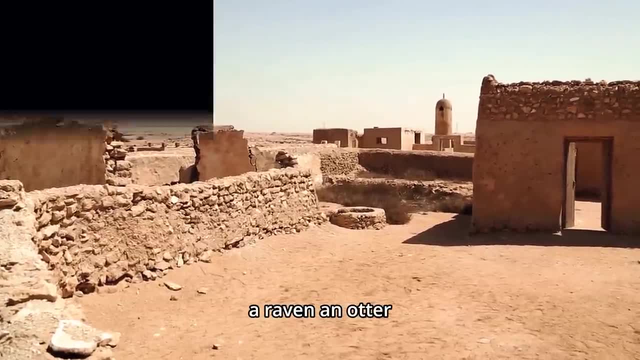 were etched into their cultural memory. The Algonquin, in their own legend, recounted the role of Macabo the Great Hare, who, with the assistance of a raven, an otter and a muskrat, labored to breathe life anew. 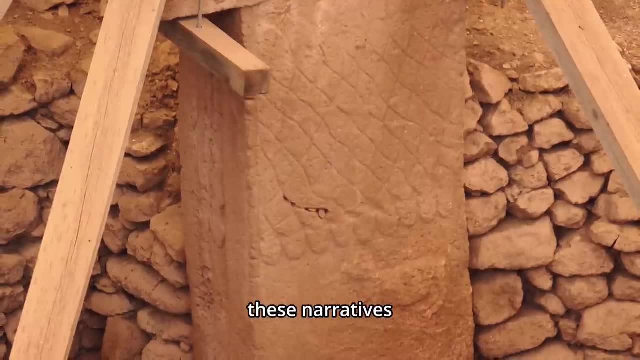 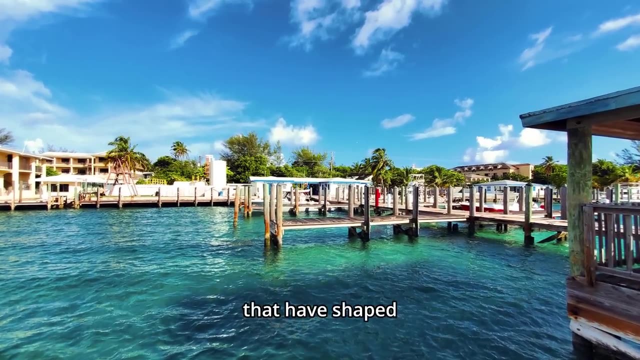 into a world ravaged by the deluge's embrace. These narratives, diverse yet interconnected, echo across the annals of human history, weaving the threads of shared experiences that have shaped our collective past. In the tapestry of indigenous myths, the Iroquois wove a tale of a time. 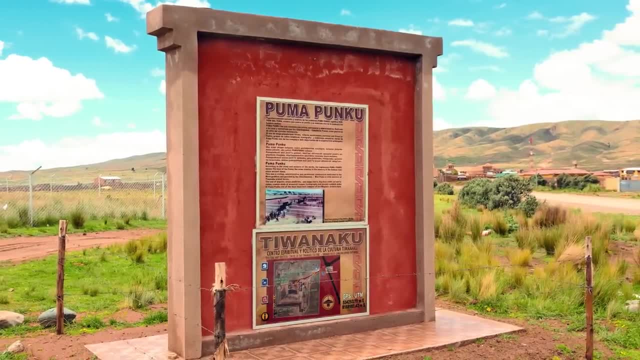 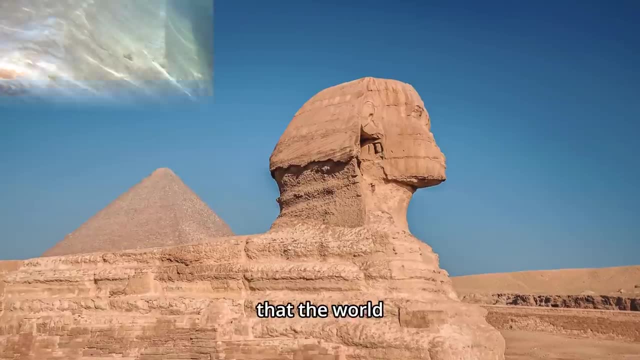 when the sea and its surging waters encroached upon the land, extinguishing all human life in its relentless embrace, The Chickasaw people, too, proclaimed that the world had met its end in a watery deluge, but amidst the deluge. 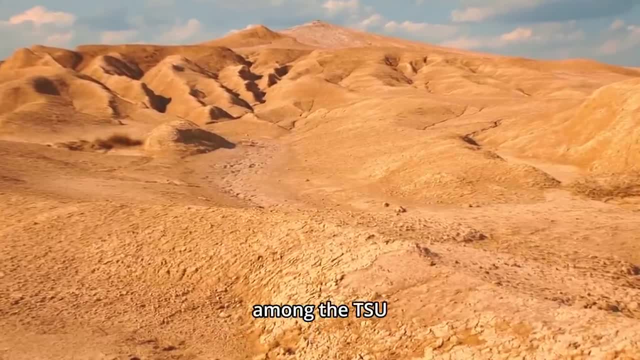 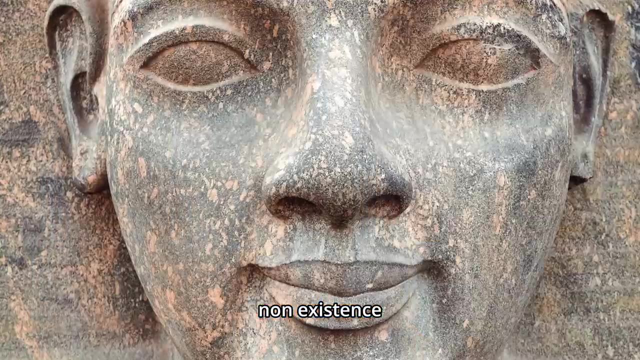 one family endured alongside two representatives of every creature kind. Among the Sioux, the stories recounted a world devoid of dry land, where humankind vanished into the mists of nonexistence, swallowed by the all-encompassing waters. These tales form a collective memory. 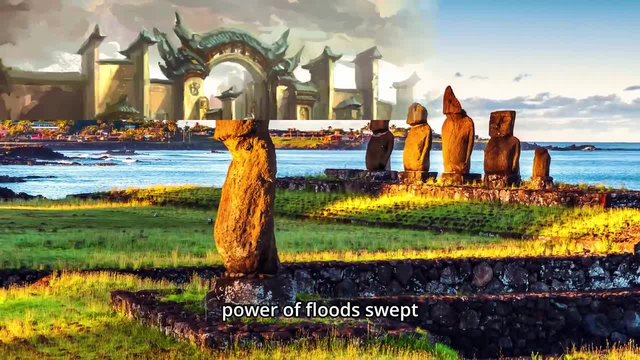 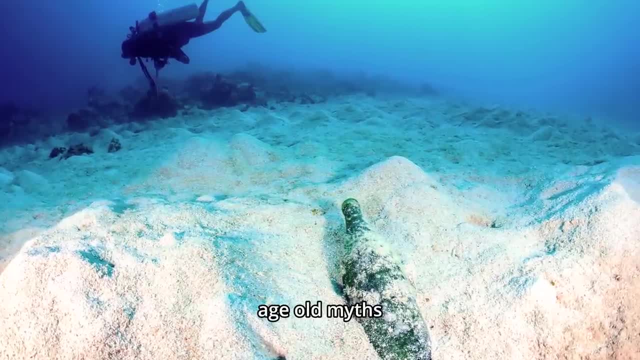 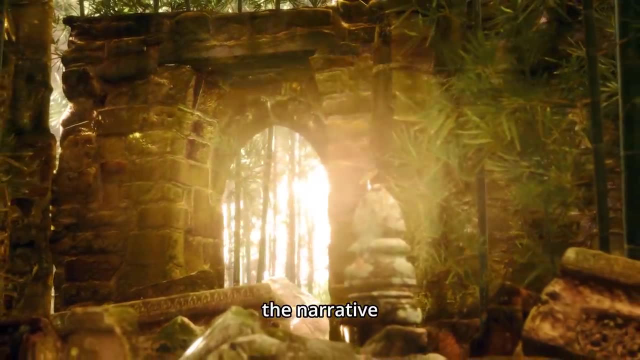 of a shared past, where the transformative power of floods swept the stage of history clean, leaving behind stories of survival and renewal. Embedded within these age-old myths and legends are subtle hints of celestial changes that heralded the onset of devastating floods. The narrative threads often interweave. 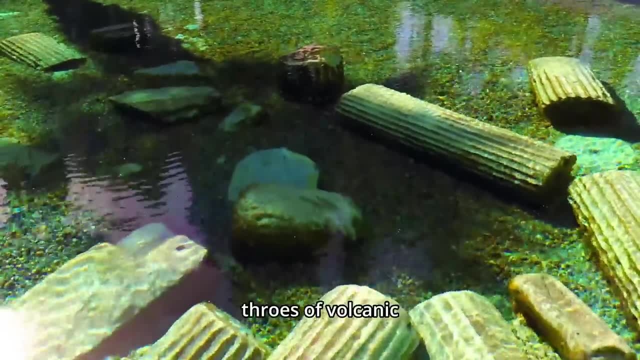 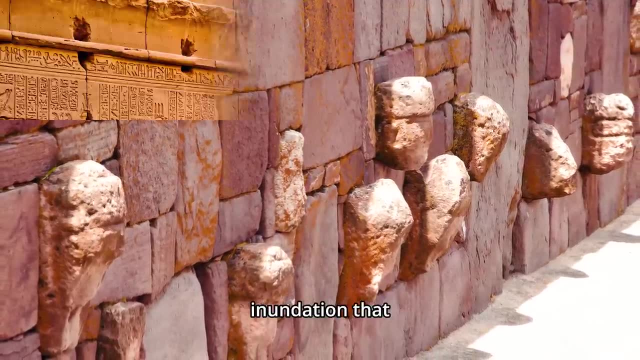 with vivid accounts of earth-shaking, earthquakes and the fiery throes of volcanic eruptions. These cataclysmic events, these tales convey, set the stage for the catastrophic inundation that reshaped the world, sculpting new landscapes and shifting the very contours. 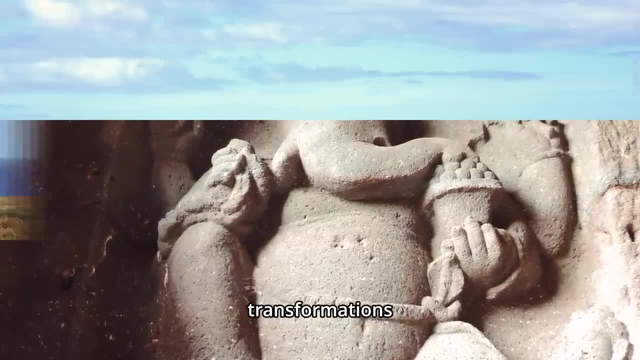 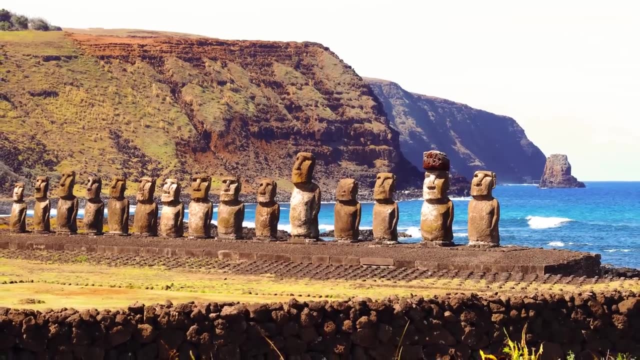 of the planet's mountain ranges. In the crucible of these colossal transformations, Earth's very axis may have undergone a dramatic tilt, or its crust might have endured a violent upheaval. Continents danced in a relentless ballet of emergence and submersion. 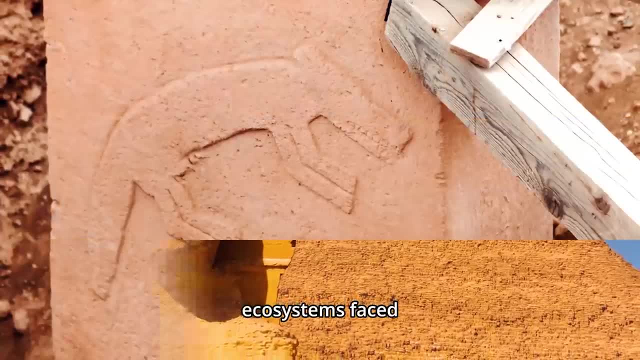 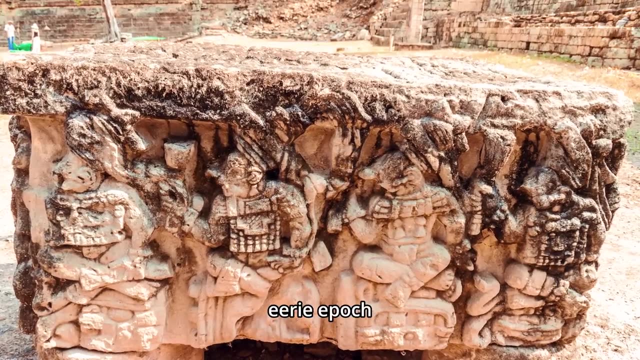 In the wake of these monumental shifts, entire ecosystems faced mass extinctions, both for the flora that graced our lands and the fauna that roamed them. The world entered an eerie epoch of global darkness, where daylight shrank before the obsidian veil. 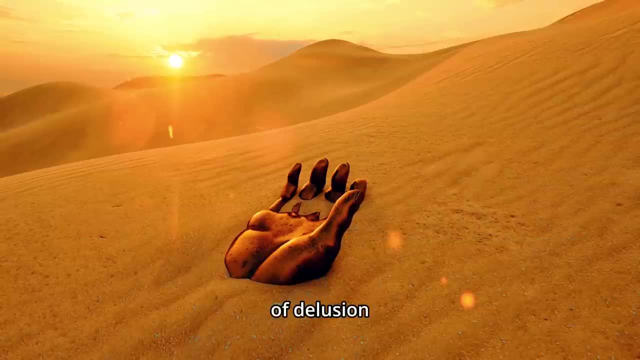 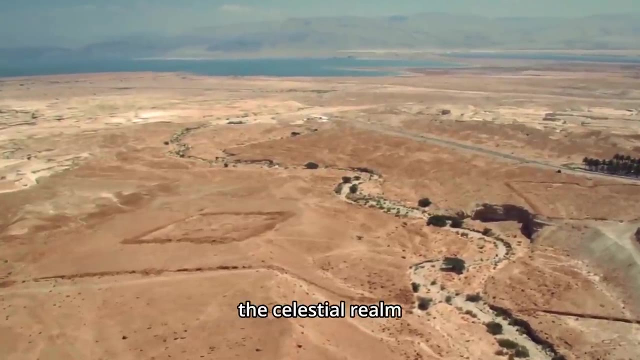 that enshrouded our planet. Amid these tales of deluge and calamity, one finds not only the foreboding veil of darkness descending, but also enigmatic transformations in the celestial realm. In the distant Tierra del Fuego, the whispers spoke of a time 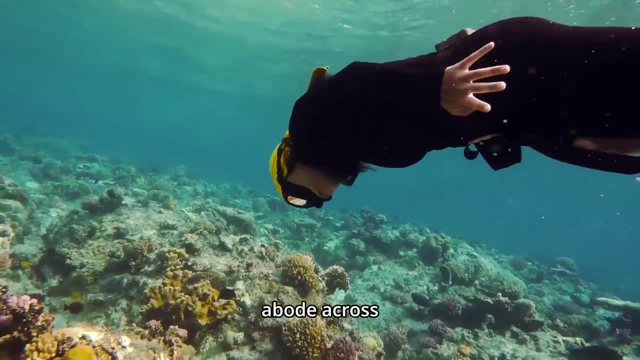 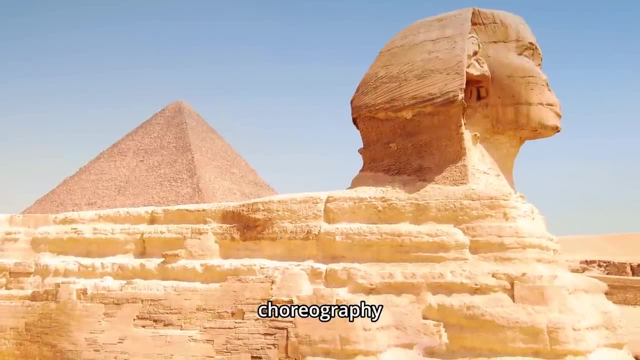 when the sun and the moon plummeted from their celestial abode Across distant China, the legends carried echoes of the sun, moon and stars shifting their cosmic choreography. The Inca civilization held in their collective memory the belief that in epochs of old, 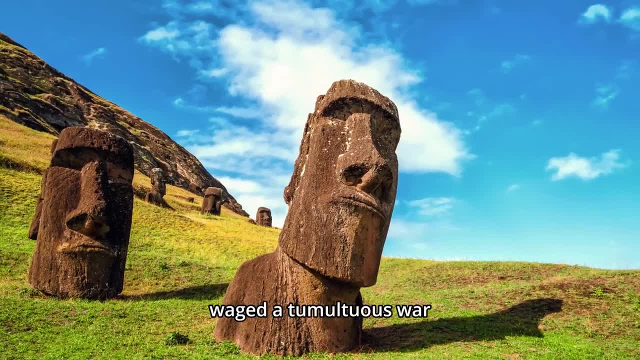 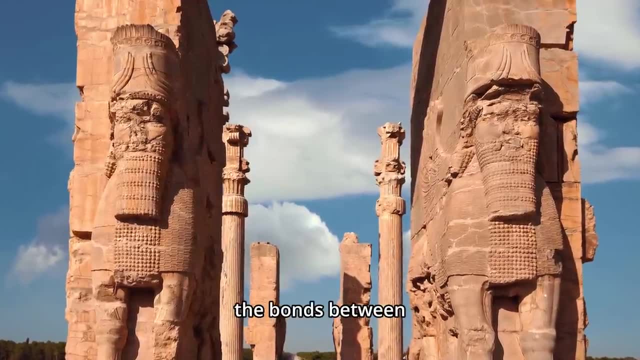 the mighty Andes themselves were rent asunder when the heavens waged a tumultuous war upon the Earth. These stories weave a tapestry of profound change where the bonds between Earth and sky were tested and reshaped in epochs long past In the annals of myth and legend. 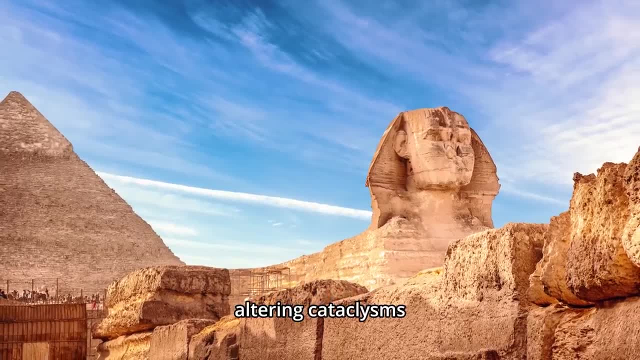 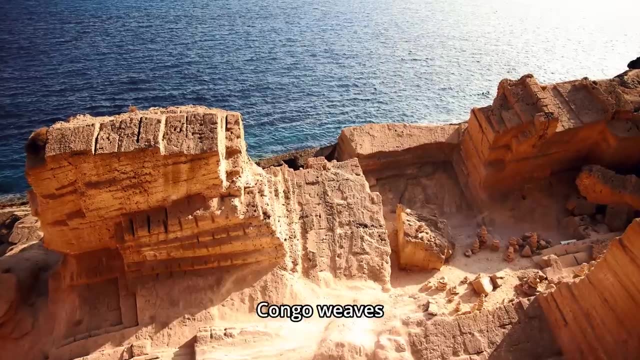 the Tarahumara of northern Mexico safeguard stories of world-altering cataclysms guided by shifts in the sun's path. A vivid African narrative from the Lower Congo weaves the tale of a time when the sun and the moon met in a celestial encounter. 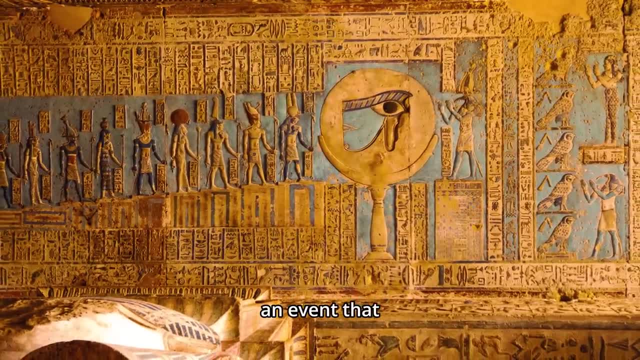 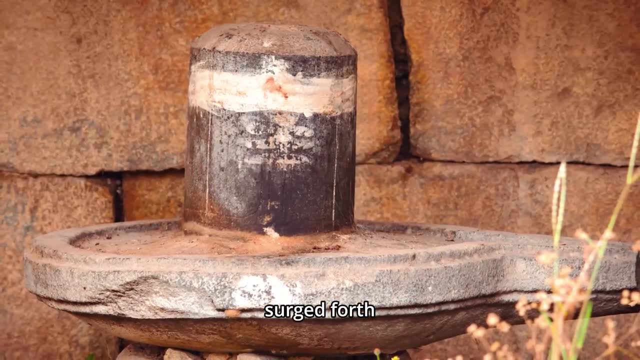 casting mud upon the lunar visage and dimming its radiant glow, an event that heralded a profound deluge Within the ancient realm of Graeco-Roman myths. the flood of Deucalion surged forth on the heels of awe-inspiring celestial phenomena. 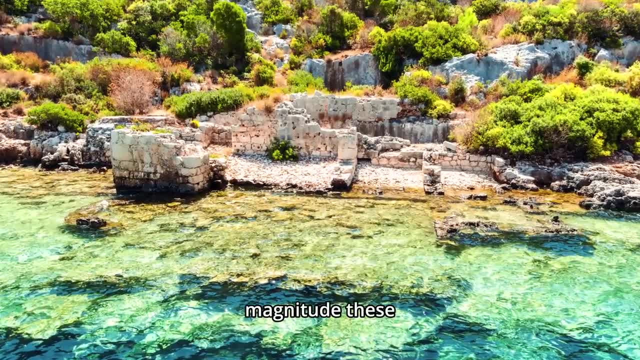 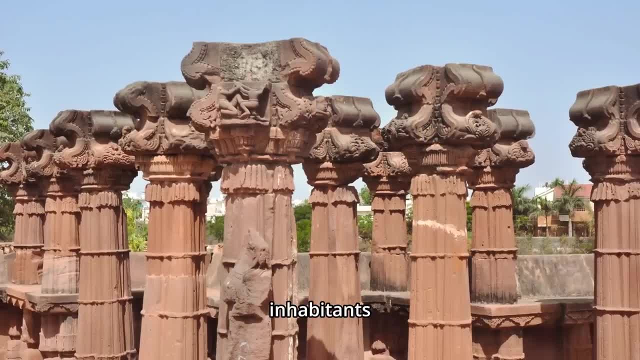 foretelling a cataclysmic inundation of unparalleled magnitude. These narratives convey how the celestial dance in the heavens held the power to shape the destiny of Earth and its inhabitants. Graham Hancock, in his work Fingerprints of the Gods, marks the global flood narrative within the timeframe. 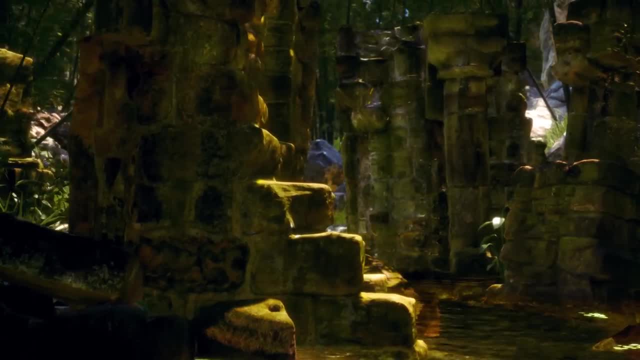 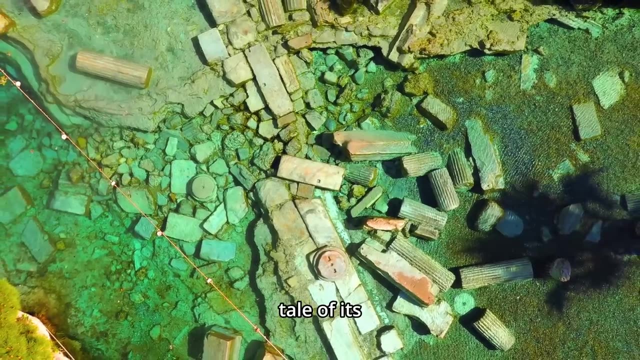 spanning from 15,000 to 8,000 BC. This intriguing dating aligns with intriguing proximity to the chronicles of Plato's Atlantis and the enigmatic tale of its cataclysmic downfall. The threads of these narratives seem to converge within this epoch. 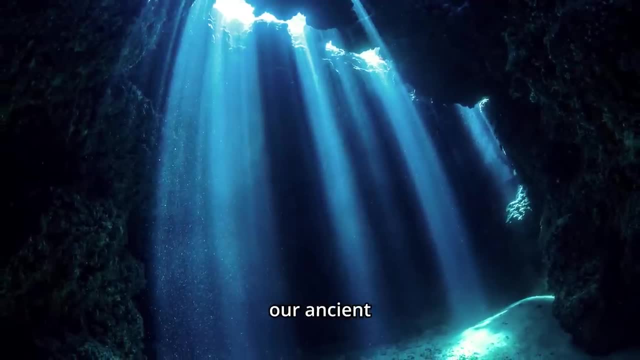 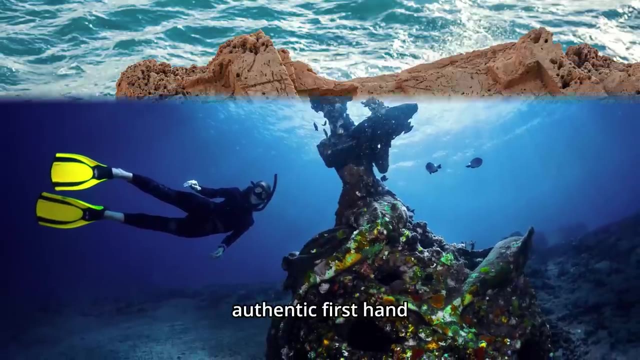 inviting us to explore the profound mysteries of our ancient past, He states. The tapestry of great cataclysmic myths appears to bear the hallmarks of authentic first-hand testimonies of the trials faced by humanity during the waning years of the last ice age. 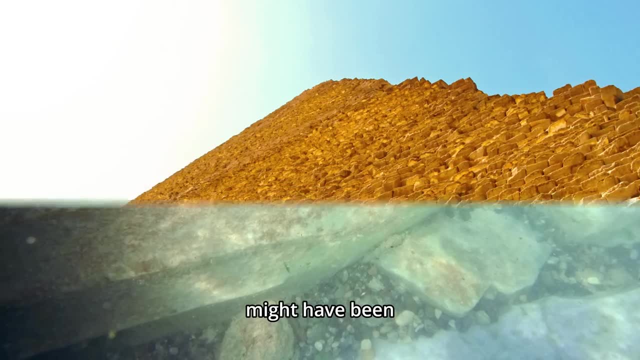 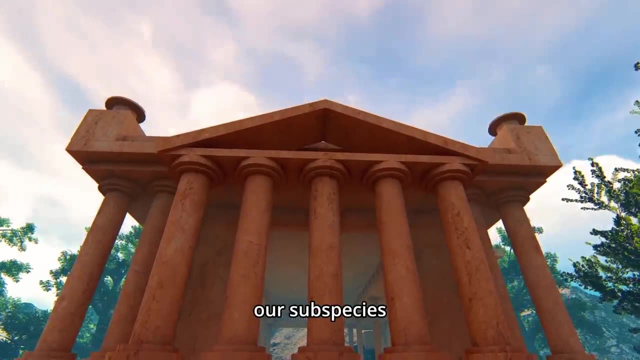 In this intriguing hypothesis, these narratives might have been woven into the fabric of human consciousness nearly as far back as 50,000 years ago, around the time of the ascent of our subspecies, Homo sapiens sapiens. These stories etched into the annals of our ancient heritage. 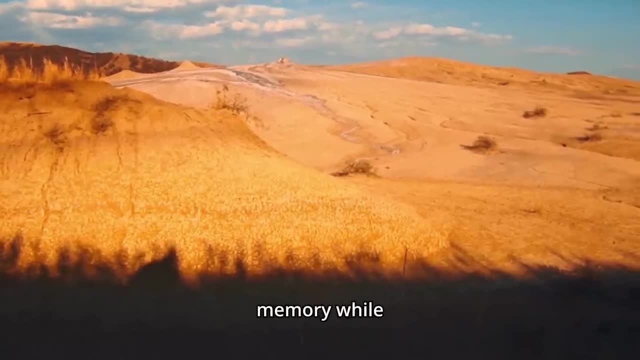 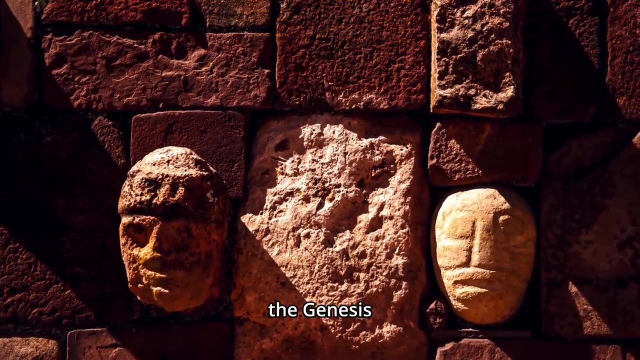 carry echoes of a profound history eternally engraved in our collective memory, While the geological records speak a slightly different tale, they point to a more recent timeframe for the genesis of these myths, The period spanning from 15,000 to 8,000 BC. 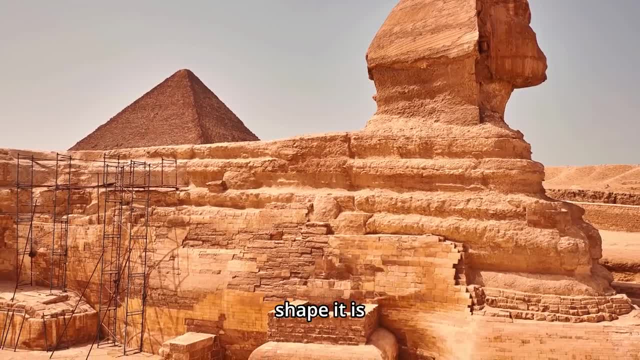 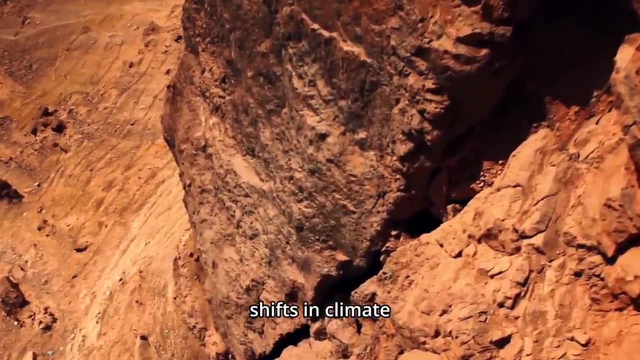 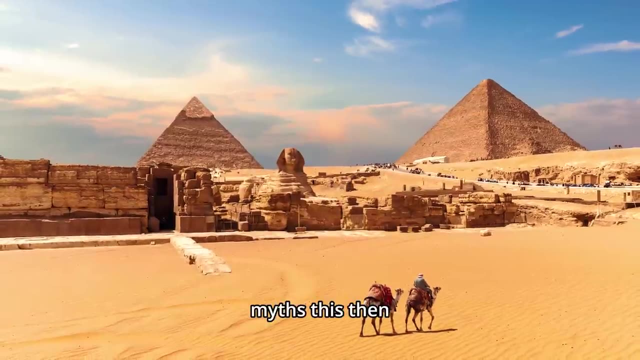 emerges as the most plausible epoch for these narratives to have taken shape. It is during this window of time that our human journey witnessed the dramatic and convulsive shifts in climate, echoing the resounding climatic transformations beautifully portrayed in these ancient myths. This then becomes the canvas upon which our collective memory paints. 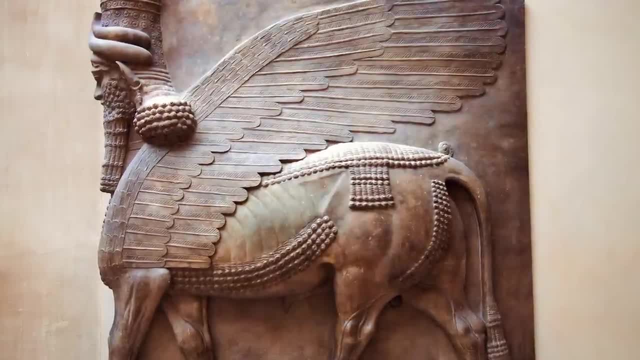 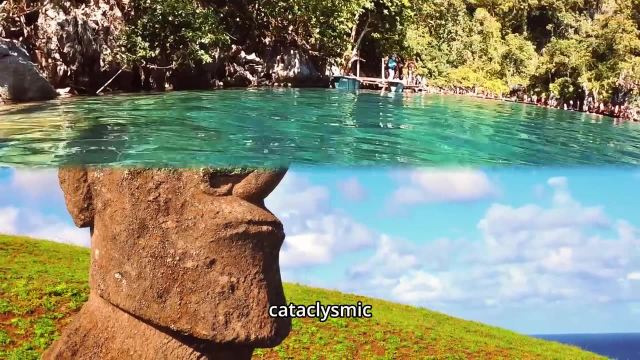 a vivid and enduring portrait of our past. Mountains of archaeological evidence culled from diverse sources converge to depict a harrowing narrative of cataclysmic events and a monumental worldwide deluge. These vestiges from our past echo with resounding clarity. 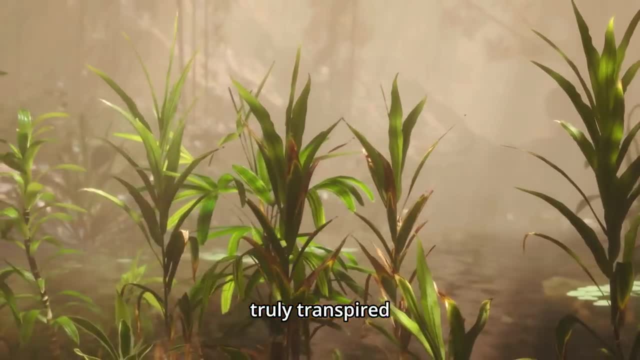 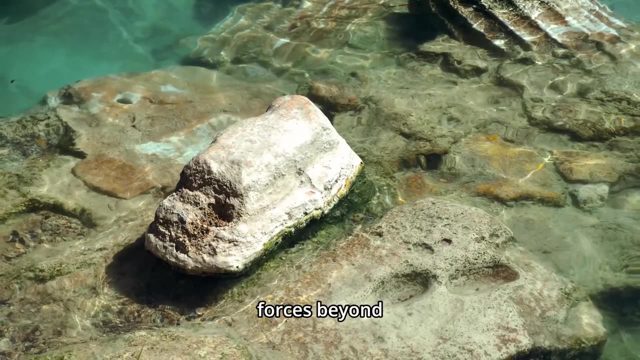 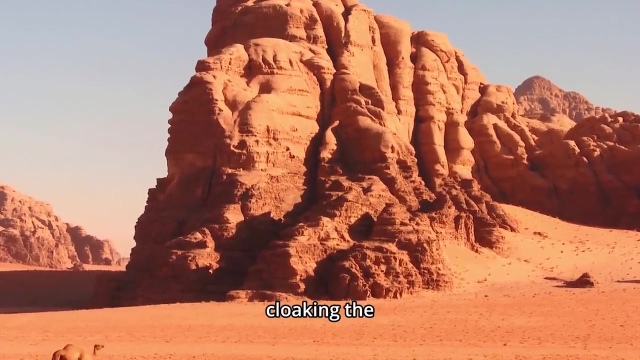 forming a tableau of ancient upheavals that truly transpired In the intricate mosaic of history. these remnants paint a vivid picture of a time when the world was reshaped by forces beyond imagination. Intriguing traces of history reveal the presence of an extraordinary amount of volcanic ash cloaking the atmosphere in the Quaternary Epoch. 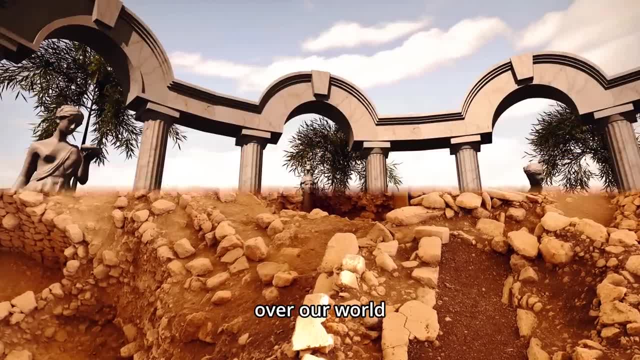 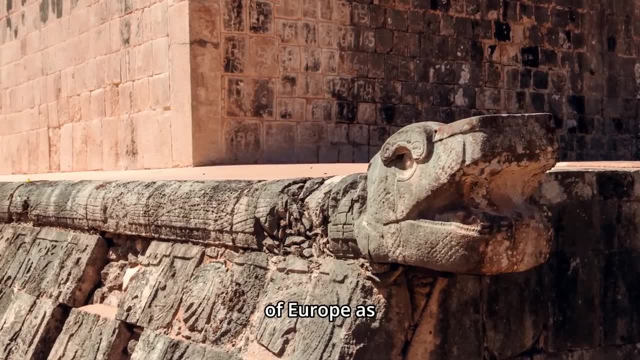 This ash cast a long and ominous shadow over our world as it veiled the radiant sun and sent temperatures plummeting. Ancient myths from the earliest epochs of Europe, as well as time-honored legends from Japan and India, recall the memory of these unnaturally dark skies. 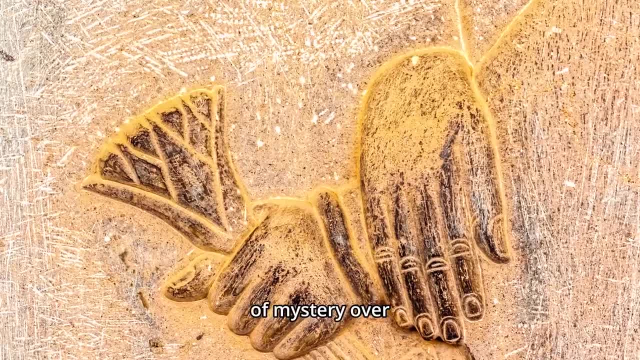 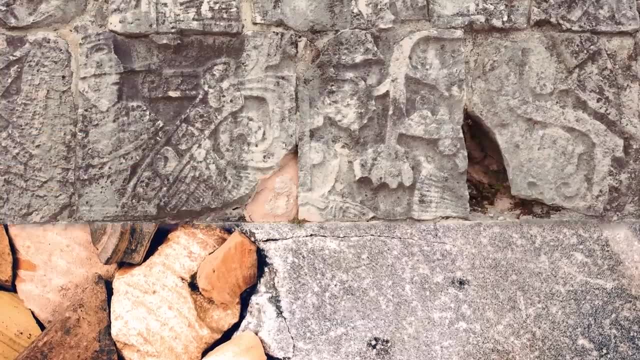 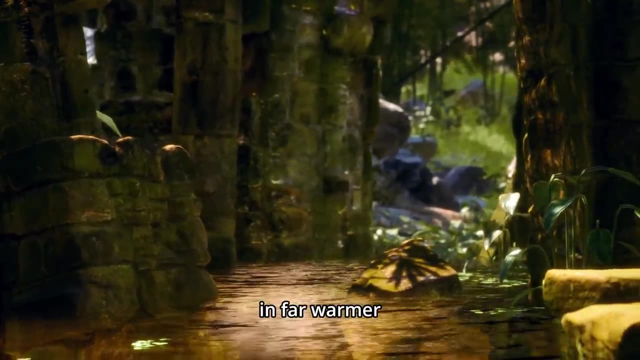 stretching their shadowed influence across years, casting a cloak of mystery over our distant past. In the Arctic's frozen embrace, a remarkable discovery unfolds: the remnants of lifeforms including lush plants, towering trees and diverse animals that once thrived in far warmer climes. 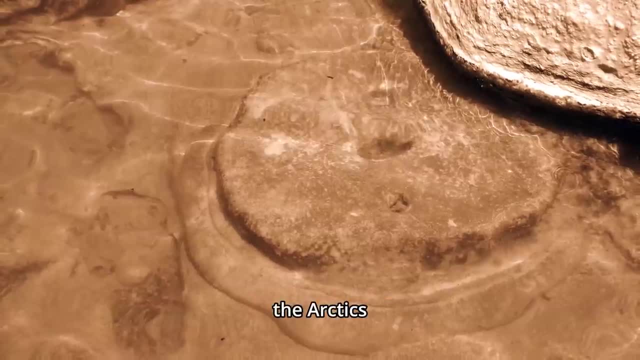 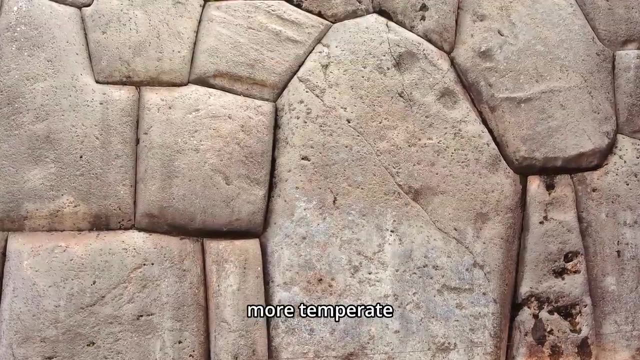 These enigmatic fossils deposited within the Arctic's icy vaults offer a glimpse into the ancient past, when the northern reaches of our planet embraced a much milder, more temperate temperament. In the hidden depths of our planet's secret chambers, the fossilized echoes of a bygone era are revealed. 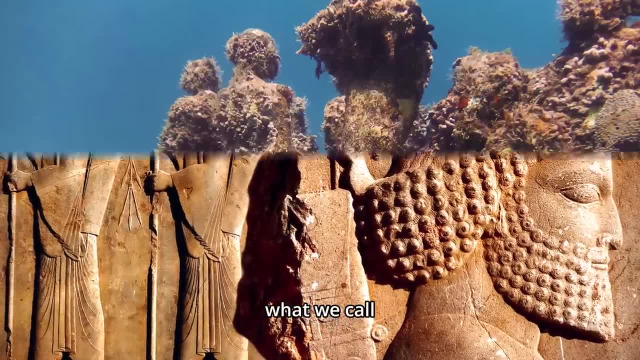 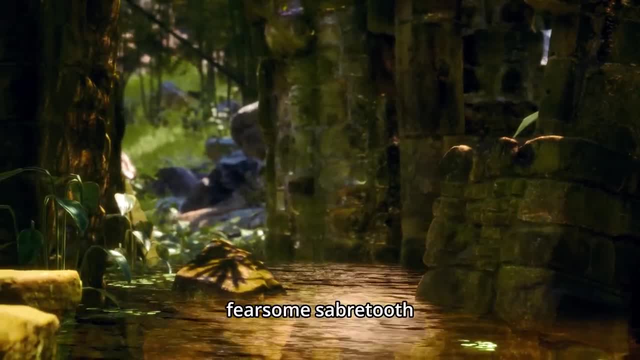 Here, in the enigmatic confines of what we call bone caves, lie the jumbled remains of an ancient menagerie: Bison lions, fearsome saber-toothed tigers, massive rhinoceroses and cunning wolves, among other prehistoric mammals. 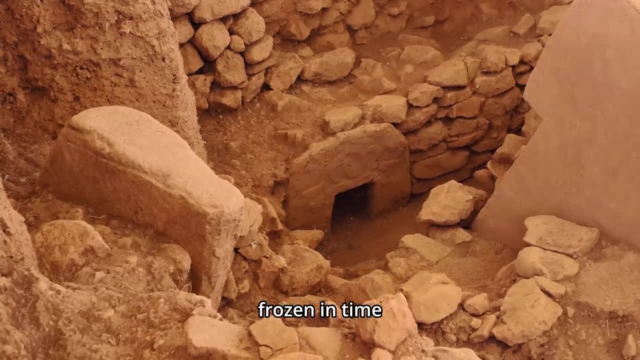 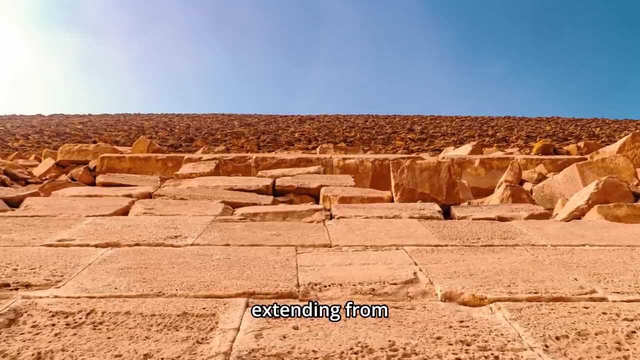 rest side by side, their earthly journey forever frozen in time In the annals of time. a chilling mystery unfolded across a frigid expanse extending from the Yukon to the icy realms of Alaska and far into the hinterlands of northern Siberia. In the 11th millennium BC, an astonishing calamity struck, as if nature herself had exhaled a breath of frost that instantly froze and preserved in time a multitude of warm-blooded creatures, These once vibrant mammals perfectly adapted to temperate climates. 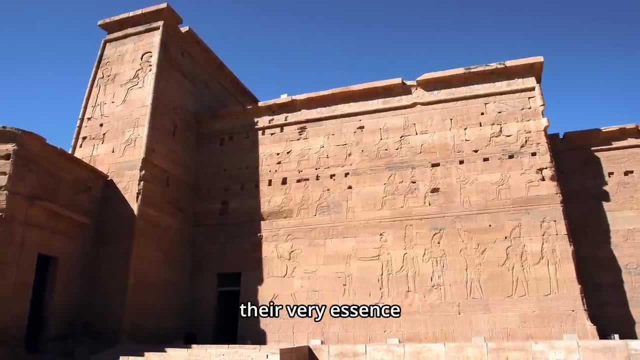 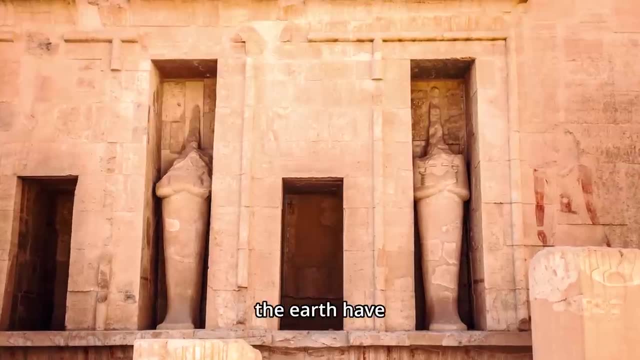 found themselves entombed in the unforgiving grasp of permafrost, Their very essence locked in a cryogenic embrace. The whispers of history, like secrets hidden deep within the earth, have yielded a striking revelation In various corners of the world. 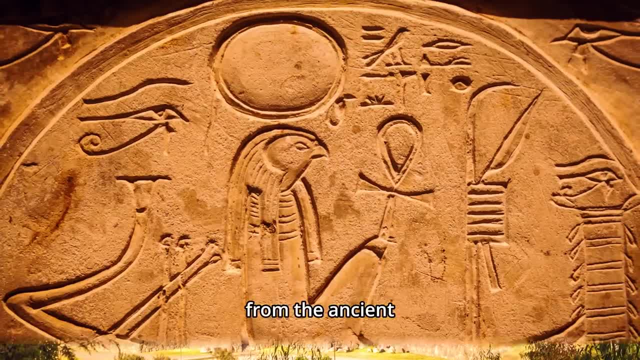 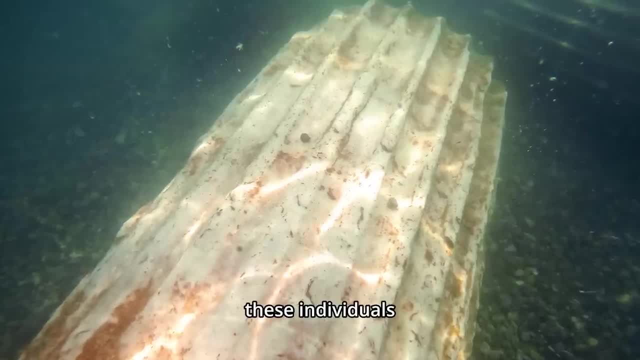 from the heartlands of North America to the pristine realms of Brazil, from the ancient landscapes of India to the rugged terrains of the Balkans, the remains of countless humans have been unveiled. These individuals, hailing from diverse ethnic backgrounds, sought refuge within the subterranean sanctuaries of caves. 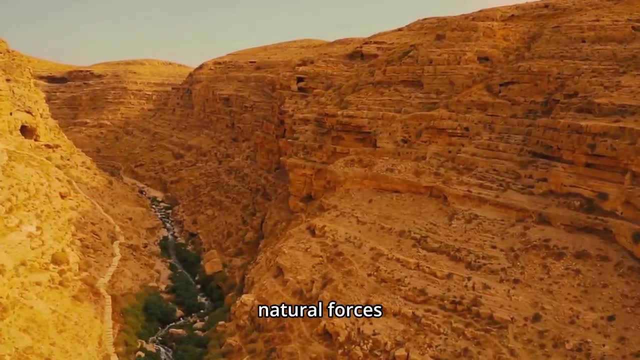 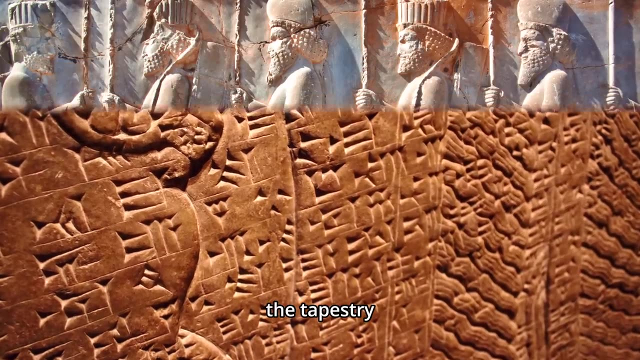 There they faced a fate ordained by natural forces, where they took their final breaths, leaving behind an indelible testament to the mysteries of ancient times. The tapestry of human history unfolds amidst the relentless grip of ice ages, a symphony of geological and climatic upheavals. 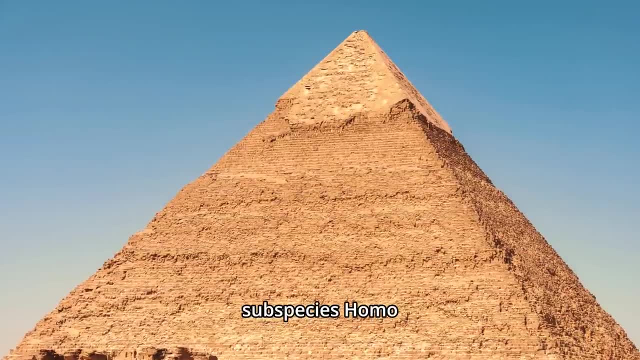 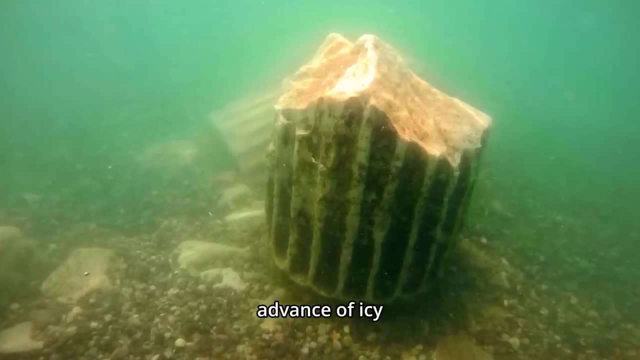 In the midst of these chilling epochs, our own subspecies, Homo sapiens sapiens, took its first breaths. Millennia were marked by an unyielding advance of icy expanses, a haunting ordeal etched deeply into the collective memory of our forebears. 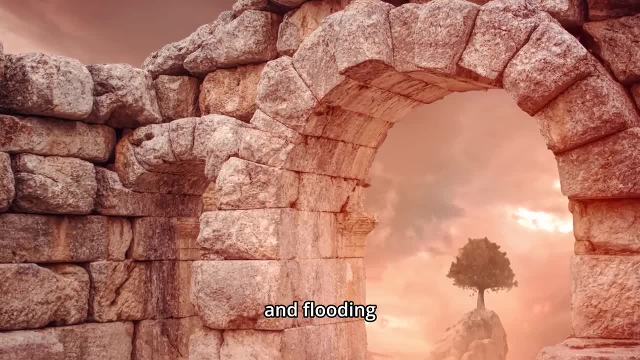 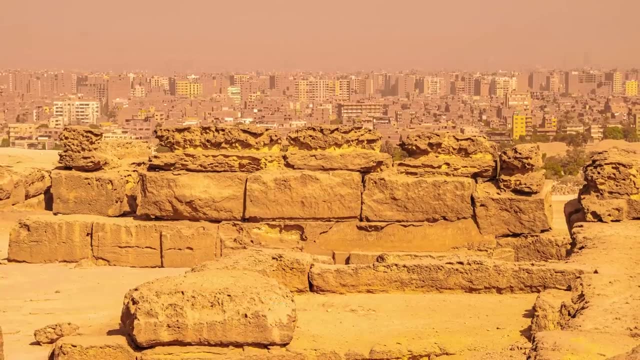 The rhythm of their existence mirrored the cadence of freezing and flooding, a testament to their resilience amidst a world gripped by fear. The closing act of these ice-cold epochs- the last 7,000 years of melting and thawing- was perhaps the most harrowing. 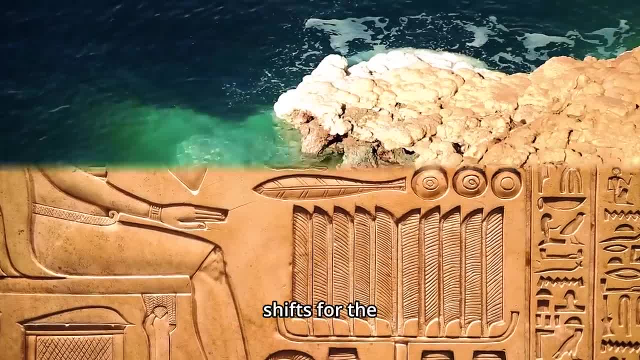 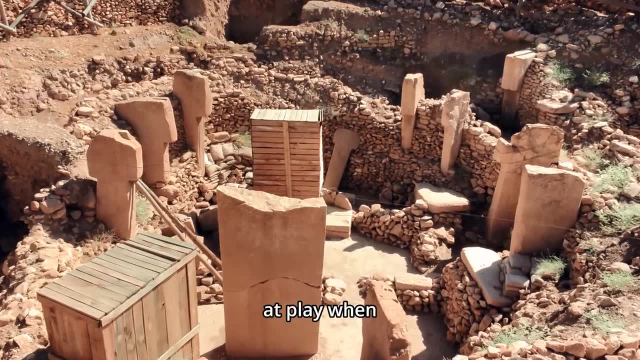 It defies explanation and is the only act of gradual climatic shifts. for the astonishing celerity of this deglaciation hints at extraordinary uncharted forces at play When we follow the tangled threads of evidence weaving together the echoes of catastrophe. 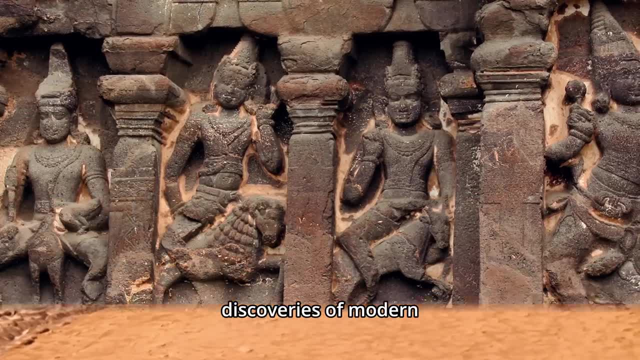 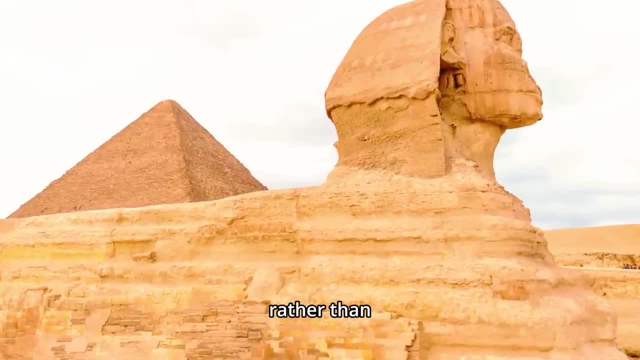 that resonate through the mythologies of cultures spanning the globe. with the discoveries of modern archaeology, a striking portrait emerges. It paints a vivid tapestry of historical truths, rather than fanciful tales or allegorical fables. While Greek historians once wove threads of connection, 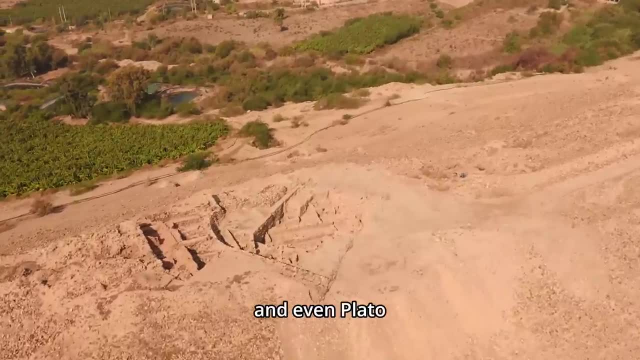 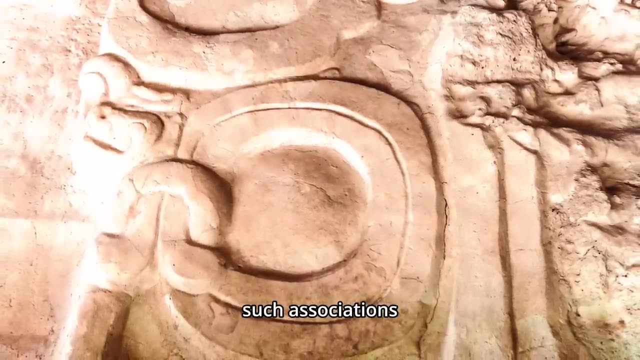 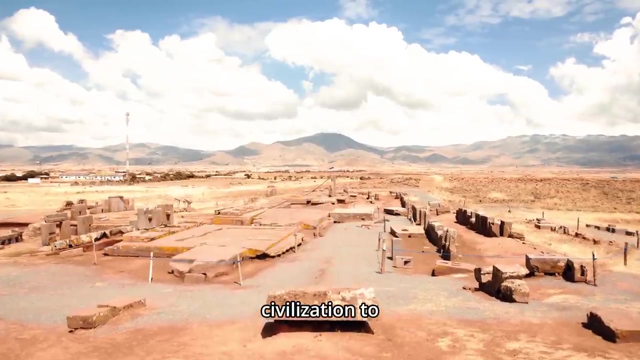 between ancient Egypt and the fabled Atlantis, and even Plato was believed to have gleaned his knowledge of Atlantis from Egyptian origins. contemporary archaeology often dismisses any such associations. Instead, the prevailing view restricts the birth of Egyptian culture and civilization to the relatively recent window of the last 5,000 to 7,000 years. 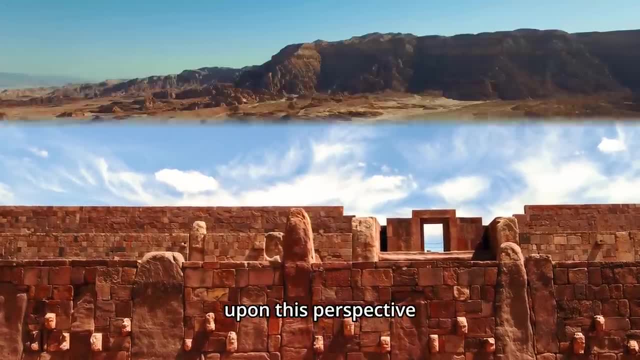 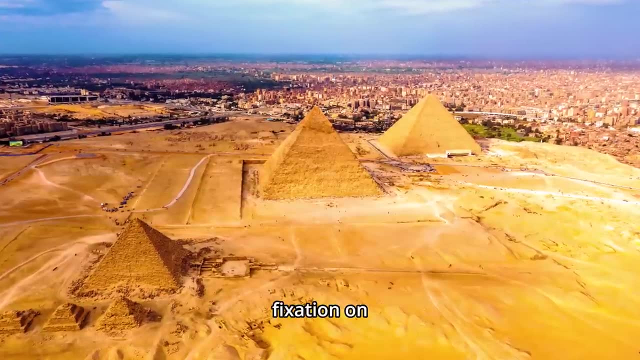 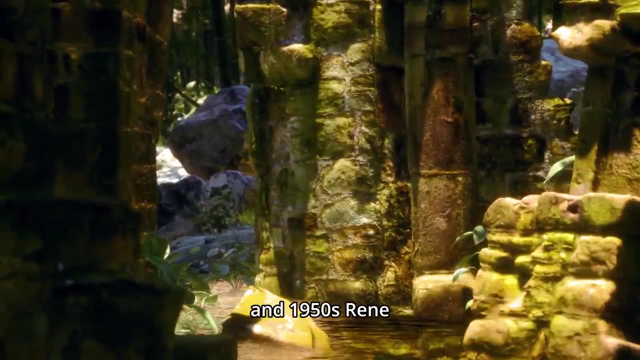 However, skeptics have cast doubts upon this perspective. They argue that the historical record is riddled with conspicuous gaps, and mainstream Egyptology's fixation on meticulous cataloguing often overshadows broader and more intriguing possibilities During the 1940s and 1950s. 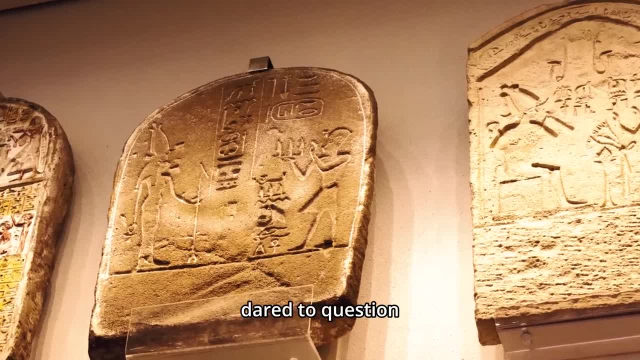 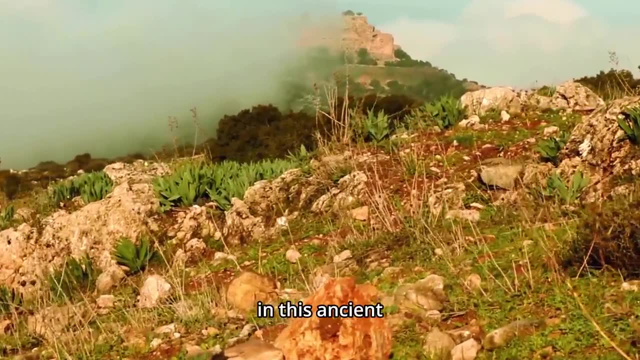 René Schwaller de Lubitsch, a French scholar and occultist, dared to question the conventional interpretations of Egyptologists. His fascination with Egypt led him to reside in this ancient land for 12 years, where he embarked on an exhaustive study of monuments and temples. 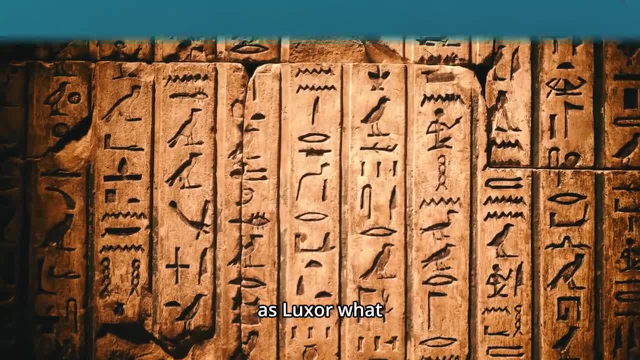 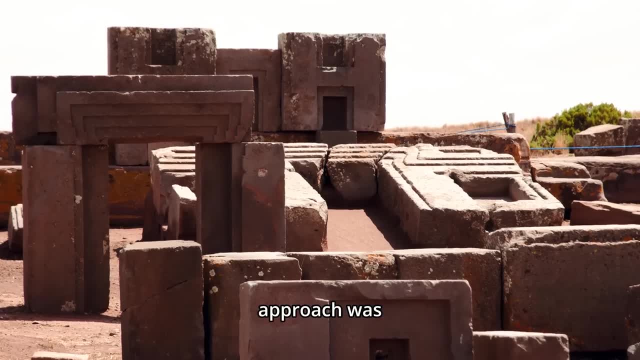 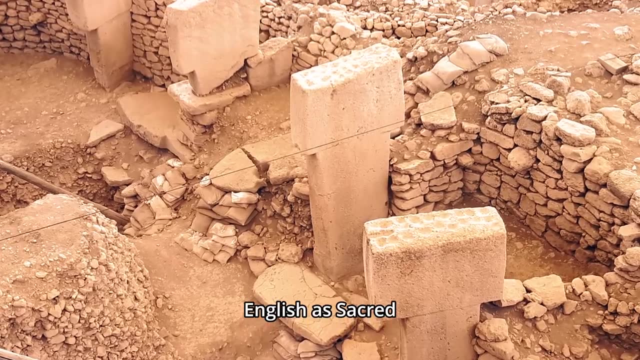 with a particular emphasis on the Grand Temple of Thebes, known as Luxor. What emerged from his research was a profound and symbolic perspective on ancient Egypt. This unique approach was encapsulated in his monumental work The Temple of Man, later translated into English as Sacred Science. 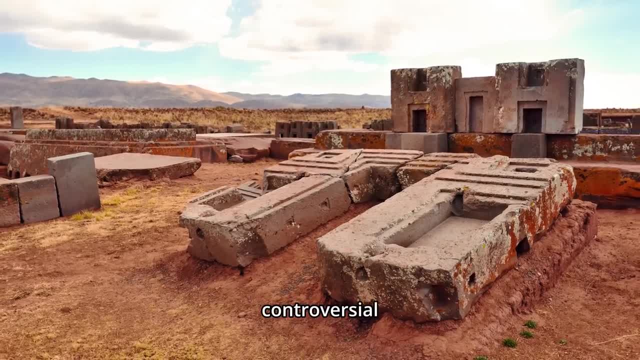 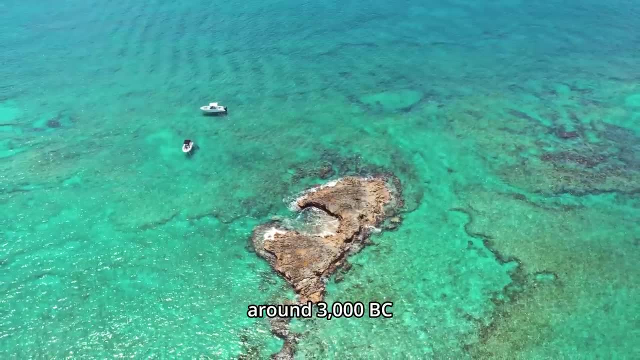 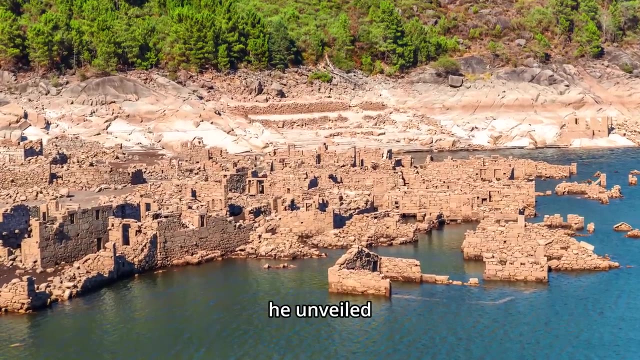 Schwaller de Lubitsch's extensive research led him to a controversial yet compelling conclusion. He argued that Egyptian civilization predated the commonly accepted timeline of around 3000 BC proposed by traditional Egyptologists. In his meticulous investigations, he unveiled the profound way in which ancient Egyptians 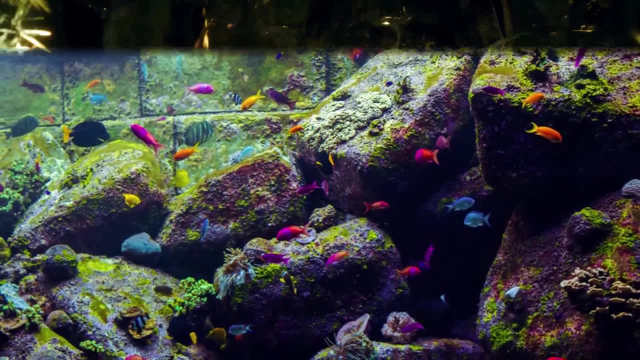 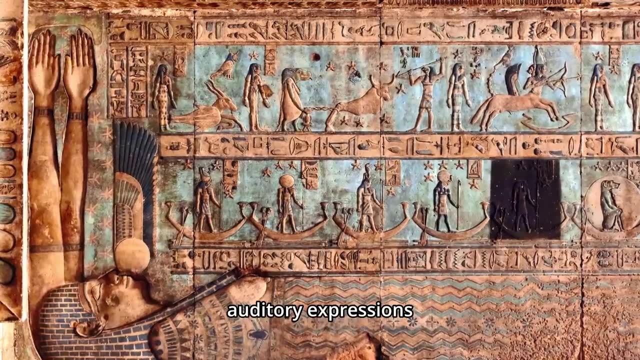 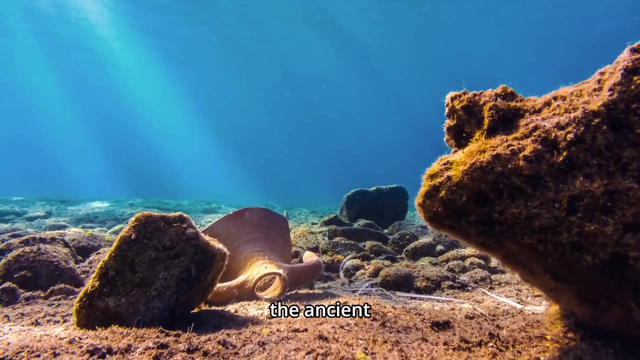 masterfully wove esoteric wisdom into their culture. This knowledge was not confined to written records, but was intricately integrated into their visual arts, auditory expressions, conceptual frameworks and even architectural symbolism. Schwaller de Lubitsch's research revealed that the ancient Egyptians 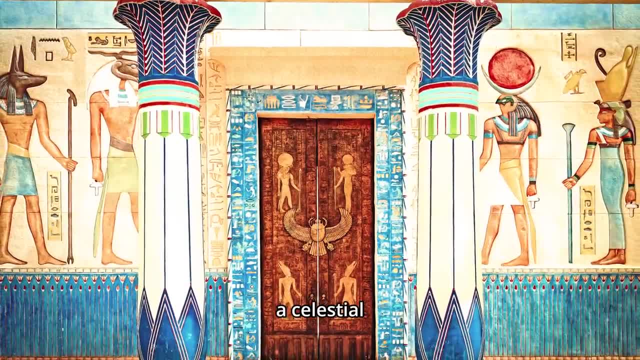 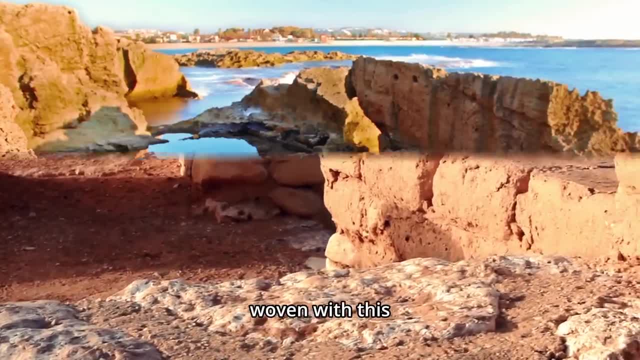 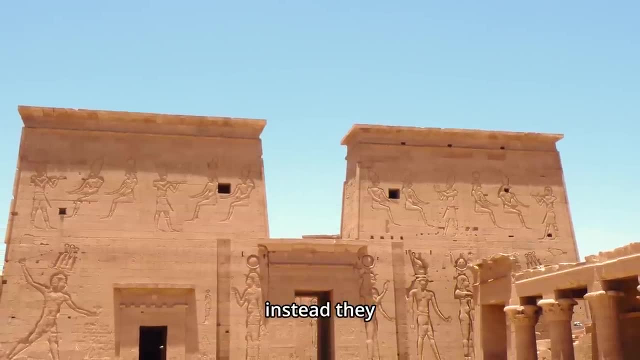 had a profound understanding of the precession of the equinoxes, a celestial phenomenon with a 25,900-year cycle. Their culture and civilization were intricately woven with this knowledge, and they intentionally sought to transcend mere cerebral intelligence. Instead, they delved into a realm of deeper wisdom. 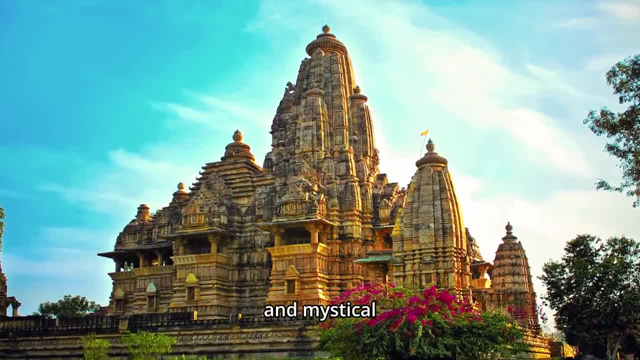 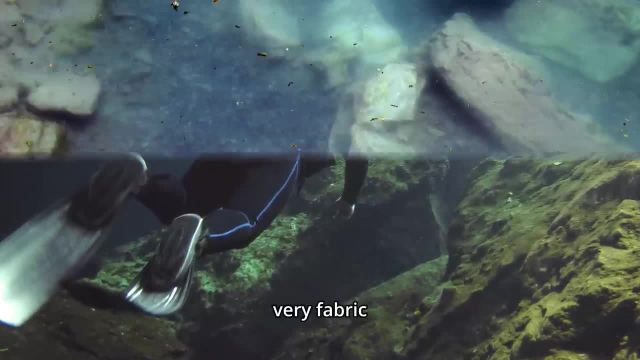 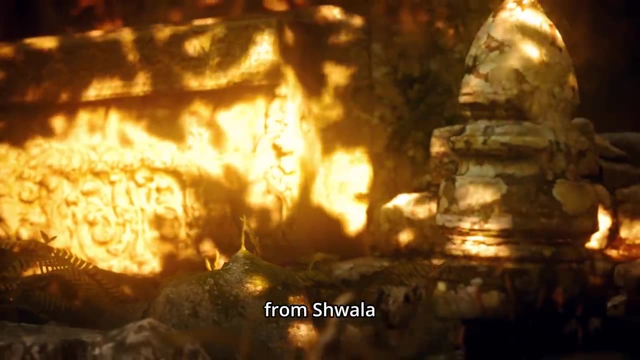 incorporating their understanding of the cosmos into their religious and mystical practices. Through sophisticated astronomical observations, they embedded these cosmic insights into the very fabric of their culture. In the decades that followed, a host of diligent investigators drew inspiration from Schwaller de Lubitsch's groundbreaking research. 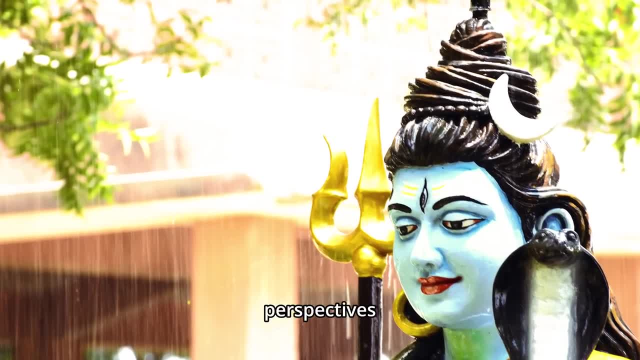 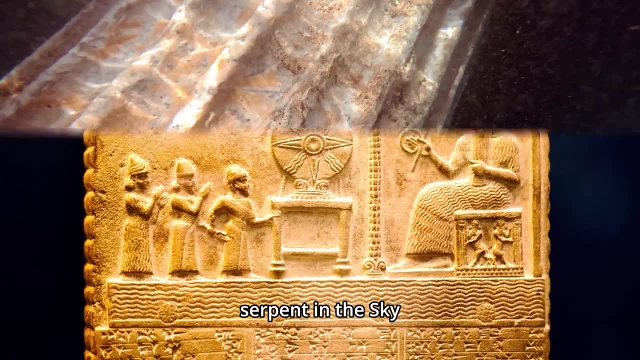 Building on his work, they offered their own unique perspectives and theories. These scholars included John Anthony West, known for his book Serpent in the Sky, Robert Temple, the author of The Serious Mystery, and the dynamic duo of Robert Bauval and Adrian Gilbert. 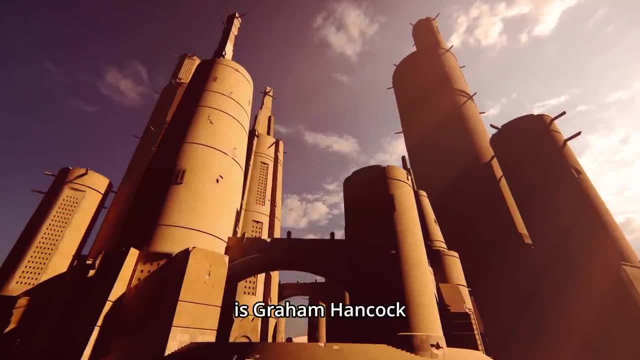 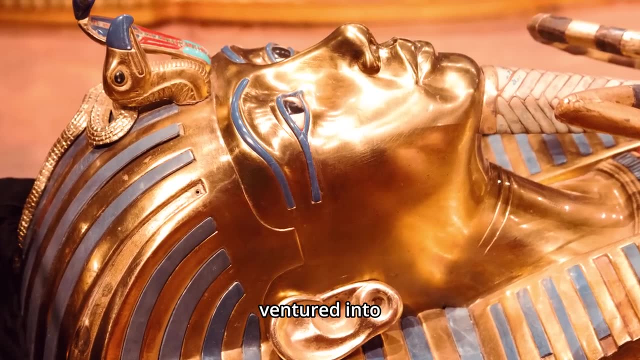 who co-authored The Orion Mystery. Not to be overlooked is Graham Hancock, who made a profound impact with his work Fingerprints of the Gods. Together, they ventured into the depths of history and archaeology, seeking to unveil the mysteries of our ancient past. 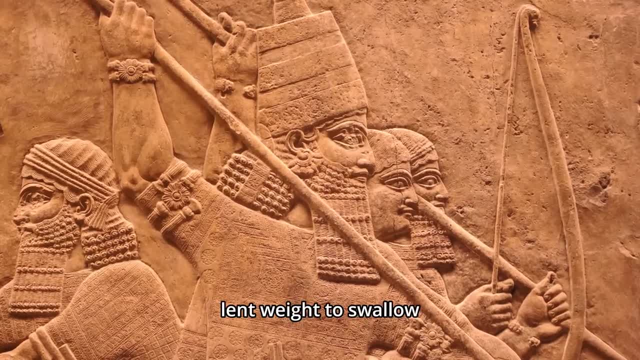 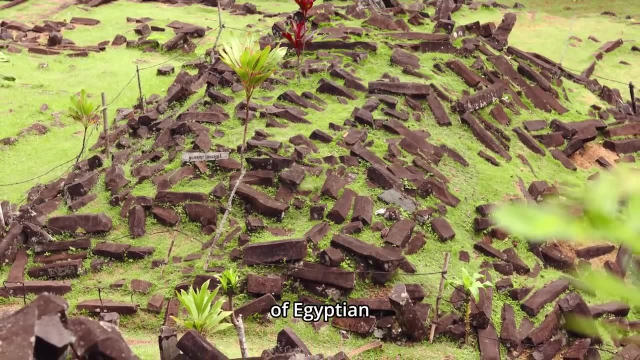 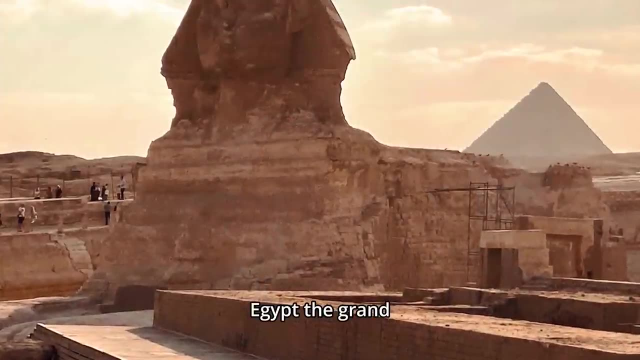 The collective research of these investigators lent weight to Schwaller de Lubitsch's audacious claim. Their findings suggested that, long before the established timeline of Egyptian civilization, the Nile Valley was home to the descendants of Atlantis. The enduring monuments of Egypt, the grand temples and majestic pyramids. 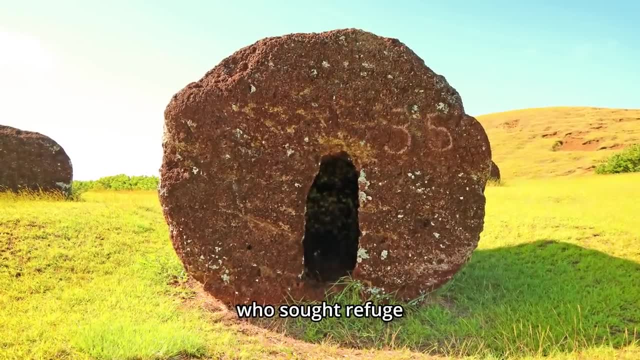 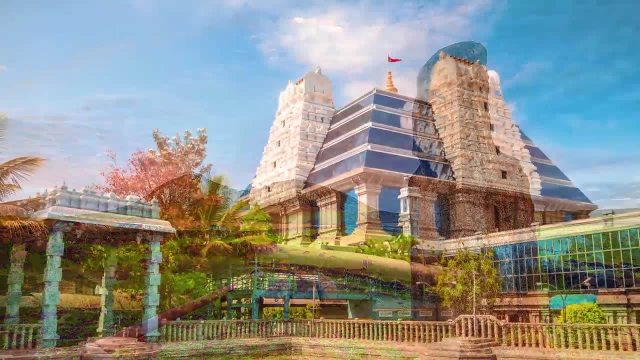 they argued, stood as the legacy of these resilient survivors who sought refuge in the valley. Gurdjieff's accounts extend to the survivors of Atlantis and their journey to ancient Egypt, detailing the lasting spiritual impact they had on the region. He narrates the story of the erudite Society of Akhaldans. 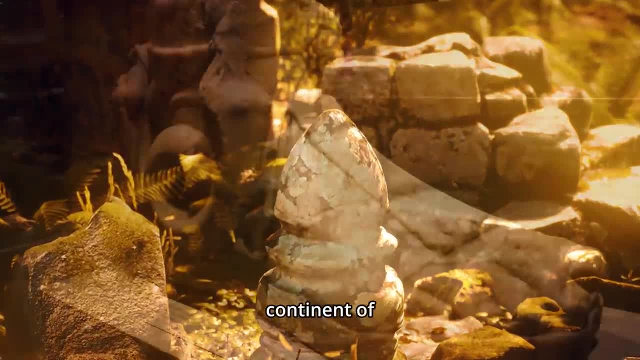 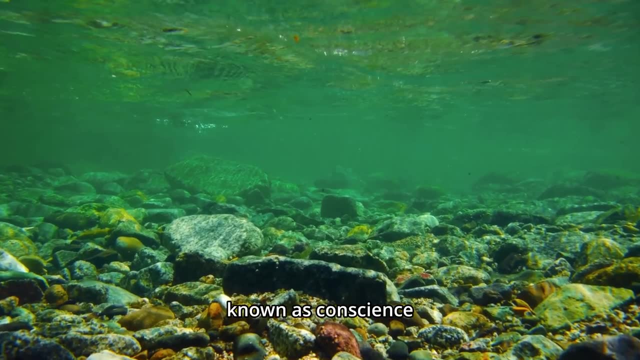 which had its origins on the continent of Atlantis tens of thousands of years prior to its eventual demise, The emblem of the Society known as Conscience took the form of an allegorical being akin to, and possibly a precursor of, the Sphinx. 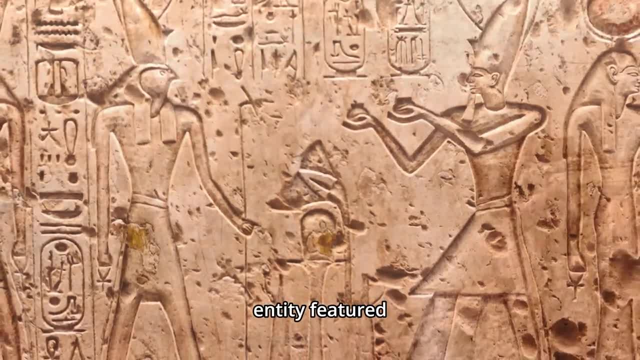 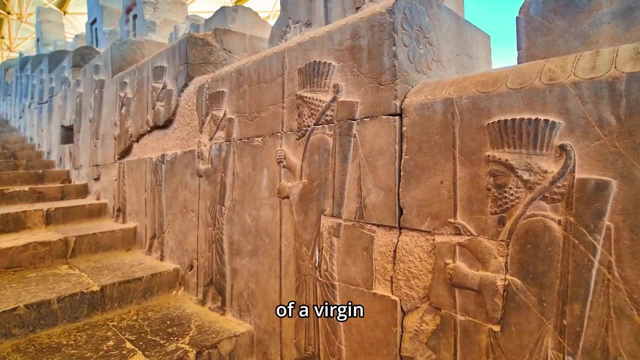 This enigmatic entity featured the body of a bull, the four powerful legs of a lion, the expansive wings of an eagle and the nurturing breasts of a virgin seagull, The name Akhaldan, symbolizing impartial love. Gurdjieff conveyed that the name Akhaldan 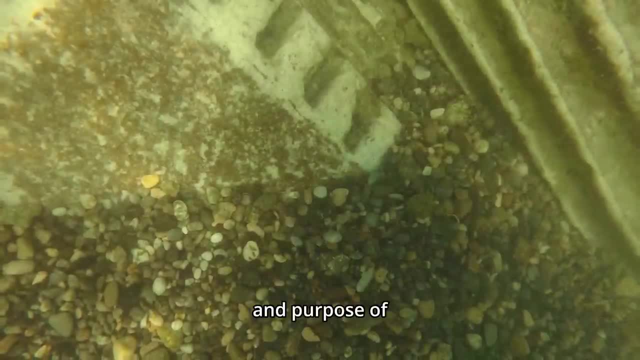 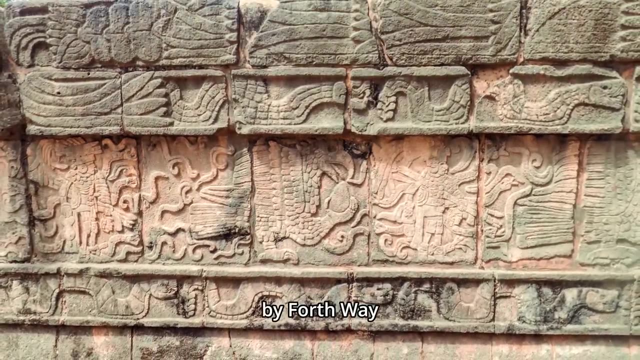 held the significance of the striving to attain an understanding of the essence and purpose of the Supreme Being. This resonates with the ancient Egyptian religious perspective as explored by fourth-way author William Paterson. In Egyptian beliefs, the universe was perceived as a harmonious 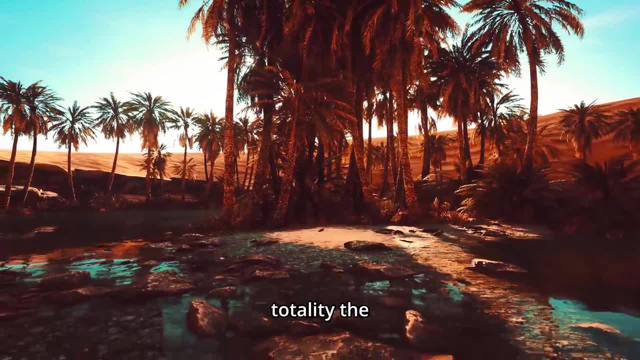 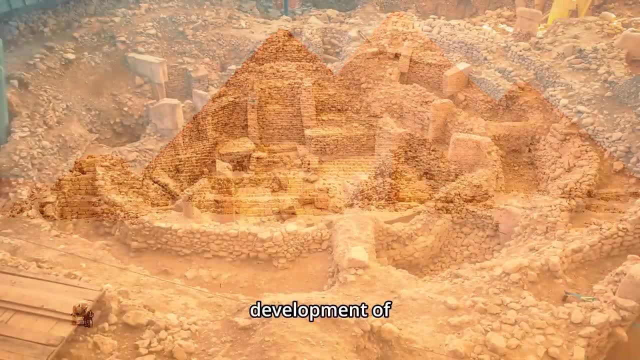 cyclical motion enveloped within an immutable totality. The impact of the Atlantean society on ancient Egypt extended to various aspects, with notable achievements such as the development of the telescope and the construction of what Beelzebub referred to as observatories, the pyramids. 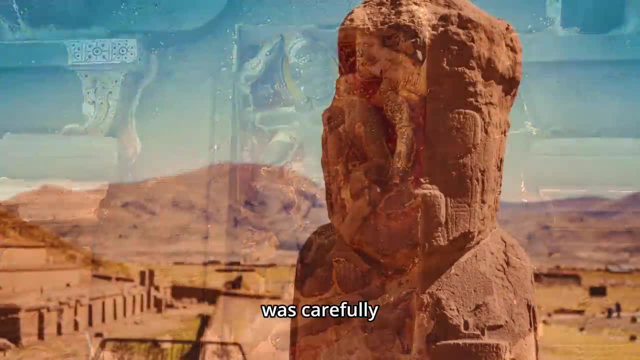 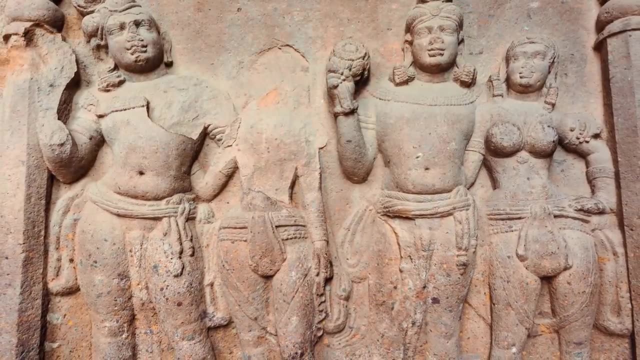 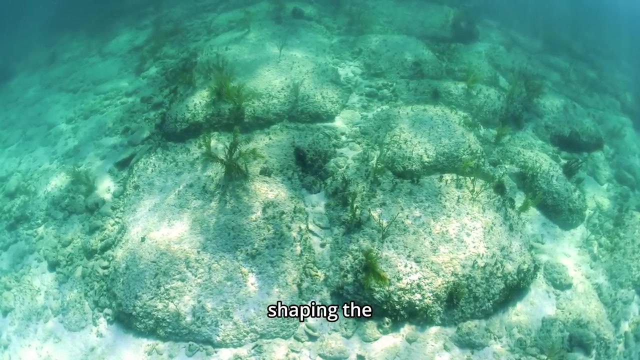 Within these pyramids, an advanced telescope was carefully positioned. Expert astronomers utilized it to study distant suns and planets within the cosmos. Moreover, they skillfully regulated and intentionally directed the movement of the encompassing atmosphere, thereby shaping the desired climate. The influence of the society of Akhaldans. 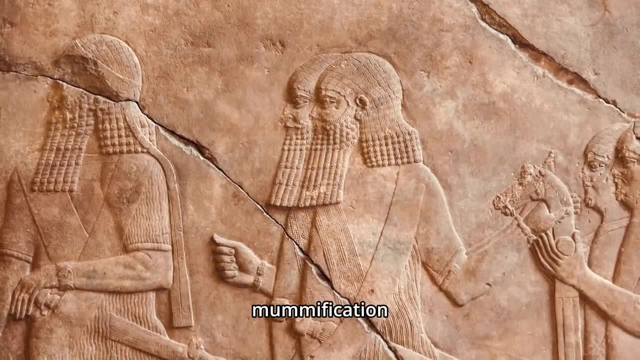 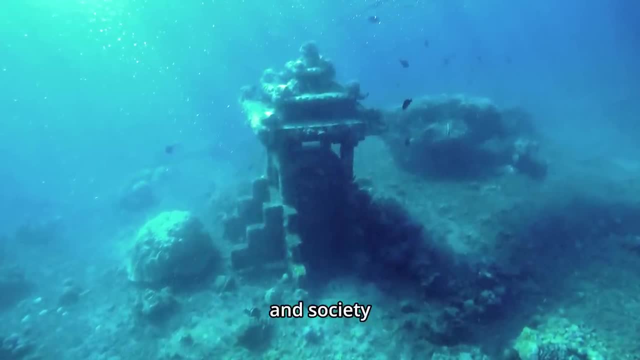 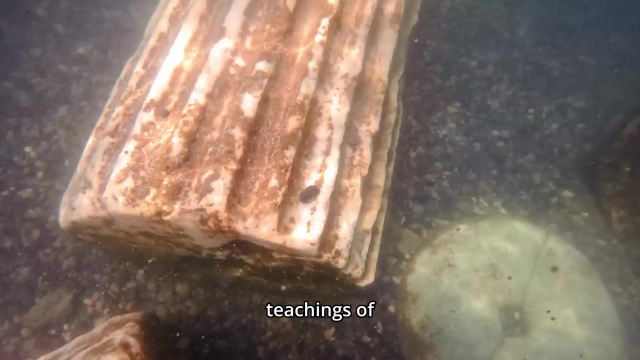 extended to the art of preserving the physical body through mummification. Their contributions, both scientific and spiritual, left a lasting impact on individuals and society. Notably luminaries such as Pythagoras and Moses were among those who benefited from the profound teachings of the Akhaldan society. 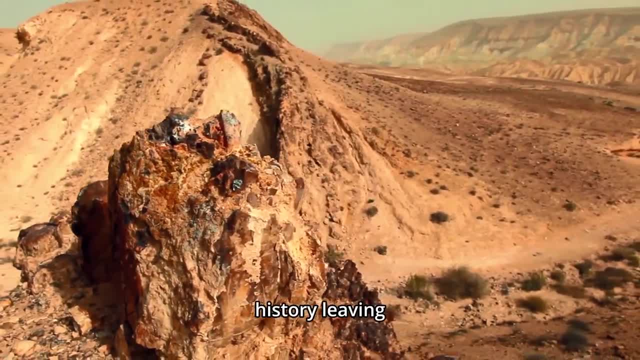 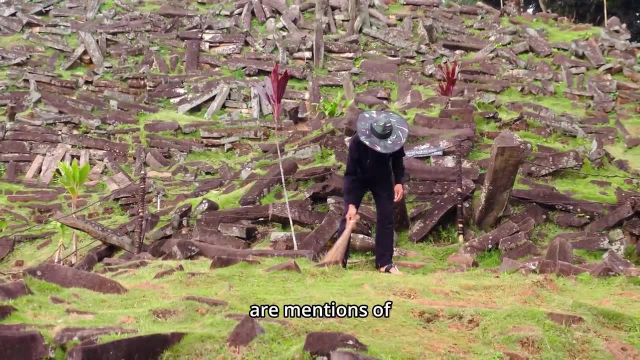 Their knowledge continues to reverberate through the annals of history, leaving an indelible mark on human civilization. In the ancient chronicles of Egypt there are mentions of the seven sages, enlightened souls who hailed from the fabled Atlantis. 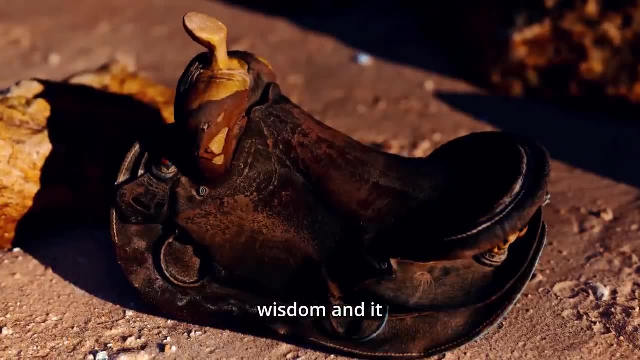 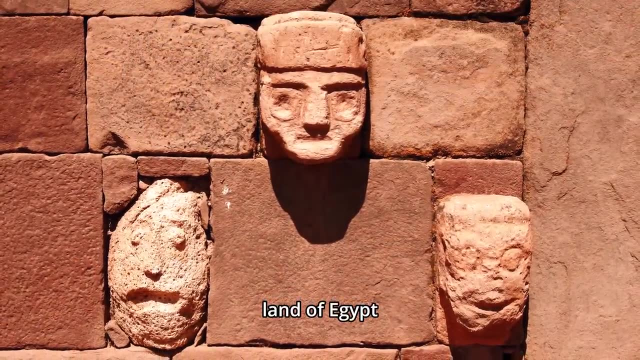 These divine beings possessed profound wisdom, and it was they who orchestrated the design and construction of the awe-inspiring temples and sacred sites that grace the land of Egypt. Guided by their celestial insights, these sages imbued Egypt with a profound spiritual legacy. that endures through the ages. The seven sages, divine remnants of an ancient cataclysm, embarked on a fresh journey following the demise of their island homeland, known as the homeland of the primeval ones. In this distant sanctuary, most of its divine inhabitants met their watery fate. 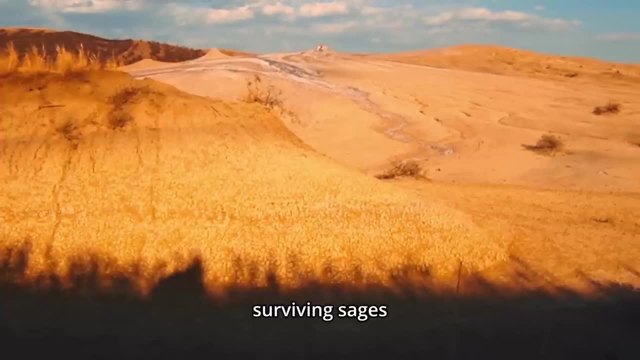 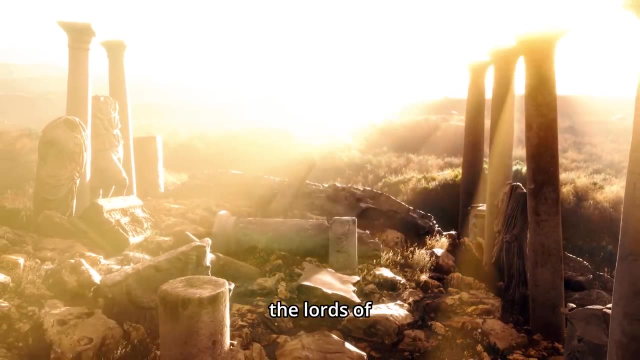 As they arrived on the sacred soil of Egypt, these surviving sages transformed into the builder gods, shaping the foundations of time itself. They emerged as the lords of light, ghosts, ancestors and the seniors of creation, bestowing their radiant illumination upon this land. 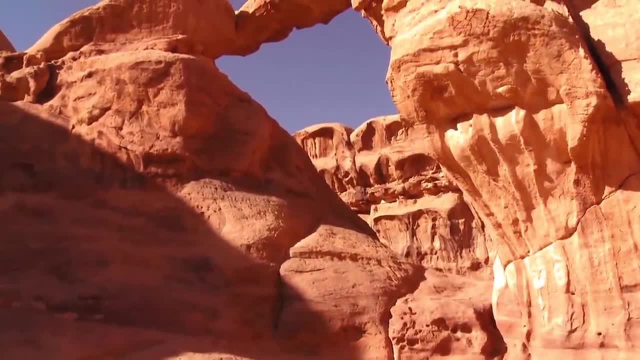 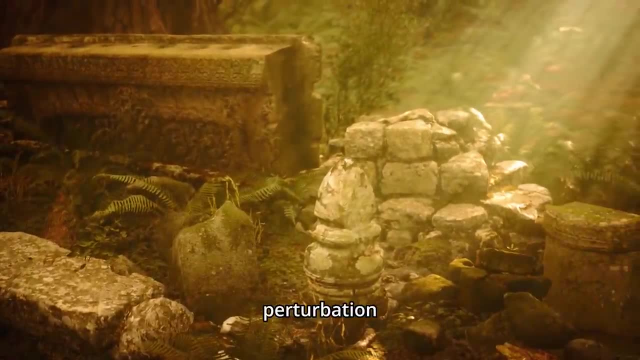 uniting gods and humanity alike at the dawn of existence. Indeed, a striking correlation emerges between Gurdjieff's account of the second trans-Apollonian perturbation, causing Atlantis to descend within the planet, and the surviving members of Beelzebub's tribe. 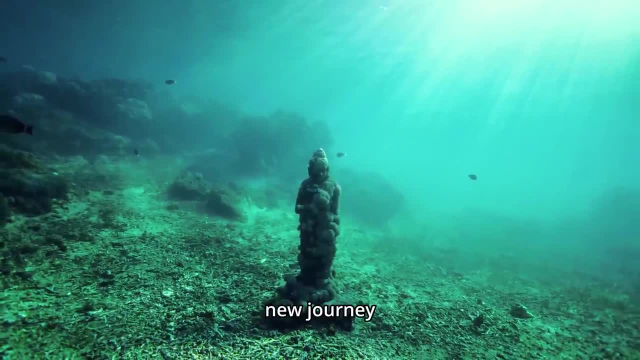 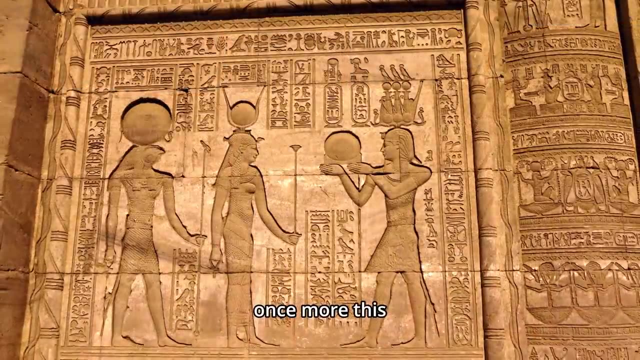 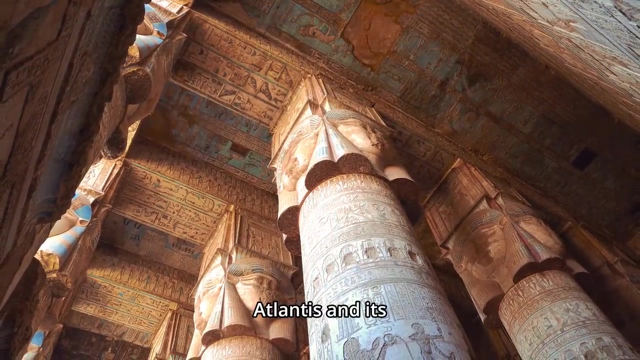 and the illustrious society of Akhaldans. They embarked on a new journey, resettling in the region of Ethiopia and Egypt, where they ignited the flames of civilization once more. This alignment between historical narratives is nothing short of precise: Edgar Cayce's accounts of Atlantis and its inhabitants' migration. 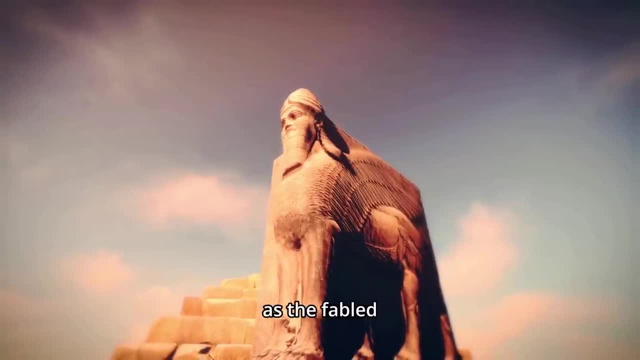 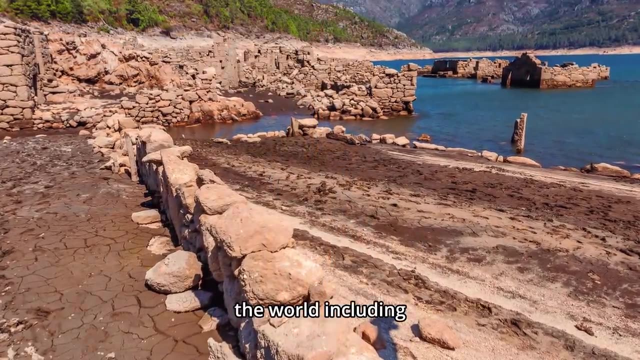 shed intriguing light on early Egyptian history. As the fabled continent succumbed to its final destruction, Atlanteans embarked on journeys that led them to the far corners of the world, including Western Europe, the Americas, Africa and Egypt, Through Cayce's life readings. 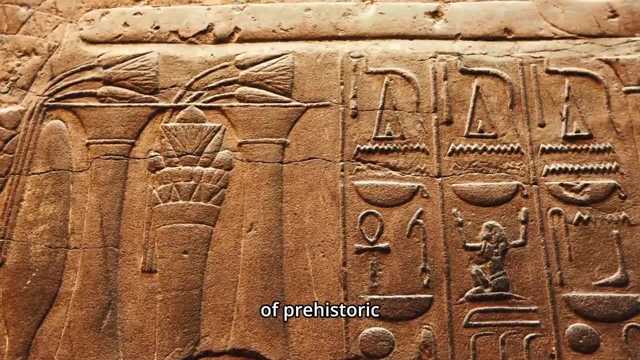 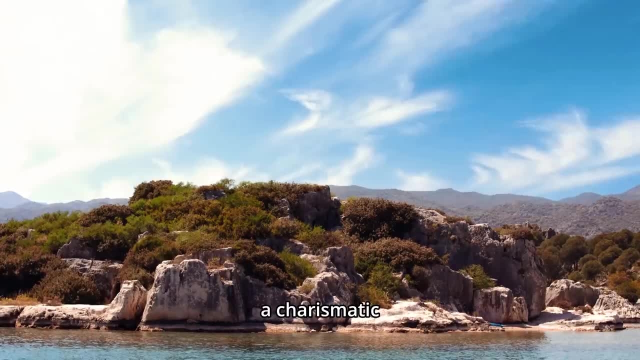 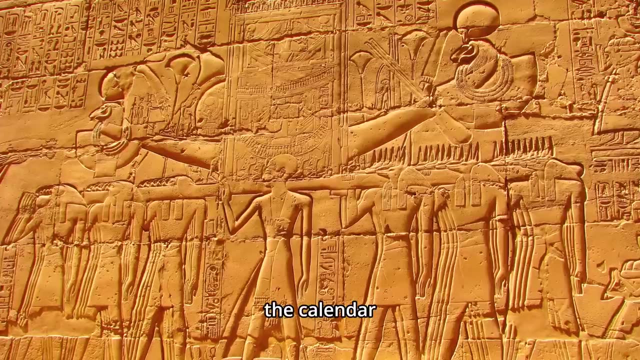 a vivid tapestry of prehistoric Egypt around 10,000 to 11,000 BC begins to take shape. In the dawn of ancient history, a charismatic leader named Arat led his people from the Caucasian region into the land of Egypt well before the turning of the calendar to 10,500 BC. 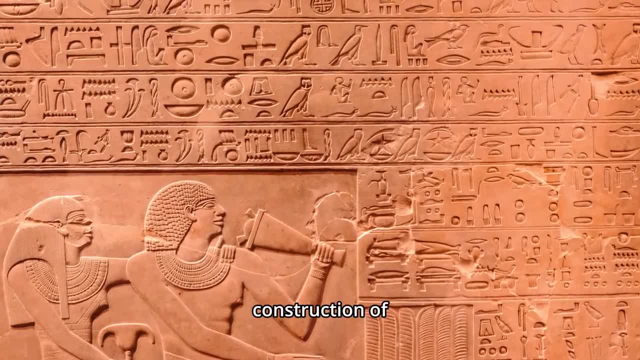 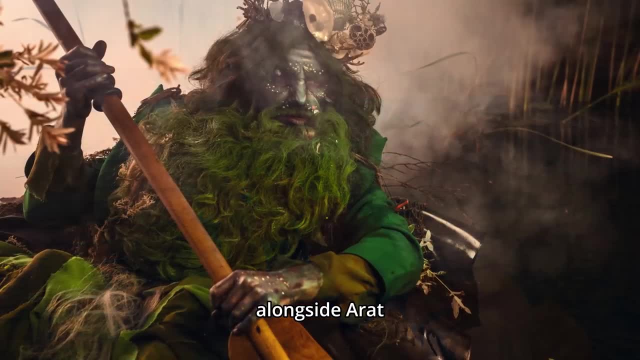 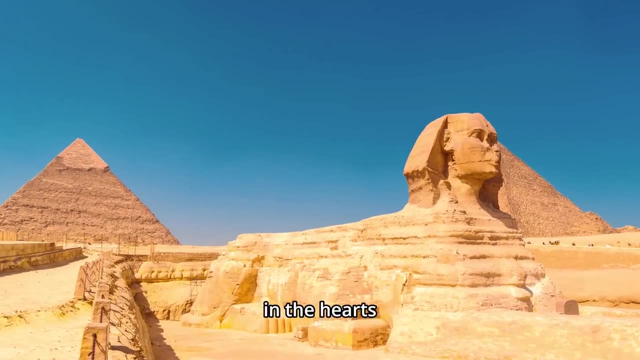 In his reign, Egypt saw the magnificent construction of the Great Pyramid of Giza and the enigmatic Sphinx, monumental symbols of his rule. Alongside Arat, there emerged a revered priest named Rata, who labored to instill a sense of order and spirituality in the hearts of the people. 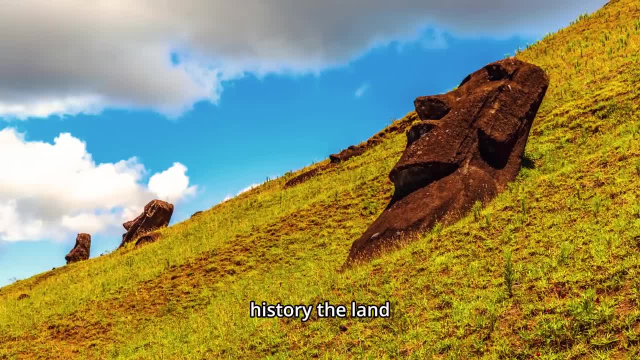 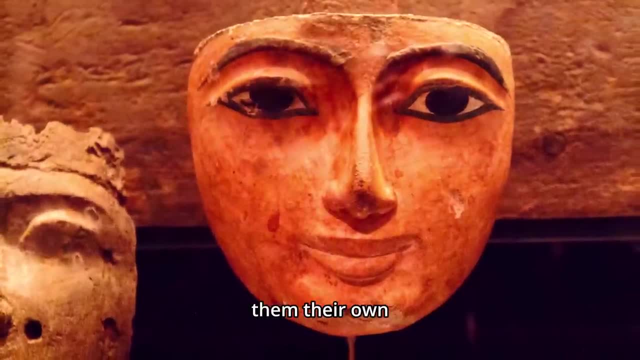 Around this transformative period in Egypt's history. the land welcomed a tide of refugees escaping the imminent demise of Atlantis. These newcomers brought with them their own traditions and wisdom, mingling their heritage with the ancient soil of the Nile, where they hoped to find a new beginning. 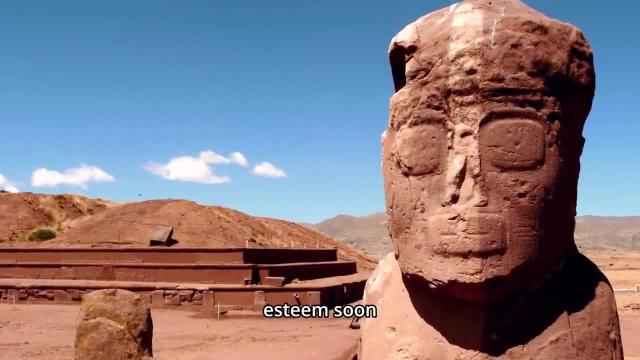 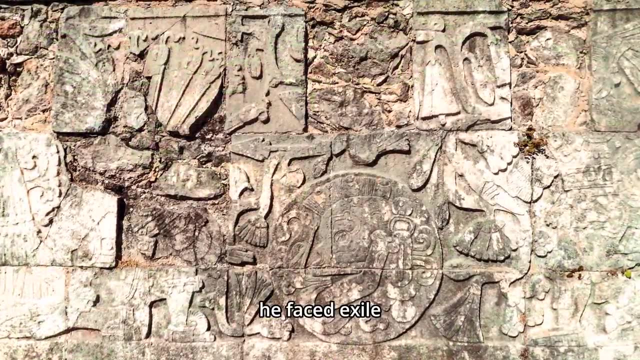 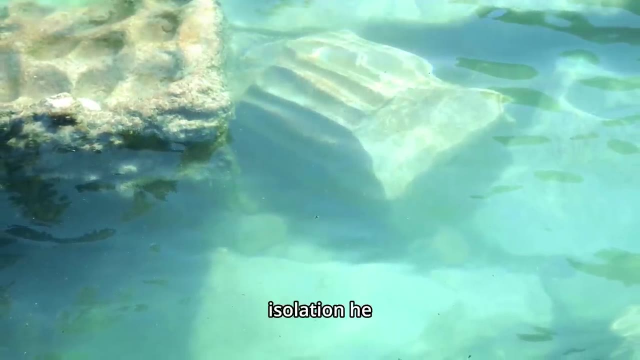 The priest initially held in high esteem, soon found himself entangled in the complex web of political strife and rivalries. As a result, he faced exile to the region that would, in time, come to be known as Abyssinia. During his period of isolation, he remained a beacon of wisdom and contemplation. 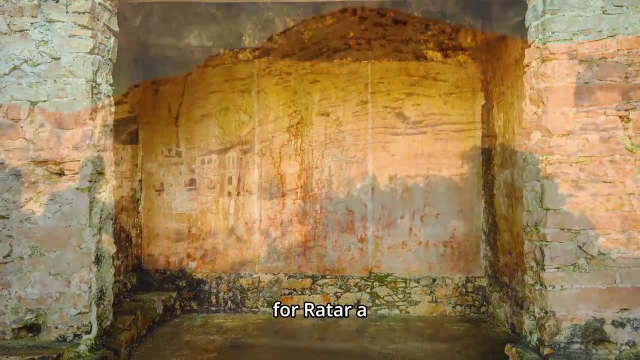 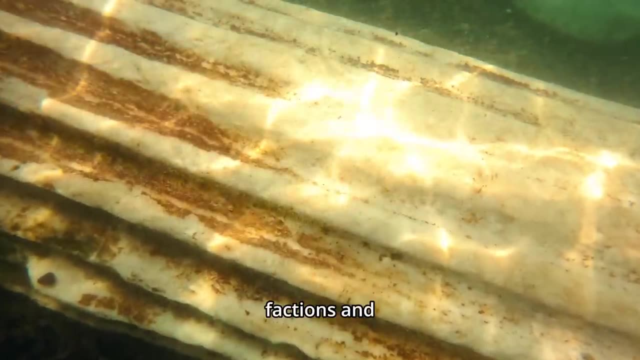 However, destiny had other plans for Rata. A time came when his unparalleled insights and diplomatic skills were urgently needed to reconcile the various factions and interests that had arisen in Egypt. Thus he was summoned back from his sojourn in Abyssinia. 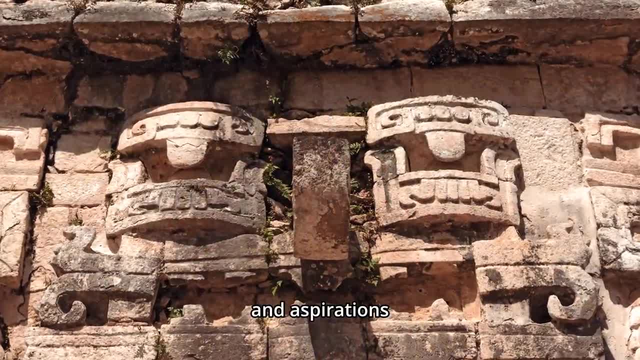 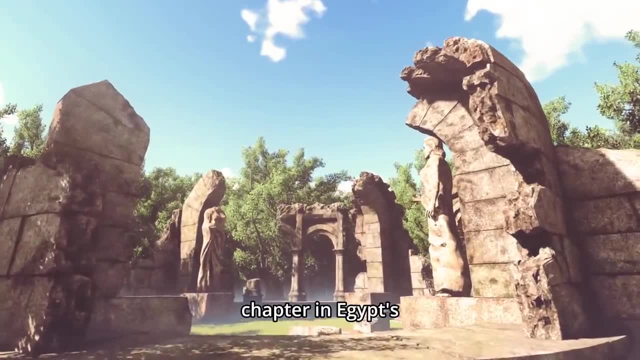 entrusted with the monumental task of harmonizing the activities and aspirations of the ruling elite, the native Egyptians and the influx of Atlantean settlers, forging a new chapter in Egypt's history, Guided by the wisdom of priest Rata and the Atlantean settlers. 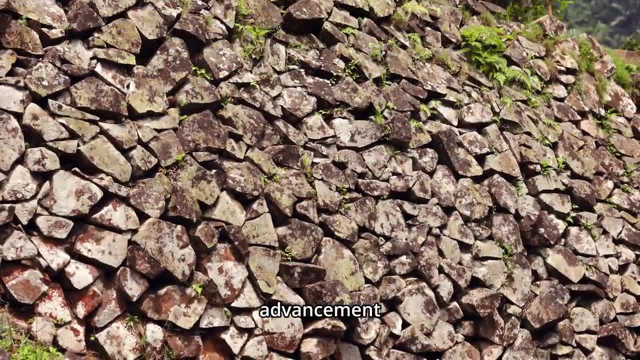 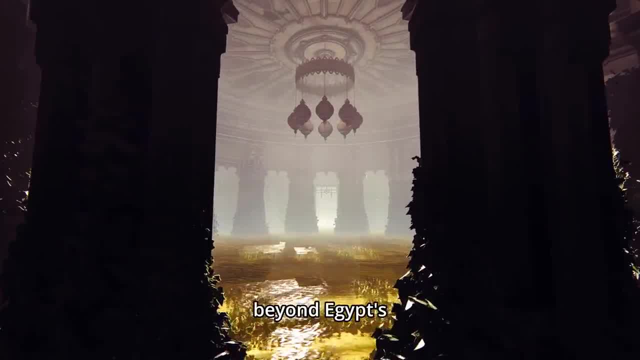 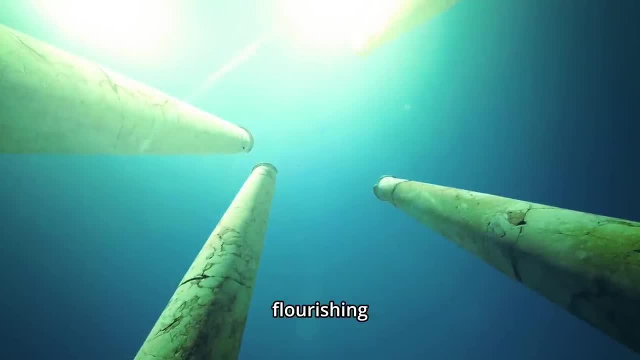 Egypt entered a golden age of both material and spiritual. Together, they initiated a cultural renaissance, their ambitious vision stretching beyond Egypt's borders to touch the farthest corners of the known world. It was a time of enlightenment and intellectual flourishing, a period when art, science and spirituality found fertile ground in the Nile Valley. 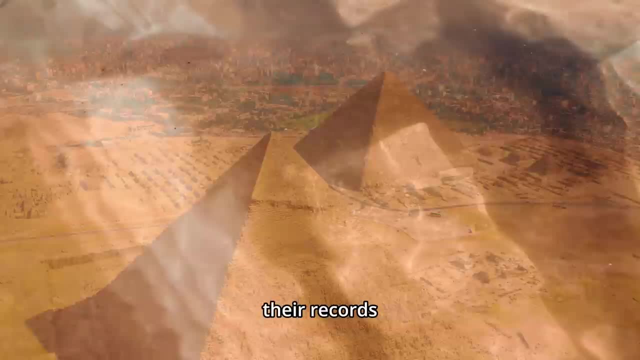 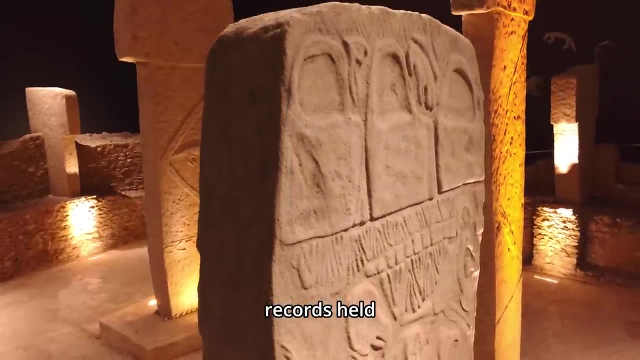 In Egypt, the Atlanteans preserved their records, a testament to their lost civilization, awaiting discovery in the sands of time. These records held the secrets of their advanced society, yearning to reveal the hidden truths of a bygone era to those who would come to seek them. 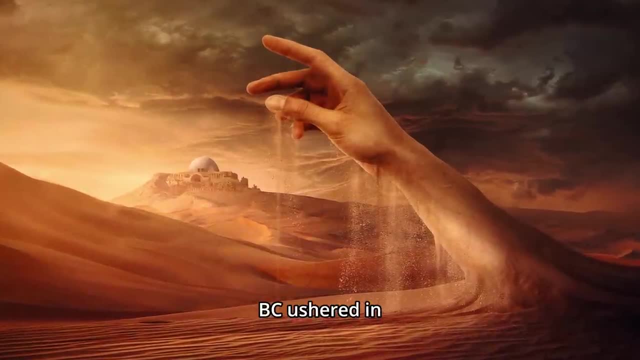 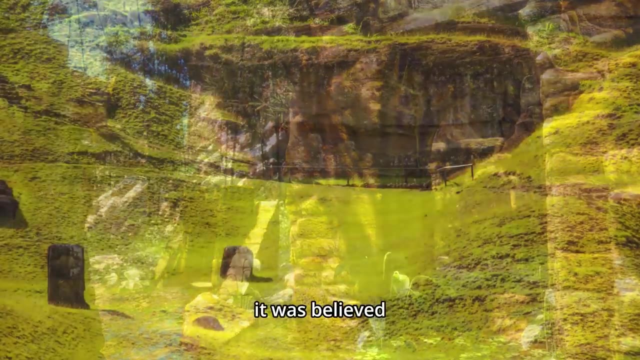 In the vast canvas of history. the 11th millennium BC ushered in what was often referred to as Egypt's Golden Age. During this remarkable epoch, it was believed that the gods themselves ruled over the land. This era coincided with the processional Age of Leo. 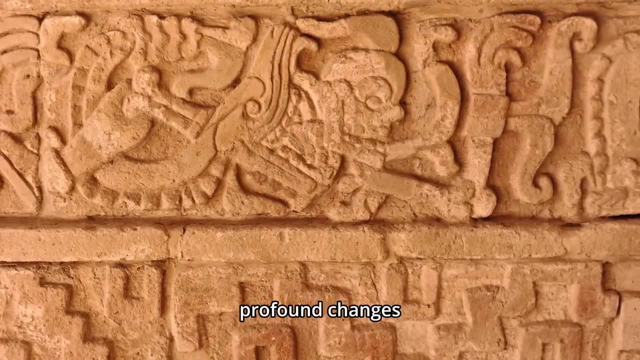 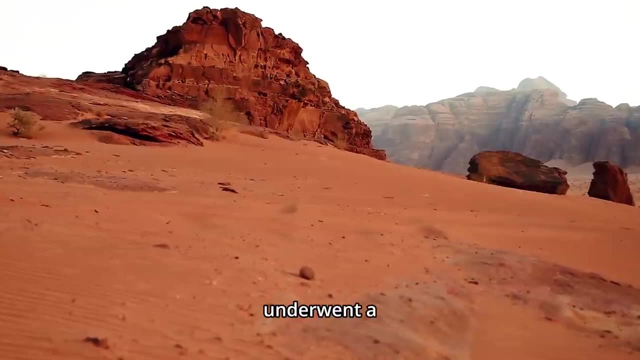 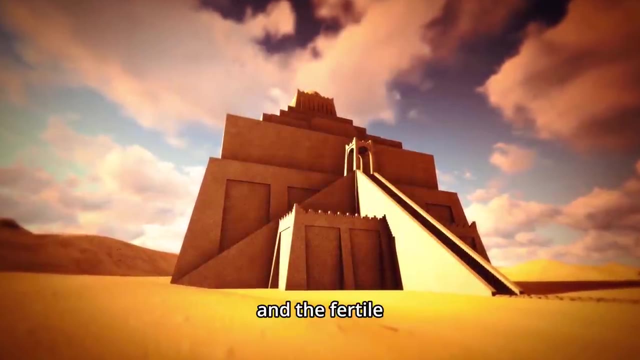 a cosmic alignment that bore witness to profound changes on Earth. As the massive glaciers in the northern hemisphere relinquished their icy grip, the world underwent a transformative shift. With the receding ice, rainfall patterns experienced a resurgence and the fertile embrace of the Nile Valley bloomed. The Nile, already a lifeline for Egypt, became even more abundant, fostering a lush and verdant landscape. This was a time when the gods' dominion harmonized with the reinvigorated Earth, creating the fertile ground from which Egypt's magnificent civilization would ultimately grow. 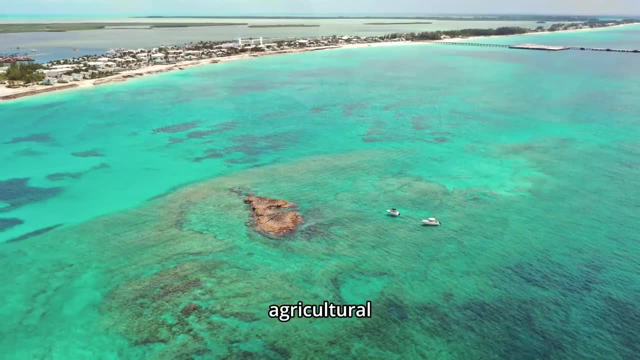 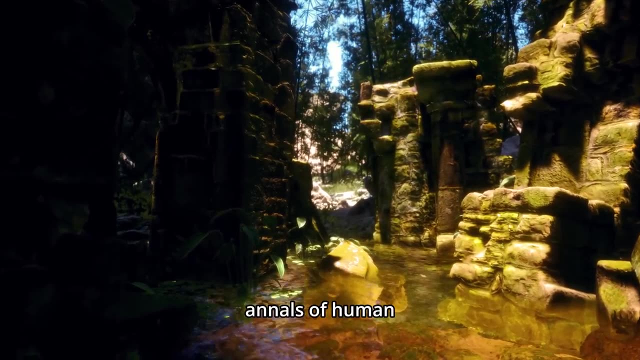 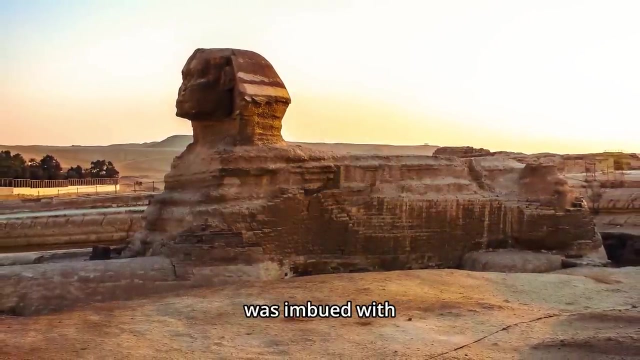 Egypt found itself in the embrace of a precocious agricultural development, a period of transformation that marked one of the earliest agricultural revolutions, a pioneering leap in the annals of human history. This remarkable phase, standing as a testament to ancient innovation, was imbued with the wisdom of those who possessed an advanced understanding of botany and agriculture. 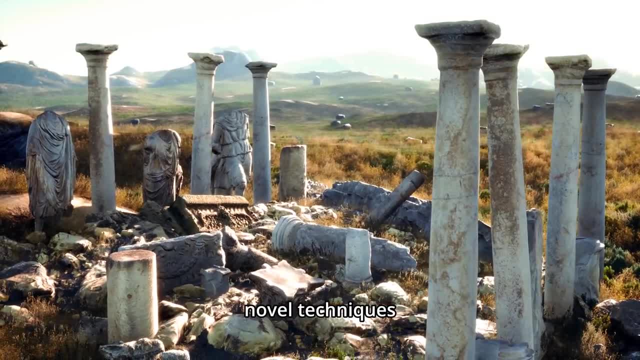 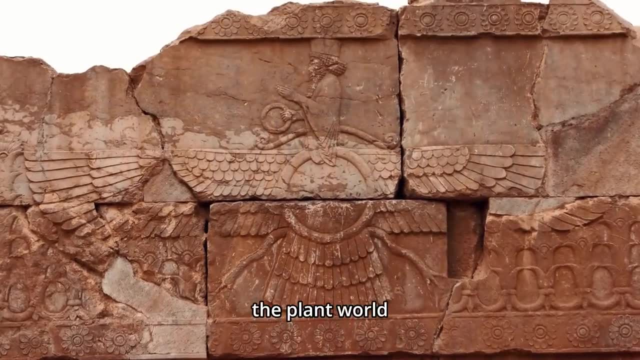 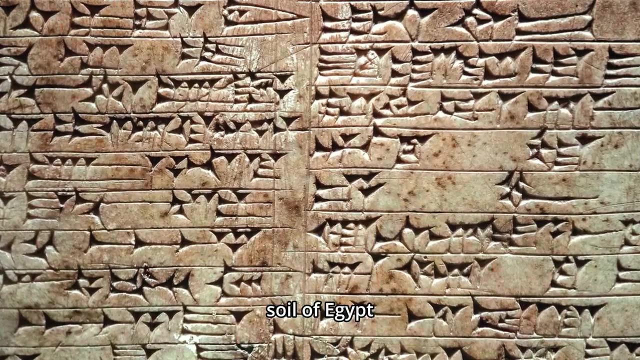 It was these trailblazers who introduced novel techniques revolutionizing the way Egyptians cultivated their lands. With an innate understanding of the plant world, they harnessed their knowledge to improve crop yields and nurture a bountiful harvest. In the fertile soil of Egypt, the seeds of agriculture took root. 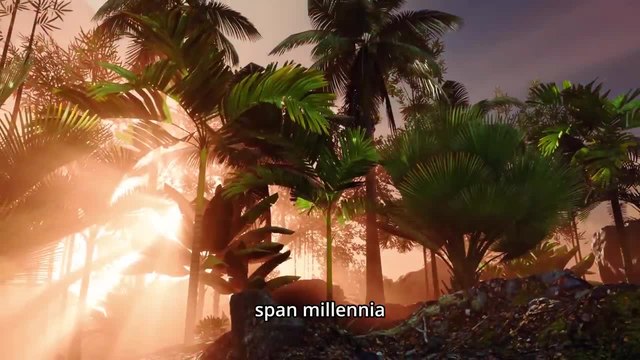 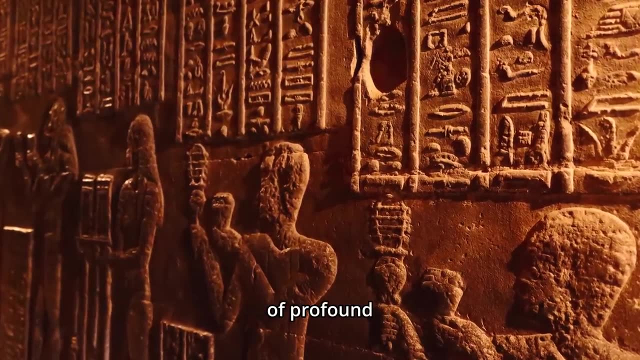 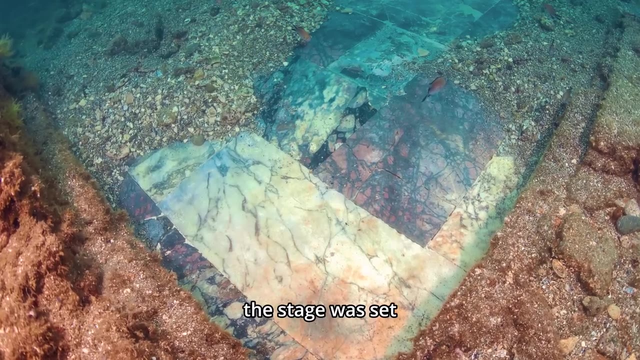 paving the way for a flourishing civilization that would later span millennia. Around 3500 BC, the sands of time carried with them a transformation of profound significance, ushering in an era of evolution and progress. in the heart of Egyptian civilization, The stage was set with a Neolithic culture. 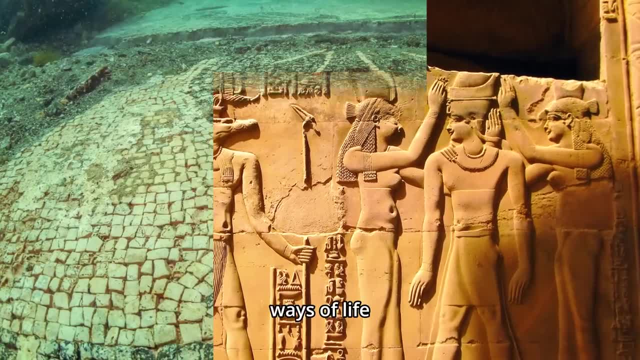 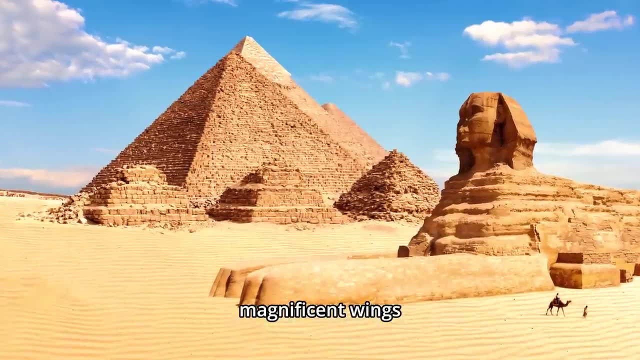 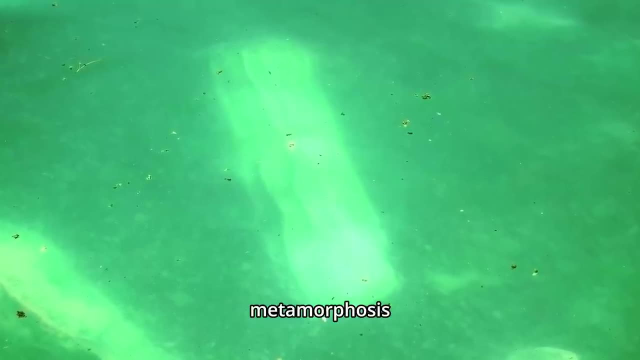 still characterized by a tribal nature and simpler ways of life. But it was during this juncture, under the benevolent gaze of history, that change unfurled its magnificent wings. In a display of visionary genius and collective ambition, the Egyptian society underwent a spectacular metamorphosis. 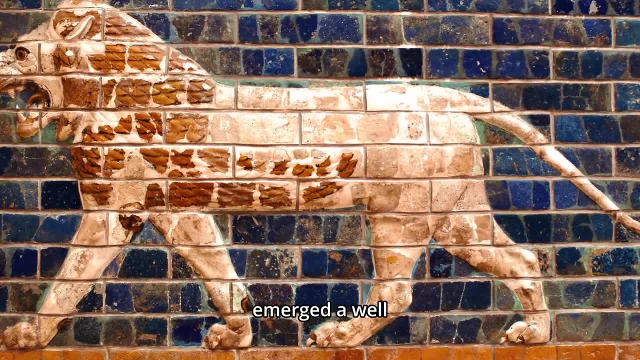 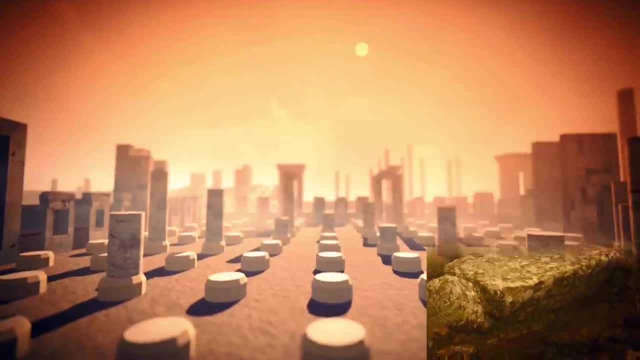 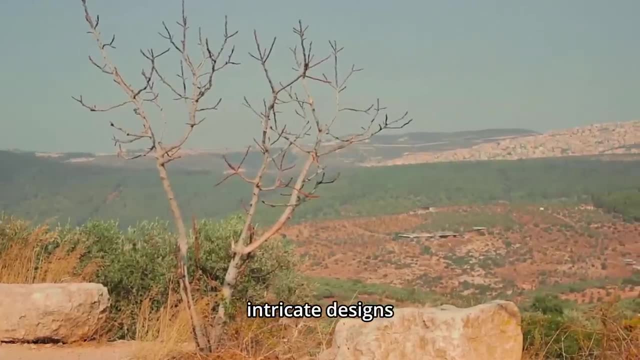 Gone were the primitive days of yore, and in their place emerged a well-organized, structured civilization. This epoch bore witness to a symphony of advancements: the birth of writing, a medium for preserving knowledge and wisdom. the mastery of intricate crafts, weaving intricate designs into the fabric of daily life. 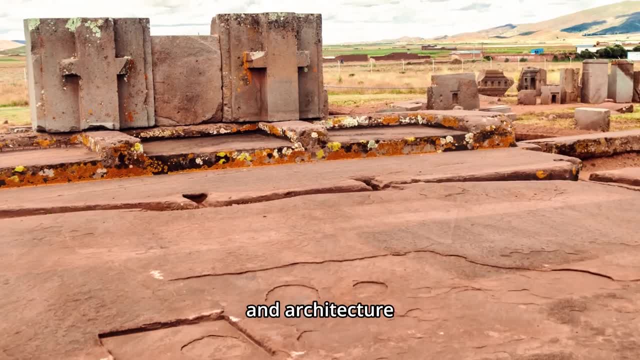 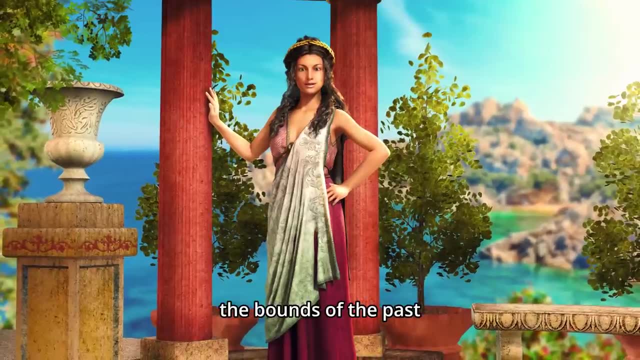 and towering above all the grandiloquent works of art and architecture that, to this day, leave the world in awe. With unwavering determination and a desire to transcend the bounds of the past, the Egyptians infused with an innate thirst for progress. 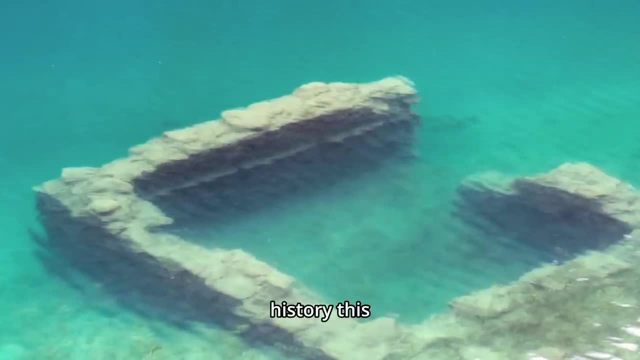 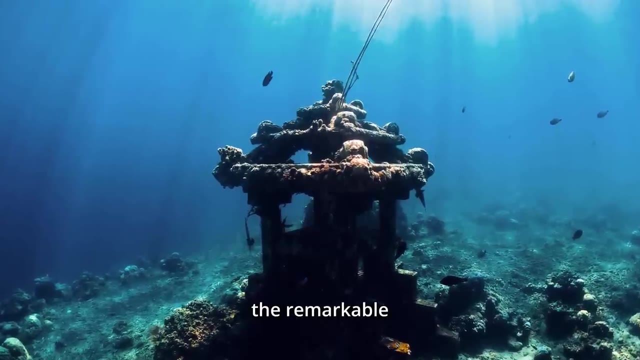 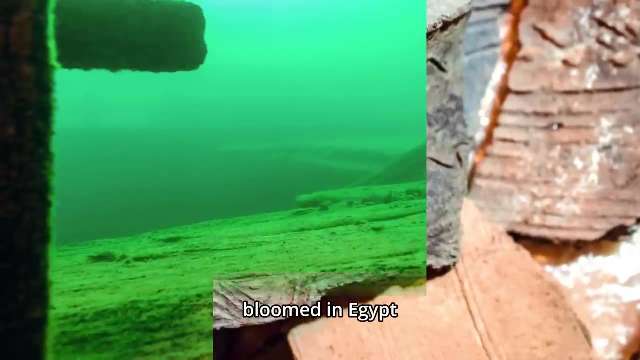 left an indelible mark on the annals of human history. This extraordinary era, built on the foundations of art, culture and knowledge, was a testament to the remarkable potential of the human spirit. In the annals of time, a period of remarkable cultural efflorescence bloomed in Egypt. 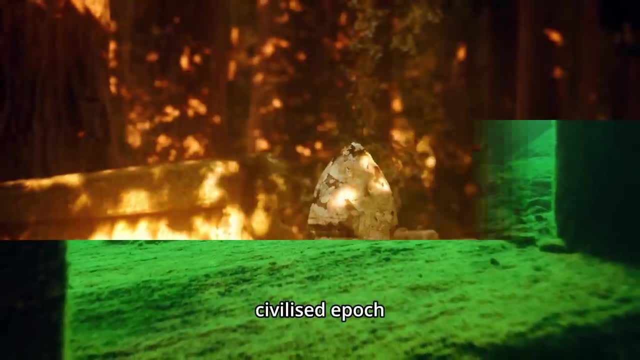 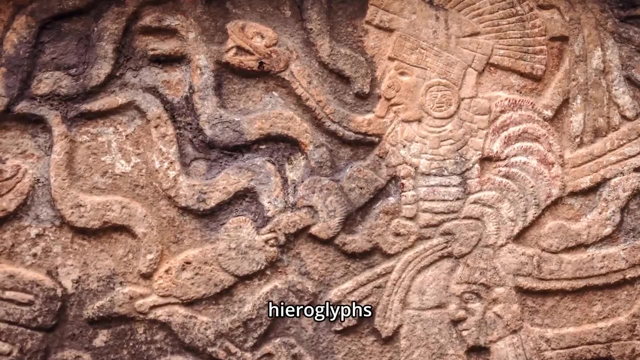 It was as though, from the depths of history, a long civilized epoch had awakened, casting off the cocoon of obscurity to reveal its magnificent wings, Hieroglyphs. the ancient script appeared as if conjured by the muse herself. 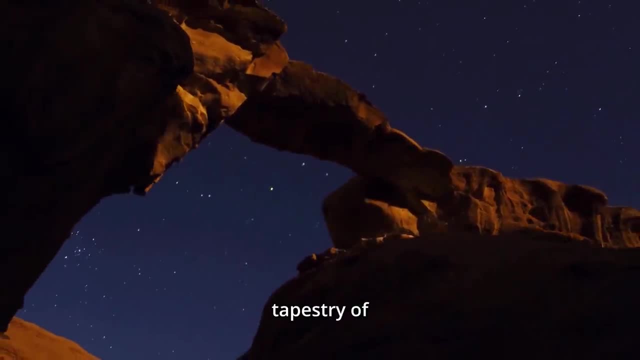 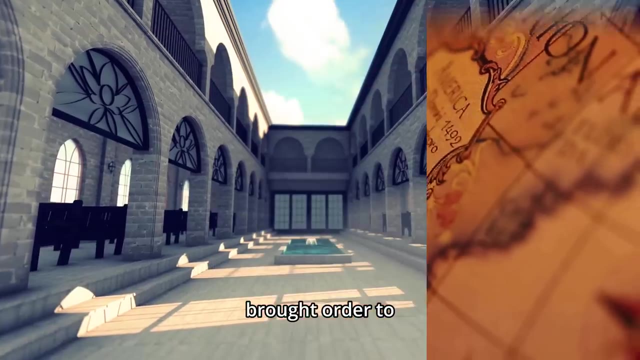 They burst forth, fully formed, etching the tapestry of knowledge and wisdom with their intricate characters. The calendar precise as the movements of the heavens brought order to the passage of time, Social structures and censuses organized the collective heartbeat of society. 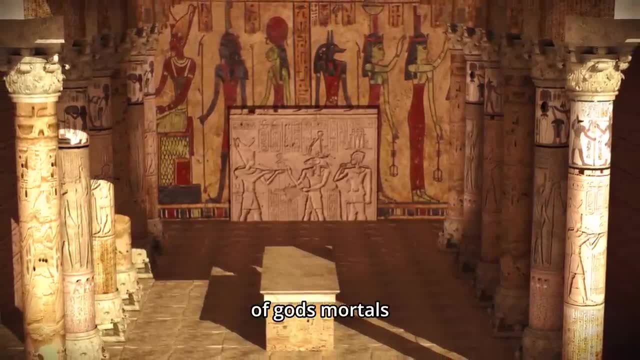 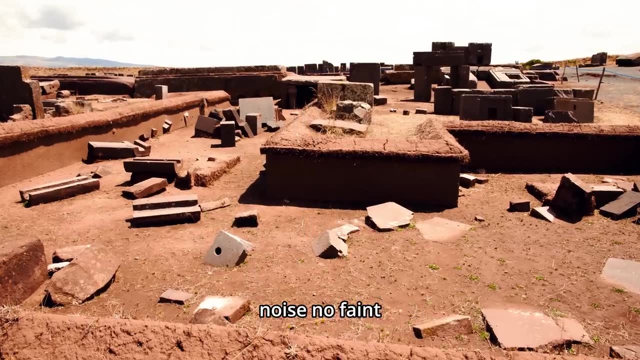 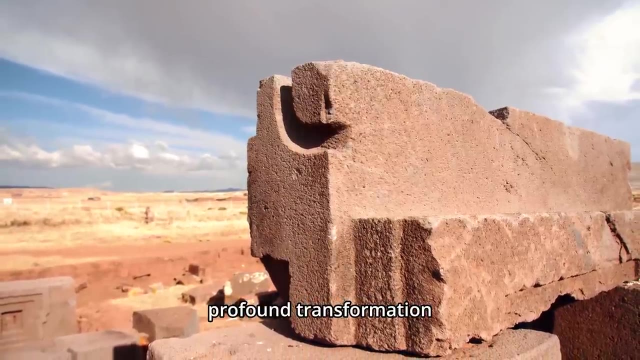 while a rich mythology wove stories of gods, mortals and the grand tapestry of existence. In this renaissance of culture, there was little background noise, no faint echoes from the past to explain these fundamental developments. It was as if Egypt had undergone a profound transformation in the blink of an eye. 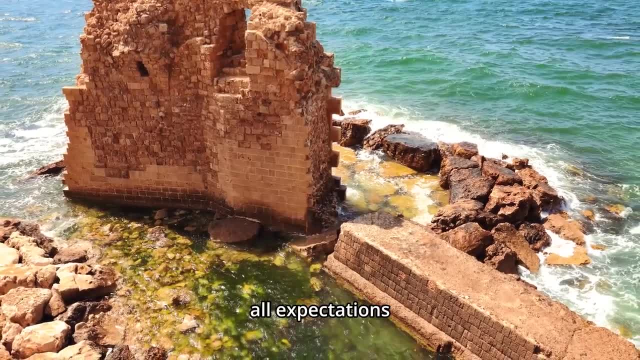 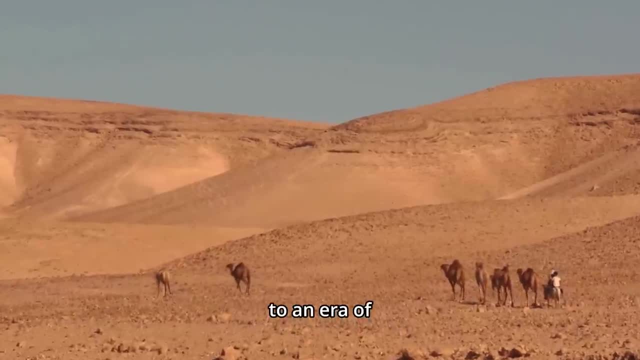 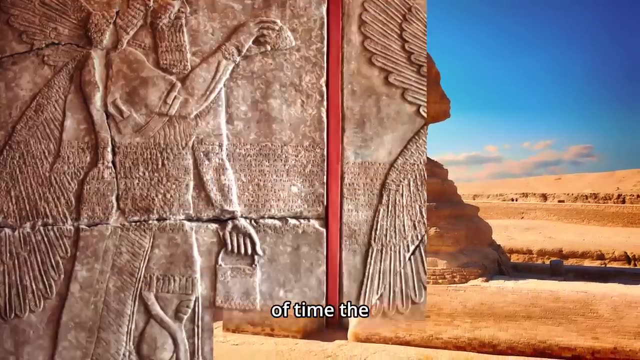 unleashing a burst of creativity and intellect that defied all expectations. This historical period, illuminated by the torch of ancient wisdom, bore testimony to an era of prehistoric civilization that prepared the stage for the grand drama of human history. Upon the sands of time, the footprints of Egypt's past tell a story that defies the gradual, measured progression of human societies. 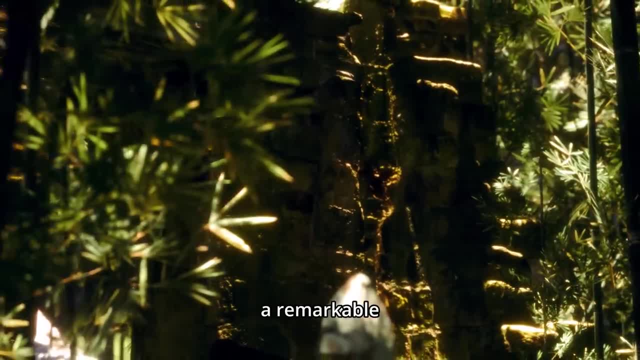 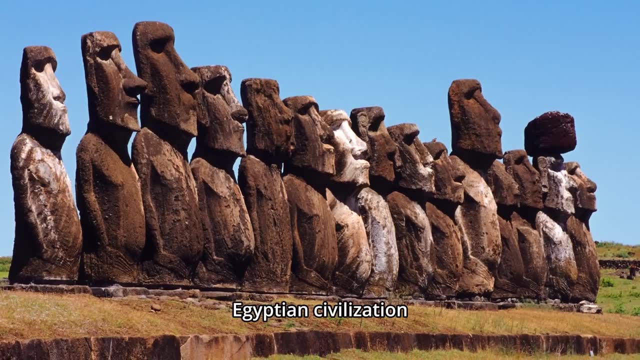 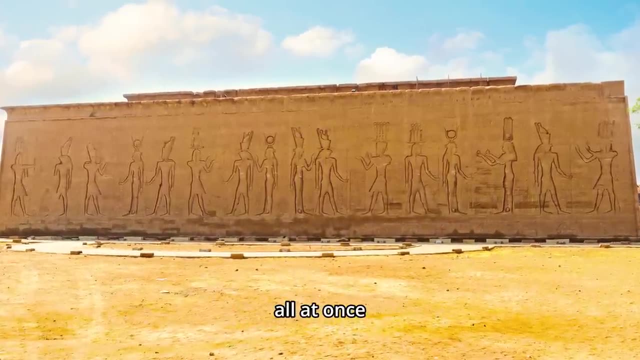 Instead, the evidence etched in stone and earth speaks of a remarkable emergence, an ascent, not of laborious evolution, but of sudden and profound transformation. Egyptian civilization, in all its grandeur, did not unfold with the measured footsteps of history. It emerged all at once, fully formed, like the phoenix reborn from its own ashes. 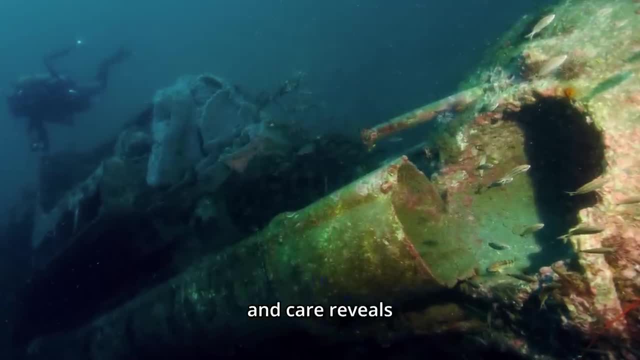 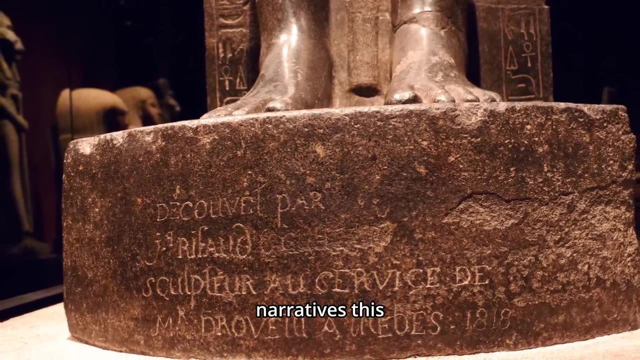 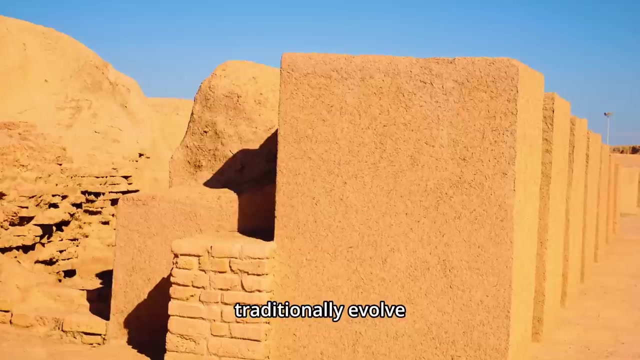 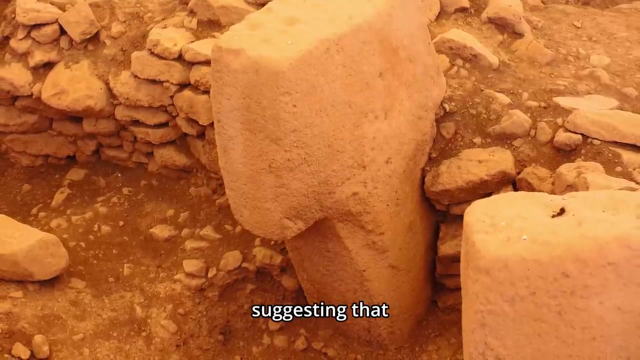 An archaeological tapestry woven with precision and care reveals a period of transition so fleeting that it defies the conventions of historical narratives. This rapid rise, as if whispered by the gods themselves, challenges our understanding of how civilizations traditionally evolved. It beckons us to question the mysteries and untold stories that lie hidden within the annals of time, suggesting that there may be more to the birth of Egypt's grand civilization than meets the eye. 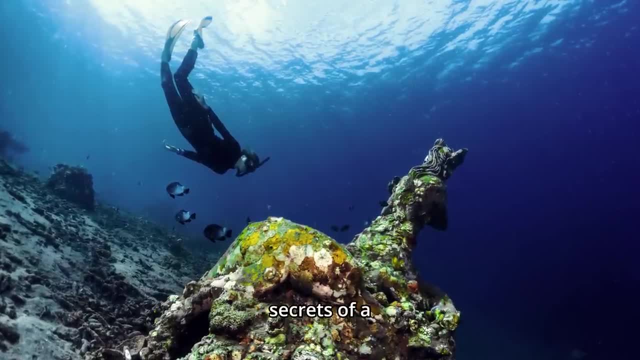 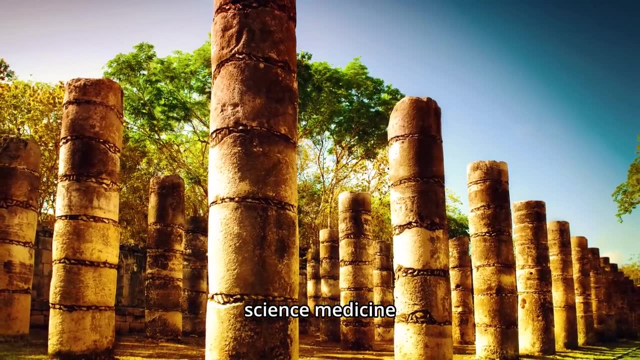 In the realm of ancient Egypt, where sand and stone whispered secrets of a forgotten time, the arts and sciences flourished with a brilliance unparalleled. Science, medicine, mathematics and astronomy were not mere disciplines but the luminous gems in the crown of this sophisticated civilization. 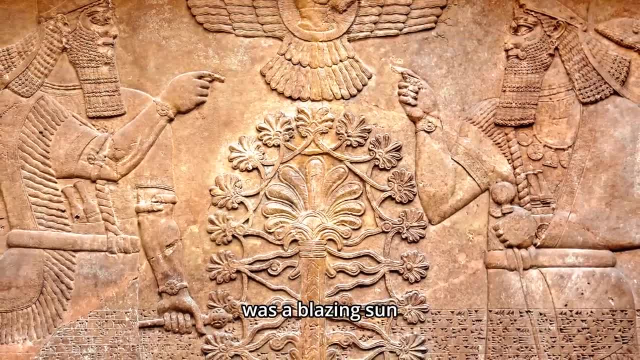 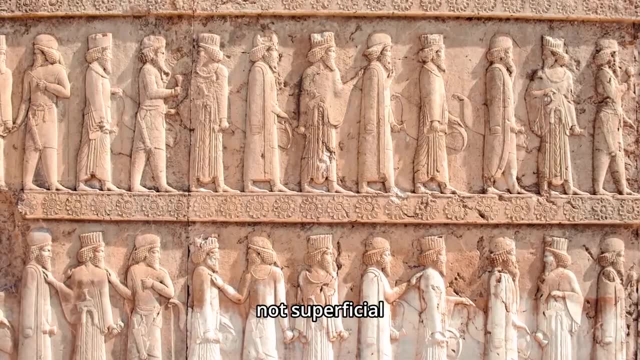 Here, knowledge was more than a glimmer in the eyes of scholars, It was a blazing sun illuminating the path to universal truths. The understanding of laws governing the cosmos was not superficial but profound, reaching heights that modern scholars may hesitate to acknowledge. 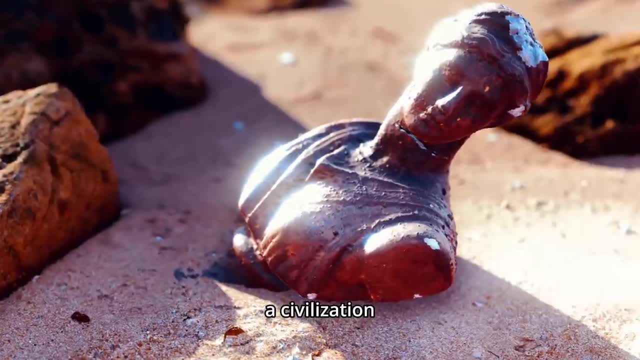 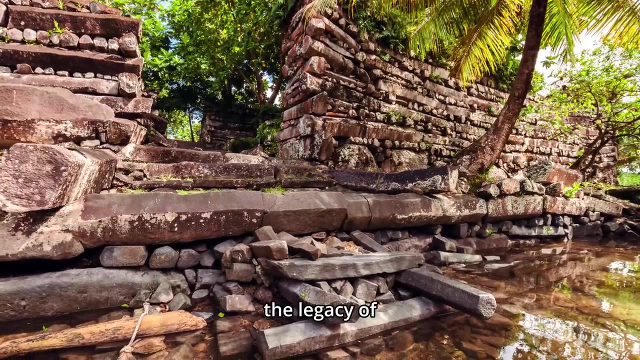 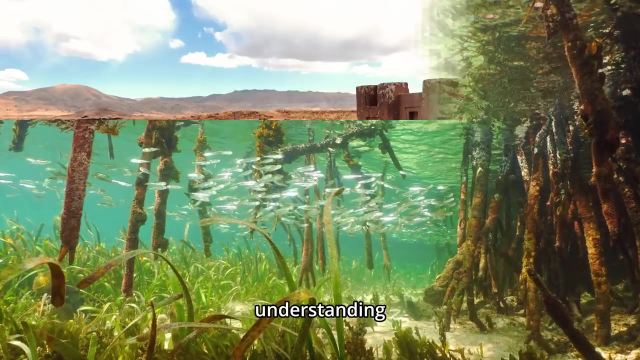 In the enigmatic heart of Egypt, a civilization thrived in harmony with the cosmos, where precision and wisdom were woven into the very fabric of life. The legacy of Egypt resonates with echoes of this remarkable sophistication, inviting us to unlock the door to the deeper understanding that lies beneath the surface of history. 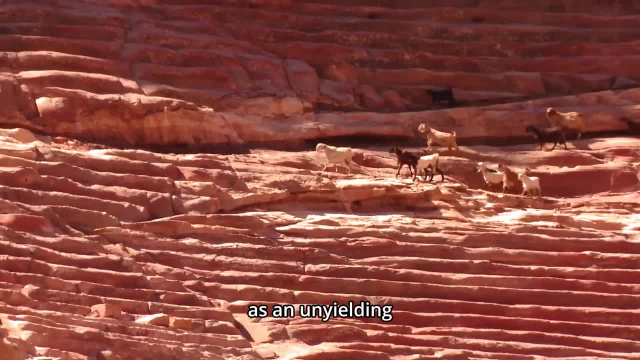 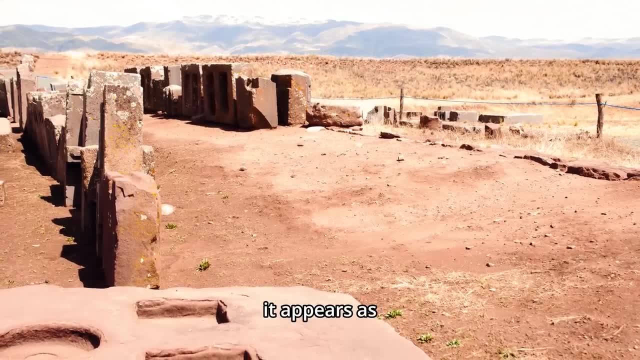 Egypt, the land of enigma, stands as an unyielding testament to the unfathomable depths of human knowledge. For every facet of wisdom and creativity, it appears as though Egypt burst forth with completeness, as if it had drunk from the eternal well of understanding. 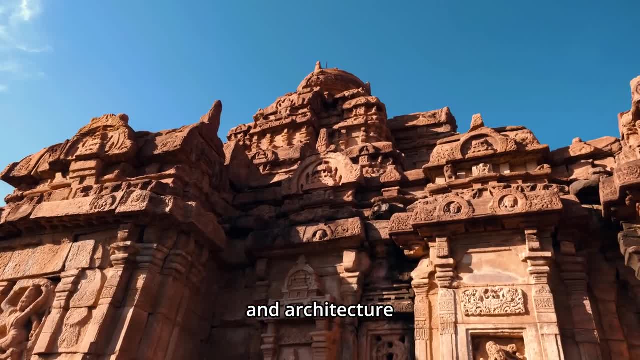 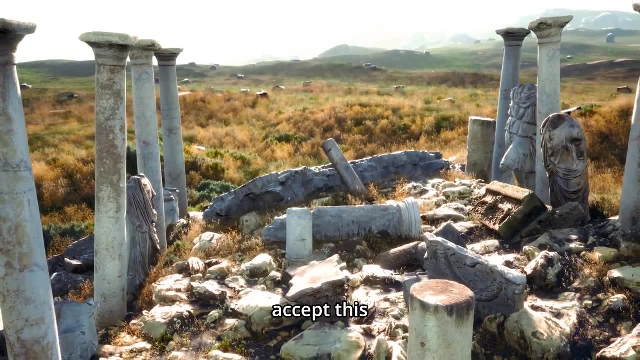 In science, art and architecture. Egypt's early triumphs are unmatched and often unmet by later generations. Orthodox scholars grudgingly accept this extraordinary fact, but tread lightly on the mystery it begets, while its myriad implications remain largely unspoken. 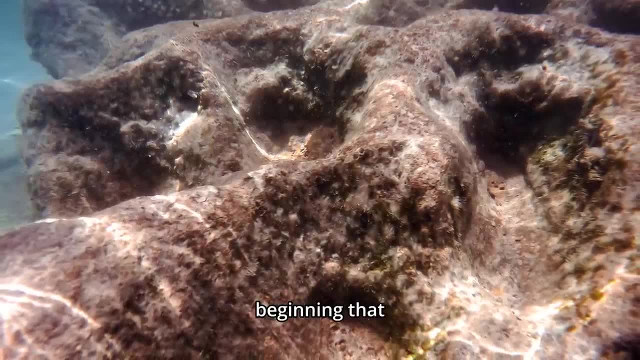 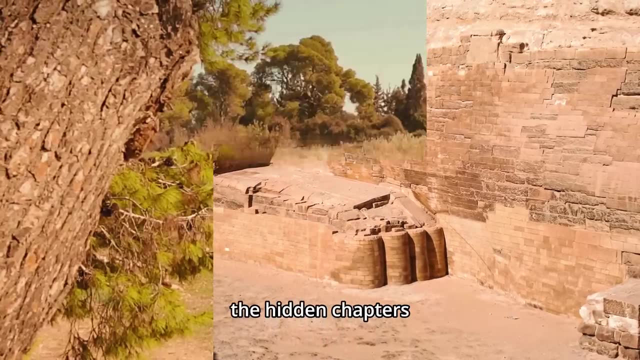 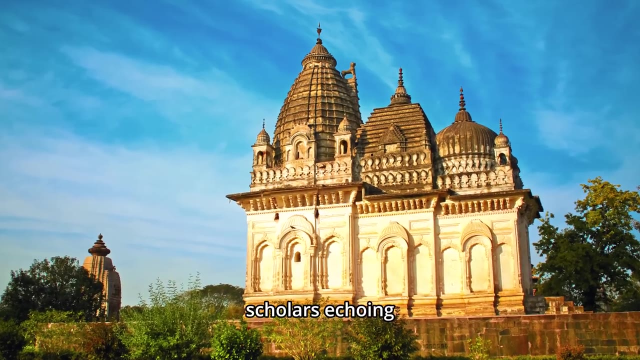 The narrative of Egypt tells a story of an astonishing beginning that defies explanation, challenging us to delve into the enigmatic reservoirs of human achievement and contemplate the hidden chapters of our shared history. The inexplicable marvels of ancient Egypt continue to baffle modern scholars, echoing through the corridors of history. 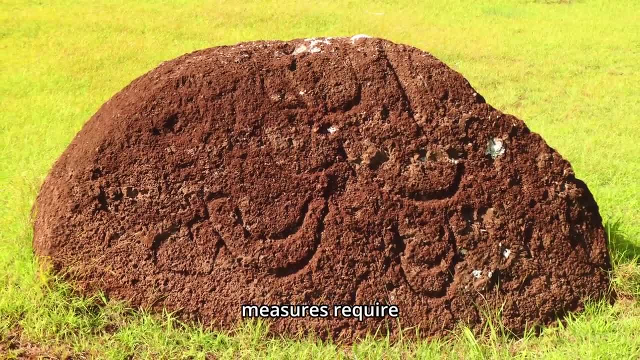 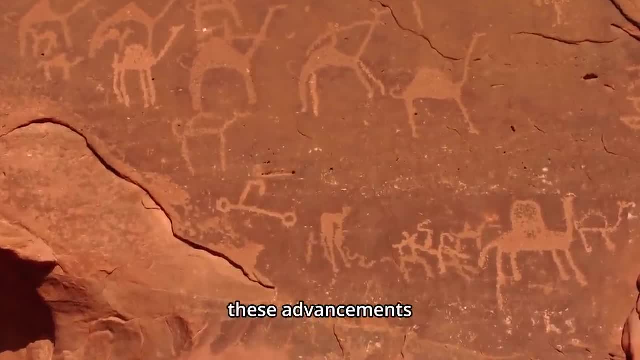 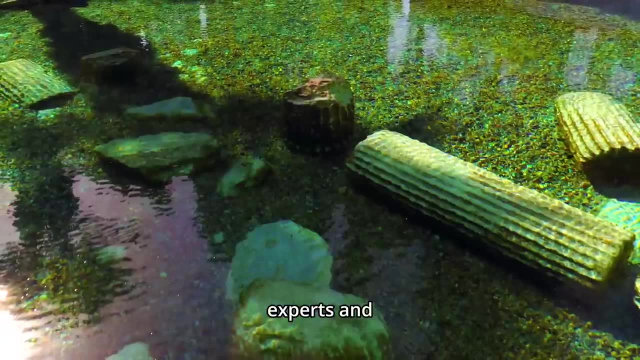 Technological achievements, by all rational measures required generations, if not millennia, to develop. Yet in the case of ancient Egypt, these advancements emerged seemingly overnight, with no discernible precursors. It's a conundrum that leaves experts and enthusiasts alike in awe. 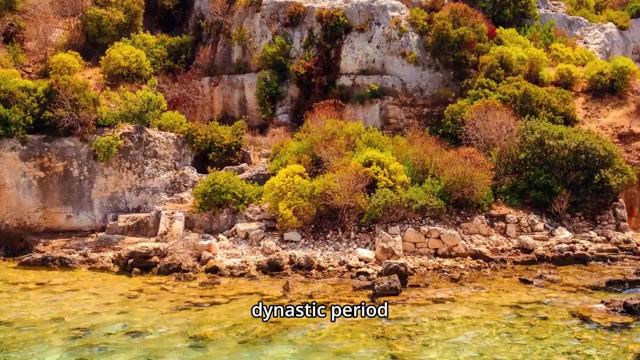 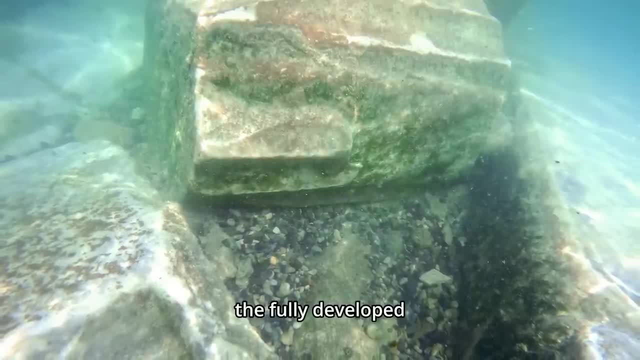 Intriguingly, when we delve into the pre-dynastic period around 3500 BC, we find an absence of written language, a stark contrast to the fully developed hieroglyphs that would later grace the walls of the land's iconic monuments. 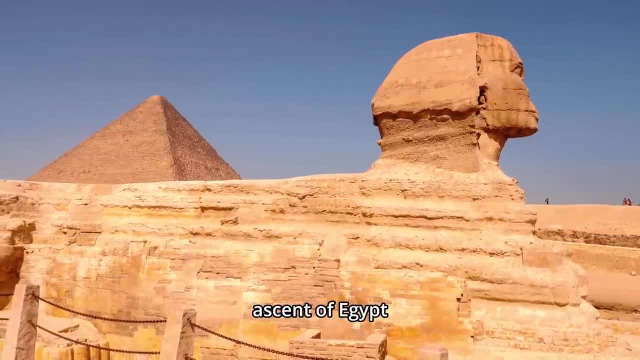 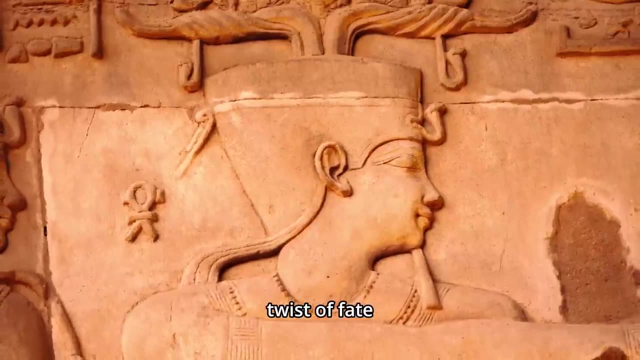 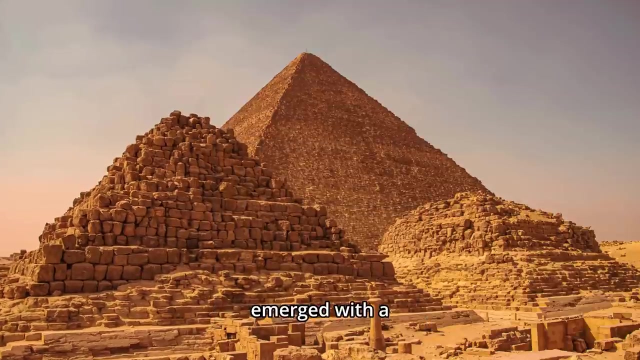 It's a testament to the rapid and mysterious ascent of Egypt's civilization, a reminder that history's riddles often outnumber its answers. In a curious twist of fate, just shortly after that enigmatic threshold, the very hieroglyphs that now adorn the ruins of ancient Egypt emerged with a completeness and sophistication that astounds the modern observer. 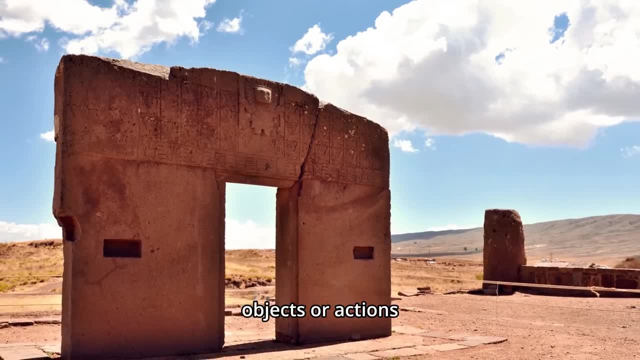 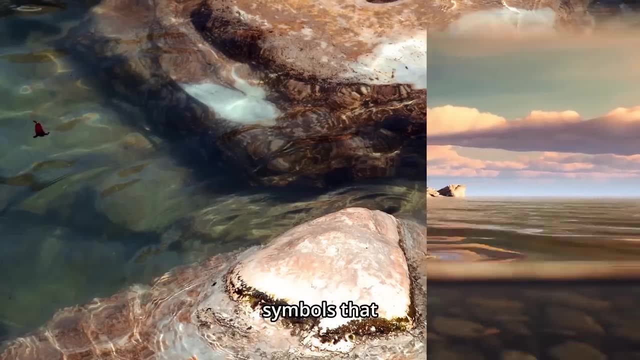 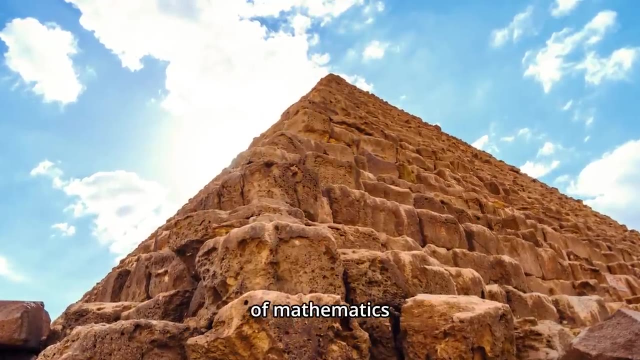 Far from being rudimentary illustrations of objects or actions, this written language was, from its inception, intricate and meticulously organized. It featured symbols that represented the essence of sounds and an intricate system of numerical representation that spoke to a deep understanding of mathematics and communication. 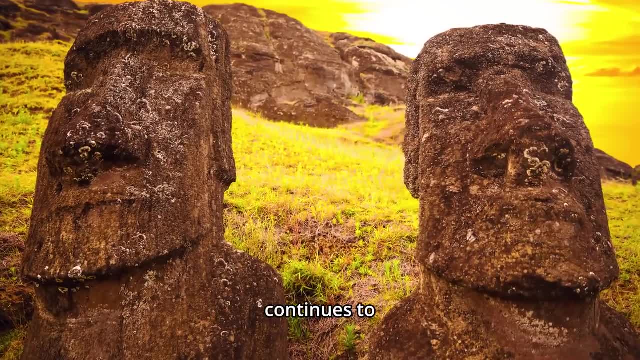 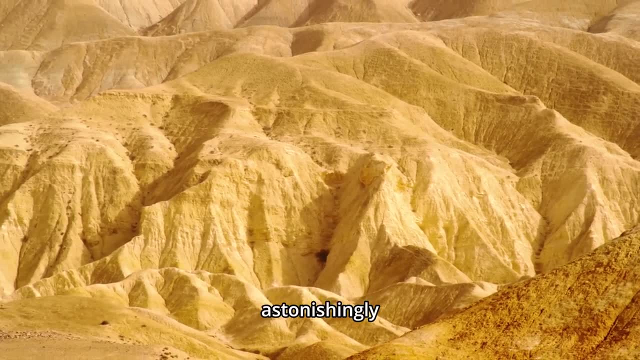 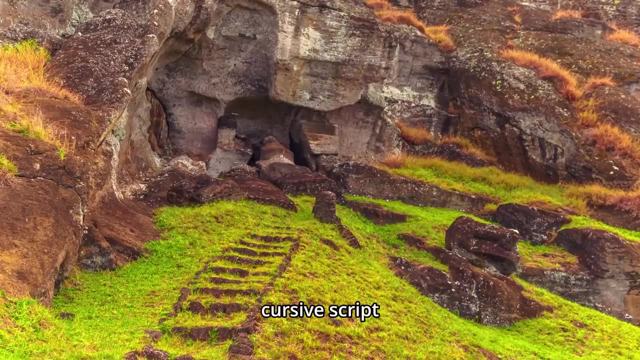 The abrupt birth of such a complex script continues to defy rational explanation, leaving us to ponder the profound enigma of Egypt's distant past. Astonishingly, even the most ancient hieroglyphs displayed a level of stylization and convention that implies an advanced cursive script was already in use by the time of the first dynasty. 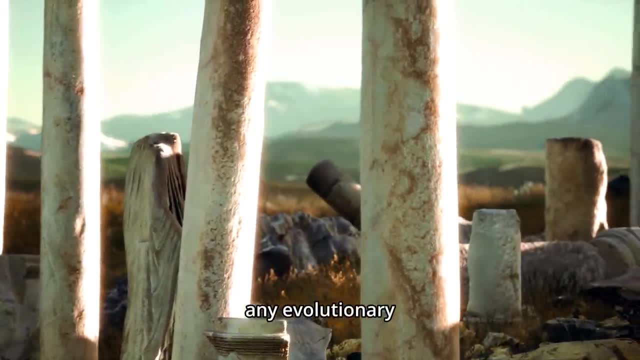 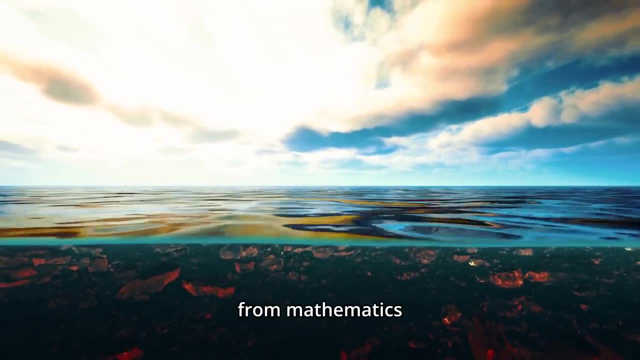 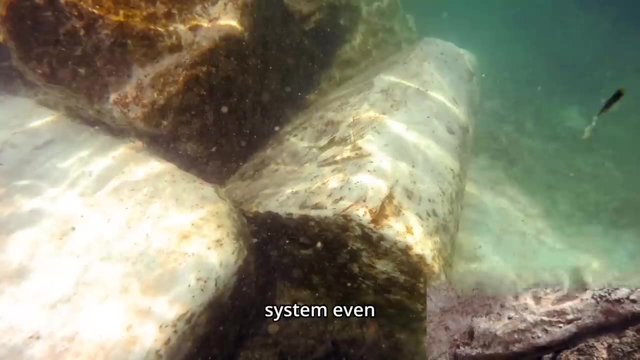 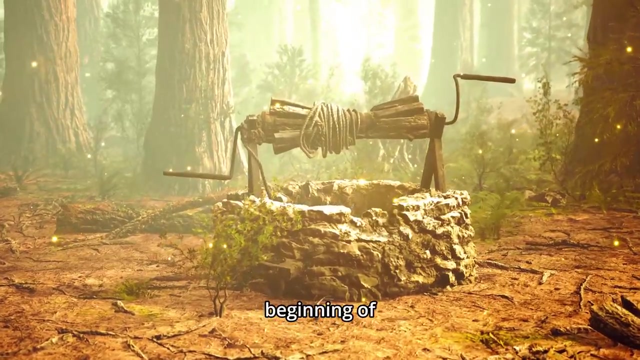 What sets this apart is the apparent lack of any evolutionary process from simplicity to sophistication. This curious phenomenon extends to various fields, from mathematics, medicine, astronomy and architecture to Egypt's intricately woven religio-mythological system. Even the core content of revered texts such as the Book of the Dead was in existence right from the beginning of the dynastic period. 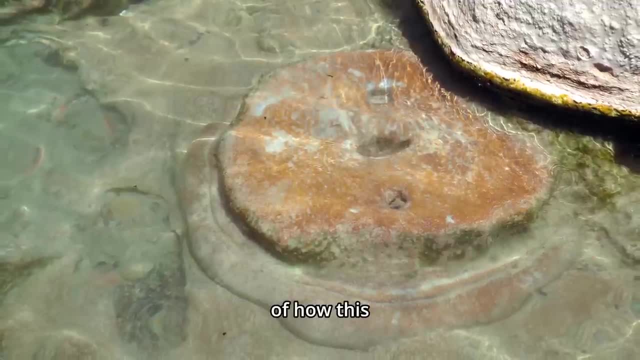 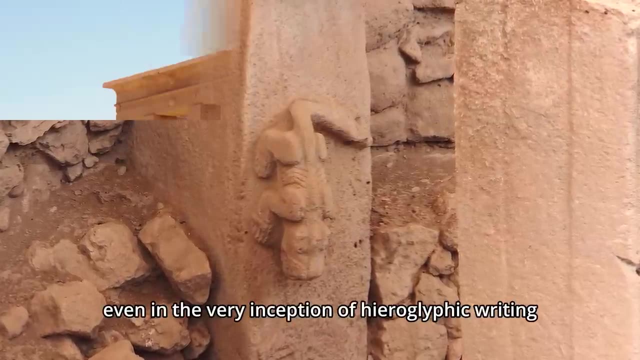 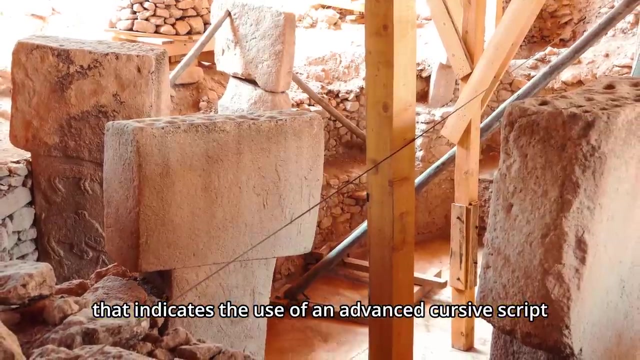 The absence of a gradual development leaves us grappling with the mystery of how this profound knowledge seemingly appeared fully formed in the annals of ancient Egypt. Even in the very inception of hieroglyphic writing we find a level of stylization and convention that indicates the use of an advanced cursive script as early as the dawn of the first dynasty. 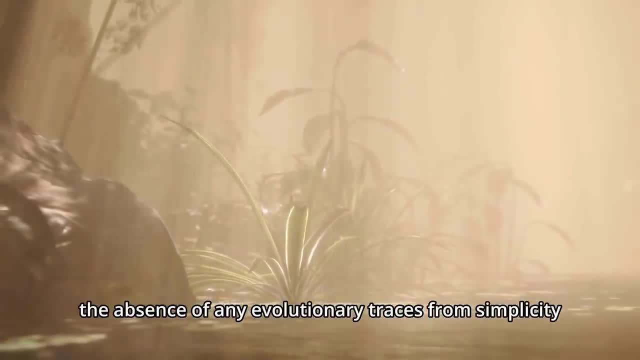 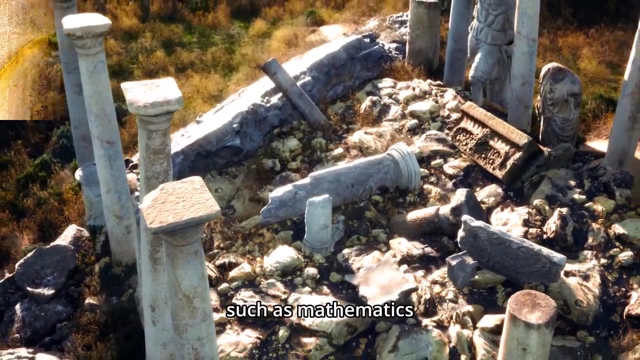 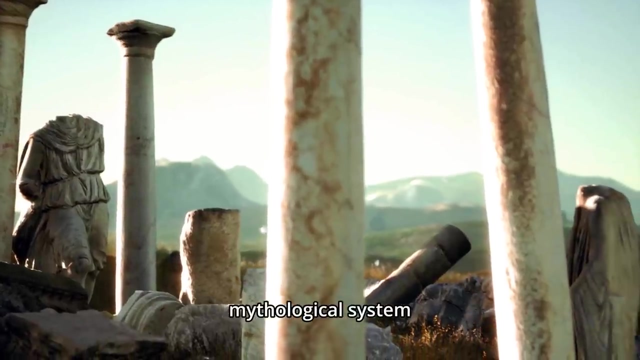 The remarkable aspect of this development is the absence of any evolutionary traces from simplicity to sophistication. This peculiarity extends to various domains such as mathematics, medicine, astronomy and architecture, as well as Egypt's immensely complex religio-mythological system. 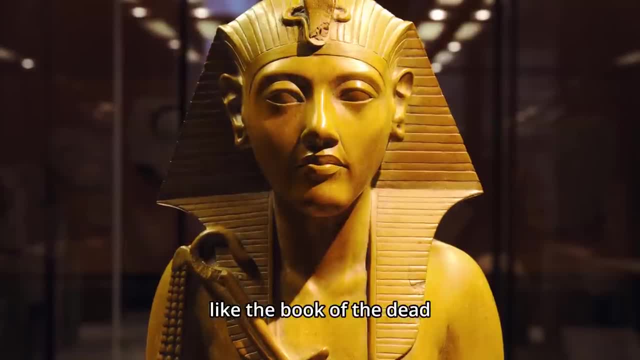 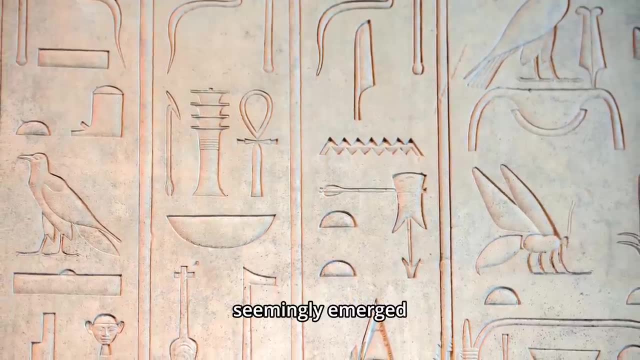 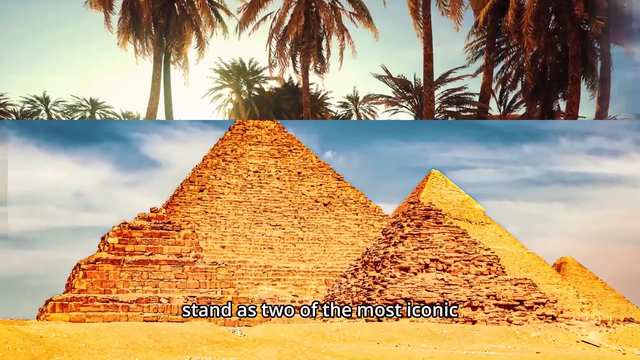 Even the core content of revered texts like the Book of the Dead existed from the very outset of the dynastic period. The enigma lies in how this wealth of knowledge seemingly emerged fully formed. in the annals of ancient Egypt. The Great Pyramid of Giza and the Enigmatic Sphinx stand as two of the most iconic and immediately identifiable structures in the entirety of Egypt. 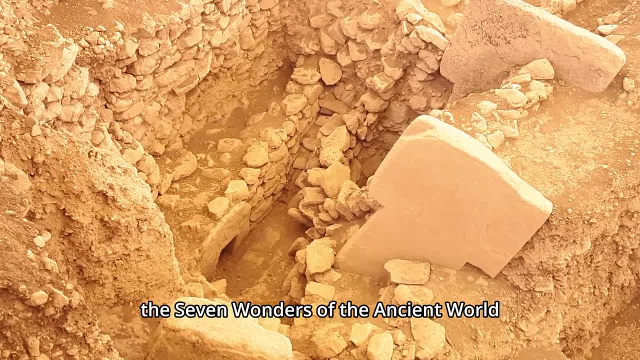 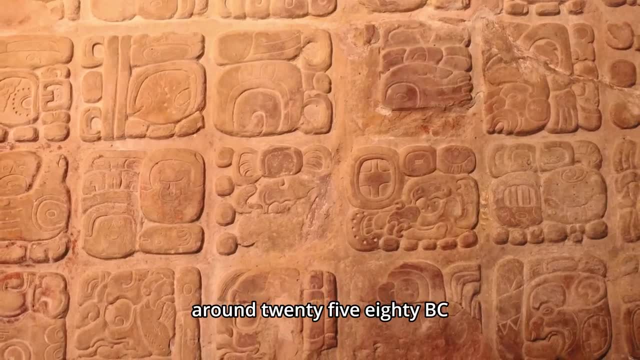 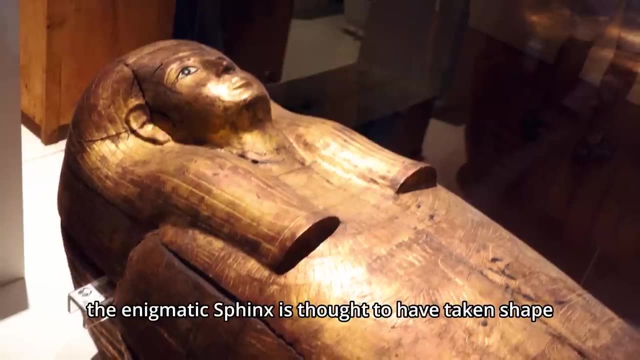 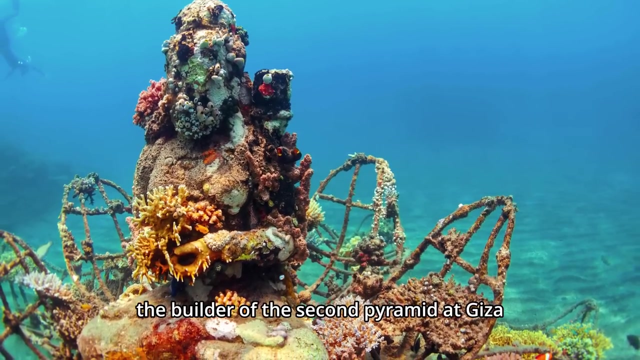 Revered as one of the Seven Wonders of the Ancient World. conventional archaeology attributes their construction to the reign of Pharaoh Khufu around 2580 BC, presenting them as grand pharaonic tombs. Meanwhile, the Enigmatic Sphinx is thought to have taken shape approximately two decades later, around 2500 BC, for the Pharaoh Khafre, the builder of the Second Pyramid at Giza. Yet there is a significant body of thought contending that these iconic structures boast a far more ancient lineage than the traditional narrative suggests. According to the visionary insights of Edgar Cayce, the Great Pyramid was constructed between 10,490 and 10,390 BC under the guidance of Hermes, who was believed to have safeguarded the wisdom of Atlantis. 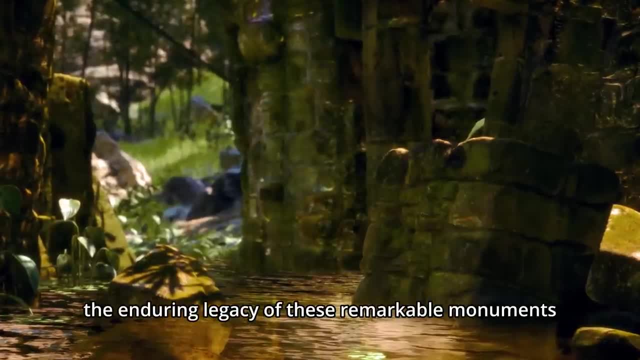 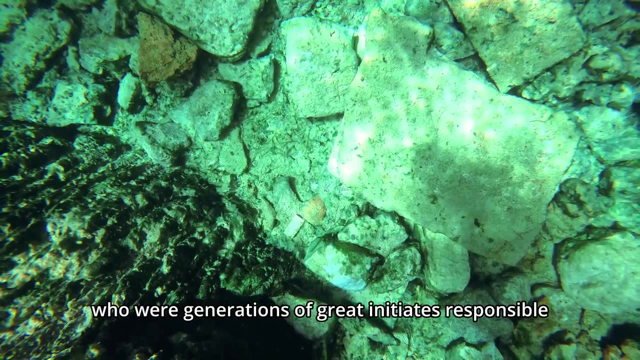 Gurdjieff maintained that the enduring legacy of these remarkable monuments can be traced back to ancient times. It can be attributed to the descendants of Atlantis, particularly the Akhaldans, who were generations of great initiates responsible for the construction of the pyramids and sphinx. 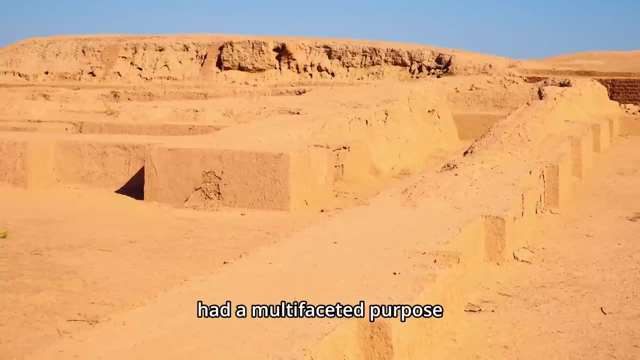 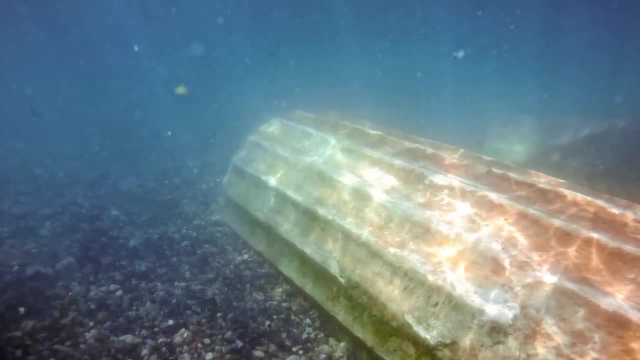 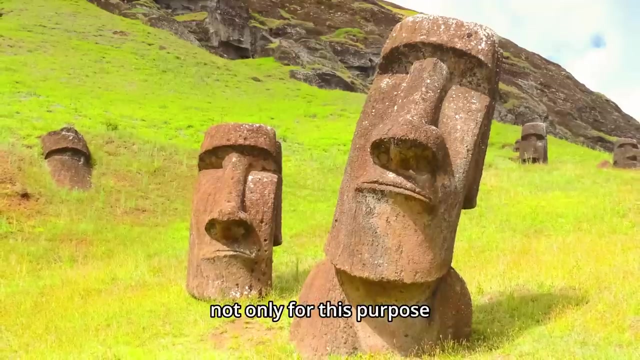 Gurdjieff asserted that the pyramids at Giza had a multifaceted purpose. Among their functions, he believed that they served as advanced astronomical observatories, allowing the Akhaldans to closely study the cosmos. Additionally, the two smaller pyramids were designed not only for this purpose, but also to manipulate local knowledge. 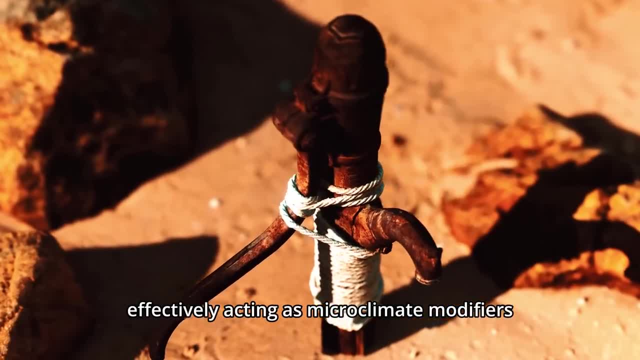 Gurdjieff said that the pyramids were designed in a way that allowed them to study the cosmos. Gurdjieff said that the pyramids were designed in a way that allowed them to study the cosmos. This intricate design aimed to enhance the accuracy of their astronomical observations. Robert Bauval and Graham Hancock's research unveils a compelling theory regarding the Great Pyramid's design and construction. They propose that this extraordinary structure was meticulously aligned with the circumpolar stars and the precession of the equinoxes. Notably, they emphasize that the pyramids' shafts are precisely oriented toward key circumpolar stars like Orion and Sirius. 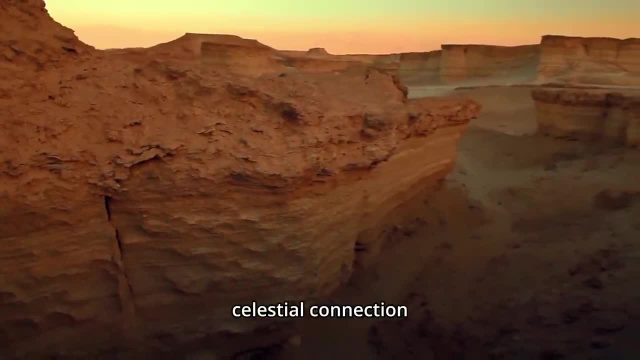 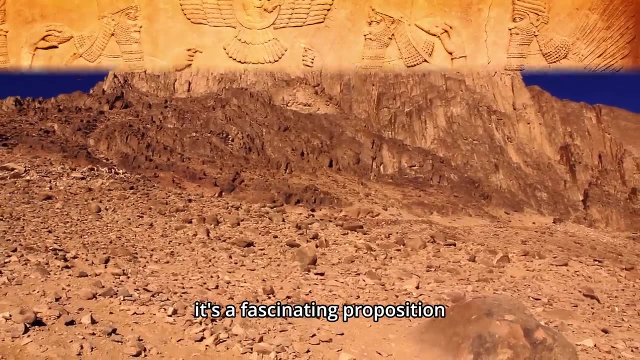 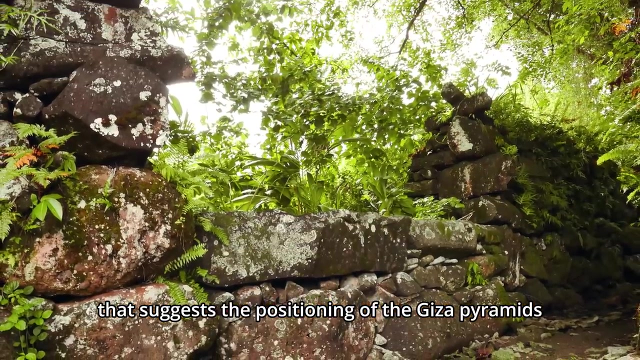 underscoring their significance in the pyramids' celestial connection. This alignment suggests a deep understanding of astronomical phenomena by the ancient builders. It's a fascinating proposition put forward by various researchers, particularly Robert Bauval, that suggests the positioning of the Giza pyramids was part of a grand design. 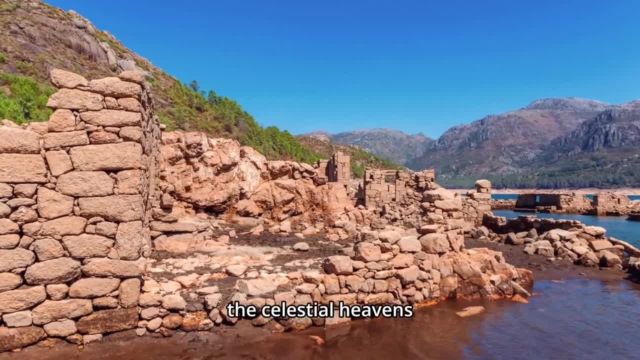 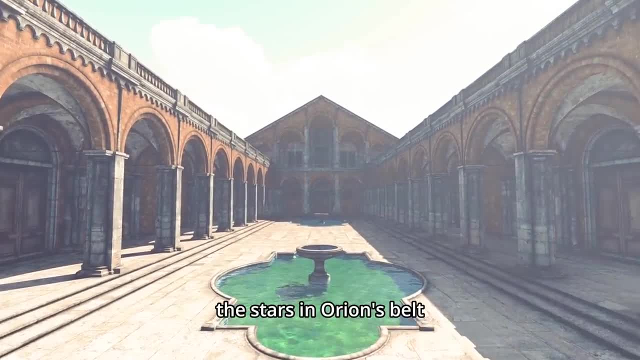 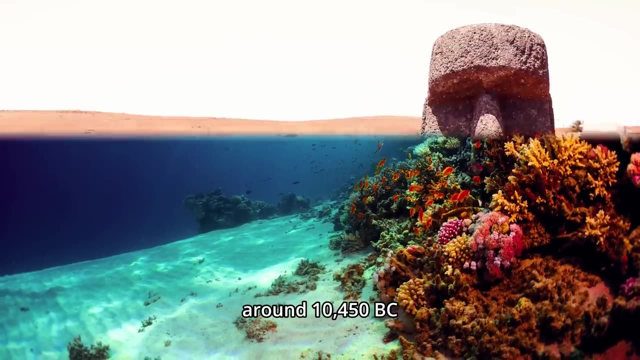 reflecting a precise representation of the celestial heavens. According to this theory, the three pyramids at Giza were deliberately aligned to mirror the stars in Orion's belt. This celestial alignment corresponds to a specific time in history, around 10,450 BC. 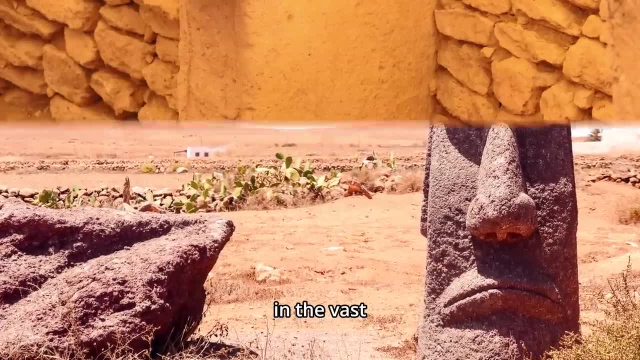 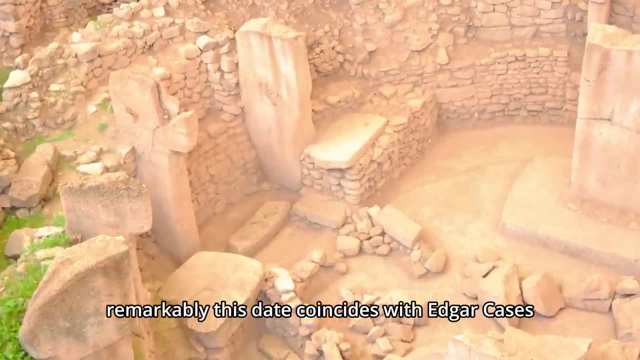 when Orion was at its closest to the southern horizon in the vast 25,900-year cycle of the precession of the equinoxes. Remarkably, this date coincides with education. There is a particular case's assertion that the Great Pyramid's construction was planned around 10,500 BC. 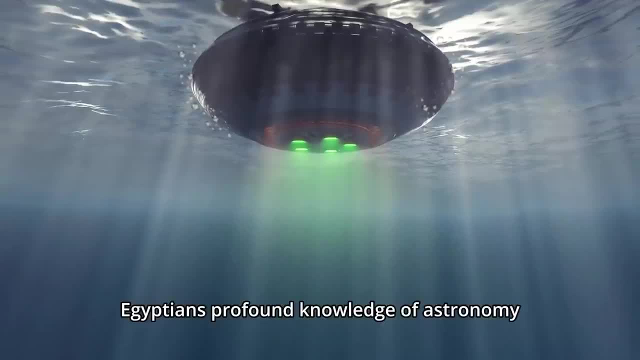 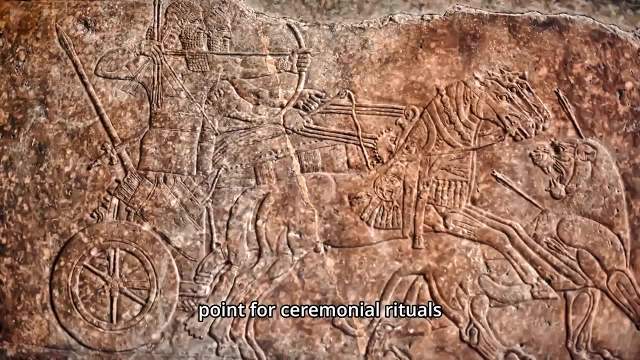 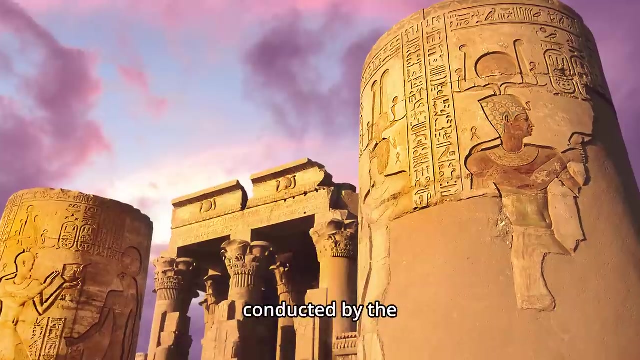 This alignment underscores the ancient Egyptians' profound knowledge of astronomy and their ability to incorporate it into their architectural and religious designs. Point for ceremonial rituals. These individuals suggest that the pyramids served as a center for initiation and spiritual rites conducted by the Egyptian mystery schools. 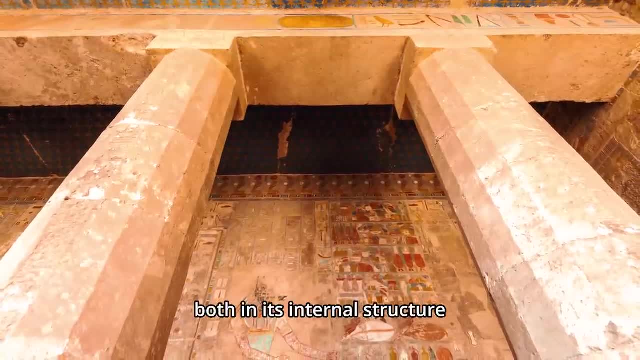 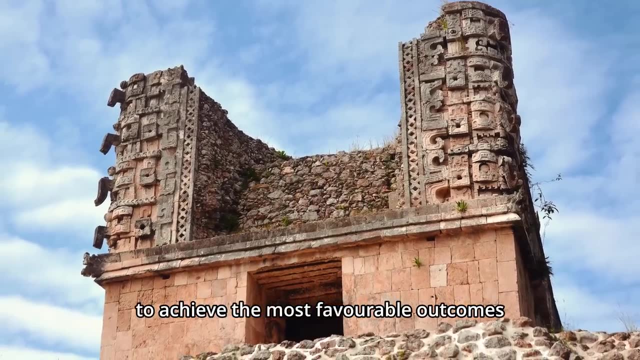 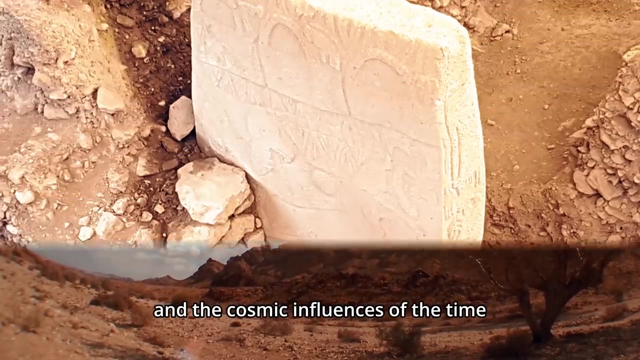 The architectural design of the Great Pyramid, both in its internal structure and external form, is believed to have been meticulously coordinated to achieve the most favorable outcomes. It was intricately designed to create a profound psycho-spiritual connection between individuals and the cosmic influences of the time. 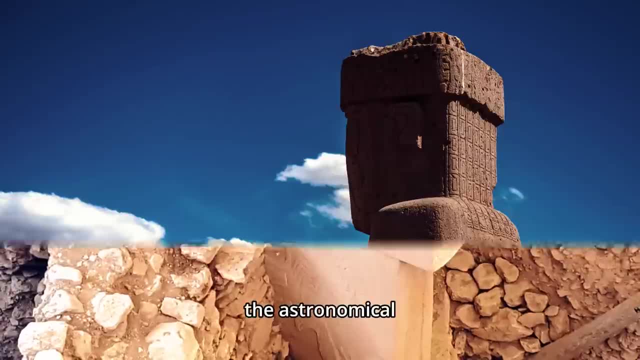 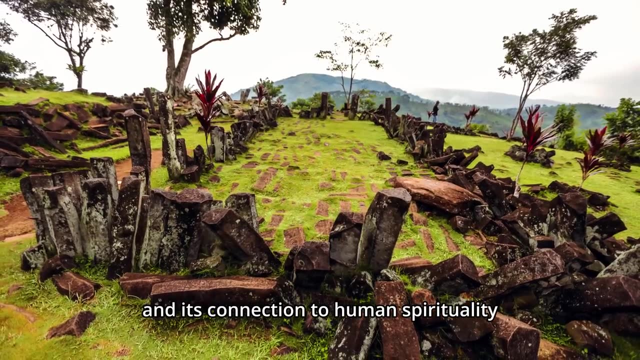 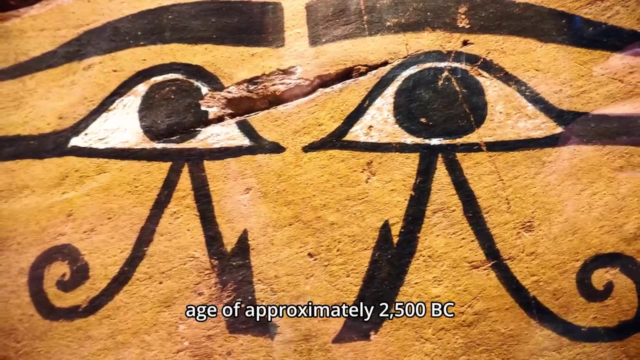 These ceremonies and practices were closely aligned with the astronomical events of their era, reflecting the ancient Egyptians' deep understanding of the cosmos and its connection to human spirituality. The geological evidence surrounding the Sphinx strongly challenges its conventional age of approximately 2,500 BC. 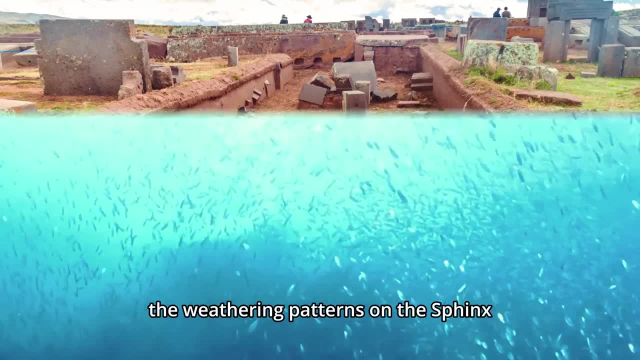 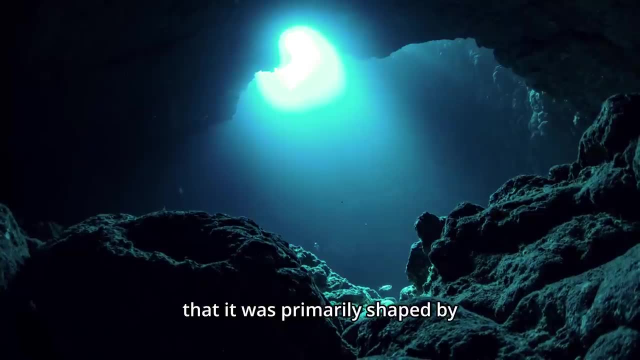 A pioneering observation made by Schwaller de Lubitsch revealed that the weathering patterns on the Sphinx were a result of water erosion, a stark contrast to the commonly held belief that it was primarily shaped by the abrasive forces of wind-blown sand. In his work Sacred Science, 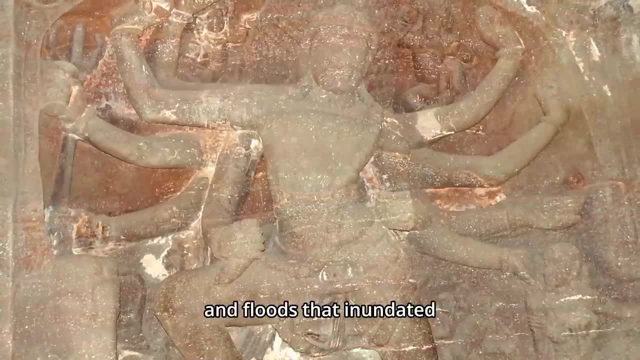 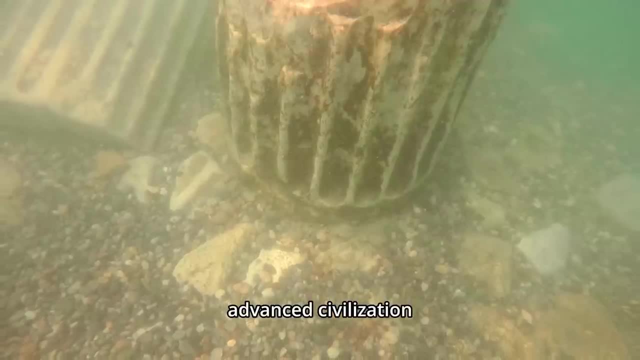 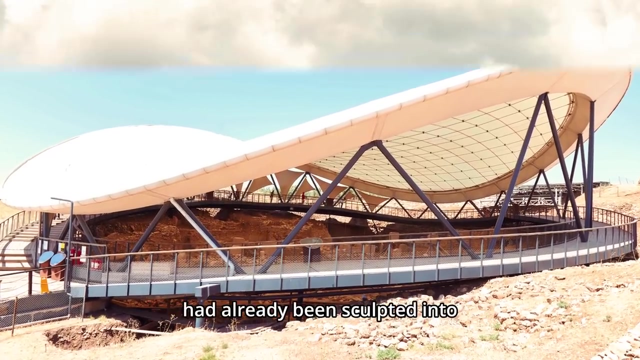 Schwaller de Lubitsch pointed to the cataclysmic rains and floods that inundated Egypt around the 11th millennium BC. He further suggested that a highly advanced civilization must have predated these massive water events. This in turn led to the assumption that the Sphinx had already been sculpted into the rock of the West Cliff at Giza. 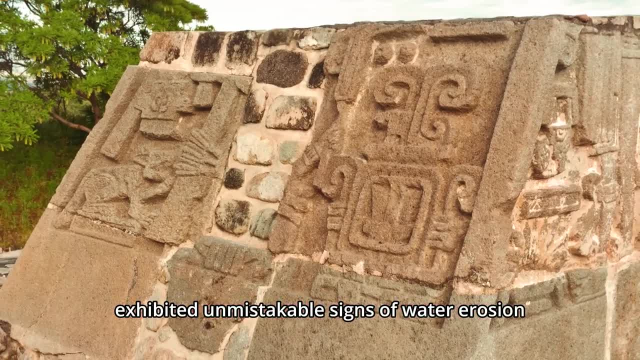 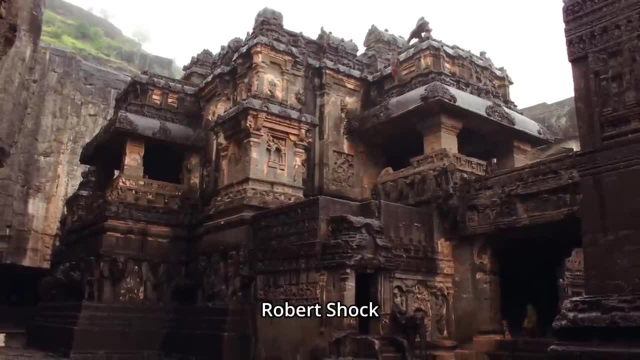 where its lion-like body exhibited unmistakable signs of water erosion. The hypothesis put forth by Schwaller de Lubitsch gained substantial support when American geologist Robert Schock meticulously studied the Sphinx's structure. Schock's comprehensive examination yielded a striking conclusion. 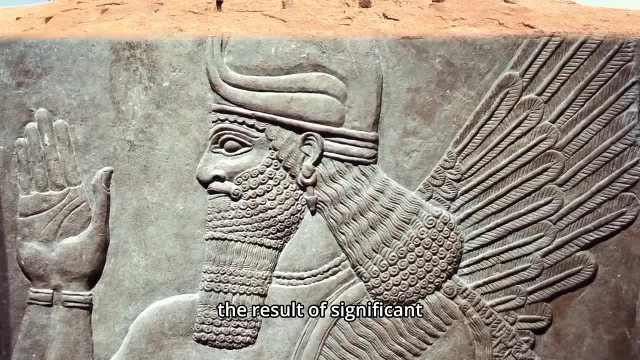 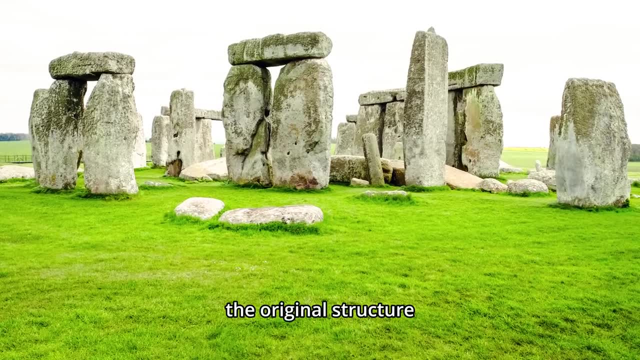 The weathering and erosion observed on the Sphinx were the result of significant precipitation-induced effects. What's more, he emphasized that the core body of the Sphinx, the original structure, predated the reign of Pharaoh Khafre. This revelation cast doubt on the conventional dating of the Sphinx. 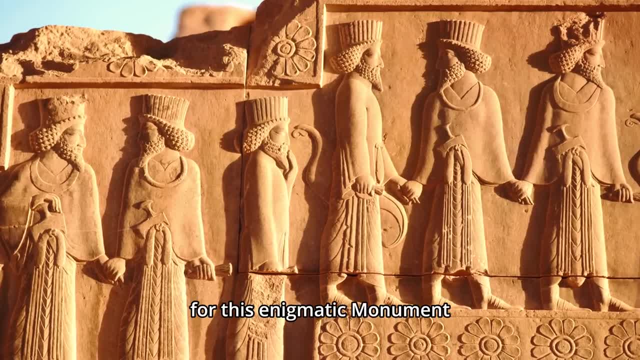 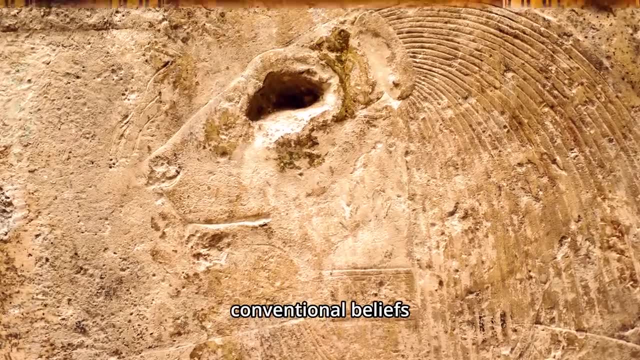 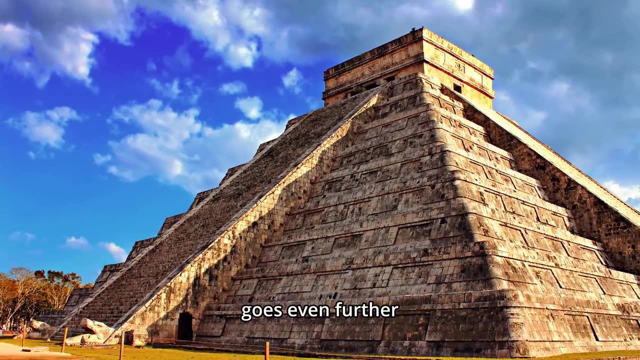 and hinted at an even more ancient origin for this enigma. Robert Schock's assessment of the Sphinx's construction date presents a radical departure from conventional beliefs, placing it between 5000 and 7000 BC. John Anthony West, however, goes even further, suggesting a much earlier origin, potentially as ancient as 15000 BC. The telltale signs of water erosion on the Sphinx align with a climatic context that predates the well-documented rise of Egyptian civilization. These revelations challenge established timelines and beckon us to explore the deeper mysteries surrounding this iconic monument. The Sahara, once a vibrant and verdant savanna, thrived with life until around the 10th millennium BC. 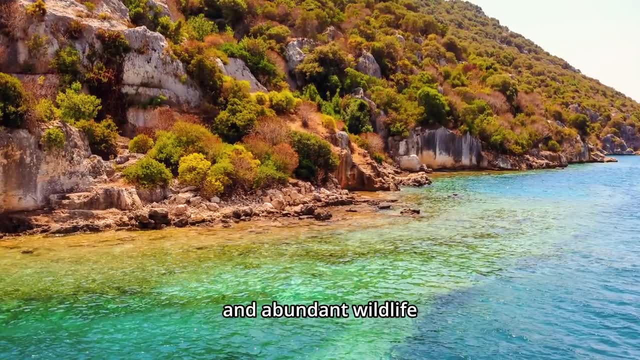 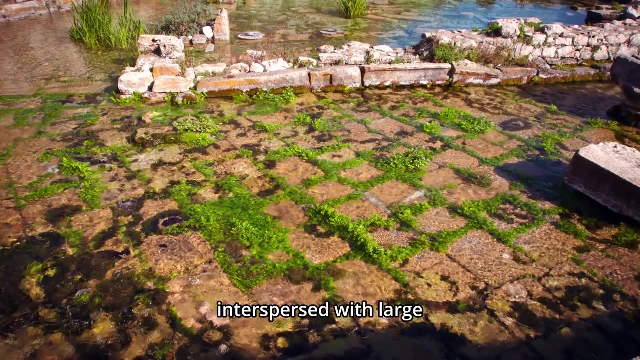 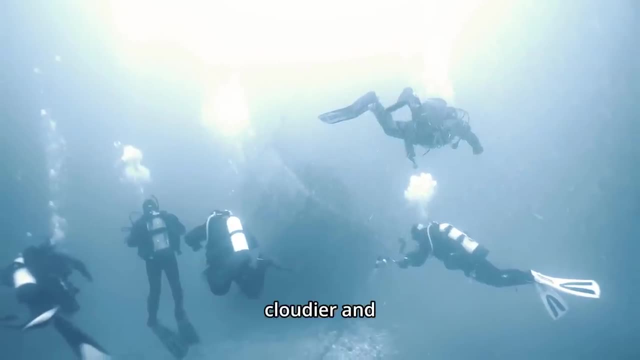 This lush landscape teemed with lakes and abundant wildlife stretching across Upper Egypt. Further to the north, the delta region featured marshy terrain interspersed with large fertile islands. During this period, the climate was markedly cooler, cloudier and notably wetter than the arid conditions we know today. 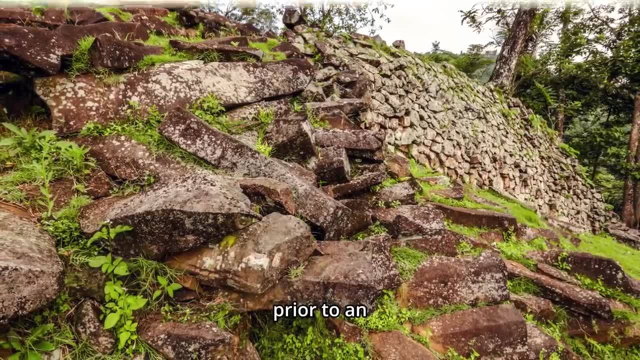 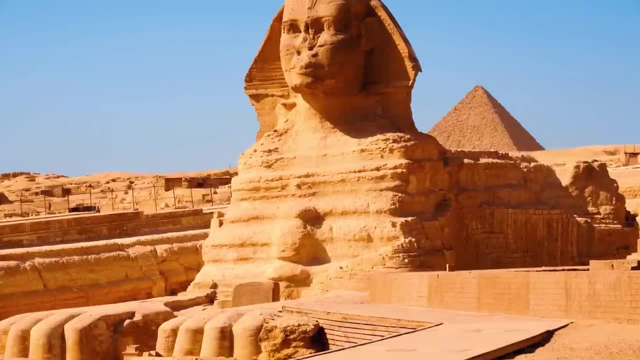 In fact, for approximately two to three millennia prior to and a millennium after 10,500 BC, the skies poured down a relentless and abundant rainfall, Following what appeared to be a pivotal ecological shift. the deluges arrived, leaving their indelible mark. 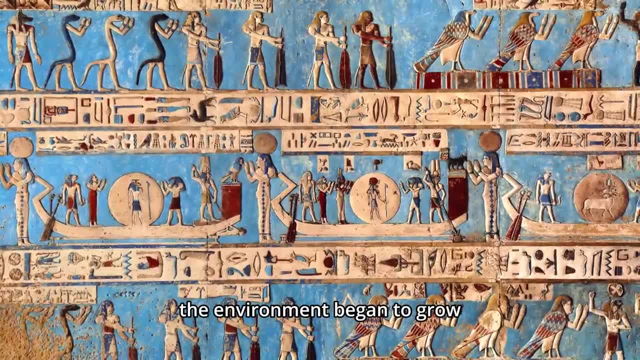 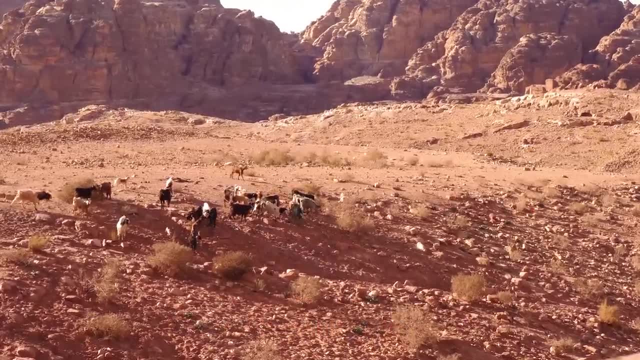 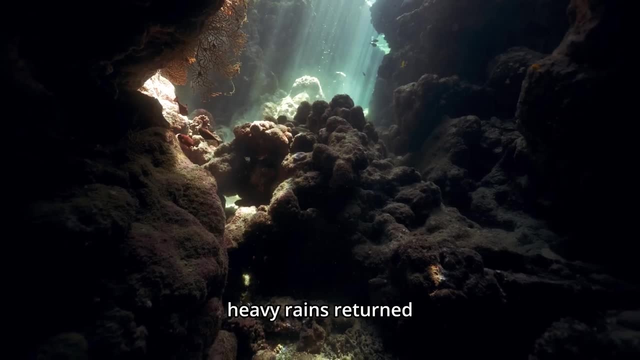 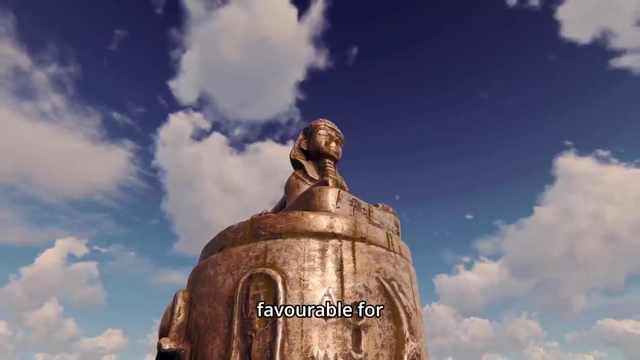 Once these floods receded, the environment began to grow progressively arid. This phase of desiccation persisted until roughly 7000 BC, giving way to a transformative era known as the Neolithic Upheaval. Over the course of a thousand years, heavy rains returned, followed by another three millennia of more moderate rainfall, creating conditions once again favorable for agriculture. 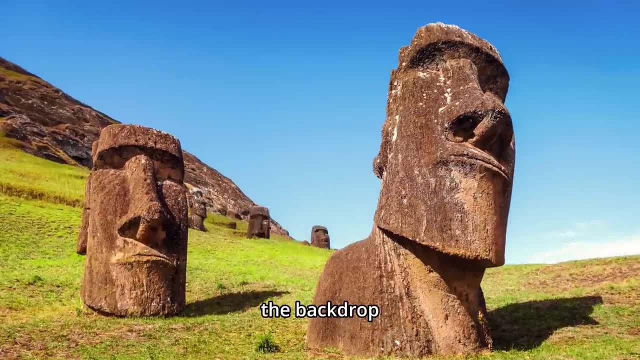 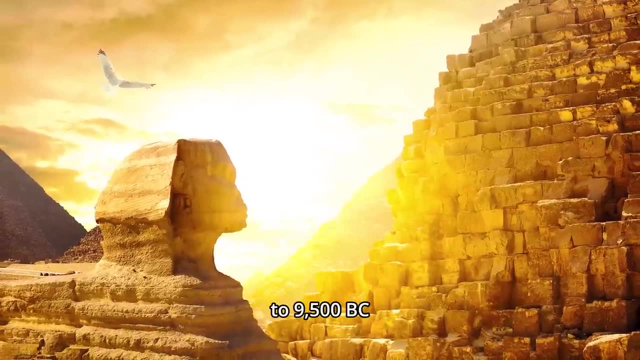 In the grand tableau of Earth's environmental changes, the backdrop for the enigma of Egyptian civilization takes form: A period of rain and floods from 13000 BC to 9500 BC, Then a prolonged dry spell until around 7000 BC. 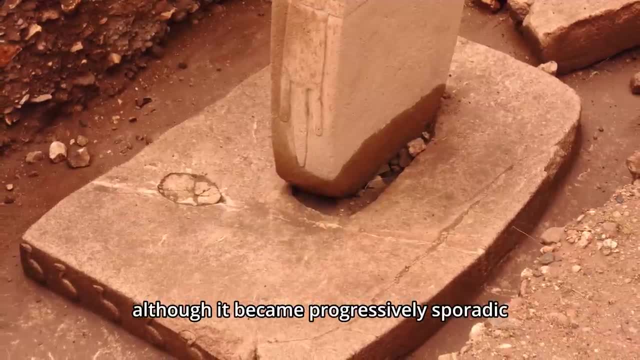 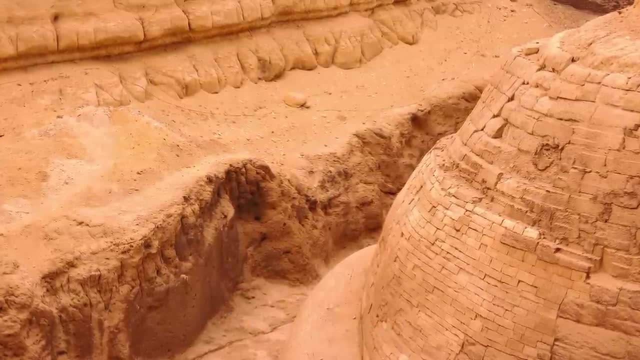 Followed by another era of rain, although it became progressively sporadic until roughly 3000 BC, And finally a return to an enduring arid phase. Graham Hancock and Robert Bauval suggest that the Sphinx's construction around 10500 BC. 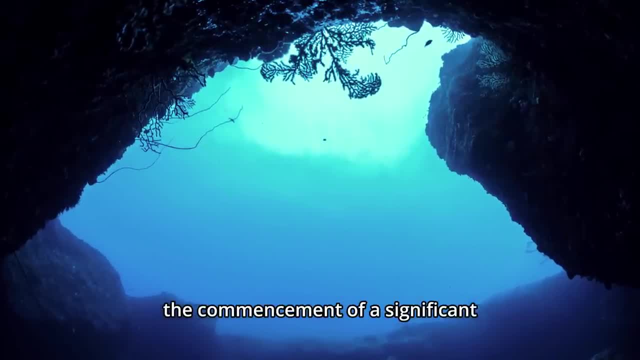 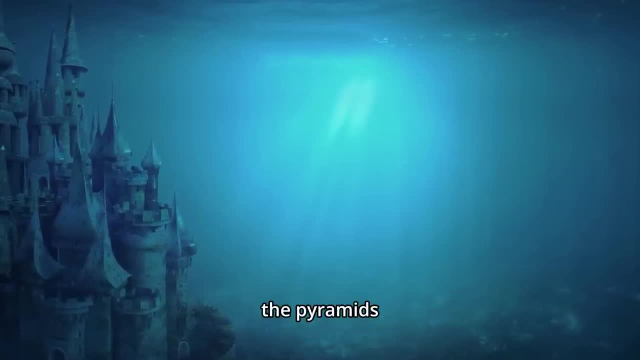 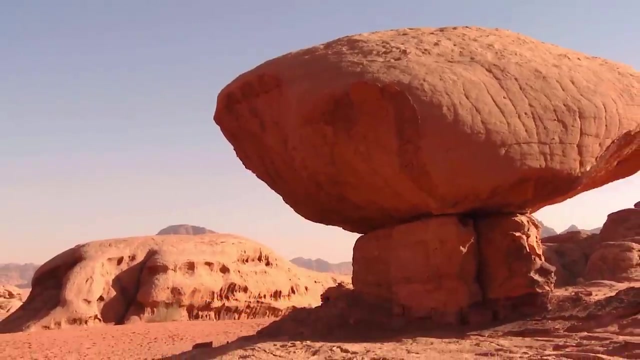 was a deliberate choice to mark the commencement of a significant astronomical cycle. These ancient astronomer priests had a plan not just for the Sphinx, but also for the pyramids. They designed the spatial arrangement of these structures to mirror the celestial pattern of Orion's belt, imparting an important message to future generations. 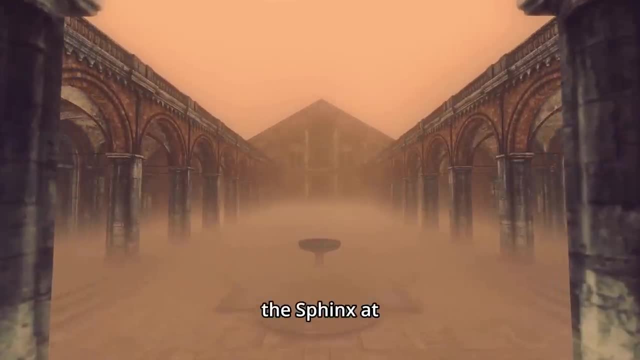 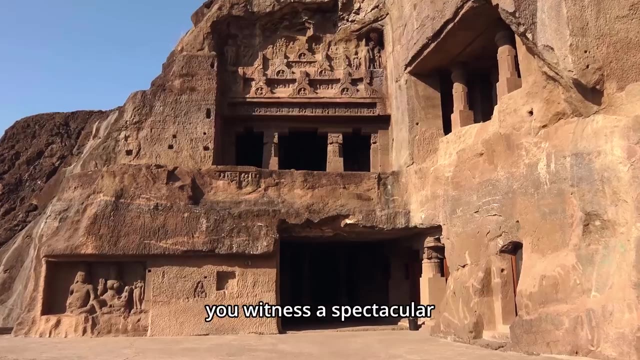 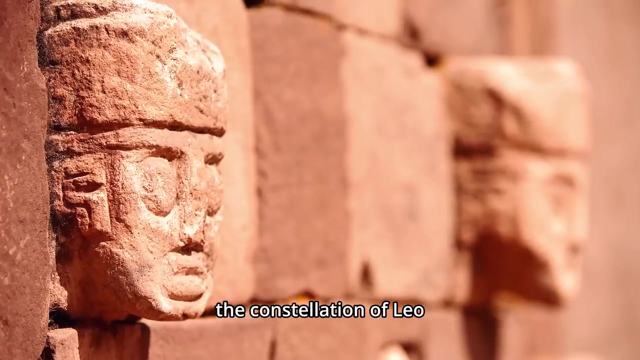 Picture yourself standing between the massive paws of the Sphinx at the break of dawn during the spring equinox of 10500 BC. As you gaze eastward, you witness a spectacular celestial event: Just moments before the sun's first rays touch the horizon, the constellation of Leo, symbolized by a majestic lion, rises majestically above the eastern horizon. It's a breathtaking alignment that marks this era and adds to the enigmatic allure of the Sphinx's origins. Now let's pivot to the south and in the vast canvas of the sky, we observe the prominent constellation of Orion. Within this constellation, the three stars forming Orion's belt are poised in an arrangement that directly mirrors the layout of the pyramids at Giza. 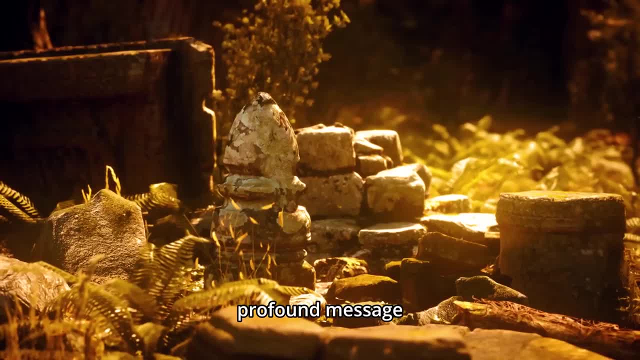 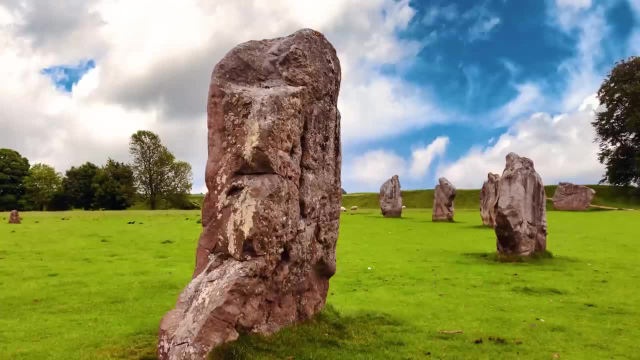 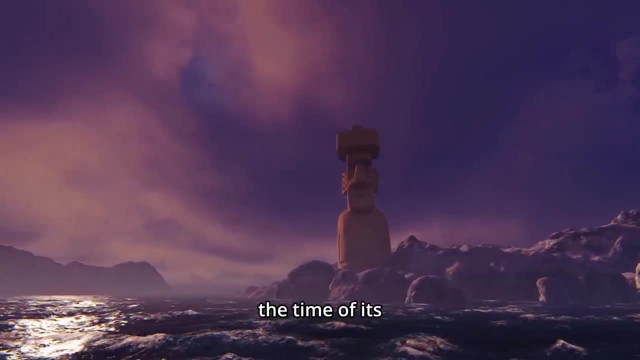 It's as if the architects of the pyramids intended to convey a profound message, not just about the construction of the Great Pyramid but also, by extension, the origins of the Sphinx. The alignment of these celestial connections speaks eloquently. The southern air shaft of the Great Pyramid marks the time of its construction. 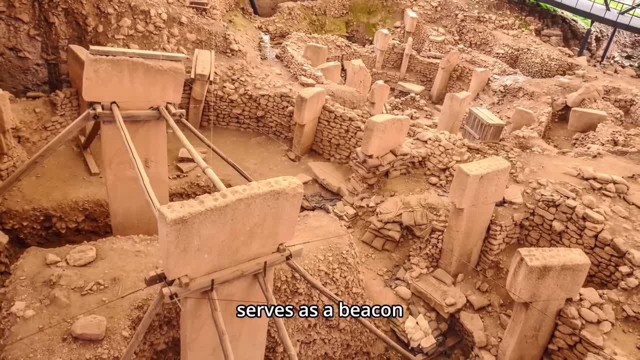 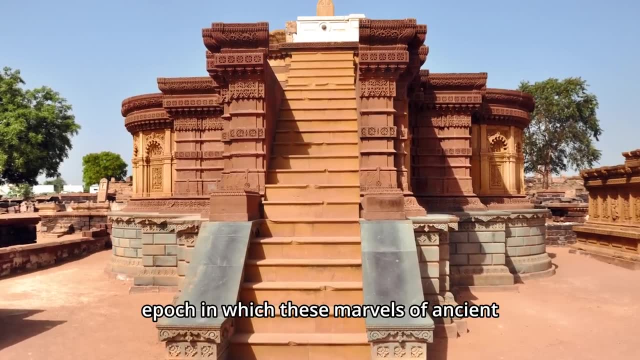 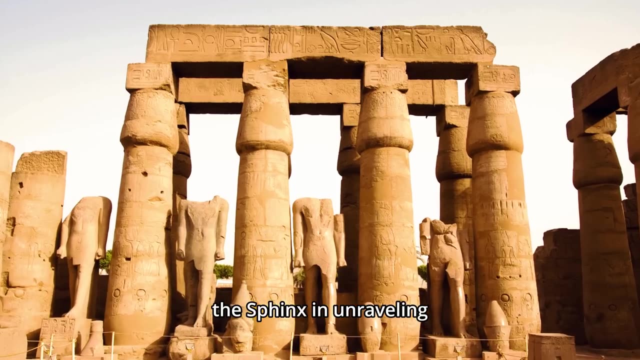 and the precise positioning of the pyramids to mirror Orion's belt serves as a beacon guiding our focus back to 10500 BC, the age of Leo, and the profound epoch in which these marvels of ancient Egypt were created. Recent investigations have unveiled the pivotal role of the Sphinx in unraveling the enigmas of human origins and our historical journey. 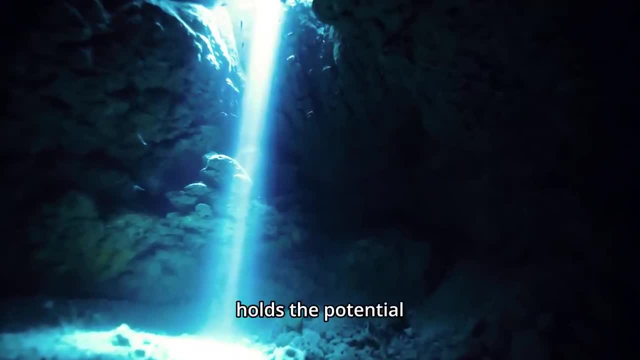 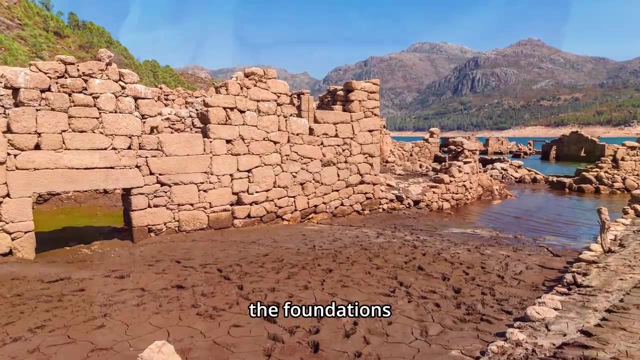 The Sphinx, like a sentinel of ancient wisdom, holds the potential to disclose the secrets of our genesis and the dawn of our existence. This quest builds upon the foundations laid by Robert Bauval's The Orion Mystery and Graham Hancock's Fingerprints of the Gods. 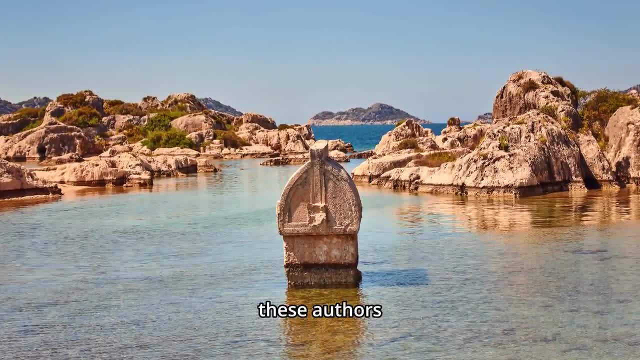 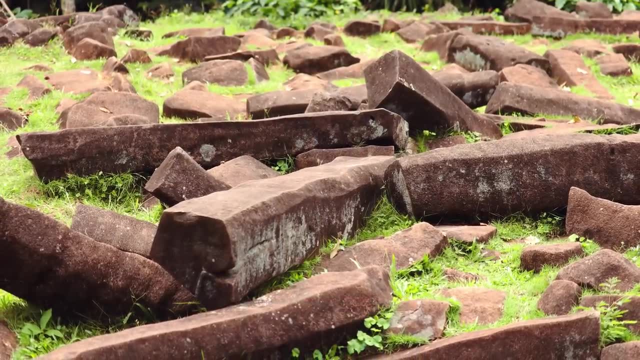 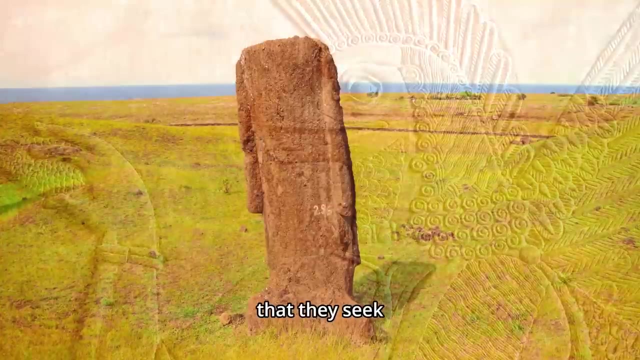 Through the marvels of computer simulations, these authors embark on a celestial time travel, transporting us to the prehistoric skies of two significant epochs: 2500 BC and 10500 BC. It is within the patterns of these astral heavens that they seek the keys to unlock the mysteries of our past and provide insights into our very origins. 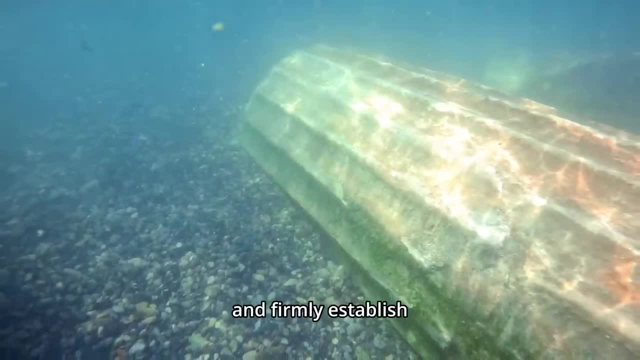 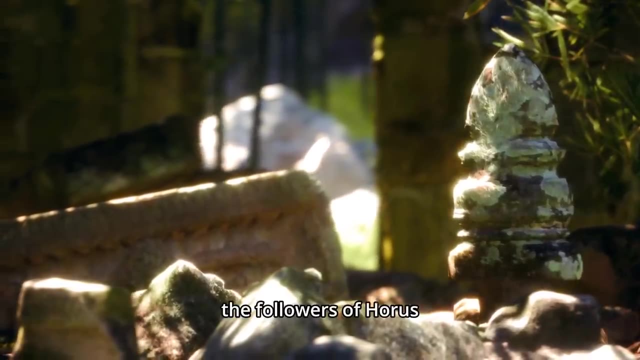 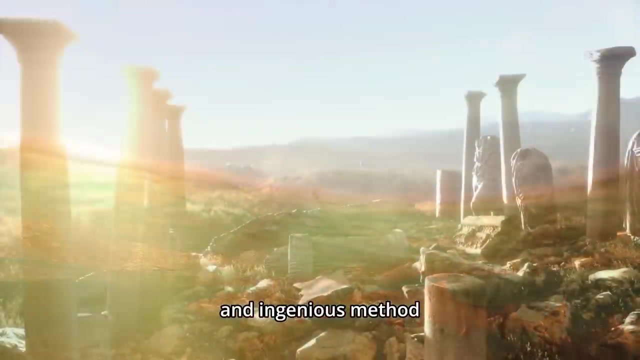 In their daring pursuit, they uncover and firmly establish a compelling hypothesis. They identify a select group of priestly custodians aptly named, the followers of Horus, who ingeniously harnessed the celestial heavens as a leguminism, a deliberate and ingenious method for the deliberate transmission and safeguarding of knowledge across the ages. 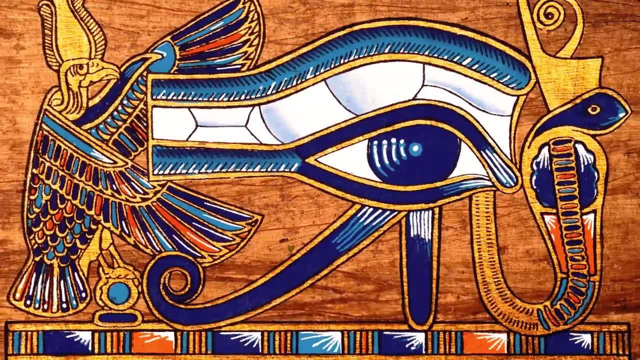 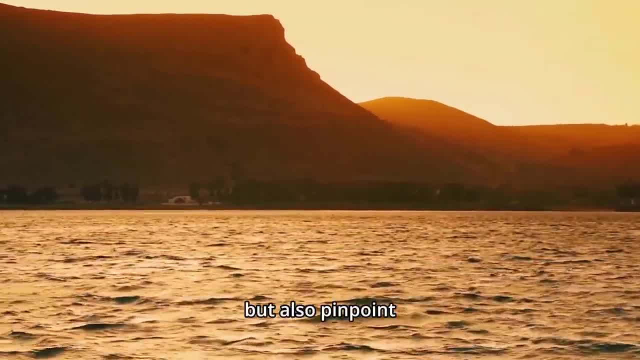 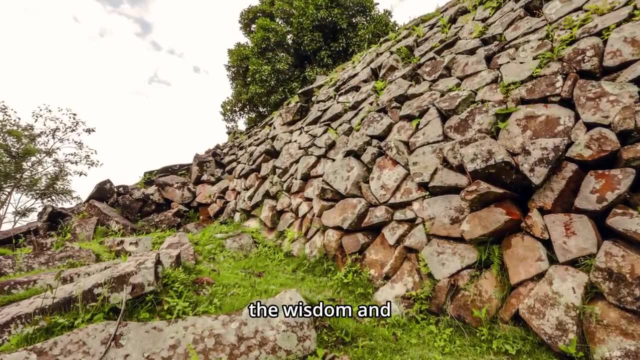 accounting for the distortions inherent to the patterns. This is the passage of time. With meticulous research, Hancock and Bauval not only offer a plausible solution to the Sphinx's enigmatic riddle, but also pinpoint the elusive Hall of Records. This fabled repository is rumored to safeguard the wisdom and insights of an exceedingly advanced prehistoric civilization. 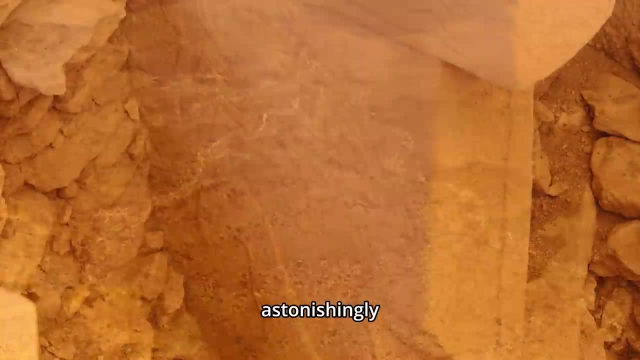 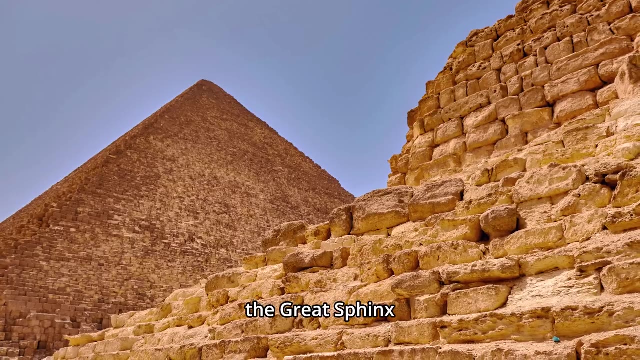 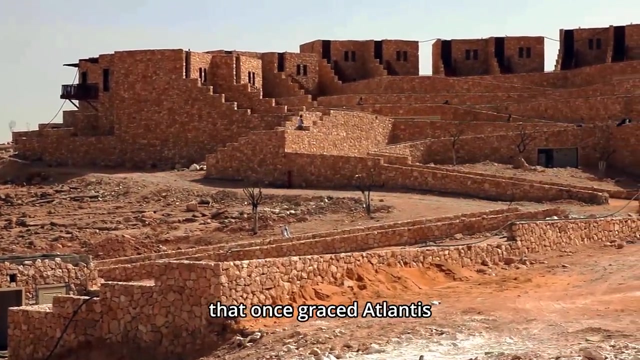 that succumbed to a colossal Great Flood. Astonishingly, their quest leads them to conclude that this hidden trove lies a mere hundred feet beneath the mighty hind paws of the Great Sphinx. Gurdjieff delved into the profound inner significance of the original prototype of the Great Sphinx that once graced Atlantis. 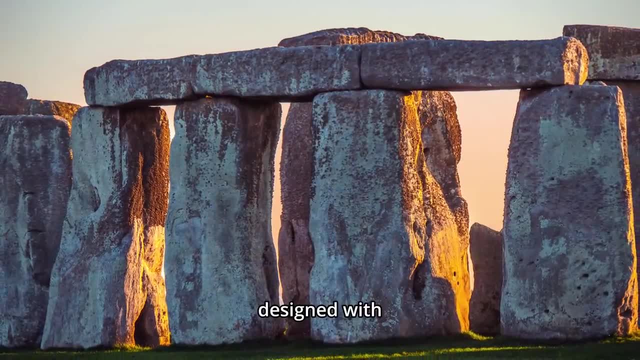 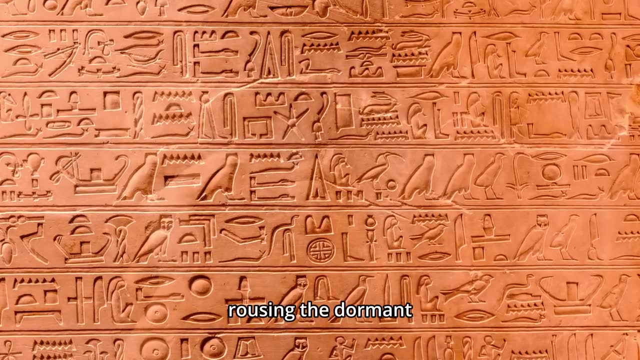 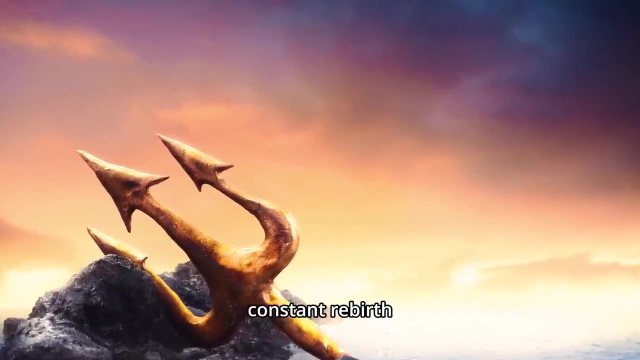 This allegorical figure was a deliberate instrument designed with the purpose of delivering a profound shock or stimulus to the very core of human existence, rousing the dormant consciousness that resides within each individual. The symbol of the trunk, as the bull, embodies the idea of constant rebirth and rejuvenation. 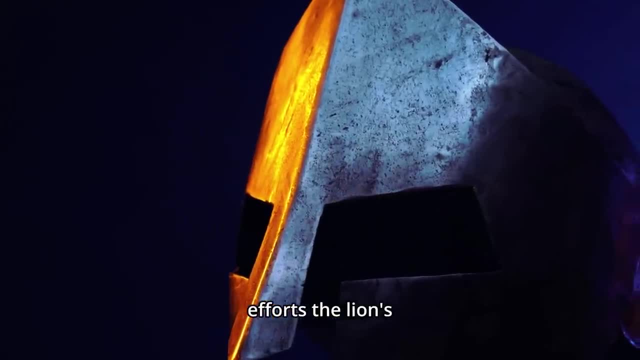 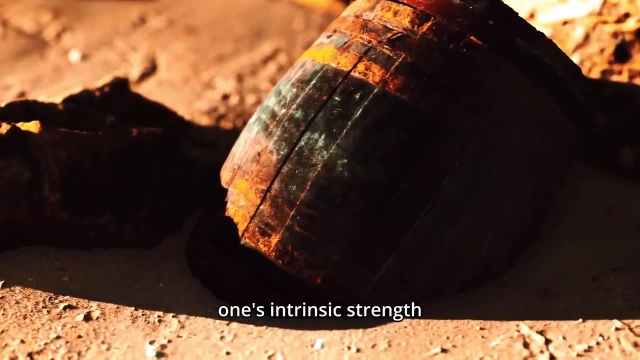 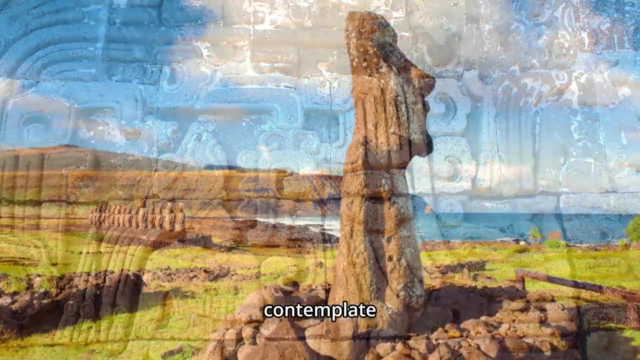 achieved through unwavering diligence and tireless efforts. The lion's legs evoke the attributes of courage, self-esteem and a profound belief in one's intrinsic strength to surmount life's challenges. The wings of the majestic eagle serve as a reminder to persistently contemplate the most profound questions concerning life and the nature of existence. 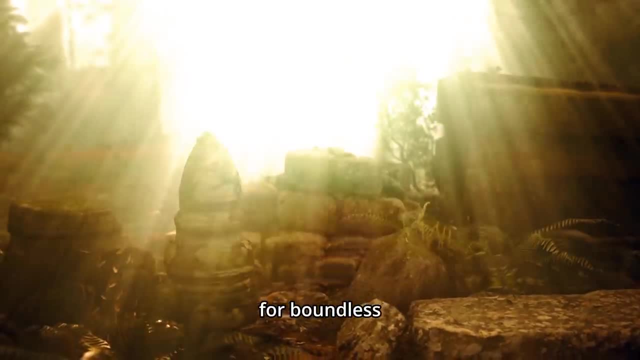 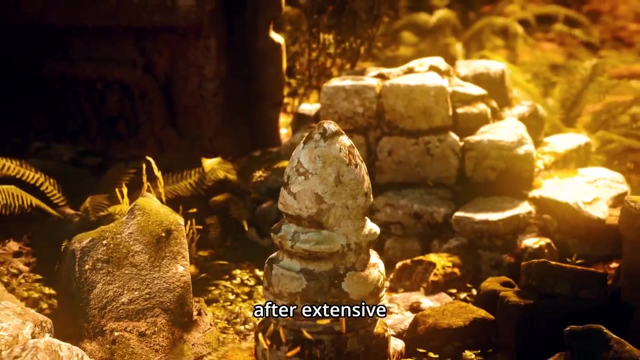 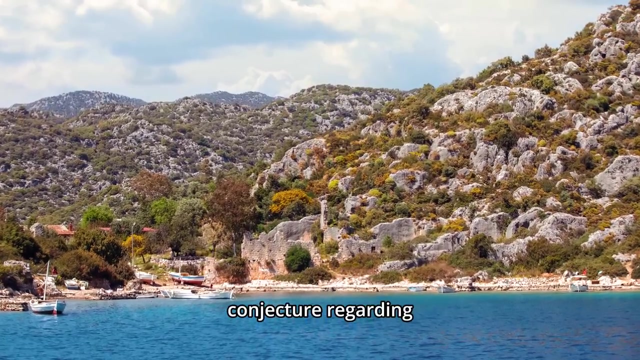 The head resembling the breast of a virgin conveys the desire for boundless love to reign perpetually both in inner and outer functions of one's conscious existence. After extensive research into the cultures of prehistoric and ancient worlds, Graham Hancock ventures into the realm of conjecture regarding the possible intentions of the pyramid builders. 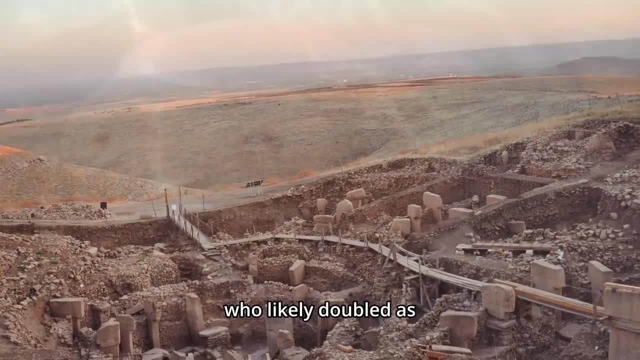 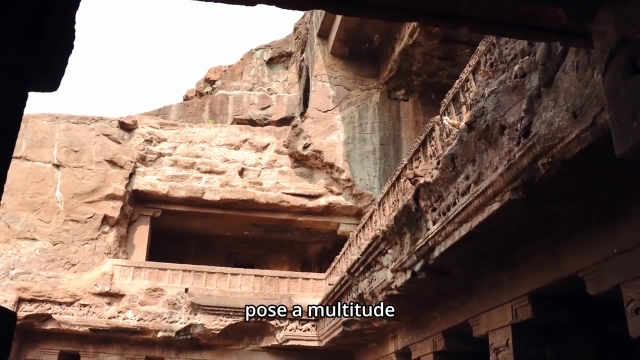 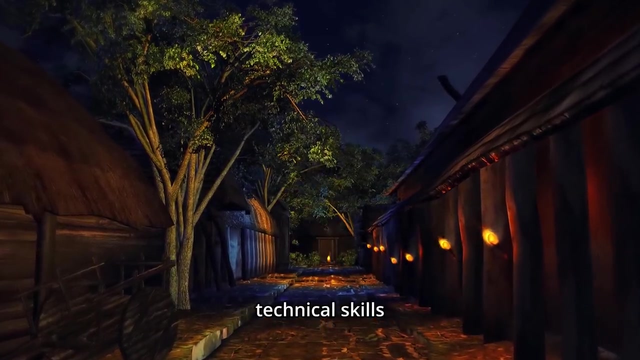 These enigmatic individuals, who likely doubled as the cryptic cartographers charting the globe during the waning days of the last ice age in the northern hemisphere, pose a multitude of questions. Among these, one might ponder the following: Why did these people possessing advanced technical skills and a high degree of civilization 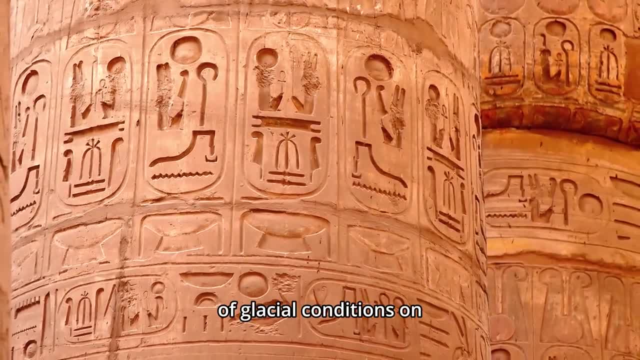 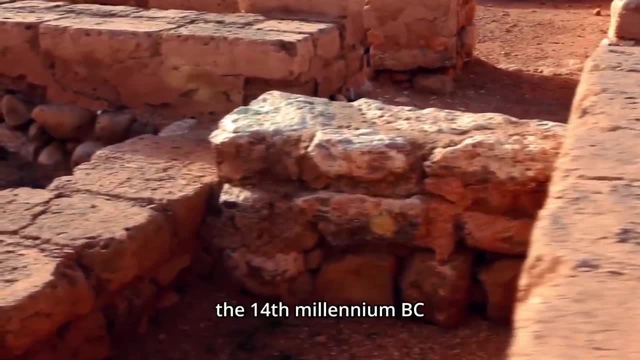 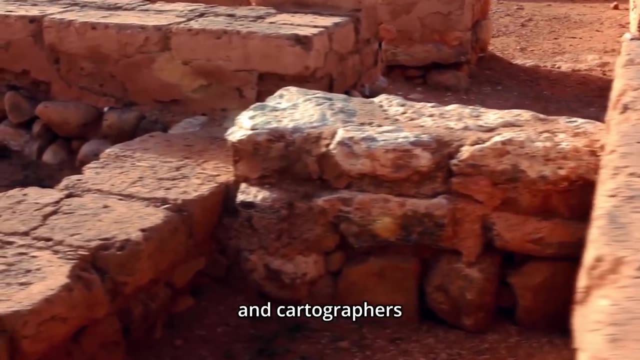 become so fixated on meticulously documenting the gradual encroachment of glacial conditions on the mystifying southern landmass of Antarctica. This obsession apparently spanned from around the 14th millennium BC to the conclusion of the 5th millennium BC. Might these ancient architects and cartographers have embarked on the ambitious task of creating a lasting cartographic testament. 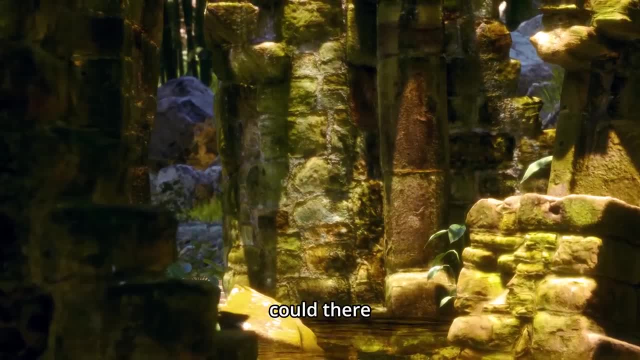 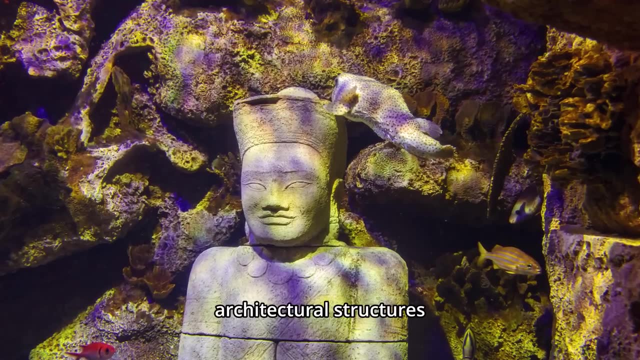 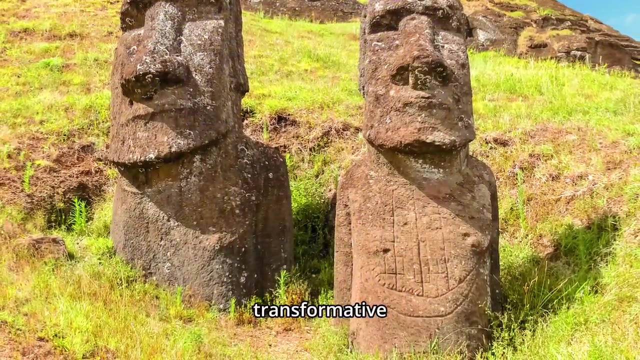 to the gradual obliteration of their own homeland, Could their intense drive to communicate a message to posterity through a multitude of mediums, including myths, maps, architectural structures, calendrical systems and mathematical harmonies, have been linked to the cataclysmic upheavals and transformative geological events responsible for this loss. 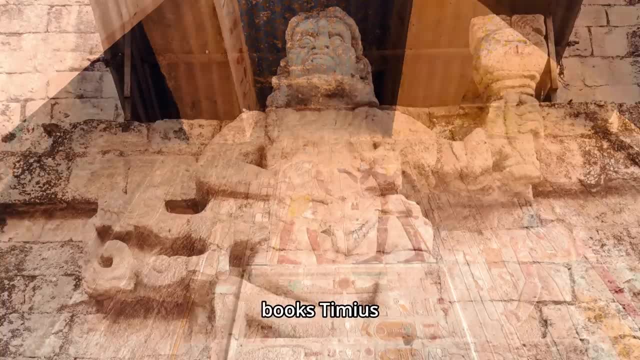 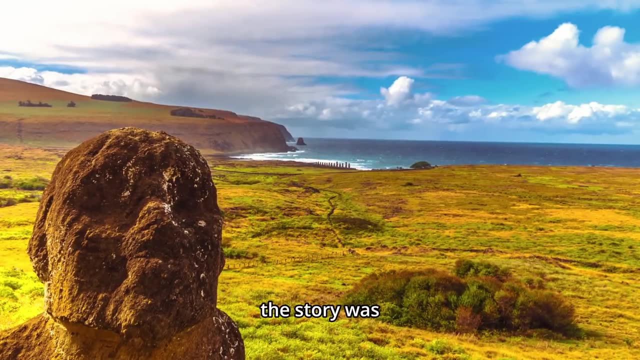 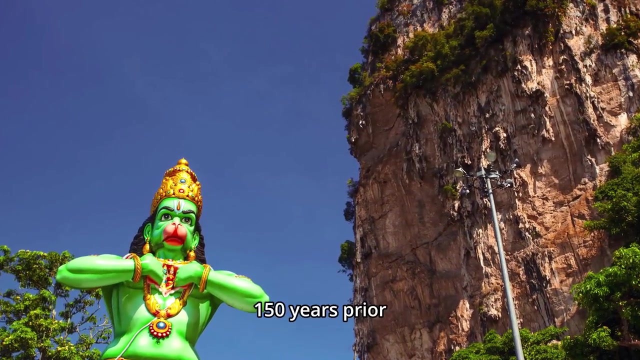 Chapter 2 In Plato's accounts found in the books Timaeus and Criscus, he shares a tale of a magnificent empire that thrived in the distant past. The story was relayed by an Egyptian priest from Sais to Solon during his visit to Egypt roughly 150 years prior to Plato's era. 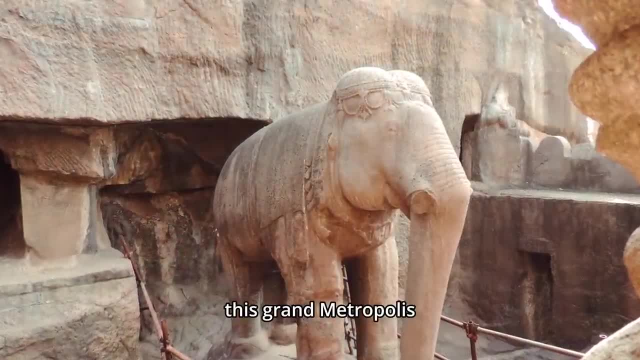 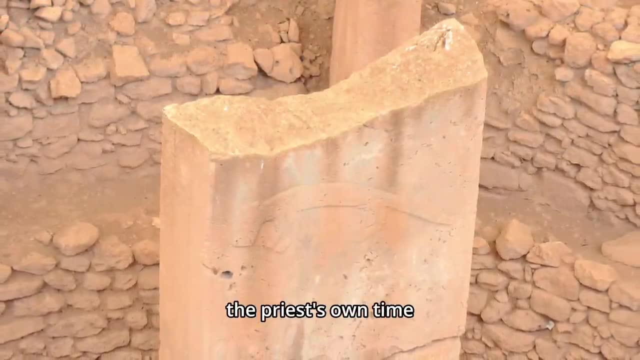 According to the priest's account, this grand metropolis, which served as the epicenter of a powerful empire, had flourished a staggering 9,000 years before the priest's own time. Remarkably, this city situated on the far side of the Atlantic. 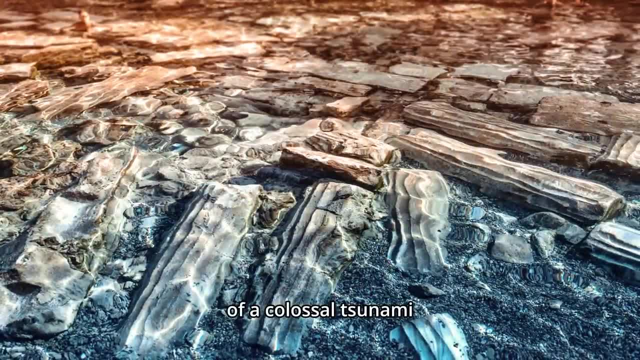 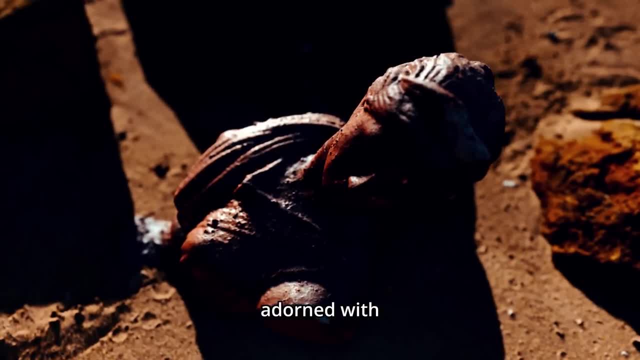 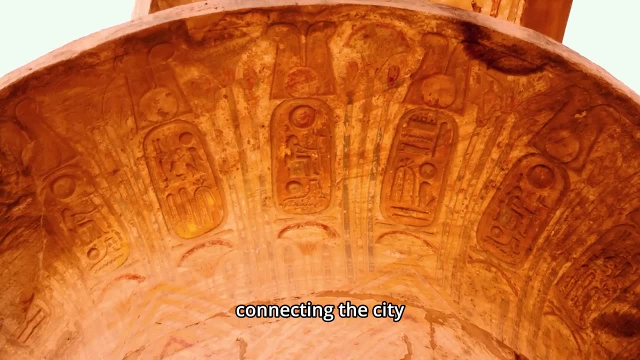 met its demise in a catastrophic event reminiscent of a colossal tsunami. At the heart of Atlantis, the fabled island there, lay an exquisite capital city adorned with intricate details. It boasted a protected harbor that facilitated the departure and arrival of ships, connecting the city with far-flung destinations across the globe. 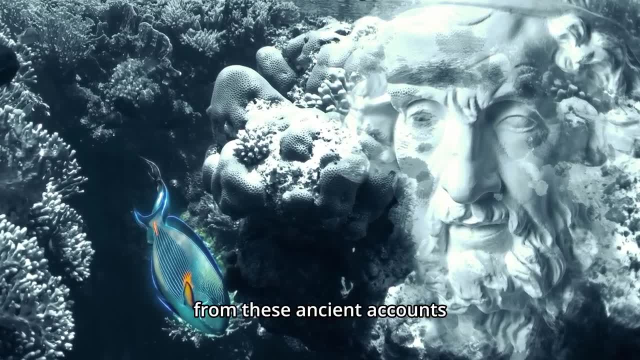 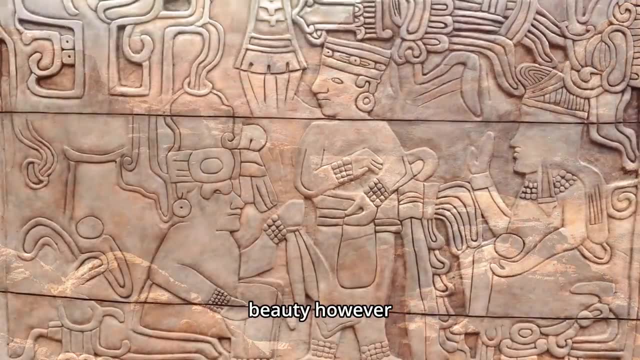 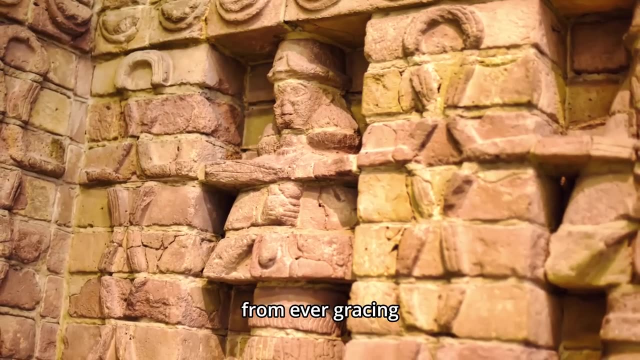 The treasure trove of knowledge collected by Solon from these ancient accounts, as relayed by Plato, held the potential to inspire an epic poem of unparalleled beauty. However, the sands of time and the constraints of Solon's own life prevented this poetic masterpiece from ever gracing the written page. 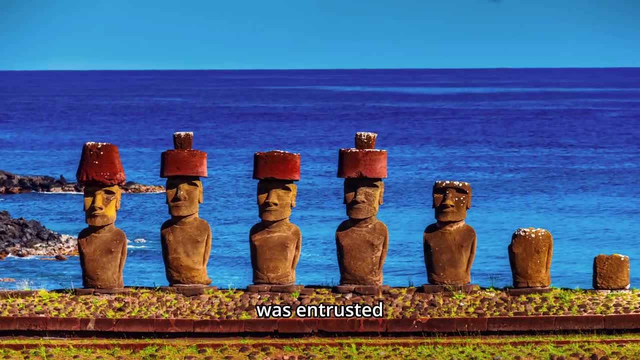 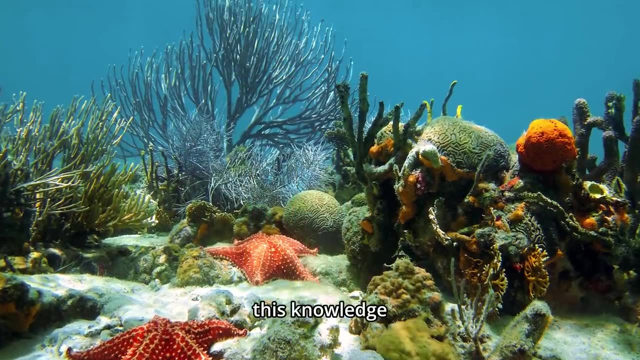 The tale, as relayed by Plato in his work, was entrusted to an elderly sage named Criscus Junior, who had reached the ripe age of 80. He shared that this knowledge had been handed down through the generations originating with his grandfather. 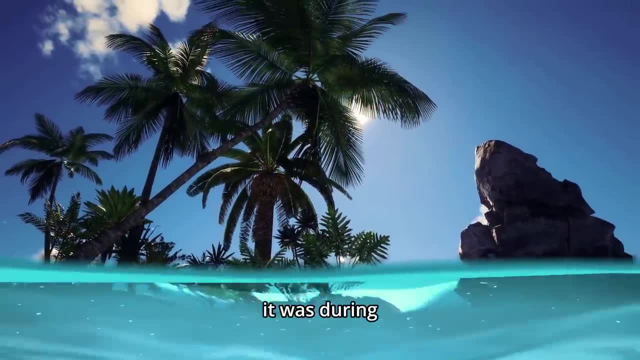 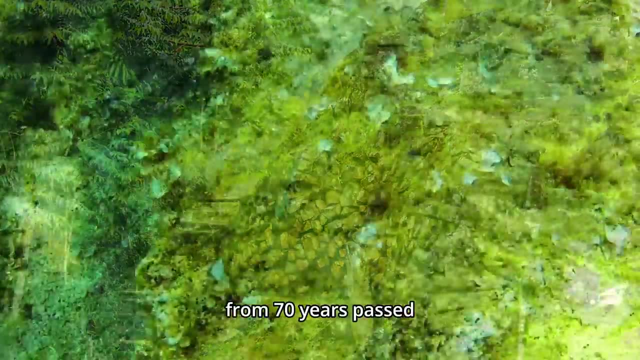 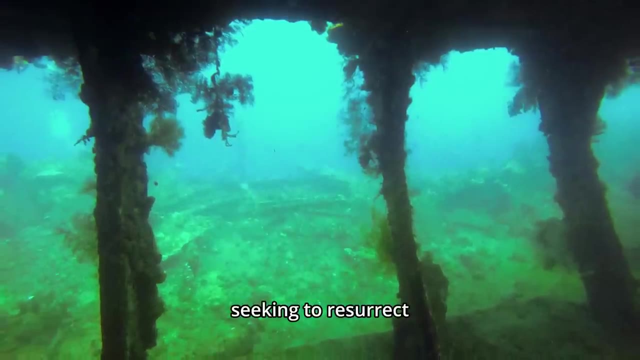 a familial connection to the wise Solon. It was during a festive occasion when Criscus was a mere 10-year-old that he first encountered this narrative, an ancient echo from 70 years past Enshrouded in the mists of time. he embarked on a night of contemplation seeking to resurrect the vivid details of that long-ago story. In contrast to what some may assume, the tale of Atlantis was not a narrative born solely from Plato's quill. Evidence points to its existence in pre-Platonic times. Fragments of a lost poem by Hellanicus of Lesbos, believed to predate Plato's works, allude to the enigmatic island. 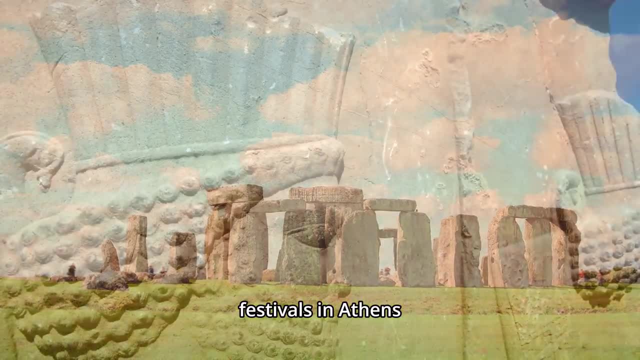 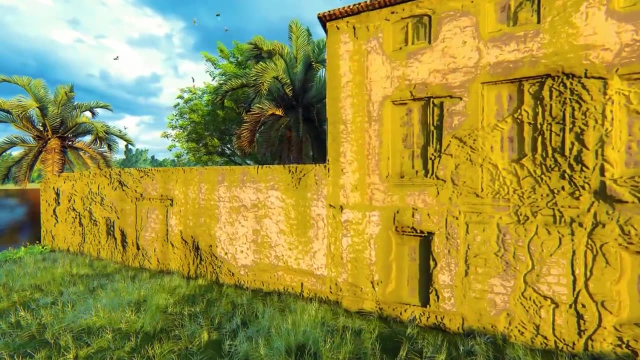 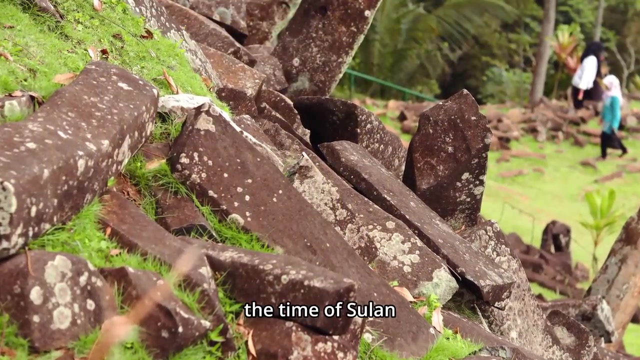 Furthermore, during the grand Panathenaic festivals in Athens which precede Plato's era, ornate peplar displayed artistic depictions of this ancient saga. With knowledge of the story's presence in Egypt, it becomes plausible that Pythagoras, who traversed those lands around the time of Solon, may have been privy to this enigmatic legend. 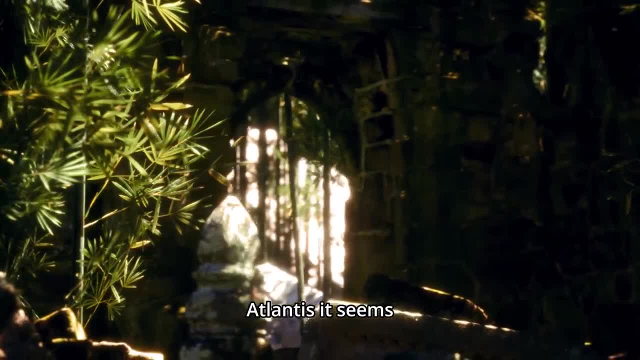 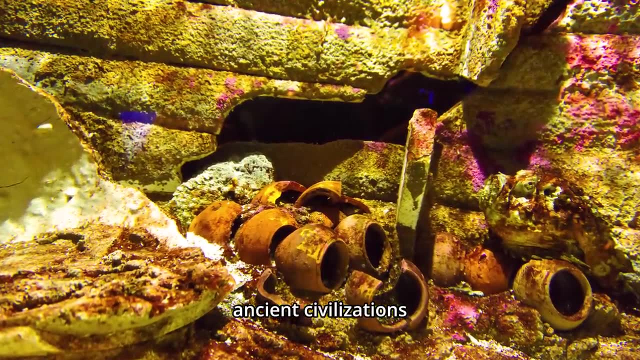 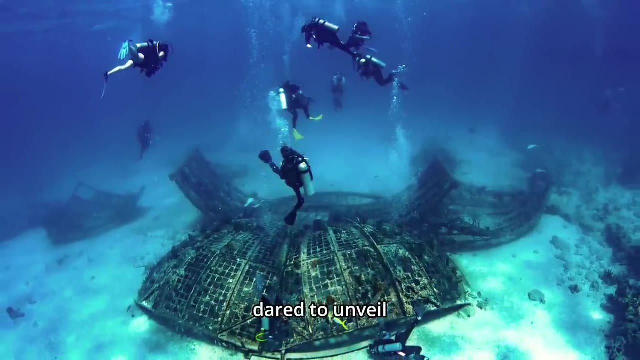 Atlantis, it seems, was a tale with roots extending deep into the annals of time, known to a select few across various ancient civilizations. The teachings of Pythagoras were shrouded in secrecy, guarded by stern consequences for those who dared to unveil its mysteries, a practice that persists in certain modern-day faiths like the Ishmaelite and Druze religions. 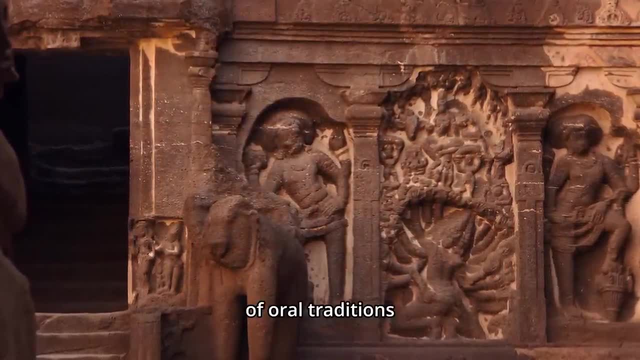 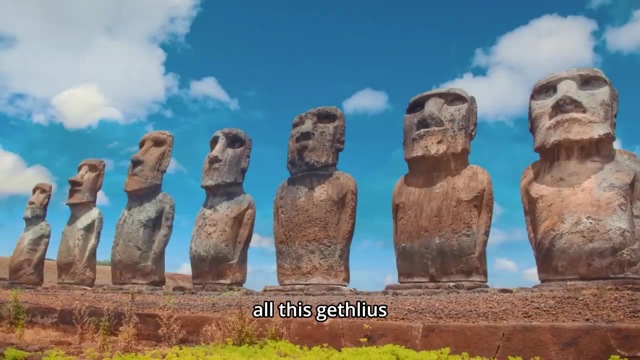 The Pythagorean wisdom was disseminated through a combination of oral traditions and written texts, Creating a delicate balance between the spoken word and the written page. Aulus Gethlius, a historical source, recounts a fascinating tale of two exceptionally prized books. 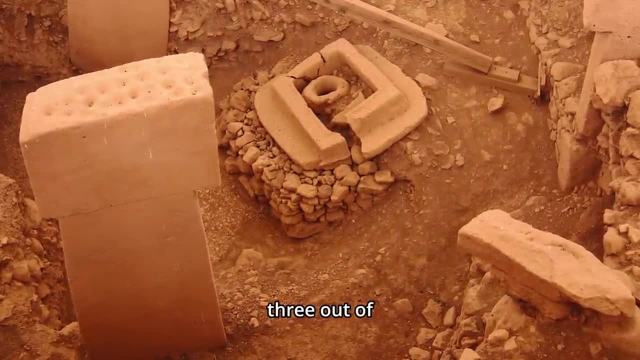 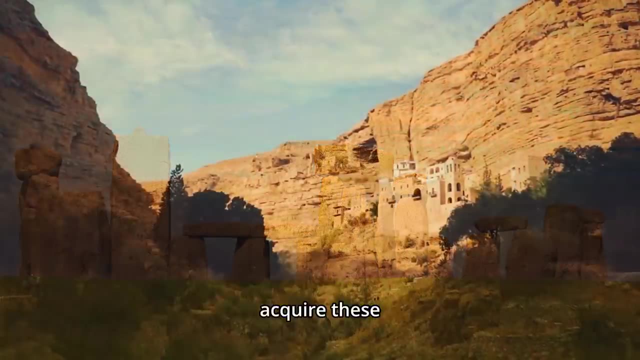 These were none other than the Sibylline books, of which only three out of a total of nine were initially offered for sale. It's told that King Tarquinius Severus of Rome hesitated to acquire these books when first presented with the opportunity, perhaps due to the weighty responsibility that their possession would entail. 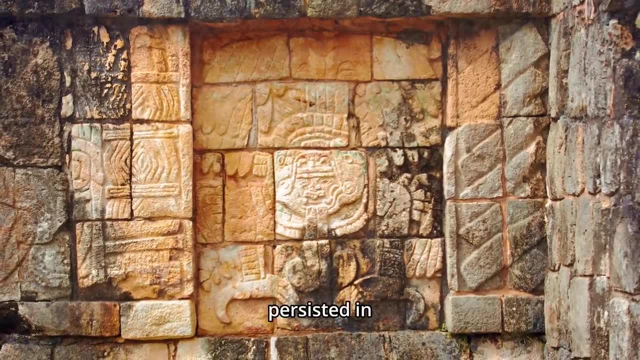 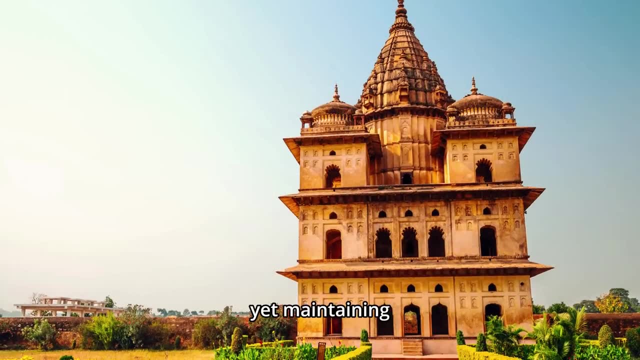 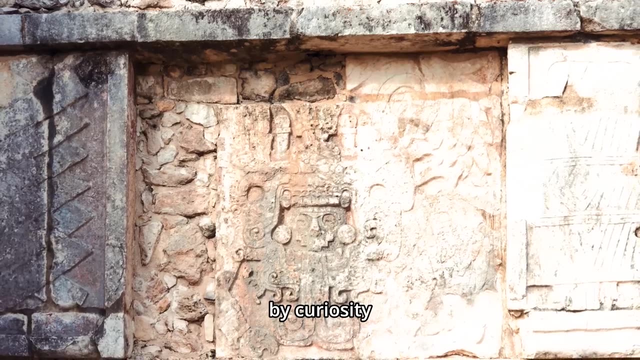 In a curious twist, the merchant selling the Sibylline books persisted in offering them to King Tarquinius Severus, even after destroying three of the nine volumes, then three more, yet maintaining the original price. It was only when the trio of books remained that Tarquinius, perhaps driven by curiosity or a sense of destiny, made the purchase. 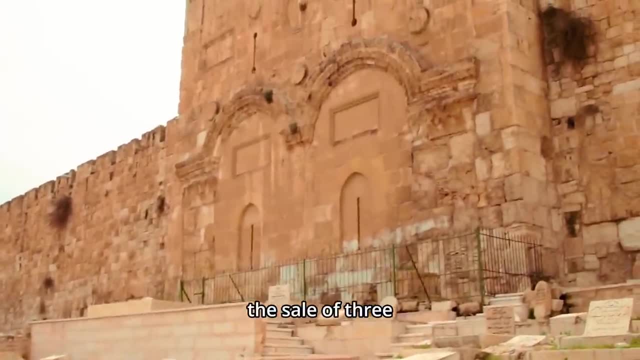 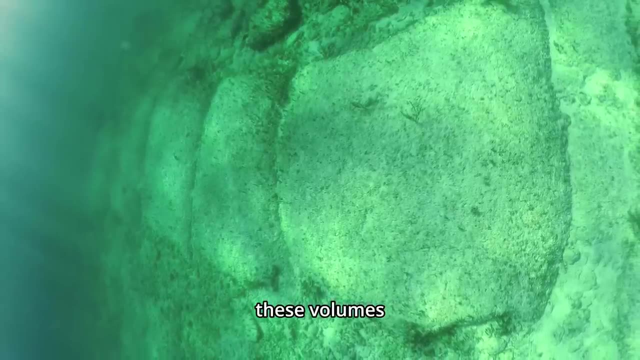 The transmission of Pythagorean wisdom also involved the sale of three significant books by the Pythagorean philosopher Philolaus to the renowned philosopher Plato. These volumes, once acquired by Plato, became the foundational source material for his work Timaeus. 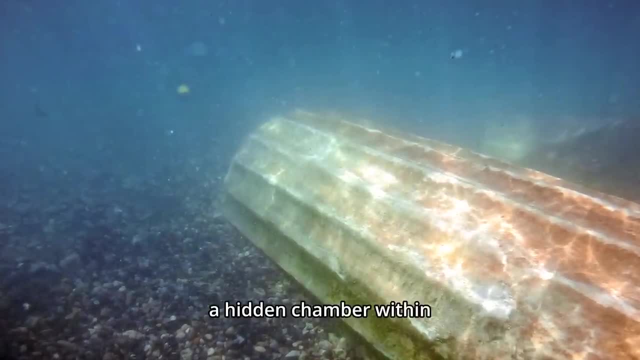 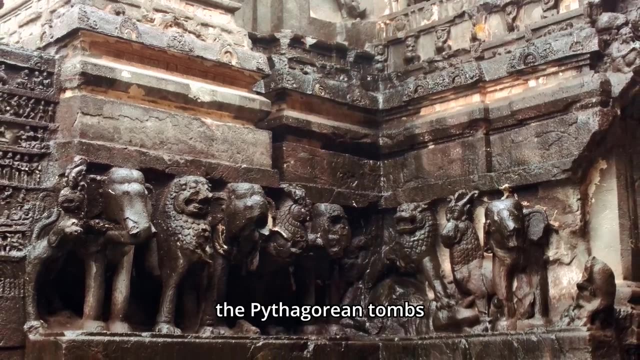 Plato's intricate dance with knowledge, enigmatic as a hidden chamber within the heart of Atlantis, may indeed hold secrets locked away. If he drew from the Pythagorean tomes, the oath of silence might have shackled his quill, preventing direct quotations and leaving gaps in the written legacy. 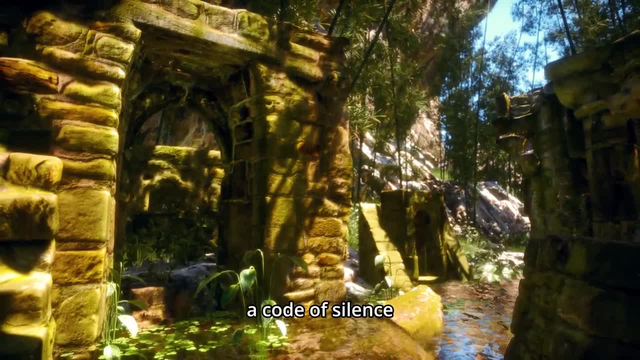 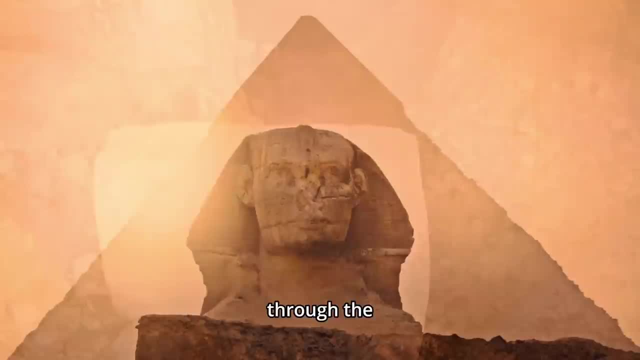 The mysteries that shroud Timaeus become a code of silence. It is only by leaving scholars to fathom the concealed wisdom that dwells in the enigmatic crevices of this ancient tale. Through the tapestry of time, the tale of Atlantis has woven a thread that binds generations. 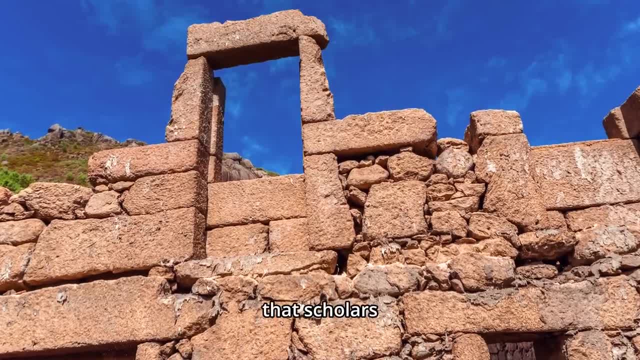 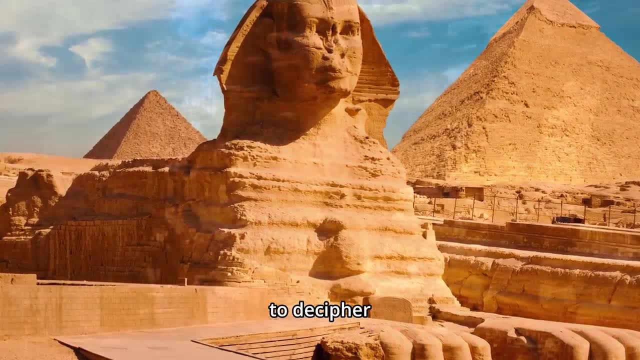 Since antiquity it has been a riddle that scholars and seekers have tirelessly pondered. Even now, its siren call still beckons to those who seek to decipher the enigmatic story. From philosophers to astronomers, this narrative remains a celestial body in the intellectual cosmos. 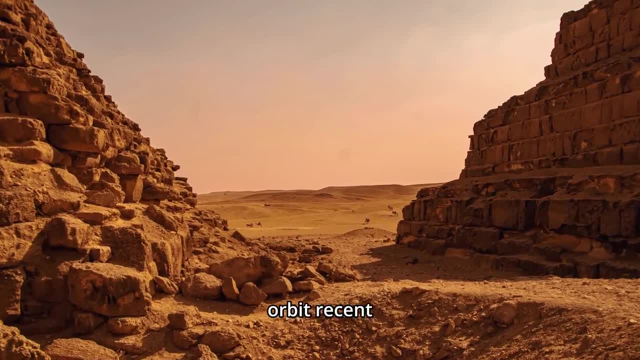 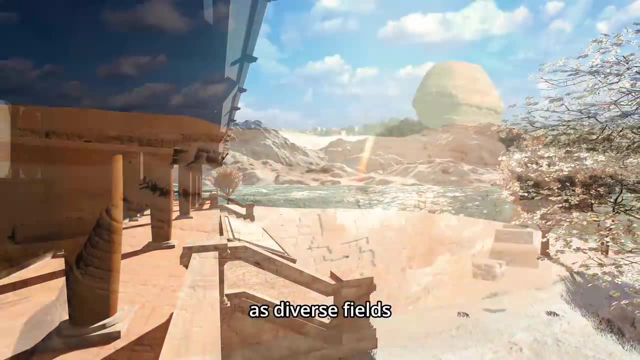 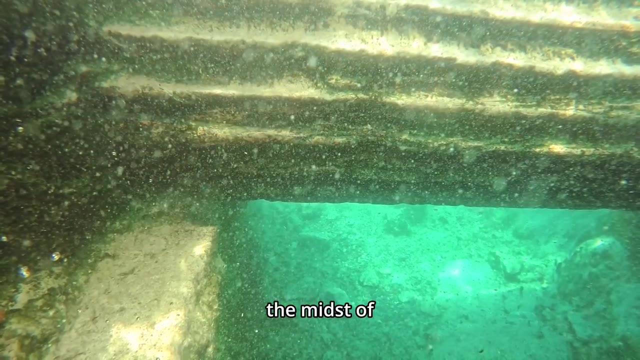 Pulling curious minds into its orbit. Recent conferences hosted by Greek universities bear testament to the enduring allure of Atlantis, as diverse fields and thinkers continue to delve into its mysteries. The origins of human existence remain veiled in the mists of time, an enigma still waiting to be unraveled. 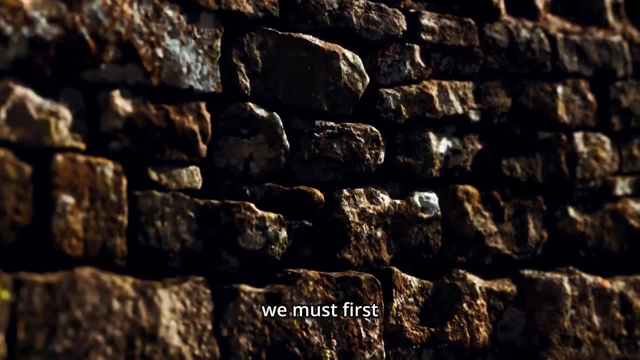 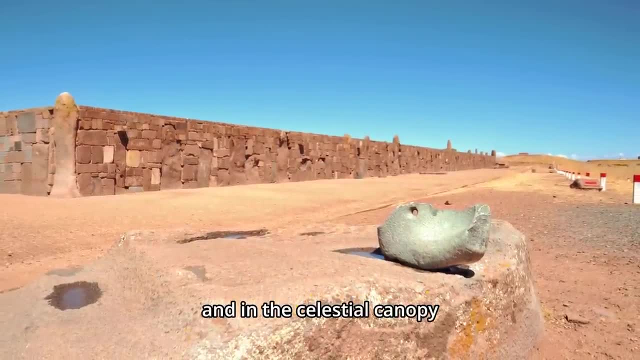 Yet to bridge the chasm of our ignorance, we must first recognize a forgotten civilization that charted the contours of our world, both on the Earth's surface and in the celestial canopy, long before the annals of the earliest known societies were even penned. 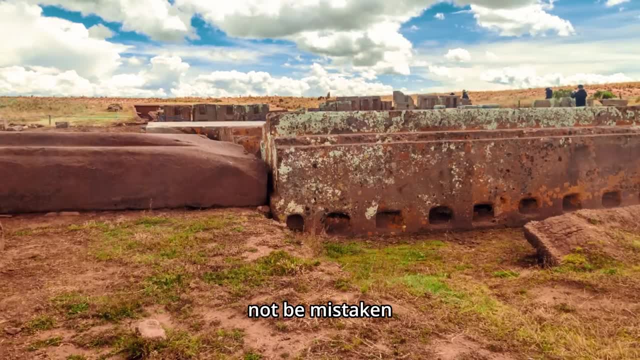 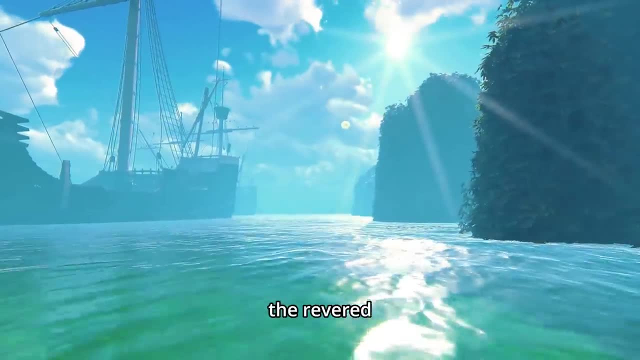 Let us be clear that these enigmatic pioneers should not be mistaken for Neanderthals or primitive cave-dwellers. They are not the hazy specters of the past, but the revered divine figures etched into the collective memory of ancient civilizations. 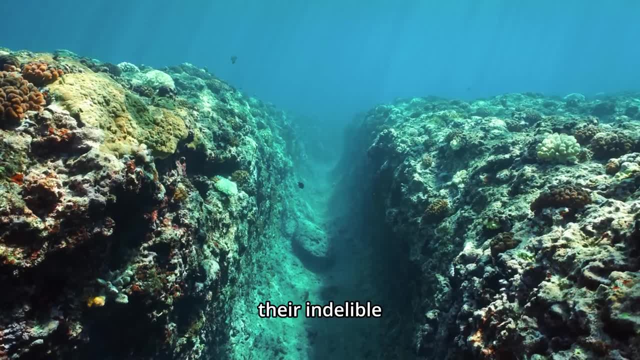 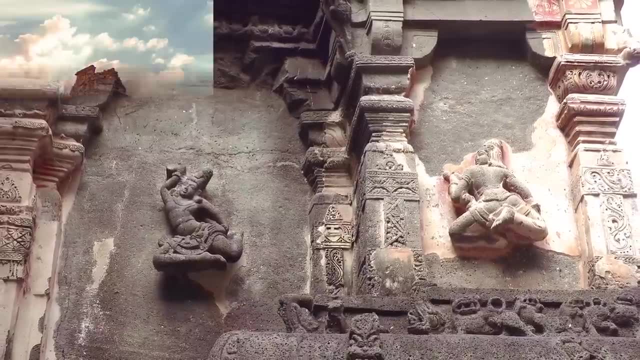 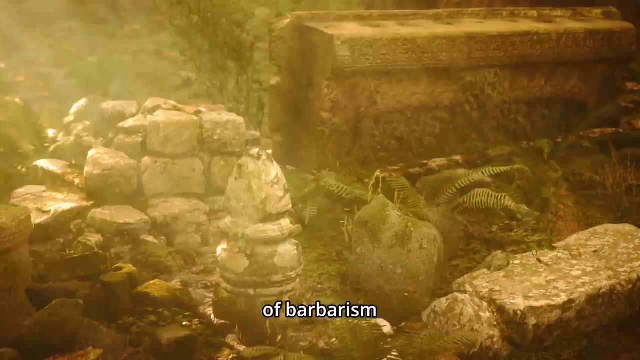 They are the architects of societies, their indelible footprints echoing through the ages, scattered like cryptic puzzle pieces across the tapestry of our planet. The prevailing historical narrative often depicts our human ancestors as primitive beings evolving from a state of barbarism towards higher intelligence and sophistication. 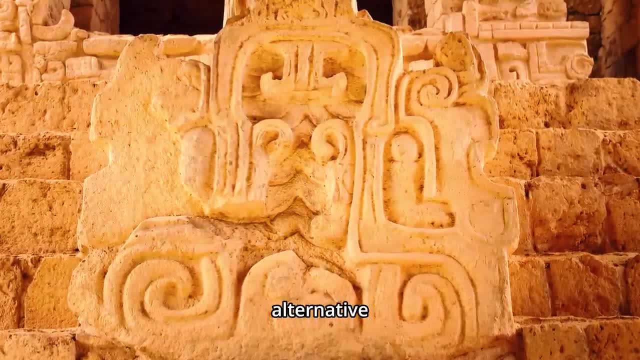 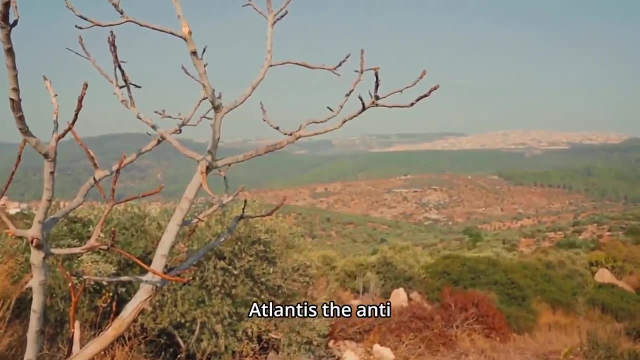 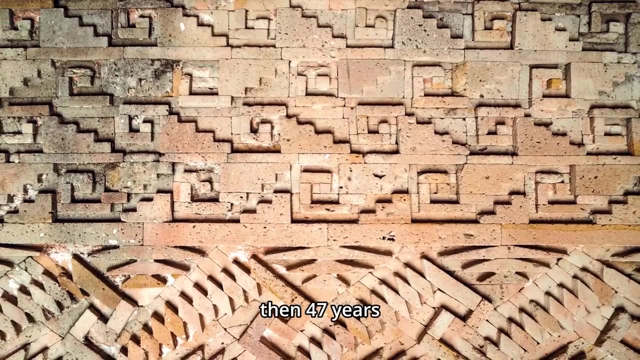 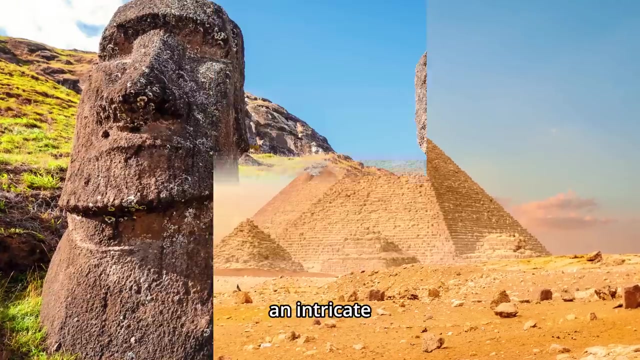 Yet the tides of evidence now reveal an intriguing alternative. In 1882, Ignatius Donnelly boldly released his groundbreaking work Atlantis: the Antediluvian World, championing the existence of advanced civilizations in ancient times. Then, 47 years later, in 1929, the pages of history unveiled another enigma: the Piri Reis map, an intricate medieval cartographic creation. 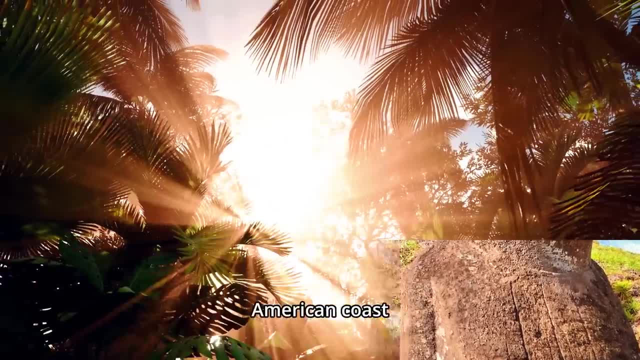 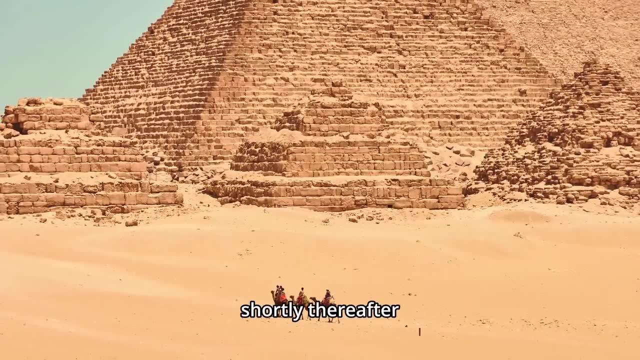 This remarkable map not only charts the South American coast, but also reveals a depiction of Antarctica as it existed before the icy embrace of the last glacial age. Shortly thereafter, a series of astonishingly precise maps appeared. These maps emerged, shedding further light on this ancient enigma. 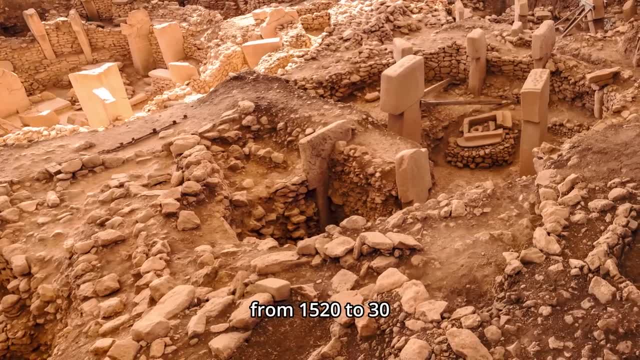 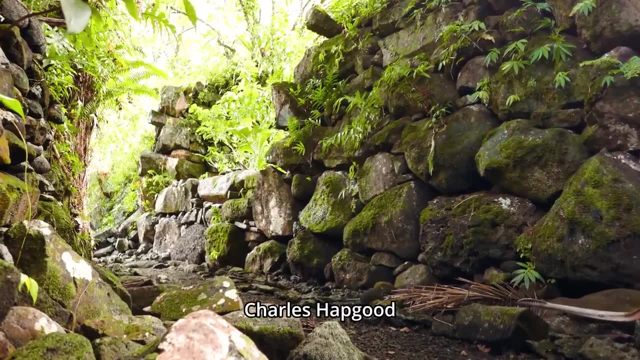 These included the Ribeiro maps from 1520 to 30,, the Ortelius map of 1570, and the Wright-Molineux map of 1599.. It was Charles Hapgood who took up the mantle of scrutiny, dedicating extensive study to these maps. 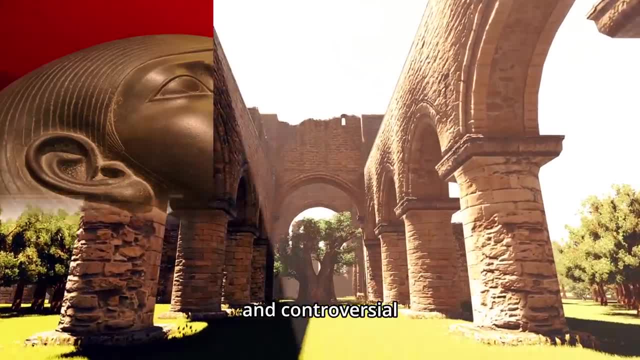 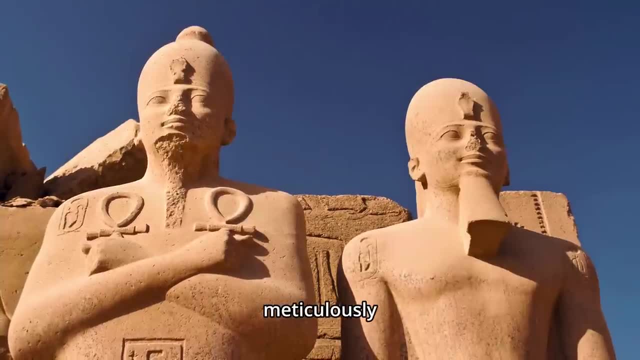 His determined research led him to a remarkable and controversial conclusion. An advanced civilization existing in the depths of history had not only thrived, but had also meticulously mapped the entire Earth. Hapgood's daring theory centered around Earth-crustal displacement. 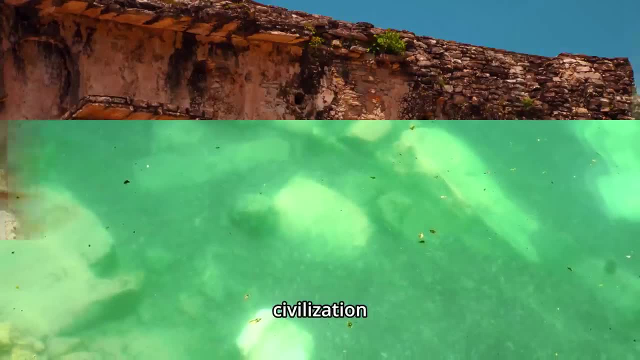 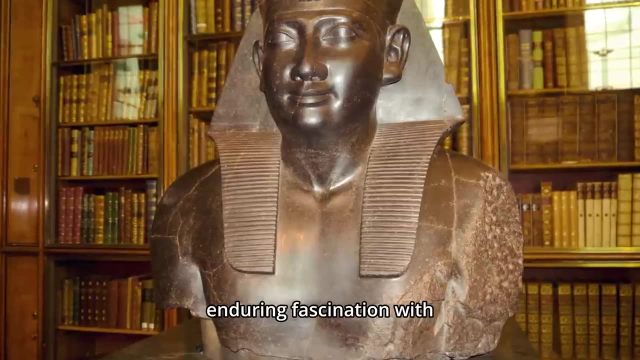 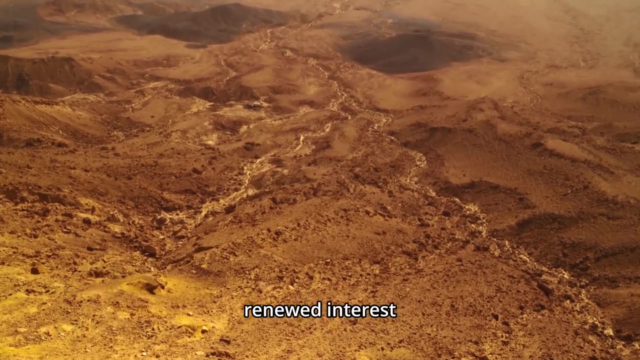 a radical concept that included the presence of a pre-existing civilization in Antarctica. This unconventional idea captured imaginations and led to an enduring fascination with the subject. Brad Steiger, in his 1978 book Worlds Before Our Own, renewed interest in this mysterious domain. 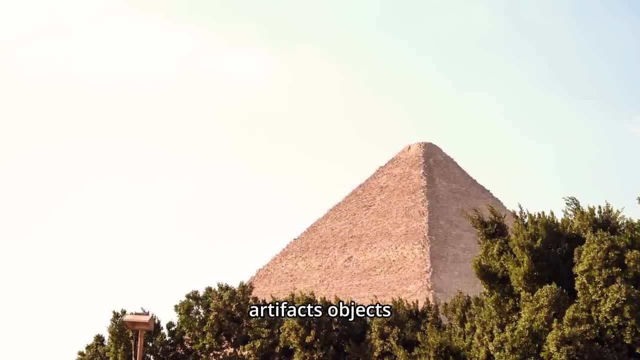 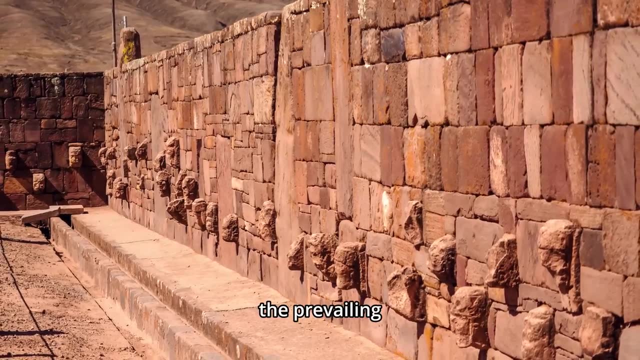 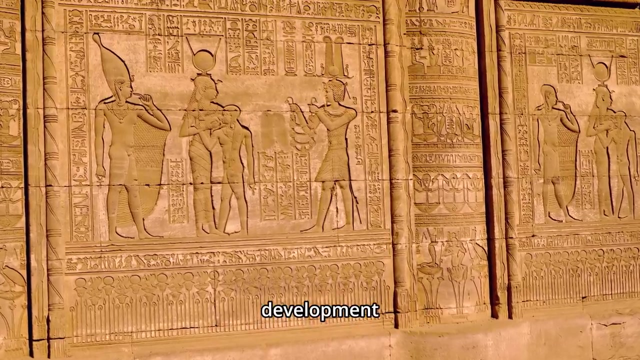 He specialized in the study of out-of-place artifacts, objects that appear to challenge conventional timelines and narratives. In this field, the prevailing notion is that as you dig deeper into the Earth's history, you should uncover progressively more primitive artifacts if humanity's development followed a linear path. 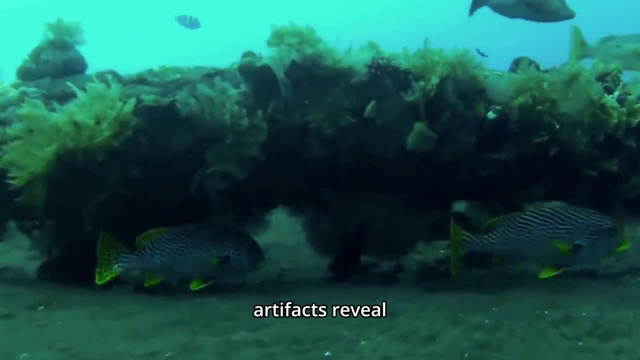 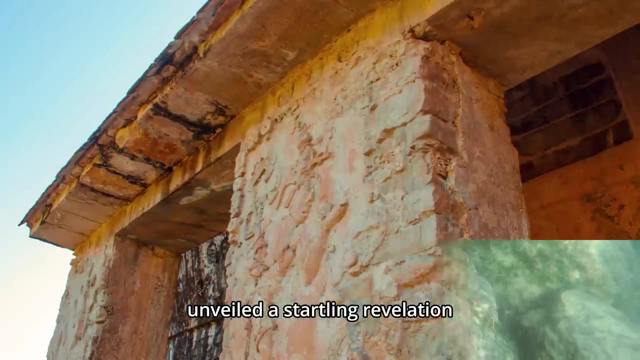 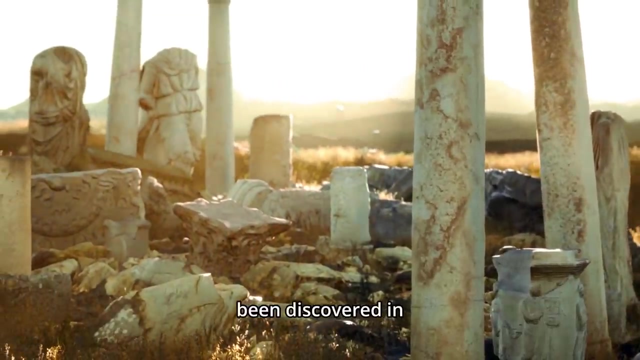 Yet, as explorations of out-of-place artifacts reveal, reality doesn't always conform to this expectation. Steiger's investigations unveiled a startling revelation: Advanced human artifacts, far from fitting neatly into the expected narrative, have been discovered in Earth's most ancient geological layers. 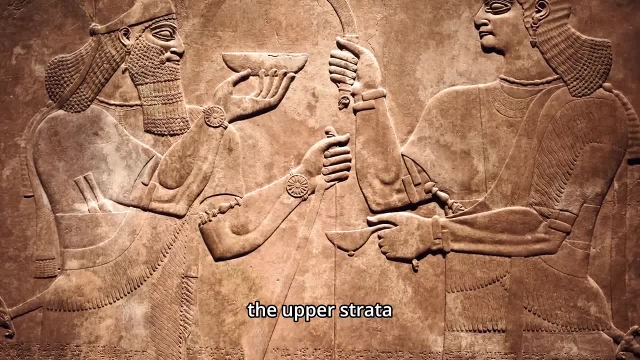 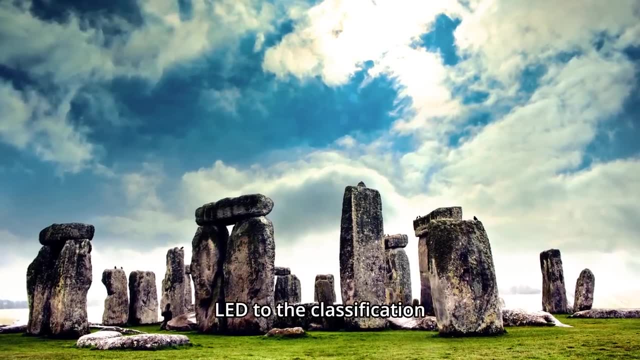 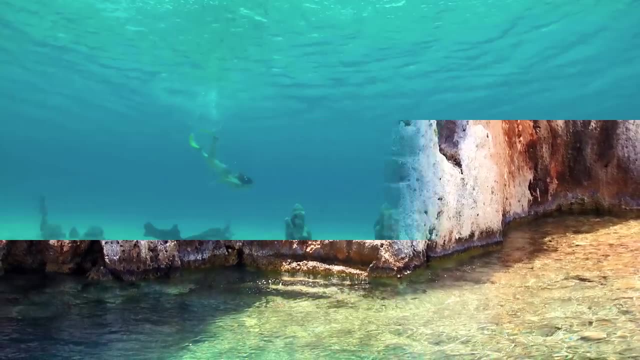 In a remarkable twist, primitive artifacts have appeared in the upper strata, defying conventional placement. This enigmatic contradiction to established scientific norms led to the classification of these anomalies as out-of-place artifacts, challenging our understanding of human history. In the present day, these emerging ideas and the mounting evidence are challenging the prevailing narrative of ancient civilizations. 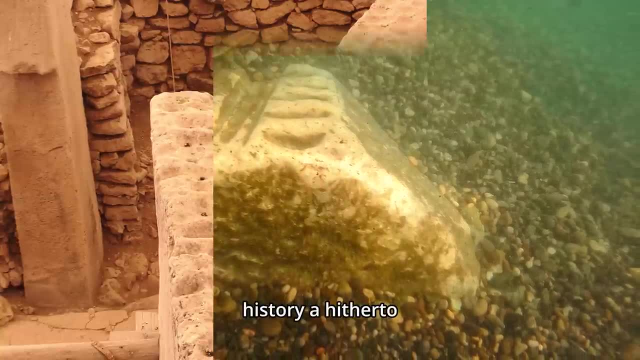 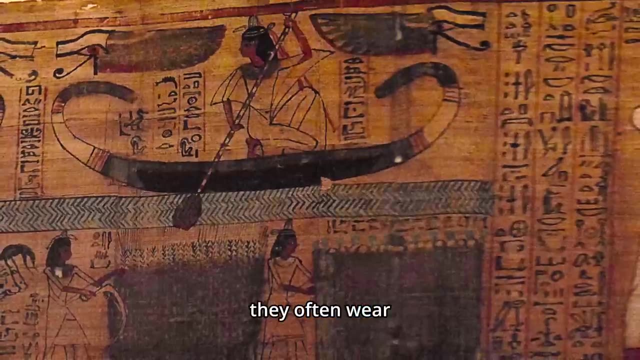 It's akin to a forgotten chapter in our history, a hitherto unsung epic. While fragments of this epoch still linger in the annals of myth and folklore, they often wear the mask of magic and otherworldly abilities, veiling the profound truths of this forgotten era. 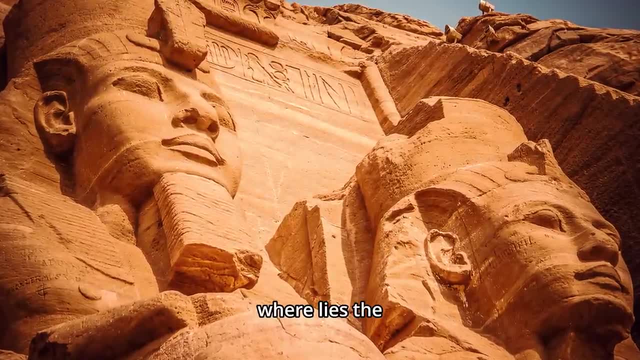 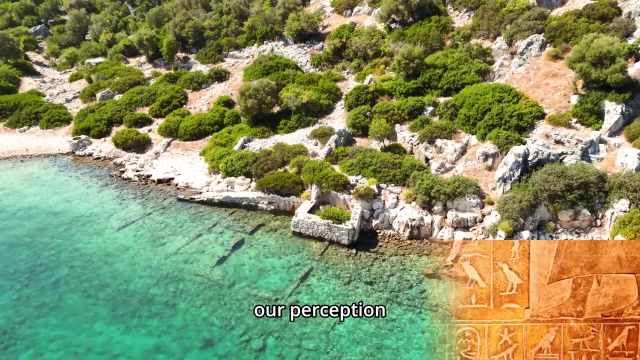 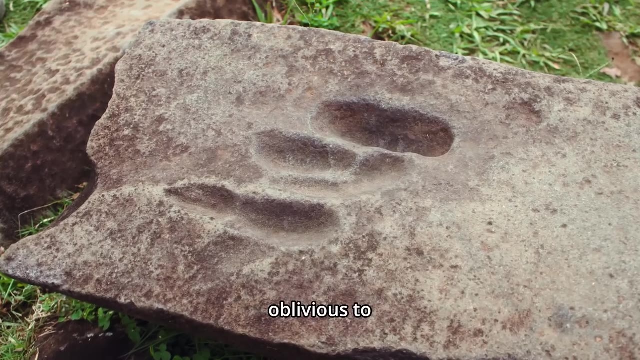 Now arises the pivotal inquiry: Where lies the tangible proof substantiating the hypothesis of ancient, sophisticated civilizations? Our perception and interpretation of facts could be a crucial factor here. The evidence may be right before us, yet we remain oblivious to its existence. Moreover, the search for such evidence has been hindered by our limited perspective. 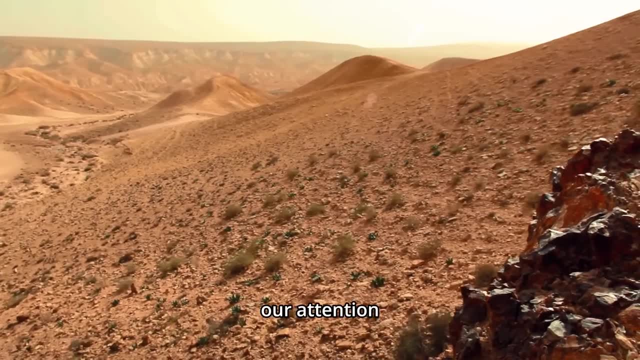 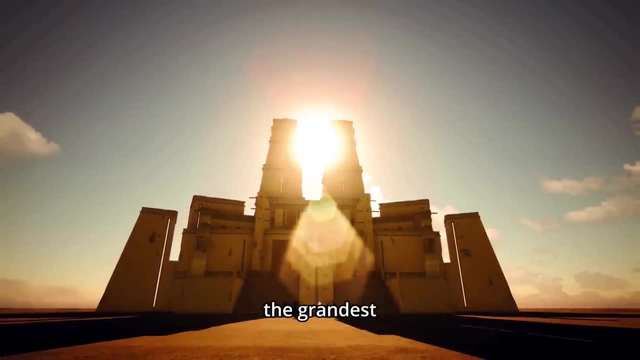 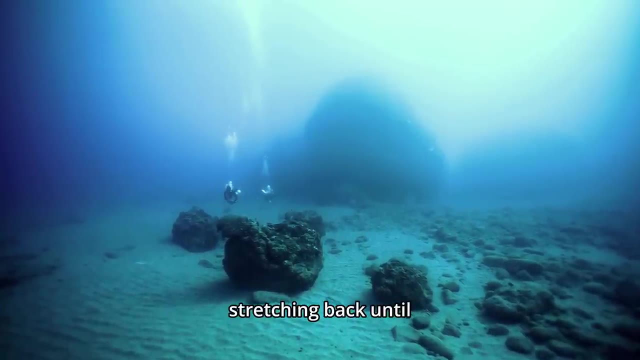 Still, there are intriguing hints and clues that beckon our attention, suggesting that a more profound investigation is in order. Why not begin by recognizing that the grandest human-made structures on Earth may be far more ancient than convention suggests, For millennia stretching back until the completion of the Empire State Building in 1931,? 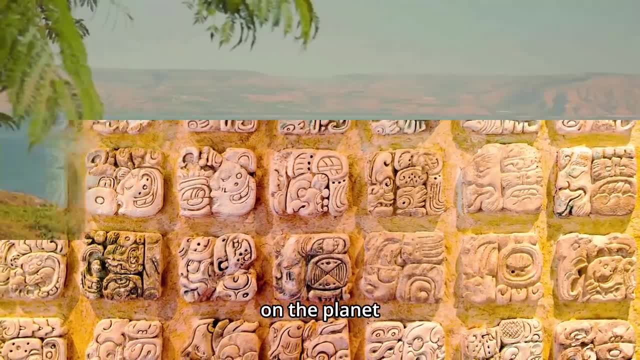 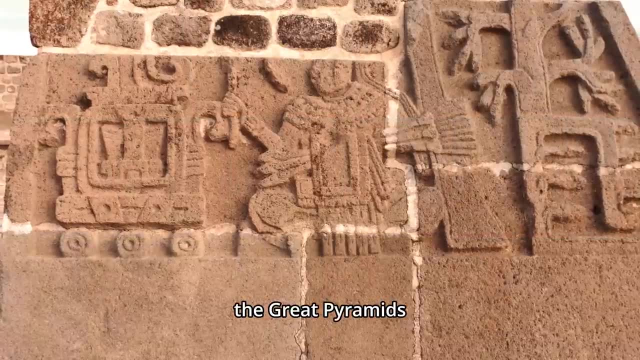 the Great Pyramid stood as the tallest structure on the planet, retaining its title as the most colossal, singular edifice ever raised on our planet. Yet the Great Pyramid's enigma is not confined to this. It is confined to architecture and engineering alone. 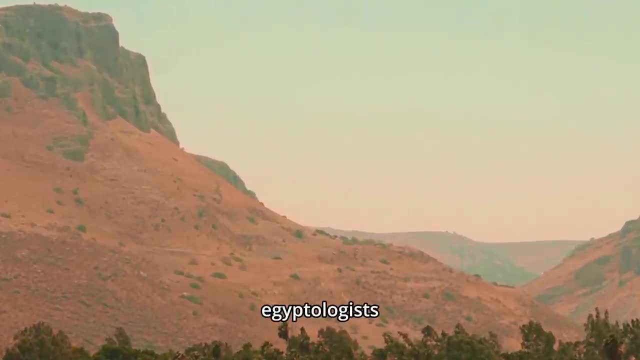 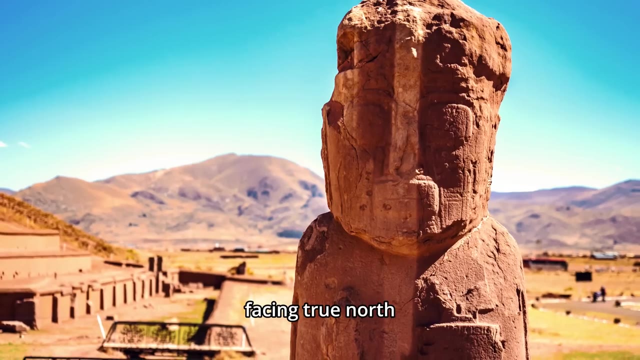 Its mysteries extend to the realm of geography. Egyptologists affirm that the Great Pyramid boasts the most impeccable alignment of any structure on Earth, directly facing true north, with a mere three-sixtieths of a degree of deviation. The North Pole's position shifts with the ages. 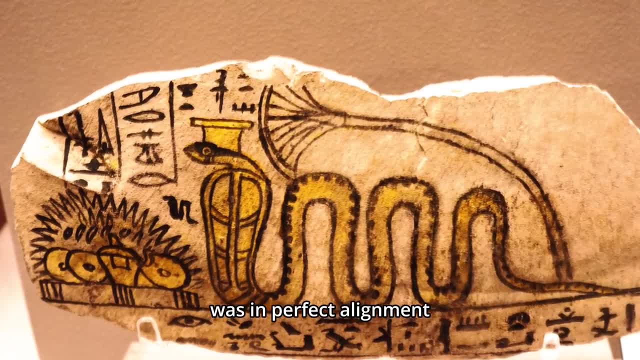 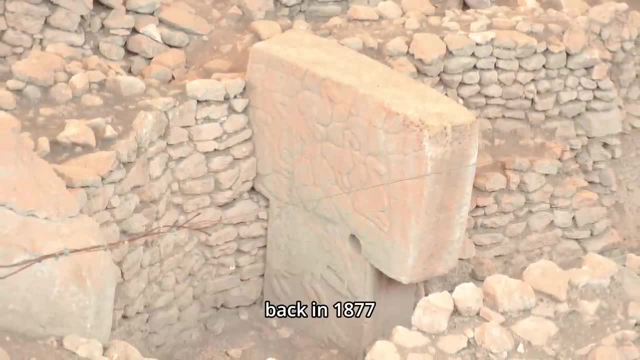 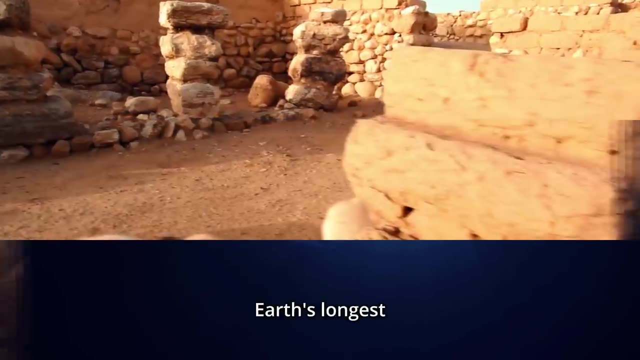 and there was a specific juncture when the pyramid was in perfect alignment with this ever-moving point. Intriguingly, Dr Joseph Seyss, a theologian and author, back in 1877, presented an astonishing revelation. The Great Pyramid of Giza stands at the exact intersection of Earth's longest line of longitude and the longest line of latitude. 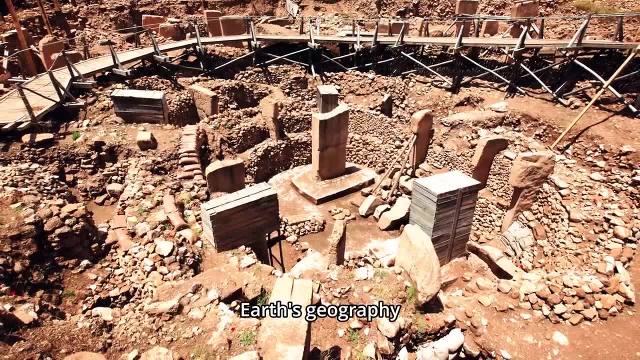 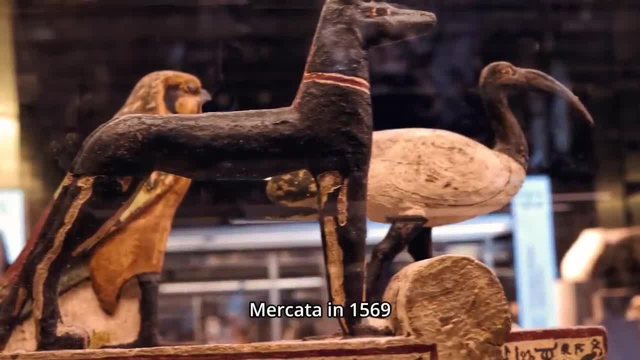 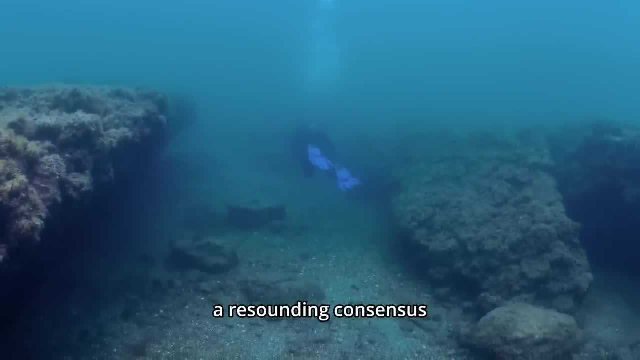 This remarkable precision implies an intimate understanding of Earth's geography, akin to the sophisticated Mercator projection, a groundbreaking map projection developed by Gerardus Mercator in 1569.. Furthermore, contemporary engineers and scientists have reached a resounding consensus: Replicating the Great Pyramid using our most advanced technology remains an insurmountable challenge. 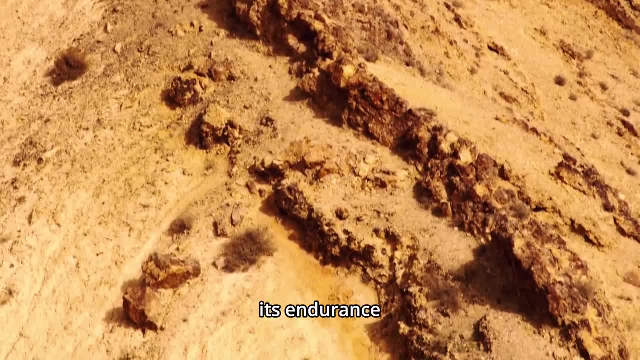 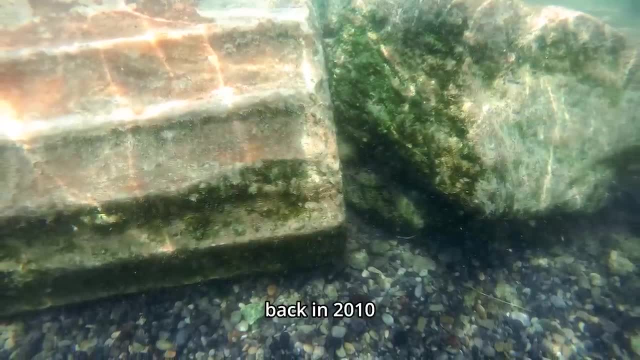 To recreate this architectural marvel and ensure its endurance for millennia would pose an overwhelming structural conundrum, one that modern engineering can hardly resolve. Back in 2010,, engineer Marcus Schulte ventured to speculate that the endeavor, if at all possible, 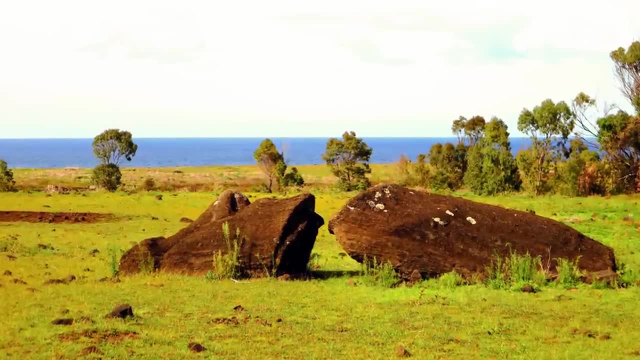 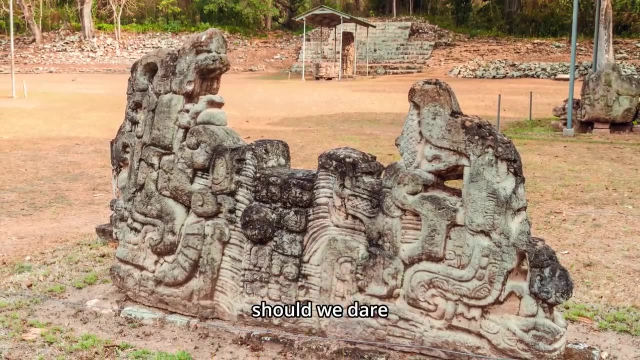 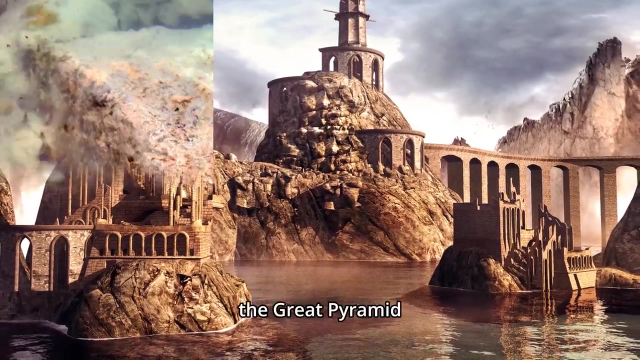 would come at a staggering cost of $35 billion. Fast forward to today and this colossal undertaking would likely demand a budget closer to $50 billion, should we dare to embark on such an awe-inspiring journey, Contemplating the enormous financial investment needed to replicate the Great Pyramid? 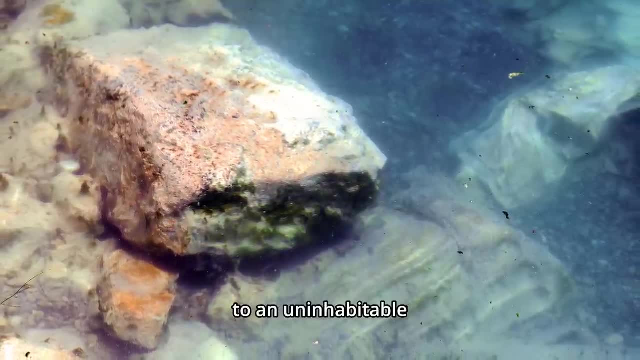 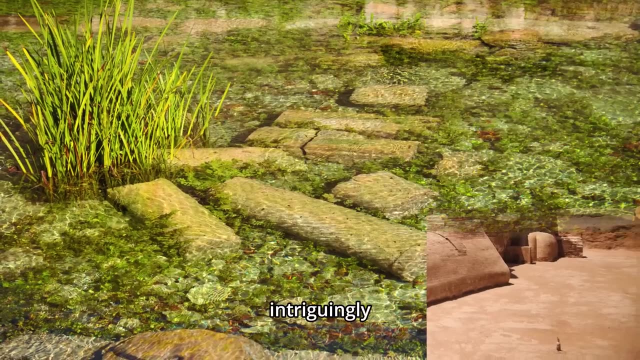 it becomes evident that dedicating such colossal sums to an uninhabitable structure devoid of expected profit would be an unfathomable decision by today's standards. Intriguingly, when we delve into the remarkably detailed record-keeping of ancient Egyptian life, 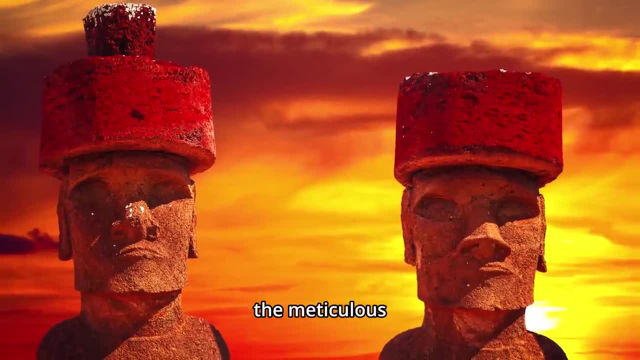 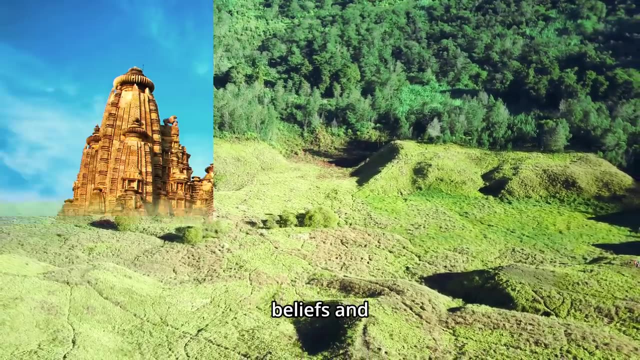 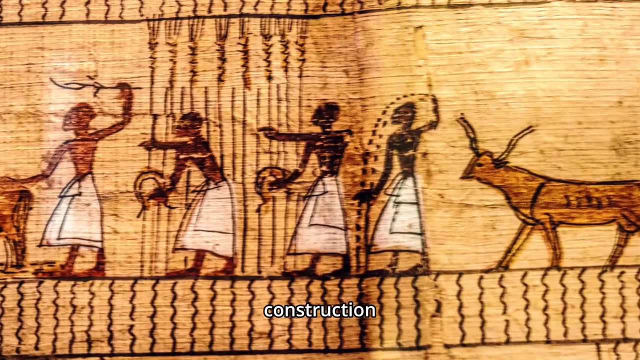 we encounter an enigmatic silence. The meticulous hieroglyphic records chronicle even the minutiae of daily existence, providing insights into their society, beliefs and activities. However, curiously absent from this rich tapestry of history is any mention of the construction of the Giza Necropolis. 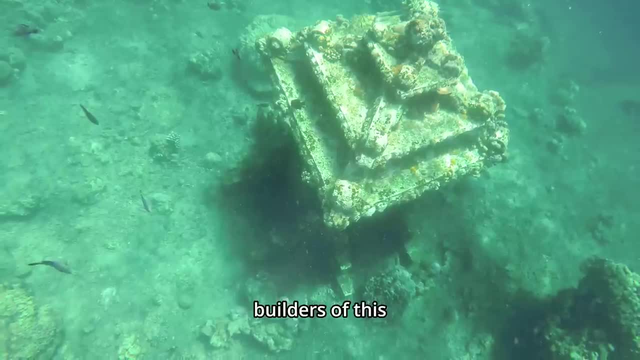 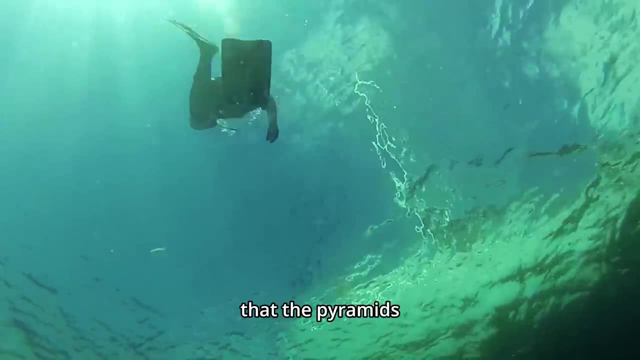 It raises questions about the true architects and builders of this awe-inspiring wonder. Intriguing clues lead us to contemplate an even more profound possibility: that the pyramids might predate the ancient legends of the Great Flood, When the Great Pyramid was first unveiled to modern eyes. 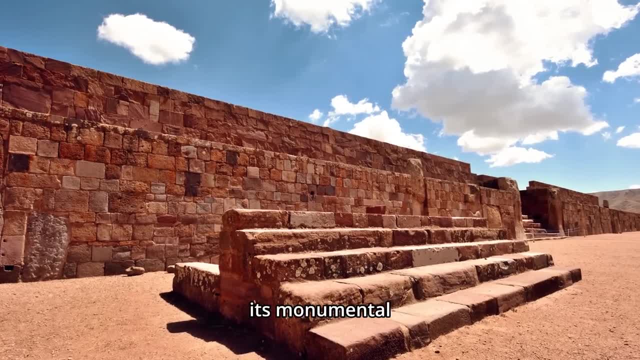 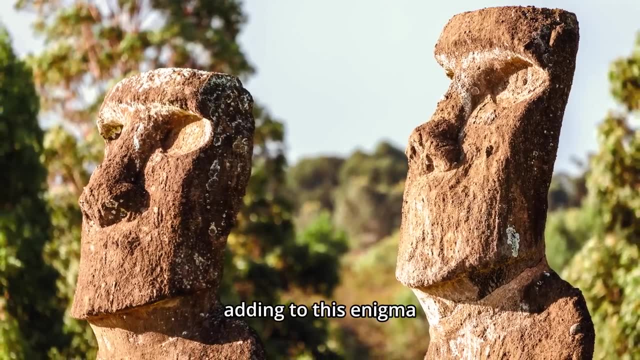 explorers made a startling discovery: Hidden within its monumental chambers were incrustations of natural salt suggesting a connection to a watery past. Adding to this enigma, in the 1750s Captain Frederick Norton, a renowned naval explorer. 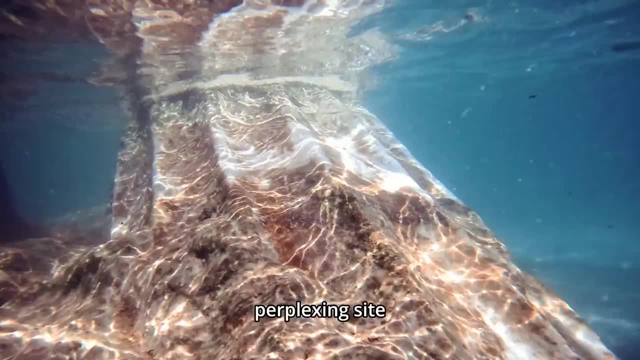 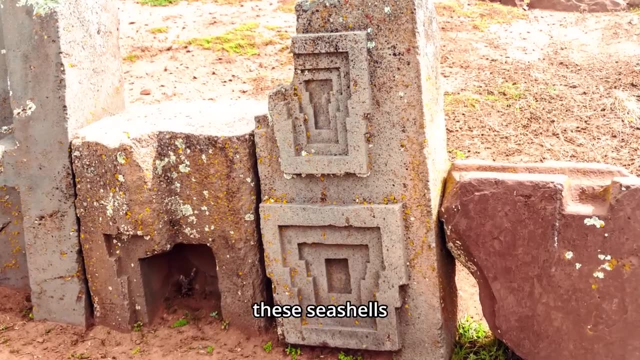 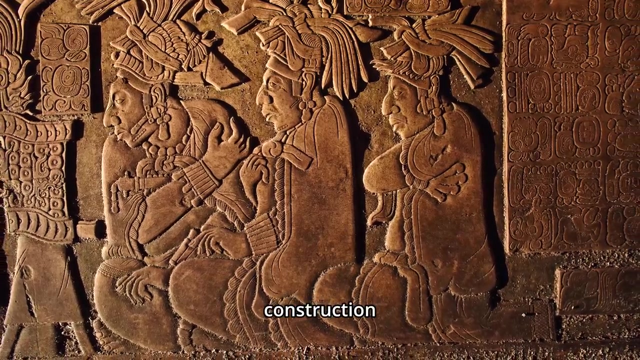 ventured to the Giza Plateau and reported a perplexing sight. He documented the presence of a significant number of seashells strewn across the plateau. These seashells, far from their natural aquatic habitat, cast a shadow of doubt on the conventional timeline of the pyramids' construction. The ancient historian Herodotus in his enduring work Histories echoed the puzzling presence of seashells and indications of saltwater deposits around the pyramid complex. These remarkable observations add to the mounting evidence that the Giza Plateau might have once been submerged beneath the waters. 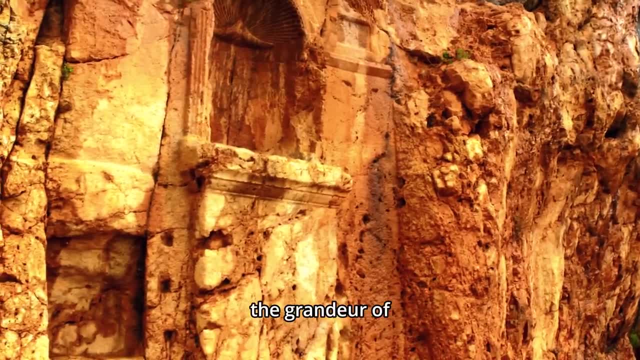 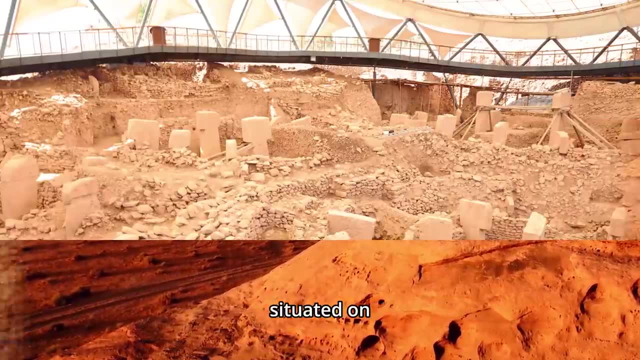 Moreover, the inability of the Egyptians to replicate the grandeur of the pyramids on even a smaller scale becomes evident when one examines the trio of structures known as the Queen's Pyramids, situated on the north side of the Great Pyramid. This stark contrast between the majestic Great Pyramid and its smaller counterparts. 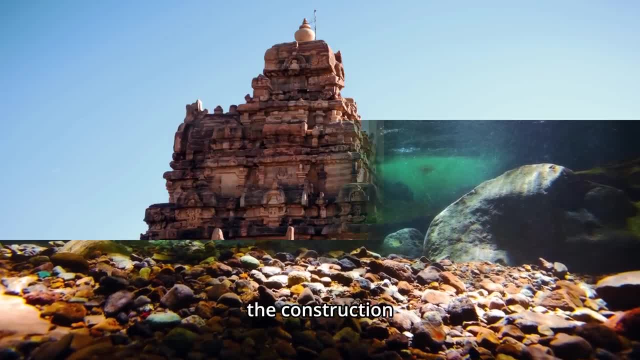 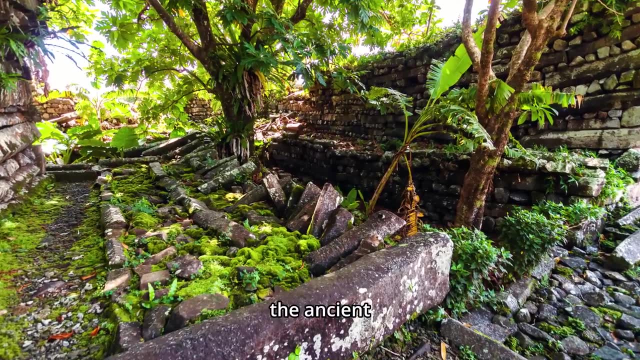 raises questions about the true origins and techniques behind the construction of these ancient marvels Contemplating the grandeur of the pyramids. one can't help but wonder if the ancient Egyptians, in their reverence for these monumental structures, founded their entire civilization in the shadow of the Giza Plateau. 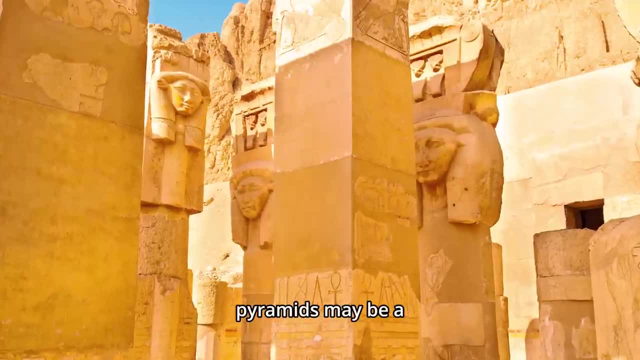 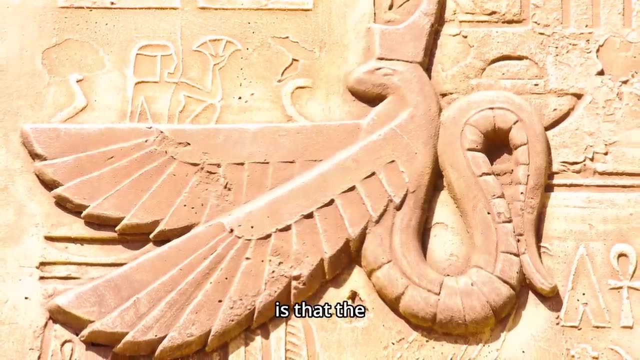 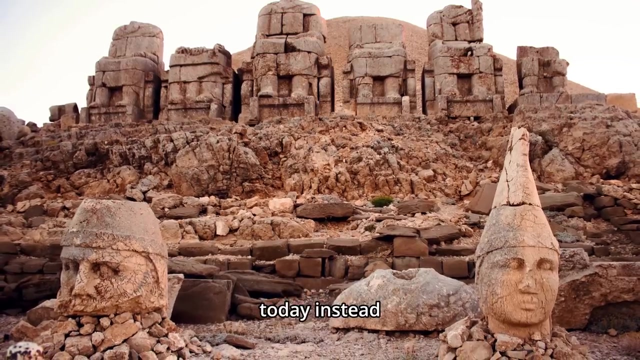 A fascinating theory posits that the three pyramids may be a terrestrial homage to the trio of stars in Orion's belt. What makes this theory even more intriguing is that the alignment of the pyramids doesn't precisely match the positions of the stars. Instead, they seem to correspond to the celestial arrangement of 12,000 years ago. 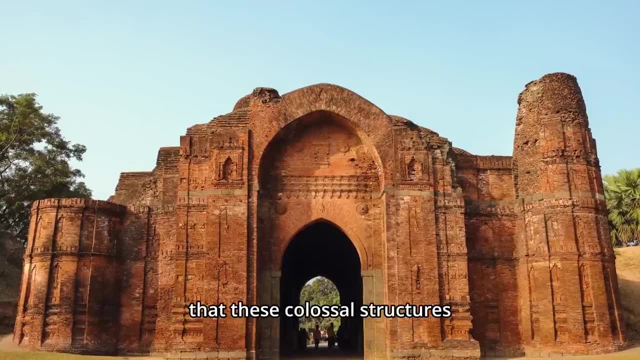 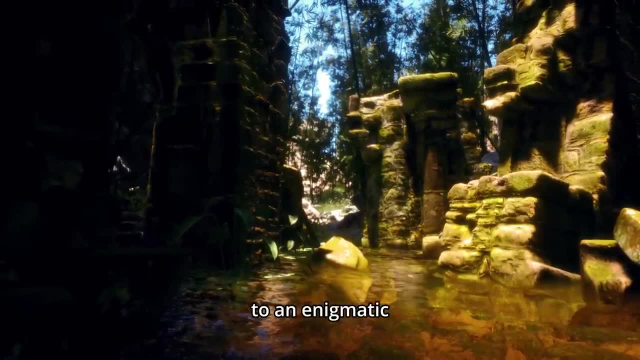 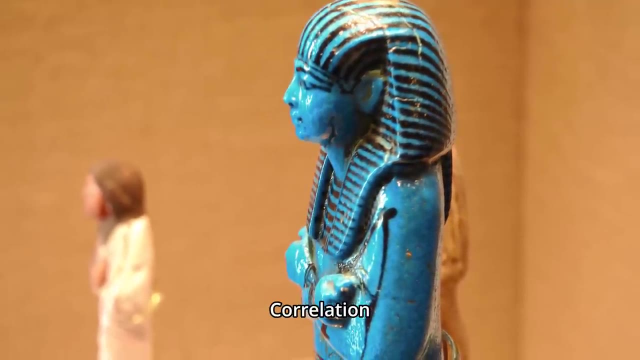 This astonishing hypothesis implies that these colossal structures could have been constructed nearly 8,000 years before the dawn of traditional Egyptian culture, opening a portal to an enigmatic epoch when the world's history was written in the shadows of the pyramids. Accepting the validity of the Orion Correlation Theory raises profound questions. 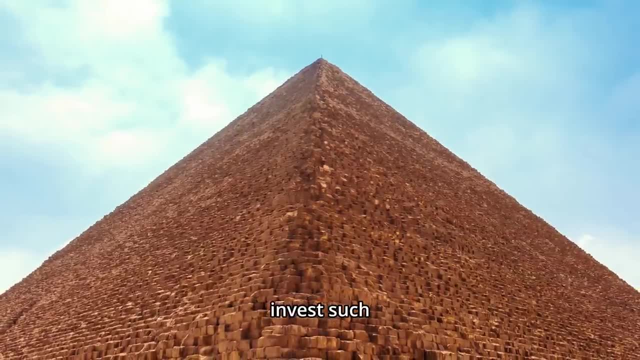 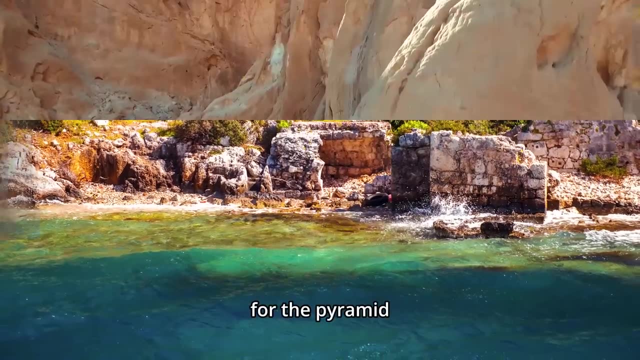 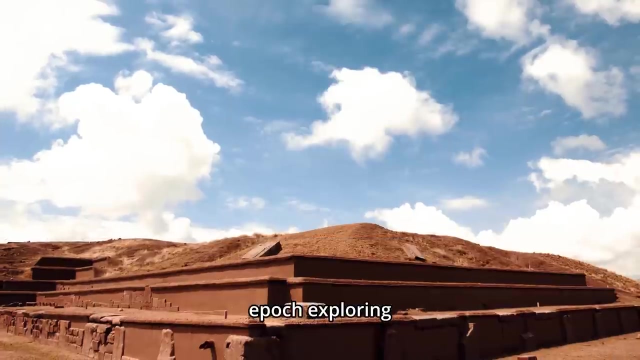 Why did these enigmatic architects invest such immense effort in erecting these colossal monuments? Does this specific date hold extraordinary significance for the pyramid builders? What momentous events or celestial phenomena were unfolding during this mysterious epoch? Exploring these questions takes us on a captivating journey into the shadows of history. 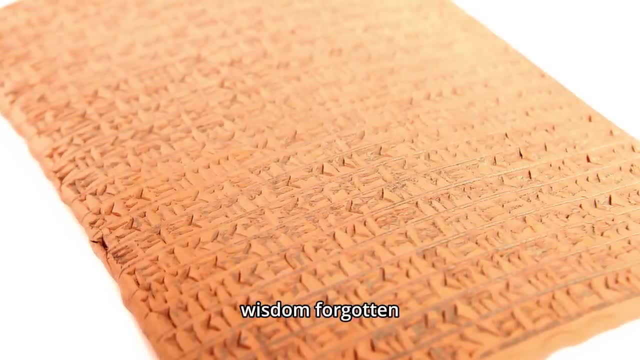 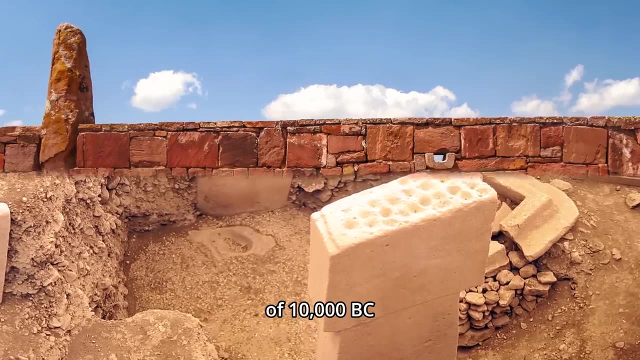 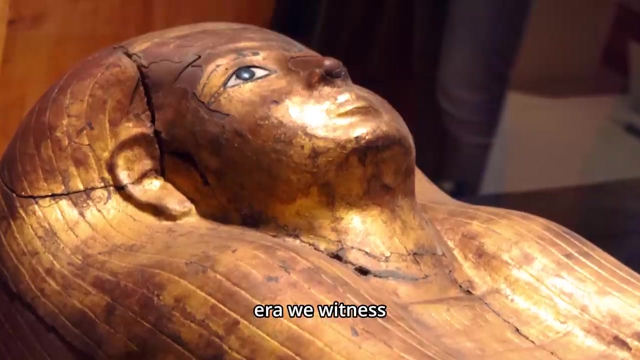 where the secrets of the pyramids may unveil ancient wisdom, forgotten civilizations and a profound connection between Earth and the cosmos. The significance of 10,000 BC looms large as it coincides with the termination of the late Ice Age. During this era, we witness the dawn of human settlements. 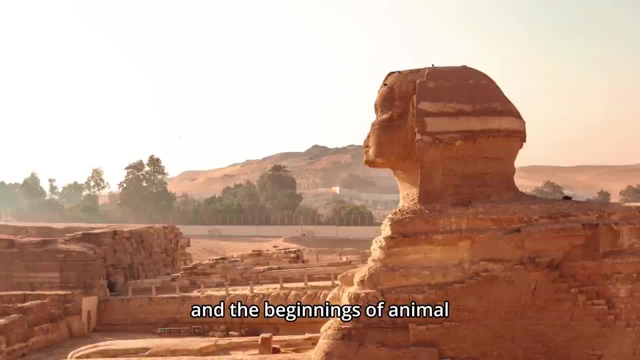 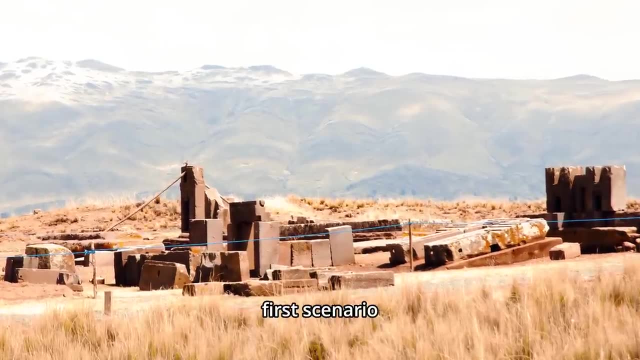 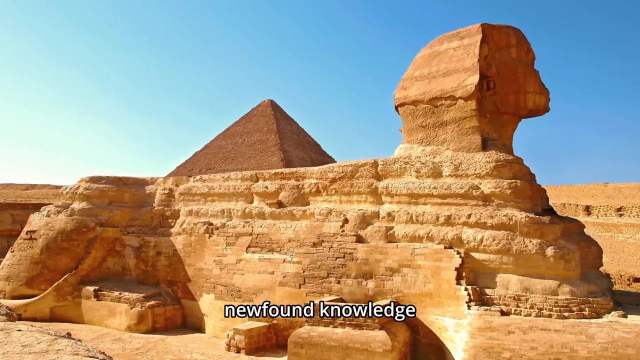 the emergence of wooden structures and the beginnings of animal domestication. These rapid advancements leave room for two compelling scenarios. The first scenario suggests that humanity reached a pivotal juncture in their enduring evolutionary journey, propelling them forward with newfound knowledge and capabilities. 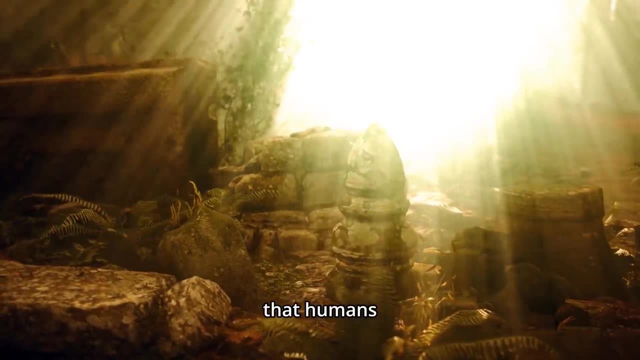 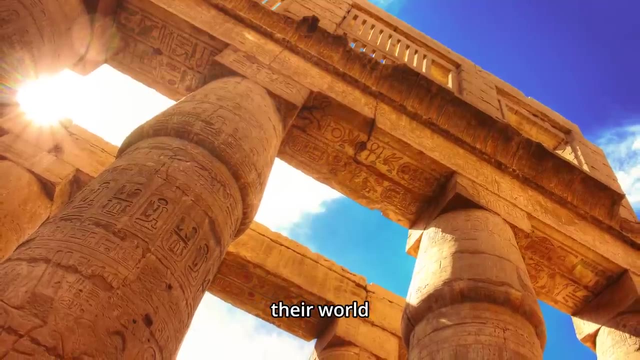 In contrast, the second scenario hints at the possibility that humans were in the process of recovery from a global cataclysmic event, their resilient spirit guiding them as they rebuilt and reinvented their world. 10,000 BC stands as a critical juncture in our shared history. 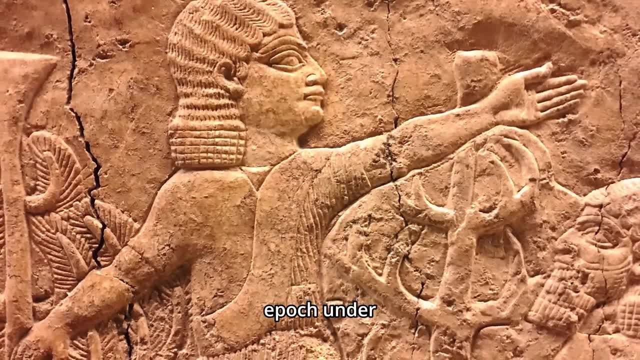 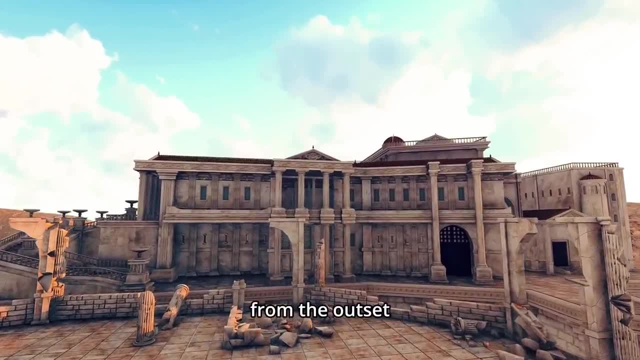 inviting us to explore the mysteries of this transformative epoch. Under the veil of the lesser-known theory envisioning survivors of a cataclysm, it becomes clear that establishing cities from the outset would be an improbable feat. In such a scenario, these resilient survivors would disperse across the globe. 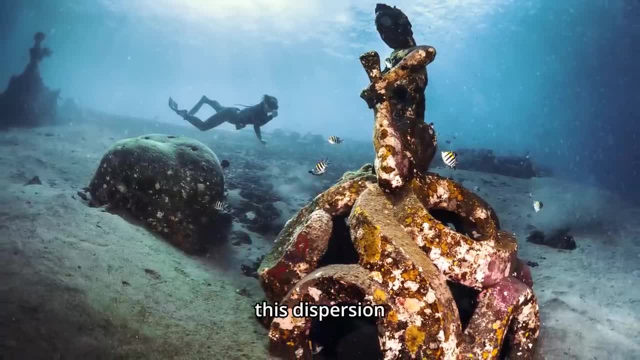 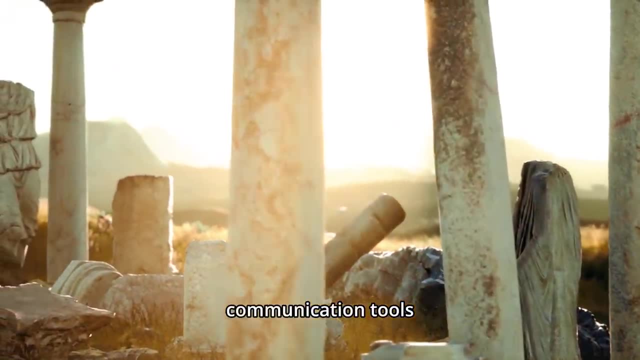 each group venturing into different territories. This dispersion would inevitably give rise to linguistic deviations. In the absence of advanced communication tools, maintaining contact with one another would prove an insurmountable challenge. The ancient world still untamed by interconnectedness. 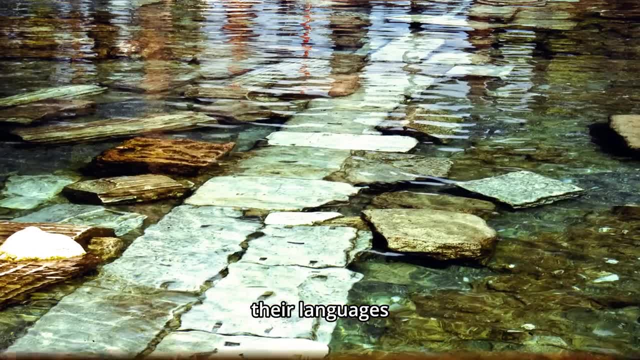 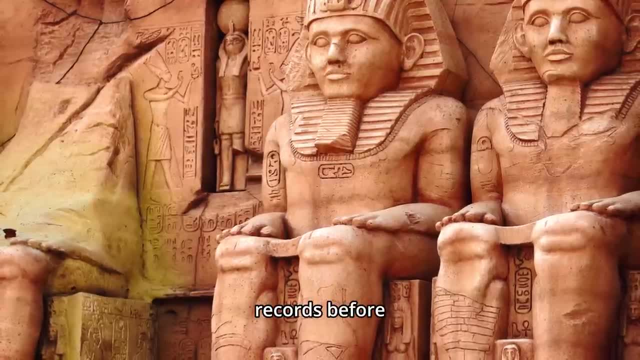 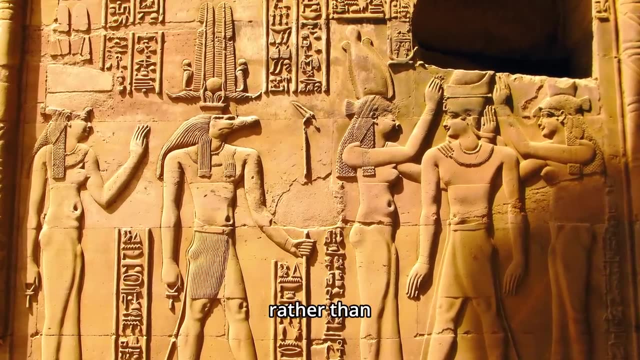 would be marked by isolated pockets of survivors, their languages diverging with each passing generation. This theory could help elucidate the absence of historical records before the emergence of the city of Uruk, around 4500 BC, In this alternative narrative, rather than a continuous trajectory of progress. 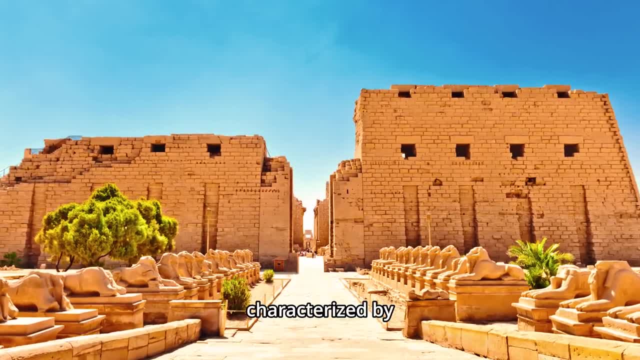 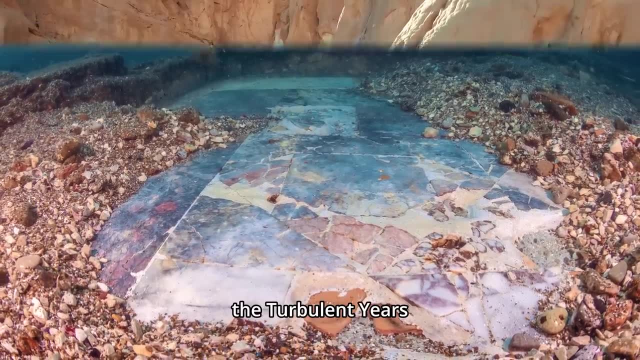 humanity might have endured a prolonged period of stagnation characterized by rudimentary tools and a lack of innovation. Eric A von Fanger's book Noah to Abram, The Turbulent Years. New Light on Ice Age, Caveman, Stone Age, The Old Kingdoms. 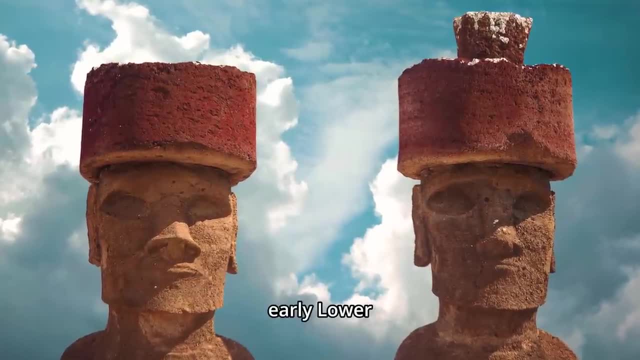 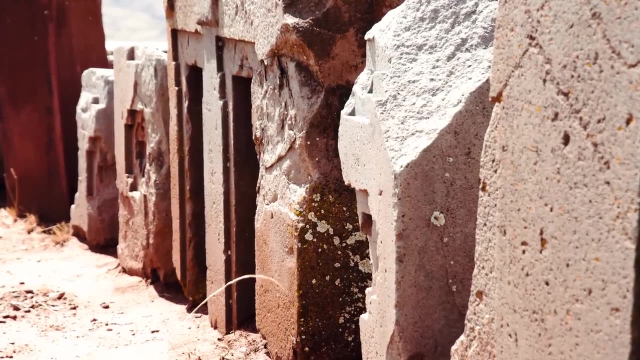 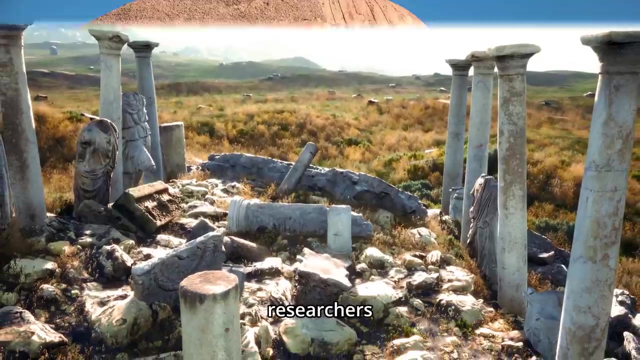 sheds light on intriguing parallels between what we know of early Lower Paleolithic cultures and a post-cataclysmic society striving to rebuild upon the remnants of their forebears. As the body of evidence continues to expand, the idea of a cataclysmic past is gaining broader acceptance among researchers and scholars. 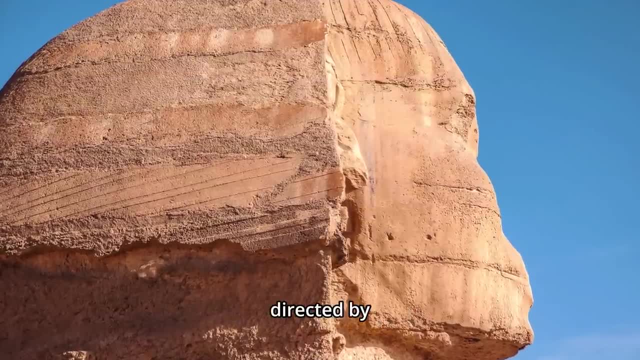 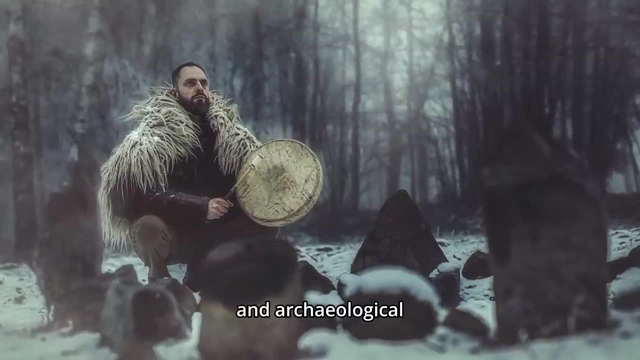 The movie 10,000 BC, directed by Roland Emmerich, embraced the cataclysmic scenario, a choice that drew criticism from academic and archaeological communities, who found it historically and archaeologically inaccurate. Returning to the enigma of the pyramids, 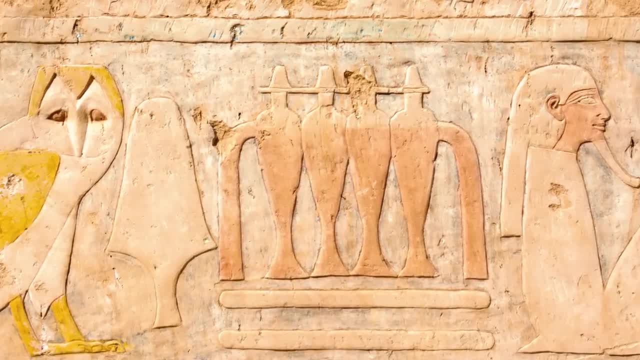 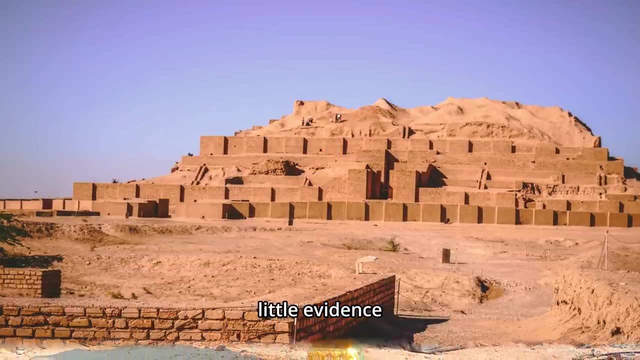 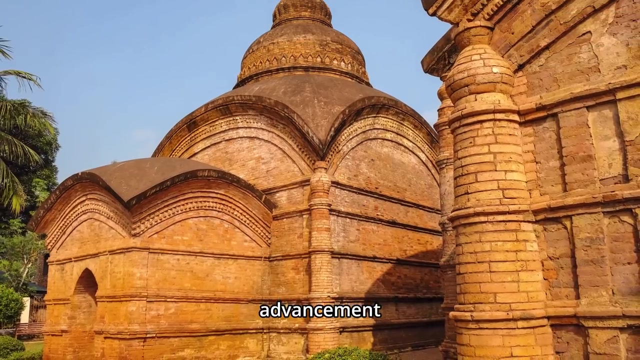 their construction might indeed signify an earlier global catastrophe. Shortly after 10,000 BC, there is a remarkable emergence of various cultures worldwide with little evidence of preceding developmental stages, raising intriguing questions about the catalyst for this simultaneous advancement. These early societies made an astonishing transition from hunter-gatherers. 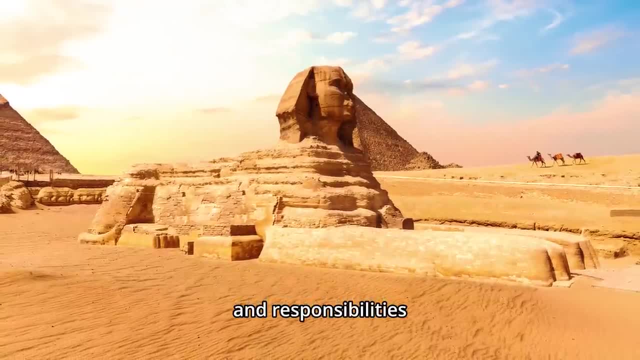 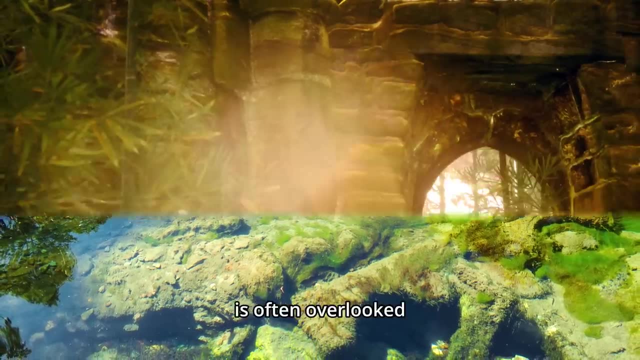 to fully-fledged citizens with rights and responsibilities. The Egyptian civilization in particular holds the key to unraveling this enigma, though its significance is often overlooked due to its challenge to mainstream theories, As John Anthony West eloquently put it. 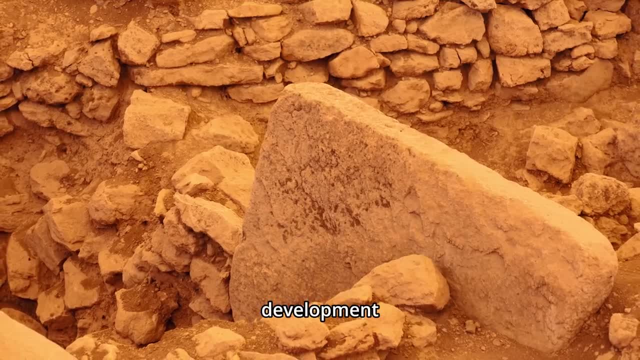 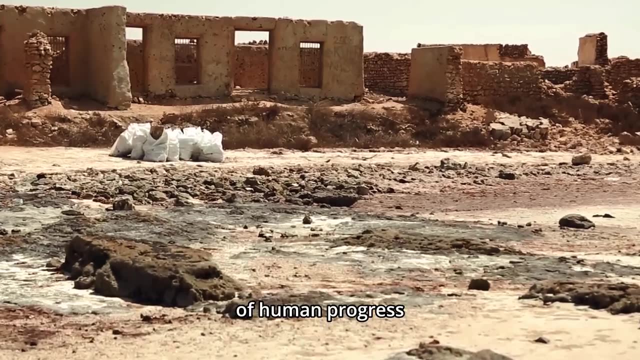 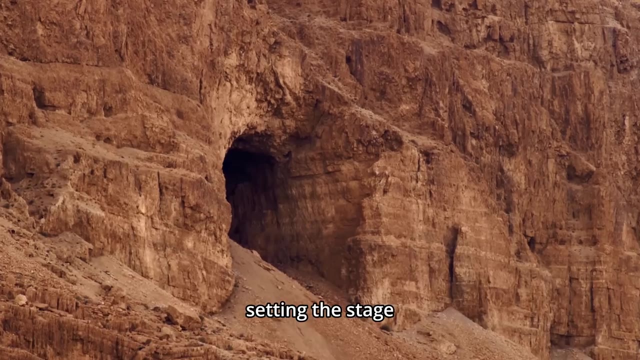 the origins of Egyptian civilization were not a mere development, but rather a profound legacy, a realization that urges us to reconsider the conventional understanding of human progress. The rapid emergence of cities was likely accompanied by a deep understanding of intricate social structures, setting the stage for advanced civilizations. 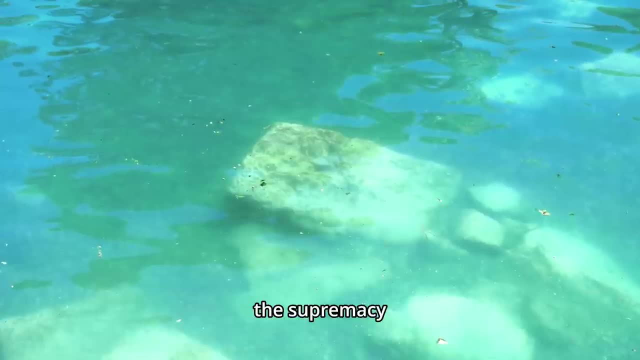 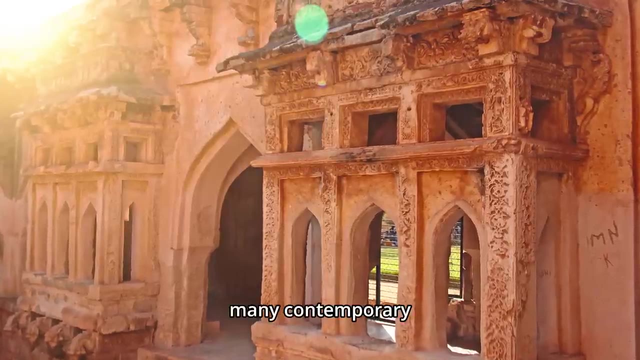 Moreover, the age-old debate over the supremacy of ancient Egypt versus ancient Greece remains an intriguing puzzle, Notably Herodotus, and many contemporary historians have pondered this incongruity with Solon's accounts, adding to the historical tapestry. 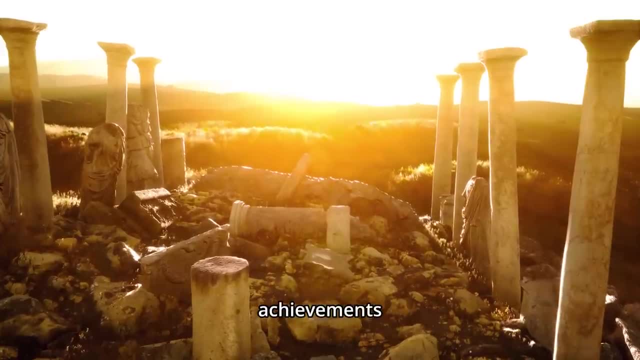 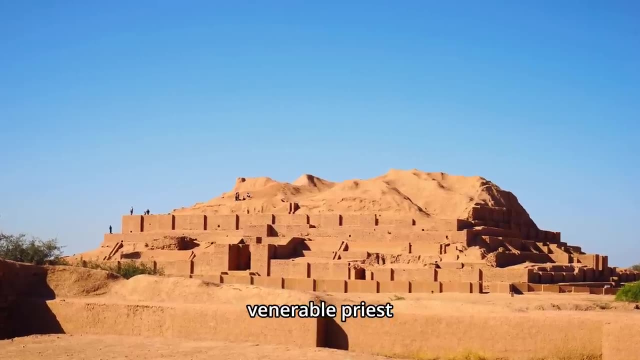 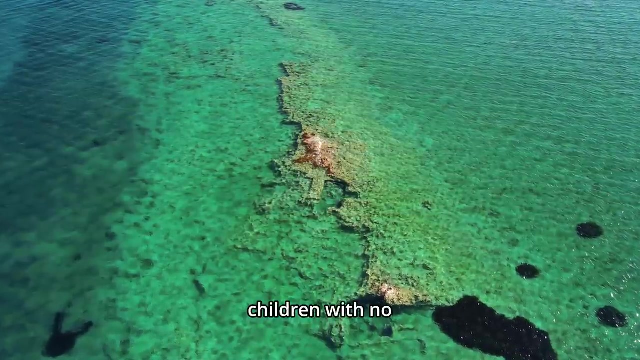 underscoring the need to reevaluate the disparities in their respective achievements. In the ancient city of Sais Solon, the wise Athenian statesman conversed with a venerable priest who offered a profound observation: O Solon Solon, you, Hellenes, remain perpetual children with no elders among you. 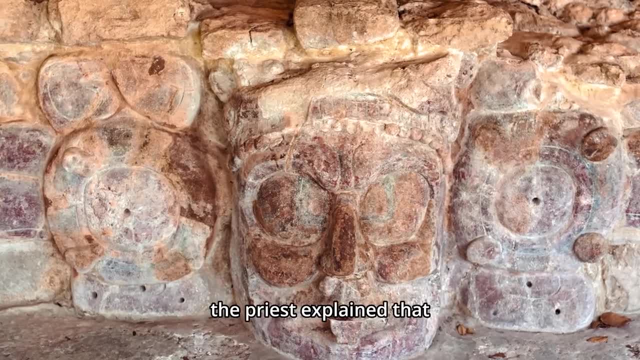 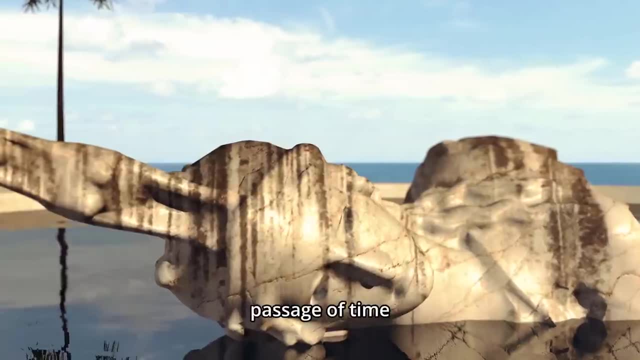 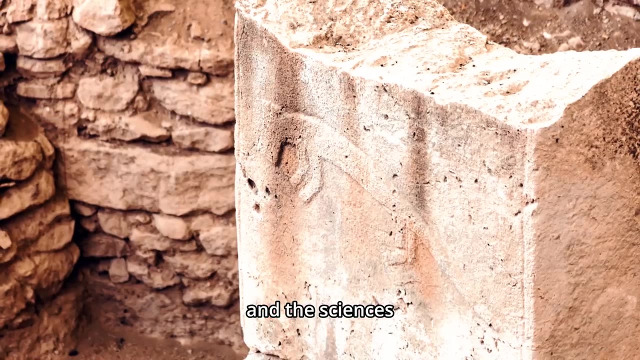 Solon, intrigued. inquired further, The priest explained that the Hellenic minds were youthful, bereft of the ancient wisdom and enduring knowledge that could only be born from the passage of time. He elaborated: Your people lack old beliefs handed down through generations, and the sciences among you are not marked by the wisdom of age. 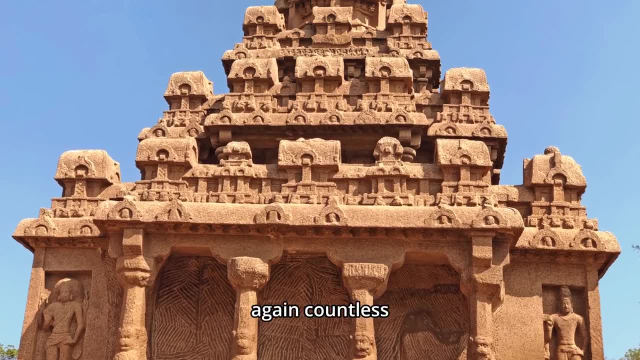 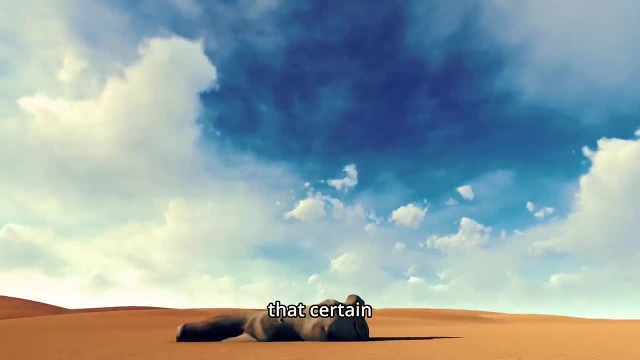 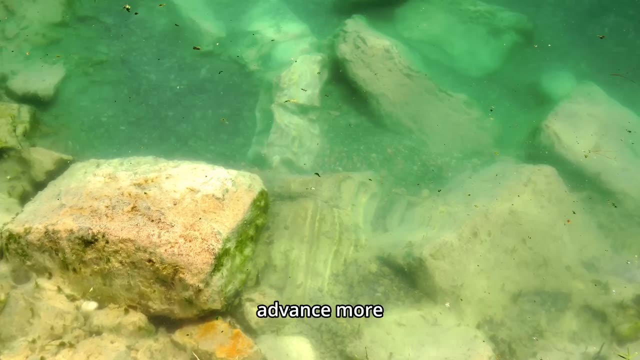 There is a reason for this, For there have been, and will be again, countless episodes of humanity's decline, brought about by myriad causes. It is plausible that certain survivors retained precious knowledge inherited from those enigmatic first people, enabling them to thrive and advance more rapidly than others. 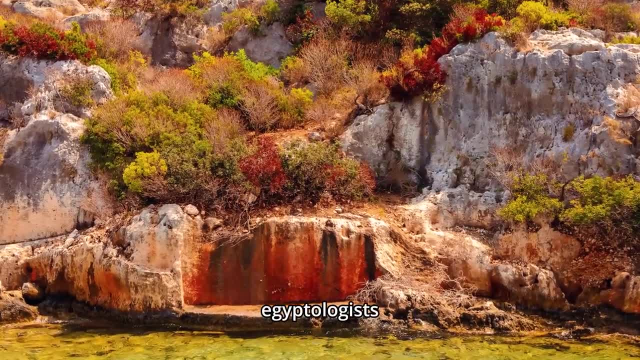 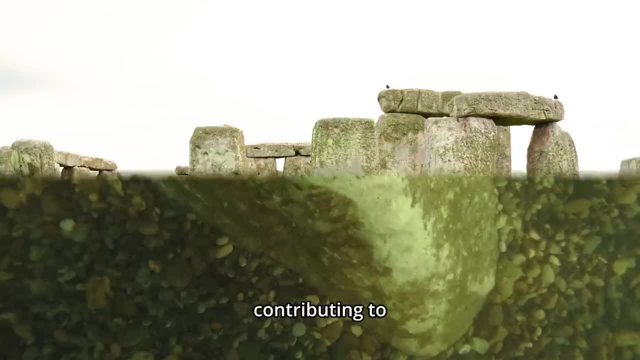 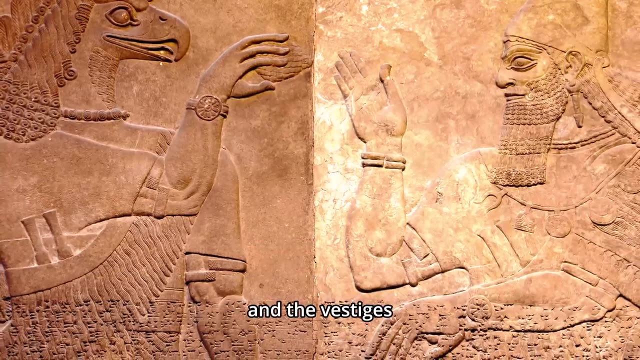 Consider, for instance, the findings of Egyptologists who suggest that the high priests of ancient Egypt held a reservoir of profound esoteric wisdom credited with contributing to the flourishing of the Egyptian civilization. These first people possessed advanced sciences, and the vestiges of their knowledge may well persist to this day, concealed within the intricate tapestry of human history. 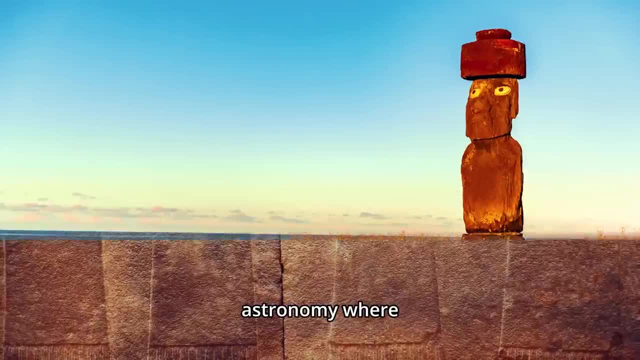 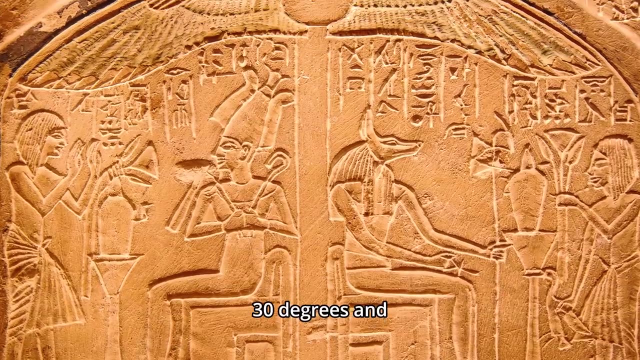 Consider, for instance, the field of astronomy, where the concept of artificially dividing celestial longitude zones into twelve zodiac constellations, each spanning thirty degrees, and the profound understanding of cosmic precession appear to trace their origins back to a more advanced culture. 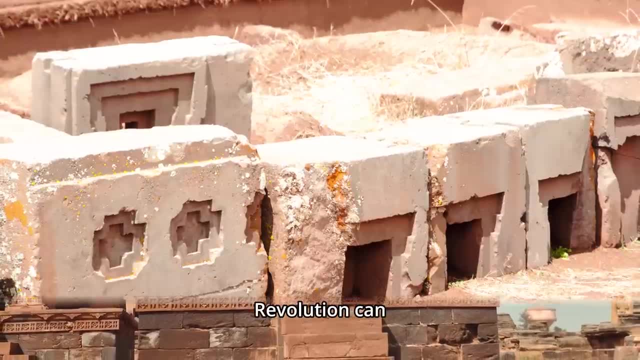 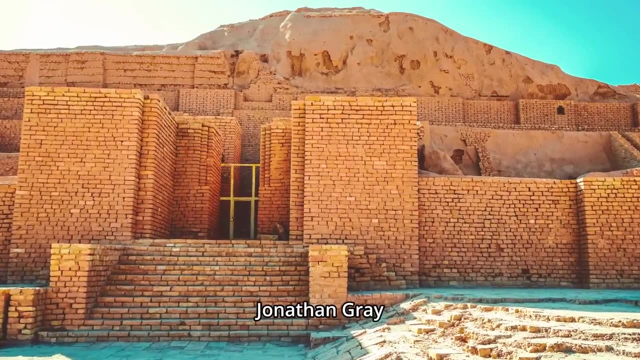 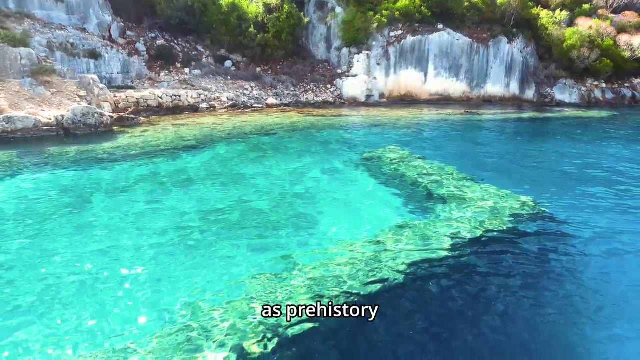 In this context, the Copernican Revolution can be viewed as a rekindling of ancient wisdom that had been lost to time and is now experiencing a renaissance. Jonathan Gray once articulated: against the backdrop of conventional history during that enigmatic era we refer to as prehistory: 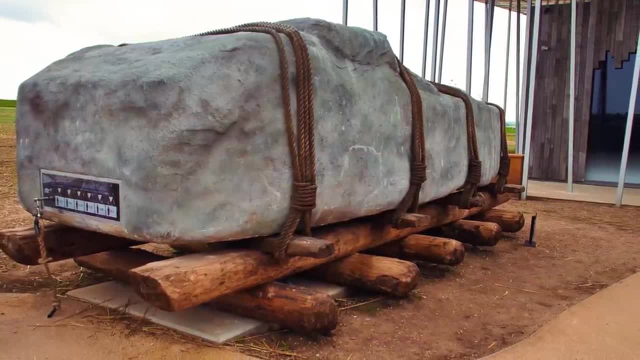 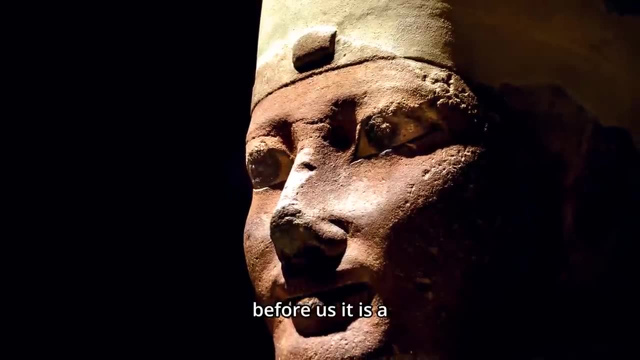 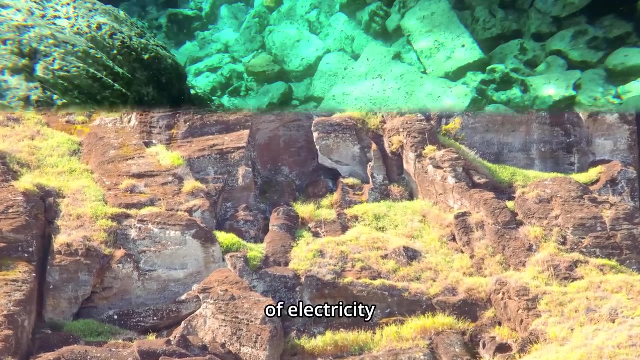 a profound reservoir of astronomical wisdom thrived. It beckons one to delve deeper, revealing that a civilization of intellectual titans likely walked the path before us. It is a proposition that carries compelling merit In the realm of physics, it is evident that a grasp of electricity was part of the prehistoric repository of wisdom. 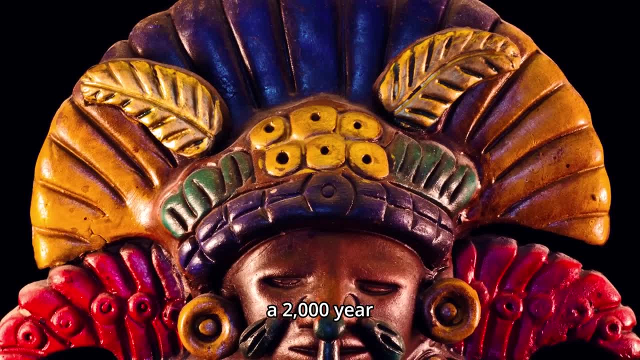 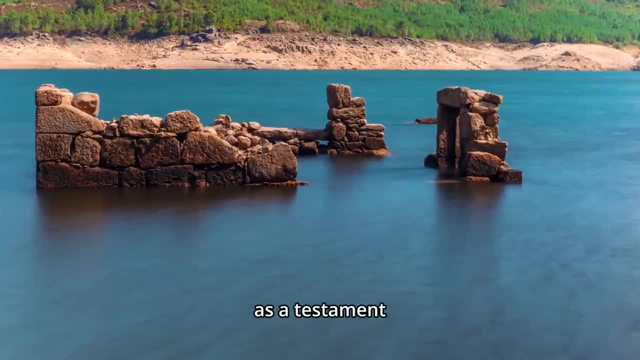 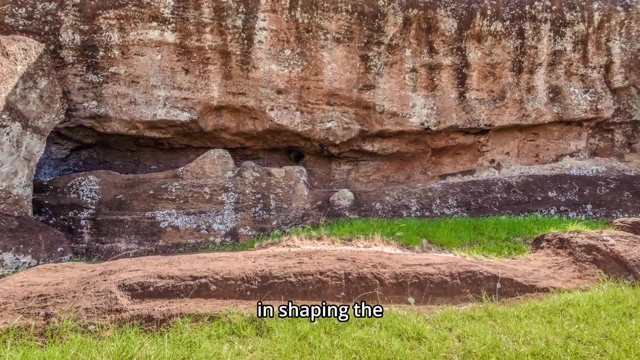 As previously discussed, the unearthing of a 2000-year-old battery by German scientist Wilhelm Koenig at the National Museum of Iraq in 1938 serves as a testament to this ancient knowledge. In the sphere of geography, it becomes clear that ancient maps played a pivotal role in shaping the age of maritime exploration. 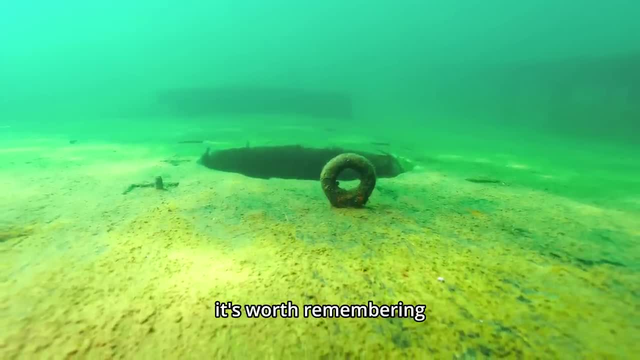 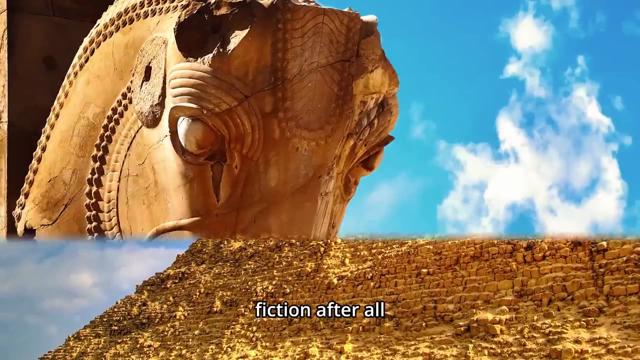 So, as we contemplate these enigmas, it's worth remembering the words of Tom Clancy: the distinction between fiction and reality. Fiction, after all, must adhere to logic and coherence. Indeed, the facts presented in this narrative may appear puzzling. 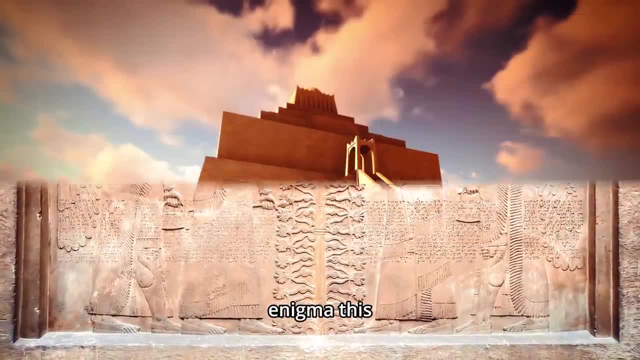 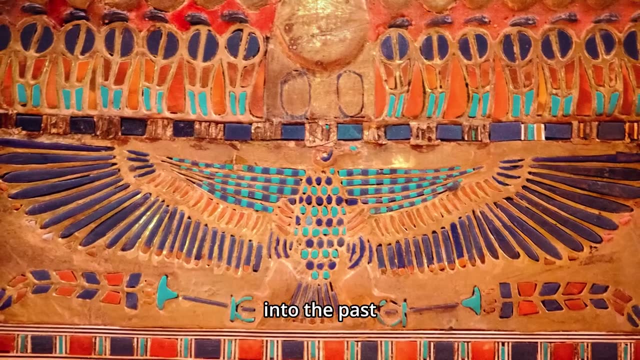 but that's the essence of mysteries: they challenge us to unravel the enigma. This video doesn't aim to provide an exhaustive historical account, but rather serves as an enticement to delve deeper into the past. Understanding our history holds great significance and carries profound implications for our present and future. 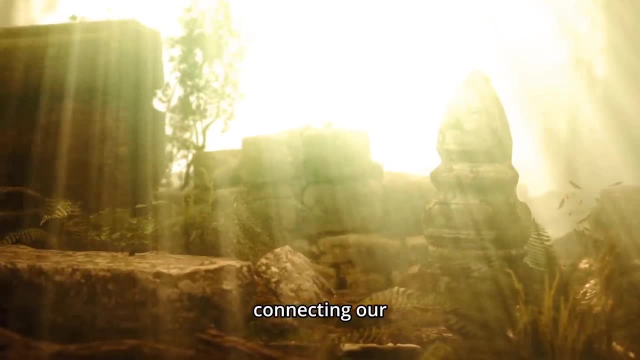 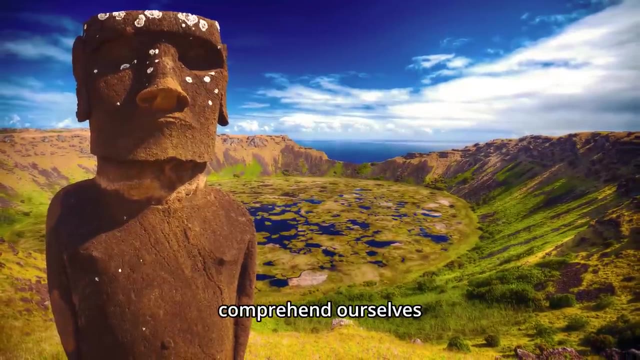 It's a continuum, a seamless thread connecting our past, present and the path to the future. The more we uncover about our history, the better we comprehend ourselves and the direction we're headed. The evidence is abundant, though not everyone acknowledges it. 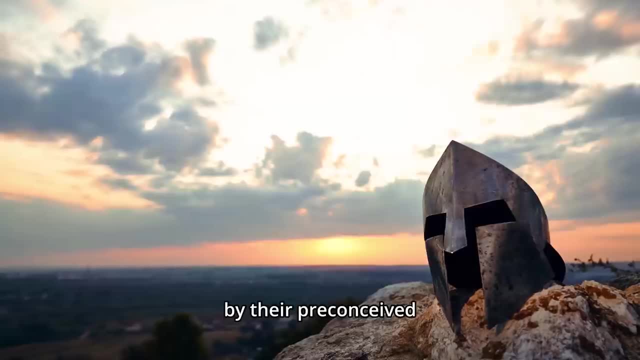 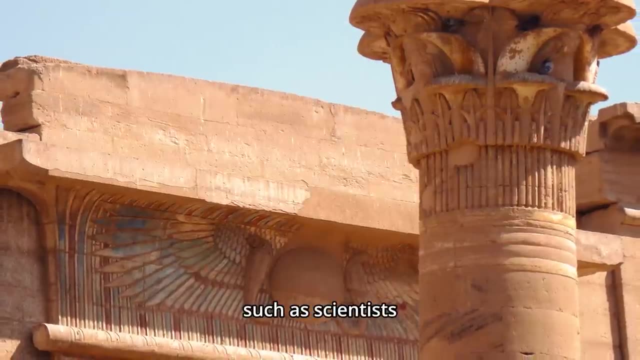 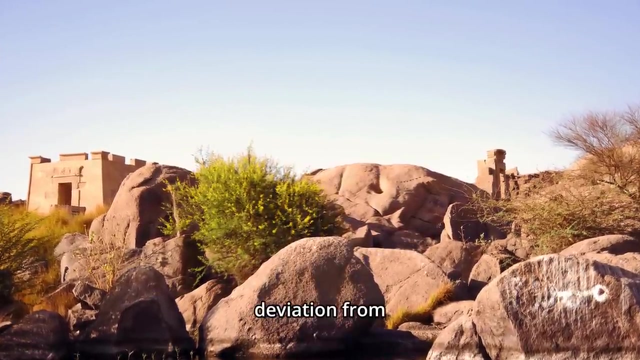 How individuals respond to anomalies is often shaped by their preconceived notions about history. These reactions can also be influenced by prevailing modern philosophies such as scientism, presentism and practices like obscurantism. In the realm of science, any deviation from the norm could be the spark of a groundbreaking discovery or a paradigm shift. 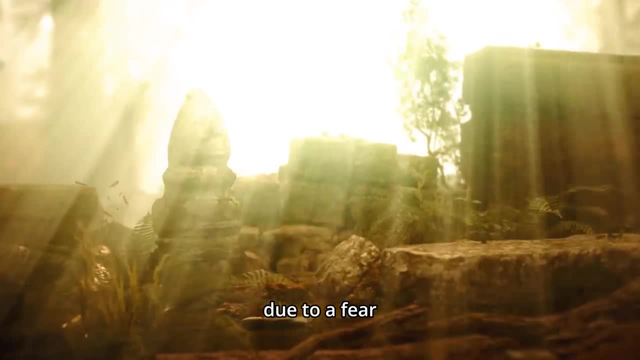 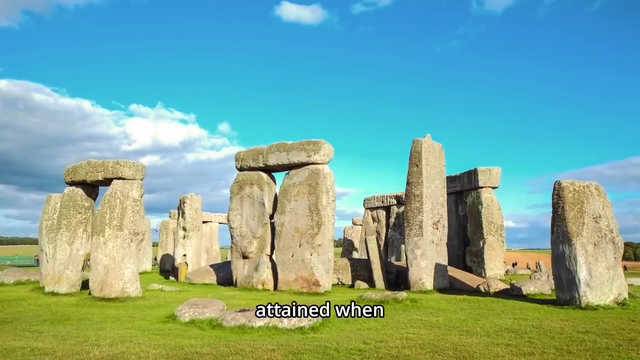 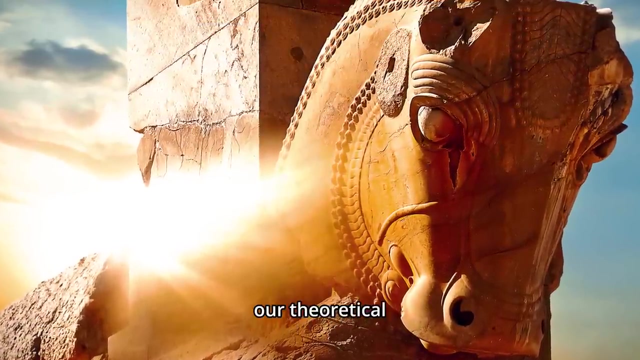 Yet it's sometimes brushed aside or disavowed due to a fear of change and an attachment to the status quo. Genuine scientific and intellectual progress can only be attained when we are open to exploring the anomalous. It's essential to adapt and, when necessary, reconfigure our theoretical foundations until what once seemed anomalous becomes the new norm. 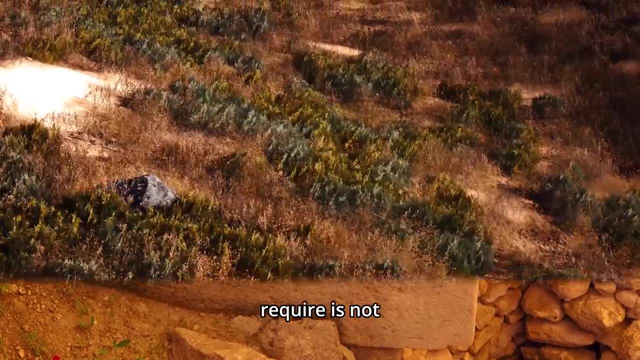 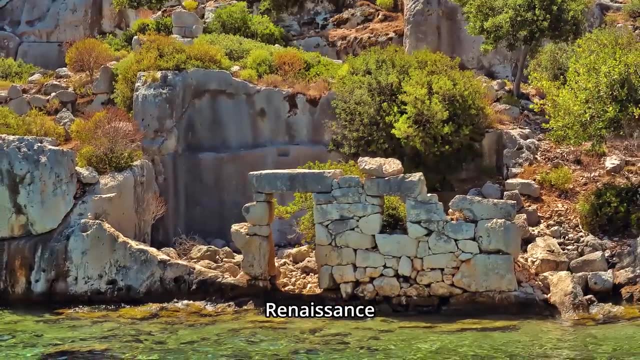 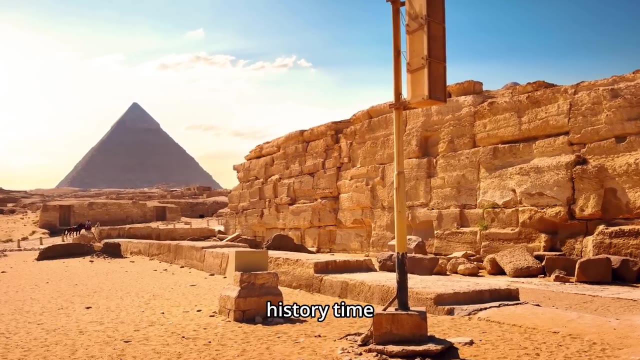 as described by Thomas Kuhn. What we truly require is not merely a shift in paradigms but, even more significantly, a reawakening of scientific thought, a true renaissance. Chapter 3: Civilizations have risen, reached their zenith and faded into the annals of history time and time again. 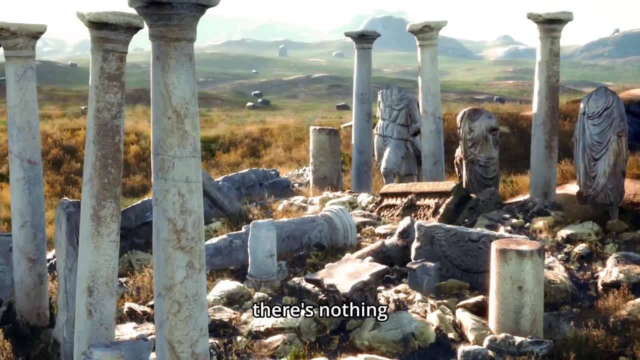 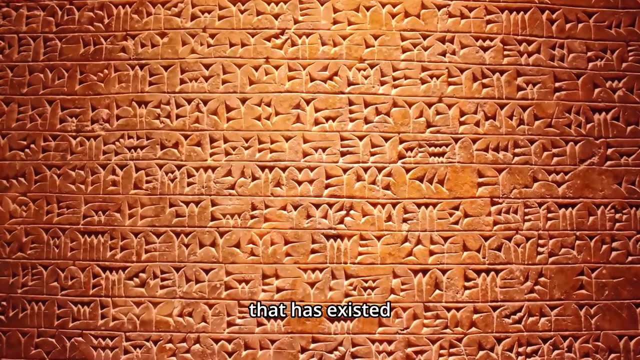 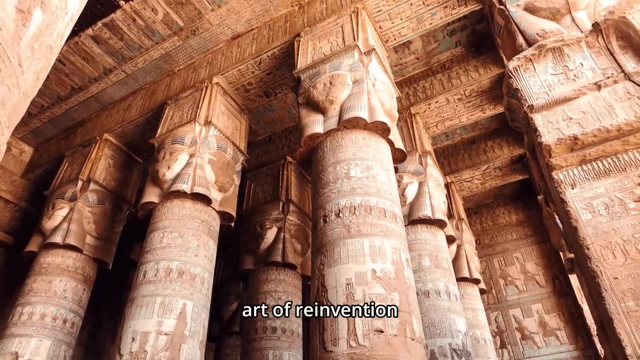 The past is an echo of the present and there's nothing entirely novel in the world. Every revelation we make is merely a reimagining or a renewed finding of something that has existed before, a reminder that history is cyclical and human innovation is, in essence, the art of reinvention and rediscovery. 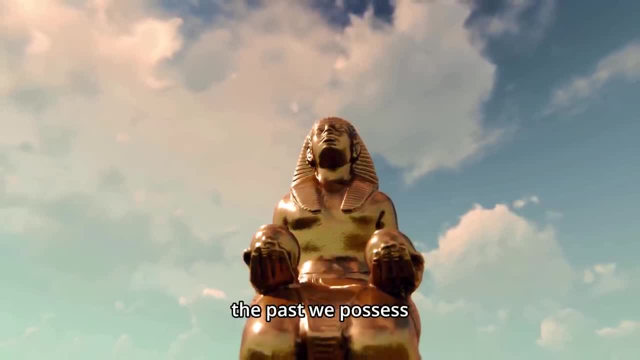 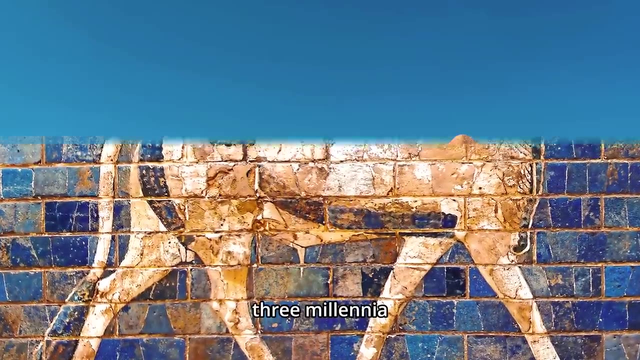 In our quest to unravel the mysteries of the past. we possess a relatively comprehensive understanding of the most recent two millennia, but when we cast our gaze back three millennia earlier, we are confronted with a historical narrative pieced together through imperfect archaeological reconstructions. 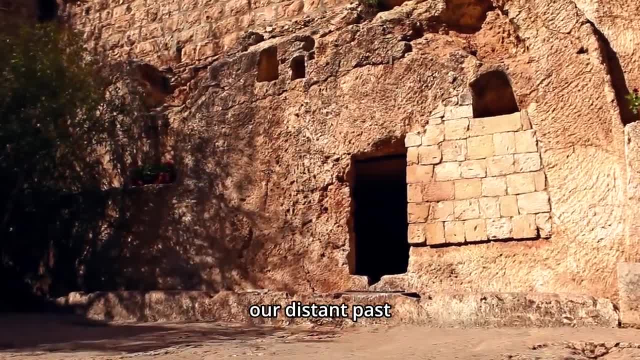 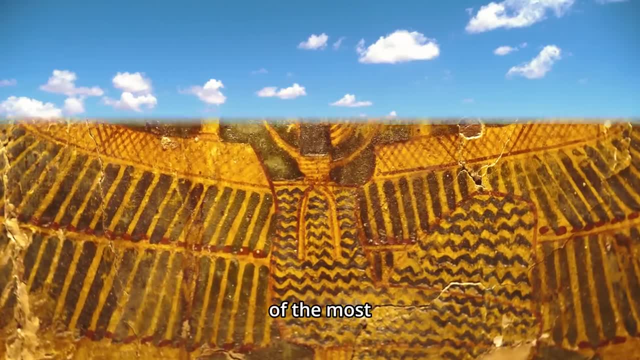 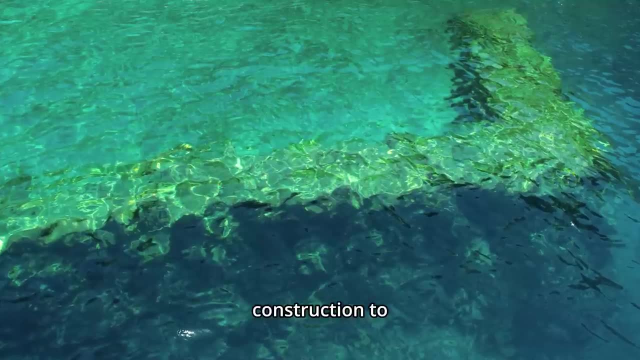 As we endeavor to piece together the puzzle of our distant past, there are numerous enigmatic gaps that remain unexplained. Even though the Great Pyramid of Giza is one of the most scrutinized monuments globally, we still grapple with uncertainty, unable to conclusively attribute its construction to the Egyptians. 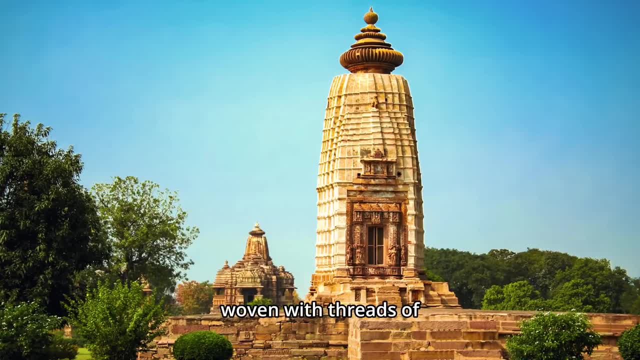 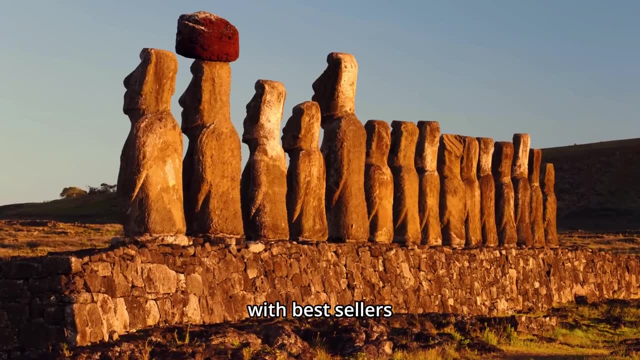 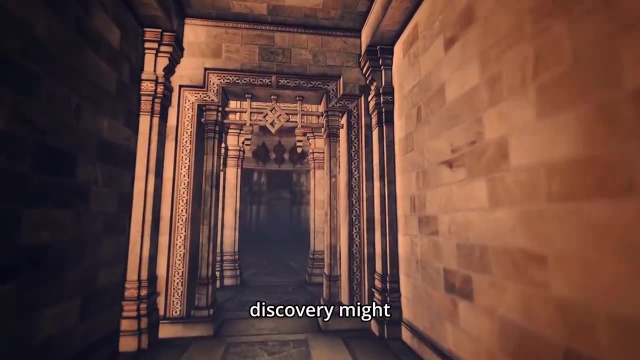 The past, it seems, is a tapestry woven with threads of uncertainty and intrigue. Peter Tompkins, a renowned American journalist and prolific author with bestsellers to his name, once offered a tantalizing perspective. He posited that each new revelation and discovery might serve as a key unlocking the entrance to an entirely uncharted realm of ancient civilization. 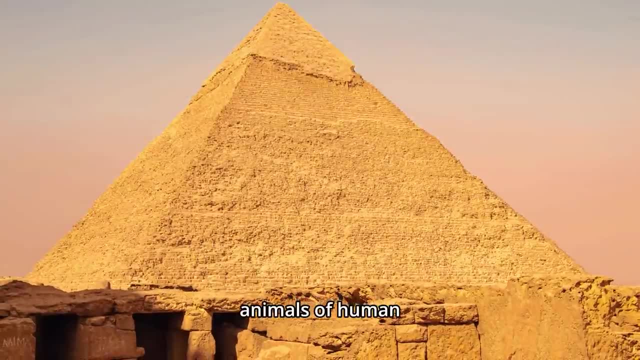 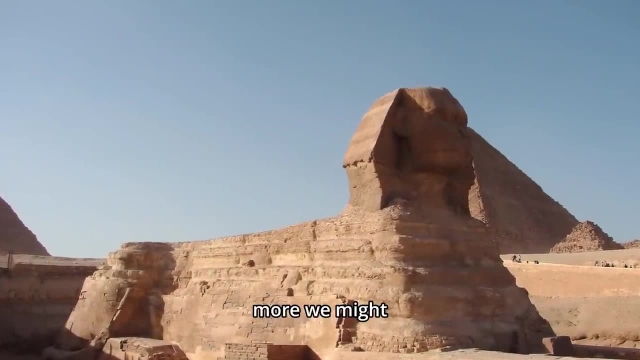 This in turn could potentially stretch the annals of human history far beyond the boundaries previously ascribed to it. In his words, the more we uncover, the more we might unearth a past more profound and extensive than we have ever dared to acknowledge. 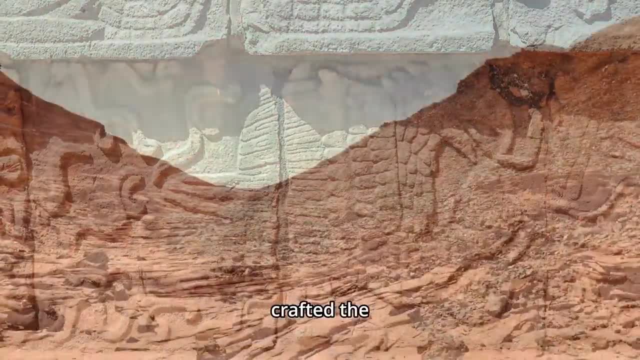 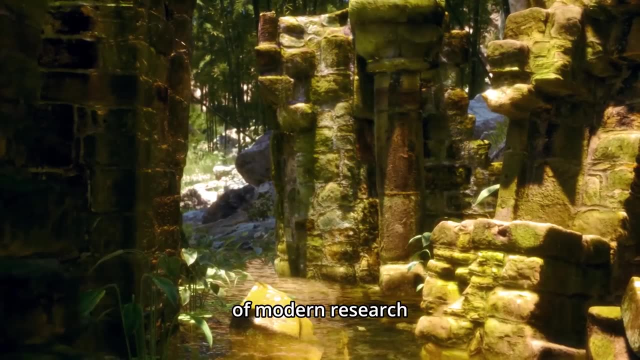 At the time when Stonehenge and the intricate ley lines were crafted, the British Isles were believed to be inhabited by tribes that appeared primitive and cave-dwelling. Yet in the light of modern research, it becomes clear that Stonehenge, with its remarkable astronomical precision. 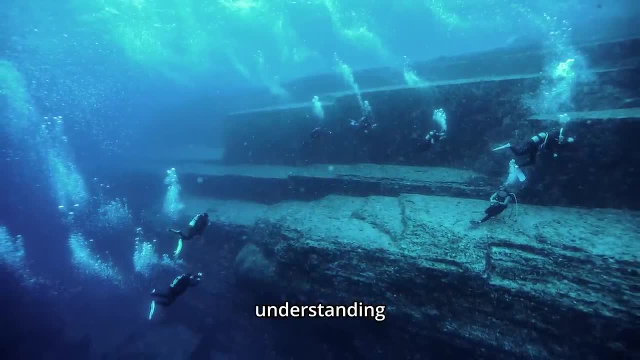 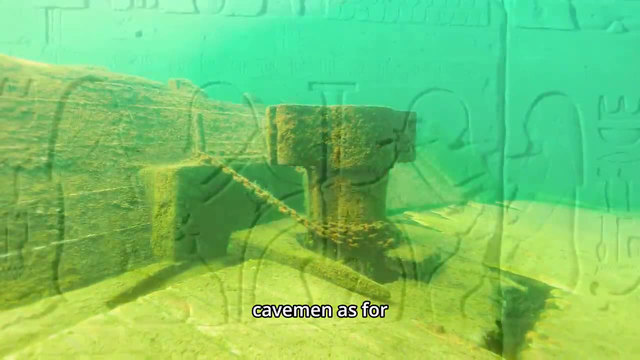 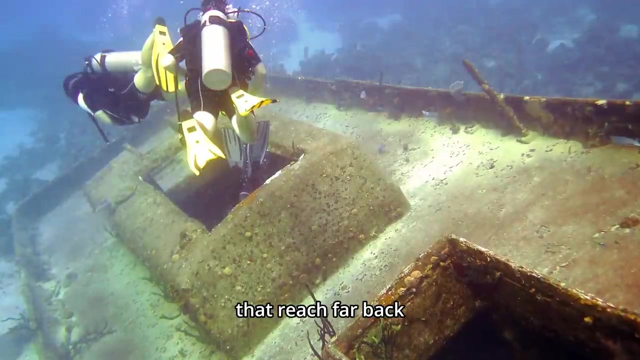 bears the signature of a culture equipped with an advanced understanding of the cosmos. The construction of this remarkable site hardly aligns with the abilities of so-called cavemen. As for the enigmatic ley lines that crisscross the landscape, they too seem to hold secrets that reach far back into ancient history. 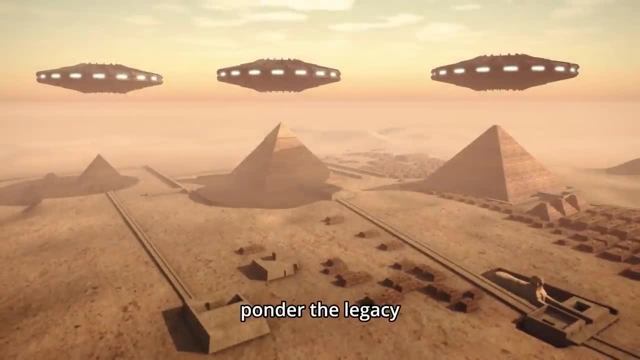 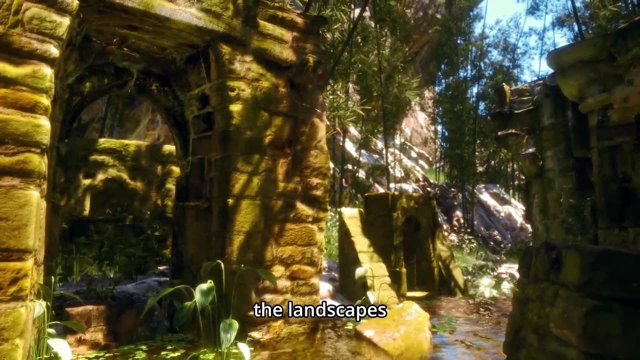 Their origins predate even the Roman invasion, leaving us to ponder the legacy of knowledge from an era that continues to elude our grasp, Much like the massive mounds that grace the landscapes of North and South America, the Great Pyramid, that magnificent sentinel of the Egyptian desert. 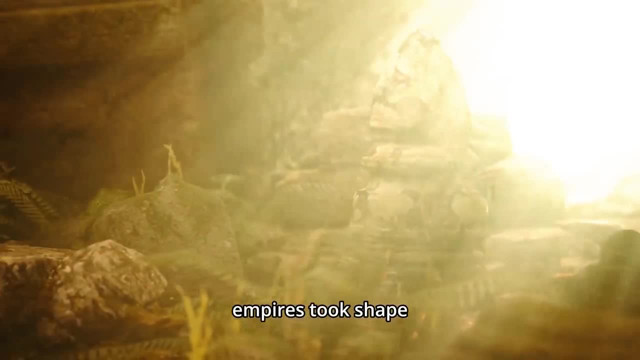 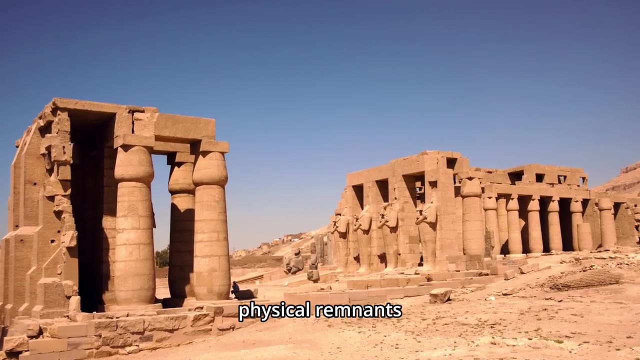 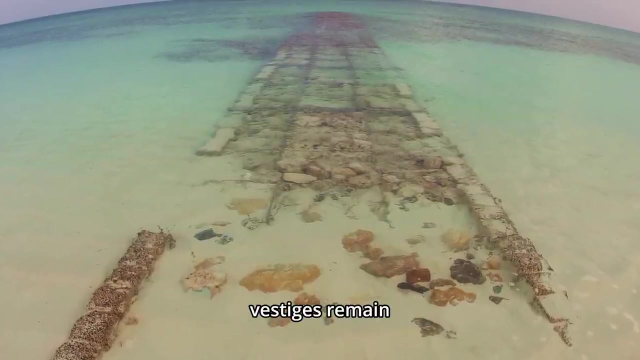 might have stood in grandeur long before the first Egyptian empires took shape. This global civilization and its intricate mythos are vividly reflected in the awe-inspiring physical remnants scattered across the world. Yet it is a peculiar and persistent enigma that many of these profound vestiges remain shrouded in mystery. 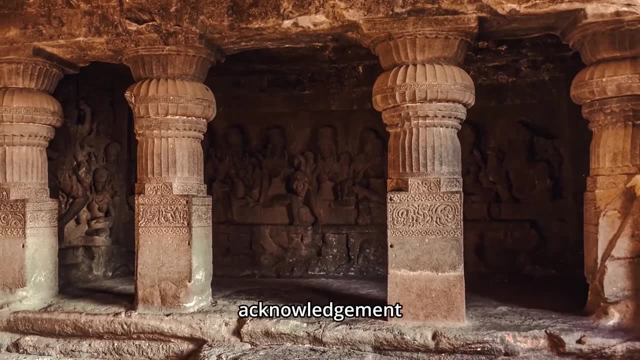 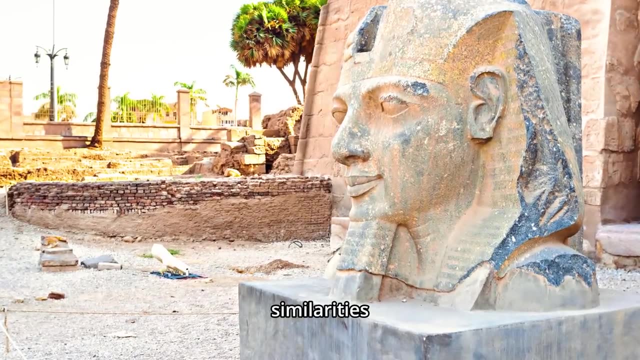 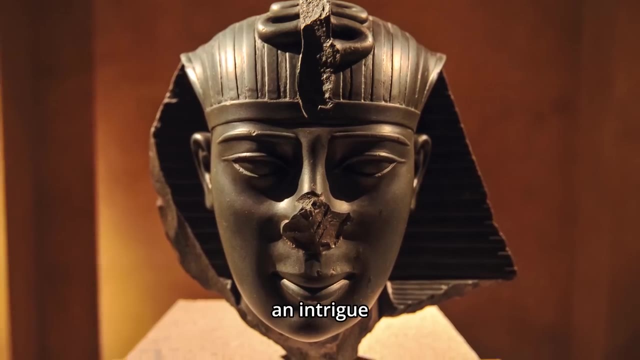 escaping the comprehensive explanations or even the acknowledgement of mainstream authorities. As we traverse the globe, we encounter ruins whose origins and striking similarities remain enigmatic, leaving us in a state of perpetual wonder. John Keel, with a sense of awe and intrigue, postulated: 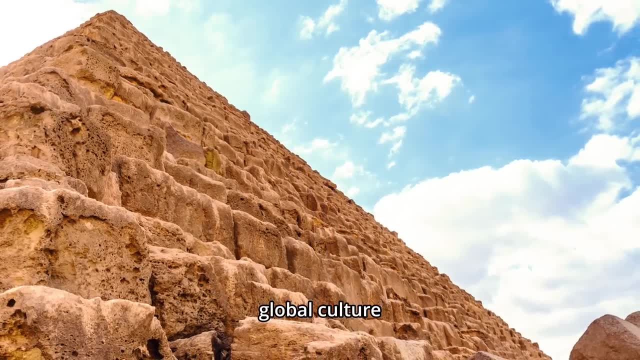 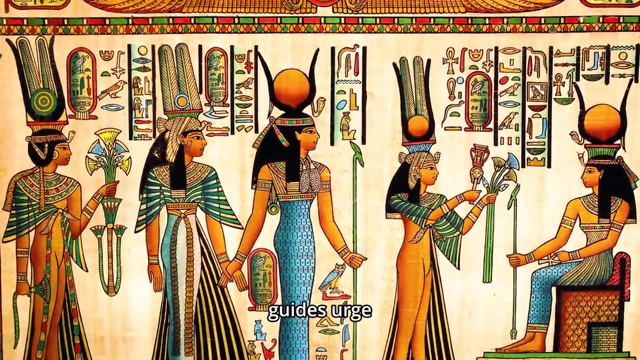 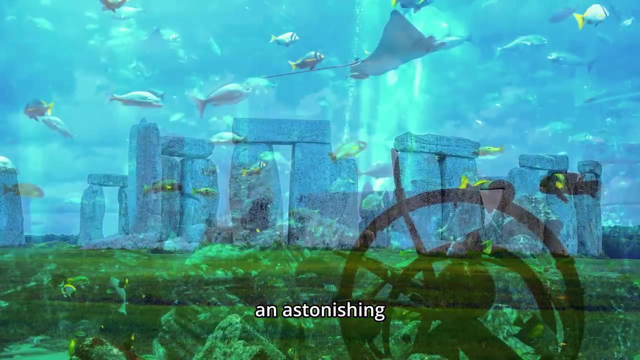 there must have been a singular global culture. at some point in the ancient annals of history, A mysterious inspiration or perhaps enigmatic guides urged the ancients to embark on extraordinary feats of construction and creation. While not definitive, an astonishing parallel emerges when one compares the temple pyramids of Peru. 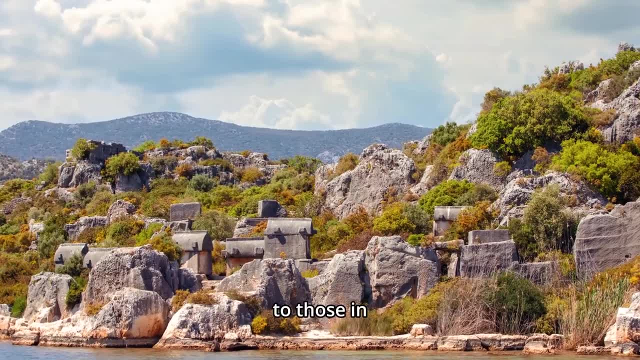 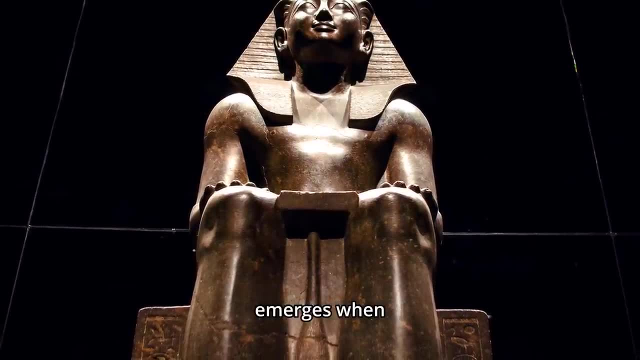 the Aztec constructions and the pre-Aztec counterparts to those in Mesopotamia, which can be traced back to the ancient Akkadians and Sumerians. A remarkable affinity emerges when one scrutinizes the architectural details of Central and South American structures alongside their counterparts in India. 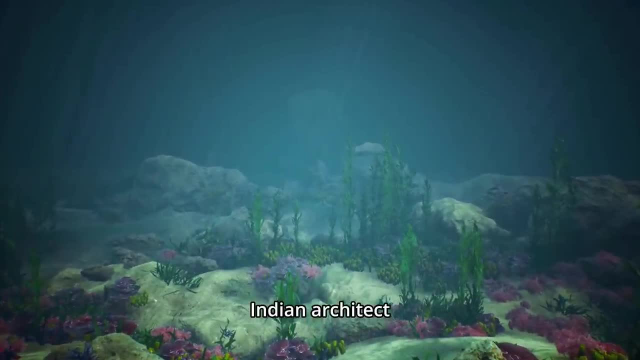 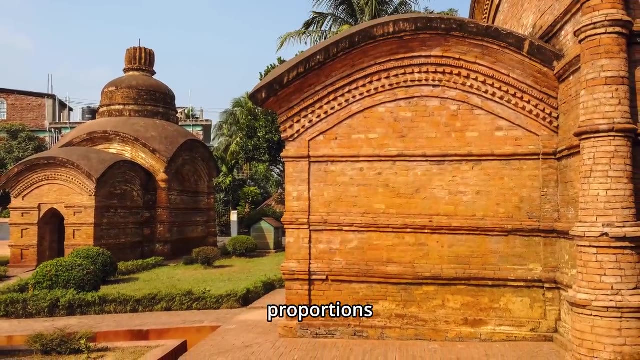 Sri V Ganapati Stapati, an Indian architect, found that the designs of Machu Picchu's edifices, encompassing elements like doors, windows, proportions, roof styles and even column sizes, mirrored those discovered in Mohenjo-daro. 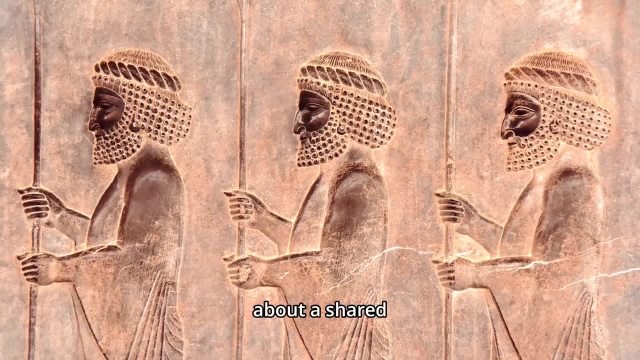 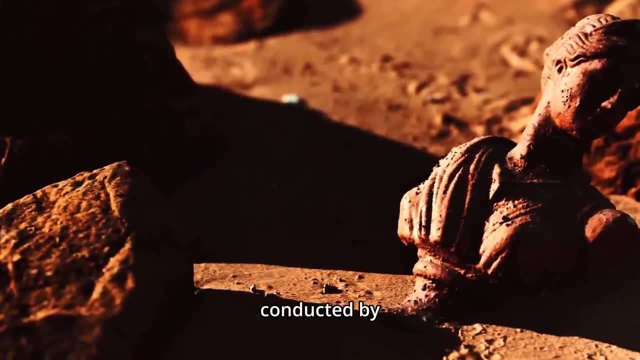 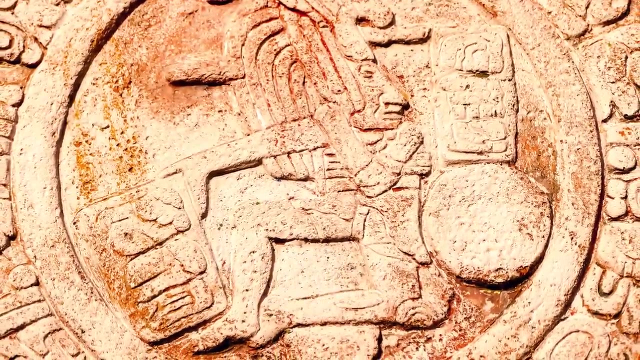 The parallel is striking and fuels speculation about a shared cultural or architectural influence across vast distances and time. Carbon dating investigations conducted by a team of Indian researchers have unveiled astonishing revelations about the age of the Indus Valley settlements. Their findings suggest that these settlements, spanning across Pakistan and northern India, 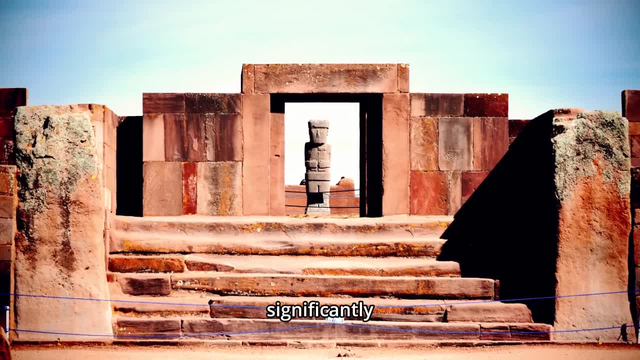 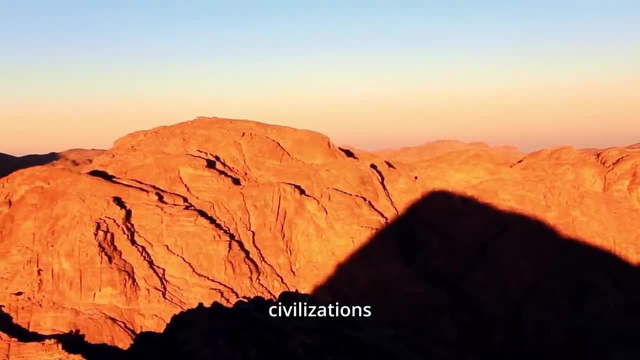 might extend back as far as 8,000 years, significantly older than previously estimated. Such a timeline could potentially predate the Mesopotamian and Egyptian civilizations. Remarkably, some experts propose that specific sections of Machu Picchu may reach back 6,000 years. 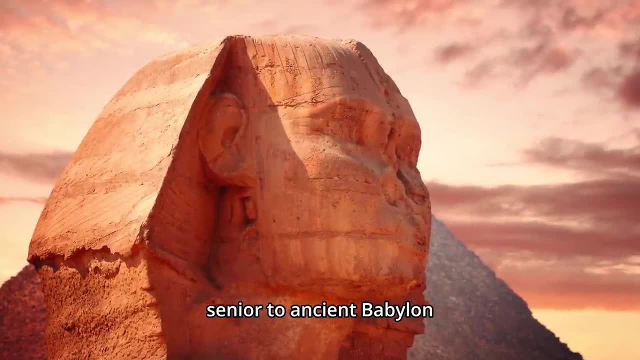 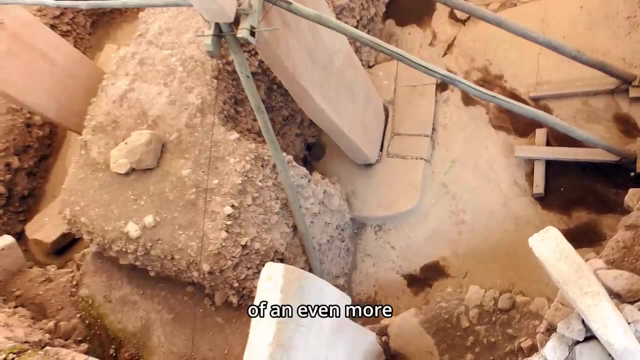 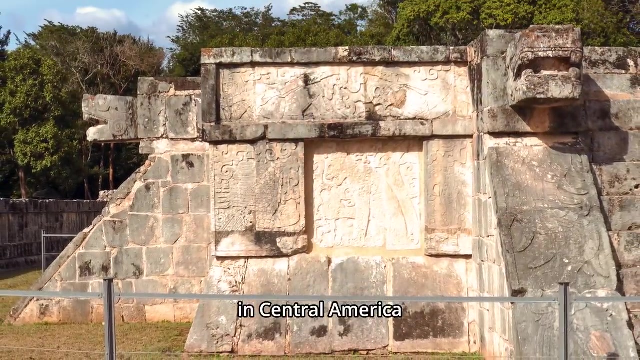 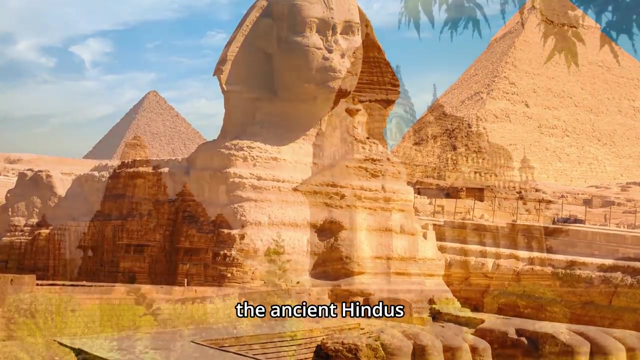 making it approximately 1,000 years senior to ancient Babylon. These intriguing revelations challenge conventional historical timelines, raising the possibility of an even more ancient and interconnected global history. When architect Stapati explored the Mayan structure, he discovered striking resemblances in both design and construction techniques shared by the Mayans and the ancient Hindus. 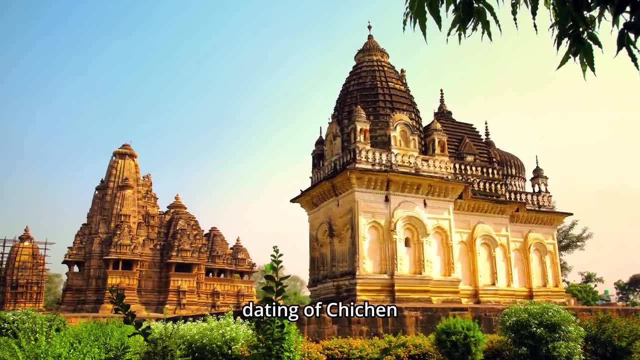 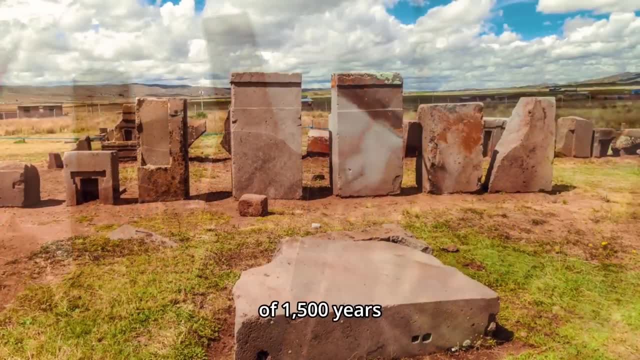 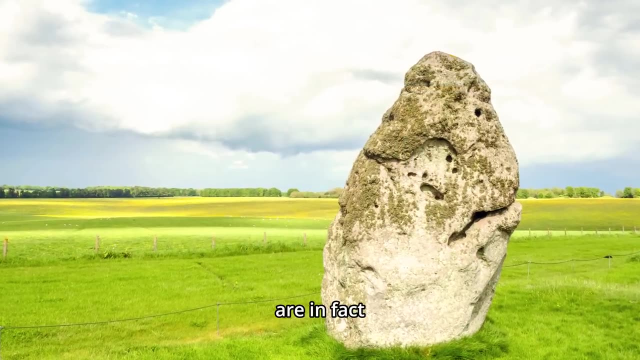 According to Jack Churchwood, the conventional dating of Chichen Itzar's stepped pyramids, temples, columned arcades and other stone constructions to the Maya of 1,500 years ago might be profoundly inaccurate. He proposes that these structures are in fact much more ancient. 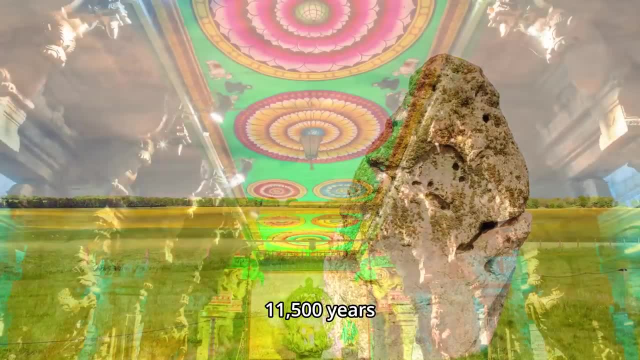 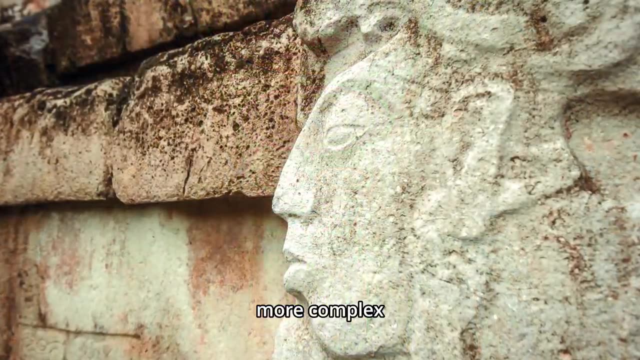 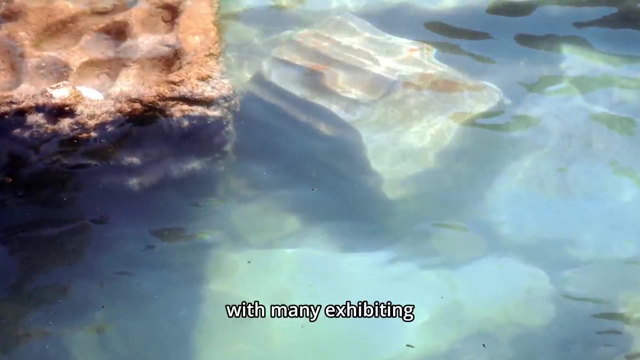 potentially dating back a staggering 11,500 years. Such a revelation challenges established historical narratives, unveiling a far more complex and interconnected past. Amidst these structures, a recurring pattern emerges, with many exhibiting signs of ancient repair and improvements through the addition of encasements layered over the original ruins. 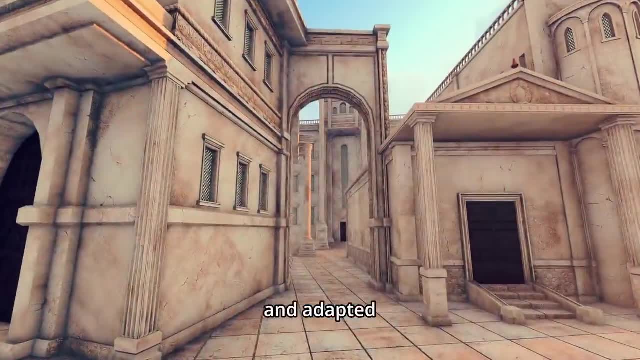 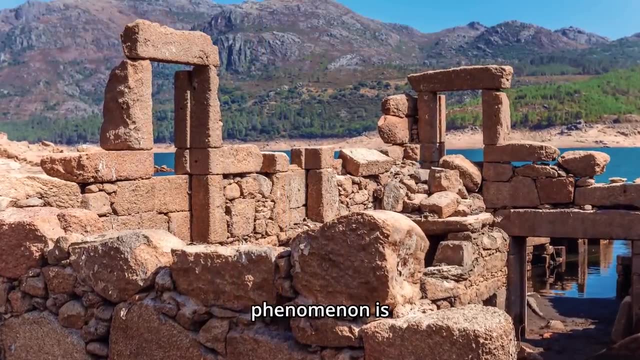 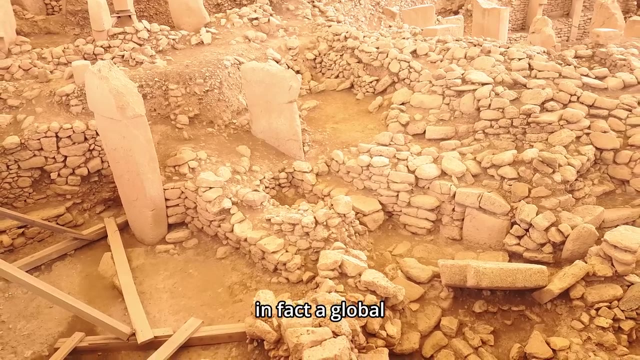 It is highly plausible that these sites were repurposed and adapted by succeeding civilizations. However, perhaps the most intriguing architectural phenomenon is the prevalence of pyramids. Pyramid construction was not limited to one geographic region, but was, in fact, a global tradition that transcended cultures and eras. 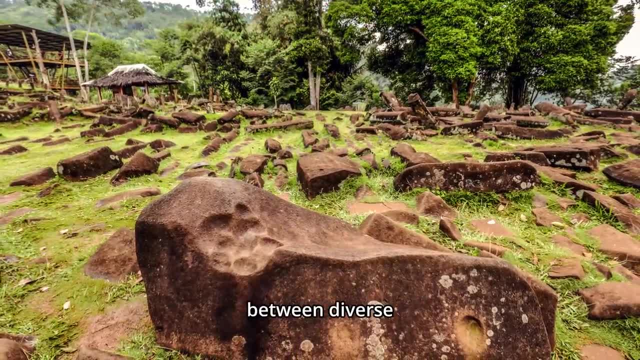 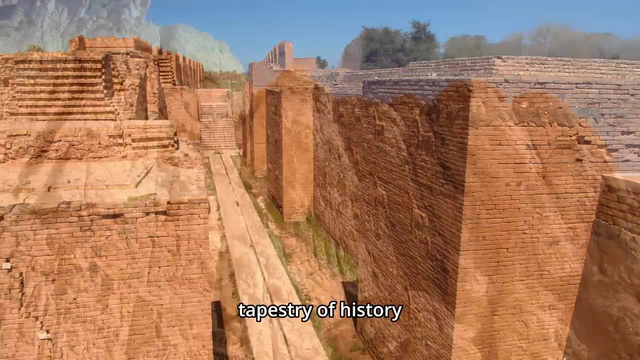 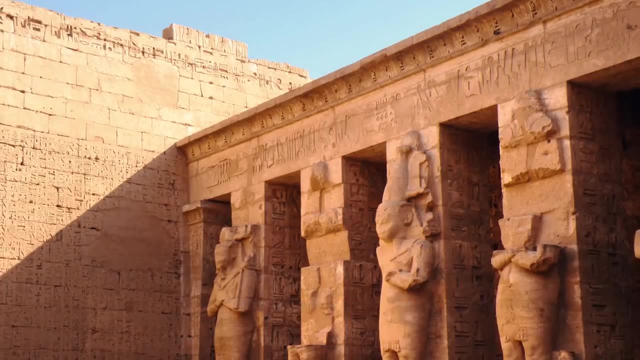 This widespread tradition hints at an underlying connection between diverse societies, one that has yet to be fully understood or appreciated. In the timeless tapestry of history, a remarkable thread emerges: the construction of colossal Mexican pyramids over six millennia ago, the enigmatic remnants of a civilization shrouded in mystery. 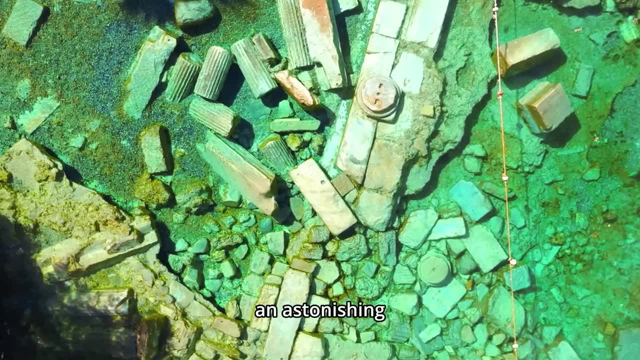 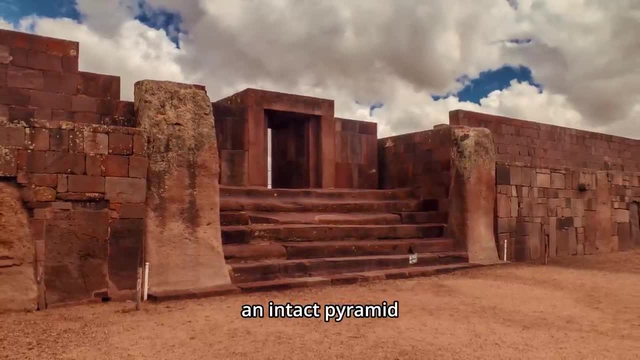 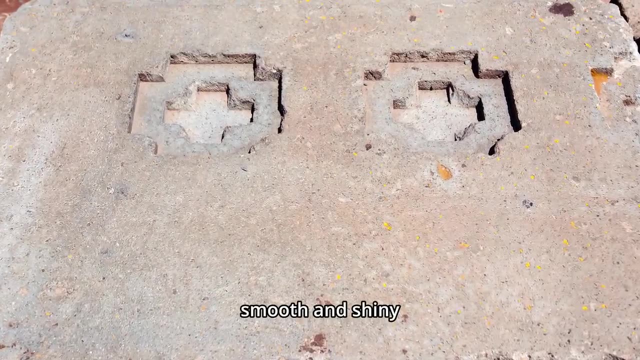 Even in the midst of the chaos of World War II, an astonishing discovery defied explanation. High in the Himalayas, near the ancient city of Lhasa, an intact pyramid was reportedly sighted. What set this pyramid apart was its surface: smooth and shiny, glistening like a gem. 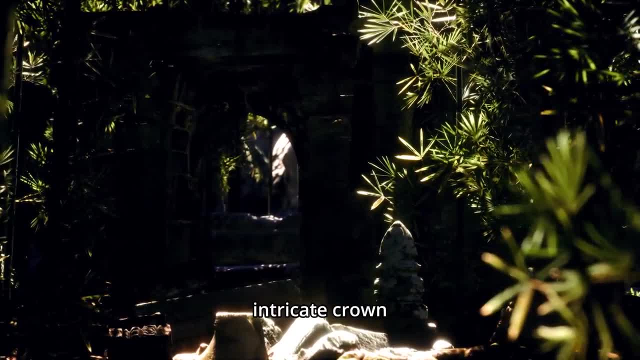 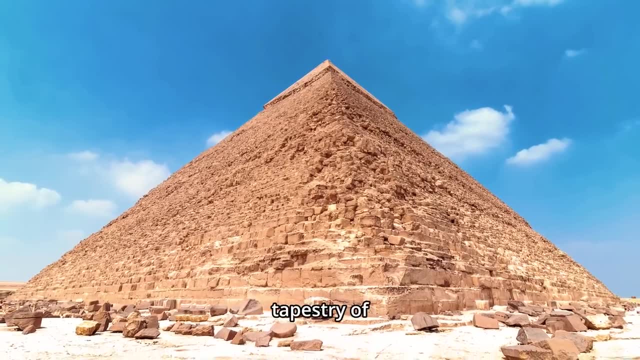 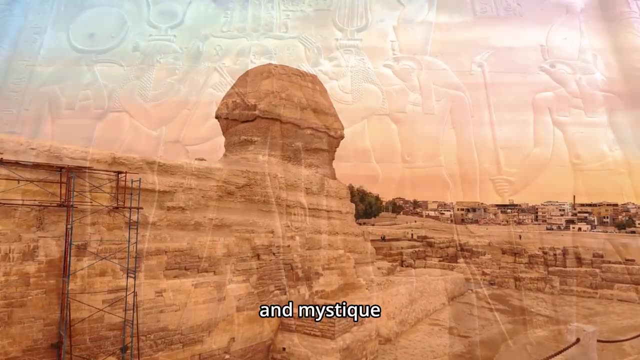 At its peak, it boasted an intricate crown of crystals. a beacon of intrigue and wonder. David Hatcher Childress delves into the remarkable tapestry of pyramids, drawing connections that span the globe. Mayan pyramids, with their grandeur and mystique, extend their presence from the heart of Central America. 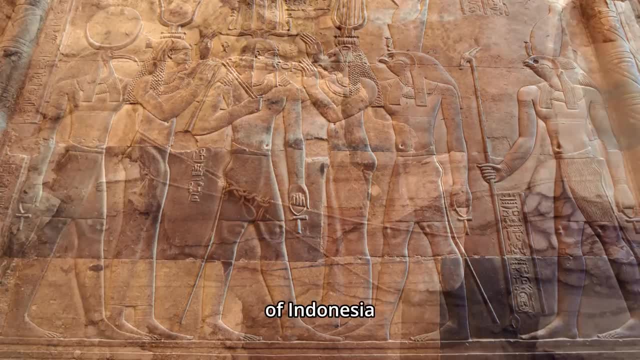 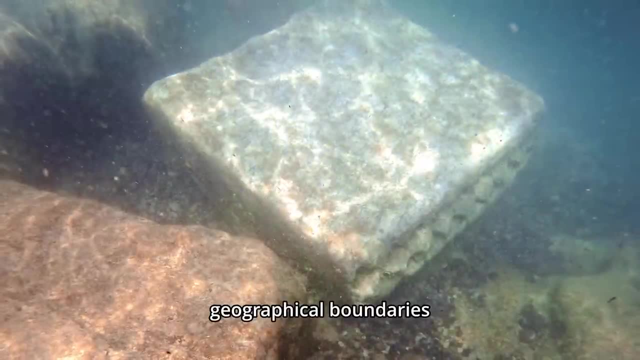 to the far reaches of Java. in the greater Sunda Islands of Indonesia, In the rugged terrain of Mount Lawu, Central Java, stands a marvel that defies geographical boundaries. The Temple of Sukur reveals a breathtaking step pyramid adorned with stone stele. 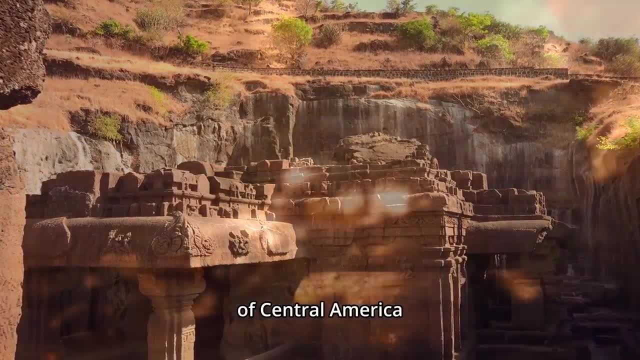 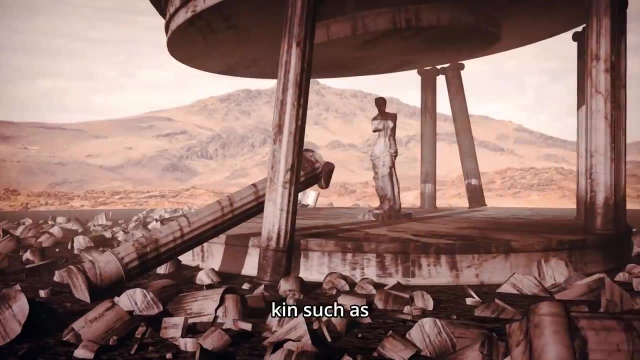 rivaling its counterparts nestled deep within the jungles of Central America. What strikes the beholder is the astonishing resemblance between the Sukur Pyramid and its distant Mayan kin, such as those found at the hallowed site of Huaxactan near Tikal in Guatemala. 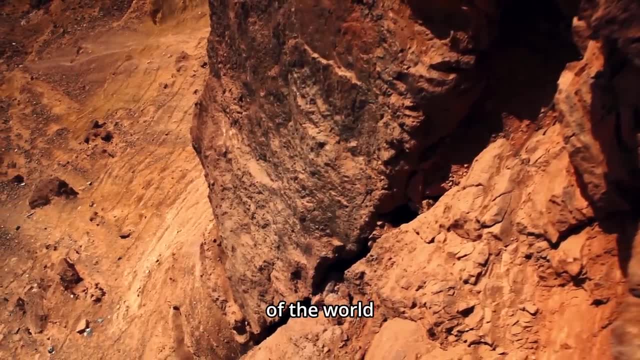 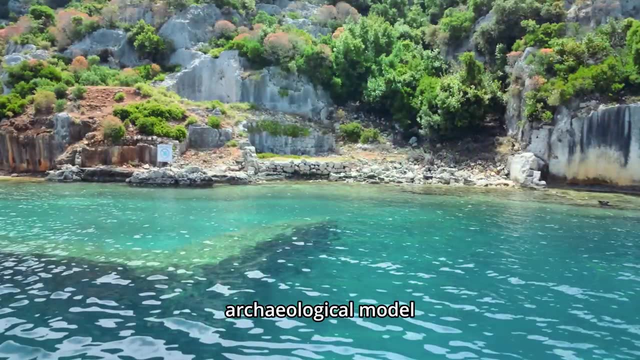 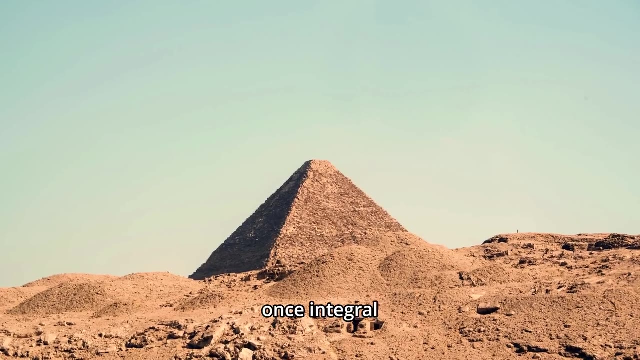 It's a testament to the enigma that unites the pyramids of the world. John Keel's exploration of our ancient past uncovers the limitations inherent in our current archaeological model. His observations point to a striking interconnectedness among these findings, suggesting they were once integral components of an advanced civilization. 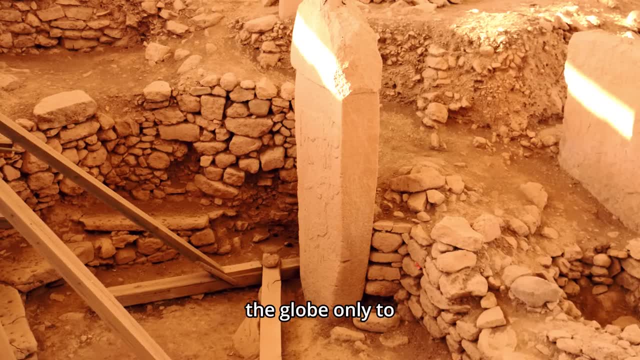 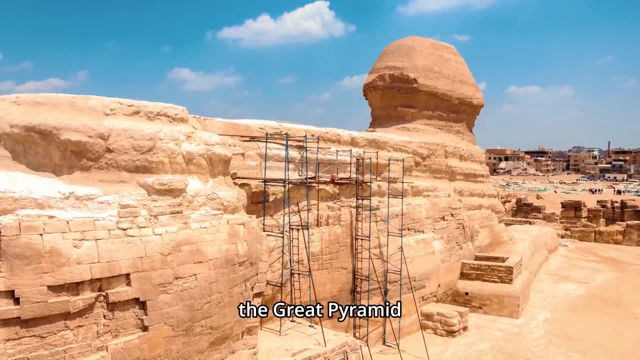 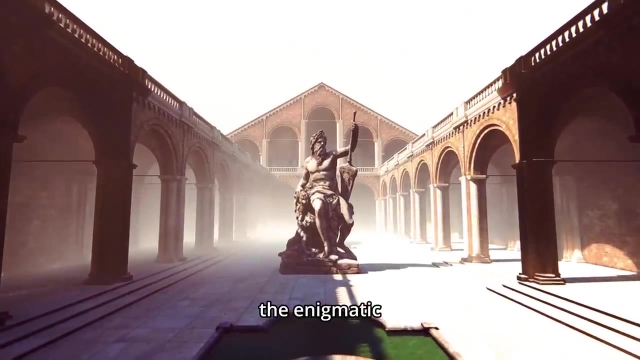 It's as if a shared culture once spanned the globe, only to vanish into obscurity. This enigma extends even further when we contemplate the Great Pyramid In the distant past, when the most ancient Egyptians first gazed upon the horizon, the Great Pyramid of Giza and the enigmatic Sphinx were mere fragments that dared to protrude above the shifting sea of desert sands. 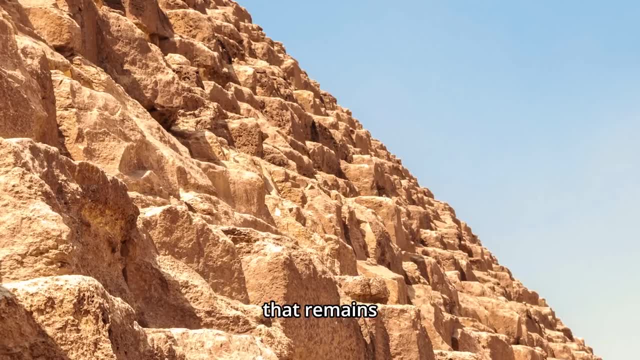 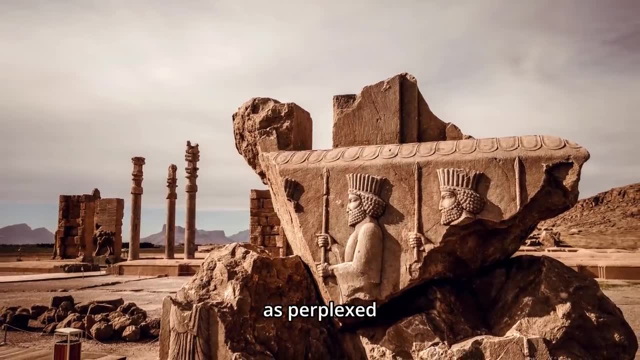 These timeless monuments stand as witnesses to an era that remains shrouded in mystery and intrigue. The ancient Egyptians who first beheld these monumental structures were as perplexed as we are today. The enigmatic Great Pyramid, an imposing testimony to human ingenuity. 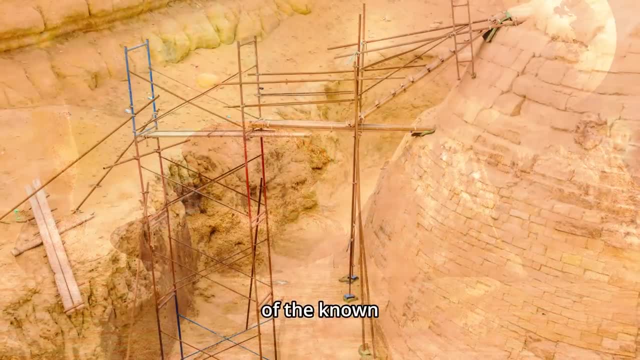 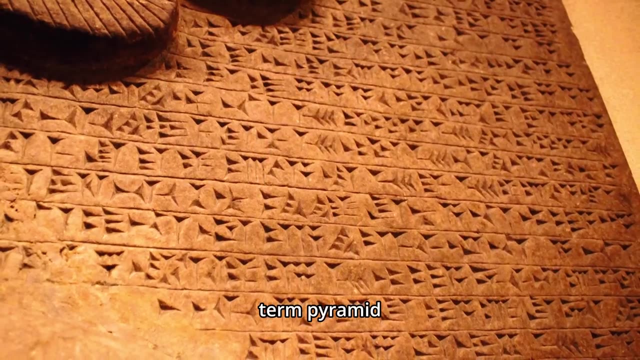 is far beyond the capabilities of the known Egyptian civilization. Delving into the origins of the word Pyramid, we encounter the intriguing term Pyramae. This word may hold a profound meaning, signifying a grand central fire akin to an altar. 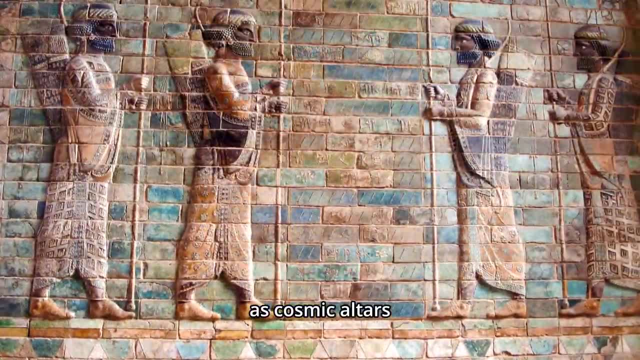 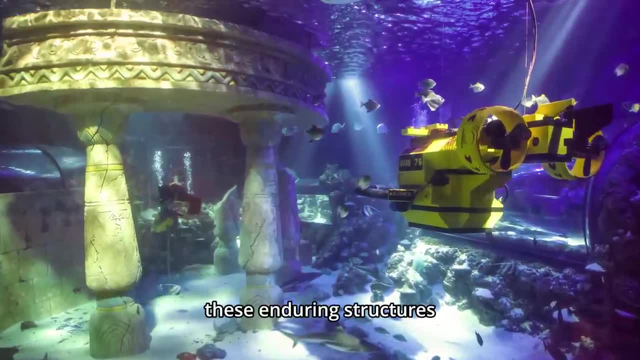 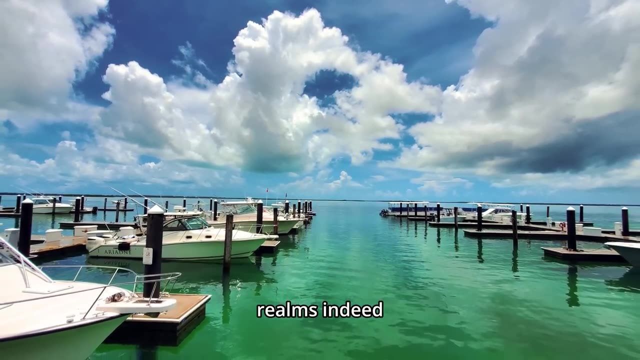 In essence, pyramids serve as cosmic altars, strategically positioned, as beacons of sacred wisdom encoding the celestial knowledge of their creators. These enduring structures symbolize a universal sanctuary that bridges the earthly and celestial realms. Indeed, the enigmatic Pyramid at Cuicuilco, Mexico, defies conventional chronologies and archaeological expectations. 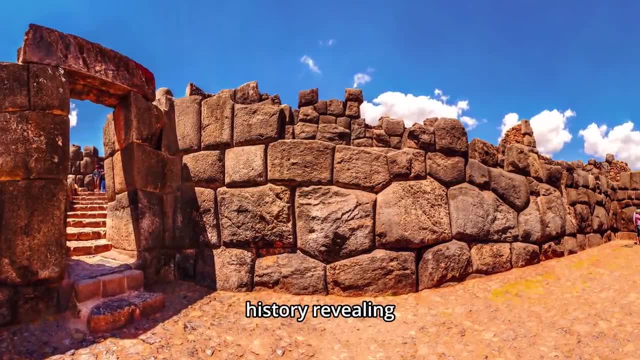 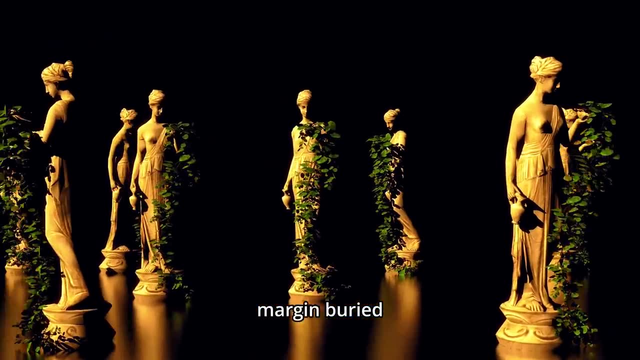 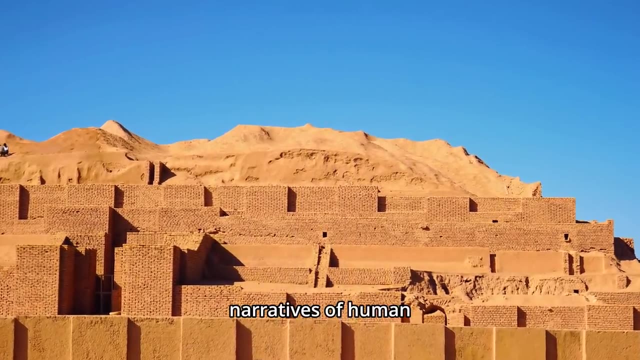 This ancient structure has pushed the boundaries of history, revealing its origins to predate the earliest known Sumerian artifacts by a significant margin, Buried beneath an 8,500-year-old layer of volcanic lava. Cuicuilco's age challenges established narratives of human civilization and its geographical spread. 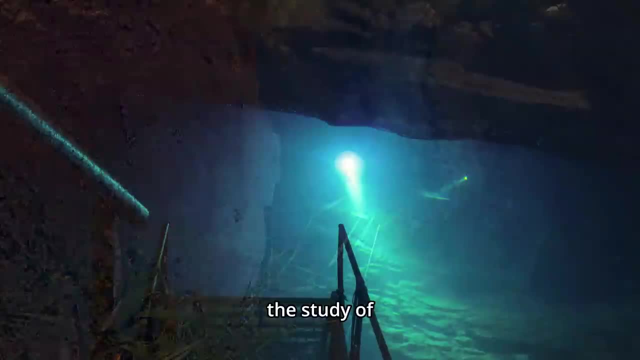 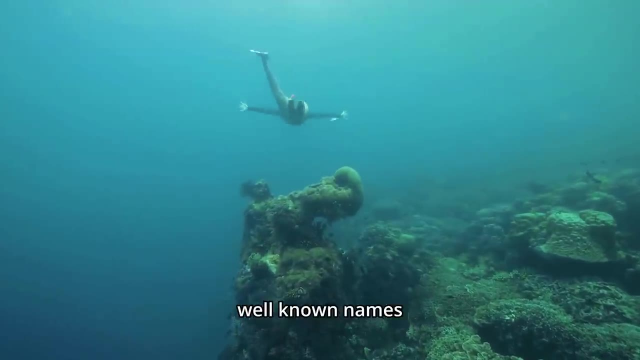 It is a testament to the mysteries that continue to unravel in the study of our shared past. If you were to ask the average person about the world's oldest civilizations, they might mention well-known names like Sumeria, Iran or Egypt, tracing their roots back to around 4000 BC. 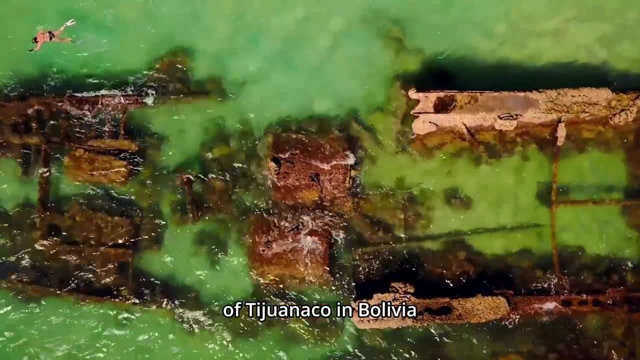 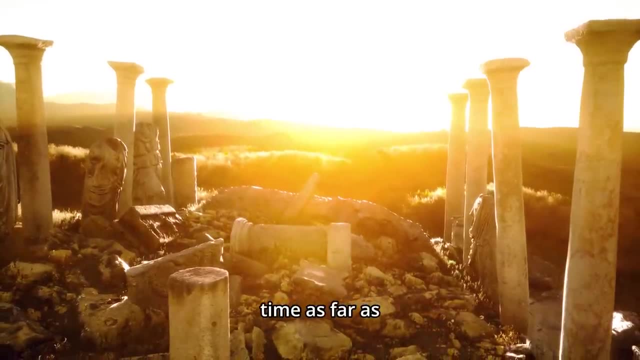 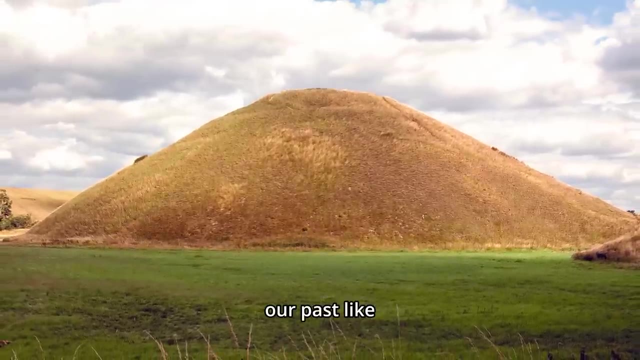 However, the mysteries hidden within the ancient ruins of Tiahuanaco in Bolivia are a far more profound picture. These enigmatic structures could potentially reach back in time as far as 15,000 years, challenging the conventional timelines of human history and beckoning us to explore the depths of our past like never before. 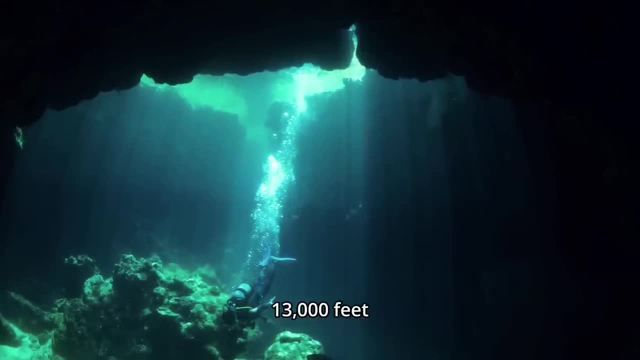 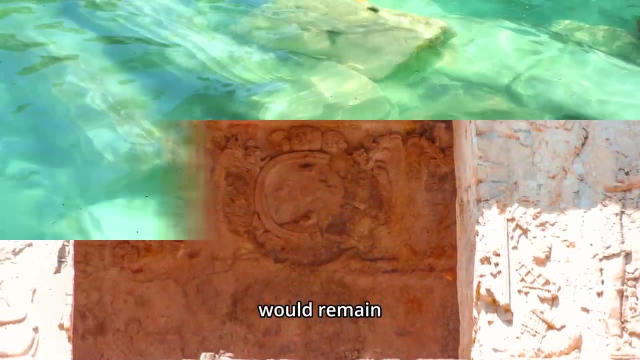 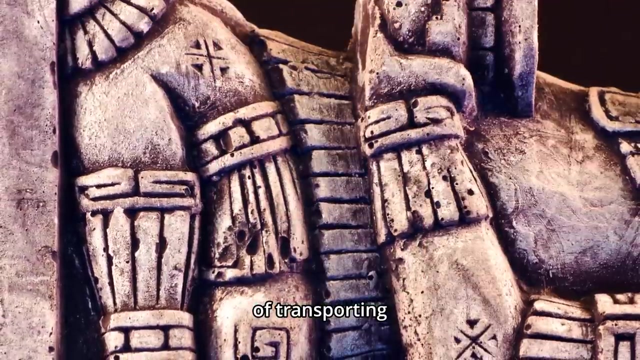 Thriving in the breathtaking, oxygen-thin atmosphere. at a lofty 13,000 feet, this ancient civilization demonstrated their mastery of modular construction techniques, which would remain innovative even in our modern era. To add to the enigma, they accomplished the extraordinary feat of transporting colossal stones. 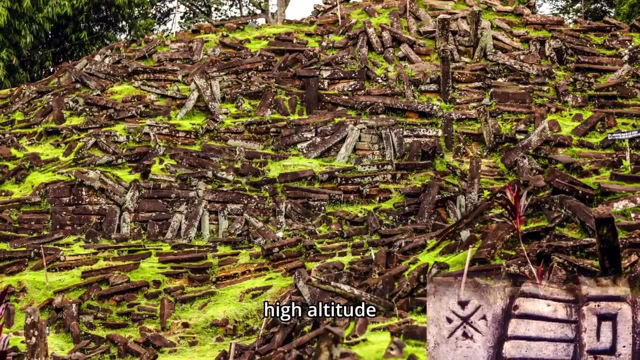 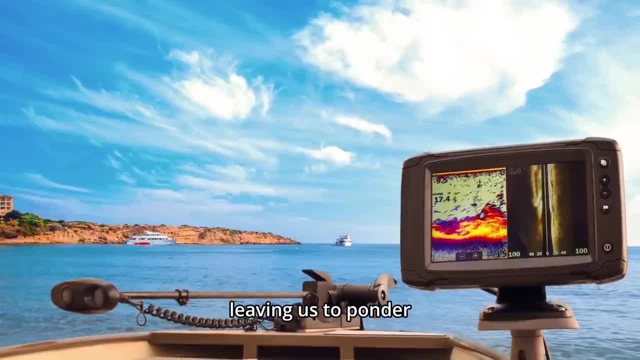 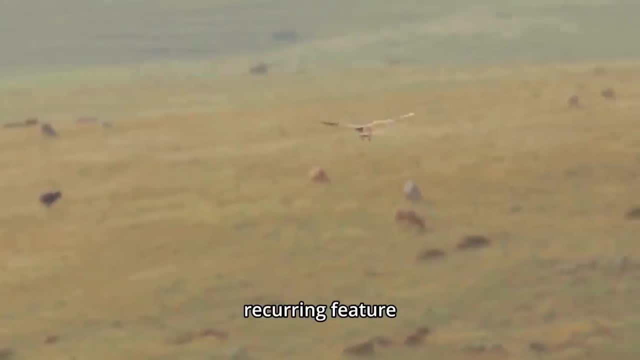 some weighing as much as 200 tons, across their high-altitude domain. Their achievements stand as a testament to their ingenuity and expertise, leaving us to ponder the remarkable capabilities of our distant ancestors. The presence of astronomical alignments, a recurring feature in ancient megalithic structures worldwide. 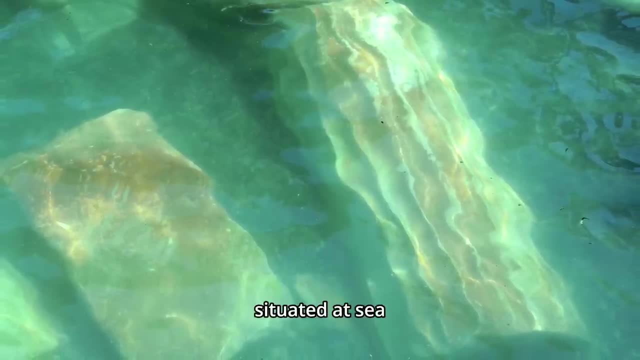 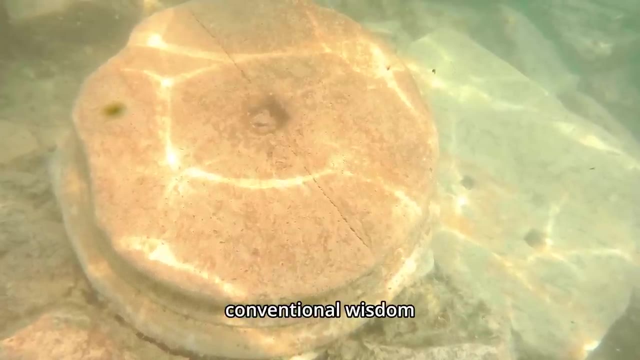 combined with the apparent fact that this city was once situated at sea level strongly hints at its profound antiquity. Naturally, these timelines challenge conventional wisdom, but it's worth noting that dates for artifacts found across the globe are gradually being extended further into the past. 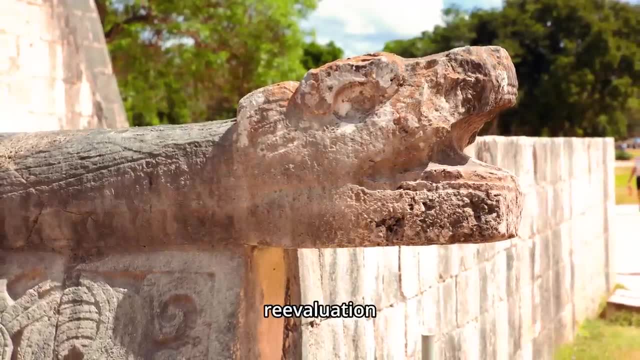 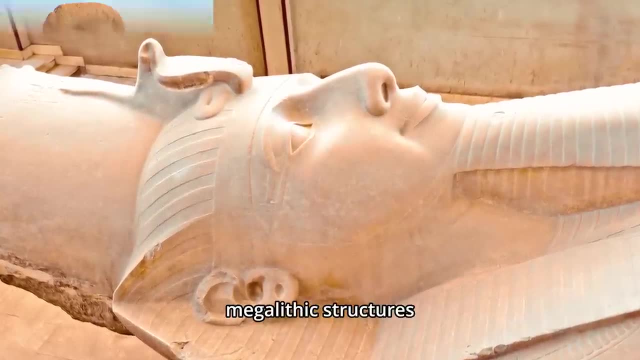 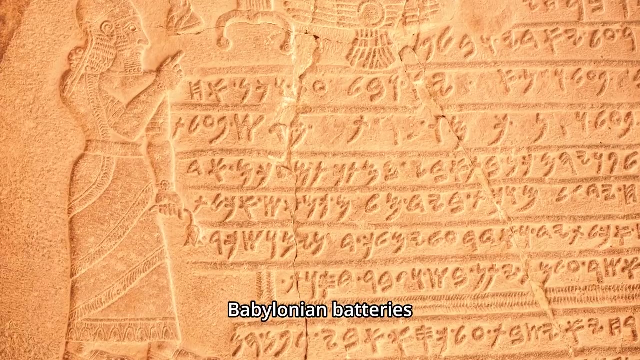 at times by several millennia. This ongoing re-evaluation prompts us to reconsider the depth of our human history. In addition to the enigmatic megalithic structures, there exists a trove of artifacts and evidence known as out-of-place artifacts, like the perplexing Babylonian batteries. 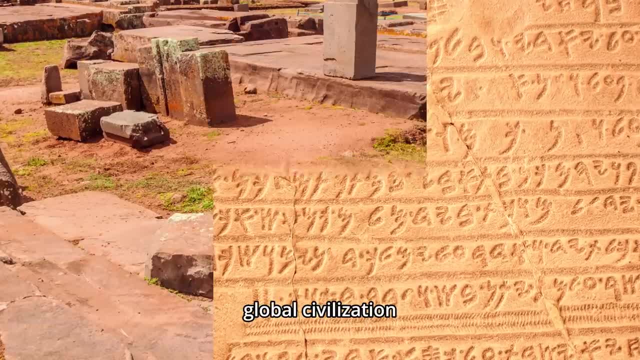 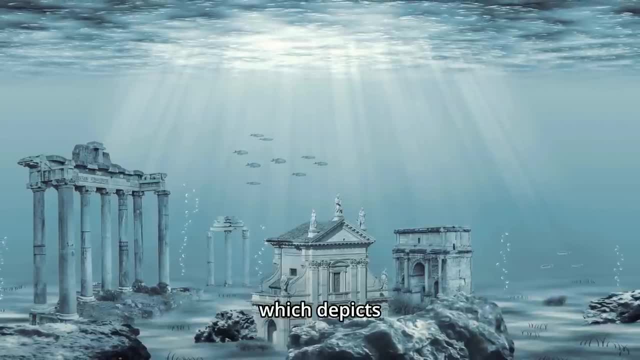 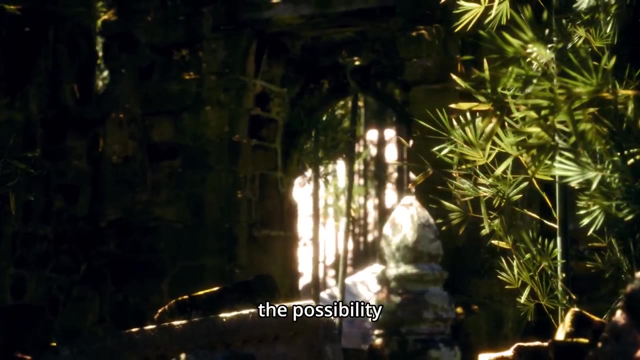 These anomalies point to the existence of a sophisticated global civilization in antiquity. Another intriguing find can be observed in a mural at Dendera which depicts what appear to be glass tubes containing electric eels. These curious depictions raise questions about the possibility of these peculiar devices. 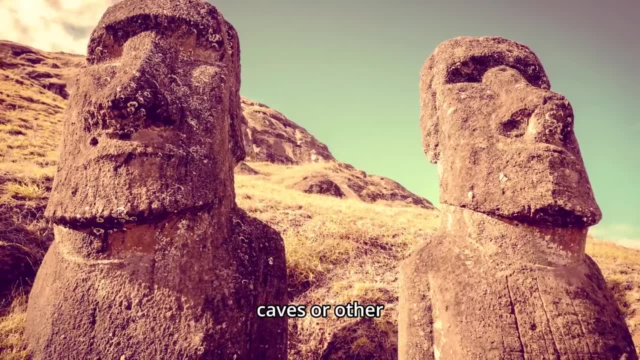 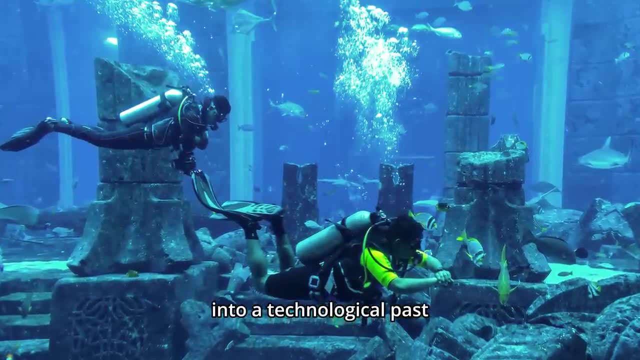 being employed for illumination in 2D. They can be found in tombs, pyramids, caves or other ancient structures. It's as if these artifacts provide us with glimpses into a technological past that defies our conventional understanding. These relics, often referred to as misplaced artifacts, 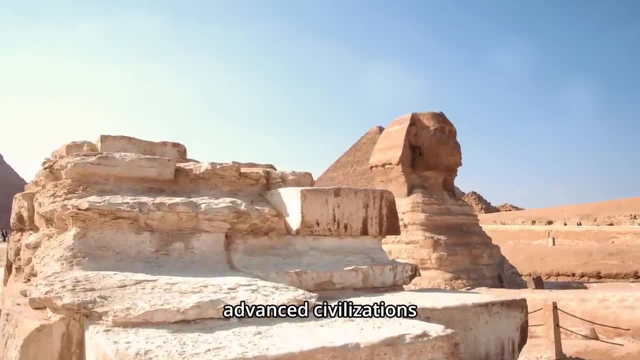 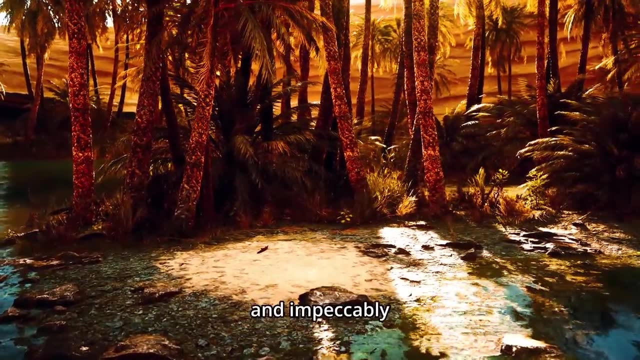 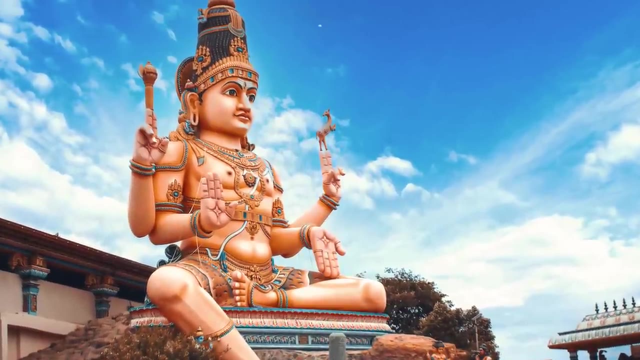 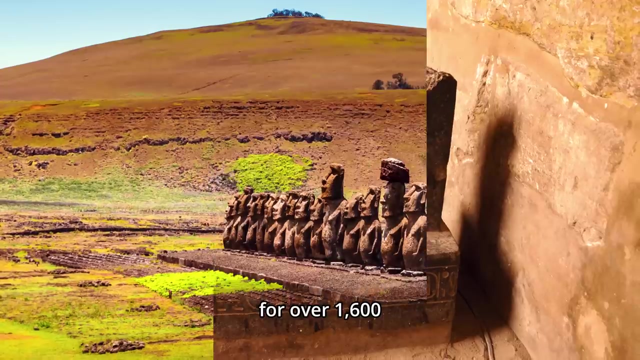 collectively paint a compelling picture of ancient and remarkably advanced civilizations predating our own. One striking example is the Ashoka Pillar in Delhi, an immense and impeccably crafted lingam constructed from iron. The true enigma lies in its astonishing durability, Despite facing the relentless onslaught of India's monsoon, rains, winds and temperature fluctuations for over 1,600 years. 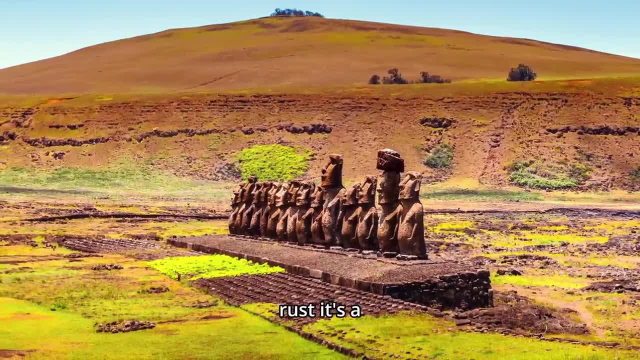 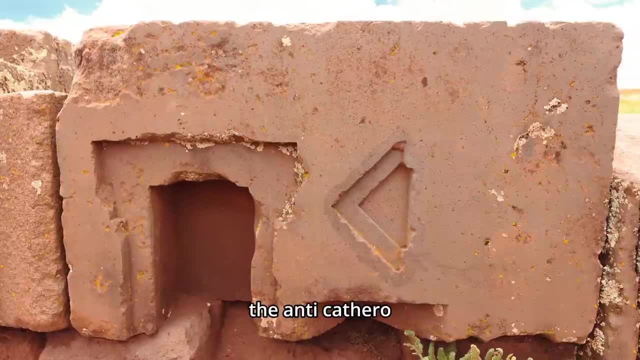 the pillar remains virtually impervious to rust. It's a testament to the exceptional knowledge and metallurgical expertise of a civilization lost in the mists of time. The Antikythera Mechanism, an extraordinary marvel hailed in the realm of science, stands as a testament to ancient ingenuity. 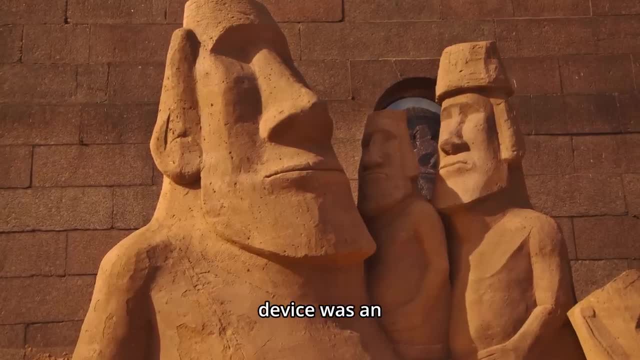 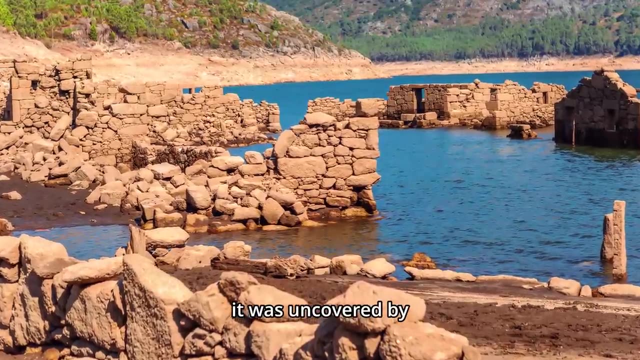 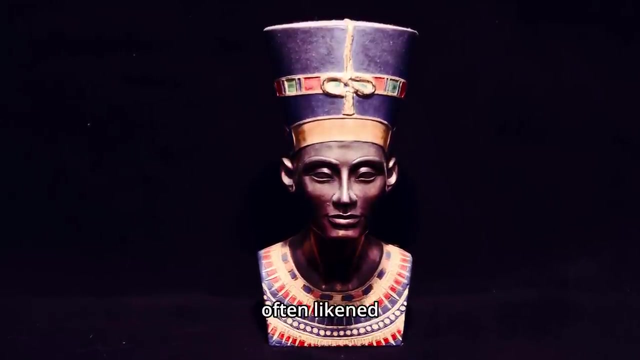 Often regarded as the world's inaugural computer, this intricate device was an ingenious invention of ancient Greece, Residing within an ancient shipwreck. it was uncovered by intrepid Greek sponge-divers on May 17, 1901.. This navigational marvel, often likened to an astrolabe, 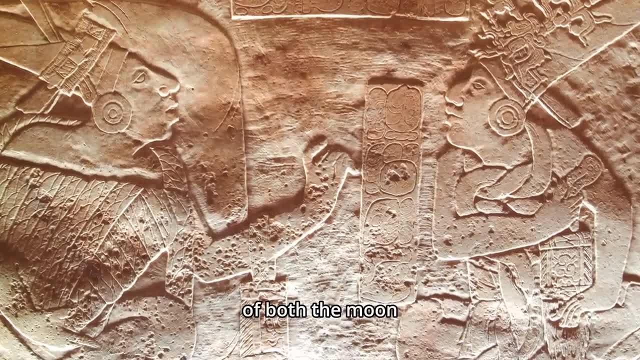 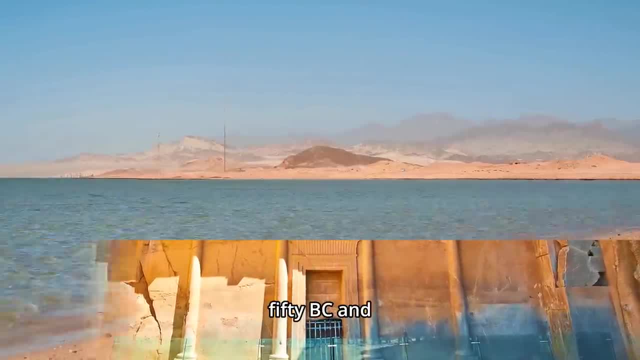 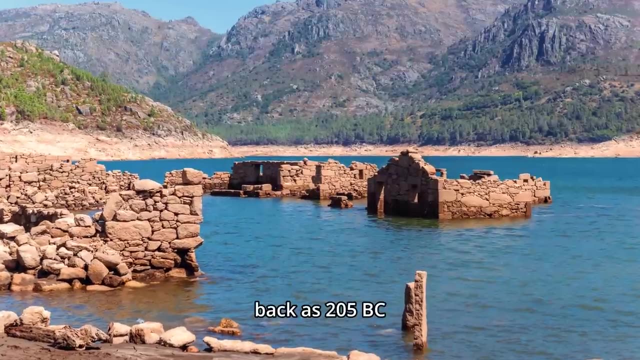 exhibited an impressive ability to compute the annual movements of both the moon and the sun. Meticulous studies indicate that its creation can be traced back to a time between 150 BC and 100 BC. An even more recent investigation suggests that its origins may extend as far back as 205 BC. 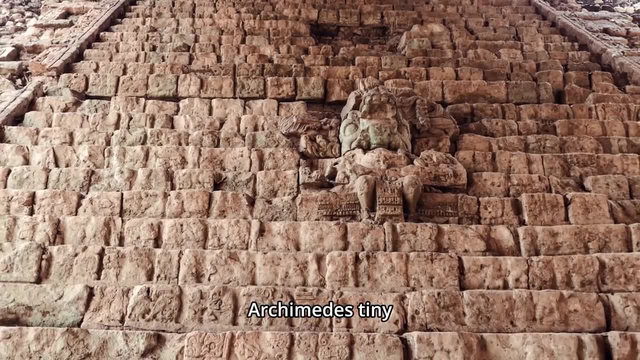 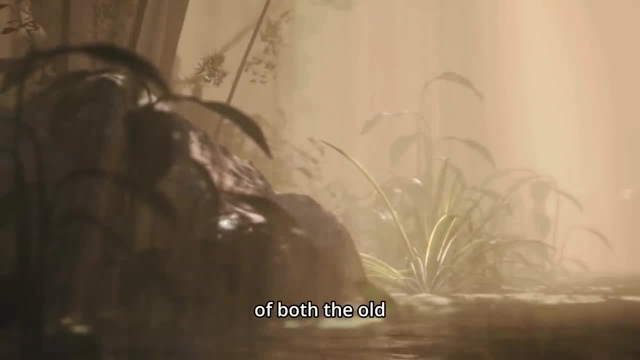 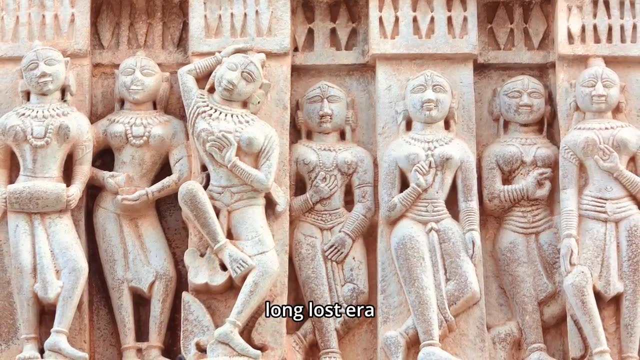 a mere seven years after the passing of the renowned Archimedes Tiny model airplanes, those intriguing artifacts of the ancient world have been unearthed in diverse corners of both the old and new worlds. These miniature marvels sparked the imagination, hinting at a long-lost era where the skies were not just a dream. 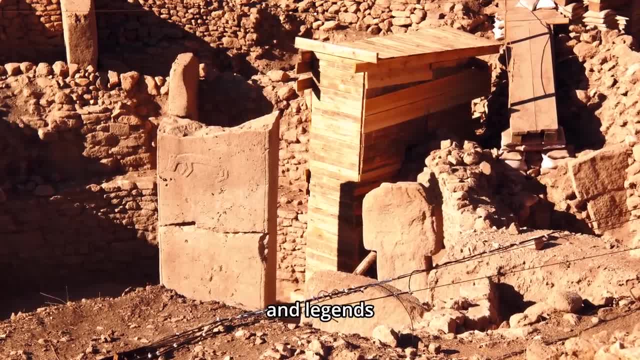 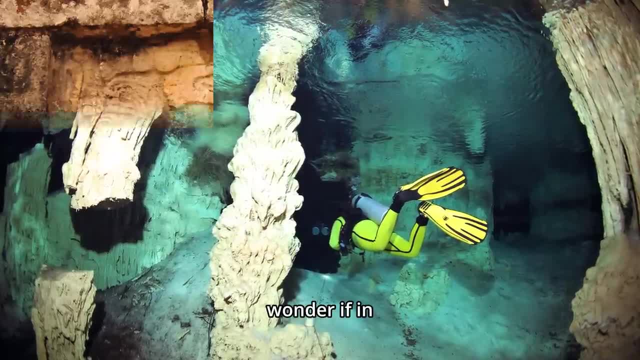 but a destination. Throughout the annals of folklore and legends from cultures worldwide, echoes of flying machines whisper across time, leaving us to wonder if, in the distant past, humanity's quest to conquer the heavens was not limited by the bounds of gravity. 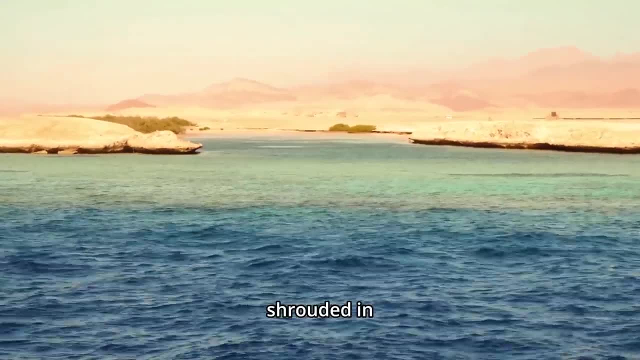 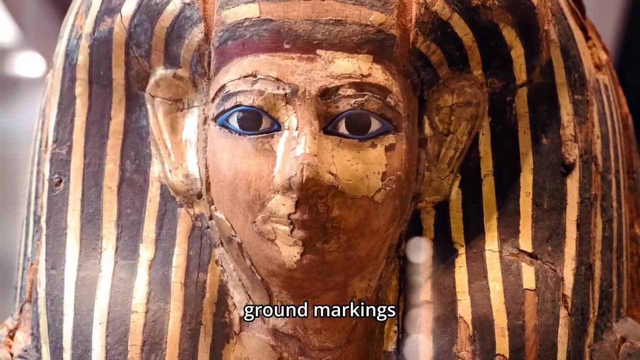 This enigmatic ancient civilization, shrouded in the mists of time, seemed to have drawn inspiration from elusive forces or beings to craft monumental ground markings only discernible from lofty vantage points, Ley lines concealed from human eyes for centuries. 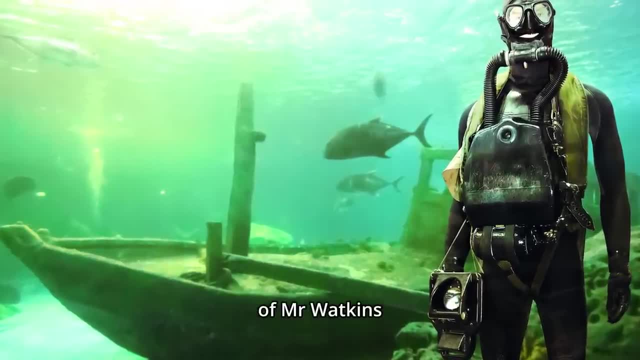 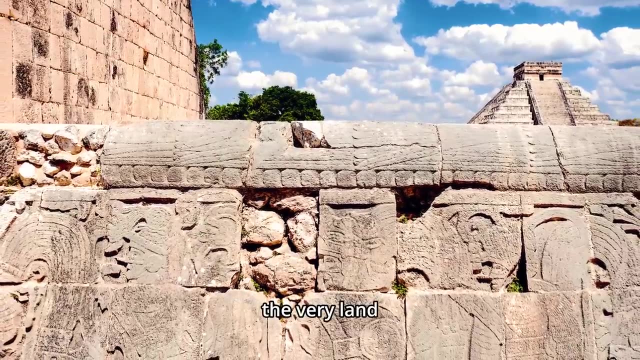 were unveiled by the perceptive gaze of Mr Watkins perched upon his hill In the wake of his discovery. aerial surveys unveiled a tapestry etched into the very land of Great Britain. Gigantic figures crafted by ancient hands sprawl across valleys and hills. 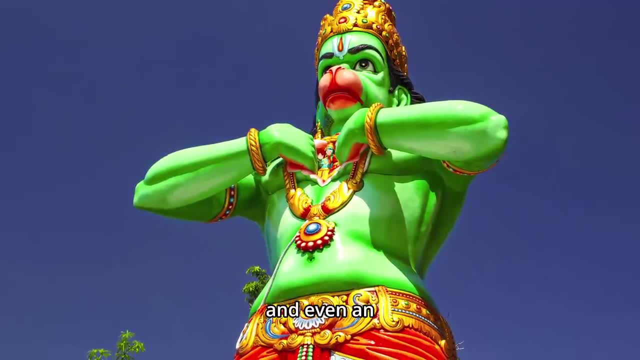 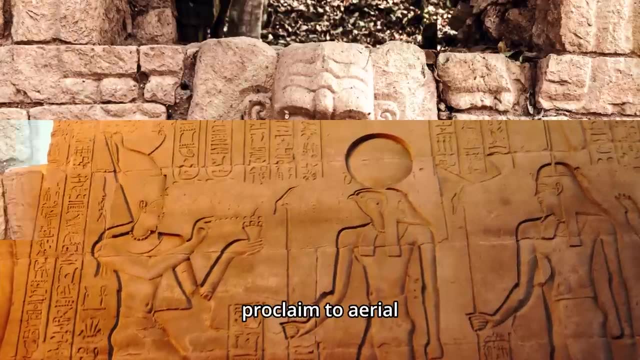 Among these colossal depictions are majestic horses and even an immense caveman Brandishing a colossal club. It's almost as if these markings were intended to proclaim to aerial visitors: cavemen reside here- a message from the distant past etched into the very earth itself. 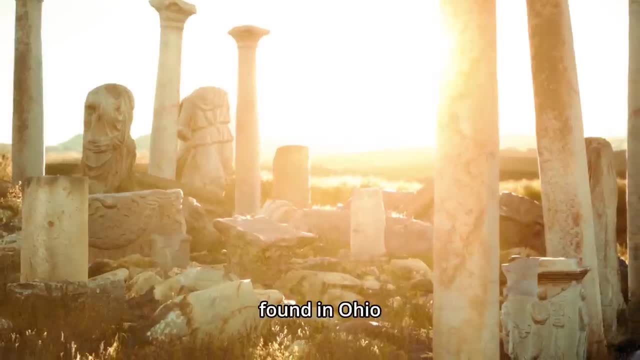 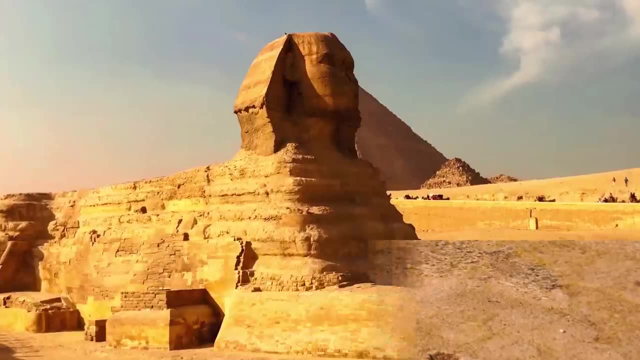 In the United States. a series of magnificent mounds found in Ohio, Mississippi and Minnesota reveal enigmatic shapes mimicking serpents and elephants. The peculiar aspect is that elephants have long been extinct in North America, stretching back thousands of years. 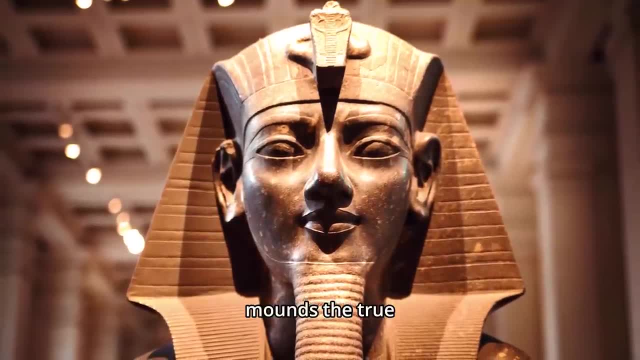 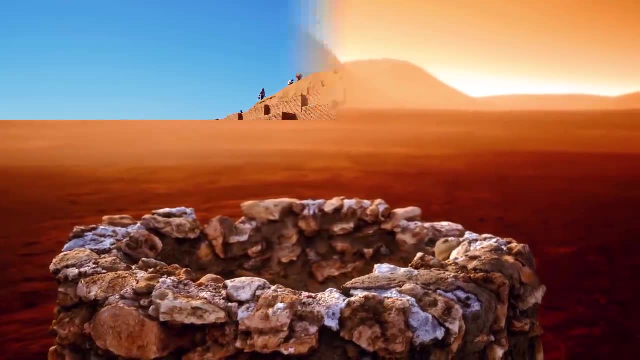 Even when standing atop one of these mounds, the true extent of their design remains hidden from view, for it is only from the heavens above that their intricate forms come into focus. These mysterious creations, etched into the very landscape, are shrouded in secrecy. 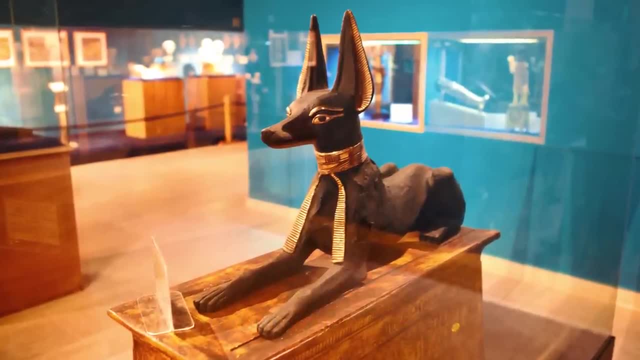 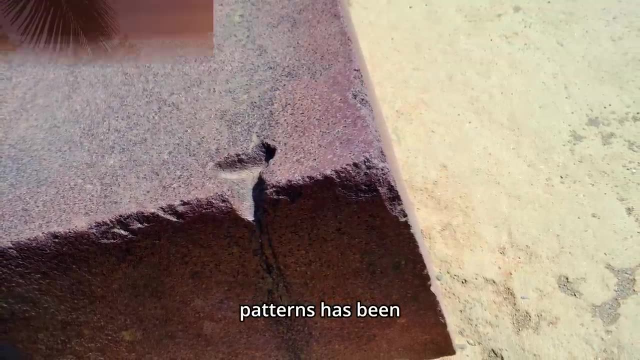 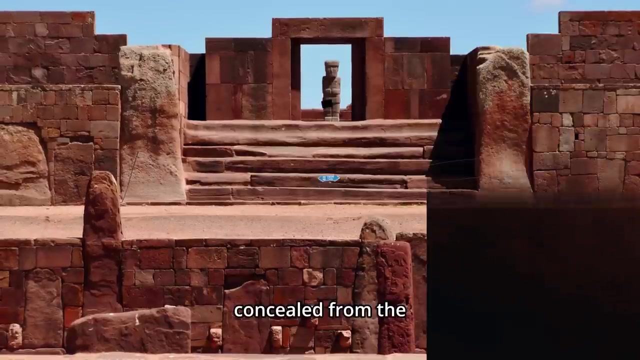 their full grandeur unveiled solely to those soaring high above, Stretching from the verdant landscapes of Florida to the rugged terrains of California. a tapestry of intricate patterns has been etched into the earth itself. Yet these cryptic designs remain veiled, their true nature concealed from the terrestrial eye. 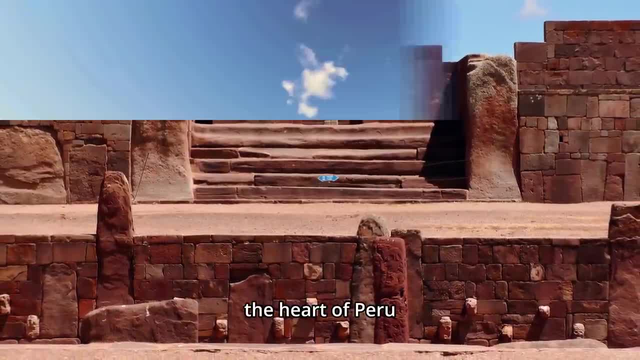 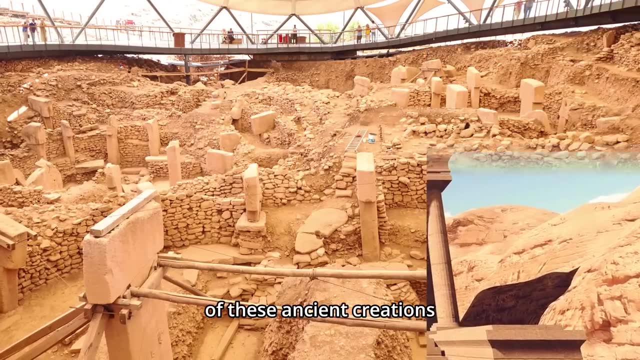 Much like the enigmatic Nazca Lines in the heart of Peru, where gigantic serpents, sprawling spiders and other mysterious creatures come to life. the full majesty of these ancient creations unveils itself only to those who soar above the land. 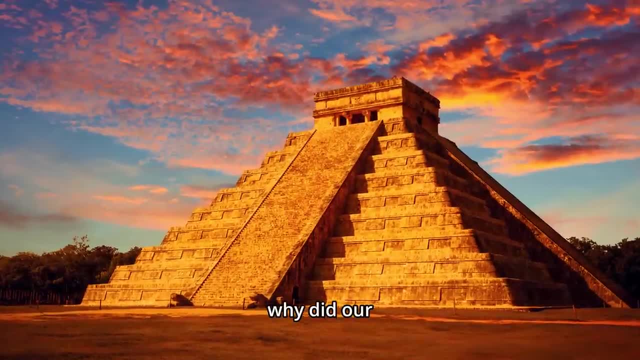 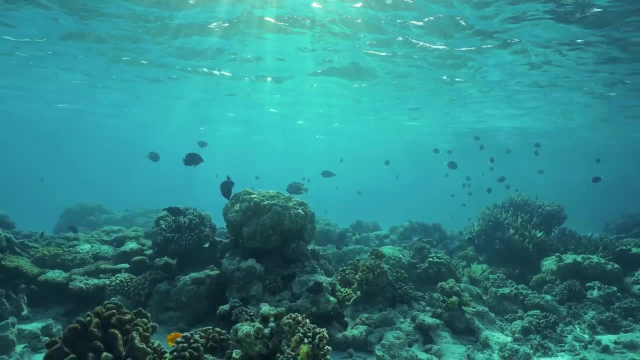 The question that beckons is this: Why did our enigmatic forebears invest such tremendous effort and dedication in crafting these seemingly purposeless mounds and formations? In the storied land of Peru, a treasure trove of 50,000 meticulously etched stones has come to light. 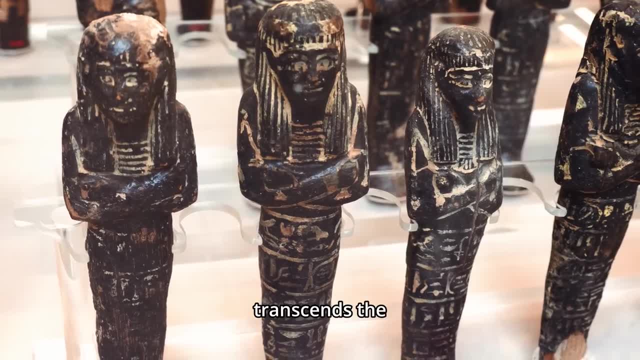 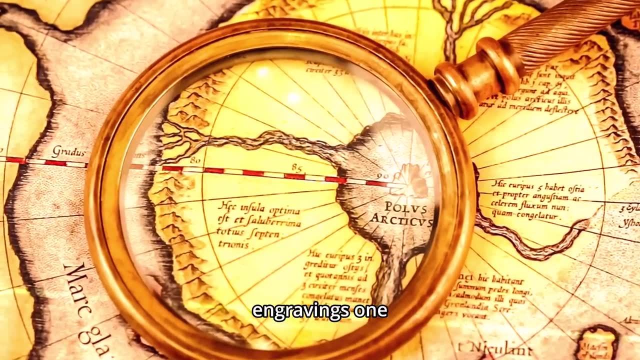 These ancient artifacts bear witness to a world that transcends the boundaries of time, where humans intermingle with creatures both living and long extinct. Among these remarkable engravings, one can discern constellations mapping the celestial realms and the intricate dance of the zodiac. 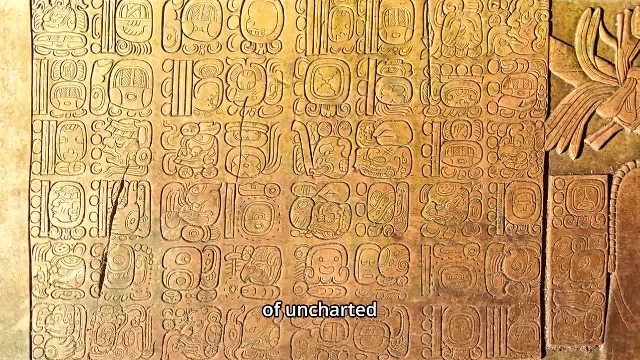 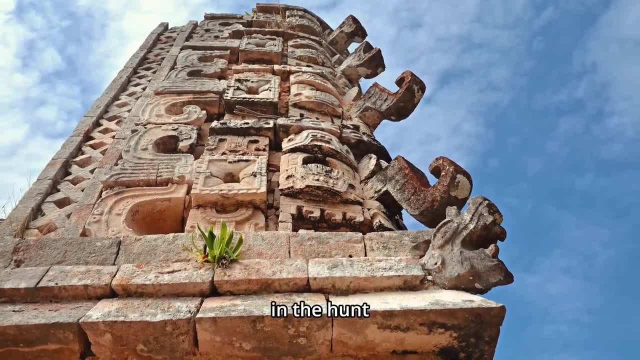 Even more astoundingly, they also unveil detailed charts of uncharted lands awaiting discovery. In this prehistoric tableau, our ancestors are depicted in the hunt, pursuing creatures that belonged to a bygone era where pterodactyls took to the skies, stegosaurs roamed the earth. 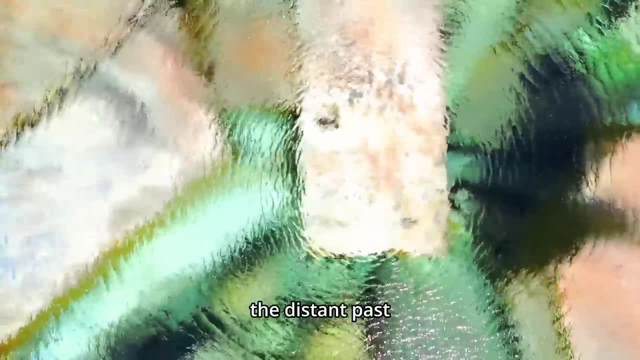 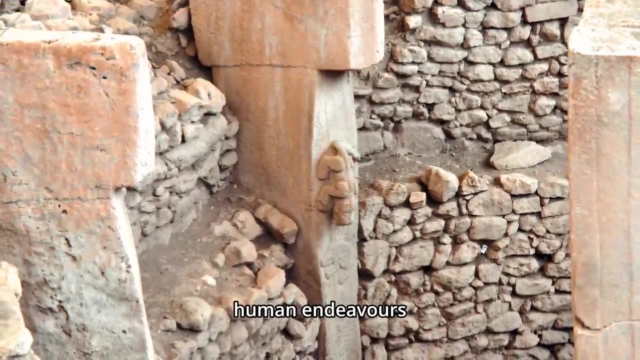 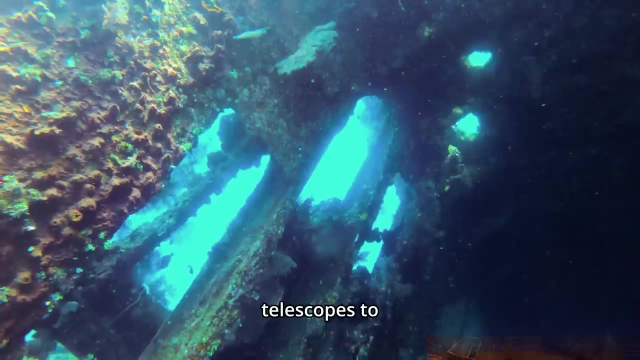 and brontosaurs cast their colossal shadows all in the distant past, some 22.5 million years ago. Even more astonishingly, these ancient stones depict human endeavors that defy our conventional understanding of history. They capture scenes of people utilizing intricate telescopes to peer into the cosmos. 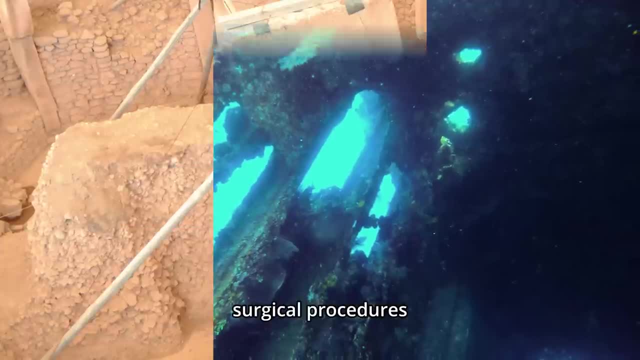 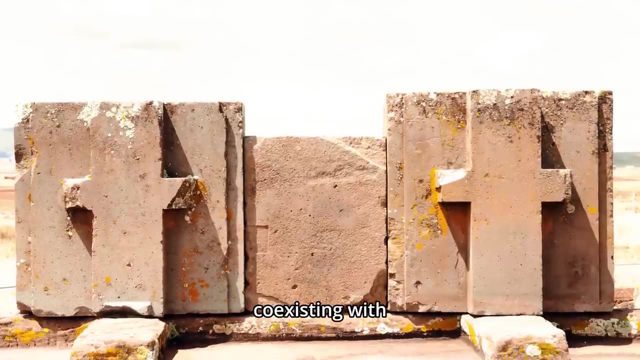 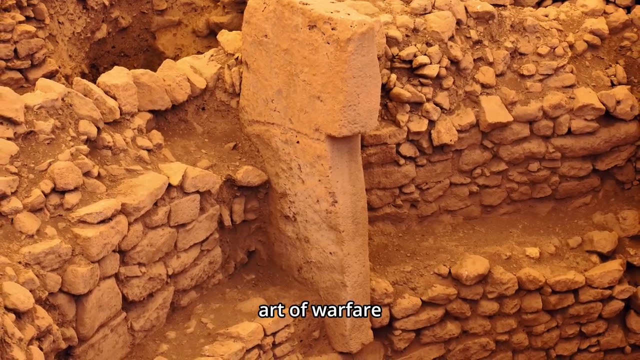 gazing upon the distant stars and conducting surgical procedures with a level of sophistication that transcends their era. Equally perplexing are the depictions of humans coexisting with dinosaurs, apparently domesticating these prehistoric giants for transportation and even employing them in the art of warfare. 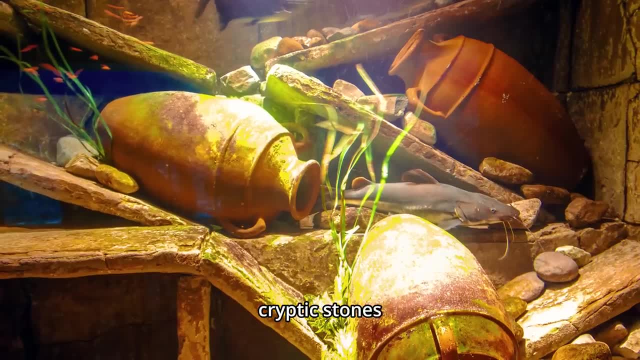 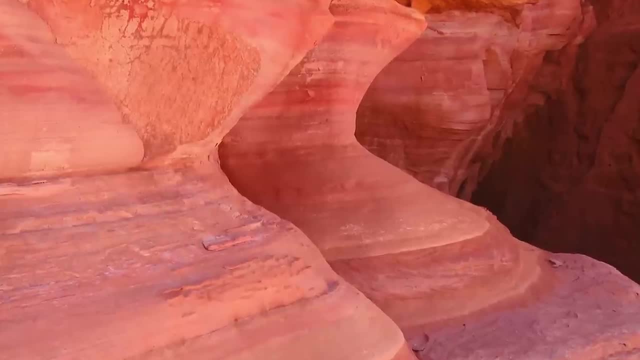 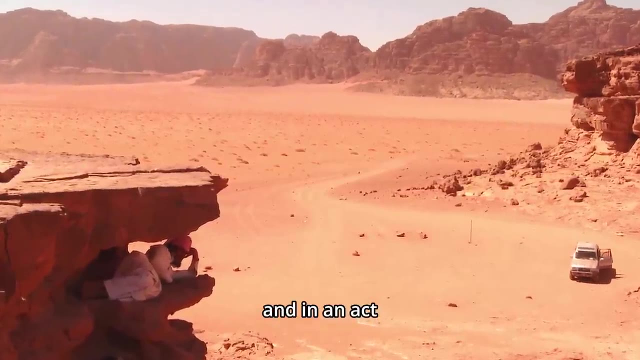 While skepticism surrounds these cryptic stones, with some being identified as modern creations, their authenticity finds a thread of credibility in history. References to these enigmatic artifacts date back to the 16th century, when a Spanish priest encountered them and, in an act of historical preservation, 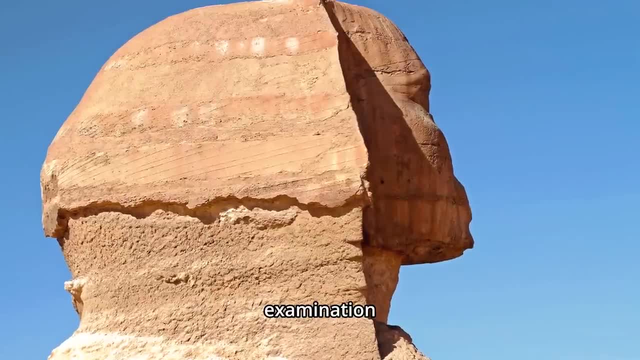 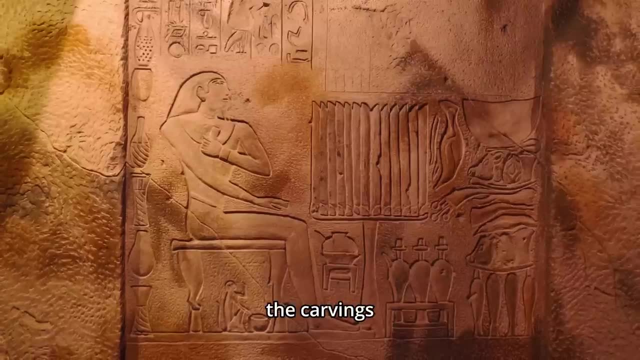 dispatched some of them to Spain for further examination. Furthermore, the study of these stones reveals another layer of mystery. The signs of oxidation on the carvings indicate that many of them have endured the test of time for several centuries. This revelation poses an intriguing conundrum. 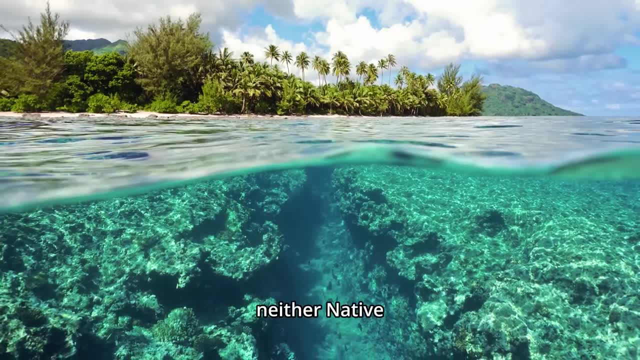 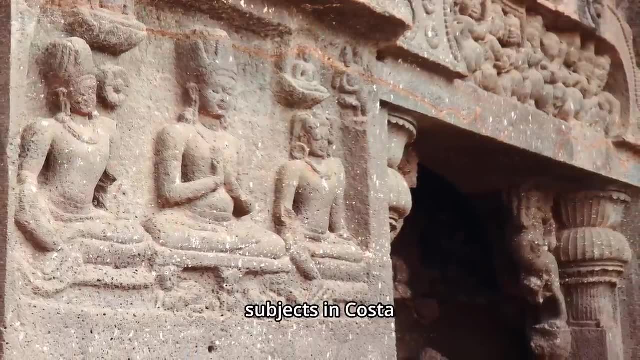 as it implies that these stones may hail from an era when neither Native Americans nor any other known civilization was believed to possess knowledge of such advanced subjects. In Costa Rica, a striking technological enigma emerges in the form of enormous, nearly flawless spherical stones. 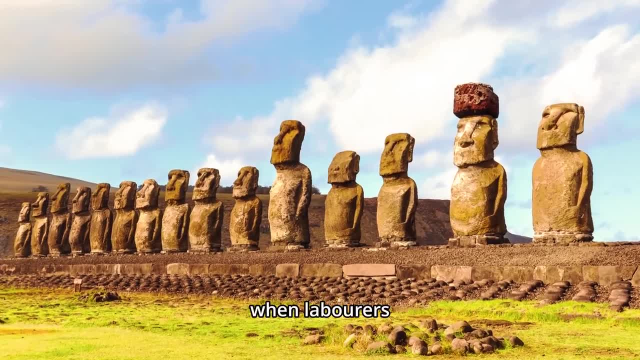 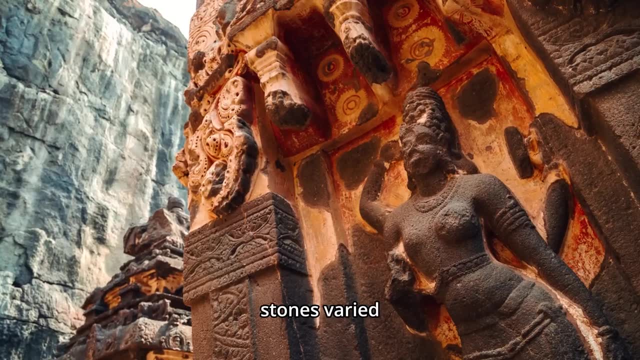 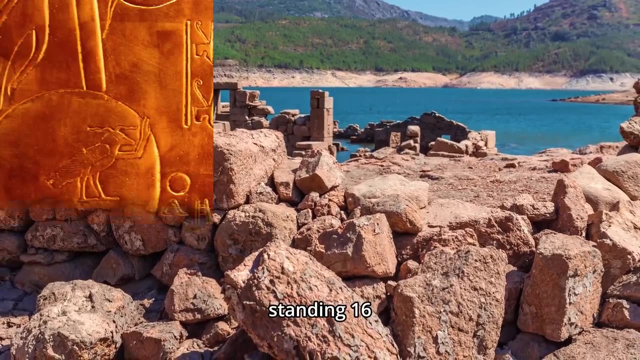 These intriguing sphere stones came to light when laborers of the United Fruit Company were preparing a site for a new banana plantation. The unearthed stones varied in size, with some as small as a few inches in diameter, while the most massive of these sphere stones weighed an astounding 16 tons. 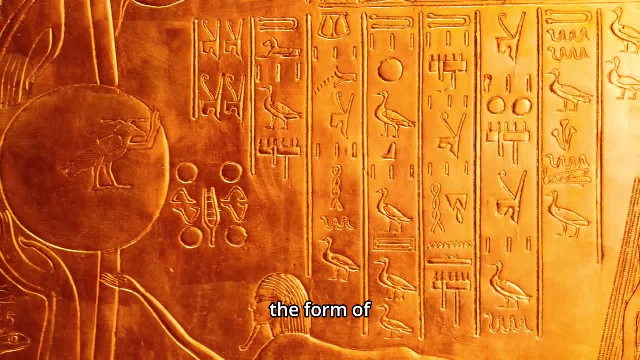 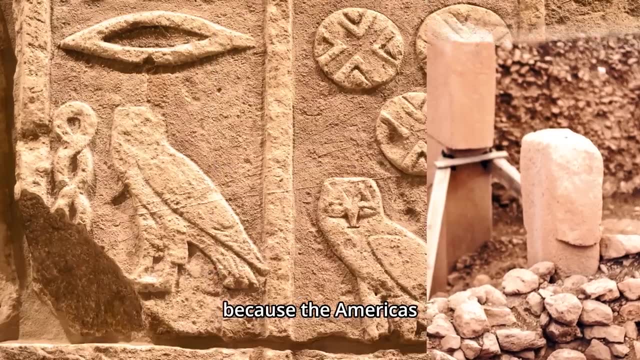 Another conspicuous anachronism presents itself in the form of images of horses and donkeys, frequently depicted in Mexican hieroglyphs. This is perplexing, because the Americas witnessed the extinction of such animals around 12,000 years ago. The widespread presence of standardized mythologies 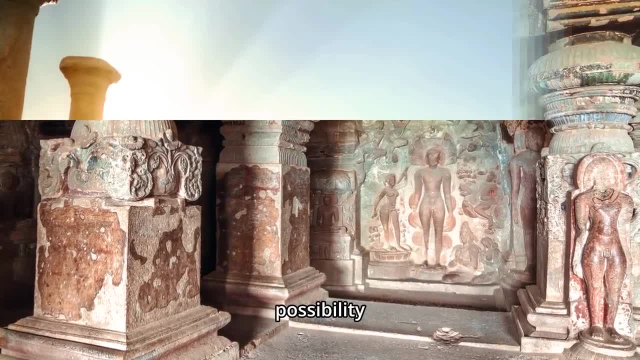 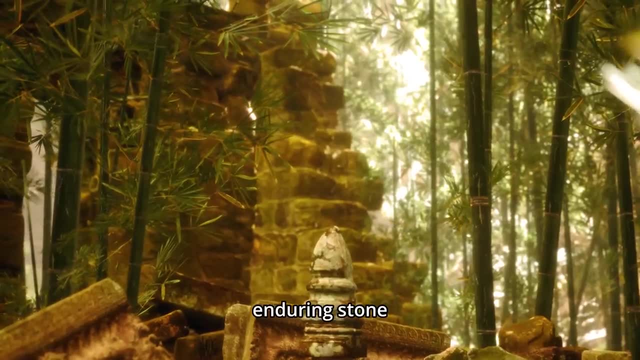 and customs across the globe compels us to consider the possibility of an ancient worldwide civilization that succumbed to cataclysms but left its legacy in both narratives and enduring stone structures. Chapter IV: While early humans toiled discovering fire and inventing the wheel, 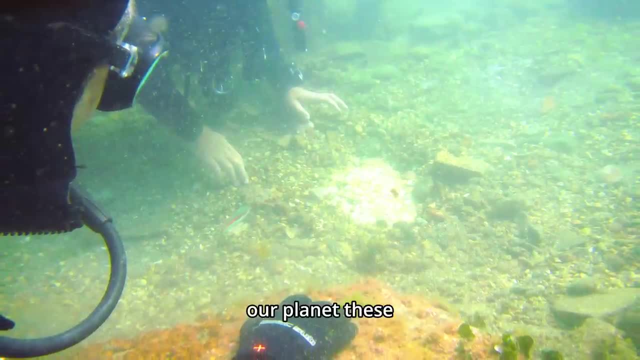 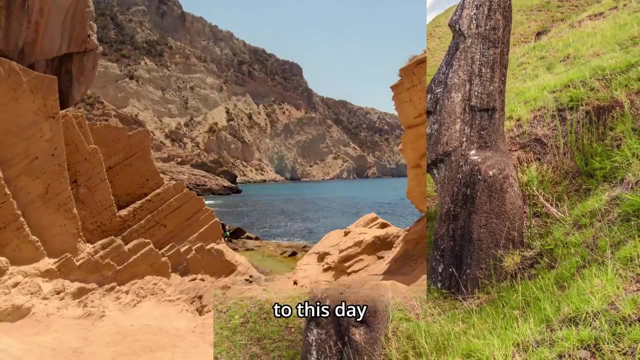 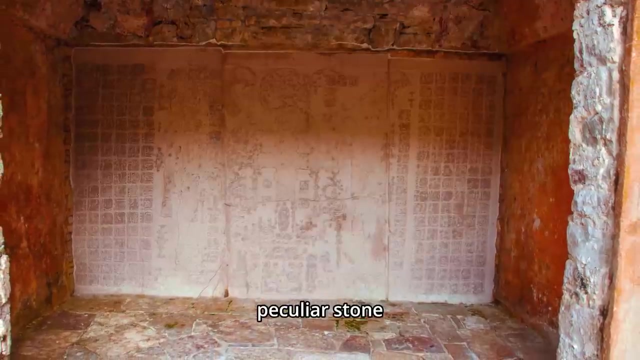 a remarkably advanced civilization was already thriving on our planet. These enigmatic beings meticulously constructed colossal stone cities, some of which endure to this day. With methodical precision, they raised immense earthen mounds across the planet's surface. Peculiar stone and metal artifacts were dispersed across every continent. 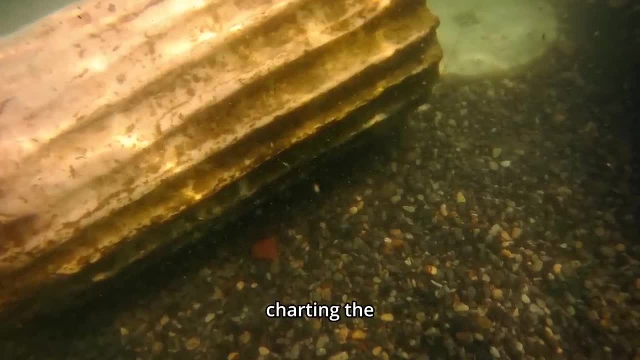 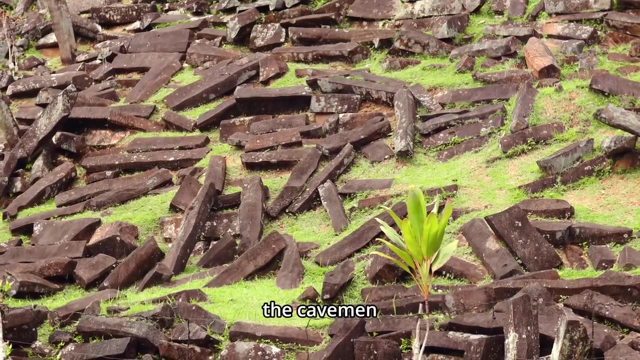 and they fearlessly traversed vast oceans, charting the entire globe. Then, without a trace, they vanished into the annals of history. The cavemen, inheritors of the earth viewed the ancient cities as hallowed ground As centuries passed. 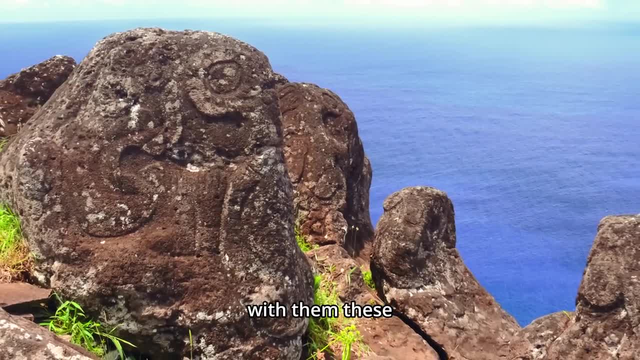 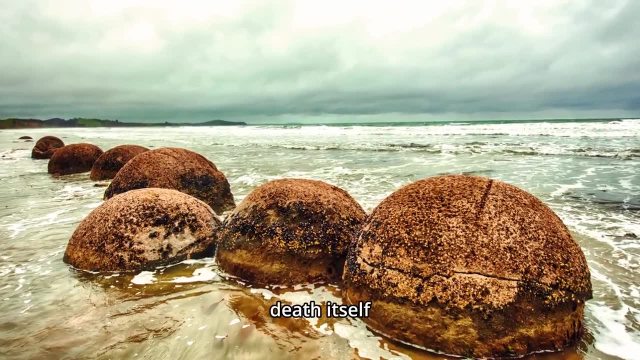 they grew aware of the presence of another enigmatic life form coexisting with them. These beings seemed to possess the elusive power of invisibility and held dominion over life and death itself. The cavemen devised names for these ethereal entities, elevating them to the status of deities. 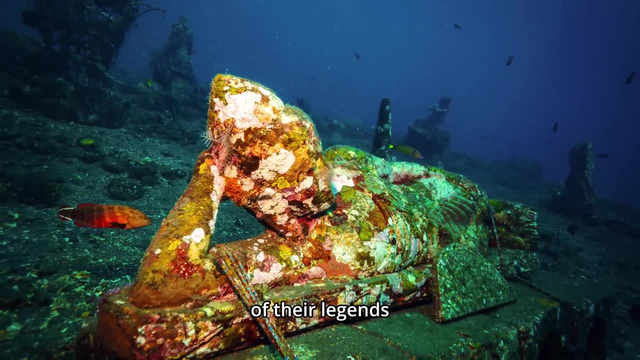 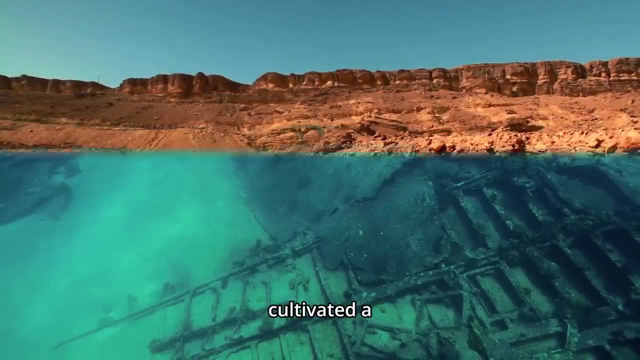 They etched the signs of this hidden realm into the tapestry of their legends and myths, preserving them through the passage of generations. Over time, these early humans cultivated a form of science rooted in their interpretations of these supernatural manifestations As the ages passed. 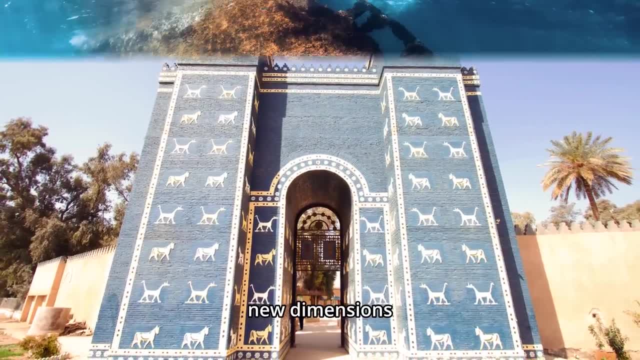 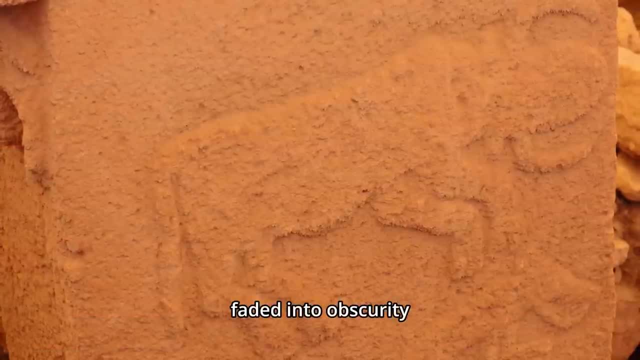 their scientific understandings evolved, taking on new dimensions. The original inhabitants of the earth, the builders of those awe-inspiring cities, faded into obscurity. their memory lost to the annals of history. However, as humanity expanded its reach across the planet, 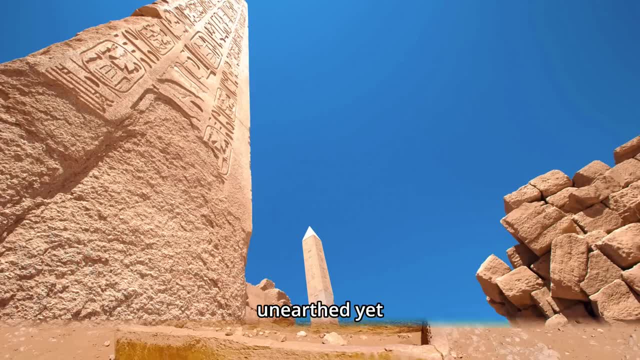 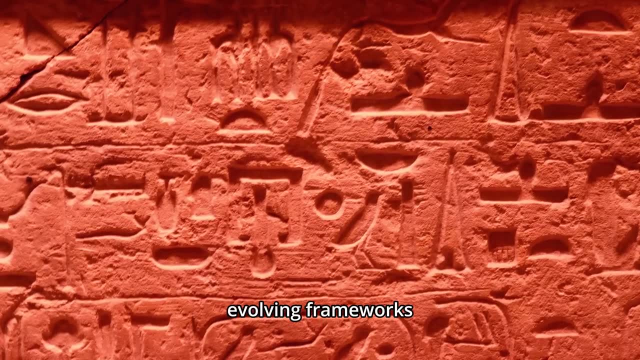 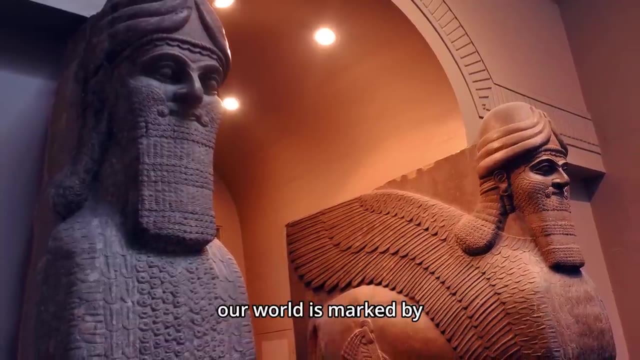 the vestiges of these enigmatic elders were once again unearthed. Yet the prevailing sciences of the modern era struggled to assimilate these traces into their evolving frameworks. Consequently, this evidence was often dismissed or overlooked. As a result, our world is marked by two distinct histories. 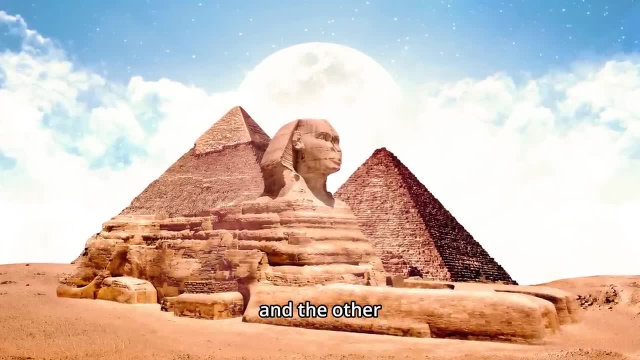 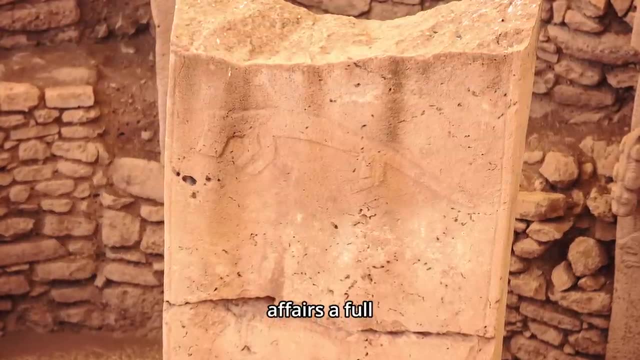 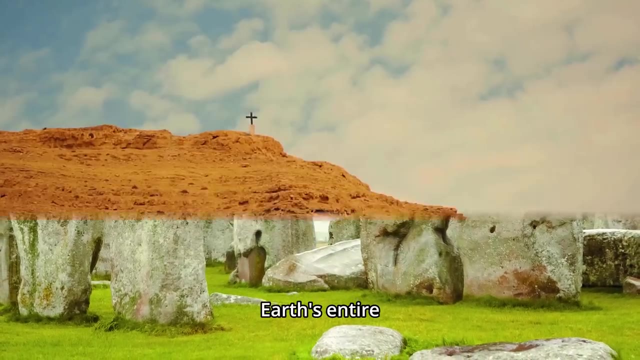 one the familiar narrative known to the majority of people, and the other the forgotten history of a profoundly ancient civilization that once held sway over human affairs. A full ten millennia ago, this long-forgotten civilization undertook the extraordinary task of intricately mapping the earth's entire expanse. 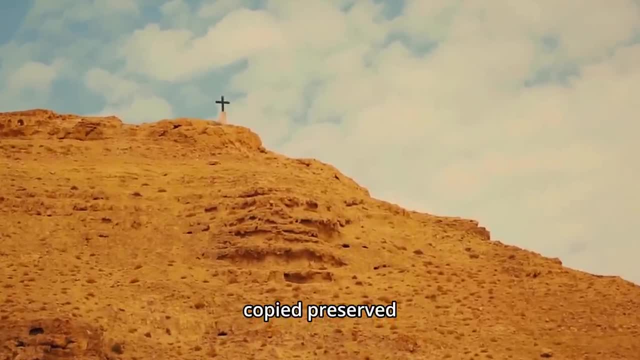 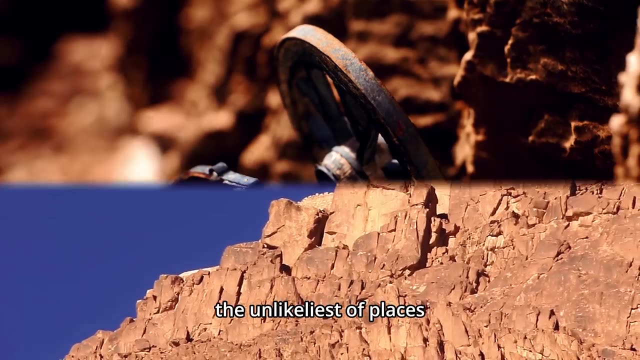 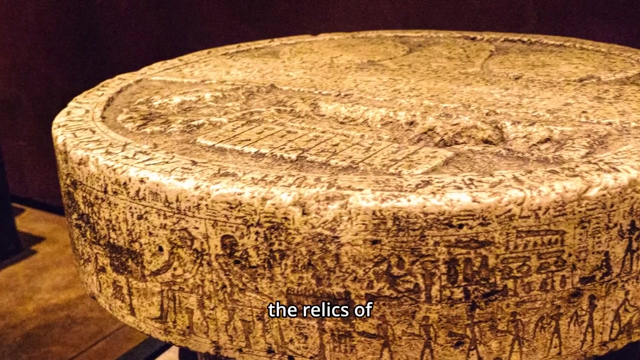 These remarkable maps were meticulously copied, preserved and transmitted across the ages. Remarkably, copies of these maps resurfaced in the unlikeliest of places: the Library of Congress. They are famously known as the Piri Rice Maps, initially found amidst the relics of the ancient Imperial Palace of Constantinople in 1929. 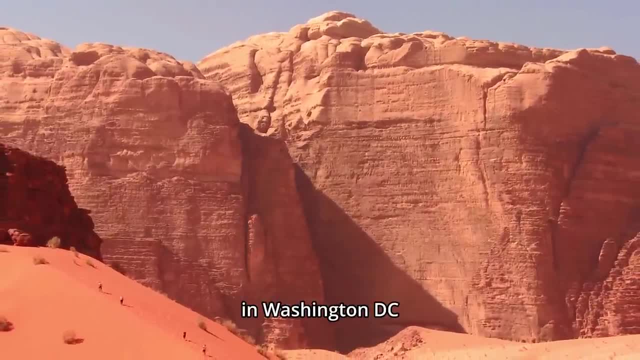 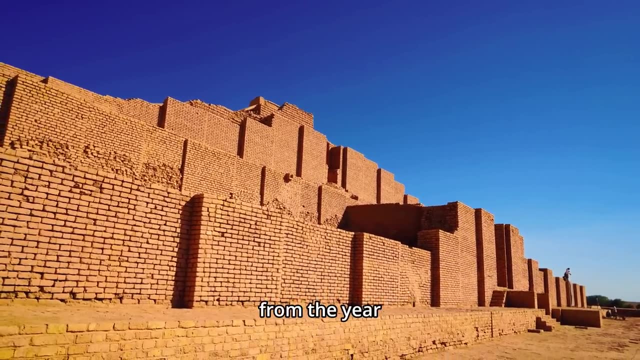 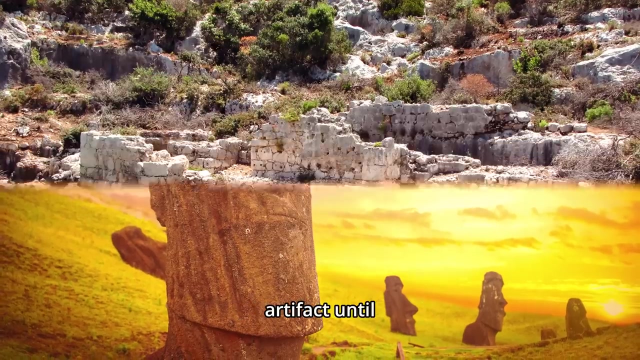 Eventually, they made their way to the archives in Washington DC, serving as a captivating link to this enigmatic past. These maps, originally from the year 1513, initially appeared as a perplexing jumble of the ancient world. They remained a puzzling artifact until the arrival of Captain Mallory. 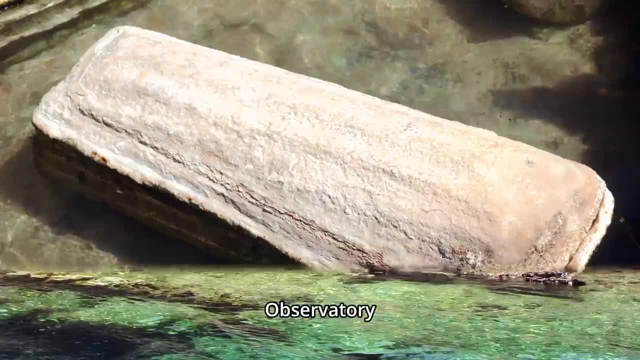 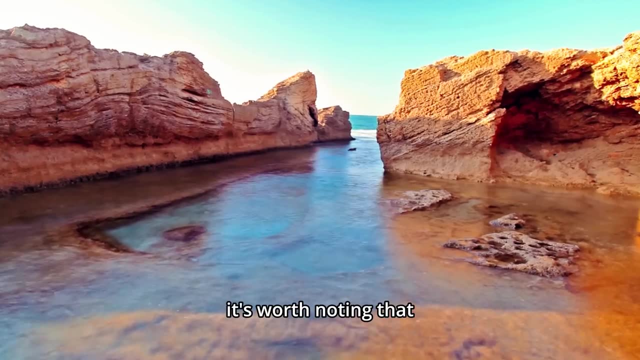 Collaborating with the US Hydrographic Office and the Western Observatory of Boston, he introduced a grid system that brought these maps into startling clarity. It's worth noting that the Mercator grid system we know today wasn't developed until 1559,. 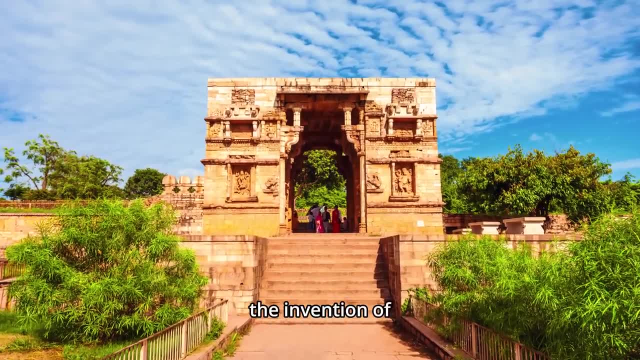 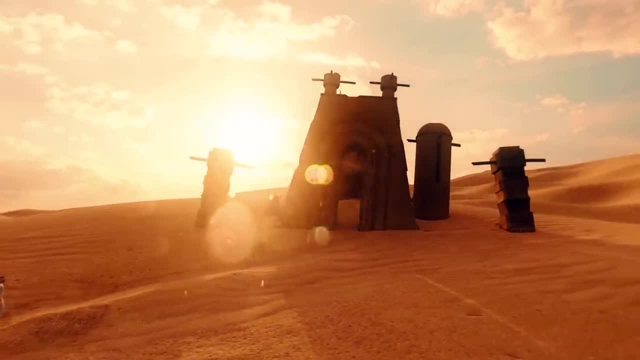 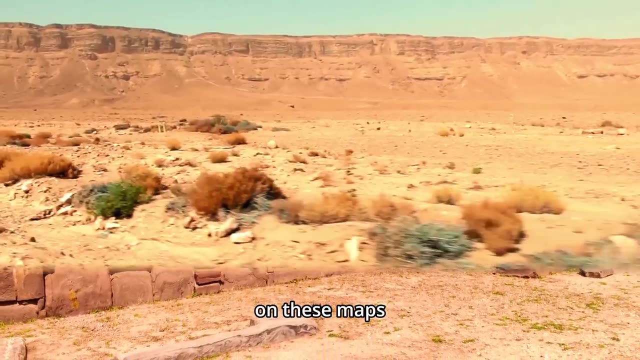 and it wasn't perfected until 1760, with the invention of the chronometer. So the ancient cartographers were compelled to devise their own unique method. Once Captain Mallory unraveled this method, the revelations were almost beyond belief. The level of detail on these maps was nothing short of astonishing. 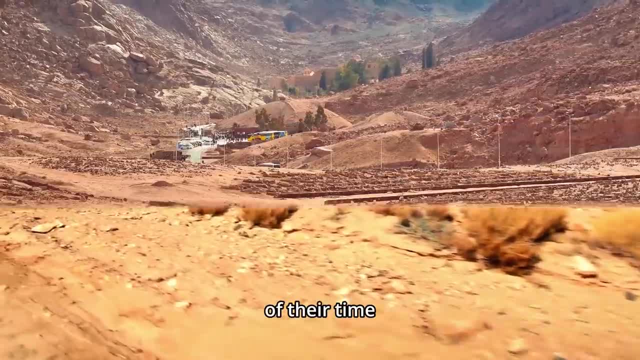 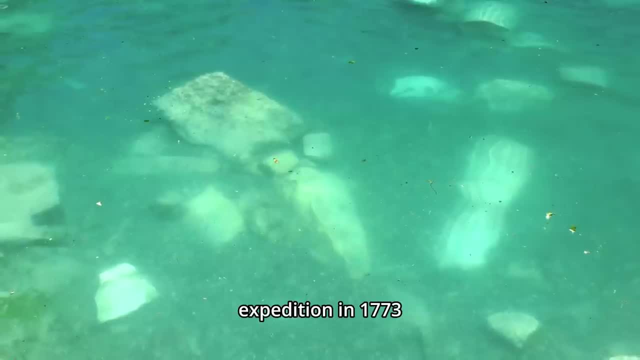 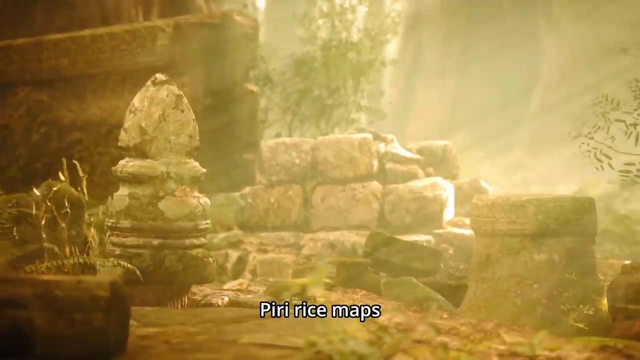 rivaling the accuracy of the most contemporary charts of their time. Take Antarctica, for example. It remained undiscovered until Captain Cook's expedition in 1773, and comprehensive exploration only occurred in the 1950s. However, the Piri Rice Maps depict the frozen continent with remarkable precision. 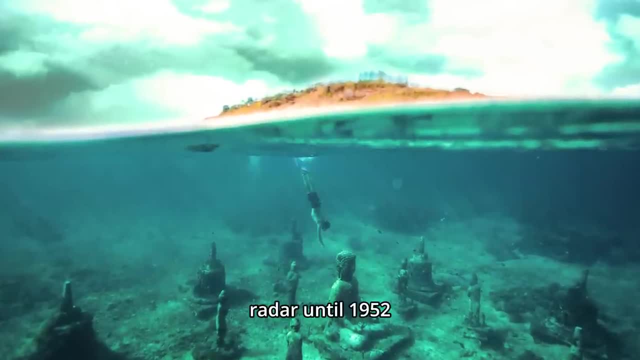 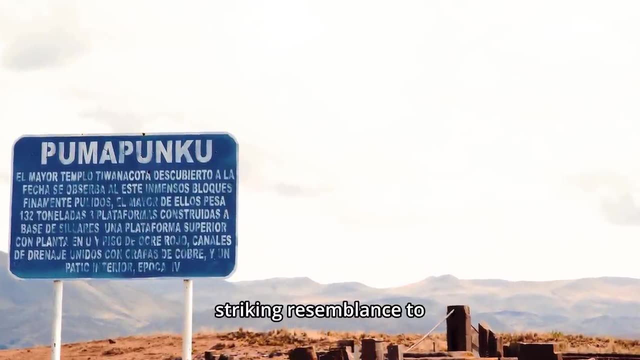 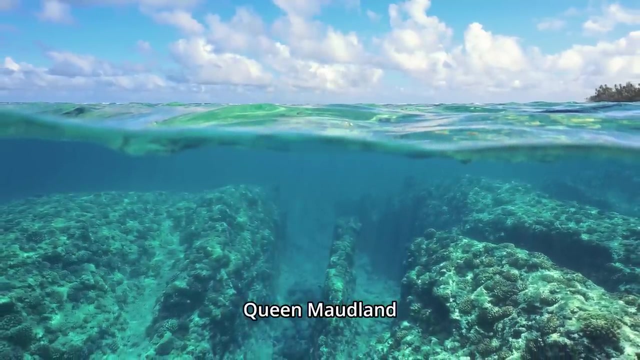 including mountain ranges that weren't even on our radar until 1952.. What's truly remarkable is that a portion of the coastline on the Piri Rice Maps bore a striking resemblance to the coast of Queen Maud Land, an area in Antarctica. The puzzling aspect is that Queen Maud Land had been concealed beneath a thick ice sheet for countless centuries. 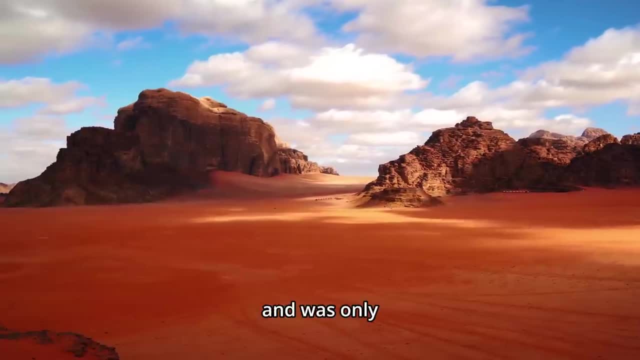 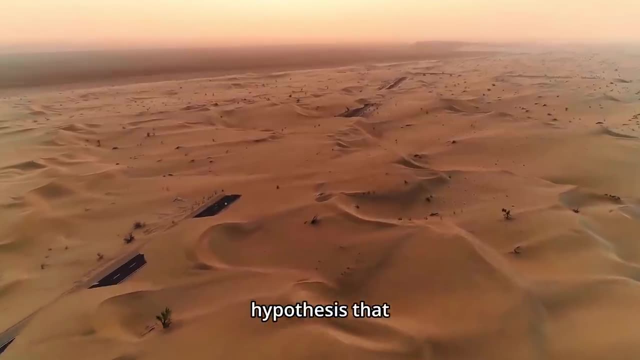 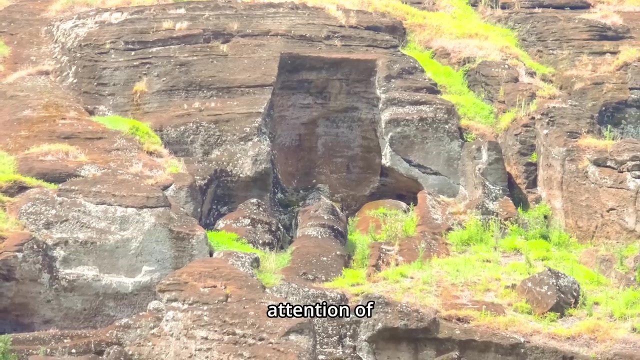 Its true shape was a mystery to the contemporary world and was only unveiled by modern mapmakers using advanced seismographic technology. Mallory's findings prompted the hypothesis that the original maps must have been created prior to the Ice Age. The remarkable discoveries captured the attention of Professor Charles Hapgood, a science historian. 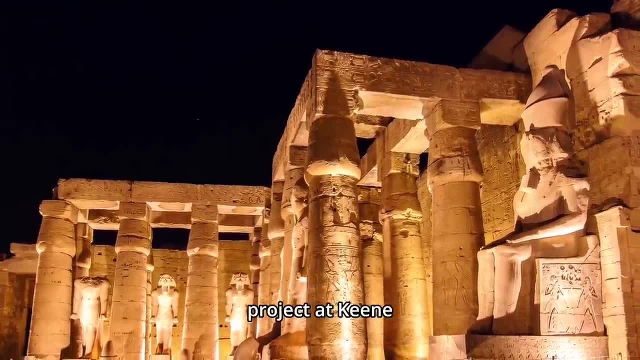 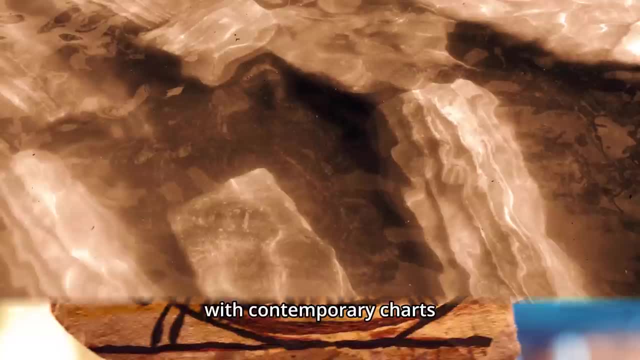 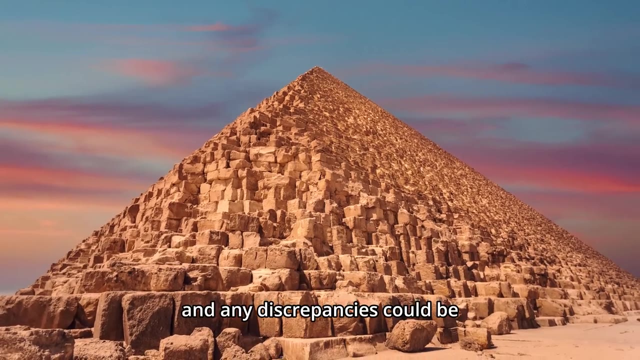 Hapgood transformed these maps into a class study project at Keene State College. His students embarked on a meticulous comparison of each map detail with contemporary charts. Astonishingly, they found that the ancient maps were rarely more than five degrees off, and any discrepancies could be attributed to land shifts that transpired after the original maps were crafted. 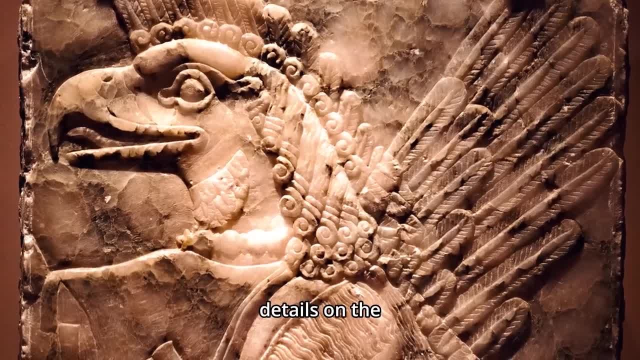 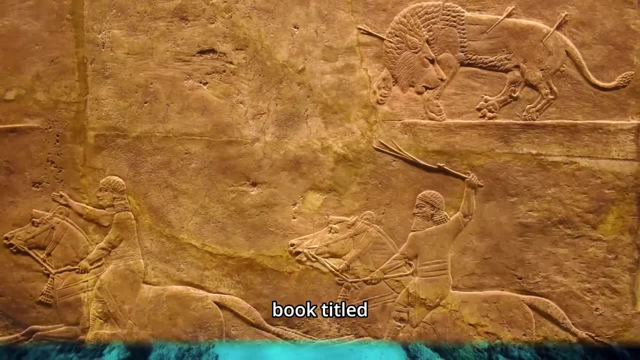 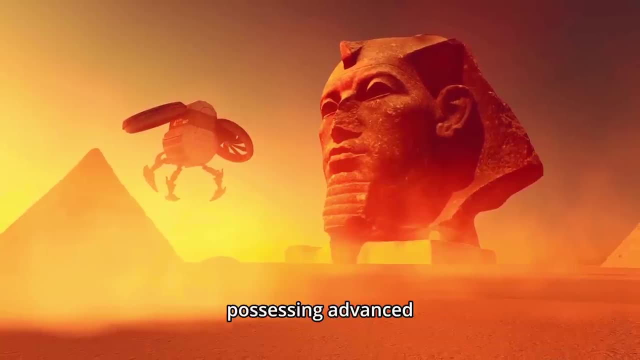 Hapgood's extensive research revealed that numerous details on the ancient maps aligned precisely with modern surveys. The findings were published in his groundbreaking book titled Maps of the Ancient Sea Kings. This work proposed the existence of a global civilization from antiquity, possessing advanced technology. 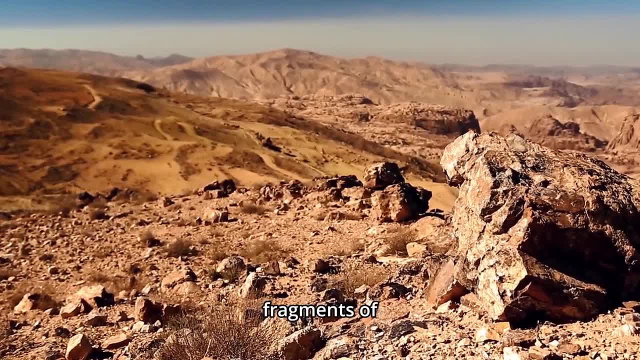 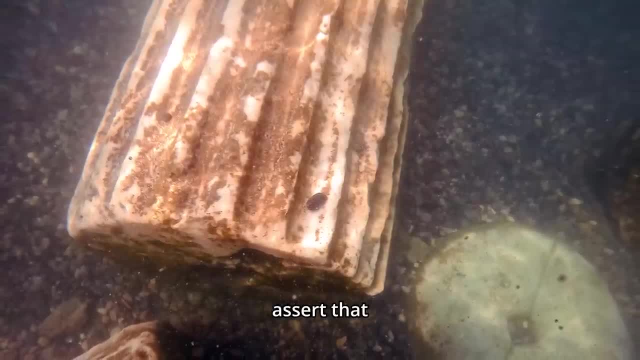 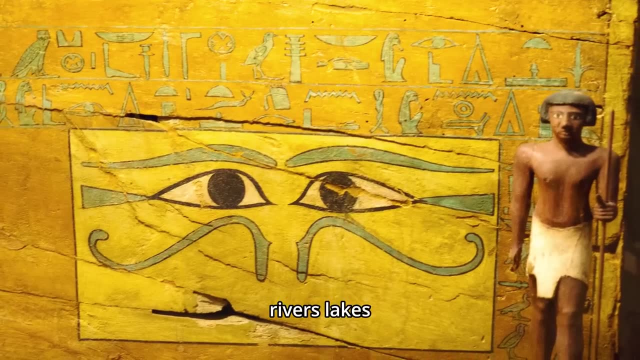 While this civilization ultimately met its demise, fragments of its knowledge endured and were eventually preserved on these enigmatic maps. Both Hapgood and Graham Hancock assert that the depiction of the Antarctic continent on these ancient maps is remarkably accurate. The presence of rivers, lakes and mountains suggests that this cartographic model may date back as far as 15,000 years ago. 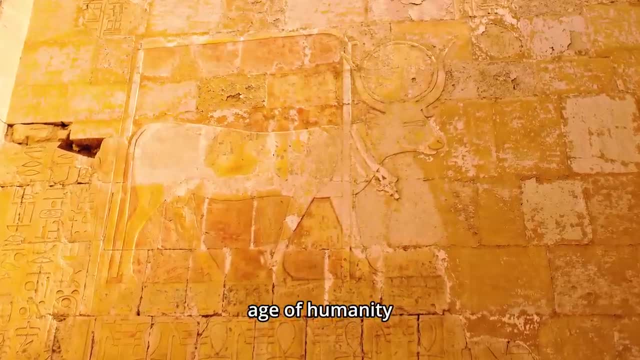 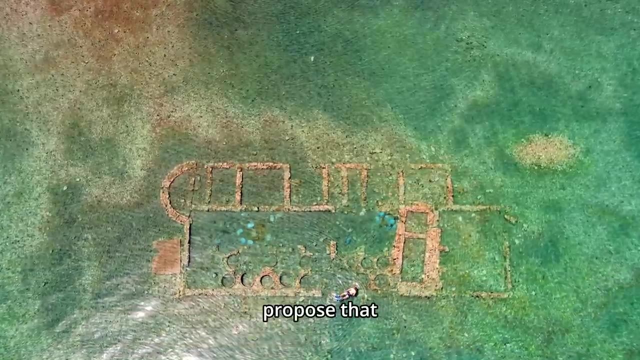 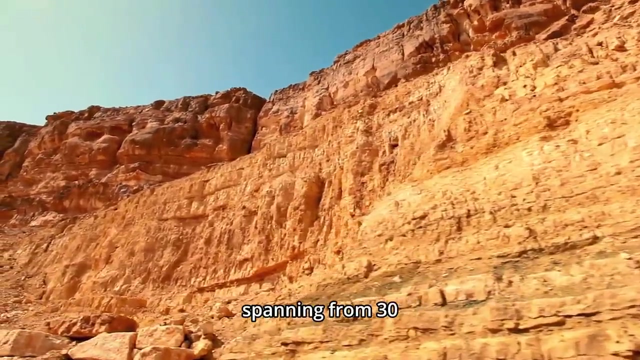 Contemporary scientists remain divided on the age of humanity, with each passing year unveiling new discoveries and fueling ongoing controversies. Some researchers propose that our existence might stretch back as far as half a million years, while others favor a more conservative estimate spanning from 30,000 to 70,000 years. 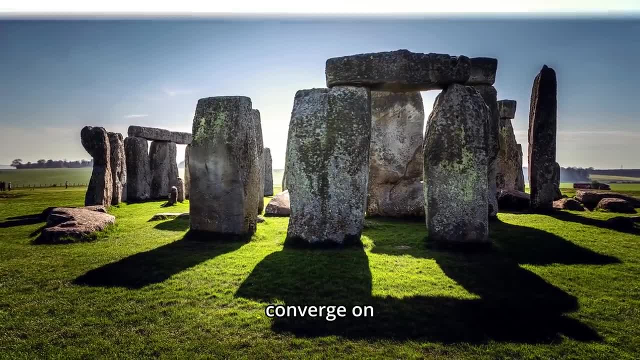 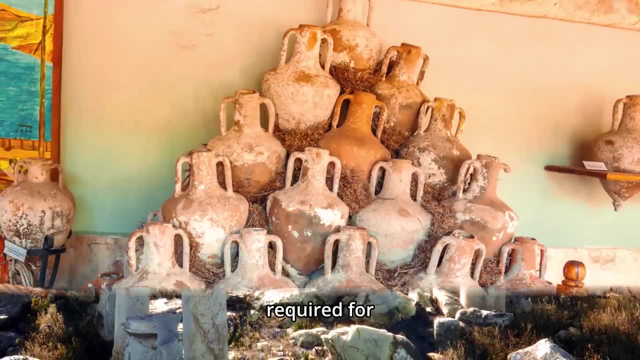 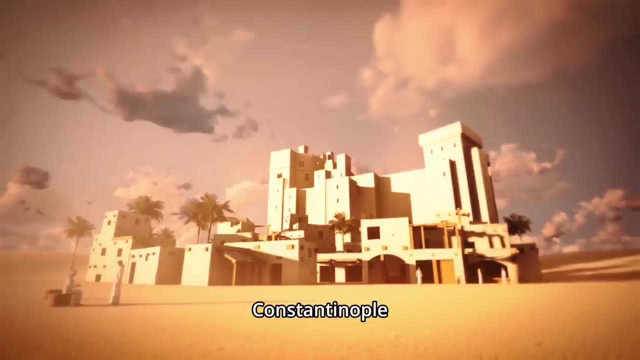 Nevertheless, these conflicting theories seem to converge on one assumption: Our ancestors around 10,000 years ago were considered primitive and lacking the sophistication required for seafaring and comprehensive earth mapping. Creating the maps in 1929, when they were discovered in Constantinople. 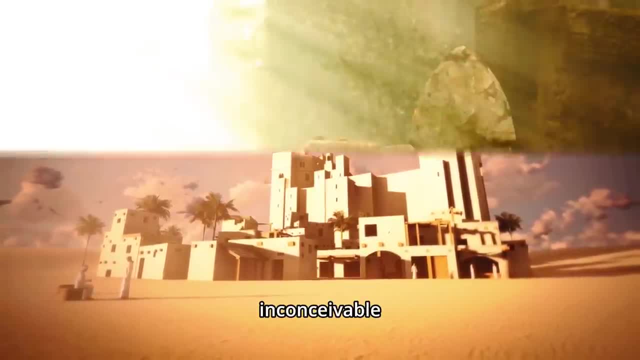 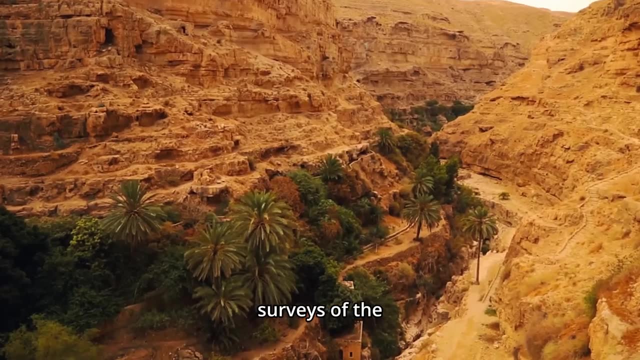 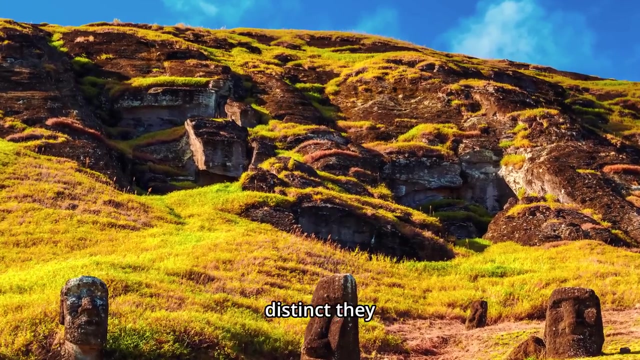 was deemed an impossibility, and even more inconceivable would have been the idea of hoaxing them in 1513.. Could it be plausible that someone might have conducted surveys of the earth before the ice age? However, the approach of contemporary scientists when faced with such findings is distinct. 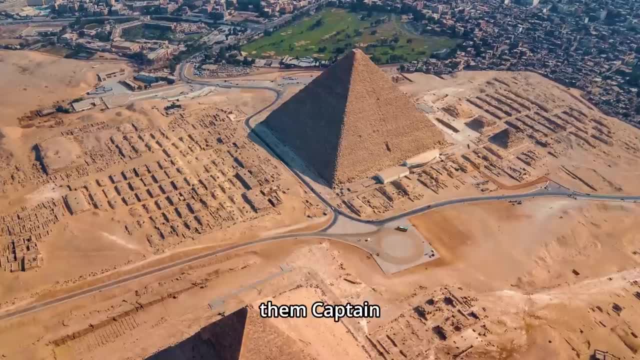 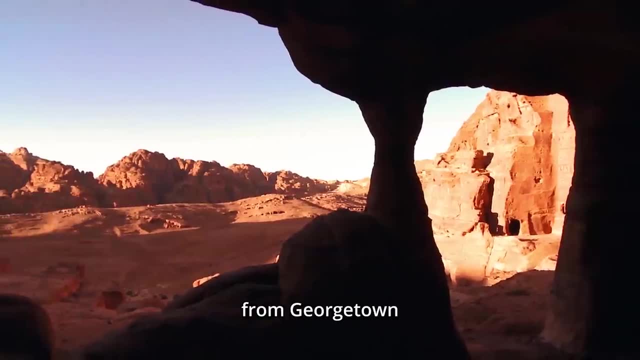 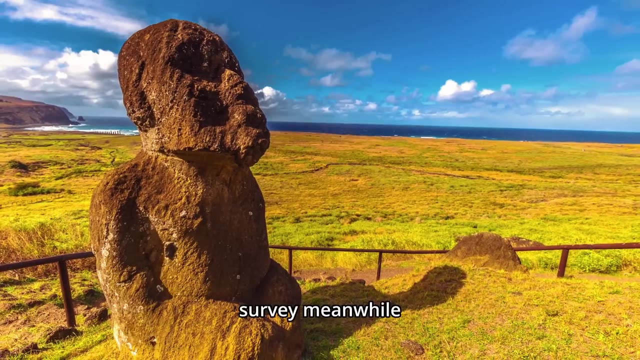 They often consign them to the museum vaults and deliberately choose to overlook them. Captain Mallory made waves when he unveiled his findings regarding the Piri Rice maps during a broadcast from Georgetown University. He ventured to suggest that these maps could have been the outcome of an aerial survey. 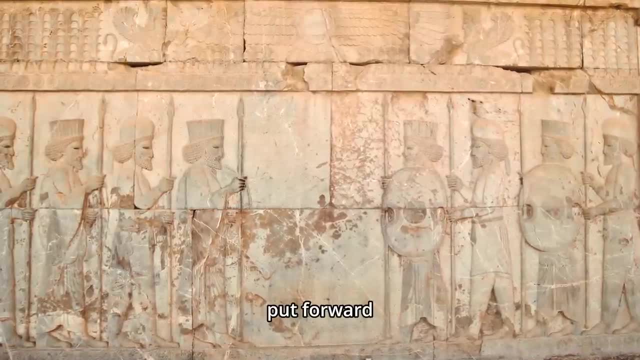 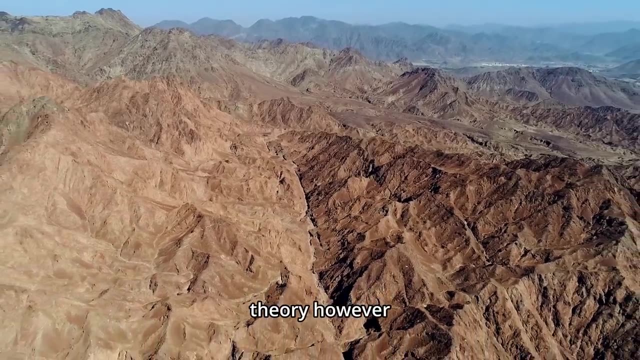 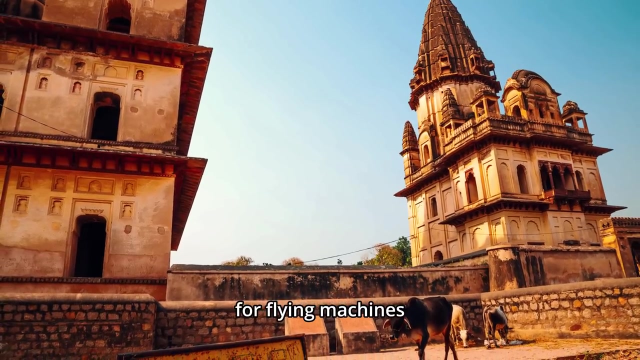 Meanwhile, Professor Hapgood more cautiously put forward the idea that they might be attributed to a lost maritime civilization. The aerial survey theory, however, would hinge on the existence of an immensely advanced technological society. In addition to the necessity for flying machines, photography would have been an essential tool for such a survey. 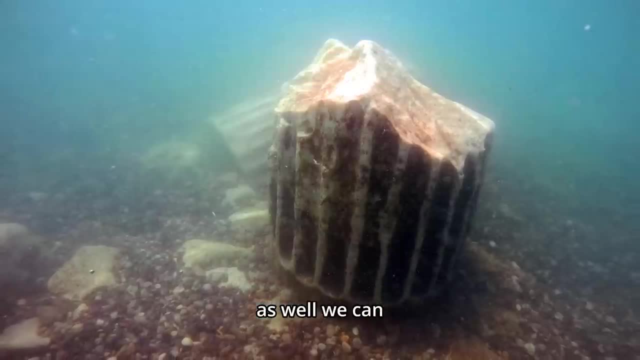 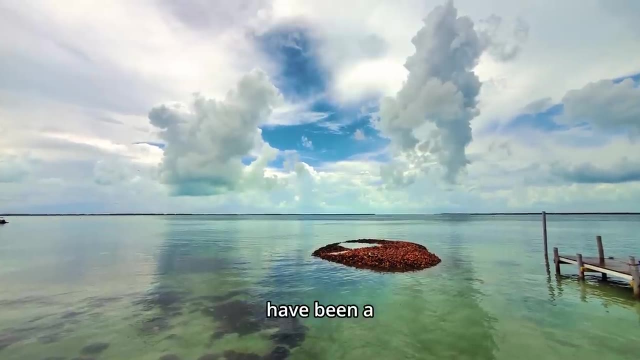 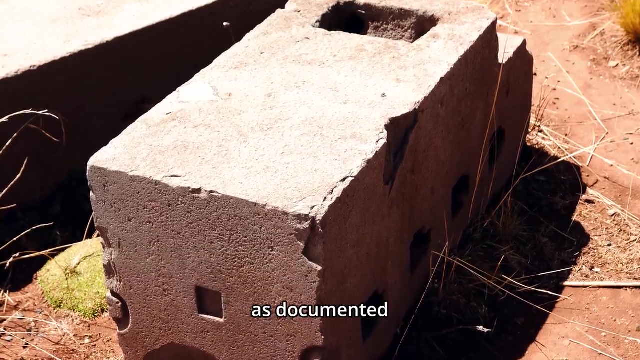 One might wonder, did the elders possess cameras as well? We can establish two pivotal facts. One: unusual objects in the skies above our planet have been a constant presence. Early humans witnessed them and they have continued to be observed throughout history, as documented in sources like the Bible. 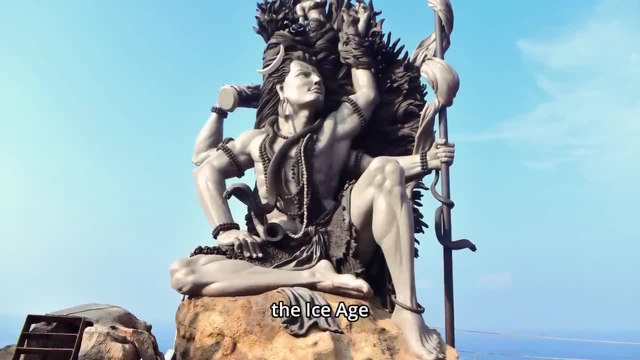 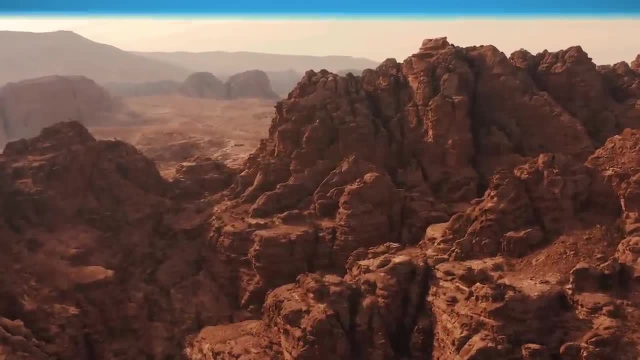 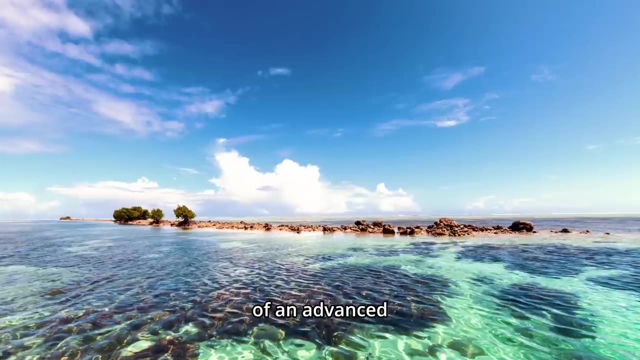 Two, the earth was mapped prior to the ice age. However, the identity of those responsible for these maps and the methods they employed remain shrouded in mystery. If indeed the Piri Rice maps originated from an aerial survey, it could imply the existence of an advanced civilization in the Americas or the Pacific. 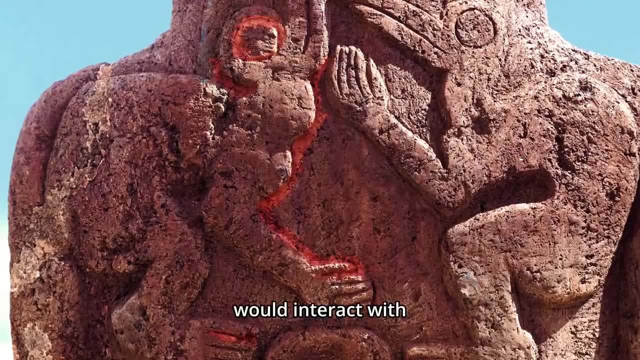 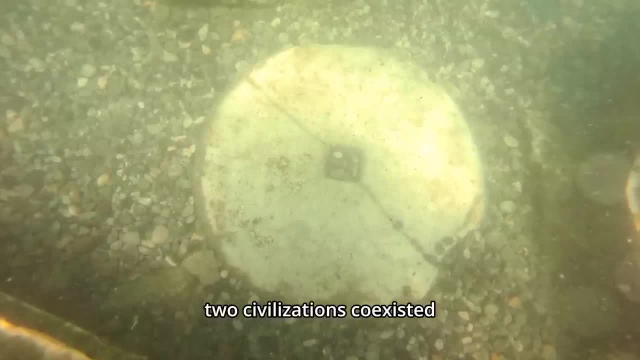 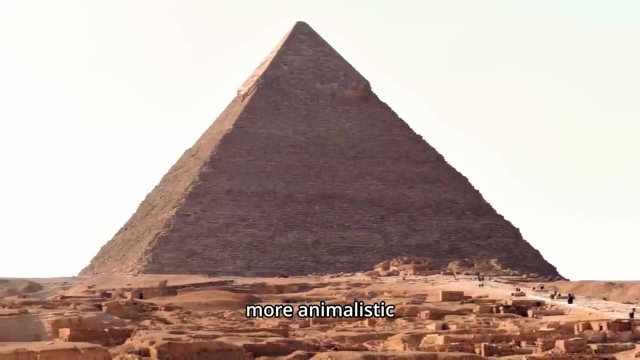 From time to time, the highly advanced civilization would interact with or pass over the cavemen, if not merely coexist in parallel. It's plausible that two civilizations coexisted simultaneously, one considerably advanced and consciously detached from the other, resembling a more animalistic existence in the caves. 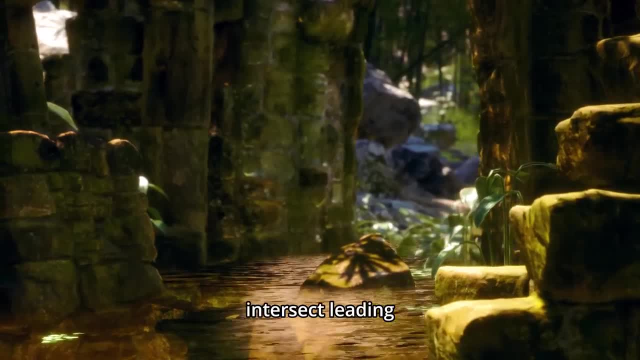 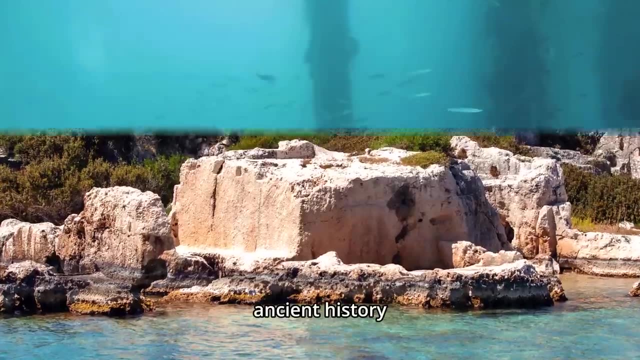 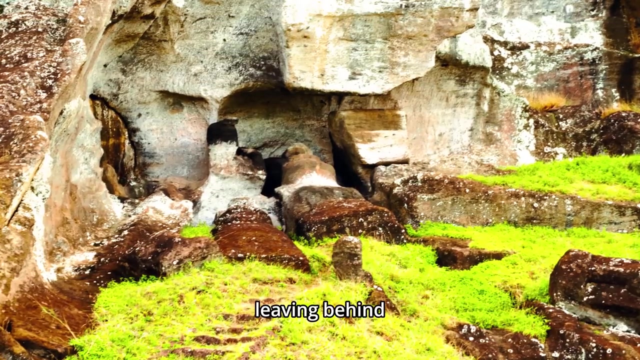 The paths of these two cultures would occasionally intersect, leading to a variety of influences, from the more advanced to the less advanced group. At a certain juncture in ancient history, the higher civilization may have encountered a catastrophic upheaval or found another means of departure, leaving behind scant evidence of their existence. 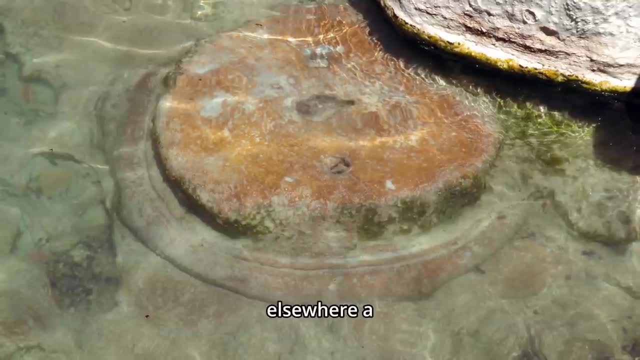 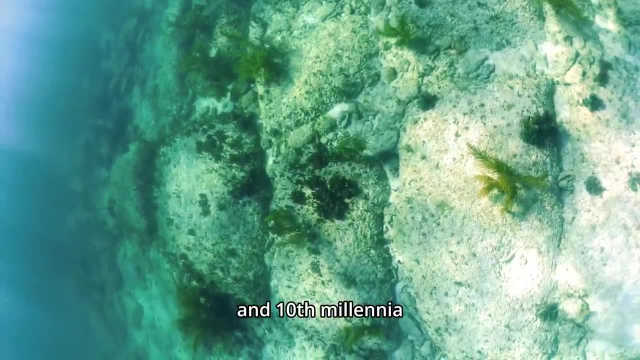 As it has been extensively illustrated elsewhere, a substantial body of evidence suggests that during the final stages of the last ice age, particularly in the 11th and 10th millennia BC, our world experienced a series of dramatic climatic shifts and profound geological disturbances. 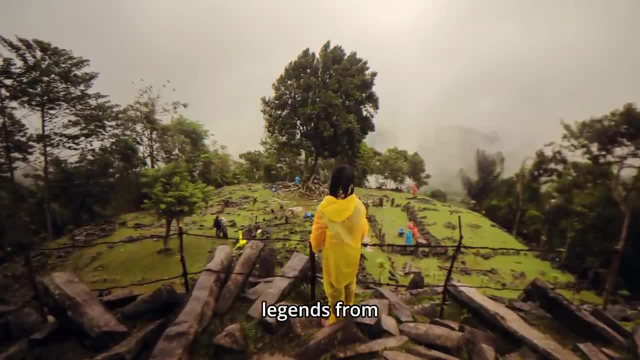 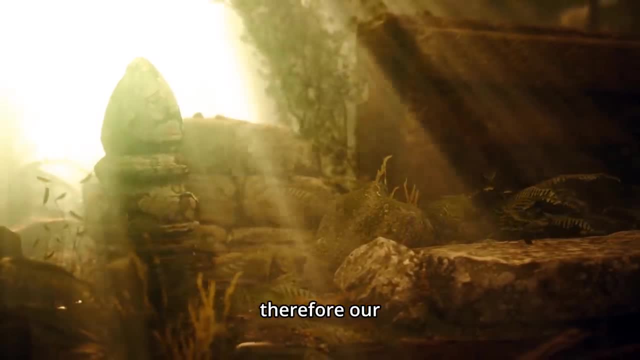 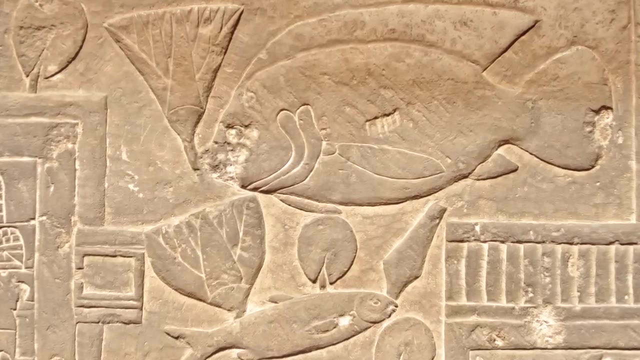 These cataclysmic occurrences seemed to find their place in legends from various cultures around the world, depicting them in vibrant and occasionally symbolic narratives. Therefore, our entire understanding of this super-civilization hinges on the observations and interpretations of early humans. Our sole evidence consists of the tenuous interactions that occurred, the traces of the superculture's impact on the subculture. 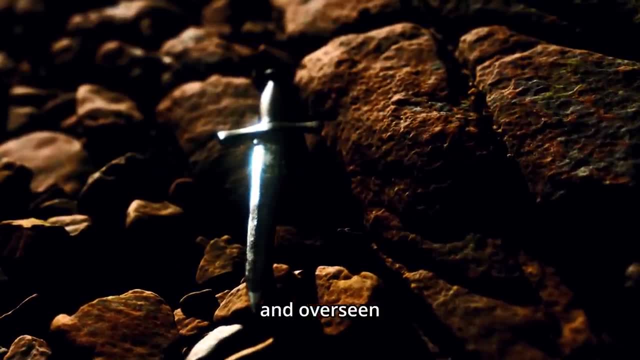 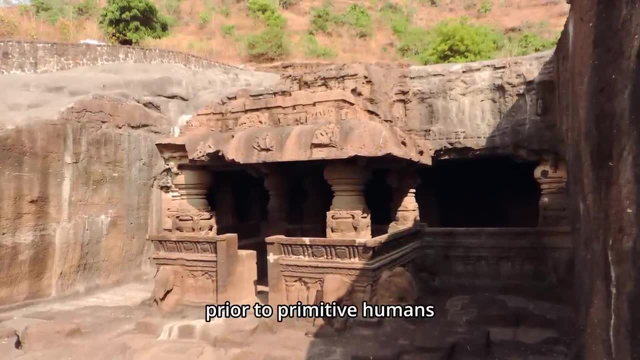 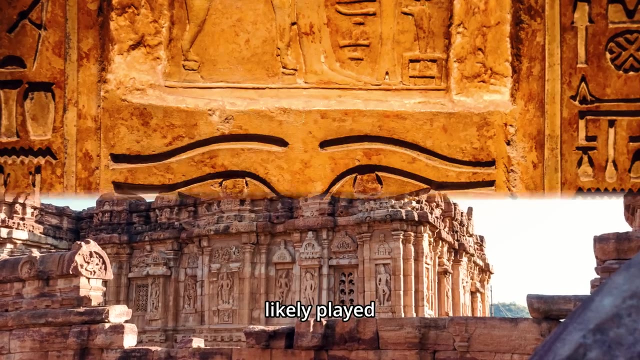 Primitive humans were deeply influenced and overseen by this superculture. There are even suggestions that individuals from the superculture may have arrived prior to primitive humans, assuming roles as rulers and godlike figures to guide their early development. Such arrivals likely played a significant role in shaping the world. 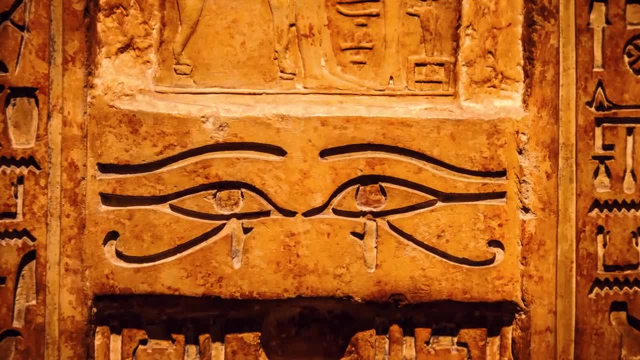 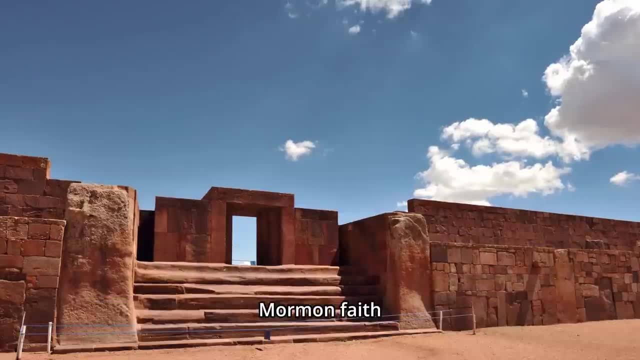 The creation of the superculture from the ancient. ancient world has been the basis of many of humanity's earliest religious beliefs. 2,500,000 inhabitants of our world adhere to the teachings of the Book of Mormon, a sacred text in the Mormon faith that claims to chronicle ancient life in North America thousands of years ago. 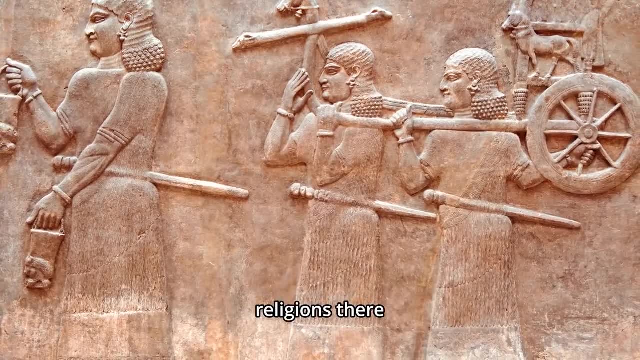 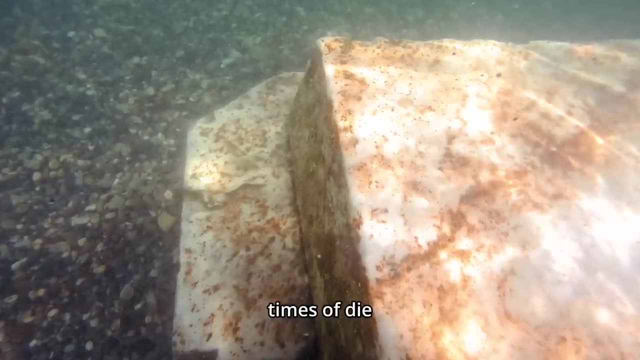 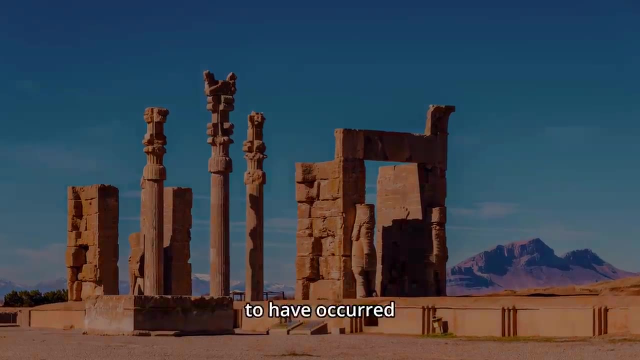 In the sacred writings of numerous cultures and religions, there are countless narratives recounting occasions when a mysterious and benevolent group extended assistance to humanity in times of dire necessity. Take, for instance, the intriguing introduction of the compass, which is believed to have occurred in those long-forgotten North American lands. 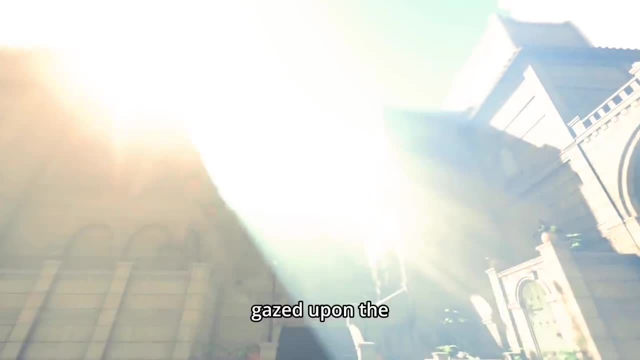 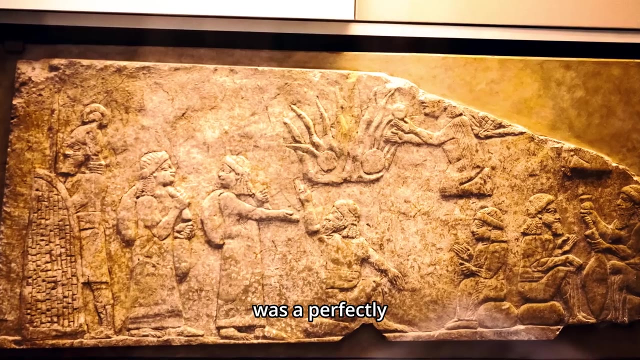 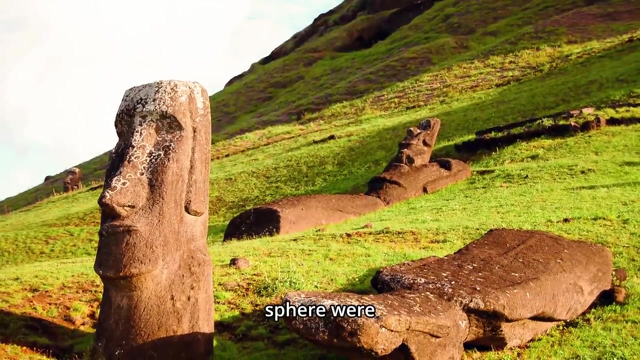 One morning, as my father emerged from his tent and gazed upon the world, he was utterly astounded to discover a remarkable object resting on the ground before him. It was a perfectly round sphere meticulously crafted from fine brass. Encased within this enigmatic sphere were two spindles, and one of them to our profound wonderment. 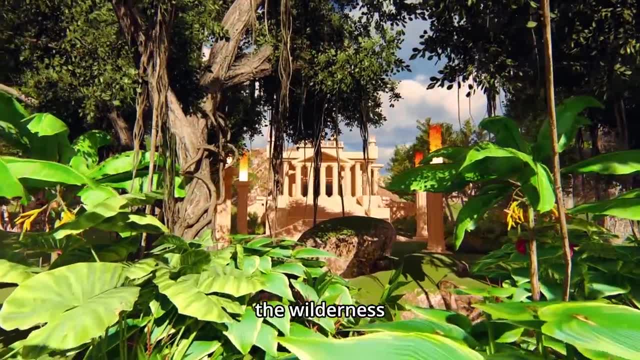 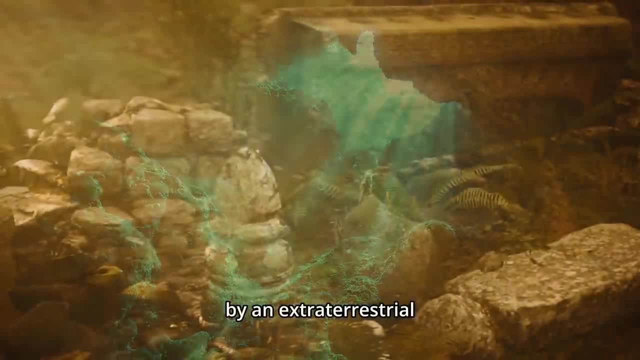 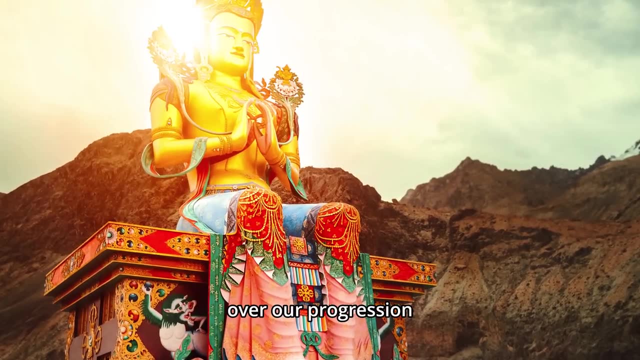 consistently indicated the path we ought to take as we journeyed through the wilderness. A prevalent theory that circulates suggests that humankind might have been originally introduced to this planet by an extraterrestrial collective. This enigmatic group, it is conjectured, has maintained a distant vigil over our progression throughout the ages. 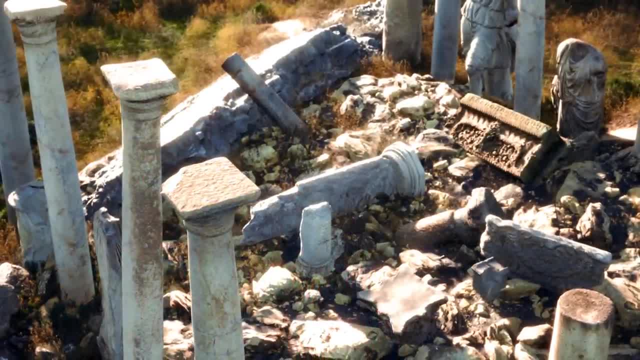 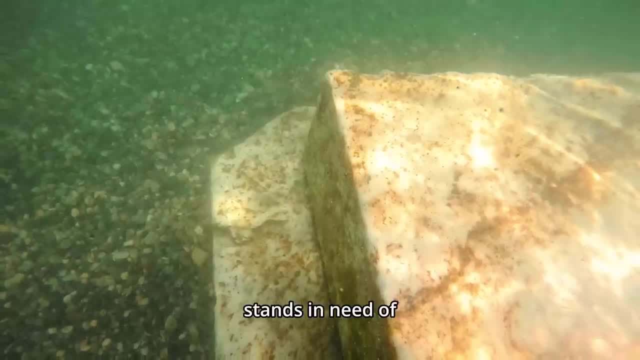 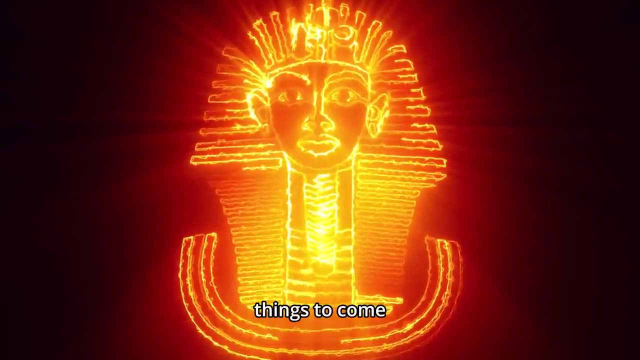 If this hypothesis held any validity, one might argue that their oversight has, in recent centuries, left much to be desired. Our species stands in need of far greater assistance than it has hitherto received. In H G Wells' visionary work Things to Come, a vision unfolds of a planet ravaged by war. 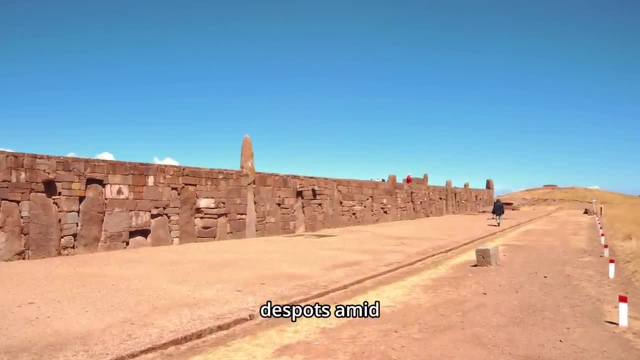 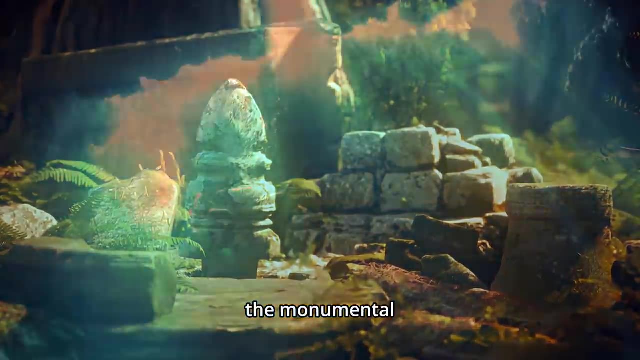 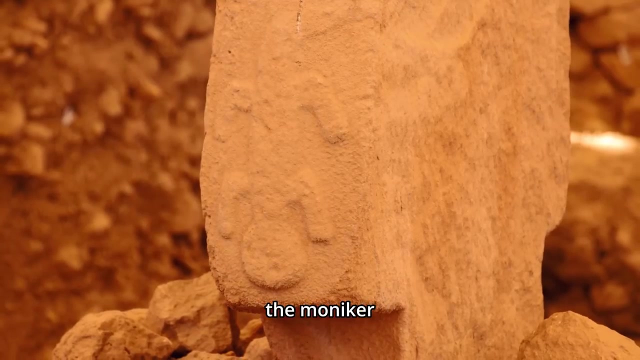 fragmented into adversarial factions led by despots. Amid this chaos, a small group of surviving scientists and intellectuals unite, embarking on the monumental endeavor of reconstructing civilization. The journey involves traveling across the globe and they adopt the moniker Wings Over the World. 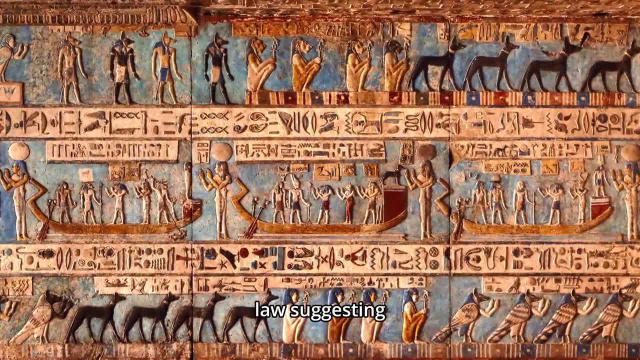 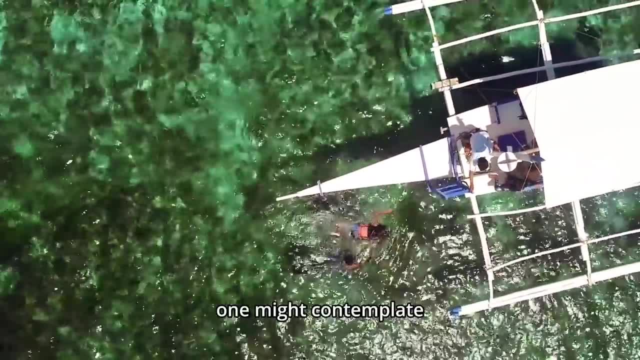 It's a concept that resonates with elements found in UFO lore, suggesting the existence of an enigmatic organization akin to WoW that has endured through time. One might contemplate the possibility that a member of such a group once bequeathed the wheel to a primitive human. 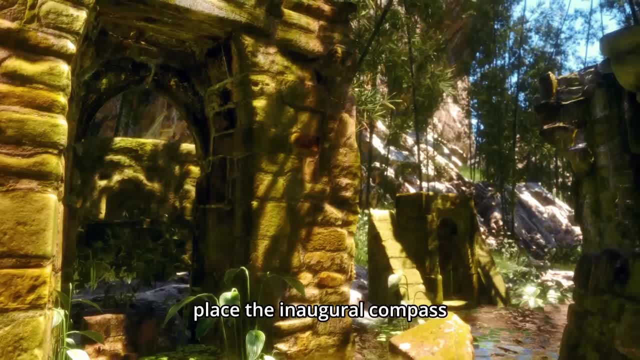 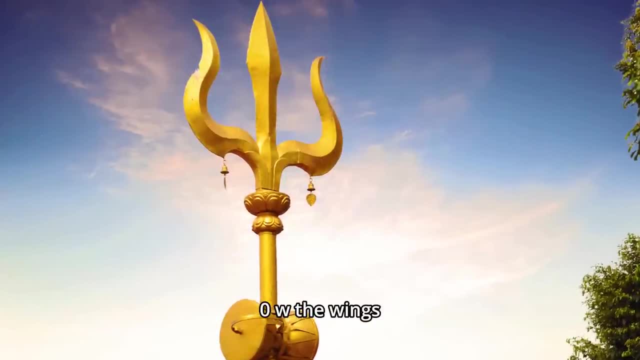 just as an unidentified benefactor purportedly placed the inaugural compass outside that Mormon tent. Imagine for a moment that a benevolent acquaintance from WoW, the Wings Over the World organization, once presented the original Piri Reis map as a gift to the ancient Egyptians. 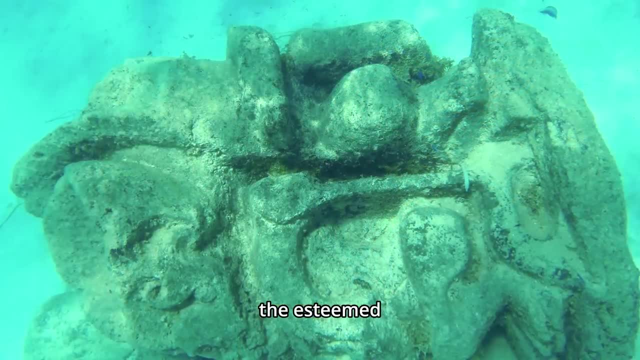 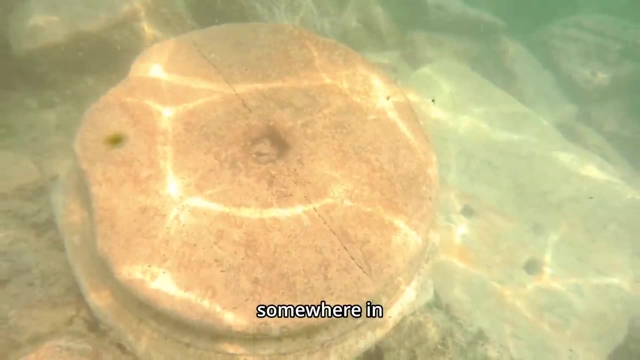 From there, it could have made its way to the esteemed halls of the Alexandrian Library and later into the regal collections of the palace in Constantinople. Somewhere in this historical journey, the key to deciphering the map's intricate grid system might have been misplaced, rendering it temporarily unusable. 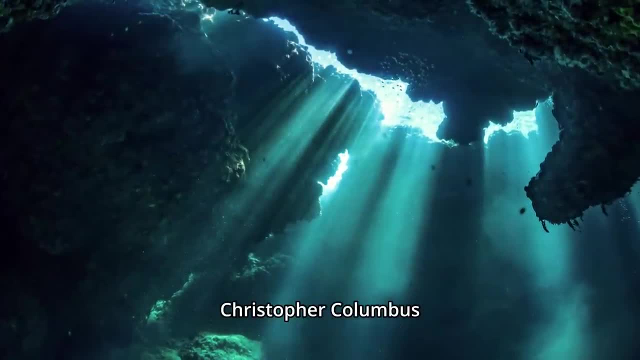 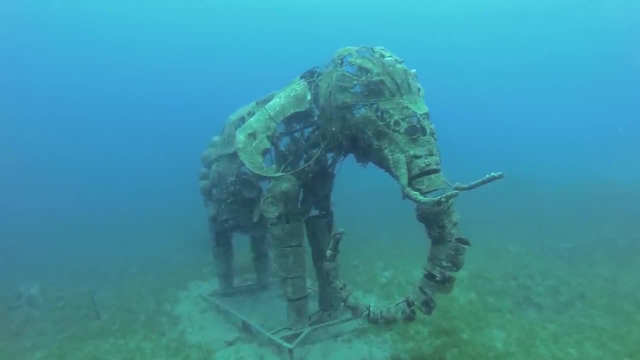 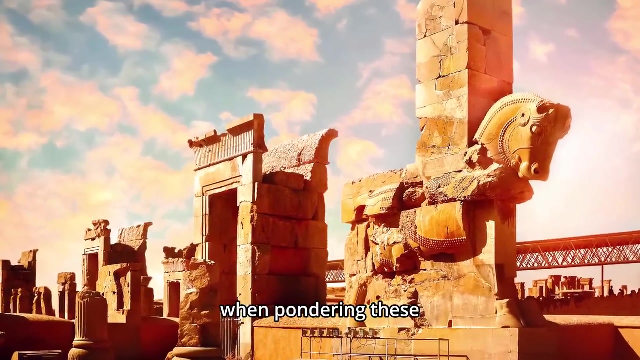 Yet it is a documented fact that when Christopher Columbus embarked on his pioneering voyage in pursuit of a shortcut to India, he possessed some remarkably unconventional maps. It's human nature to indulge in speculation, and it's all too tempting to leap to mind-boggling conclusions when pondering these enthralling mysteries. 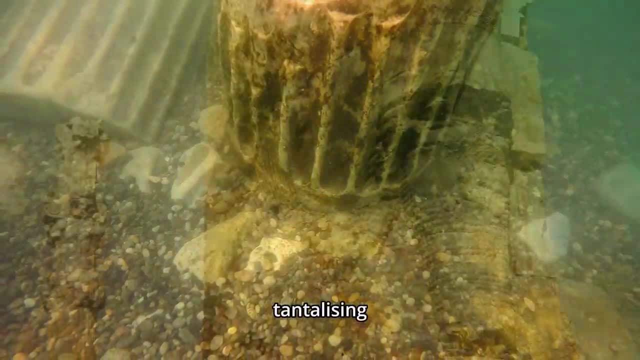 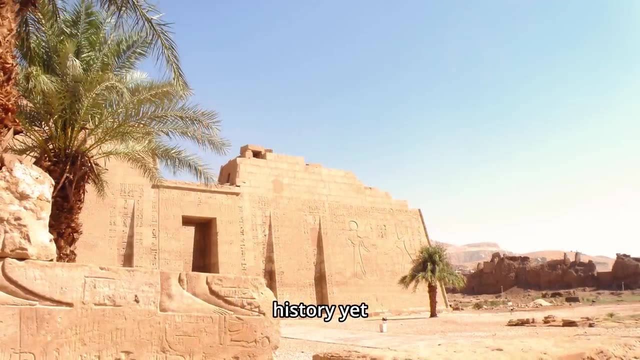 Our quest compels us to piece together the myriad fragments of tantalizing information scattered across the globe, in an endeavor to paint a comprehensive portrait of our ancient history. Yet in this pursuit, we must confront an uncomfortable verity: our own profound ignorance. 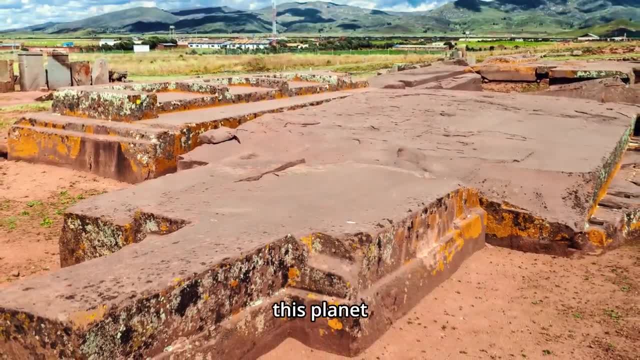 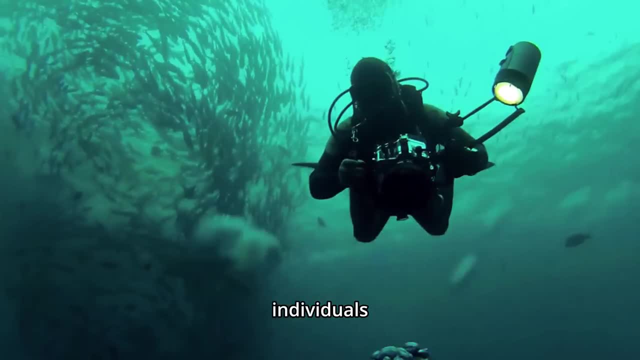 It's sobering to realize that vast expanses of this planet covering hundreds of thousands of square miles remain untouched by the inquisitive minds of scientifically trained individuals. Seasoned explorers know all too well the perennial challenge of acquiring precise maps. 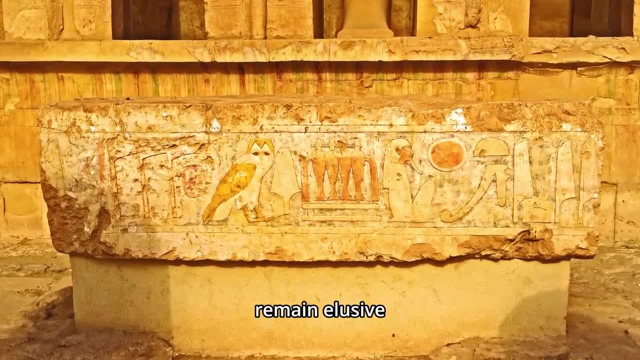 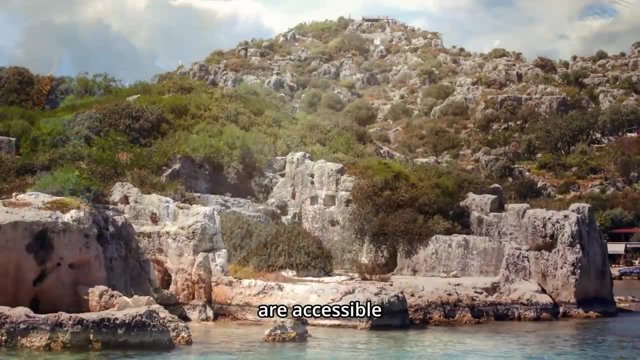 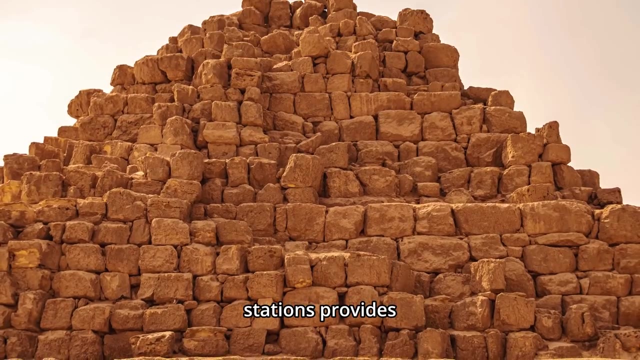 In numerous corners of the world, comprehensive maps remain elusive simply because no comprehensive surveys have ever been conducted. Moreover, even the maps that are accessible may display mountains and rivers in inaccurate locations. The typical road map you receive at service stations provides coverage solely for major highways and prominent urban centers. 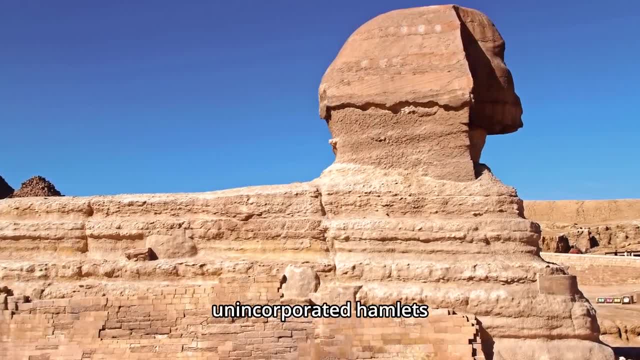 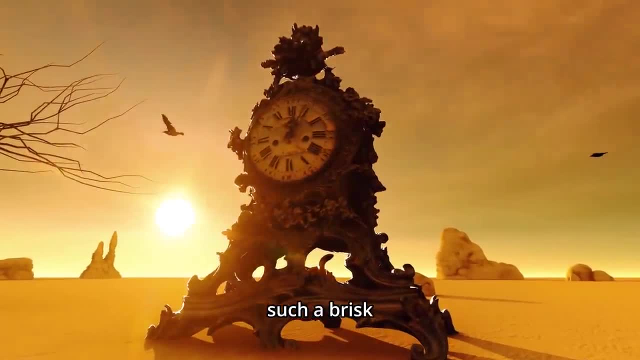 Regrettably, the countless unincorporated hamlets, numbering in the thousands, remain invisible on virtually all maps. Motorway construction proceeds at such a brisk pace that the conventional road maps tend to lag behind by a span of two to three years. 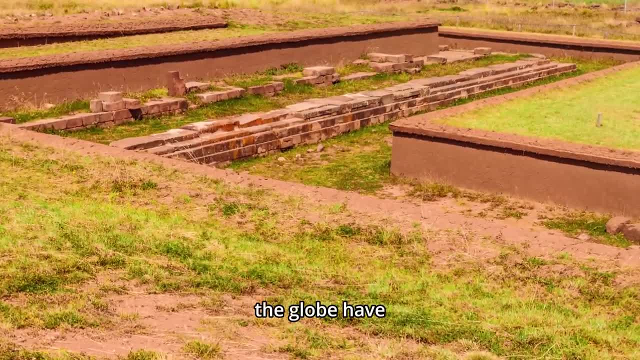 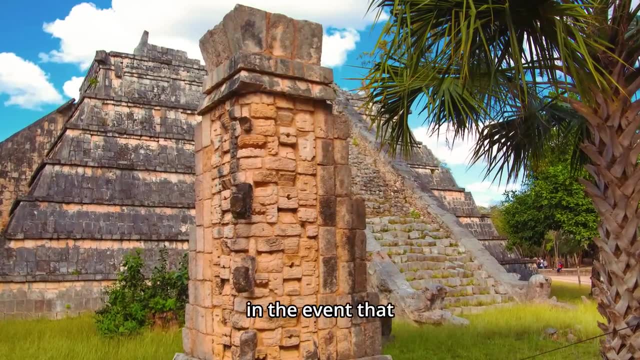 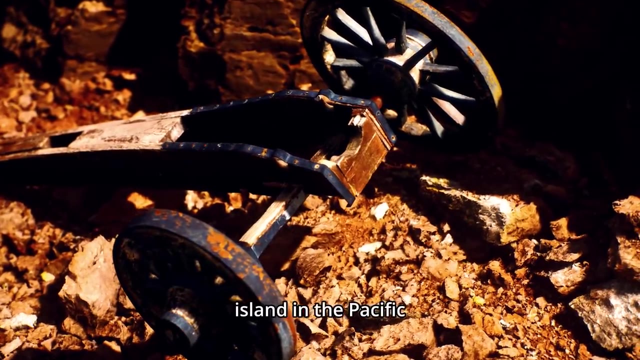 It's fascinating to consider that numerous islands across the globe have never experienced human exploration, naming or cartographic representation. In the event that the hypothetical WOW organization truly exists, they could conceivably stake claim to an uncharted island in the Pacific or Antarctica remaining utterly inconspicuous to the rest of the world. 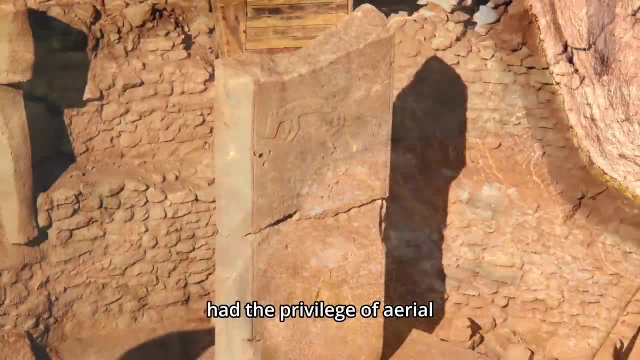 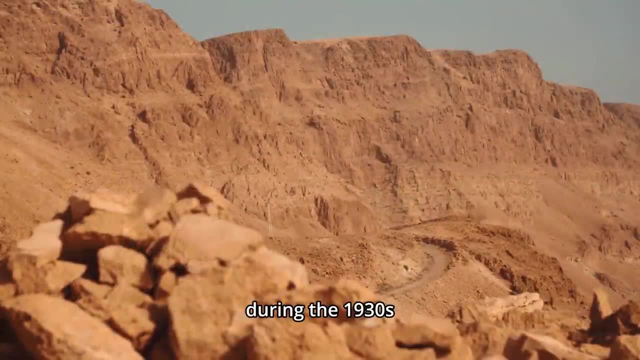 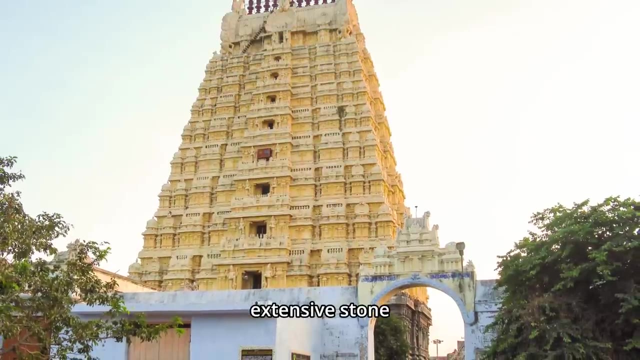 We've certainly had the privilege of aerial exploration, enabling us to observe a substantial portion of the Earth from above. For instance, during the 1930s, Charles Lindbergh embarked on a flight over Brazil, during which he marveled at the sight of an extensive stone wall hidden within the dense jungle. 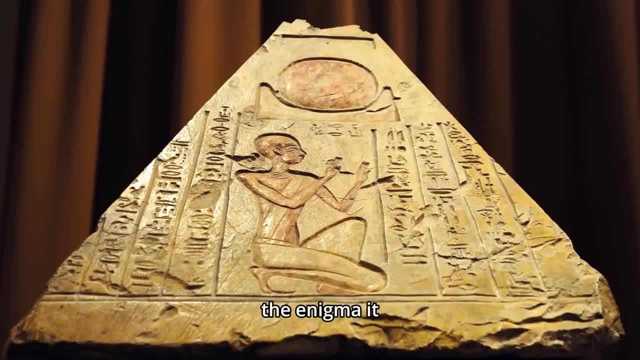 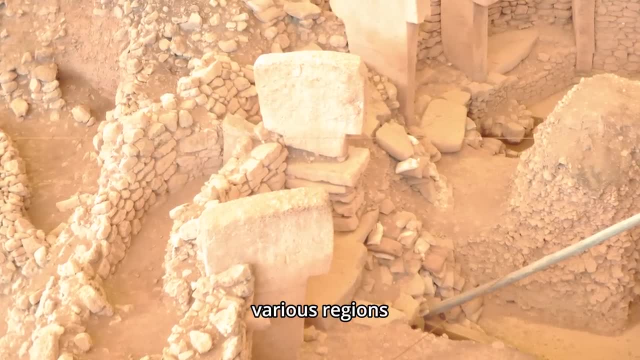 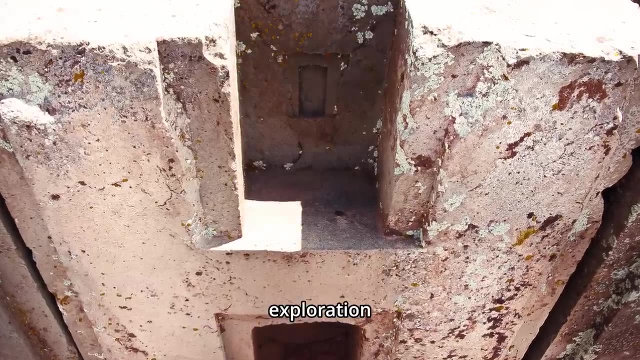 This wall appeared to stretch for miles, yet the enigma it presented was never delved into by scientific inquiry. Similarly, numerous other flights over various regions of the world have reported similar peculiarities, many of which remain shrouded in mystery, untouched by exploration and investigation. 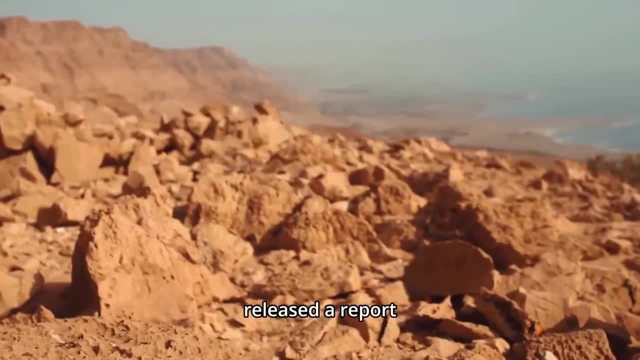 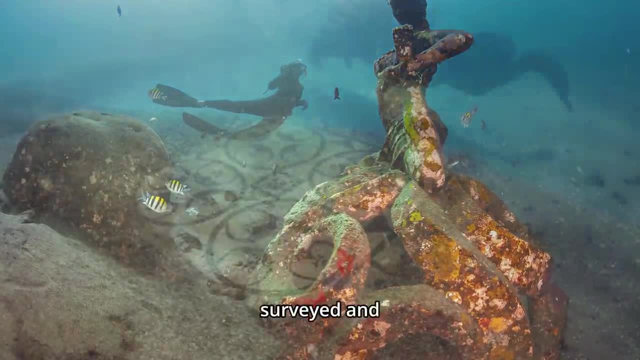 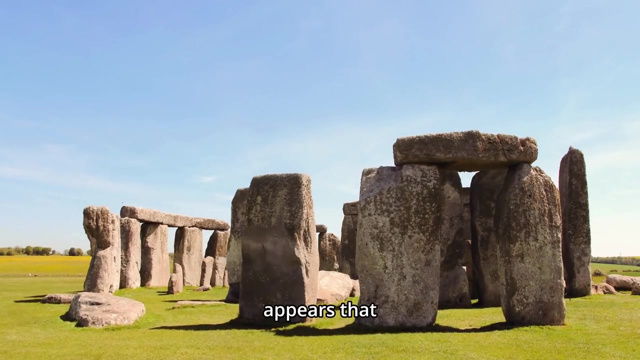 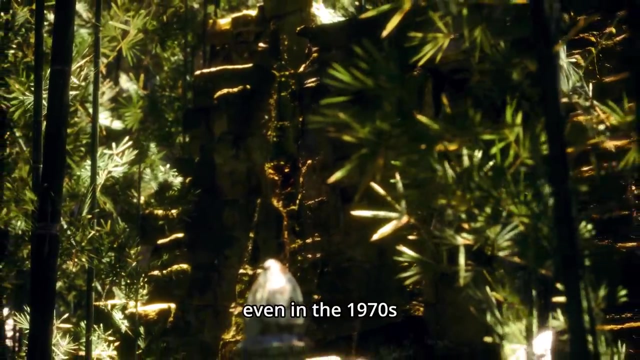 Back in 1970, the United Nations released a report that highlighted a disconcerting fact: A staggering four-fifths of our planet's surface remained inadequately surveyed and charted, and extensive areas continued to elude exploration. Strangely, it appears that the cartographers responsible for crafting the initial Piri Rice maps held a more comprehensive understanding of our world than we had even in the 1970s. 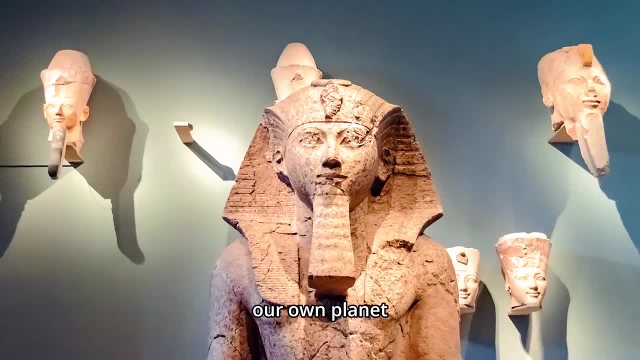 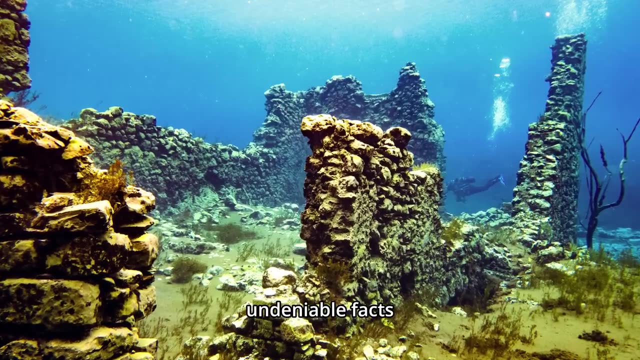 This intriguing revelation serves as a reminder that there is much about our own planet that remains veiled in mystery, waiting to be unveiled and understood. In spite of these undeniable facts, the prevailing belief among many is that our planet has been meticulously explored and every enigma has been deciphered. 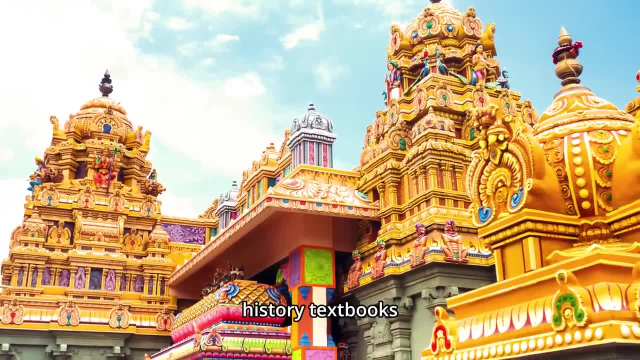 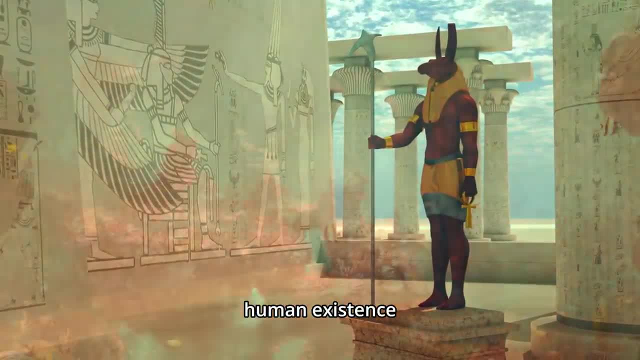 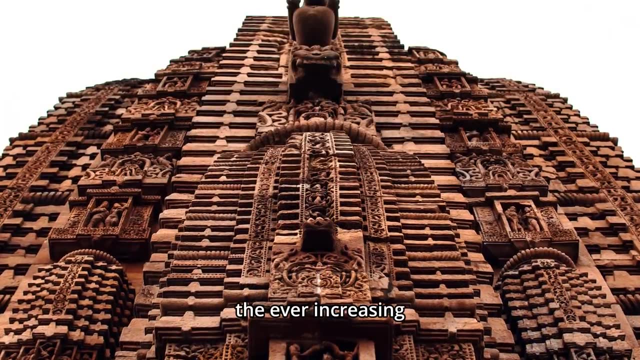 Conventional wisdom often leads us to place our trust in history textbooks. Astonishingly, countless millions continue to uphold the antiquated and discredited notion that human existence spans a mere 4,000 years. The scientific community, too, struggles to accommodate the ever-increasing body of evidence suggesting that we might not be the sole intelligent life forms inhabiting Earth. 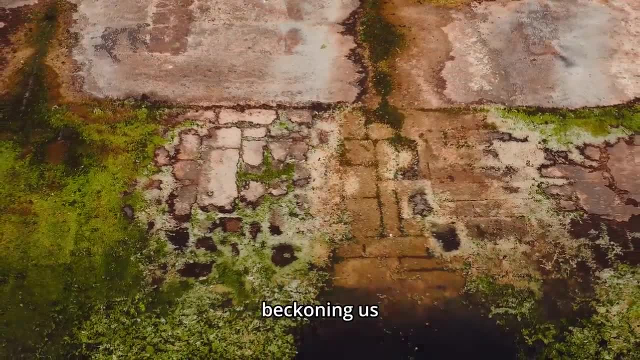 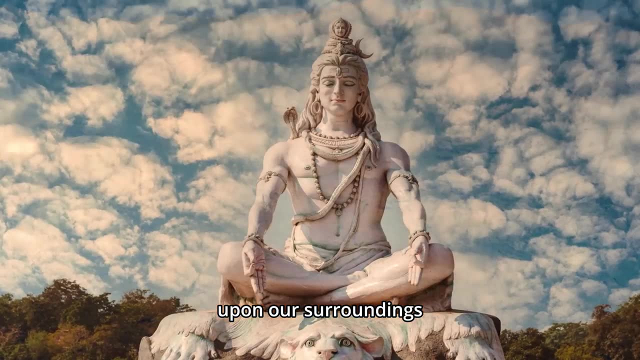 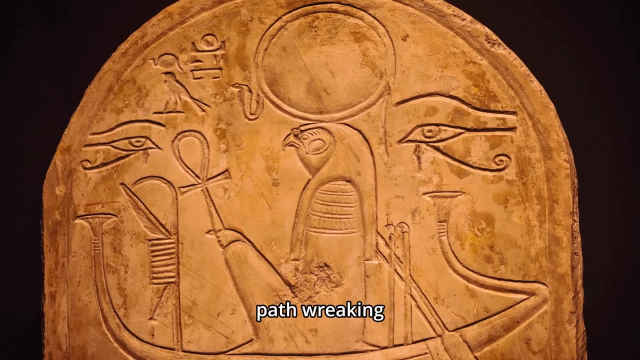 The mysteries of our world remain largely uncharted, beckoning us to seek the truths hidden behind them. The moment has arrived for us to cast a renewed gaze upon our surroundings and consider the unimaginable. The technology we've so ardently championed has often led us down a treacherous path, wreaking havoc on our environment and furnishing the very tools that could threaten the very existence of our planet. 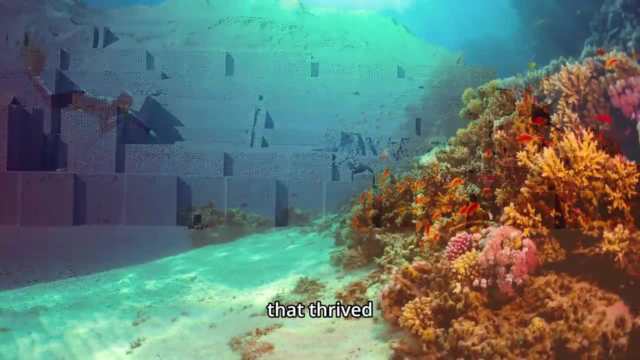 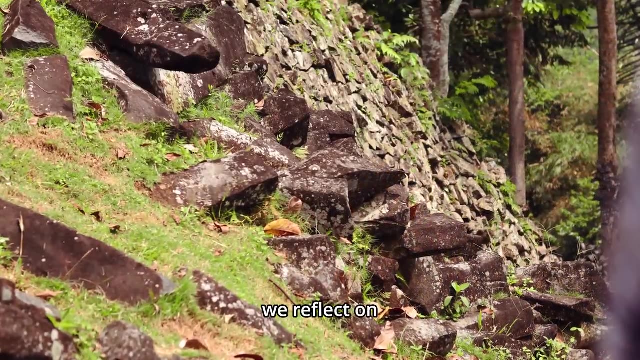 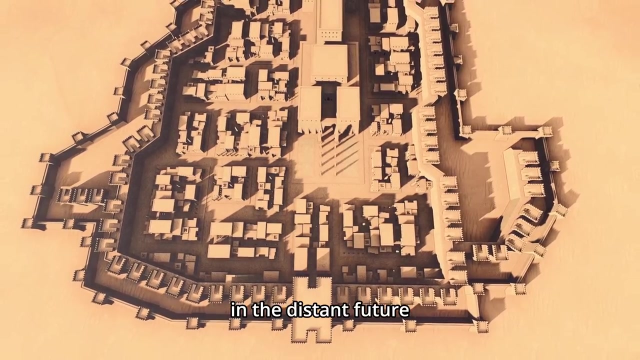 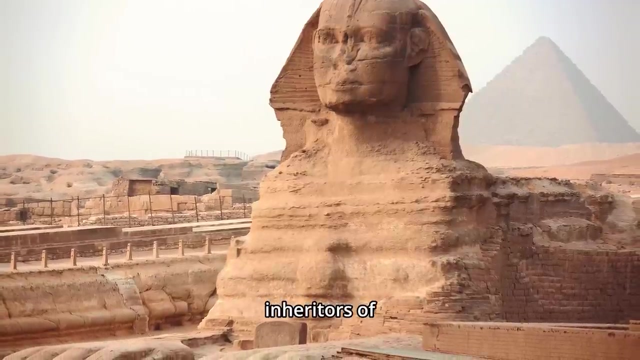 If indeed there was an immensely advanced civilization that thrived millennia ago, perhaps they too grappled with a perilous course similar to our own. It is imperative that we reflect on the lessons that history, both known and concealed, can impart. Perhaps, in the distant future, the abominable snowmen of the Himalayas and the North American counterparts, the Sasquatch of Canada, will become the rightful inheritors of our planet. 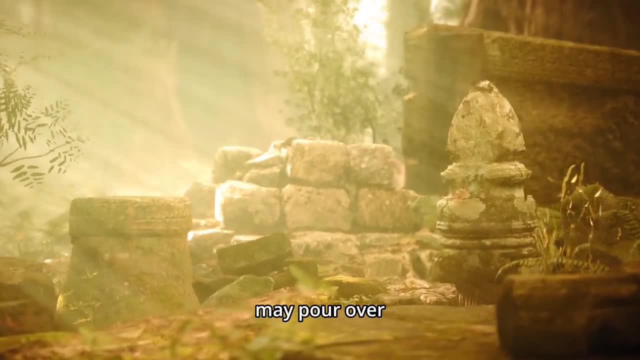 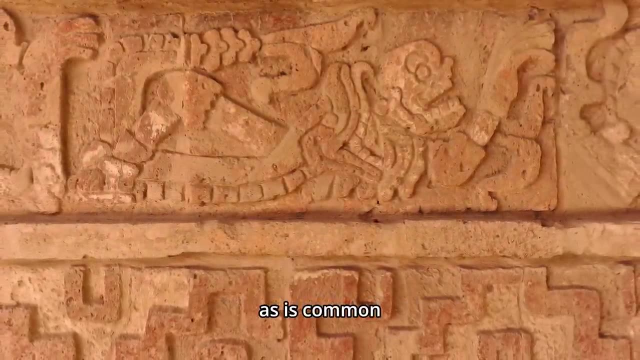 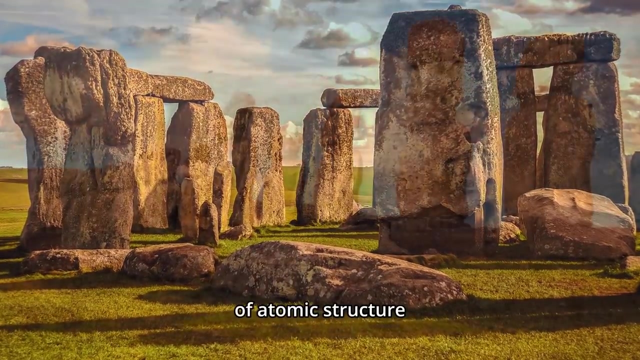 Millennia down the line, their descendants may pore over a tattered relic, a remnant of an ancient road map, and ponder our existence. Among them, as is common, there will be scholars who doubt. They will dismiss the entire notion, returning to their pursuits, such as the quest to unlock the secrets of atomic structure. 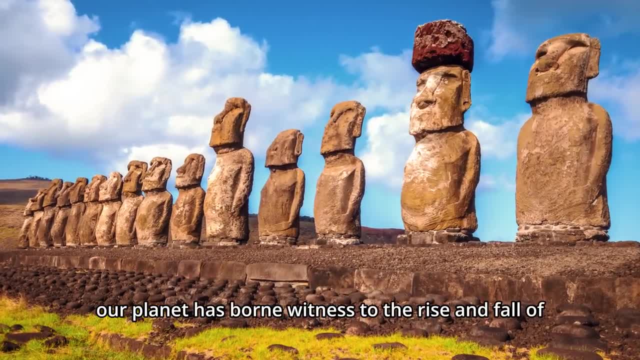 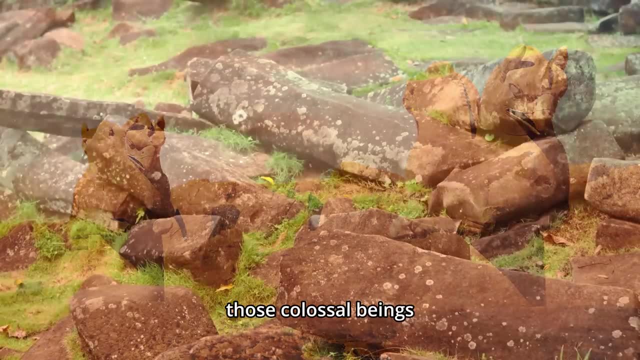 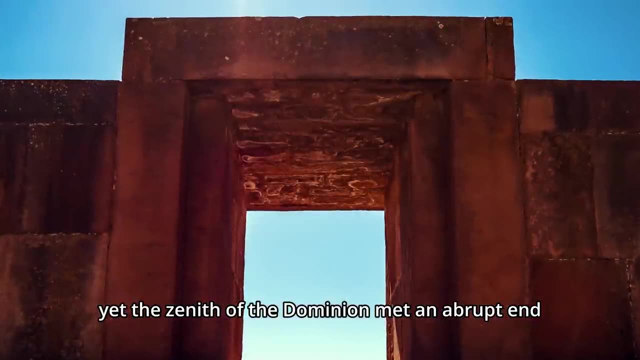 Throughout the annals of Earth's history, our planet has borne witness to the rise and fall of numerous living species. Among the most renowned are the dinosaurs, those colossal beings who reigned supreme for nearly 150 million years. Yet the zenith of their dominion met an abrupt end when a colossal asteroid measuring 12 kilometers in diameter. 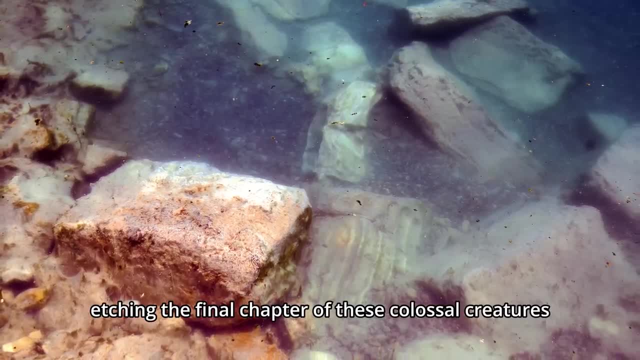 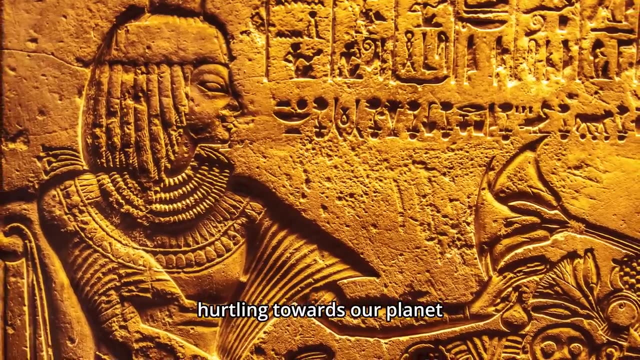 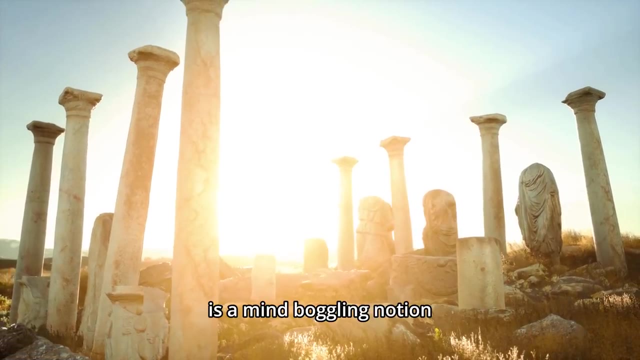 collided with the Yucatan Peninsula, etching the final chapter of these colossal creatures into the tapestry of time. The concept of celestial rocks hurtling towards our planet at speeds of up to 100,000 miles per hour, as it did some 65 million years ago, is a mind-boggling notion. 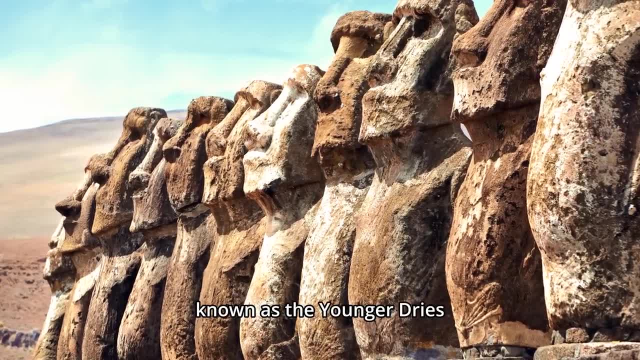 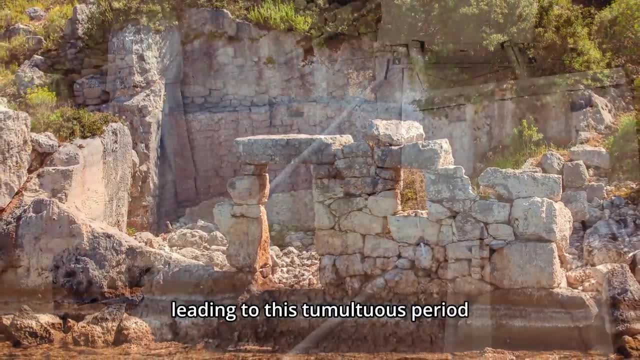 Yet a similar cataclysmic episode, known as the Younger Dryas, unfolded at the conclusion of the last ice age. In the epochs leading to this tumultuous period, the landscapes of North America were inhabited by a diverse array of magnificent creatures. 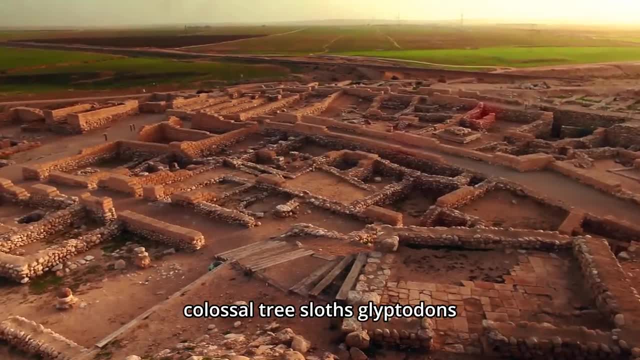 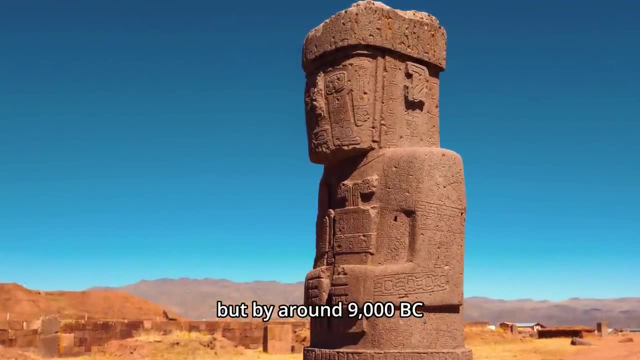 Large mammals, giant beavers, colossal tree sloths, glyptodonts and even the American cheetah roamed these lands, But by around 9000 BC these majestic beings had vanished, disappearing into the annals of history. 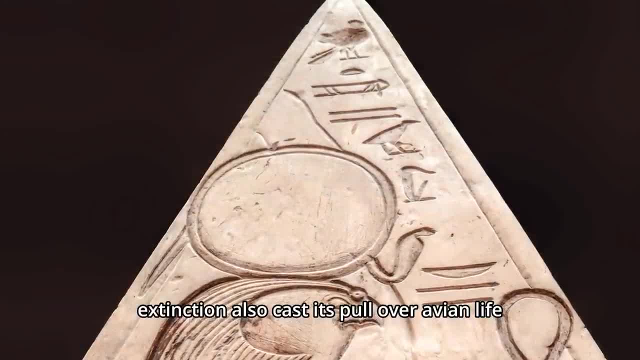 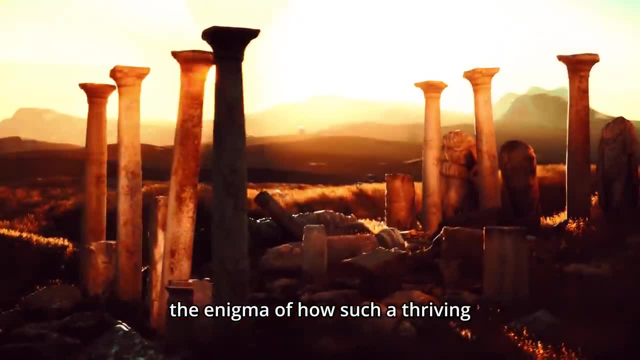 The shadow of extinction also cast its pall over avian life, With no less than 19 genera of birds vanishing from the tapestry of existence. The enigma of how such a thriving ensemble of species met their demise has intrigued scientists for ages. 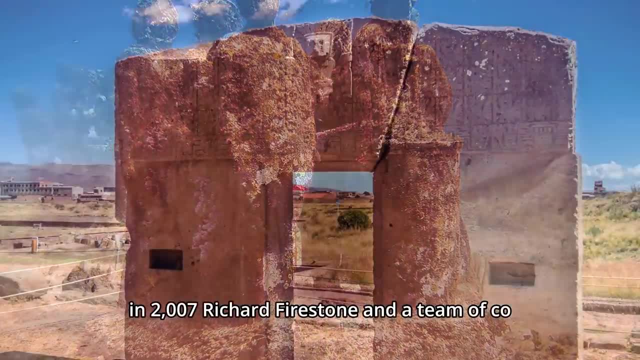 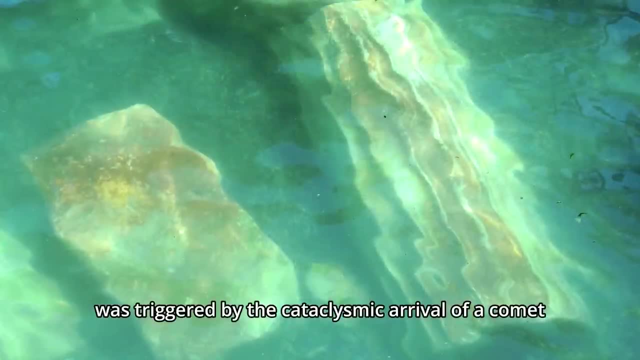 In 2007,, Richard Firestone and a team of co-authors postulated an astonishing theory. The extinction event was triggered by the cataclysmic arrival of a comet. As this cosmic traveler neared Earth, it fragmented into numerous pieces. resulting in a staggering 10 million square kilometers being engulfed by wildfires. As the conflagration consumed roughly 10% of the Earth's surface, it unleashed massive clouds of smoke and ash that ascended to the heavens. These billowing veils shrouded the sun, ushering in a rapid, near instantaneous drop in temperatures by nearly 10 degrees- a mere blink of an eye, in geological terms. 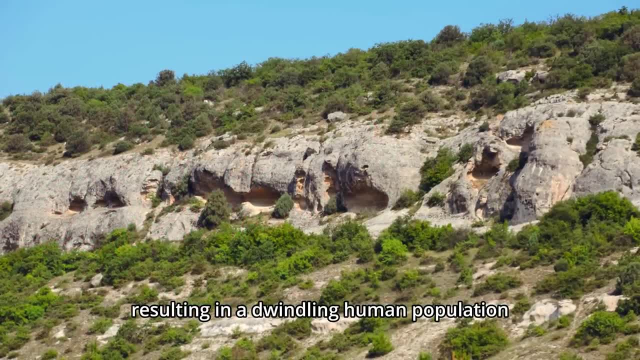 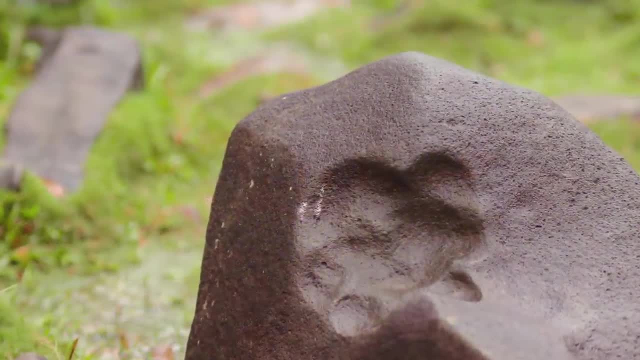 This abrupt cooling triggered a chain reaction resulting in a dwindling human population, a disruption of ocean currents and a catastrophic toll on the planet's flora and fauna. The robustness of this theory finds firm support in an array of chemical imprints found in the soil of North America. The scientific consensus points to a clear time frame for the Younger Dryas climate catastrophe, occurring between 12,800 and 11,500 years ago. Intriguingly, this timeline aligns with the era in which, according to Plato's account in the Timaeus, Atlantis purportedly met its watery demise. 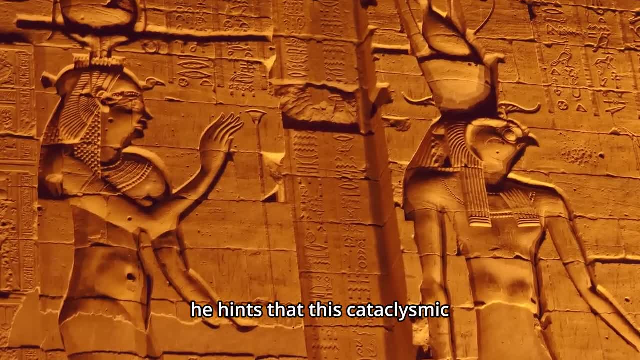 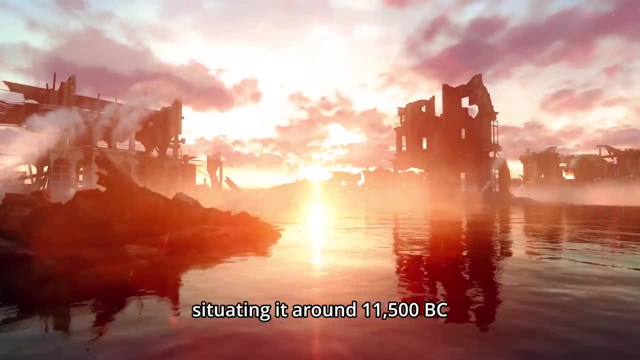 While Plato's narrative lacks a precise date, he hints that this cataclysmic event transpired roughly 9,000 years before his own era, situating it around 11,500 BC. In the waning days of the last ice age, the world was a vastly different place. 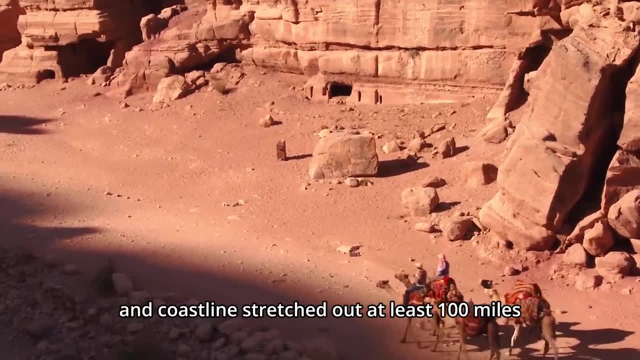 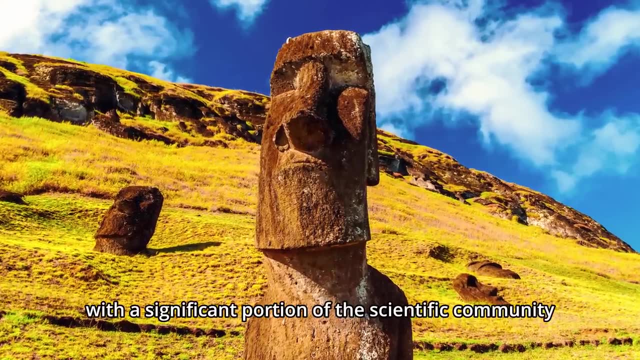 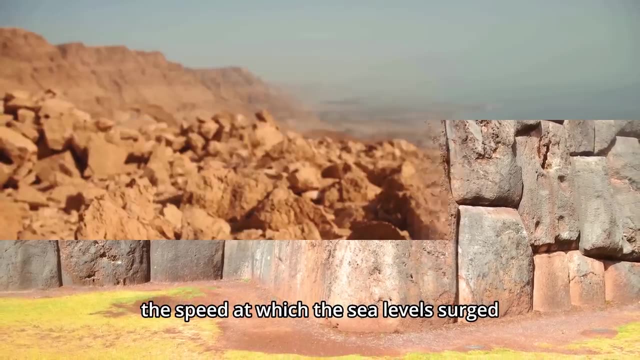 Large landmasses were still interconnected and coastlines stretched out at least 100 miles farther into the sea than they do today. This perspective finds favor with a significant portion of the scientific community. However, the enigma that persists revolves around the speed at which the sea levels surged. 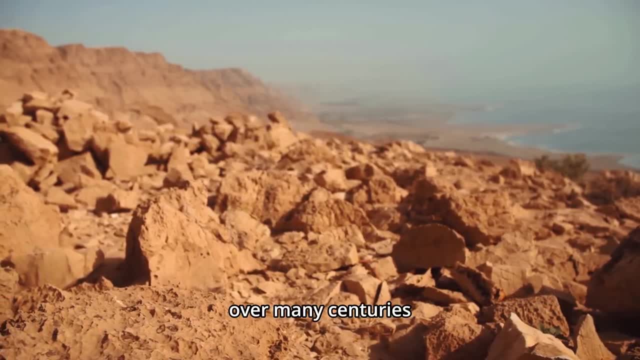 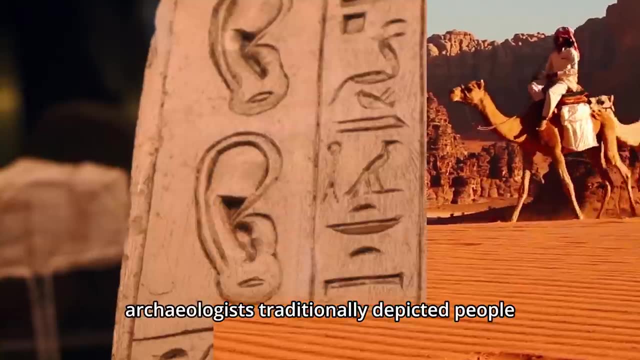 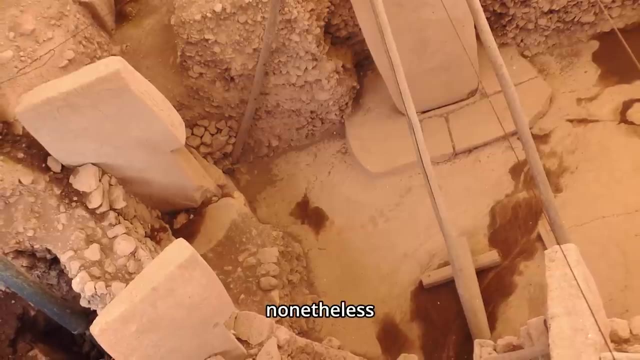 While the conventional view asserts a gradual rise over many centuries, a growing number of scientists are now pondering the possibility of a much swifter inundation. Archaeologists traditionally depicted people living as primitive hunter-gatherers before the onset of this period. Nonetheless, the mounting evidence challenges this narrative. 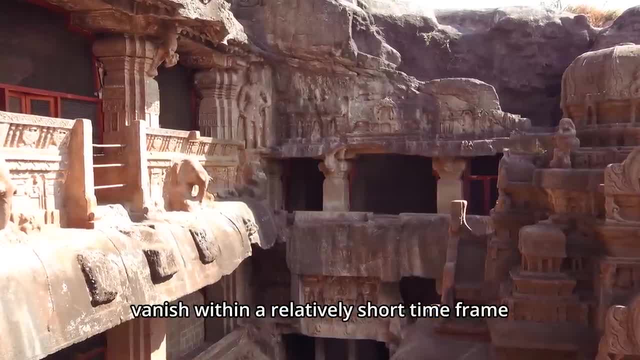 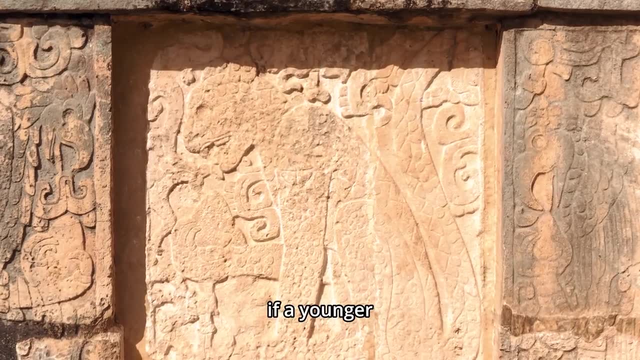 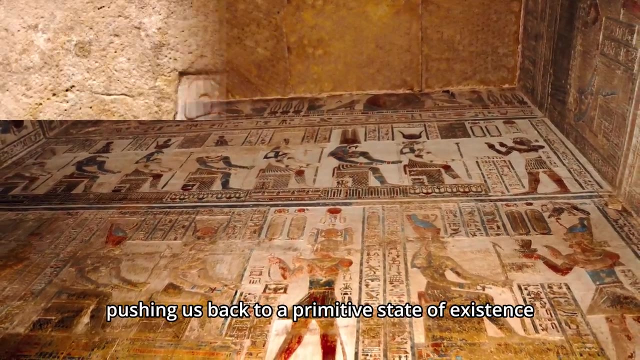 Could an advanced civilization vanish within a relatively short timeframe? The answer, it appears, is a resounding yes. Consider the impact on our civilization. if a Younger Dryas-type event were to happen in our modern era, It would undoubtedly devastate our technology, pushing us back to a primitive state of existence. 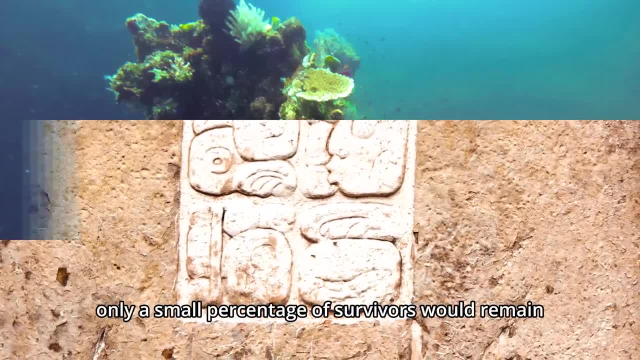 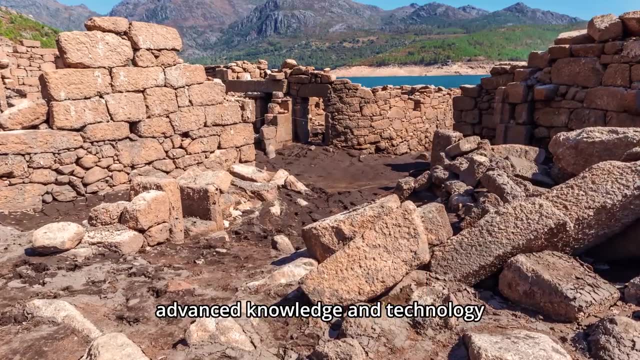 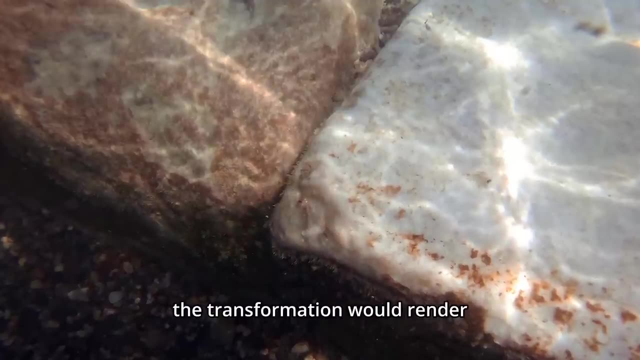 Only a small percentage of survivors would remain, and over time they would develop into a society radically different from our current one. Advanced knowledge and technology would take a backseat to the immediate priorities of survival through hunting and gathering. The transformation would render our former civilization unrecognizable. 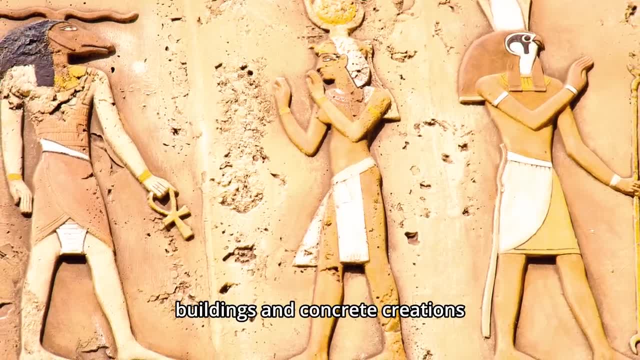 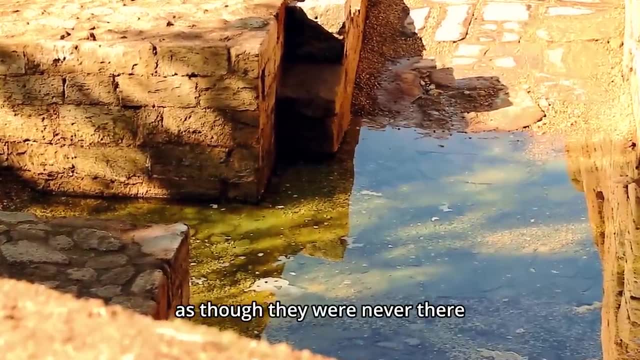 In the absence of human care, structures such as houses, buildings and concrete creations would gradually decay and crumble. With the passage of time. they would vanish as though they were never there. Water, a relentless force of nature, poses the most significant threat to human-made edifices. 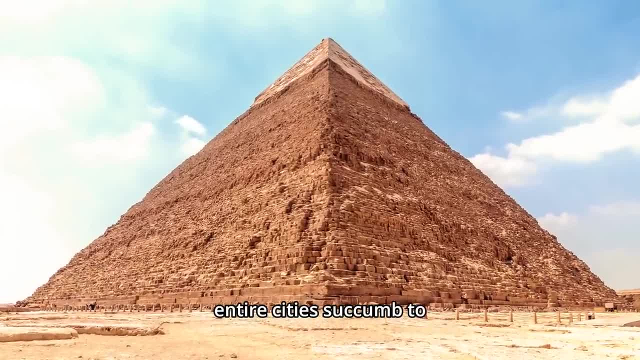 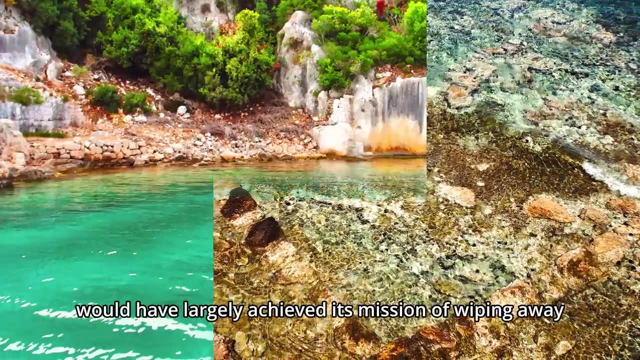 Coastal regions would witness entire cities succumb to the relentless advance of the sea. Five centuries later, the natural world would have largely achieved its mission of wiping away the last vestiges of human presence, What might endure 12,000 years in the future. 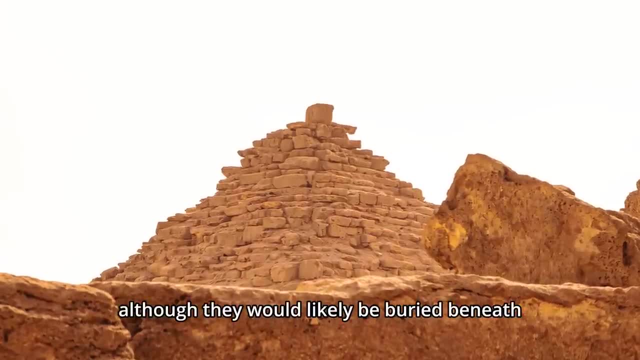 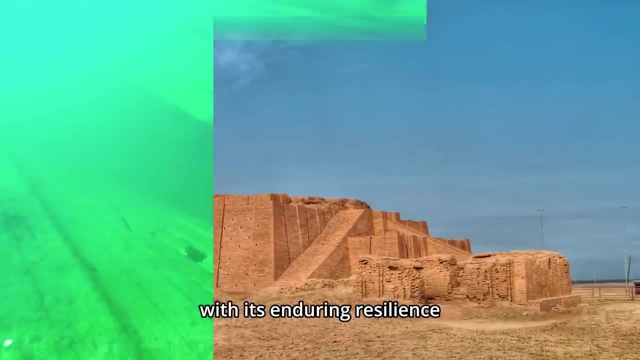 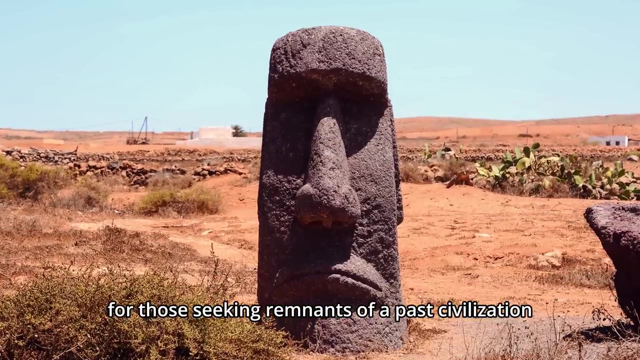 Perhaps a few coins and other precious metals, although they would likely be buried beneath layers of sediment over time. However, stone with its enduring resilience would have a much better chance of withstanding the test of time. Therefore, for those seeking remnants of a past civilization, the most promising places to explore would be ancient stone structures. 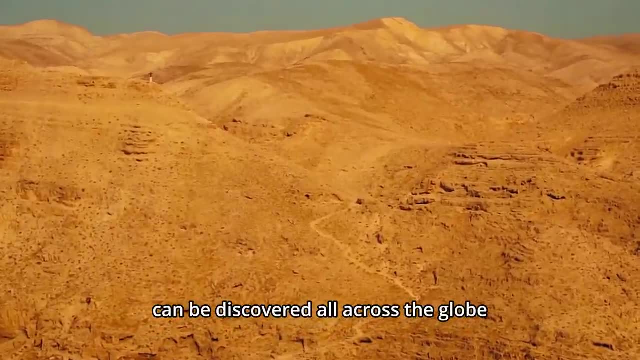 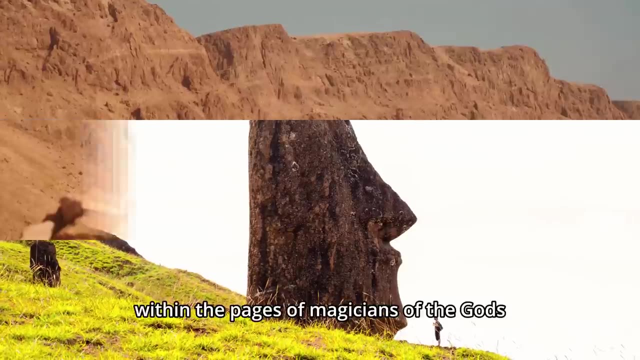 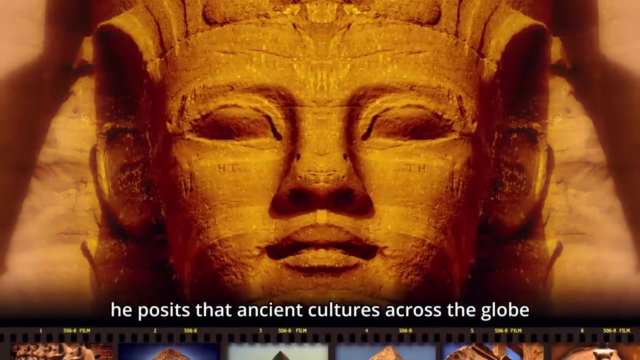 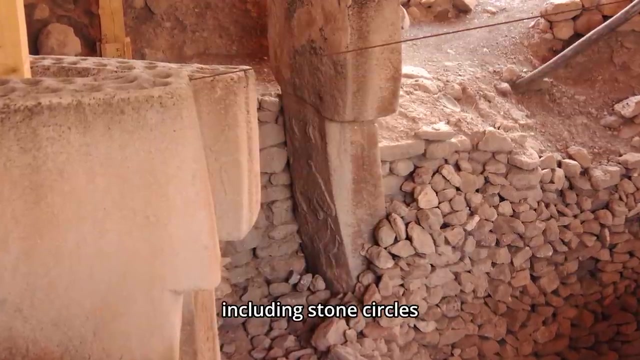 Thankfully, enigmatic stone monuments can be discovered all across the globe, taking various forms and sizes, Yet among the most enduring are stone circles. Within the pages of Magicians of the Gods, Graham Hancock weaves a captivating theory. He posits that ancient cultures across the globe possessed a profound grasp of astronomy, which they expressed through megalithic wonders, including stone circles. 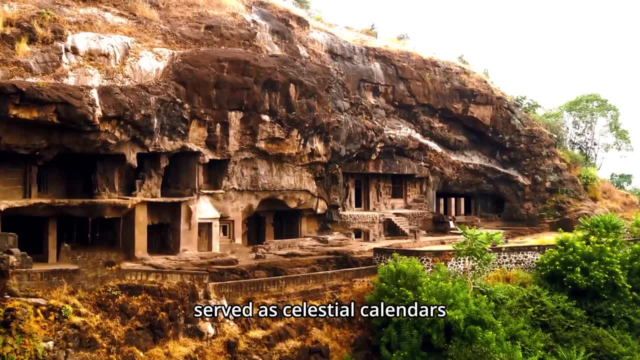 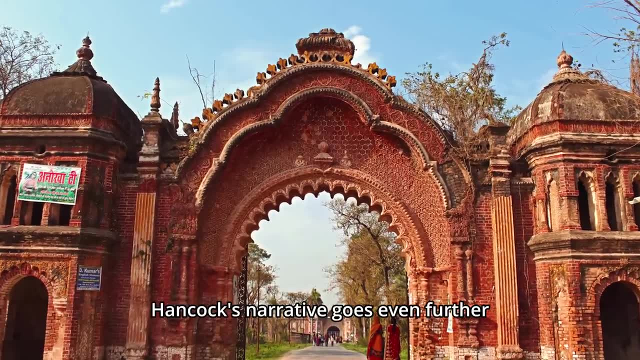 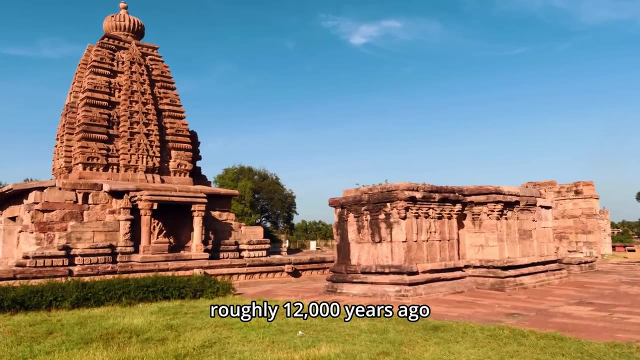 These monumental structures served as celestial calendars, meticulously marking pivotal astronomical events like solstices and equinoxes. Hancock's narrative goes even further, Suggesting the existence of a worldwide civilization obliterated by a catastrophic event roughly 12,000 years ago: the Younger Dryas event. 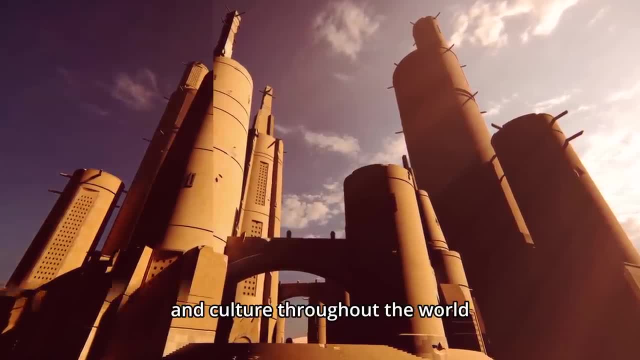 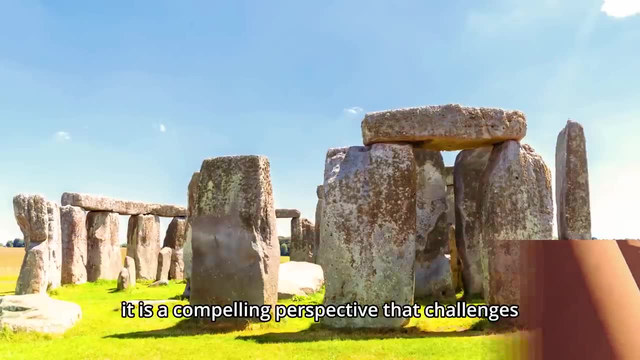 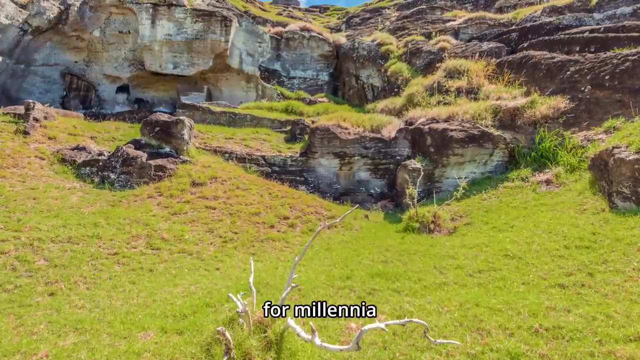 Survivors in his vision propagated their knowledge and culture throughout the world, and the enduring stone monuments stand as enduring testaments to their once vast wisdom. It is a compelling perspective that challenges our understanding of history and the breadth of human capability. For millennia, ancient civilizations have raised monumental monuments. 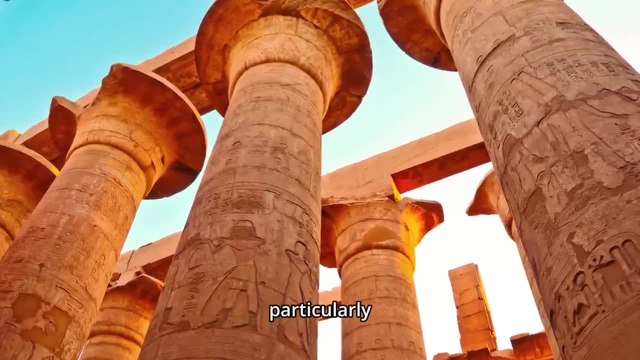 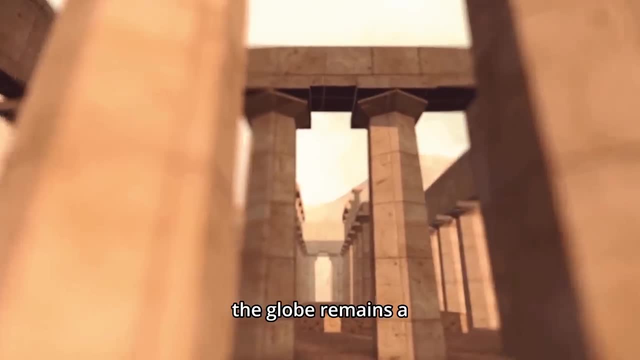 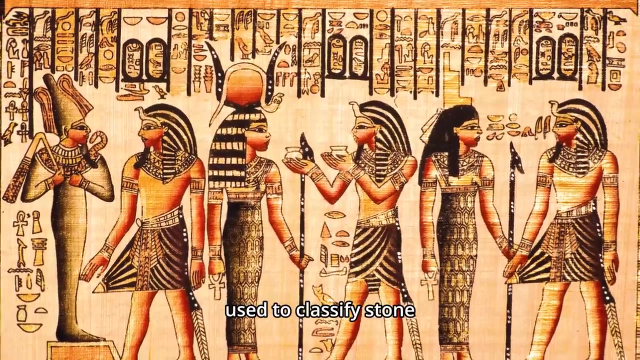 They are monumental stone circles that stand as testaments to their extraordinary skills, particularly in fields such as geometry and astronomy. Enumerating the precise count of ancient stone circles across the globe remains a formidable task, given the ever-evolving nature of archaeological research and the diverse criteria used to classify stone structures as stone circles. 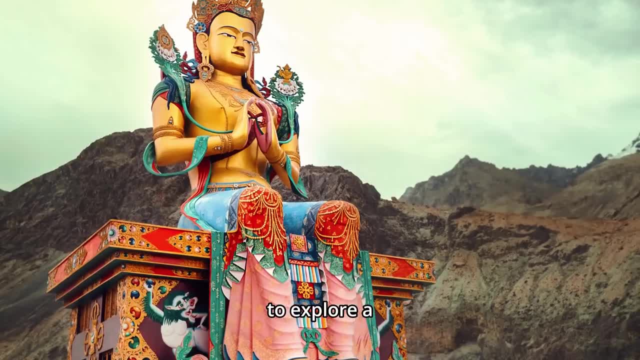 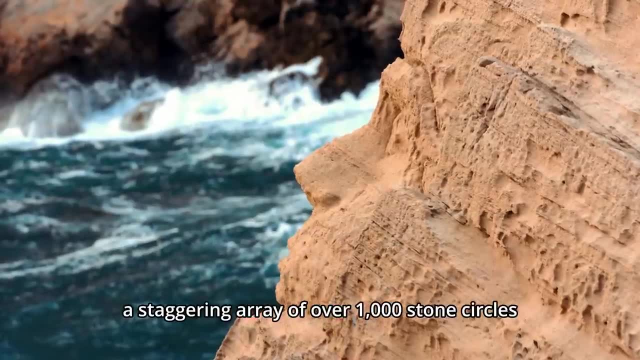 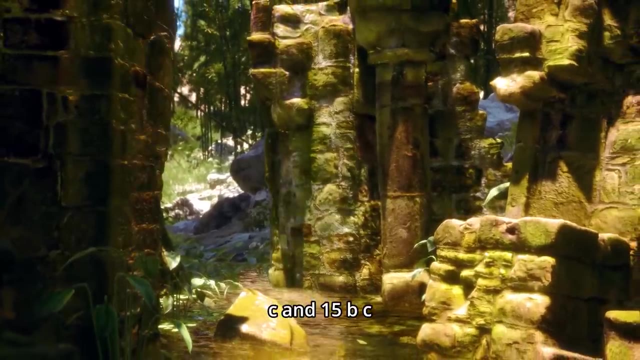 Nevertheless, let's embark on a journey to explore a selection of renowned ancient stone circles located in different corners of the world. In the British Isles, a staggering array of over a thousand stone circles hailing from the period between 3500 BC and 1500 BC graces the landscape. 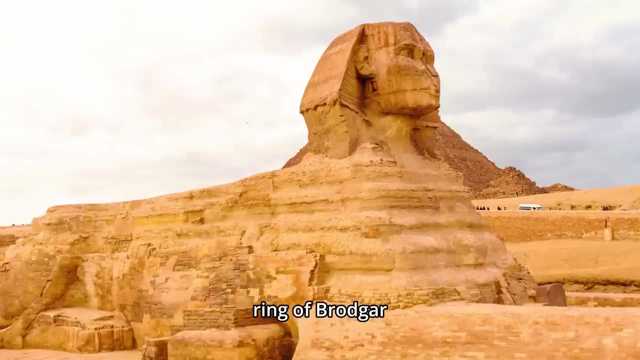 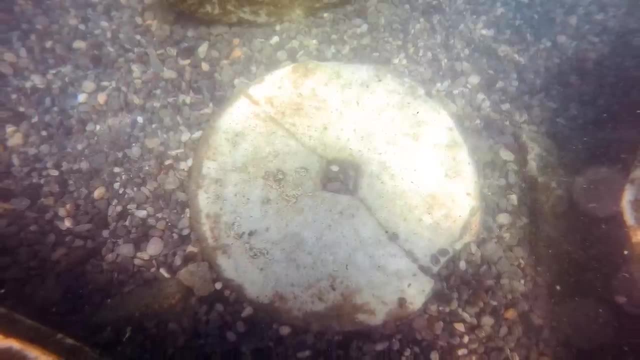 Among these ancient marvels, you'll find the enigmatic Ring of Brodgar, the mystical Arbor Low, the mystical Rollwright Stones and the captivating Mormbie Stone Circle Stonehenge, the crown jewel of British stone circles, resides in the heart of Wiltshire, England. 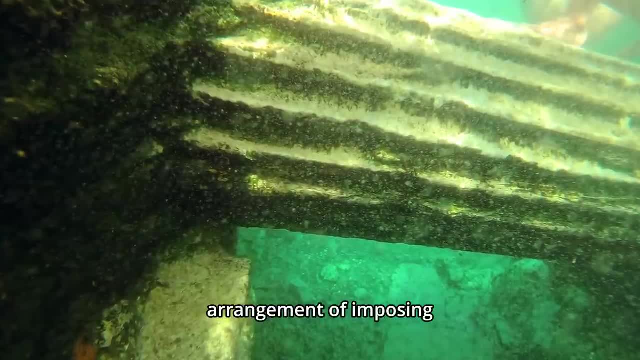 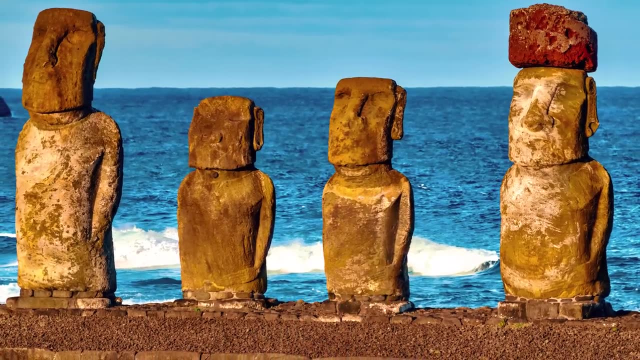 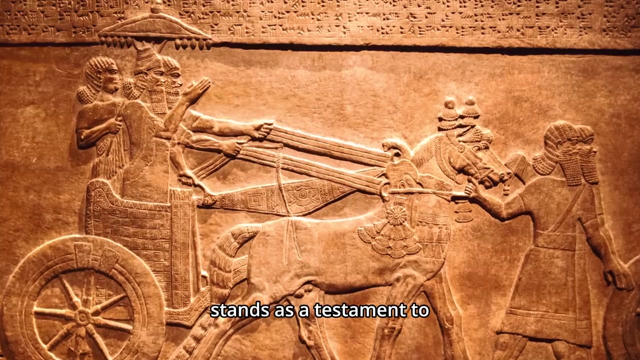 Its grandeur lies in the arrangement of imposing upright stones adorned with crowning horizontal lintels, forming a mesmerizing circular structure. This ancient marvel, dating back to a timeframe between 3000 and 2000 BC, stands as a testament to the mysteries of old. 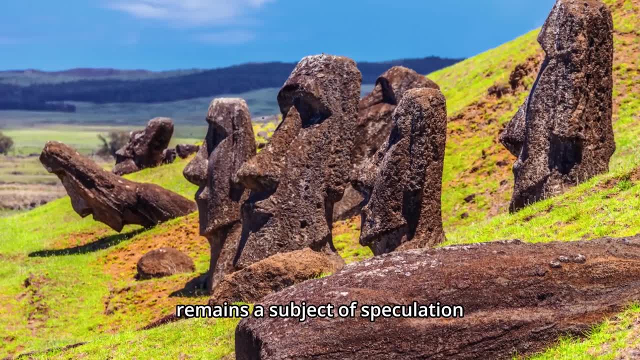 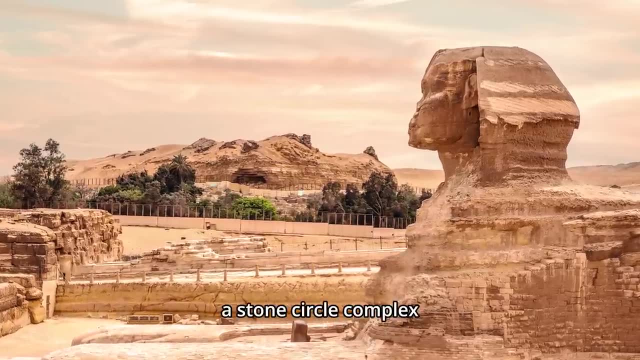 While its exact purpose remains a subject of speculation, it is believed to have played a role in ancient ceremonies and astronomical endeavors. Avebury, a stone circle complex located in close proximity to Stonehenge, stands as a colossal monument of ancient ingenuity. 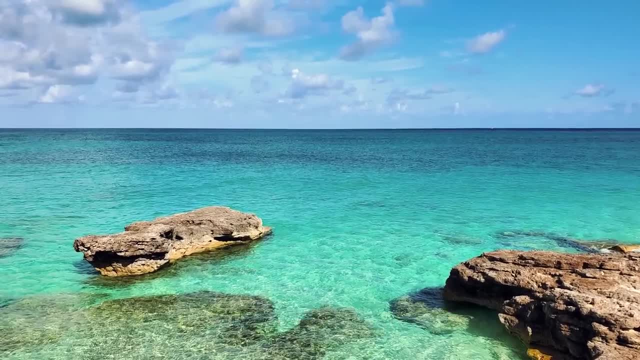 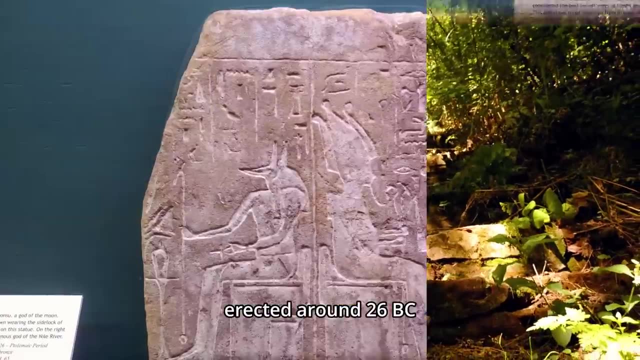 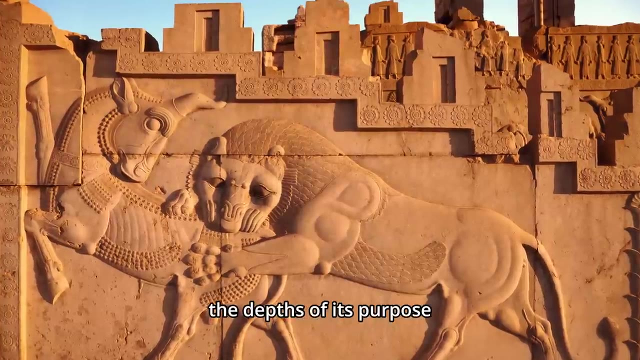 It surpasses all European counterparts in size, encircling a vast expanse with its circular earthwork and a meandering trench Erected around 2600 BC. this enigmatic structure leaves an indelible mark on history, inviting us to delve into the depths of its purpose and the civilization that brought it into existence. 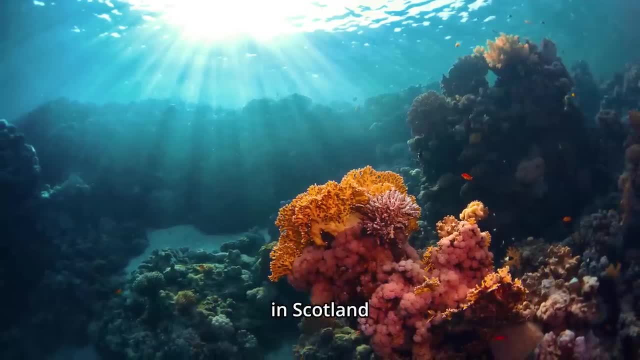 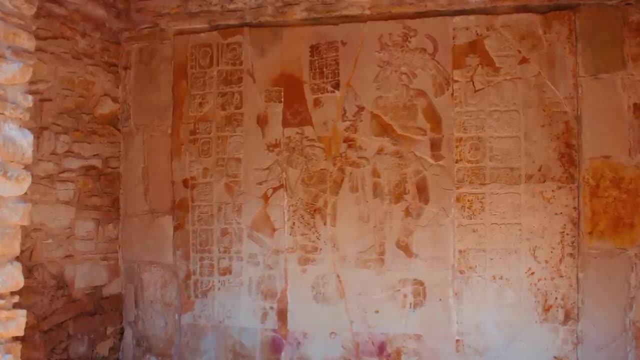 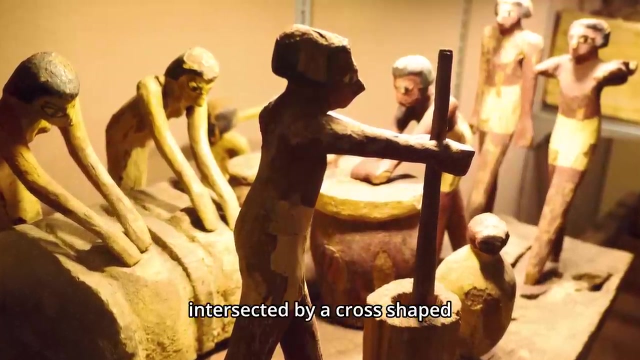 Nestled upon the rugged Isle of Lewis in Scotland, the Calanish stones create an intricate tapestry of standing stones, each with its unique size and shape. At the heart of this ancient site lies a primary stone circle characterized by a central ring intersected by a cross-shaped arrangement. 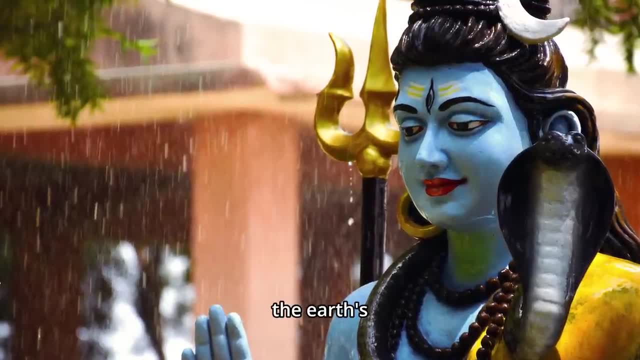 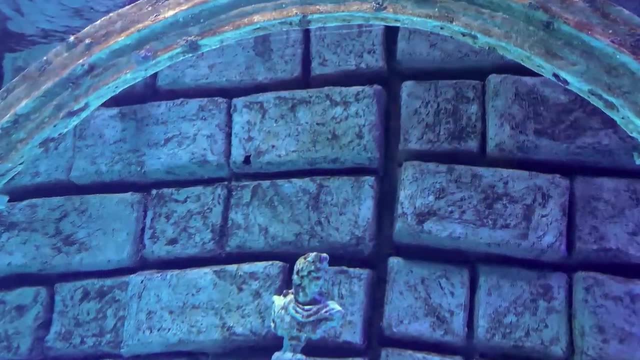 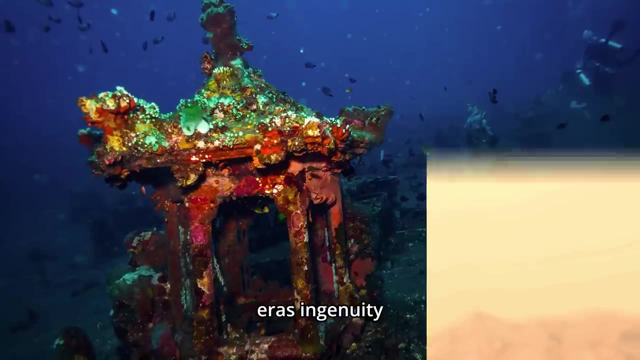 It's believed that these enigmatic stones rose from the earth's embrace between 2900 and 2600 BC, whispering tales of a distant past. Overlooking the North Sea, in the heart of Germany, the Gossik Circle stands as a testament to the Neolithic era's ingenuity. 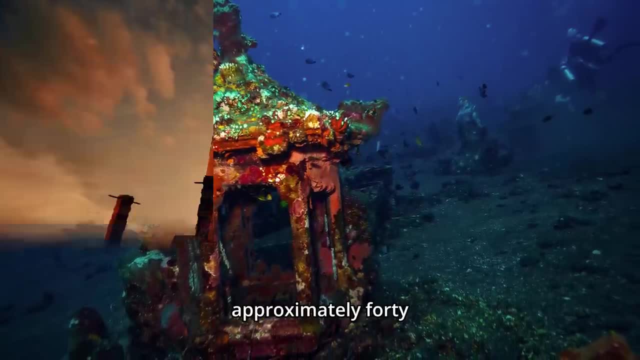 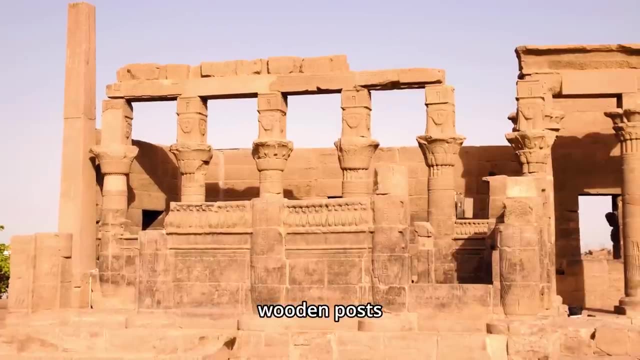 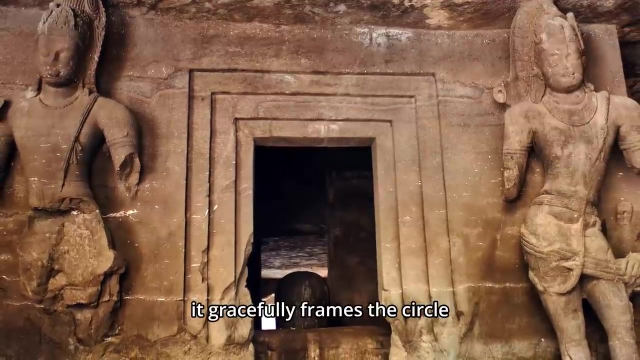 This ancient circular enclosure dating back to approximately 4900 BC boasts an intriguing history. Its design comprises concentric rings of sturdy wooden posts, meticulously aligned with the rhythms of the heavens. As the sun graces the horizon, it gracefully frames the circle during both the winter and summer solstices. 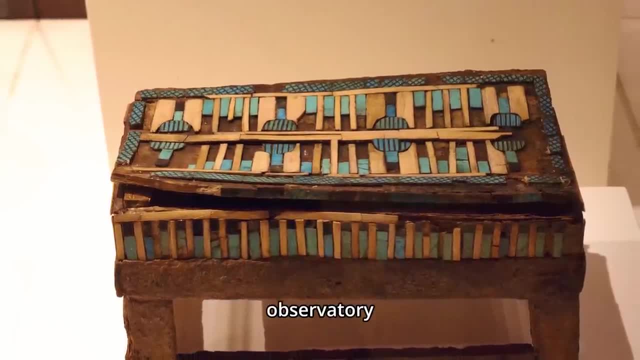 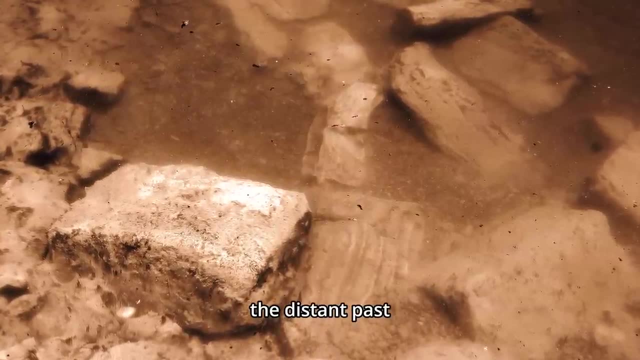 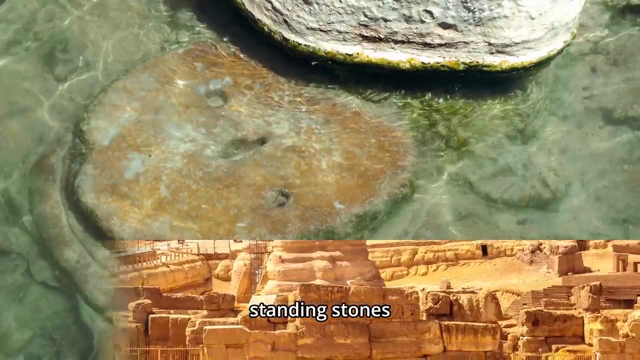 casting its light upon this prehistoric solar observatory. The enigmatic Göbekli Tepe, nestled in the heart of Turkey, offers a fascinating glimpse into the distant past, Dating back to approximately 11000 BC. this ancient site boasts towering standing stones, meticulously arranged in mesmerizing circular patterns. 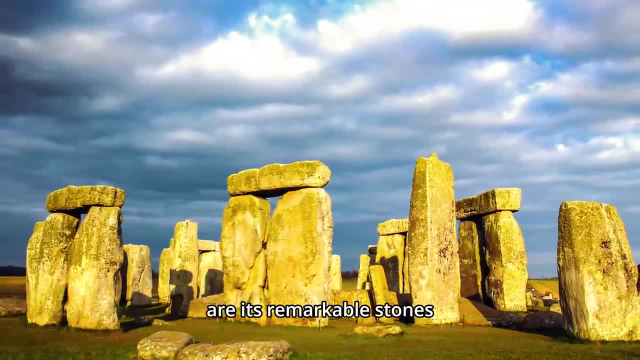 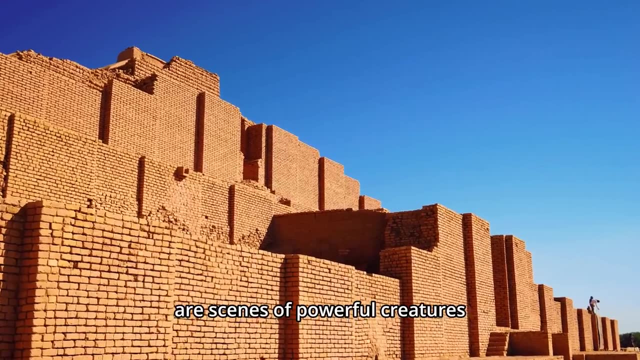 What truly sets Göbekli Tepe apart are its remarkable stones adorned with intricate carvings and reliefs. Among these artistic depictions are scenes of powerful creatures, including fierce lions, sinuous snakes and graceful birds, preserving the mysteries of an ancient era. 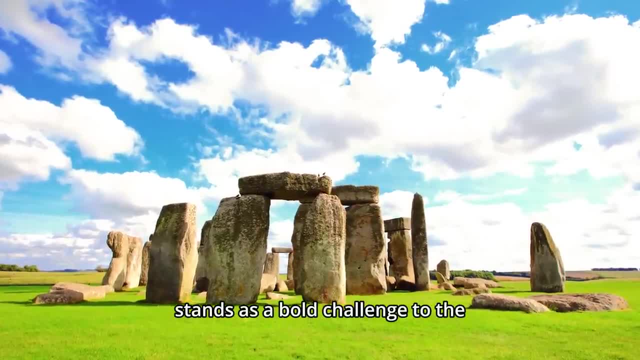 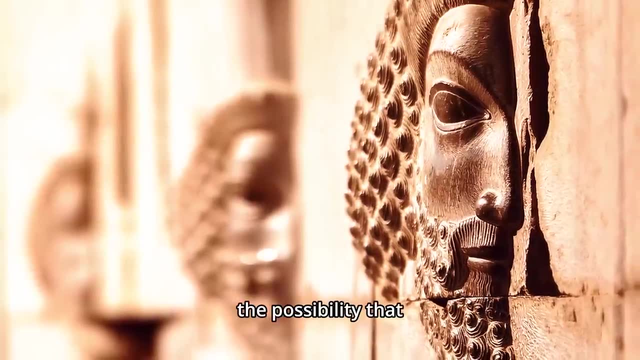 The revelation of Göbekli Tepe stands as a bold challenge to the established notions regarding the dawn of civilization and the evolution of intricate societies. It hints at the possibility that advanced religious and social systems may have blossomed at a much earlier juncture in history than formerly believed. 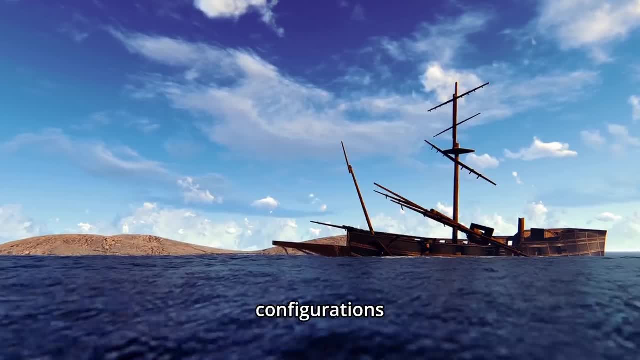 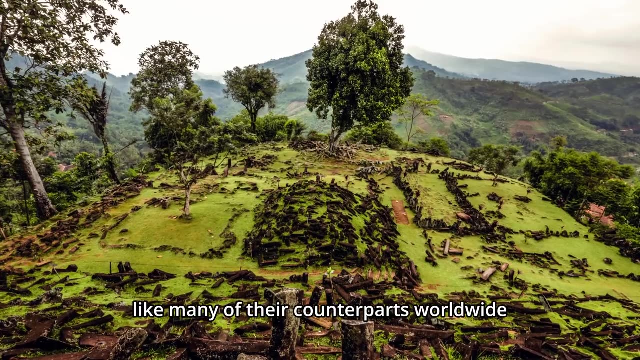 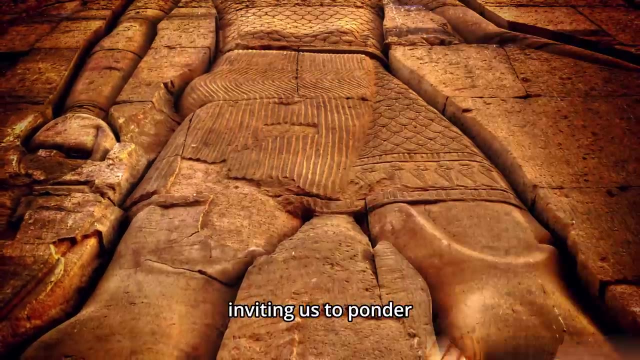 Within this intriguing site, the presence of megalithic configurations and stone circles appears to have held a crucial position in the fabric of these early communities. Like many of their counterparts worldwide, Göbekli Tepe also showcases the presence of celestial alignments, inviting us to ponder their ancient significance. 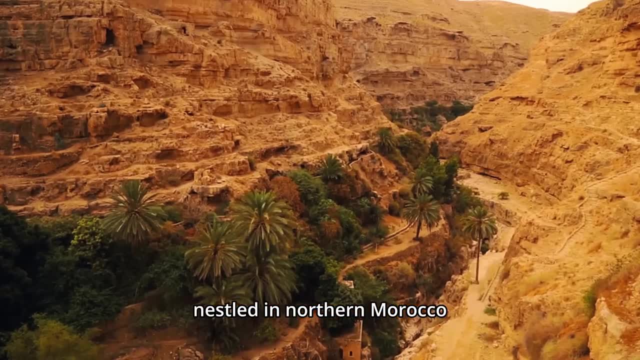 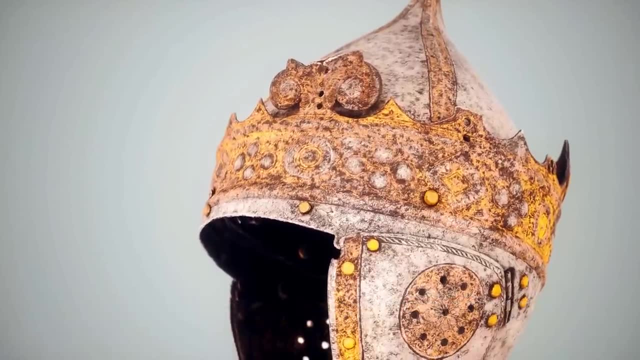 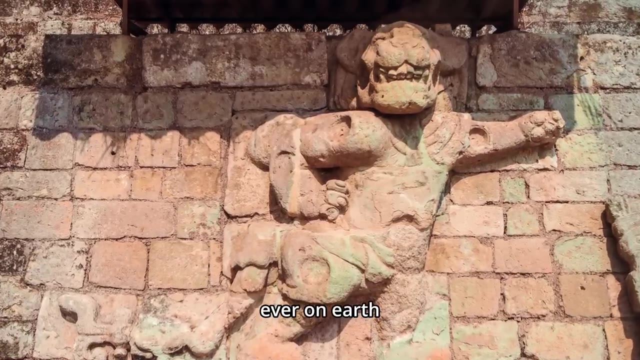 The Amzora Stone Circle, nestled in northern Morocco, boasts an astonishing assembly of 168 stones, with some towering over 5 meters in stature. This remarkable ring spans an impressive 55 meters in diameter, ranking among the largest of its kind ever unearthed. 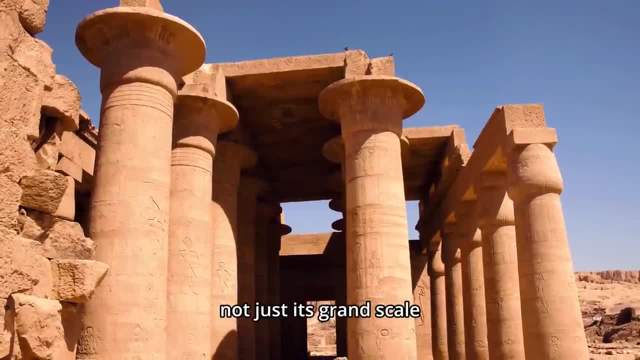 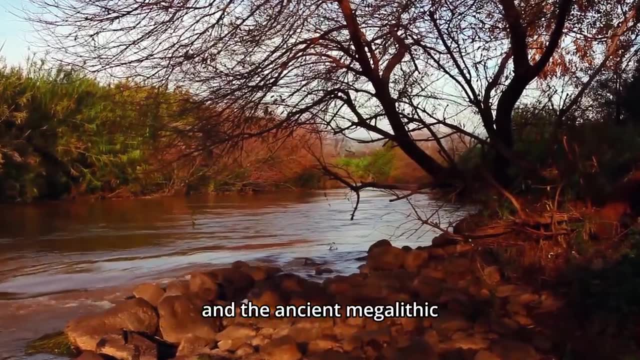 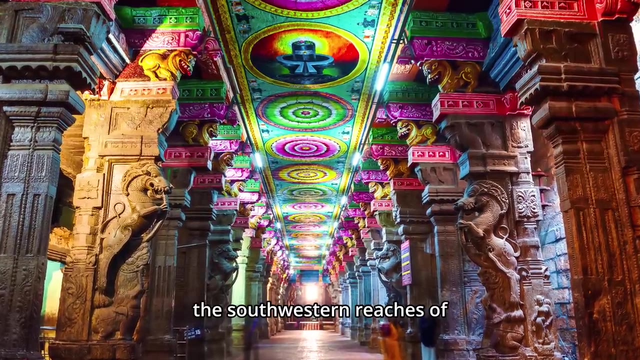 However, what truly captivates the imagination is not just its grand scale. At its heart lies a substantial barrow, forging a profound connection between this culture and the ancient megalithic artisans of France, Britain and Ireland. Nabta Playa, nestled in the southwestern reaches of Egypt's western desert, near the Sudanese border. 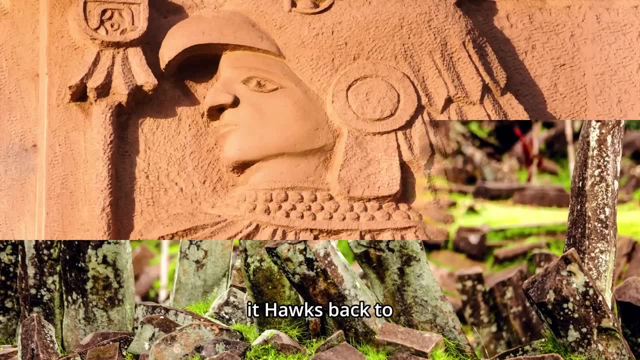 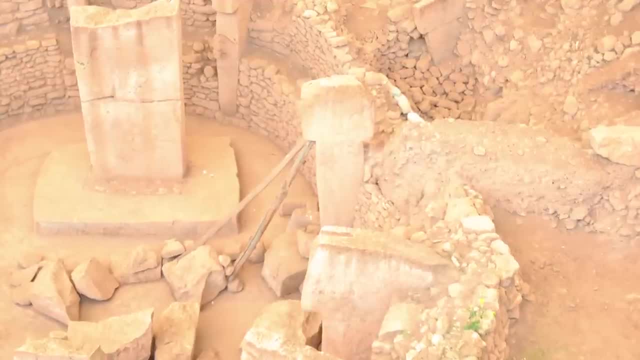 is an ancient archaeological treasure. It harks back to the Neolithic era, flourishing around 10,000 BC. Among its many remarkable features, it boasts a venerable stone circle, standing as one of the world's most ancient of its kind. 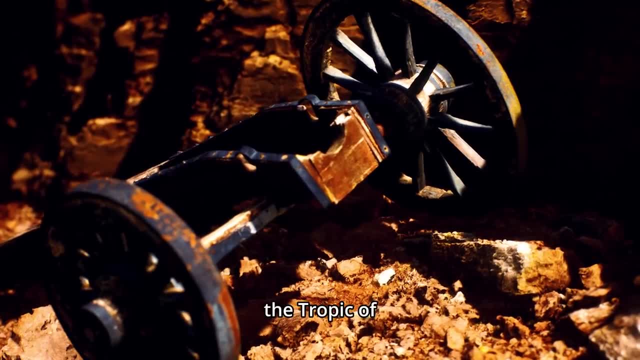 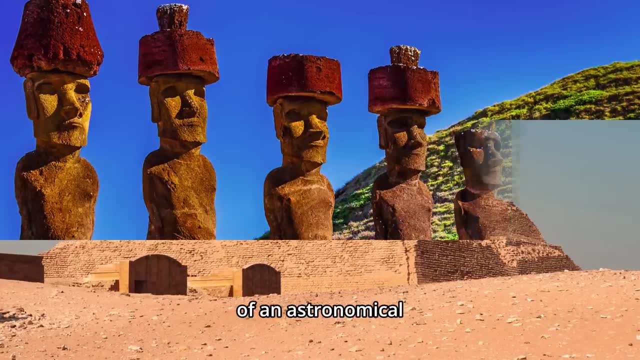 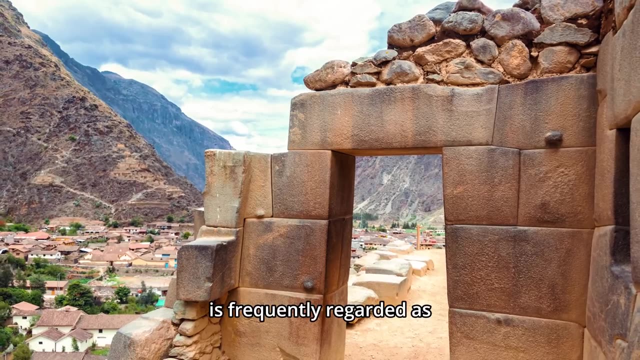 The stone circle's strategic placement directly on the Tropic of Cancer has drawn the fascination of archaeologists globally, marking it as one of the earliest recognized instances of an astronomical observatory in human history. Nabta Playa civilization, an ancient precursor, is frequently regarded as the trailblazer for the renowned and iconic civilization of ancient Egypt. 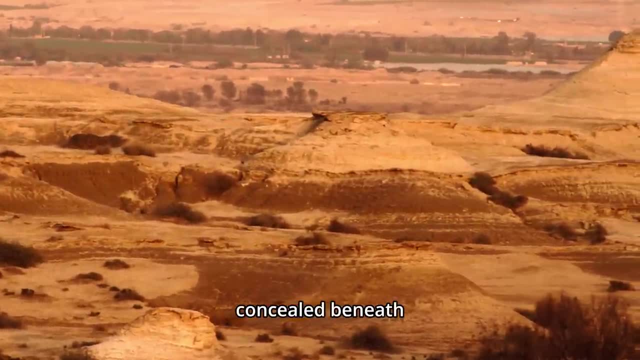 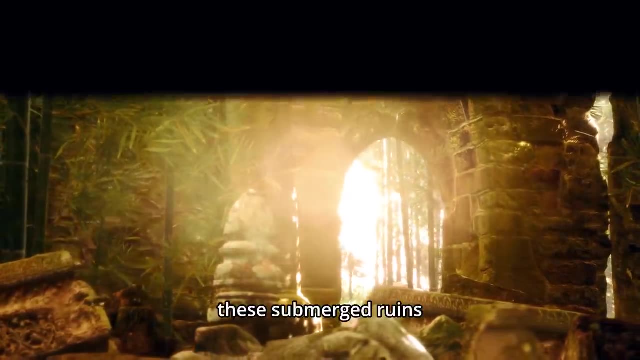 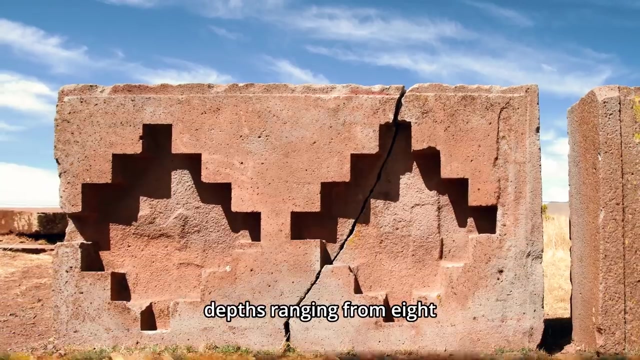 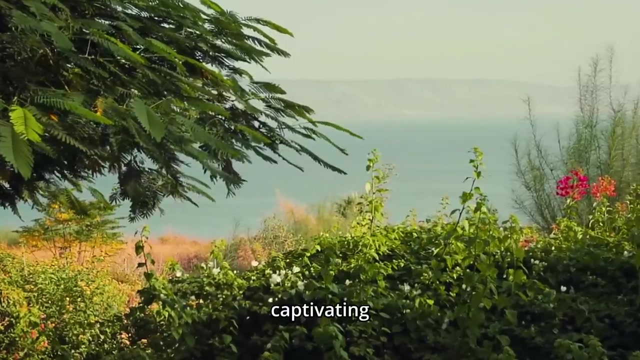 Off the coast of Haifa in Israel, concealed beneath the Mediterranean waves, rests a Stone Age settlement dating back to a remarkable 9,000 years ago. These submerged ruins represent some of the most ancient and expansive sunken remains ever unearthed. They lie at depths ranging from 8 to 12 meters and include a collection of seven substantial monoliths, once arranged to shape a captivating stone circle. In Israel, you'll discover Ru'aym el-Hiri, also known as Gilgal-Rifaym or the Wheel of Giants, positioned just 16 miles east of the captivating Sea of Galilee. Much like Stonehenge, this megalithic wonder exhibits an arrangement of concentric rings that continue to mystify archaeologists and visitors alike. Notably, the site features an opening in its outer circle meticulously aligned with the summer solstice, adding to its enigmatic allure. In the northern reaches of Poland lies Odry, renowned not for a singular stone circle, but for the extraordinary presence of ten fully intact and two partially impaired stone circles. 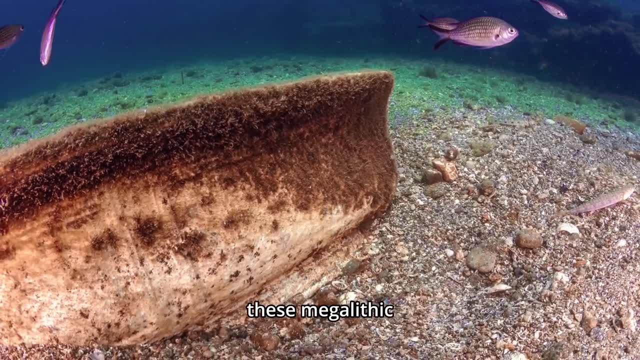 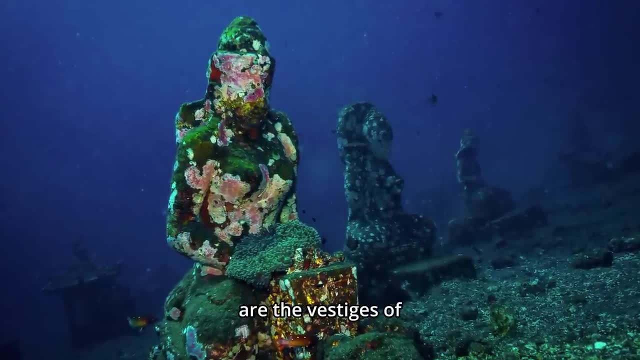 Venturing to South Africa, you'll encounter stone circles, these megalithic enigmas speckling the landscape. But there's more to these than meets the eye. These circles are the vestiges of a colossal metropolis sprawling across an expanse of approximately 1,500 square miles. Amid the picturesque expanse near the Dar River Canyon in Armenia lies Zorats Ka, often referred to as the Armenian Stonehenge. Here, across approximately seven hectares, a profound mystery unfolds. Astonishingly, some researchers assert that this site predates its famous British counterpart Stonehenge by at least 3,500 years, positioning it as one of the world's most ancient astronomical observatories. 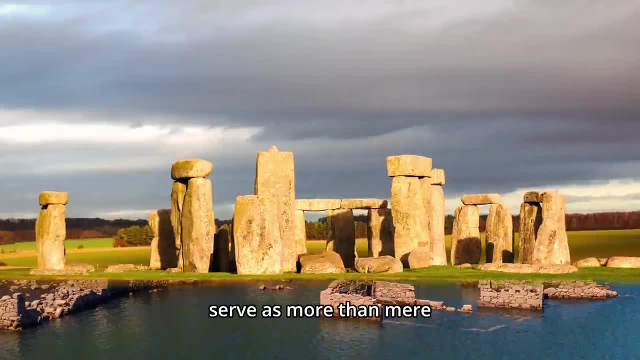 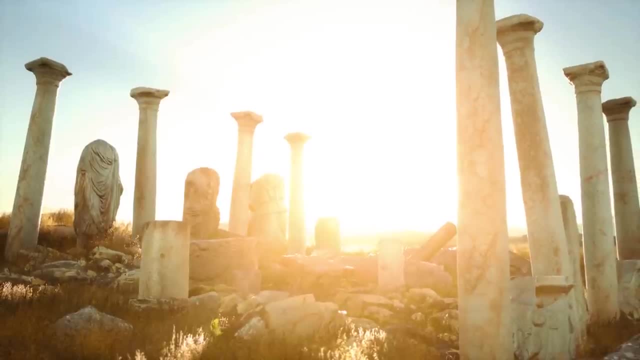 The stones, carefully placed in intricate patterns, serve as more than mere markers of time. they align with celestial events, signaling the grandeur of the summer solstice. What's more, their arrangement mirrors the very stars within the constellation of Cygnus. 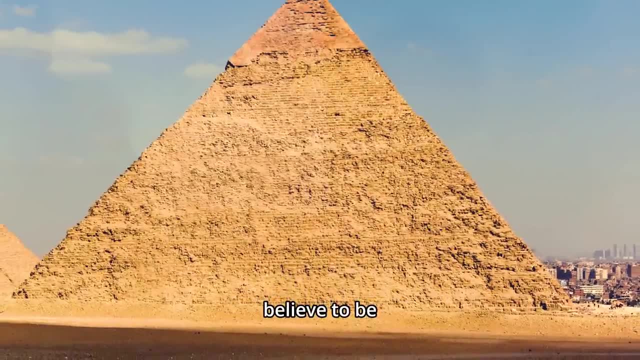 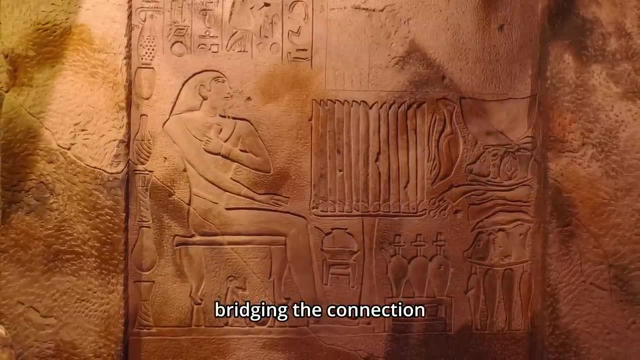 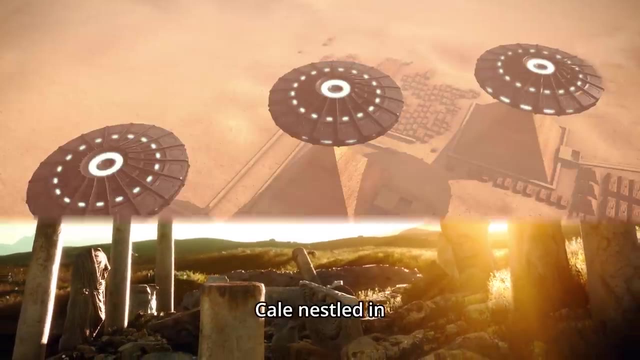 a celestial realm that certain cultures believed to be the gateway to the sky world. Zorats Ka whispers the secrets of ancient skywatchers, bridging the connection between Earth and the cosmos. Deep within the ancient Thracian fortress of Kovachevsko Kale, nestled in the heart of Bulgaria, lies an enigmatic stone circle known as the Sun Circle or Solar Circle. 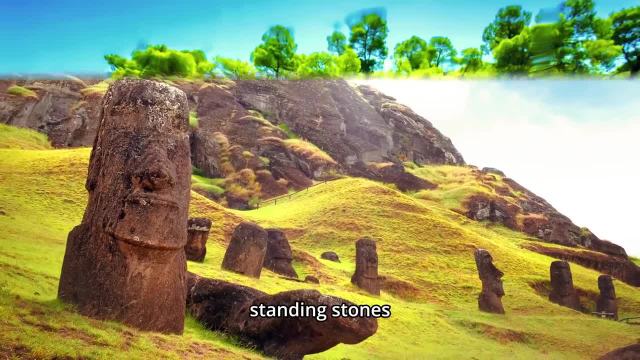 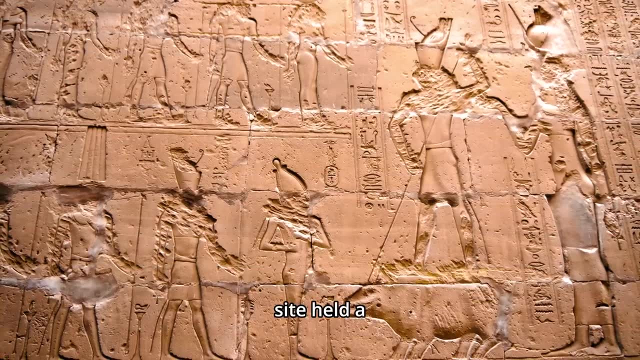 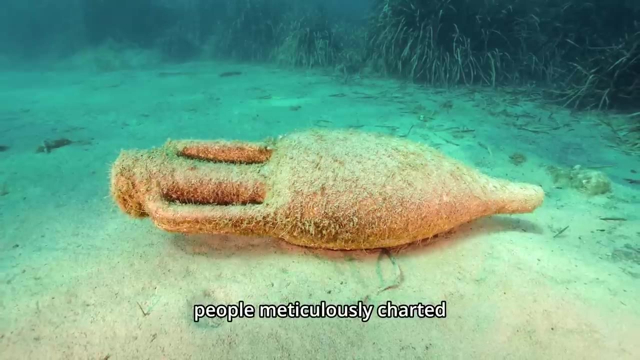 This mysterious ring comprises a series of stately standing stones, meticulously arranged in a circular pattern. Archaeologists and historians believe that this sacred site held a profound purpose. It may have served as an astronomical observatory where the Thracian people meticulously charted the movements of celestial bodies. 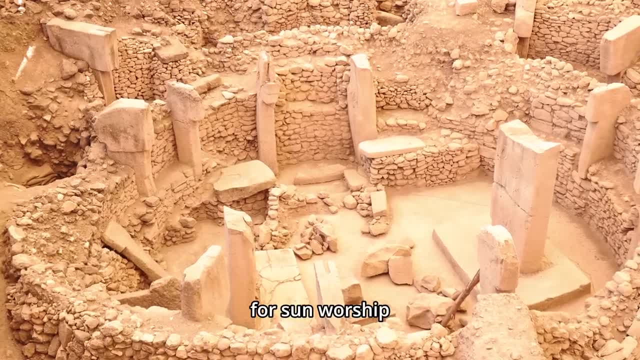 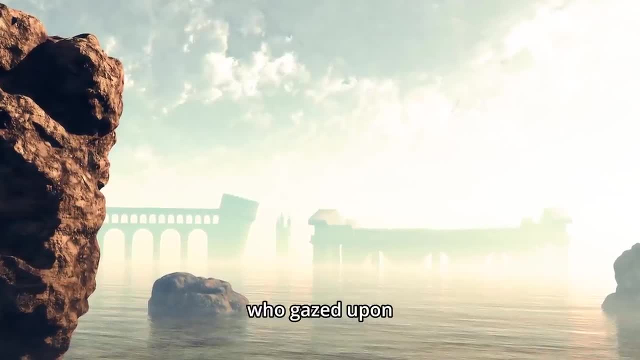 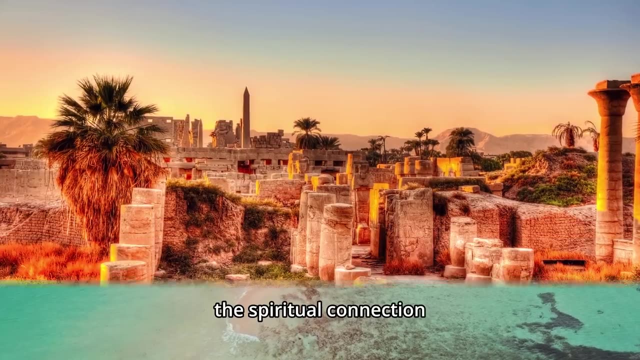 Alternatively, it could have been a hallowed place for sun worship rituals, where the radiant sun, a symbol of life and vitality, was revered and celebrated by those who gazed upon the heavens from this ancient vantage point. Kovachevsko Kale and its Sun Circle bear witness to the spiritual connection between ancient civilizations and the celestial mysteries that have captivated humanity for millennia. 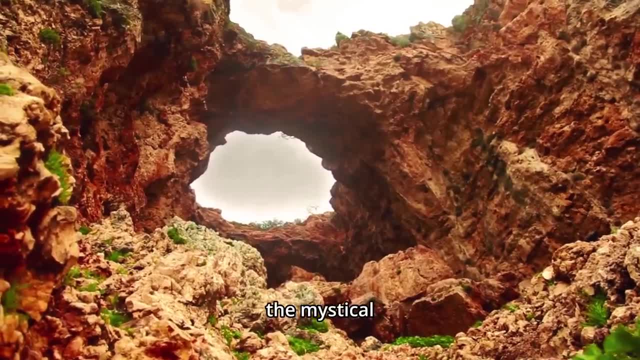 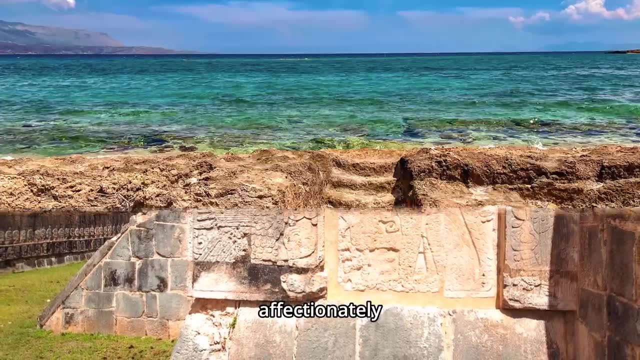 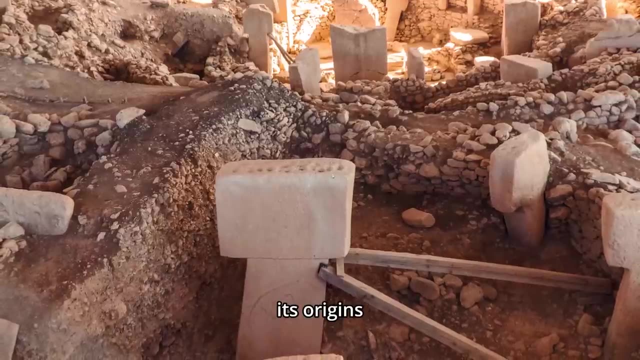 Nestled in the sun-drenched landscape of Portugal, the mystical Almondras Cromlech awaits an ancient megalithic wonder shrouded in time. This site, affectionately referred to as the Hill of the Stone Amphorae, stands as one of Europe's most venerable stone circles, its origins stretching back over 6,000 years. 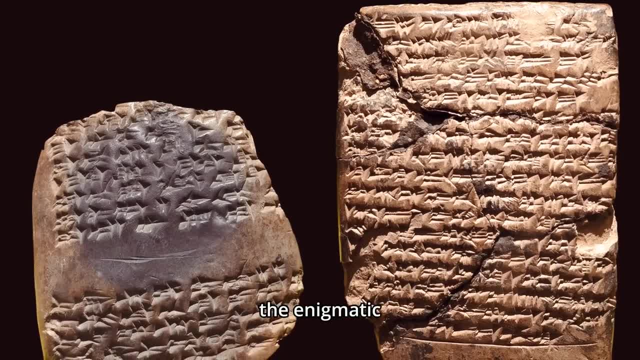 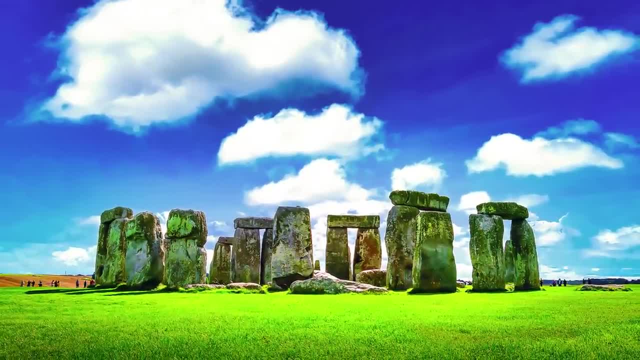 In an extraordinary feat of human endeavor, the enigmatic inhabitants of this arid plateau harnessed their collective strength to transport nearly a hundred colossal granite monoliths. These monoliths, with their rough-hewn beauty, were lovingly arranged on the undulating terrain. 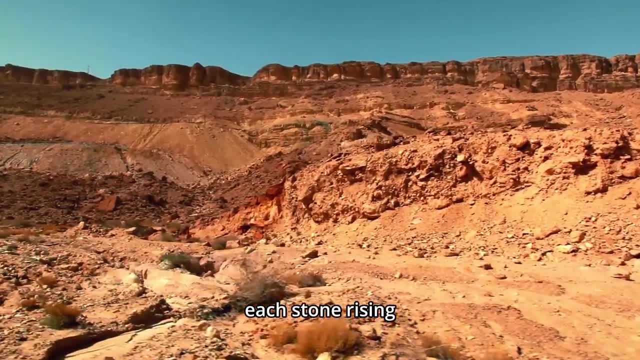 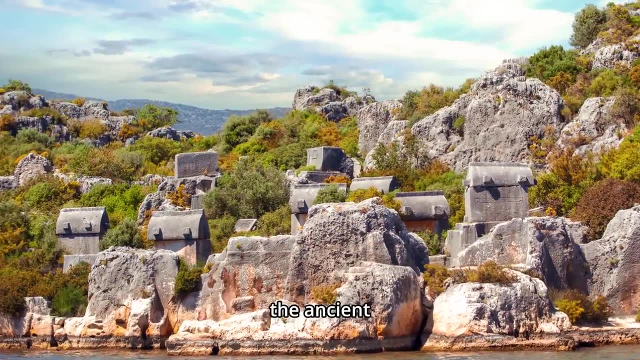 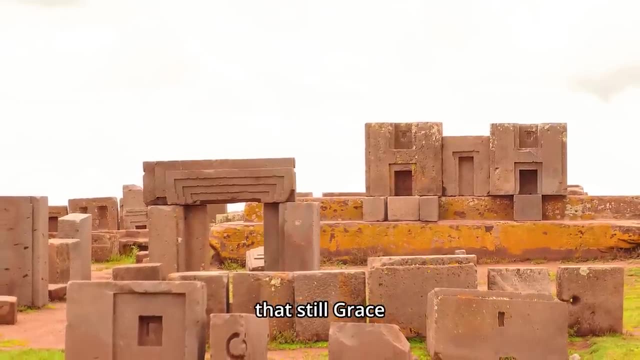 There they formed concentric circles, each stone rising to varying degrees, Their purpose steeped in enigma. Almondras Cromlech stands as a testament to the ancient people's profound connection with the earth and the cosmos, a place where the mysteries of the past are etched into the very stones that still grace the landscape today. 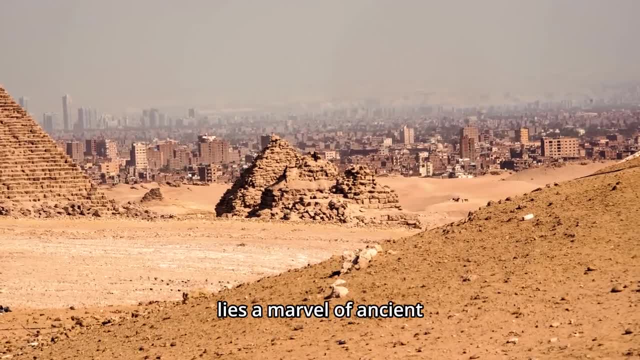 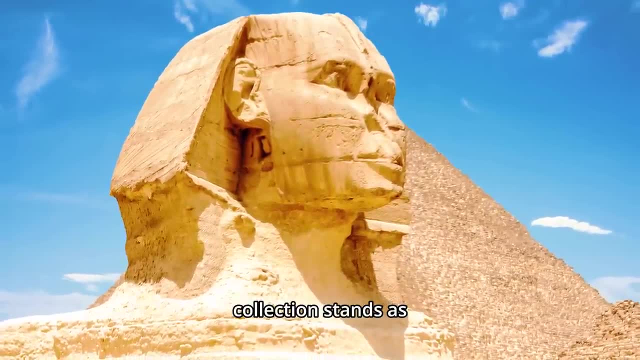 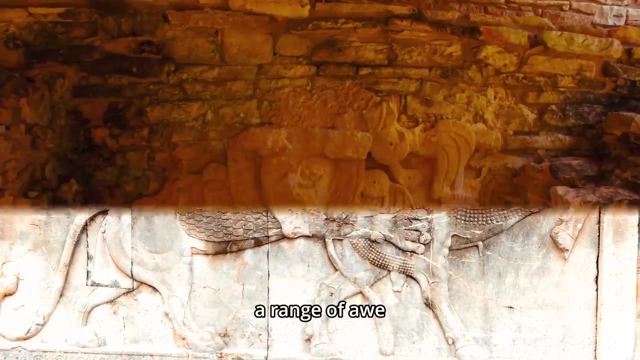 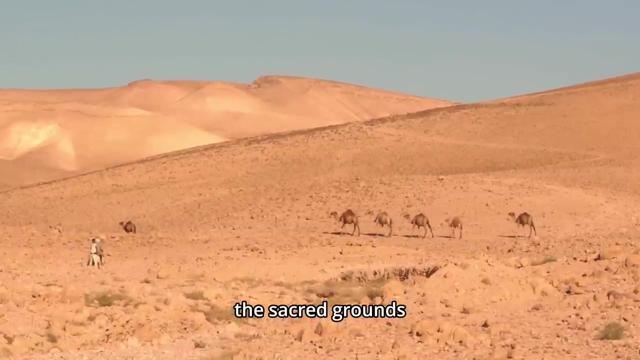 Nestled in the heart of West Africa lies a marvel of ancient craftsmanship and spiritual significance: the Senegambian Stone Circles. This extraordinary collection stands as the largest assembly of megalithic complexes ever unveiled on our planet. It encompasses a range of awe-inspiring sites, including the enigmatic Siningayane complex in Senegal, as well as the sacred grounds of Wana, Wasu and Kerbach in the vibrant landscapes of the Gambia. 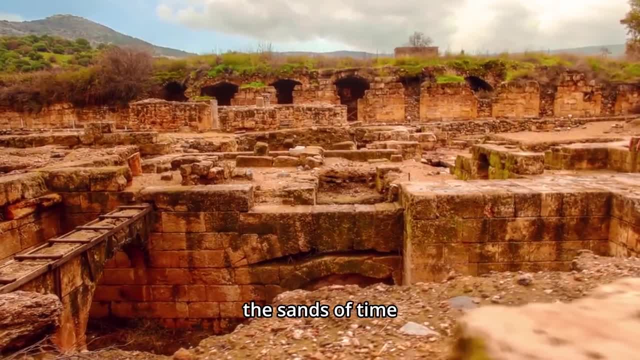 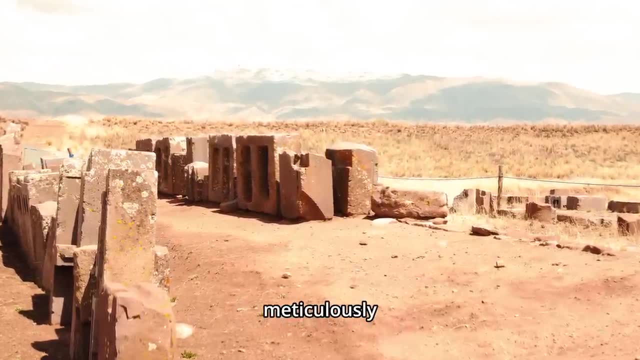 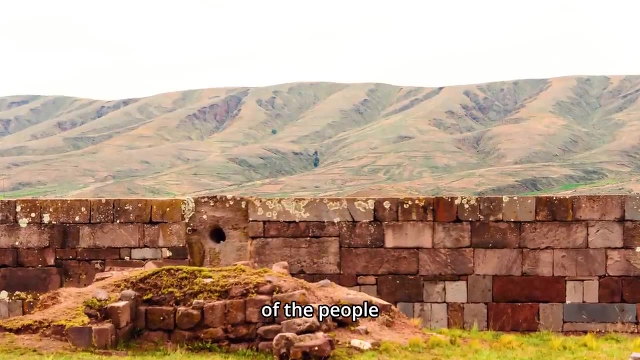 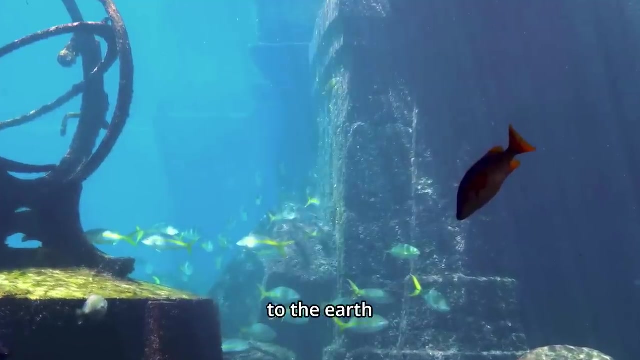 These remarkable stone circles, weathered by the sands of time, bear witness to a legacy that extends from the 3rd century BC to the 16th century AD. Meticulously arranged and imbued with profound meaning, each stone, each circle tells a story of ancient wisdom and a deep connection to the earth and the cosmos. 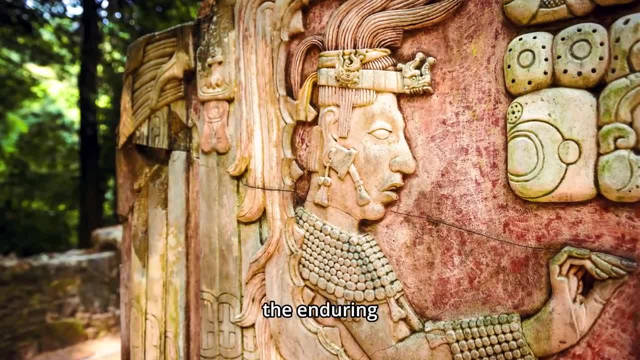 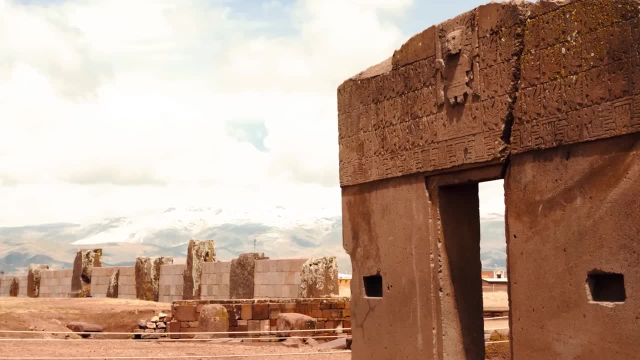 The Senegambian Stone Circles continue to stand as a testament to the enduring mysteries of the past, an open invitation for explorers and scholars to decipher their enigmatic significance In the vast expanse of the western Brazilian Amazon, spanning approximately 13,000 square kilometers. 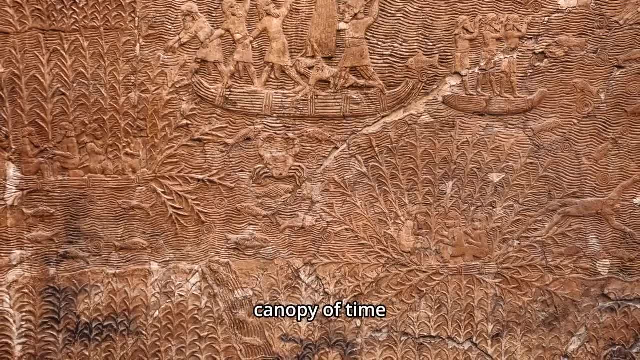 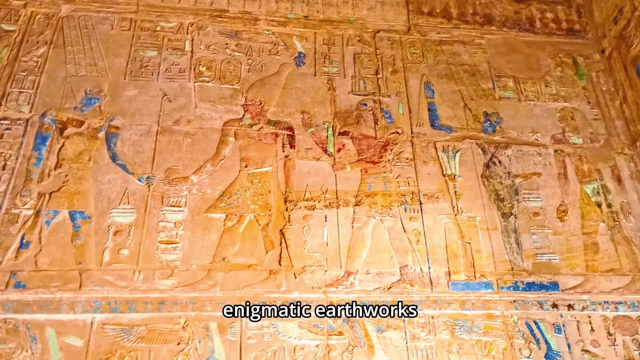 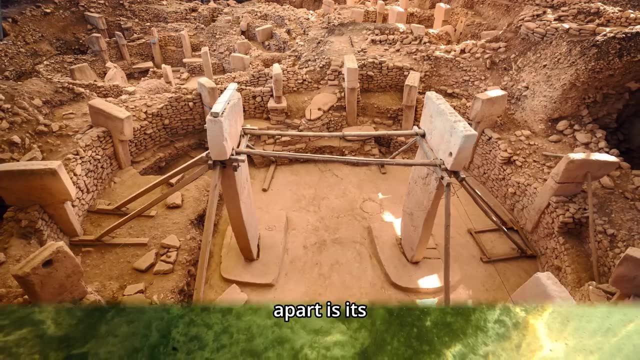 lies a stunning enigma concealed beneath the thick canopy of time. Here, like a whisper from the depths of antiquity, hundreds of colossal and enigmatic earthworks have emerged, reminiscent of the iconic circles at Stonehenge. Yet what sets this discovery apart is its profound mystique. 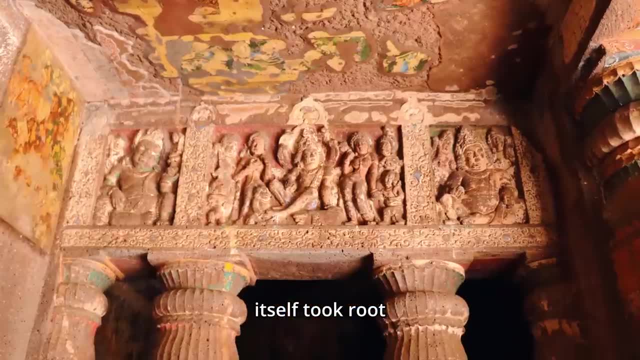 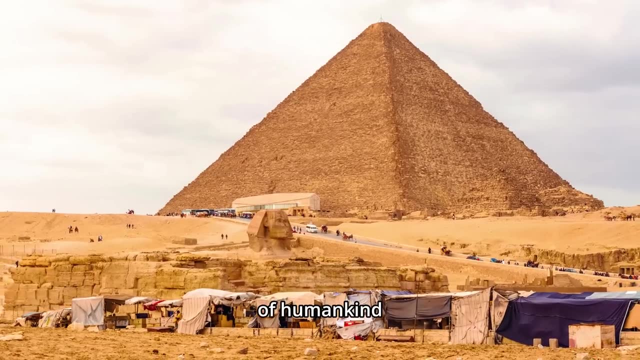 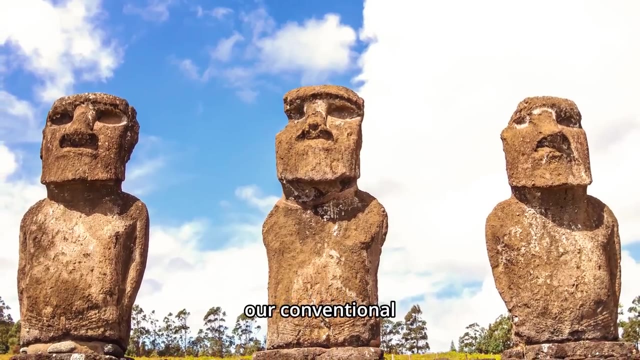 These enigmatic structures were crafted long before the rainforest itself took root in this region. For ages, it was believed that these lands had never felt the presence of humankind. The very idea that these enigmatic circles were constructed prior to the flourishing rainforest defies our conventional understanding of history. 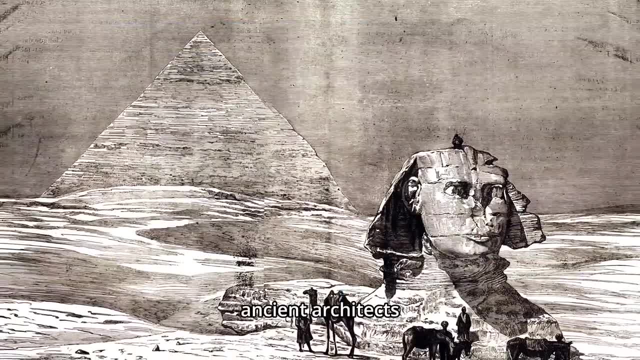 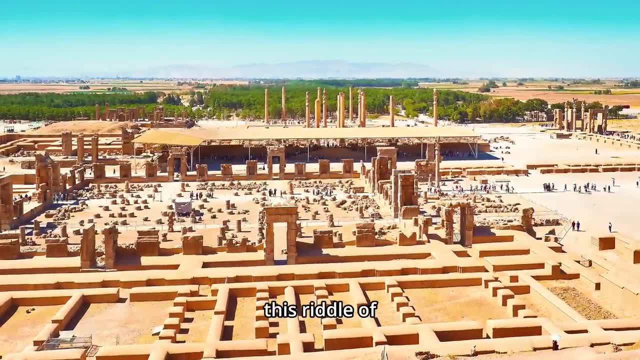 Questions abound like tendrils in the jungle. Who were these ancient architects and what compelled them to create these stone enigmas in a land where humanity was deemed absent? This riddle of the Brazilian Amazon beckons us to delve deeper into the annals of time. 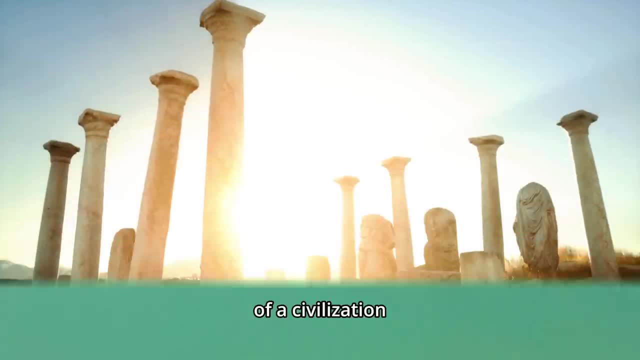 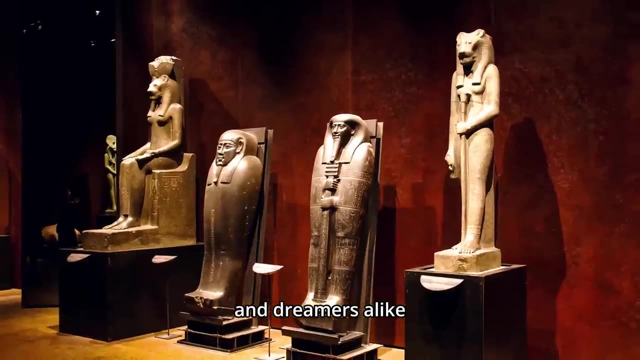 to unravel the untold tales of a civilization lost to the mists of history. It is a silent invitation to explorers, historians and dreamers alike who dare to seek the secrets hidden in the heart of the rainforest and to unlock the enigma of these ancient earthworks. 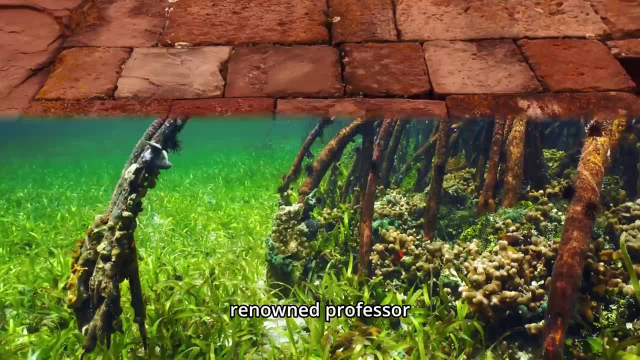 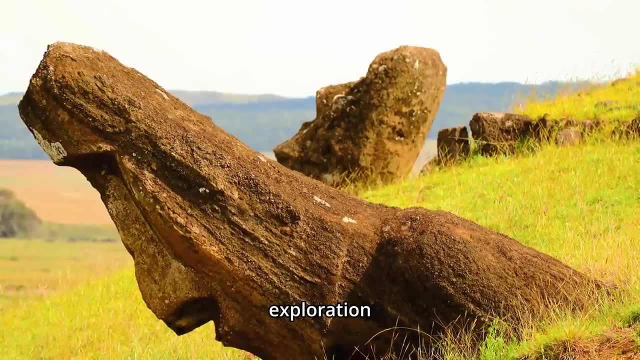 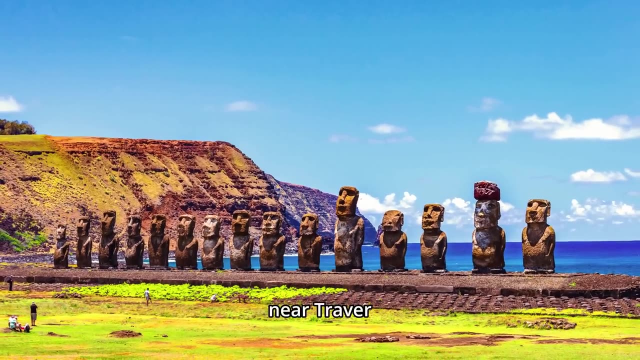 In the year 2007,, Mark Holley, a renowned professor of underwater archaeology hailing from Northwestern Michigan University College, embarked on an expedition of exploration, Initially tasked with unraveling the mysteries of ancient boat wrecks and surveying the depths of Lake Michigan near Traverse City. 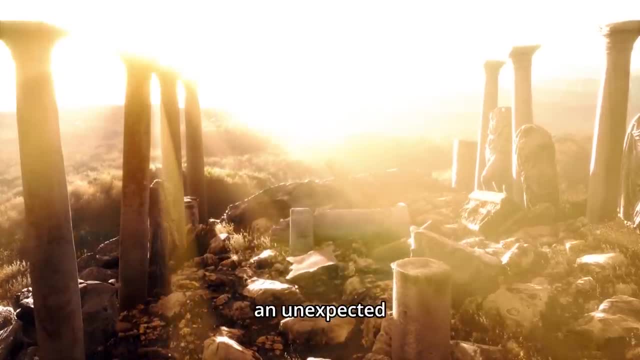 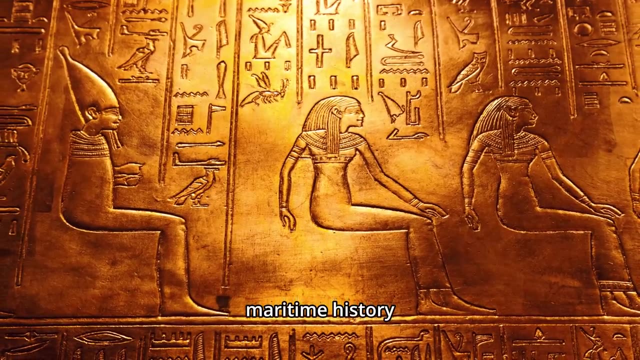 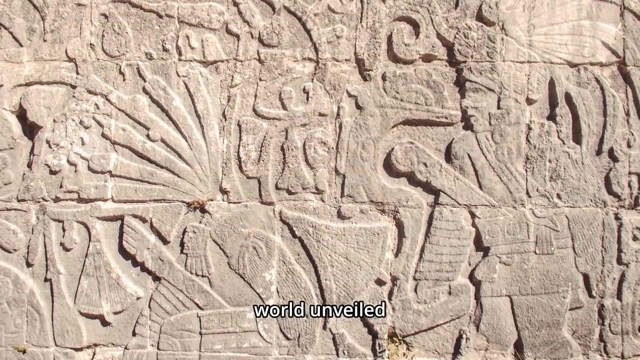 he and his colleague Brian Abbott found themselves on the brink of an unexpected revelation. What lay beneath the tranquil waters of the lake held far more than the echoes of maritime history. Astonishingly, at a depth of 40 feet beneath the tranquil surface of Lake Michigan, the submerged world unveiled its secrets. 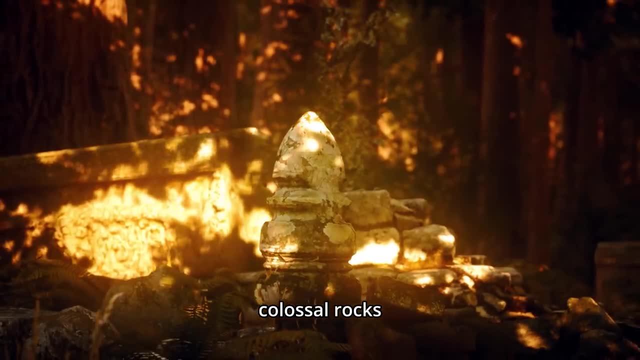 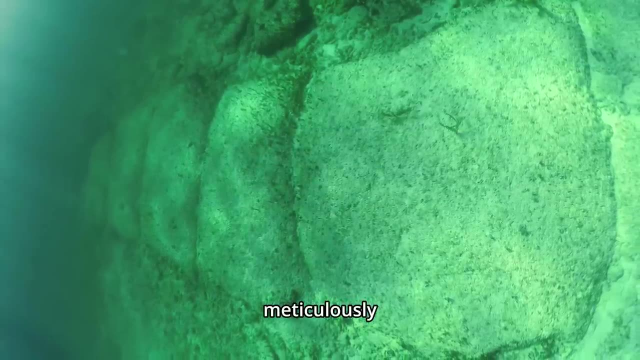 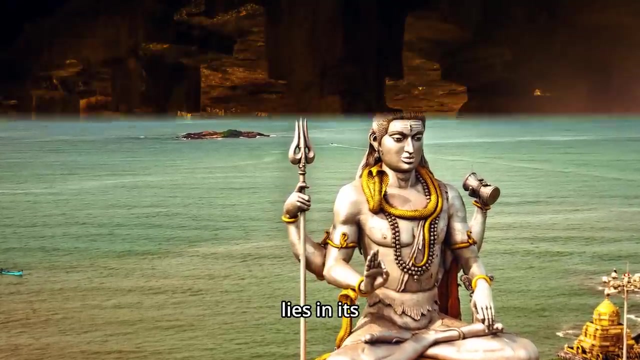 A megalithic structure composed of colossal rocks, each weighing as much as 50 tons, emerged from the aquatic depths. These massive stones were meticulously stacked atop one another to form a grand and enigmatic circle. The true marvel of this underwater find lies in its antiquity, as it predates the very existence of the lake itself. 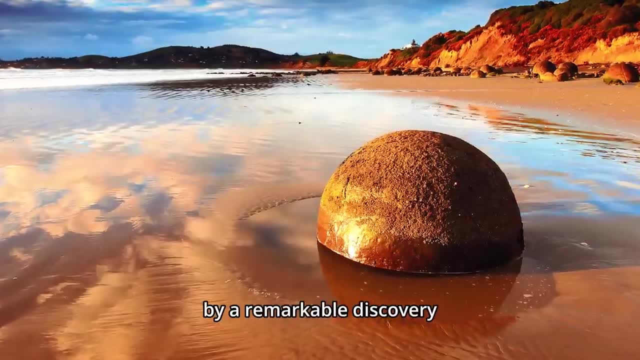 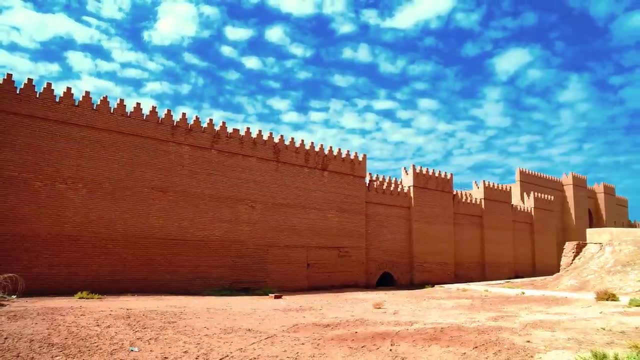 This intriguing anomaly is corroborated by a remarkable discovery: a single stone within the outer circle adorned with a prehistoric carving of a mastodon, A creature that has long been extinct. this animal ceased to roam the earth over 10,000 years ago. 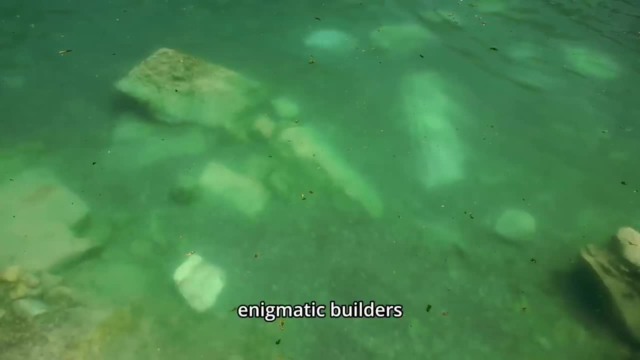 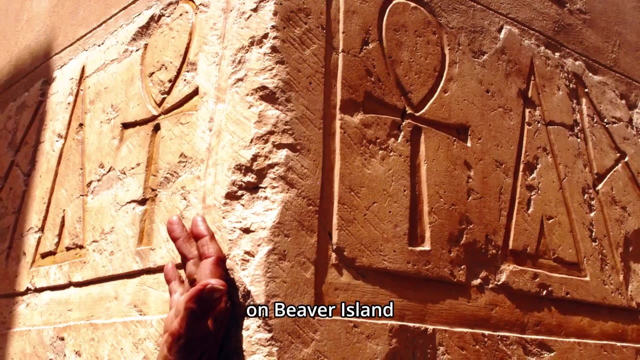 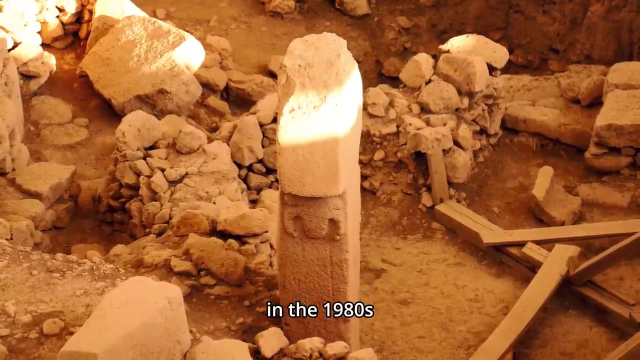 The enigma deepens as we ponder the question: who were the enigmatic builders of stone circles in America, at least a staggering 10,000 years ago? Nestled on Beaver Island in Michigan, a peculiar enigma unfurled before the eyes of bewildered researchers when stone circles came to light in the 1980s. 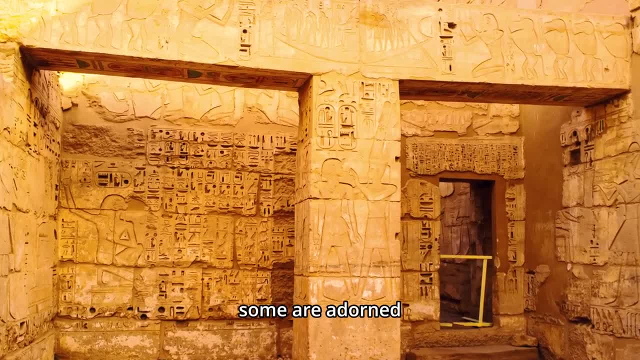 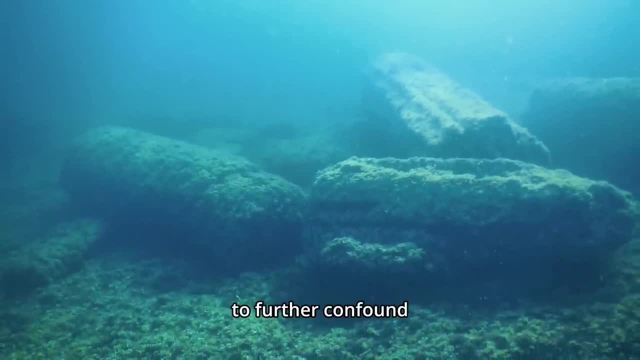 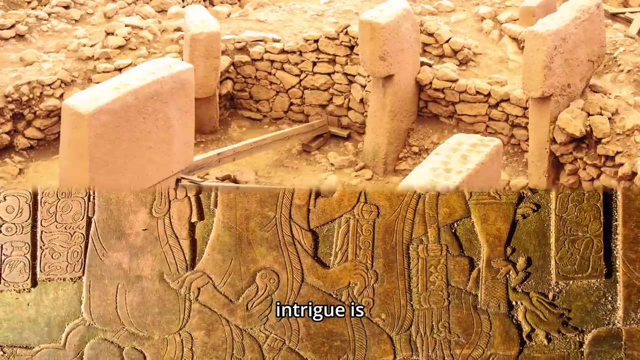 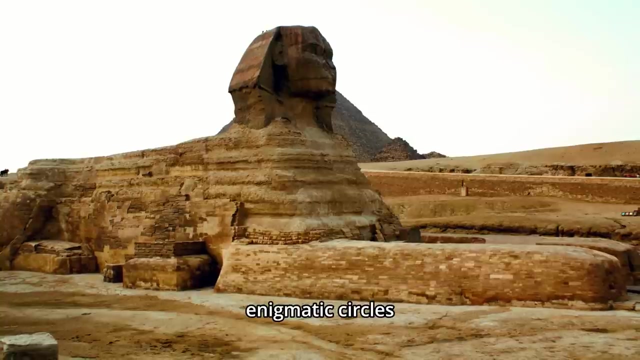 Among these ancient stones, mysteries abound. some are adorned with intricate incised lines, while others feature enigmatic circular holes at their center. To further confound the enigma, a web of astronomical alignments entwines the site in cosmic secrets. Adding to the intrigue is the testimony of the island's indigenous inhabitants, who firmly state that they were not the architects of these enigmatic circles. 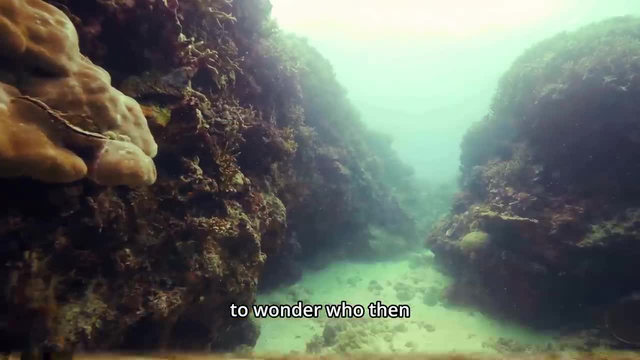 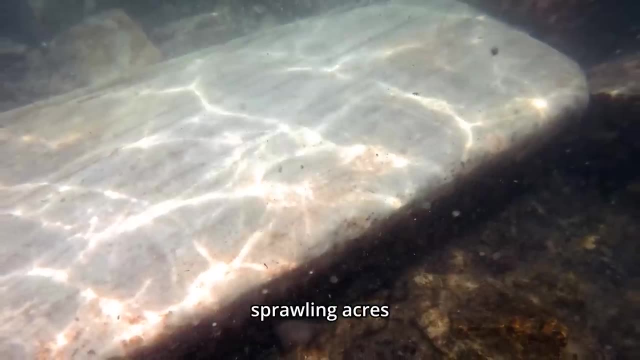 The question lingers in the air, beckoning us to wonder: Could have been the cryptic builders of these stone circles? on Beaver Island, In the expanse of 30 sprawling acres within Salem, New Hampshire, lies a place enshrouded in intrigue and known as Mystery Hill. 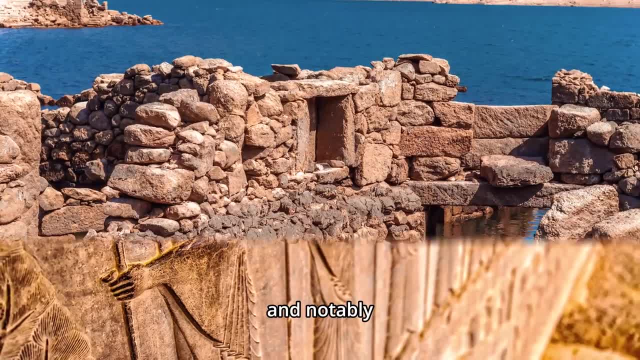 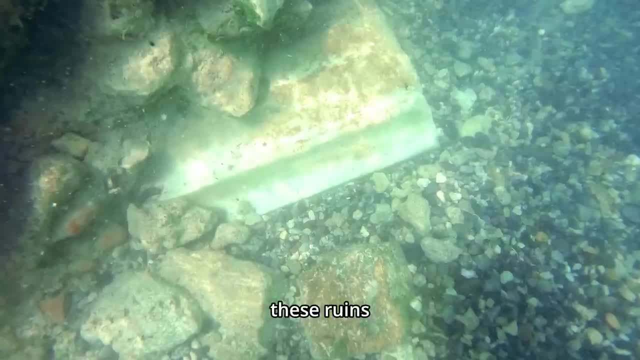 This enigmatic site harbors ancient ruins and, notably, a cryptic stone circle, its origins shrouded in the mists of time. The mystery is deepened by the fact that these ruins defy categorization within any known culture Dating back to at least 2000 BC. the riddles of Mystery Hill continue to perplex and beckon the curious to unravel its secrets. Nestled in the heart of Alberta, Canada, the Majorville Medicine Wheel stands as a testament to ancient wisdom and reverence. More than 4,500 years ago, indigenous peoples crafted this remarkable stone circle, a sacred sanctuary that transcends time. 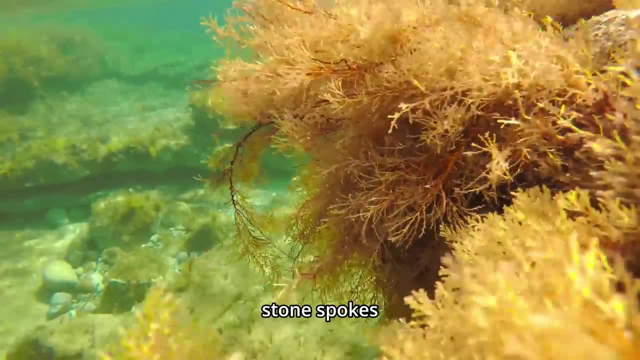 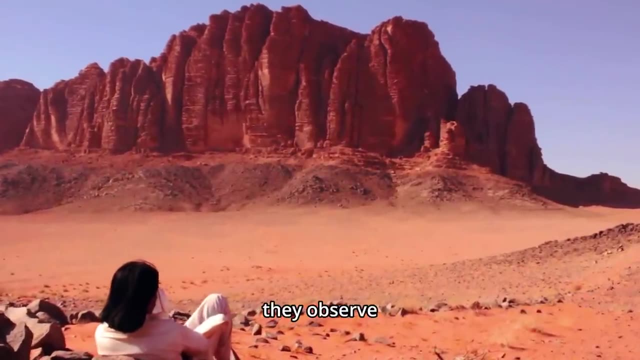 Its central cairn, forms a mystical core encircled by stone spokes reaching outward like the whispers of the cosmos. Here, beneath the expansive sky, they observed the heavens and conducted spiritual ceremonies, weaving together the earthly and the divine in a sacred dance. 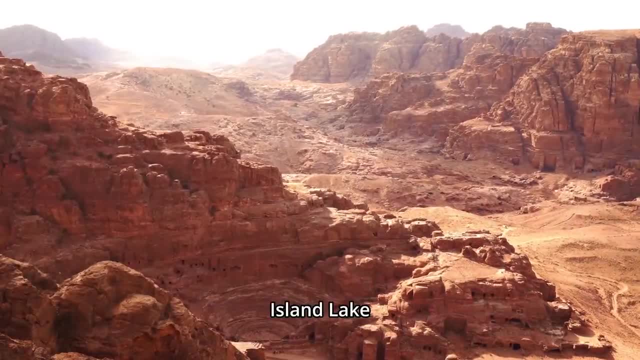 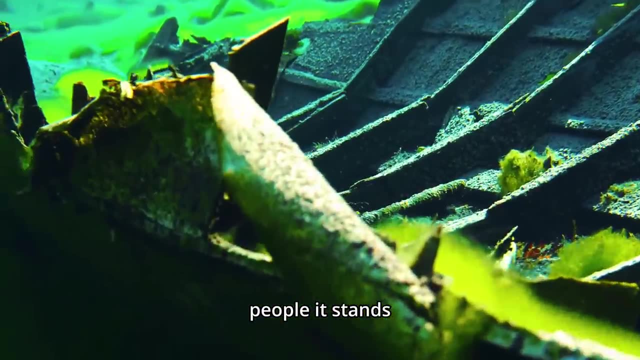 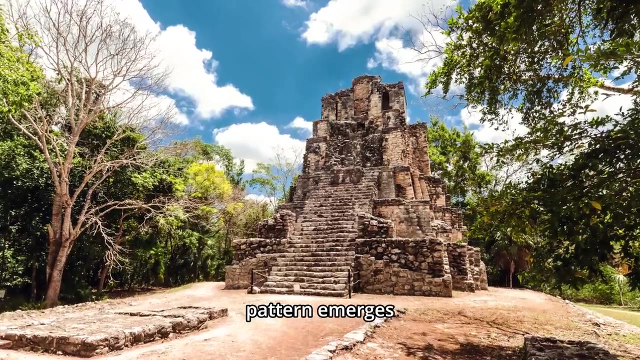 The enigmatic Sun Temple graces, Manitoulin Island, Lake Huron, Ontario. Carved into existence by the skilled hands of the Anishinaabe people, it stands as a hallowed ground for their ancient ceremonies. Within its stone embrace, a circular pattern emerges, entwined with the essence of cultural and spiritual traditions. 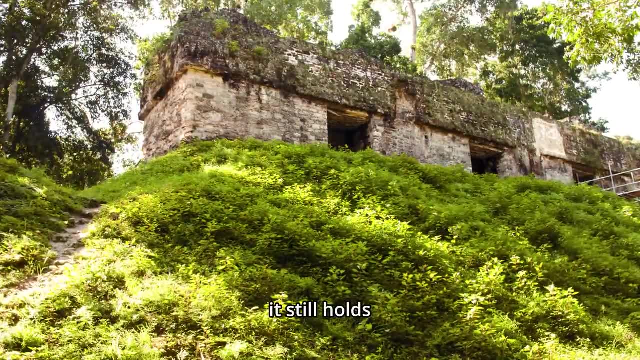 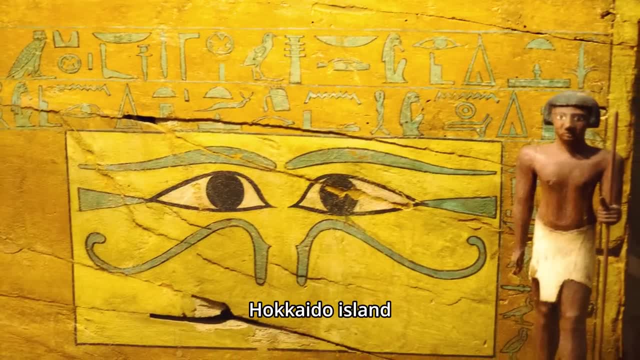 While Asia may have fewer stone circles, it still holds treasures of its own, scattered across diverse regions Set in the northern embrace of Japan's Hokkaido Island. the Reban Island. petroglyphs whisper tales from the depths of history. 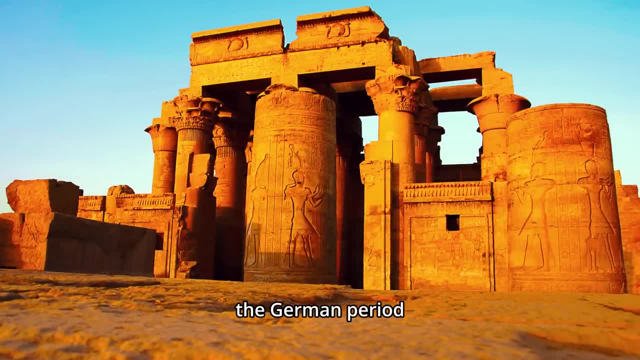 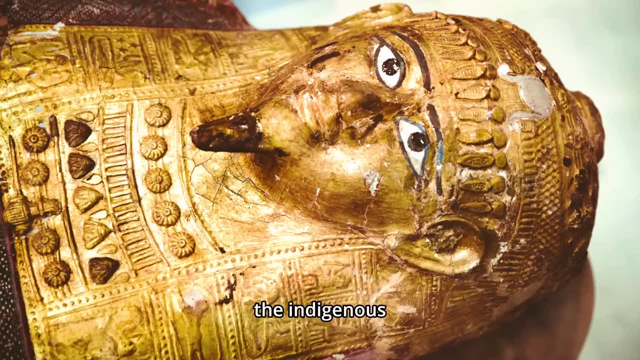 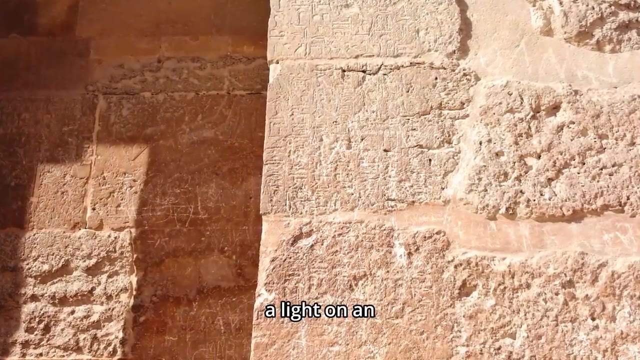 These ancient stone circles adorned with the marks of the Jomon period are a testament to the profound rituals and ceremonies cherished by the indigenous Ainu people. In the annals of history, the Hongshan culture of northeastern China shines a light on an era between approximately 4700 and 2900 BCE. 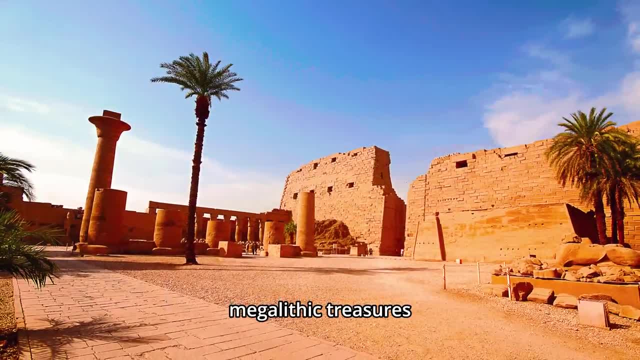 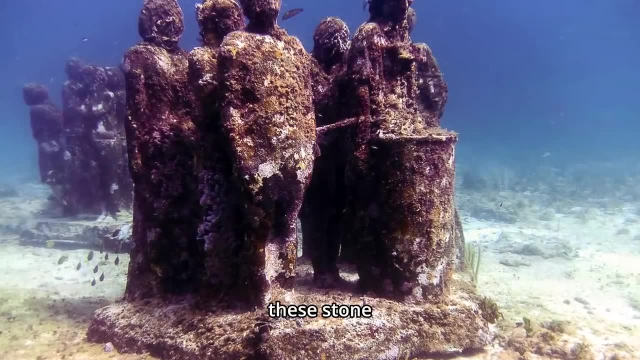 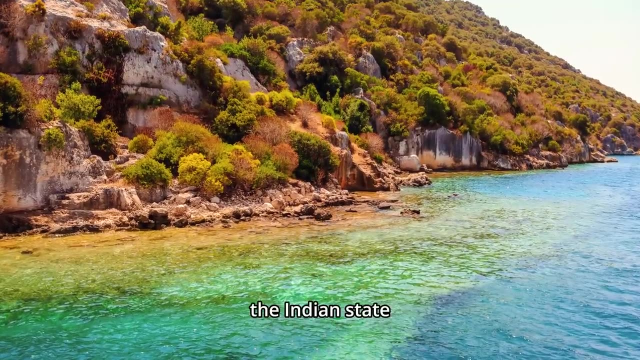 This intriguing culture left behind megalithic treasures, including enigmatic stone circles Scattered across landscapes like Liaoning and Inner Mongolia. these stone circles bear witness to the burial traditions of a bygone age Nestled in the verdant landscapes of the Indian state of Manipur. 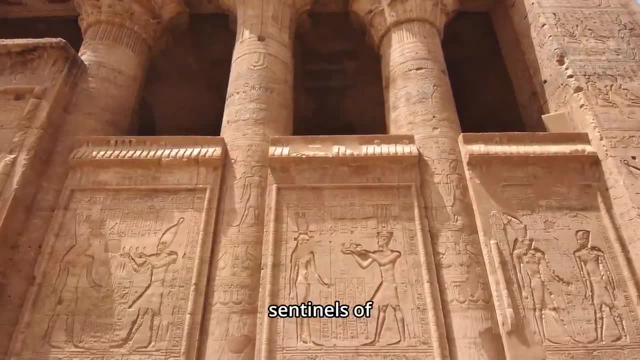 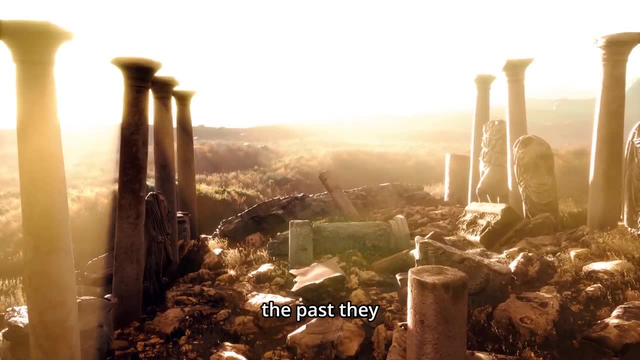 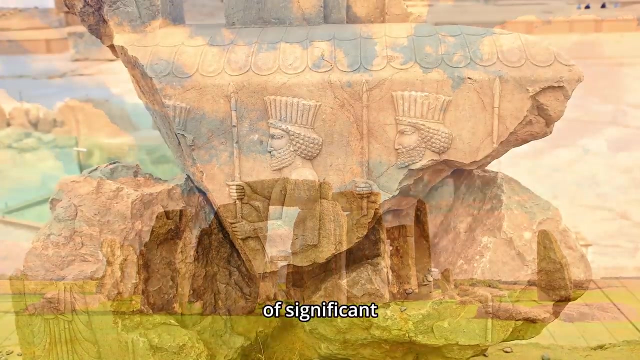 the megalithic circles stand as ancient sentinels of the Neolithic era. These enigmatic stone circles, crafted with care, provide glimpses into the past. They are believed to have fulfilled the role of funerary monuments marking the final resting places of significant individuals. 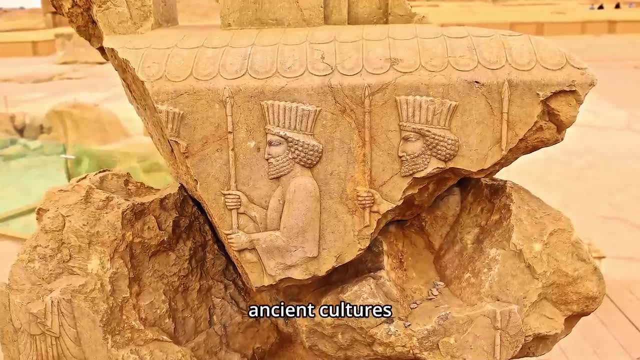 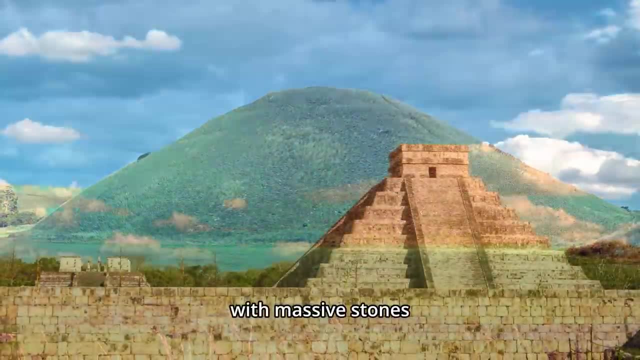 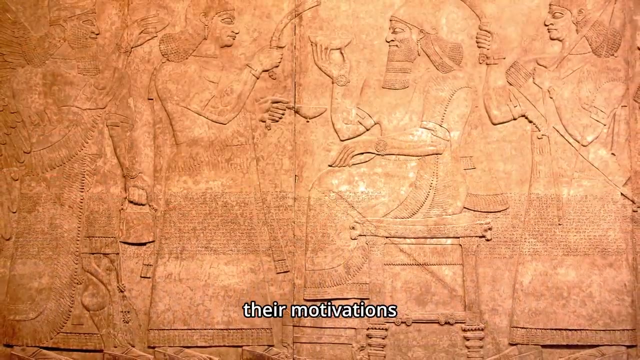 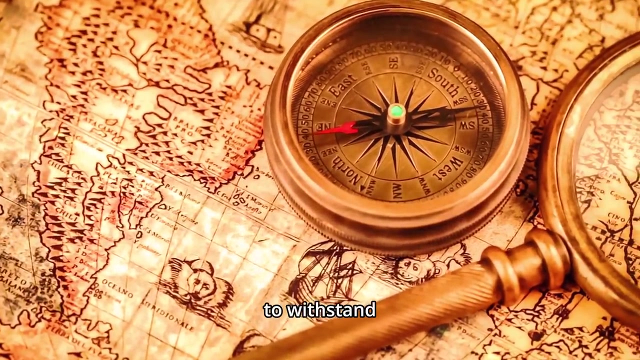 It's truly remarkable how numerous ancient cultures, spread across distant lands and divided by vast oceans, shared a common fascination with massive stones, fashioning them into extraordinary monuments that defy easy explanation. One can't help but wonder about their motivations. Could it be that they were aware of stone's durability and resilience, making it a choice material to withstand the test of time? 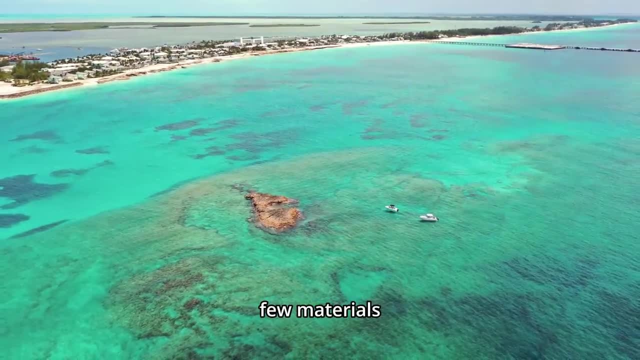 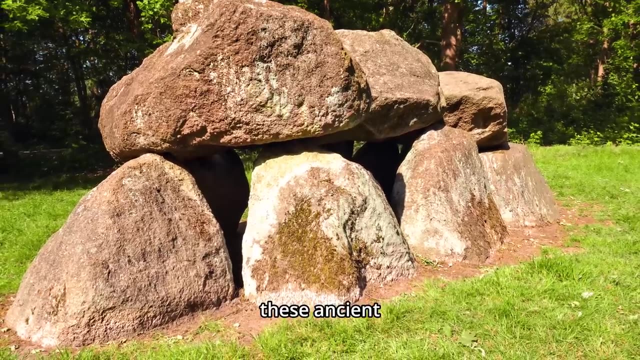 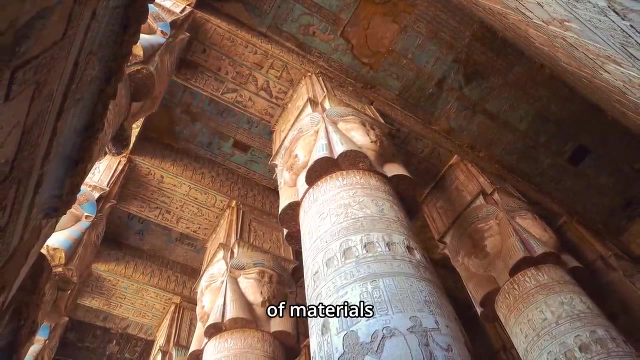 As we've mentioned before, stone is among the few materials capable of enduring even catastrophic events. Perhaps, deep within their collective memory, these ancient builders retained echoes of a history-altering occurrence, such as the Younger Dryas impact influencing their choice of materials and inspiring awe-inspiring creations. 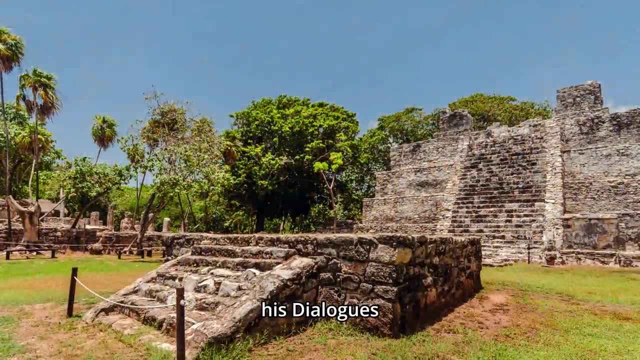 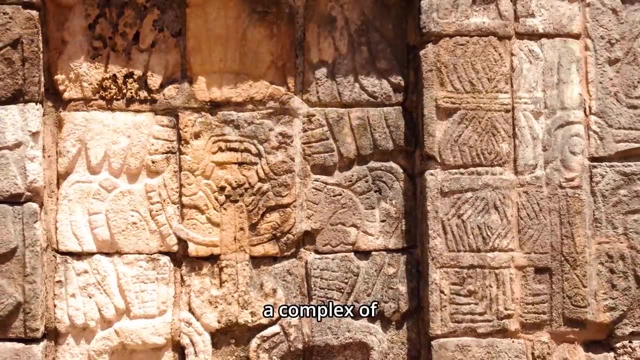 Plato's description of Atlantis as outlined in his dialogues Timaeus and Criscus is indeed intriguing. He portrayed Atlantis as a complex of concentric circles of land and water, with zones of alternating land and water extending outward from its center. 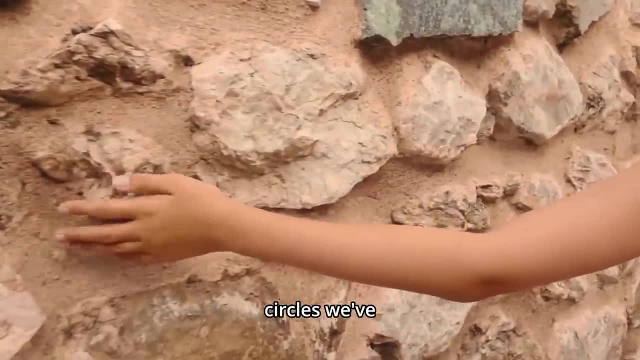 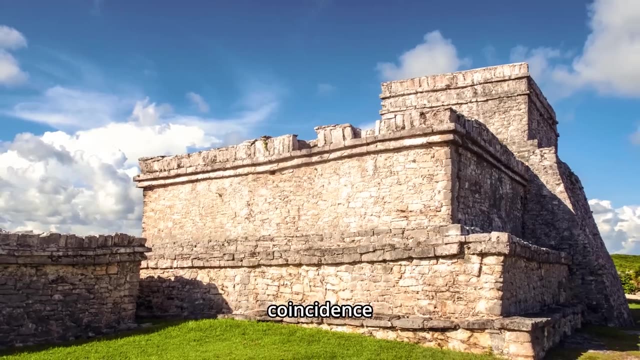 What's even more fascinating is the resemblance between some of the stone circles we've explored and the concentric circle patterns that Plato associated with Atlantis. Could this be mere coincidence or is there a deeper connection waiting to be unraveled? Could these stone circles scattered across the globe? 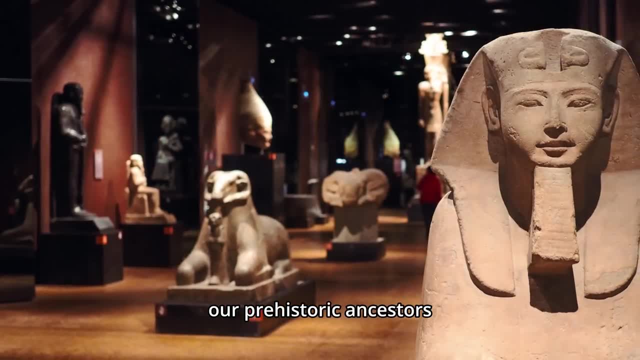 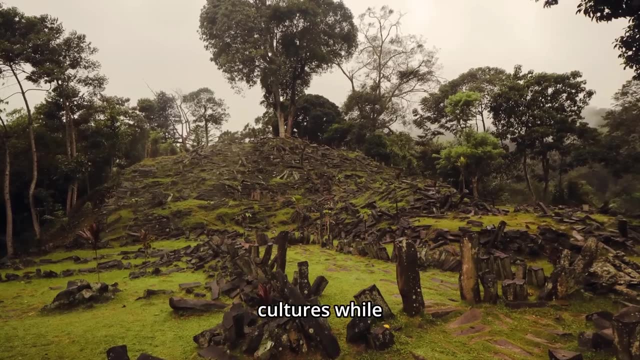 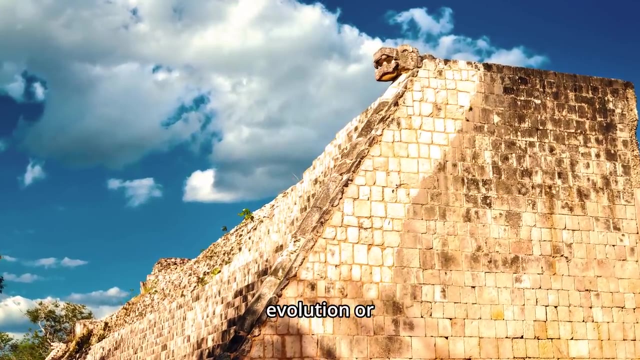 offer a glimpse into the minds of our prehistoric ancestors. Is it merely a remarkable coincidence that these structures share common features across different cultures, While mainstream historians propose that the similarities in construction and design can be attributed to convergent evolution or parallel cultural developments, 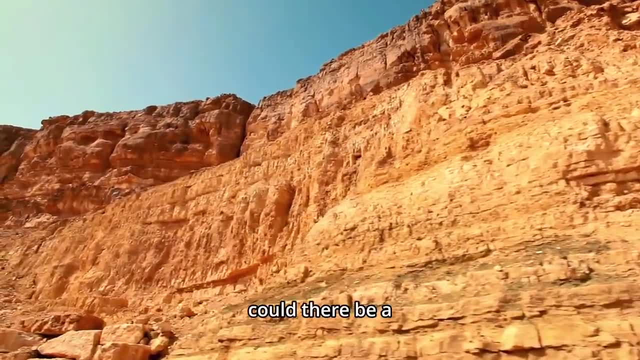 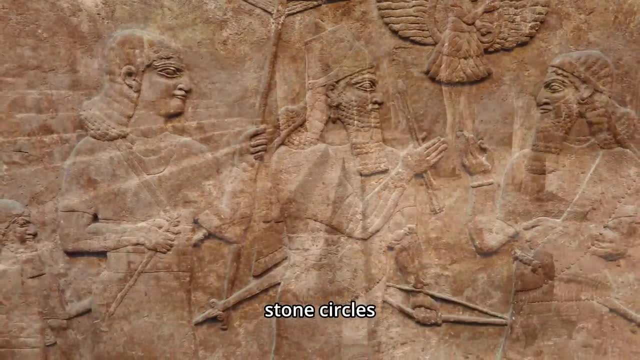 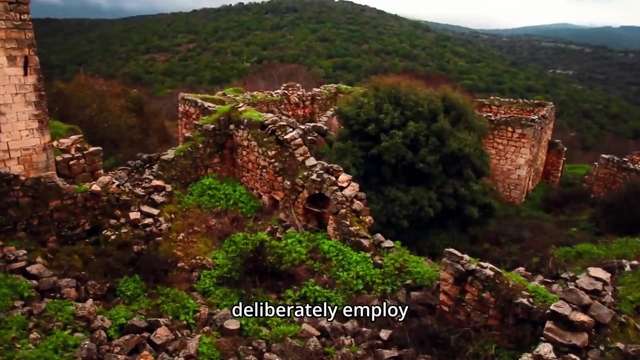 this explanation might be somewhat simplistic. Could there be a more complex, interconnected history that we've yet to uncover? The presence of geometry in these stone circles adds weight to the theory of a global civilization. It's intriguing to note that these ancient builders deliberately employed geometry in their constructions, hinting at the profound significance of these shapes in their beliefs and practices.